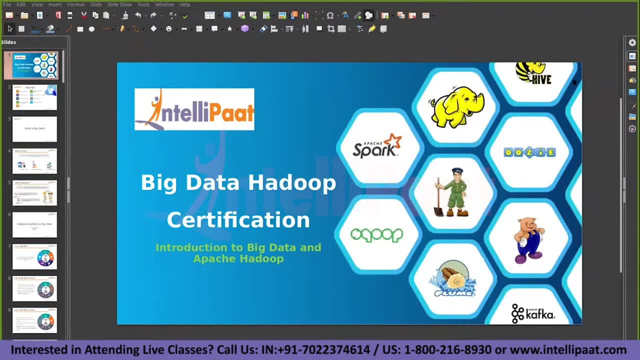 so most of you have answered like saying that, okay, this, this is. this is something to deal with the large amounts of datasets. so what is the problem that we're gonna have with large amounts of datasets? Now, what are the problems that we're gonna face with having large amounts of datasets? 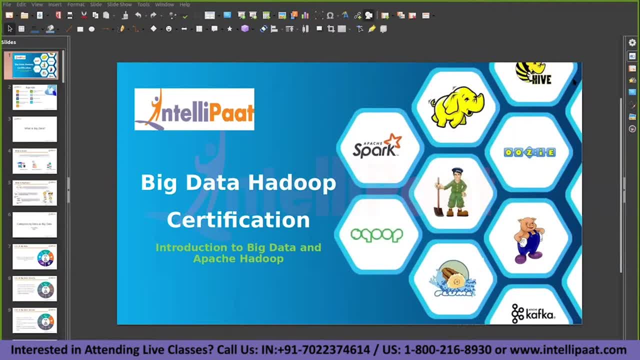 this is my question. so some of them said that it's, it's. it's cannot be stored in the regular machines. okay, so so we'll go back to the previous question. what, what is this Big Data? so definitely the term itself suggests that it's. it's something to deal with the large amounts of data. so 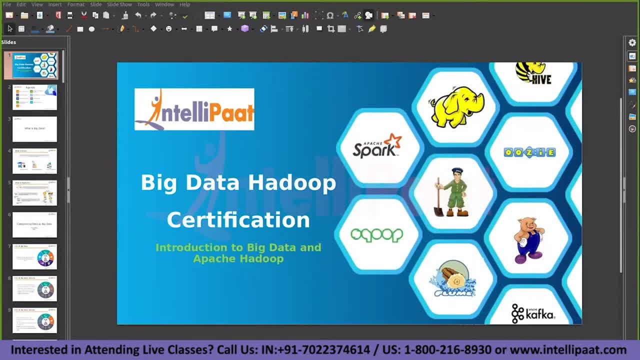 so, in addition to the size of the data, We also Can Consider the type of the data. we also consider the speed with which it is getting generated and we also consider that the need for such datasets. right, so we are. we are saying that it is large amounts of datasets. where is it coming from? first thing, right? so why is this? 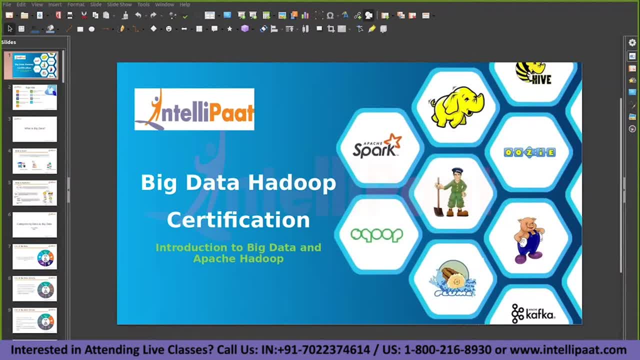 coming from. I mean, why is this coming in in such huge amounts and what is the need for you to store such large amounts of datasets? so if there is no real use, why do you even have to think about storing such large amounts of datasets? First thing: right, and with what speed it is getting generated? right, so it is generating. 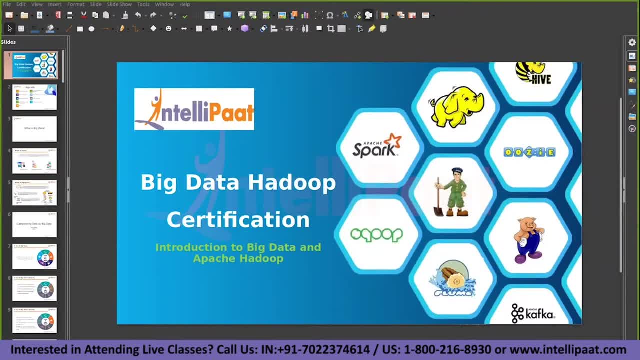 at some hundred mbs per second, and ideally it won't. but okay, hundred mbs per second, so you should be able to capture it with the same amount of speed, right? so it is getting generated at 100 mbs per second and you are capturing it at 10 mbs per second. let's say 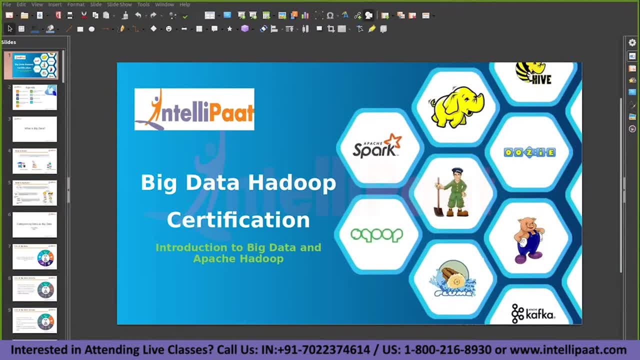 so there is definitely a lag, there is definitely a loss of data and you are, you are kind of getting lagged, so you should also be able to consume the data With with whatever speed it is getting generated. so that is one problem. so the size is definitely. 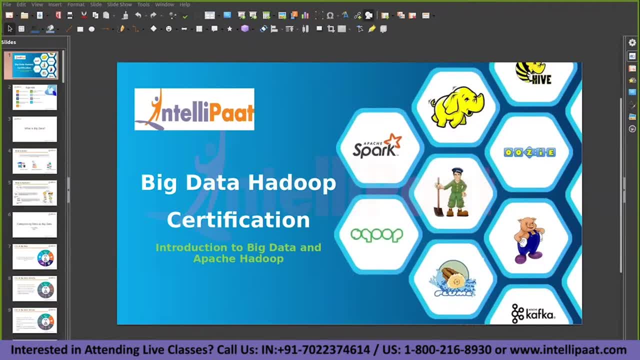 a problem. so what happens when the size increases? the storage problem will come right. so in in your traditional systems, you, you, you- are not used to handling such large amounts of data in in terabytes, petabytes, you, you generally don't design the systems for these amounts. 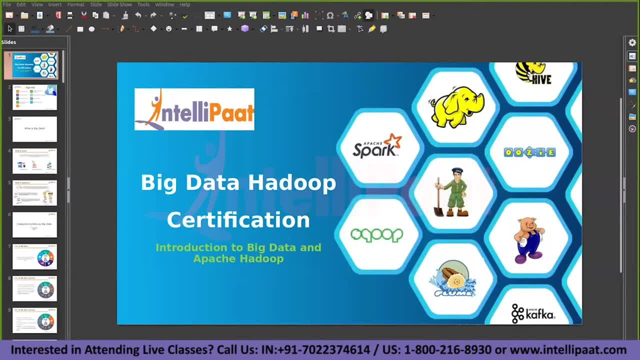 of datasets, right? so I'm talking pre Hadoop days, so before before Hadoop coming into existence. this, this is what the challenge is, so this is what the scenario is. Right, so we were not used to handling such petabytes of data, definitely, so the problem. 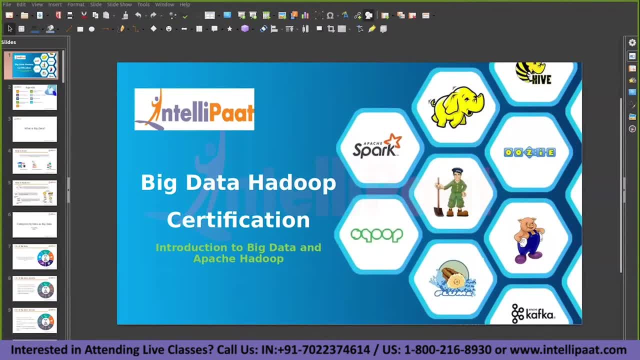 with the size is definitely with the storage. I mean we don't have the enough systems or enough enough hard hardware storage which could accumulate such large amounts of datasets. and the problem with speed is also the technology again. like what technologies are you going to use to to capture this data that is coming with high amounts of speeds? 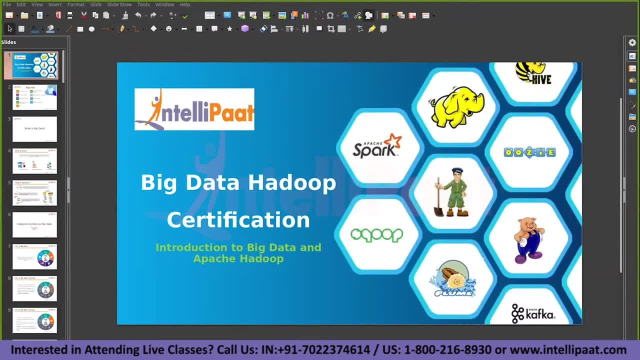 And what is the other problem that I was talking about, the type, right? so what are these? what are these types of data which I said? when I say types of data, what does this actually mean? there are some tools which you use for storing the data. right, already you have been. 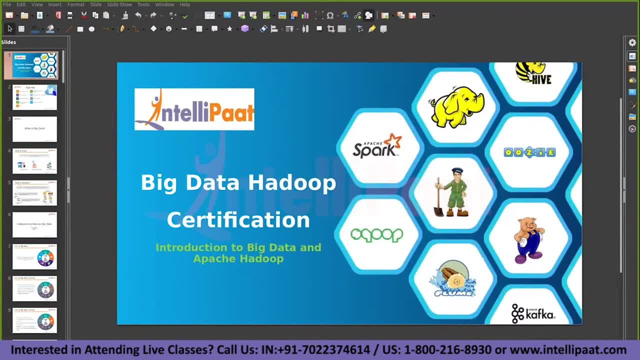 using some tools like like oracle, plsql or postgres or what else. you have mysql, right, right? so all these tools are meant for storing a certain amount of data. what type of data is going to store? it's definitely structured, Right. so you cannot, you cannot store unstructured, or you cannot store semi-structured data in. 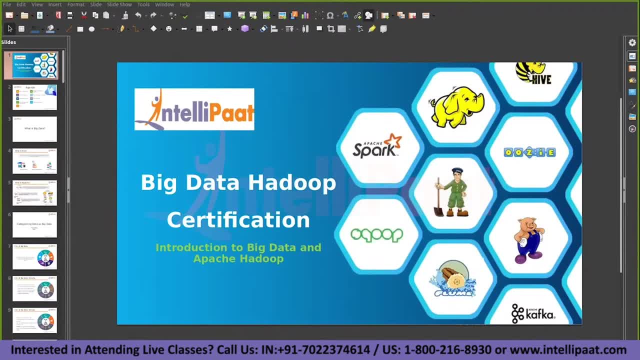 a oracle database, so we are used to mostly dealing with the structured amounts of data. so can anyone name me the unstructured data processing tools? okay, interesting answer, notepad. okay, anything else. I mean where? how do you store this data in notepad? how do you retrieve? 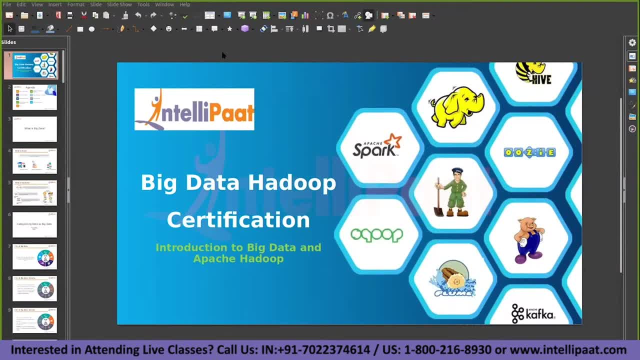 it? how do you kind of process it? I'm telling, basically, you should be able to store it. you should be able to store it, You should be able to query the results and you should be able to kind of transform the data within it. so not completely aligned with your answer, so any other, any other answers? 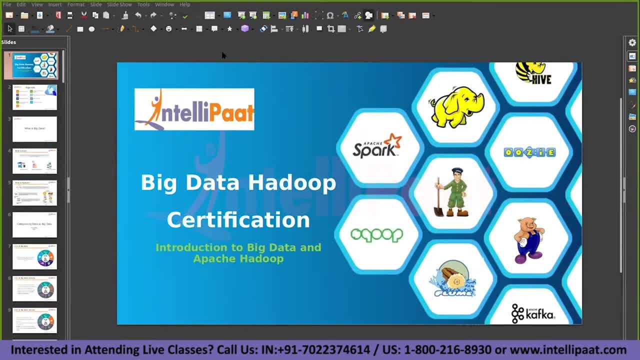 Cassandra, MongoDB is a better example. so have you heard about MongoDB? it's a document database. so there are, there are some tools so which are not known or which are not in use most, most mostly because in in earlier days it was a document database. It was completely structured data that we talked about. so what we have is is a structured 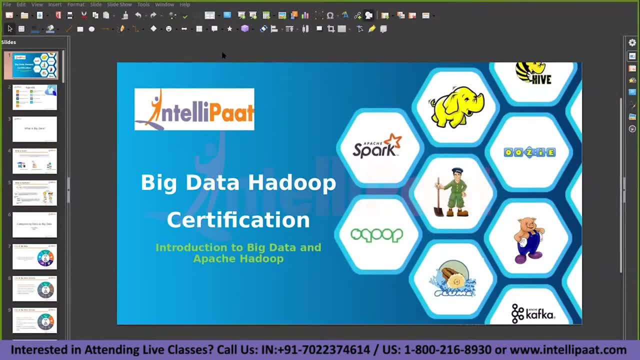 data in in terms of rows and columns. you just create the databases, create the tables and align the data to to those tables. so that is a problem. so suddenly, the the growth of this unstructured data or semi-structured data has increased a lot. and what has actually 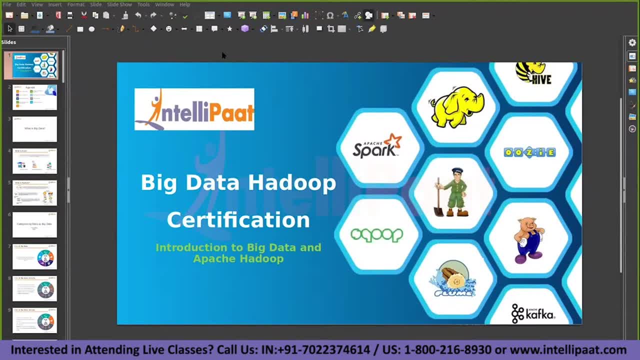 comprised for this growth? why is that there is a lot of change, or why there is why there is a lot of increase in the unstructured or semi-structured data. One simple example, or one known example for all of us, is kind of a social media right. 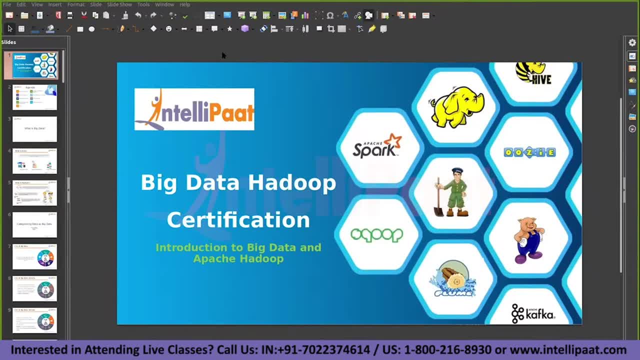 so forget about now. just think about around 10-15 years back. so, do we have Facebook? do we have insta? do we have? what are? what are the other tools? you use whatsapp, right? do we have all these things? no, right? yeah, so the usage of these tools has has increased. 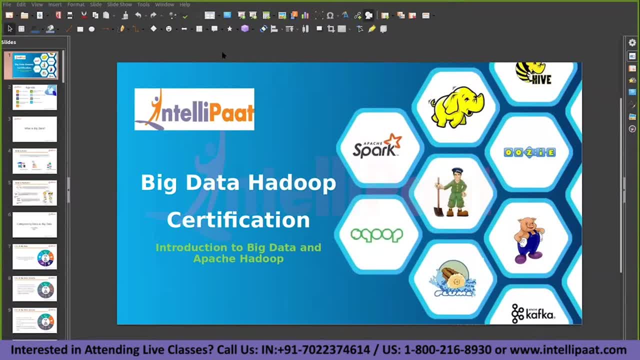 drastically. the number of google hits have increased, the number of people using the gmail, using the social media accounts, have increased and there is a lot of digital data that is getting generated now. so where does all this data go? for example, you take facebook, you, you like some page, or insta, you like some, you like some image. you have the snapchat. 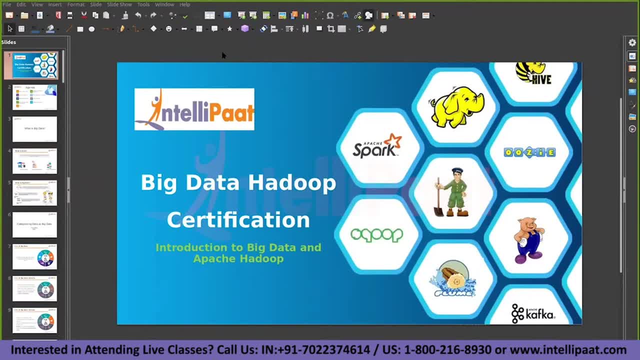 you upload some pictures, right? so what is the picture it's? it's some kind of an unstructured data only, right? so where does all this data go? you, you're doing some activity on a social media account. is is all getting stored somewhere, right? So definitely, you, whatever the likes you, you, you do whatever the um activity or whatever. 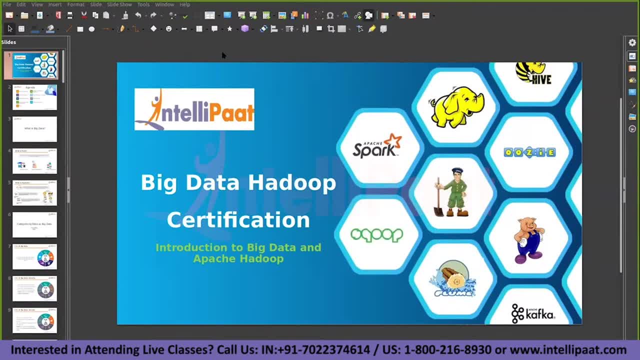 the comments you post, whatever the content you share, everything is some is is generating some amount of data. right, let's say we take an. we take a better example: amazon. you log into amazon portal, you, you search for certain records, you search for certain products, right, so you search the product. you log into the account and you search the product and next. 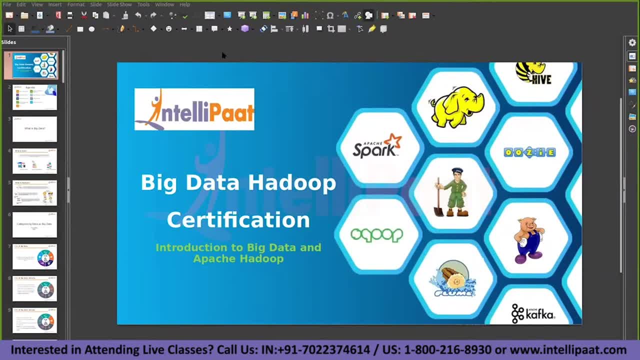 time you log in, you'll find some suggestions. Okay, So how are the those suggestions getting generated depending on your previous search? it is it is trying to identify your interest. okay, if you are, you are searching for an ipad. okay, so what are the other products which are related to the ipad? some something like a two-in-one. 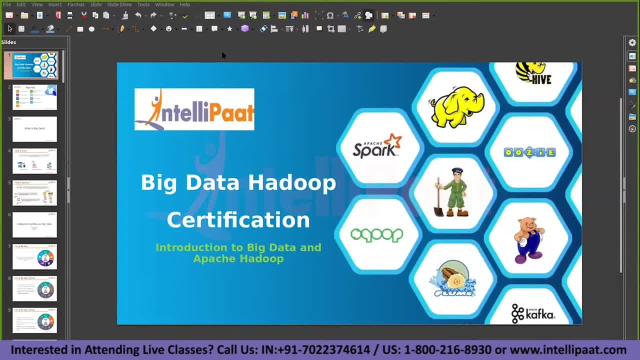 laptop, which is, which is microsoft surface pro. it's going to give you a suggestion saying that, okay, okay, so ipad is only meant for this kind of activities. we have another product, surface pro, which, which can do both, which which can, which comes with a keyboard, which comes with a pen, and all that. 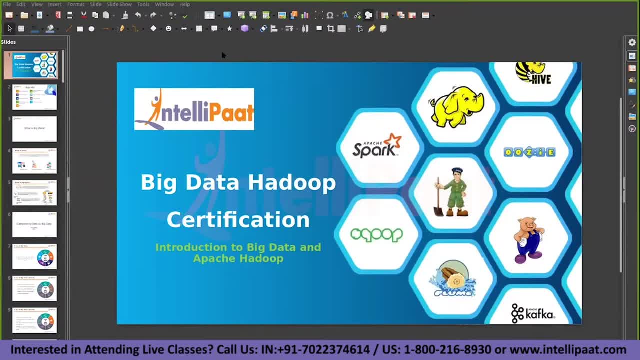 All that stuff, right? so this is some kind of a suggestion which it is giving. based on your search history and even when you log into the google or when you, when you go through some other, uh, social media accounts, you you kind of get this, we kind of getting this uh. 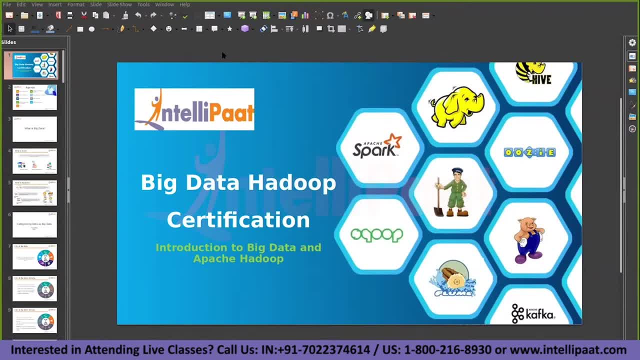 pop-ups which with the products that you have searched for, right? so how is that linking happening? i mean, how is that even linked to your, uh, social media account? so there is, there's definitely some kind of activity that is happening beyond your control. i can say: right so everything. 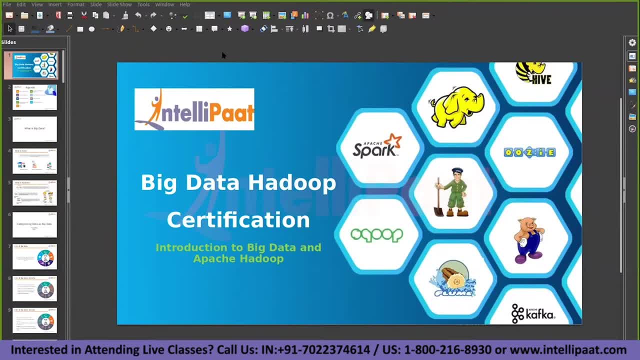 is being tracked. Your data, whatever the records that you search for, whatever the products you search for, is being tracked, it is being analyzed and based on that, it is. it is being used, uh, to give you a better experience. i can say: right, so why are you getting the suggestions? i mean 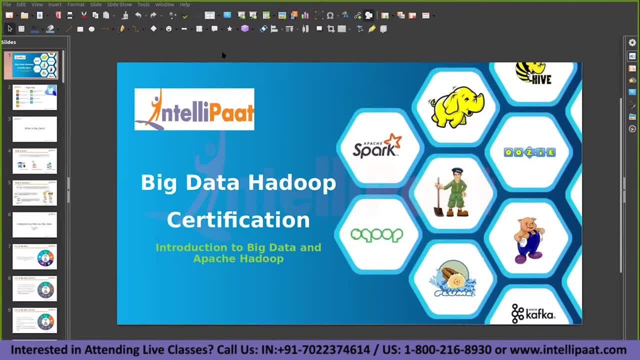 if i'm i'm looking at the suggestions and i'm finding the product which i'm actually looking for. it's. it's good for you, only right. so that is kind of increasing the user experience. so all these uh companies or all these products that you are using, is kind of increasing the 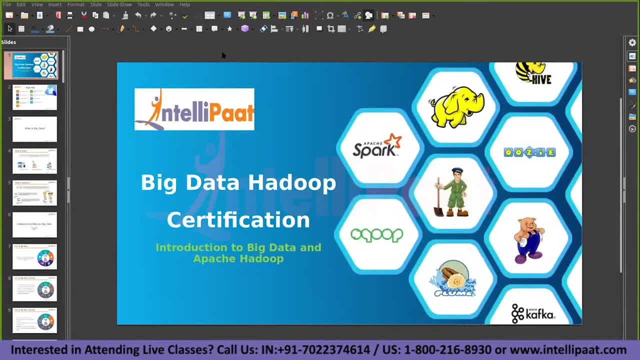 product experience. you can log into facebook. there are a lot of friend suggestions that you can use, So you might you might find a friend which you have known right. so these are all. these are all kind of activities, which is which has been increased a lot, and that is actually. 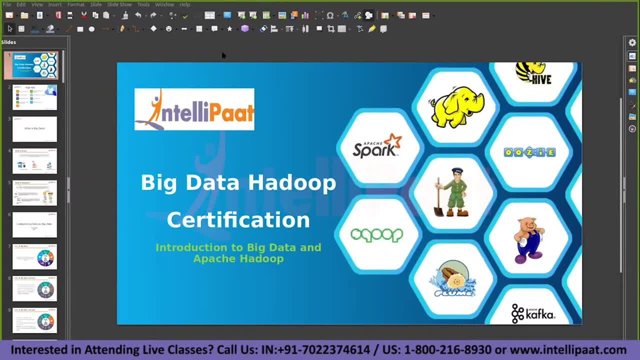 being comprised for these unstructured and semi-structured data. that's what i'm i'm trying to come up to. so definitely there is an increase in the rate of the structure- unstructured data and definitely there is a need for you to process this unstructured data or store. 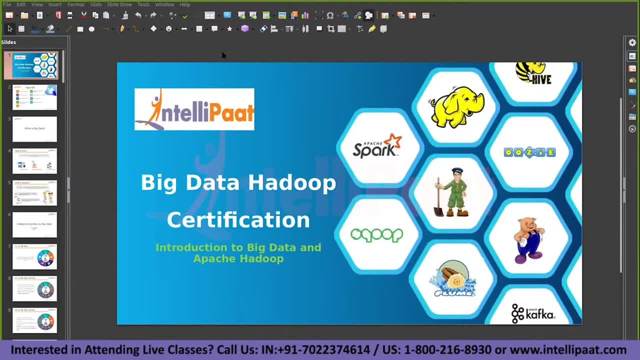 this unstructured data in a proper way. so that is what some of the problems i can say. these are all Some of the problems that we have with the data, with with this big data kind of a tool. so we should have some technology which should pretty much store any amounts of data at least. 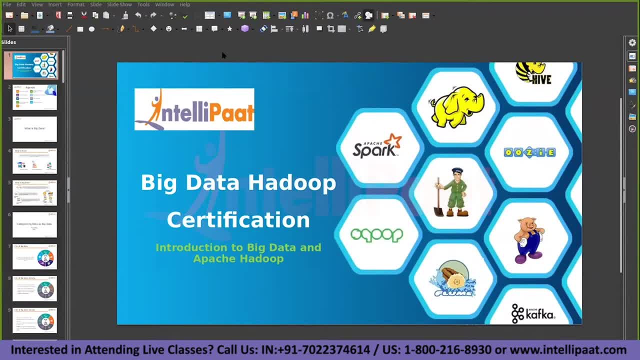 at least with whatever the questions that we have now. so my technology should do what it should: store any amounts of data. it should not have any limitations to the storage. so, getting 100 petabytes of data, you should be able to capture this, all right. so that is. 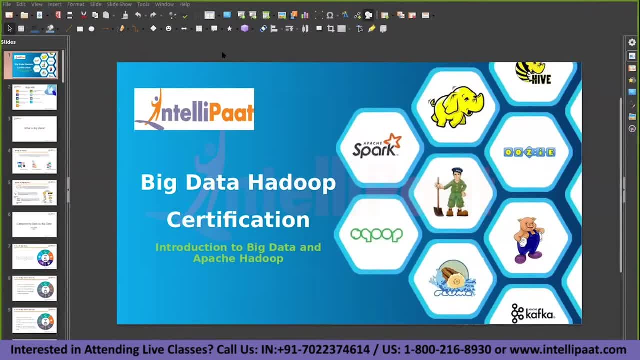 how i have to design my new system And then i have to Capture the data with whatever the speed it is generating. so you should have some tool which should capture the data with whatever the speed the data is getting generated. so what do we call this activity? a streaming activity? i can say: have you heard about this? 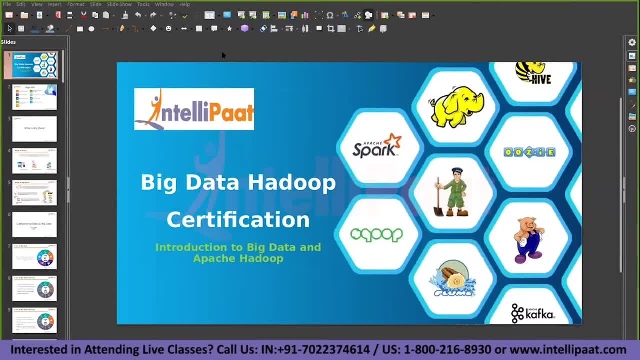 term streaming data streaming. so there is a match that is being happening on some other state, some other country and and you are able to stream the data, stream the content within within seconds of time. there is definitely a lag, some seconds of lag will be there, but you are able to stream it near real time. okay, so we call this term near real time, so there. 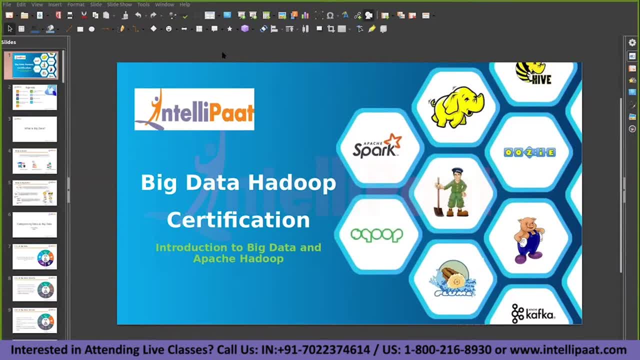 is no technology or no tool. real time it's. it's all a near real time procedure. right? so the match, which is being telecasted in some other countries, is being viewed here within, within within seconds of time. so how is it done? you, you are streaming the data. 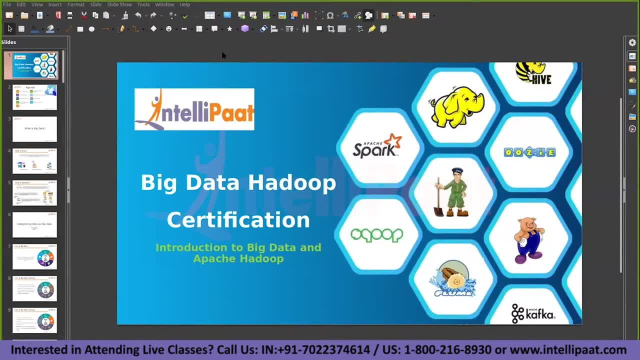 continuously from the source location to the destination location. so sources where in in the country where the match is being held on And The destination is you being a user, okay, you can log in from any particular location. you can log into so and so application, hot store or whatever, and you can. you can stream the. 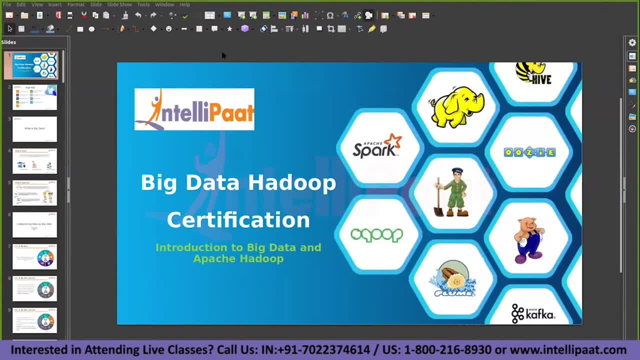 data real time and near real time. so these are, these are some of the tools i can say: right, so you should, you should have a technology, you should have, you should build a platform which should be capable of streaming the data in in a near real time procedure. right so? 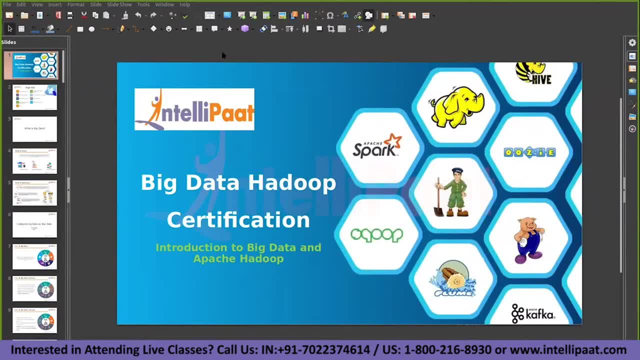 you should be able to capture the data data with whatever the speed it is getting generated, without any loss of the data. then what is the other problem? that we have been talking about types? right, so there are different types of data. so whatever the platform that you are building, you should be able to capture the data with whatever the type it is coming. 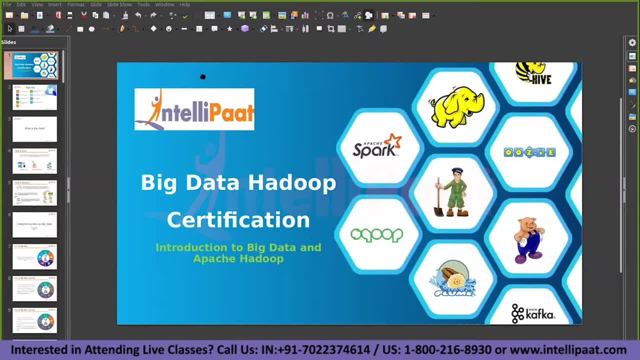 so if it is in a jpg format, you should be able to store it. if it is in a dot ext format, you should be able to store it. if it is in a dot, csv, dot, json dot, avro dot park, at whatever the format it it is going to generate, you should be able to capture it and store it. 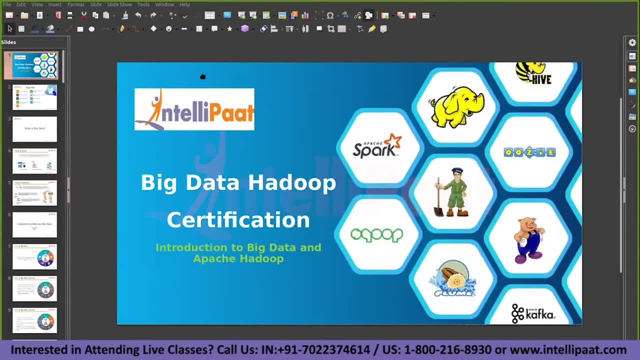 and process it okay. so these are some kind of expectations that i have from the platform now, right, so we have seen what are the challenges, some of the challenges. i can say we have seen some of the challenges, some of the major challenges, and we've also we also have some idea on what. 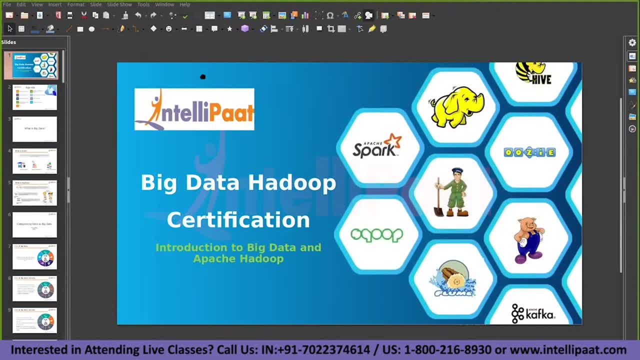 my platform has to look like, right, so it has to store any amounts of data, it has to capture the data with whatever the speed it is generating, and it also has to store any type of data. so this is pretty much my big data, right? so the tool which is being used the the platform. 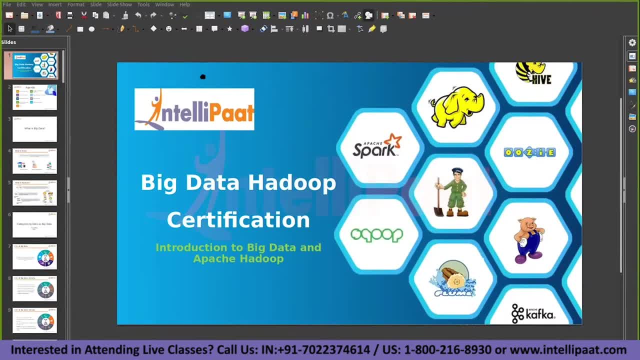 which is being used to analyze all these kind of uh challenges? is your hadoop? okay? so hadoop is a combination of multiple tools together which, uh, pretty much solves all these problems, all these challenges that we are facing in the real-time scenarios. are we clear? are we? 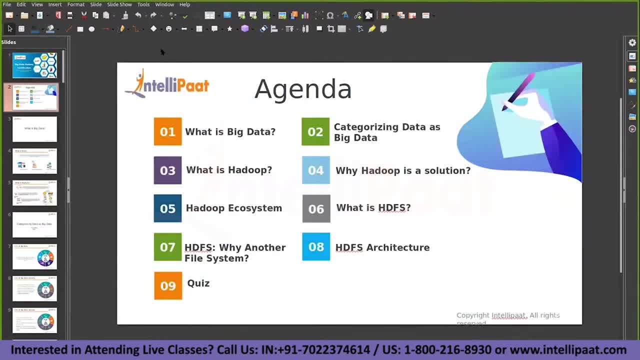 clear with the introduction. what is hadoop? why do we need to do this? why do we need to? why do we need it? what is it going to provide us? are we clear with that piece at least? any questions or any deviations with whatever you have in mind and whatever i am teaching. 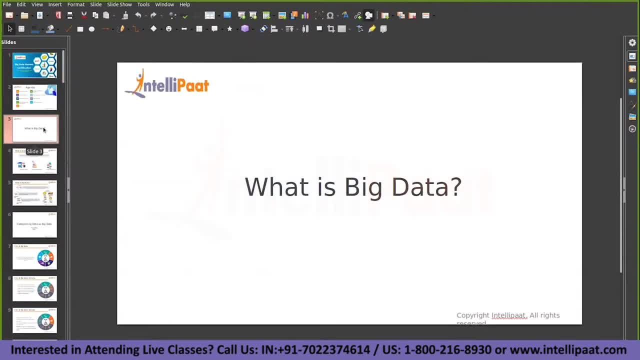 so, uh, what is big data? we at least had some uh non-theoretical or non-technical uh definition, right, so something which is, which is beyond the capability of, uh, the existing storage systems. we call that as a big data, which which comes with some speed, which comes with whatever the type and 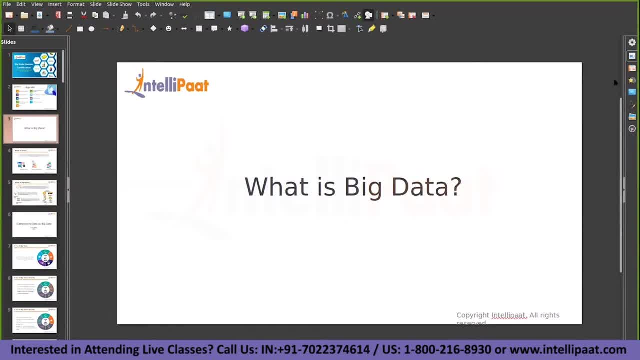 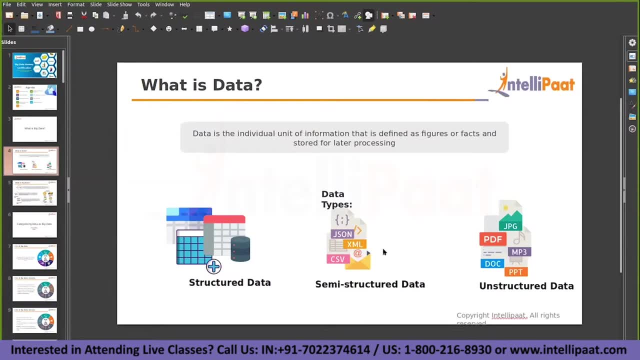 all that, you can frame it with whatever we discussed. okay, so that is going to be my big data, right? so, firstly, what is data? there are different types that we have seen: unstructured, uh, semi-structured and structured. so structured- you must have known it already- which is which? 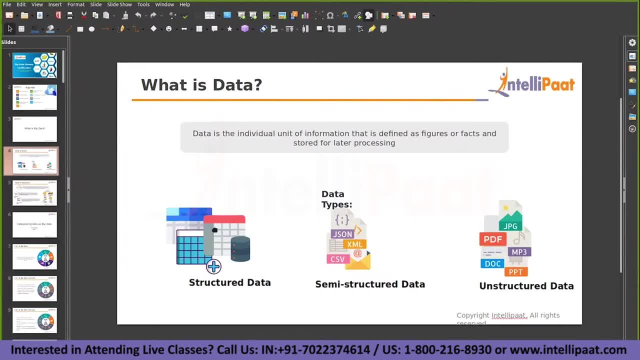 can be stored or which can be given some schema to it. you can give some structure to it, which comes with a row and a column definition. you will be able to store them in the databases and, uh, the unstructured or semi-structured data is, is a json, xml, csv, uh, we have other other such. 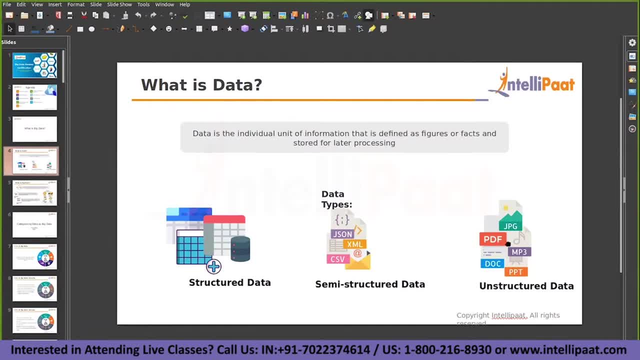 formats also, and unstructured, you have this: images, data, video data, uh, pdf, document related data. everything comes under the unstructured data. so have you heard about or have you known any tools which actually can uh, read a pdf or which actually can read a document, mp3 or whatever ppt? have you seen any tools by yourself? excel? 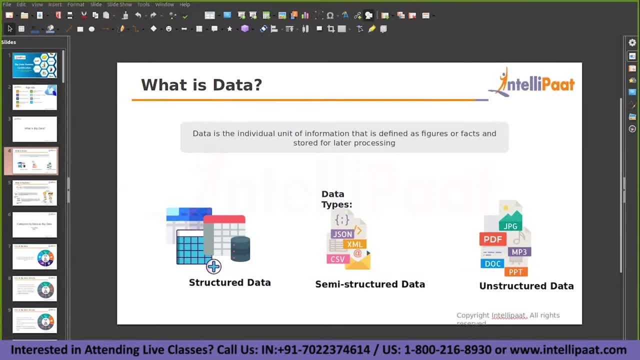 someone is giving me some kind of an interesting answers, actually. so notepad is one and microsoft excel is one. okay, so what do you do with excel? how is it unstructured data processing tool? so when i say unstructured data processing tool, i should be able to store it. okay, fine, i'm, i'm. 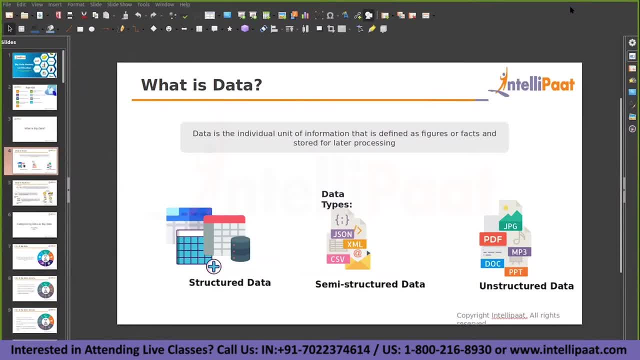 happily uh accepting that excel can be used to store the data. and how can you process it? how can you kind of uh transform the data? you write some code or you write some program, you transform the data right and that's that's gonna have some limited number of. 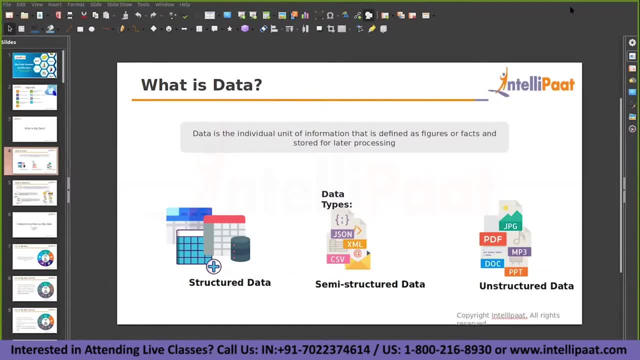 rows at least. anyways, right, excel is again. i can. i can call it as a structured data processing tool, structured data storage only, not unstructured, right? so when i say pdf document, i have a dot pdf file, okay. so most of you have seen the dot pdfs, right? 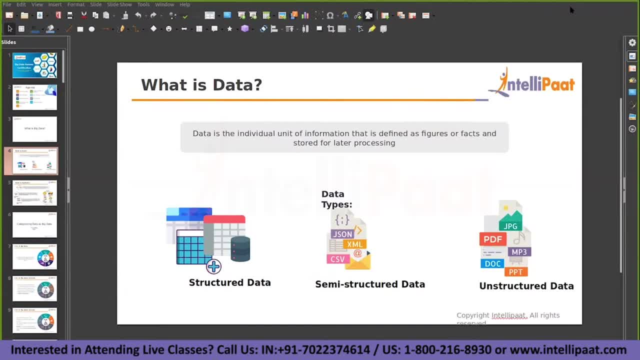 so i have a dot pdf file. have you seen a tool which can read the data of a pdf, which can analyze the data in a pdf? whatever it could be a text data or an image data, it can. it can have any data right. it can have some text, it can have some paragraphs, it can have some table. 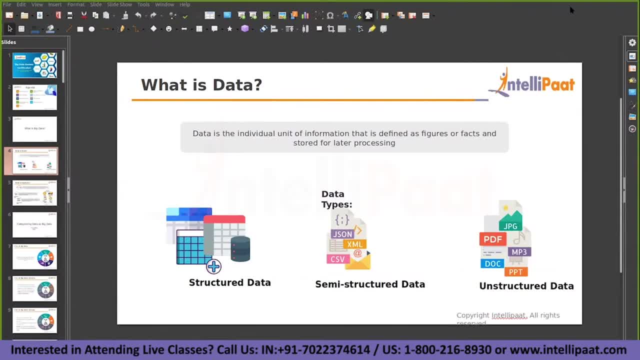 and then followed by an image, and all that. all that will be part of a pdf. so have you seen any tool which can actually do all these things: store a pdf file? this one analyze the data of a pdf, analyze the text of a pdf, analyze the image of a pdf, and all that. have you seen this, or can you? 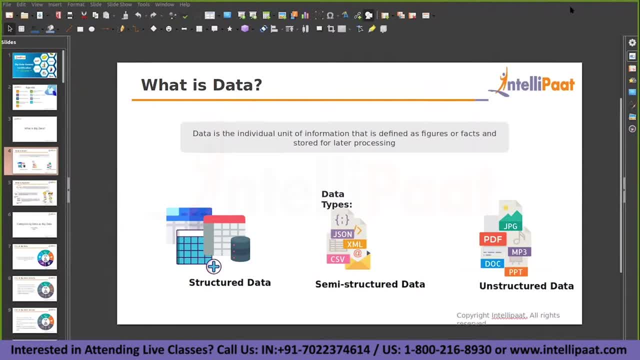 deal with it. okay, let's say we don't have a tool at all, but can you handle this by yourselves? how many of you are familiar with python or any java programming, interesting knowledge on java or python? so there are some packages, there are some libraries already developed. okay, so in python you have. 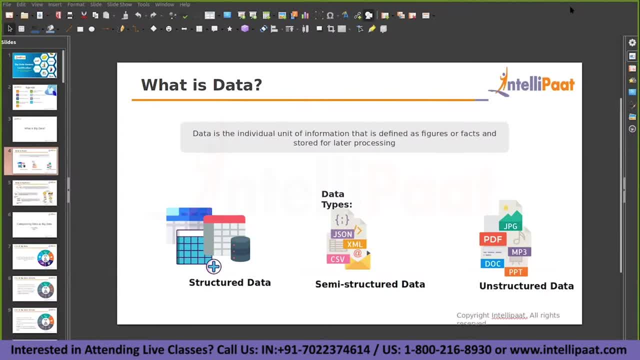 uh, pypdf, you have tesseract, so these are all some kind of uh pre-built uh libraries which can help you deal with. uh, this kind of data sets, reading a data from a pdf or a some some kind of an extension, dot, bam, dot, sam, or different, different extensions you might have. so there, 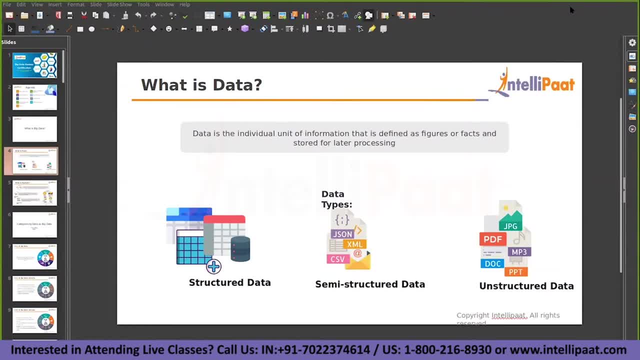 are some libraries already available, so you can, you can do it by yourself, you can. you can code some programs, you can. you can code some programs, you can. you can code some programs. you can use that library and you can import it. you can import the package and and build some. 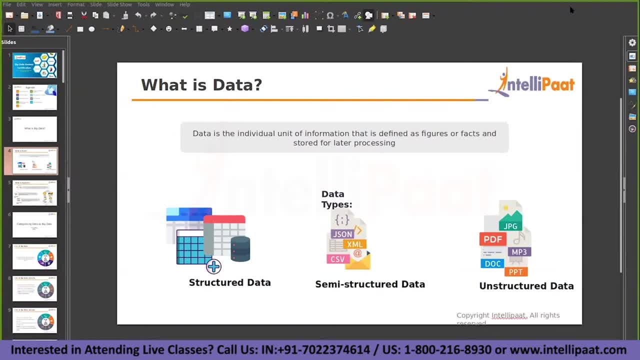 programs and you can. you can do it by yourself. that's what i wanted to say. okay, so that's what we are going to do in in hadoopa as well. so you import the existing packages and, using them, you are going to build some kind of a code to to read such files. okay, so that itself is going to be. 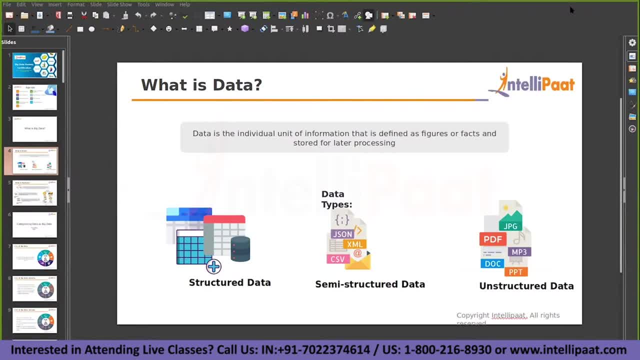 unstructured data processing. we are not going to do it very extensively and most of the are not. many clients will have the data coming in a pdf or a doc or an mpg or jpg right, so it's. it's very limited. there are very specific clients which are mostly related to health care. i can say 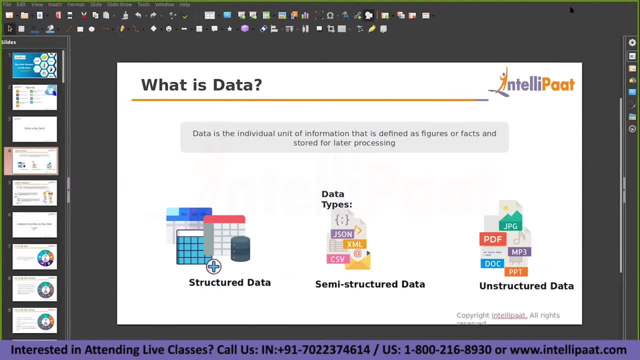 okay, so, which i have seen myself, so health care clients will have very, very odd formats of data. okay, you, you, i mean when you, when you look at the data, you don't have an option to read the data also. so what do you do? generally you open a pdf file or, if you generate some file, 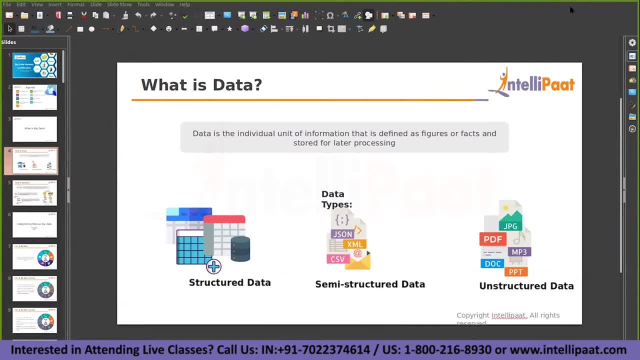 in. if you, if you get some file in some dummy format, what do you do? you open with a decknote pad plus plus, right. but even even that is not possible. you don't have a proper reader also to to read the data. so there are such kind of data coming in. you have this x-ray data coming in you. 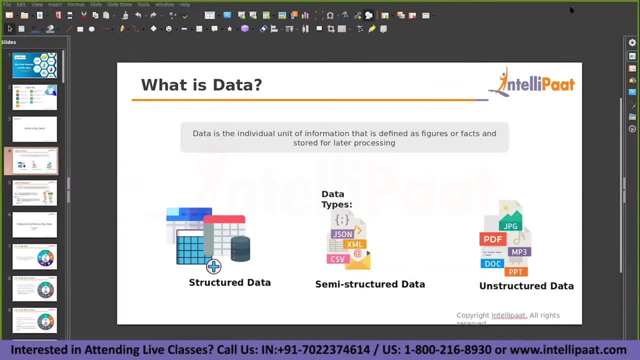 have this scans, different scans, related mri related scans, data coming in. so we have actually seen that kinds of data. so that is how the scenario is going to going to be. you will you will come across different formats of data, everything. everything falls under the unstructured. 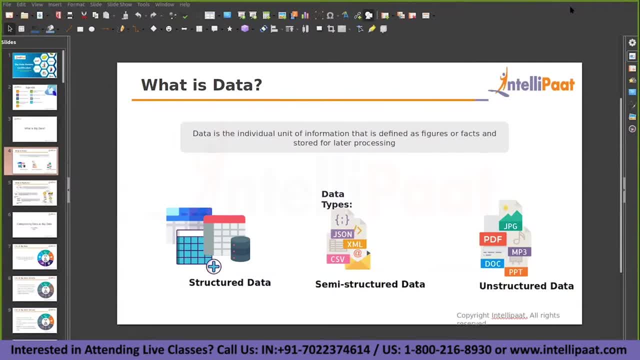 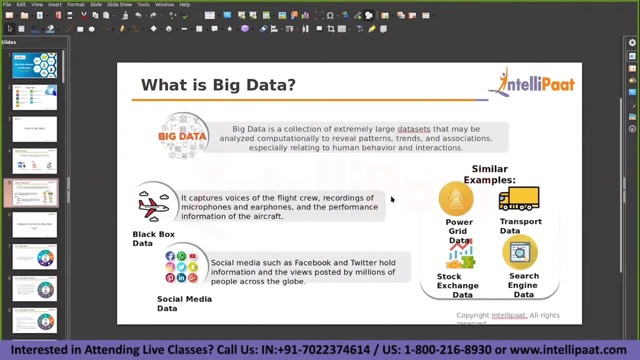 data format only. okay, so fine. coming back to where we are, when we say data, there are the different types of a bit. we've seen what is the structured, semi-structured and unstructured, and then we'll see a little bit of a technical definition. i can say it's a collection of extremely large 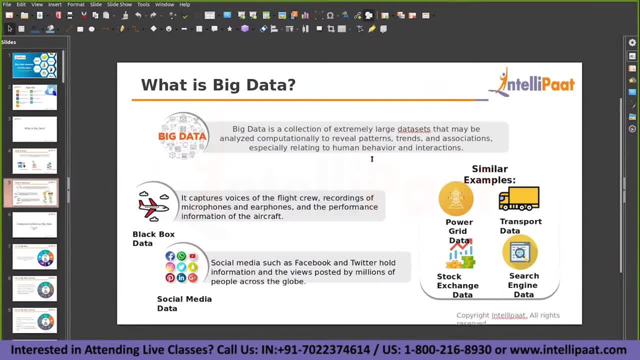 data sets that may be analyzed computationally to reveal patterns, trends, associations, especially related things related to human behavior and impacts. so so this is not a technical definition, this is just an introductory content. so where is this data coming from? uh, the data from blackbox, the data from social media is is pretty much accounting to what, uh, the big data is all about. 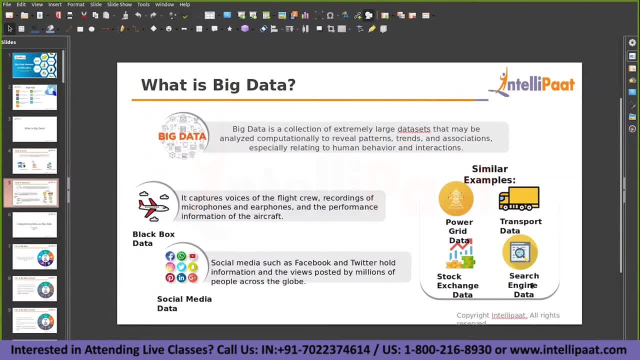 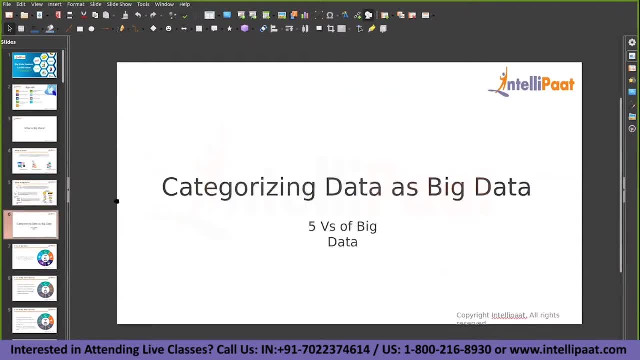 and there are other examples also: this public data, transport, the google search engine data, or a stock exchange data, or a power grid data. so everything, everything falls under this big data, right? so now categorizing data as big data. so what is this? five v's. have you heard about this five v's of big data? initially, when we learned, it was only three v's. 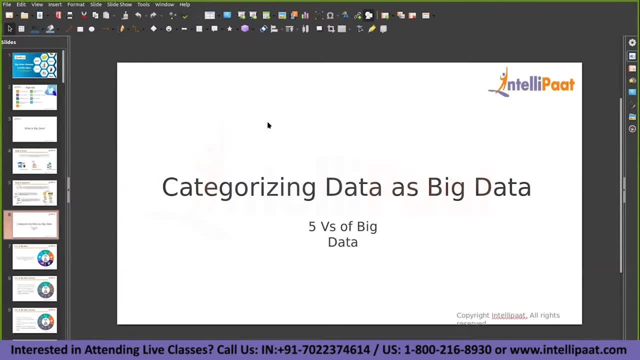 i remember right. so later on, later on, people started to name the other two v's as well. so now the documentations, everything were holding five v's. so i i remember, i pretty much remember very strongly that initially, when i uh got into this big data technologies, we were only talking. 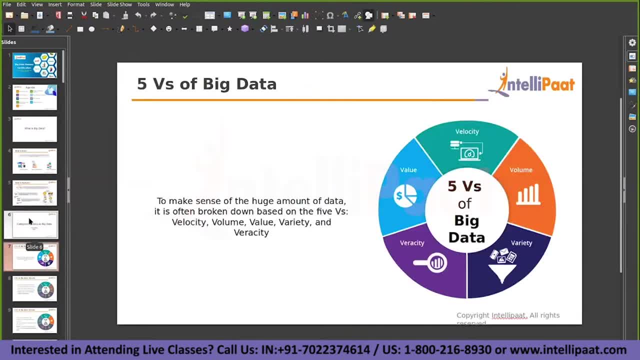 about three v's, but that's fine. so let's see. what are these five? is this, these five is we can actually categorize, categorize them as the characteristics of the big data. okay, so we've already seen three of them. what is it storage which comes under volume and what is the? 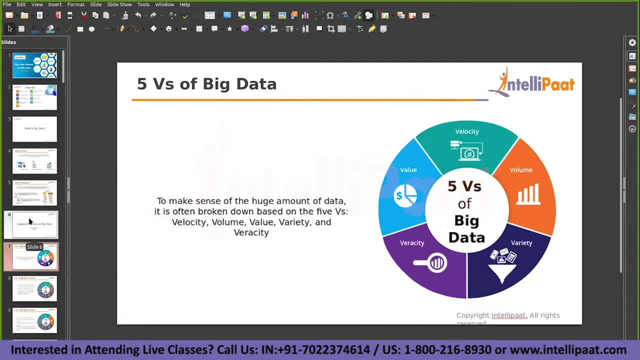 other one variety is the types of data. and what is the other parameter that we discussed? we discussed about storage problem. we discussed about type of the data problem. we discussed about one more: speed. speed is going to come under velocity, so what is the other two like value. 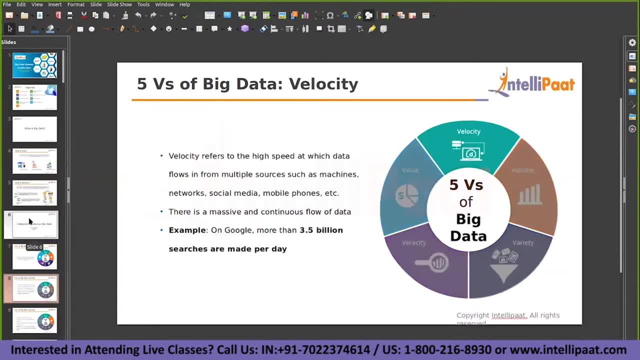 and the veracity. so we will see. we will see what are this. so first thing is the velocity. so velocity refers to the speed with which the data is coming from. so, generally, when we talk about big data, when we categorize this data into big data, one of the characteristics it can have is: 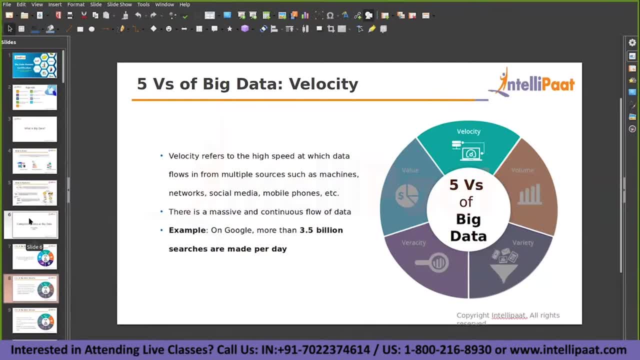 a velocity. so if the data is coming at at full speed and then we can call, we can categorize that into a big data. so now, when i, when i build a platform, your platform should have the capability capturing the data which is coming at high speeds. right? so this is my problem, this is my 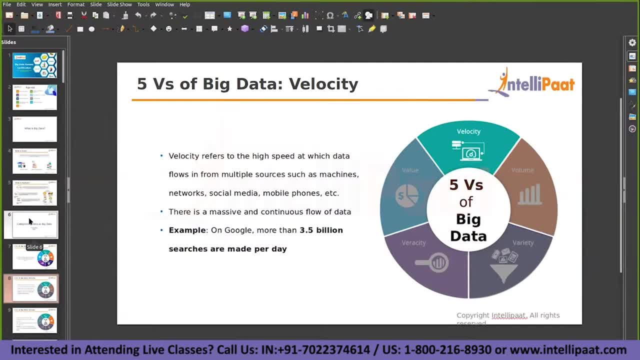 categorization, and this is my solution that i'm looking at. so with with the help of the categorizations only, i'll be able to build my solution right. so we have not yet built this solution of big data had to. so we were only talking about: what are this big data? what are the? 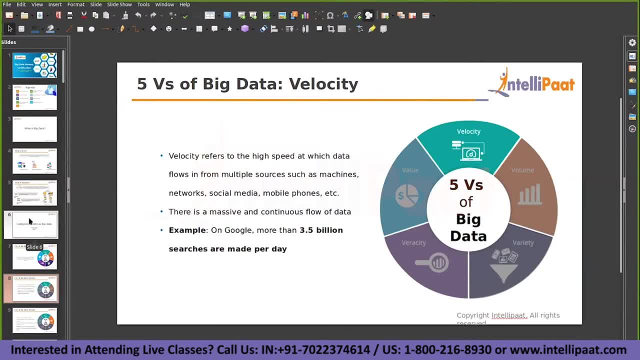 different characteristics that it's going to have, and when i'm building a platform, what i need to have or what i need to have in my mind, so that i'll be building this particular platform right. so now, first thing, i've categorized as a velocity, so if the data is coming with so and so amounts, 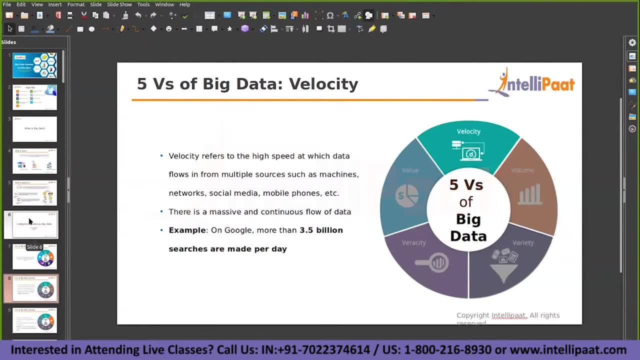 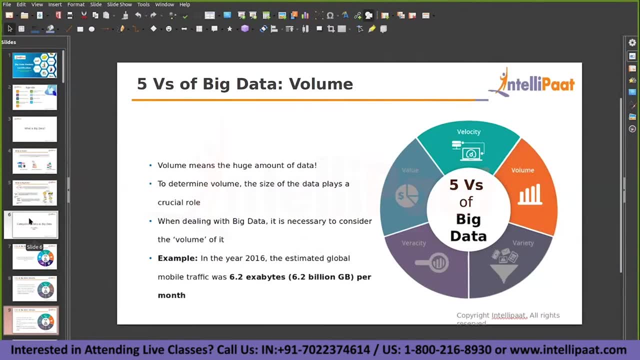 of speed, i'll categorize that as a big data. so now, when i'm building the platform, i should be able to handle this challenge right. so second thing is a volume. so when i have huge amounts of data sets, when the data size is very huge. so when do i say the data size is very huge? 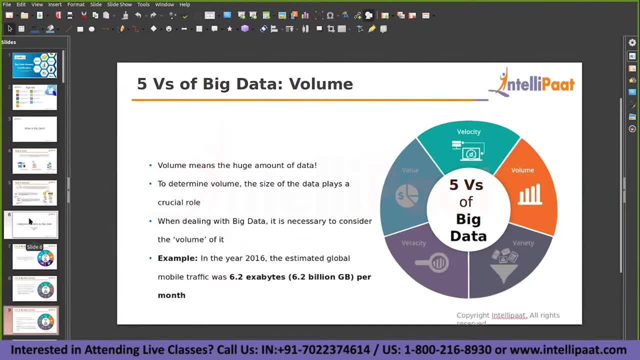 how can you even justify that? okay, this data is small, this data is huge. how can you categorize it? i mean nothing technical, a simple, simple understanding. okay, let's say, i have 100 gb machine, you have 1000 gb machine and if i have to store 500 gb, for me it is huge, for you it is. 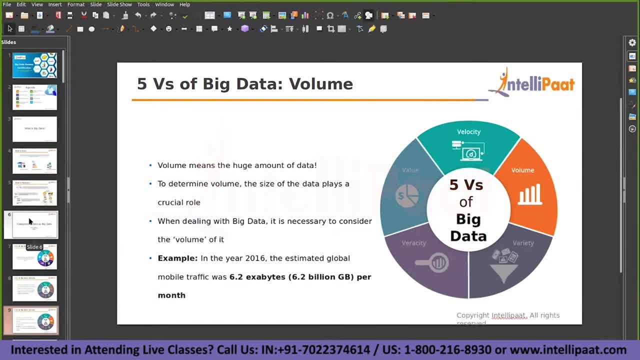 capable. i cannot say that it is a huge data, or it can. i cannot say it is a big data, agree so? so when i say this volume, i mean in terms of any any other characteristics also. so when it becomes beyond the capability of the existing software that we have, with the existing technologies that we have, 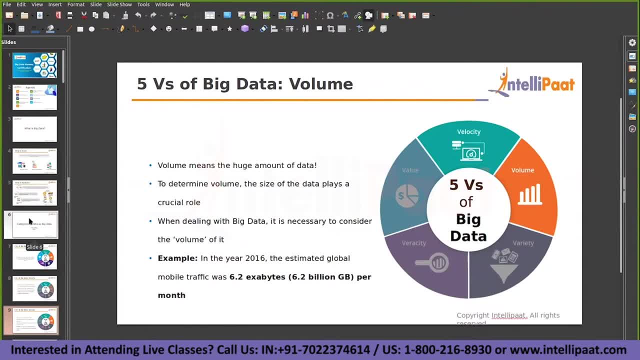 let's say i have a sql or mysql, or let's say i have oracle database, right. so when it, when it becomes beyond the capability of these known tools, these known technology tools, i consider or i categorize them as big data. so what is the capability of my sql or mysql? i see that it is becoming beyond the capability. 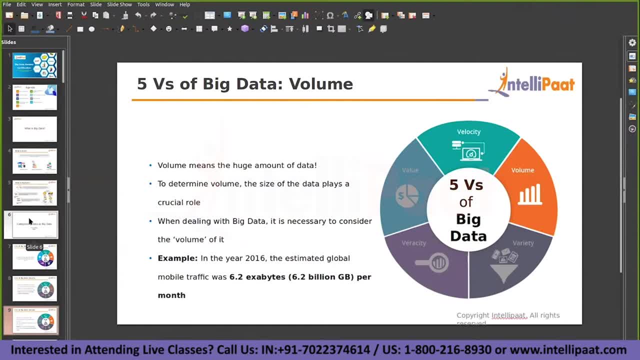 of my existing tools and technologies. i categorize them as a big data, right? so when it reaches, i mean when the size of the data reaches beyond the capability, okay, so uh, let's say how, how do we categorize? how to? how do we say that we don't have exact numbers? let's say no, okay, so what is? 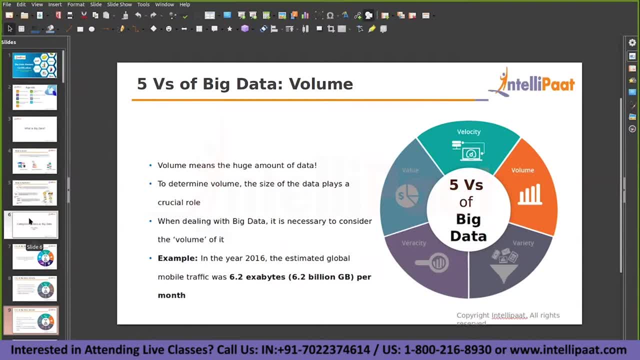 my capability of mysql and oracle and all that we don't know. so, all of a sudden, when i when i kept loading the data into an oracle database table, it became slow, right, so the query became slow. you are not able to perform joins, you are not able to perform select queries, even even a simple. 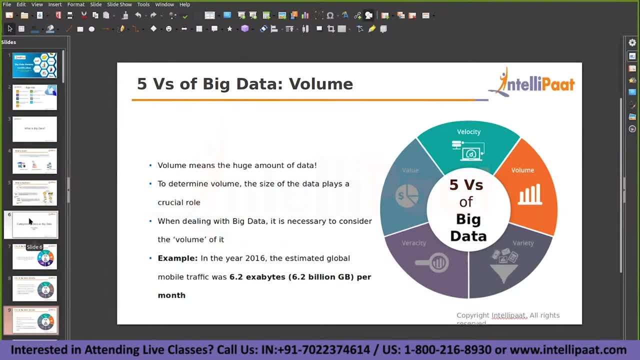 select query is taking lots of time to generate the output, so that means it is it's it's done now. so i i am i'm reaching the uh threshold level, that i cannot store more amounts of data on it. so what do you do? you break that into two different tables and you sort them that again. 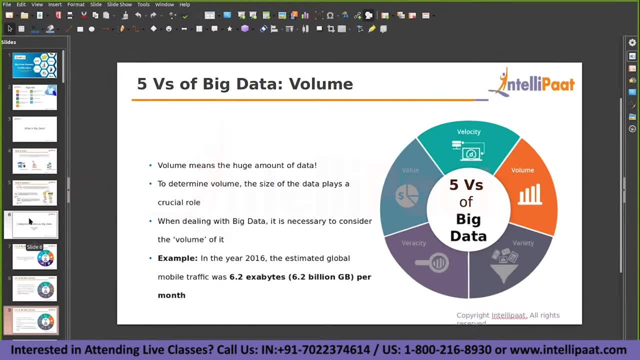 is going to be a challenge for you, right? so those are the things i mean. when the size becomes uh, beyond the reach of your existing tools and technologies, we categorize them as a big data. that's what. that's what i was trying to say. now, variety: we know what is the variety. 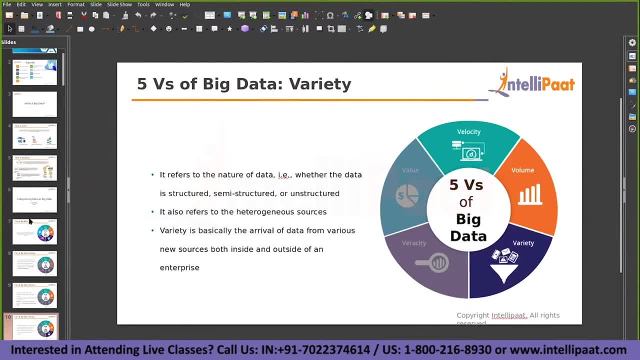 the different types of data when you have structured, unstructured and semi-structured. so it's not that we don't have the tools which can handle the semi-structured or unstructured at this moment, but it's. it's the case where, see, for example, if the data is coming in a structured 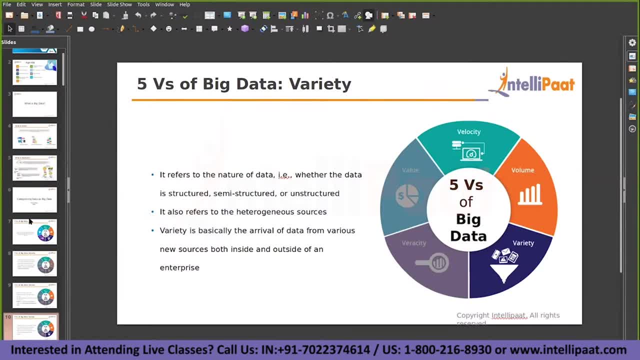 format, i'm using this tool. if the data is coming in an unstructured format, i'm using a different. it shouldn't be a case i should have a single technology. i should have a. i should. i should build a single platform which should not worry about the type of the data. okay, if it is coming in a dot, csp, extension, dot- pdf. 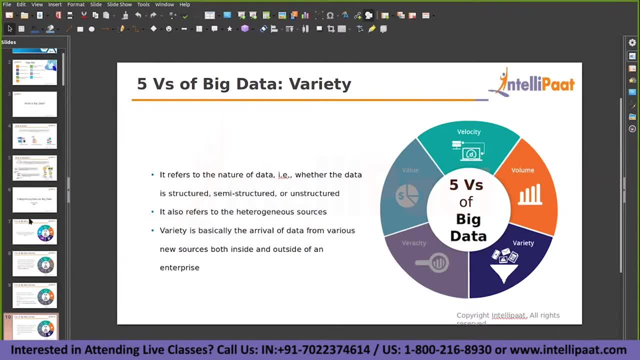 extension: dot jpg expense extension. it does not actually have to matter, it just has to store the data with, whatever the format it is coming in. so that's what my my requirement is going to be. so this is my categorization if the data is coming in different, different formats, in different. 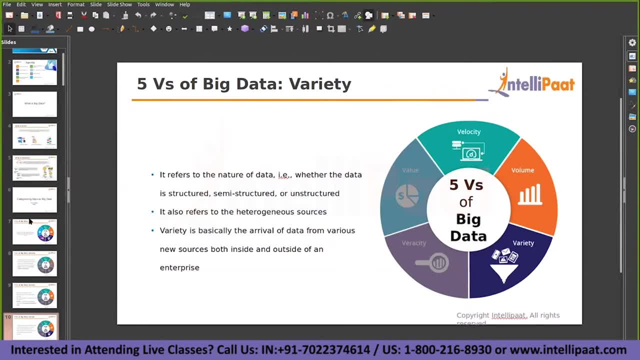 types with structured, unstructured and semi-structured. when the size becomes huge on this particular varieties, we categorize them under this: uh, variety v of big data. okay, then the veracity. so what do you mean by uh, the veracity? any, any answers? or i can say it's going to be a, a grammar related answer. i mean, who is? 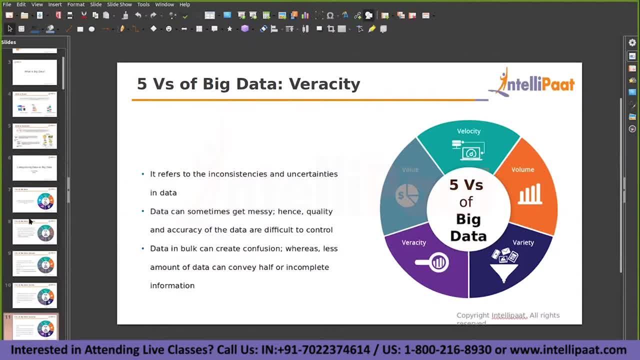 whoever is, whoever understand these terms, can answer this question. what does veracity mean? okay, so the trustworthiness of a data. i can say in simple terms: so fine, uh, your data is huge, it's speed, it's, it's whatever, whatever the characteristics can it can have, but how far is it? 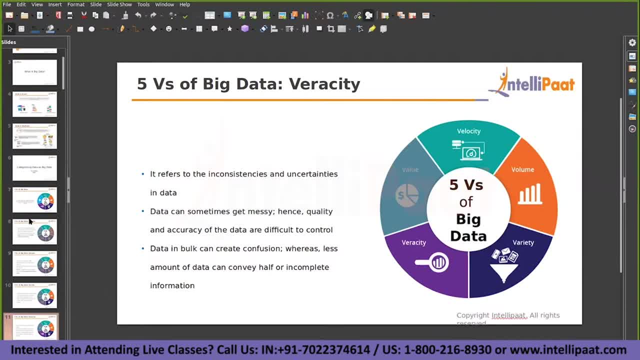 trustworthy, how far is it accurate, or how far is it, i can say, quality. so nowadays, when you, when you talk about the data that is coming in in, in simple terms, in in known languages, let's say: i am, i'm getting some 10 million records from a source. okay, you are a data engineer. 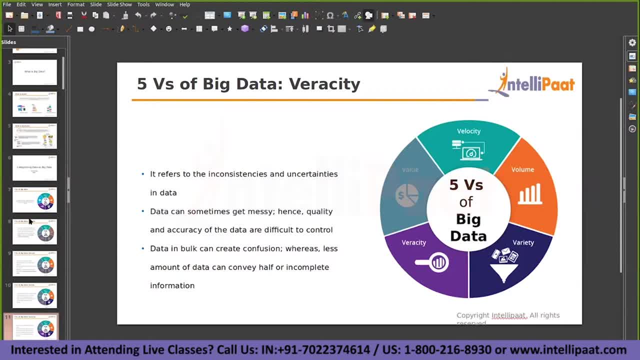 in so and so company. you're getting, uh, some 10 million records into the source, from the source, and you're supposed to store them in so and so database. what are the things that you're going to consider? you'll definitely consider, you'll definitely analyze the first. 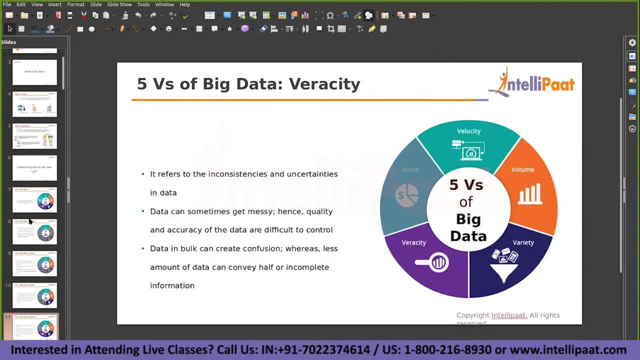 thing is that the 10 million records are not the purest data, are not the quality data or the accurate data. you may have to check for the duplicates first. right, it may have duplicates or it may have some dummy records. okay, first you will definitely consider. you will need. 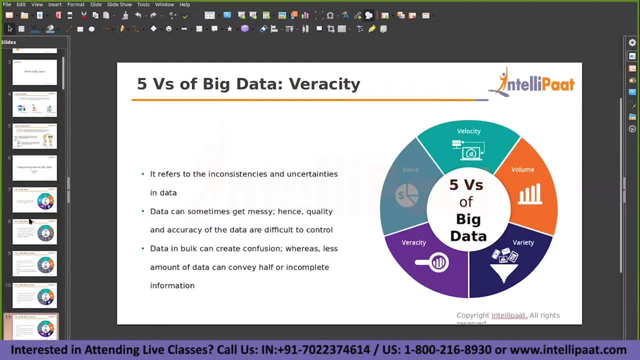 to see the gest al, and then you have to use what's yourANSность test structure, sort of rigid data. so that is theessa for this lecture and i will hopefully continue. right, or it may have some, uh, null records, right? uh, the id is. uh, let's say the id is. 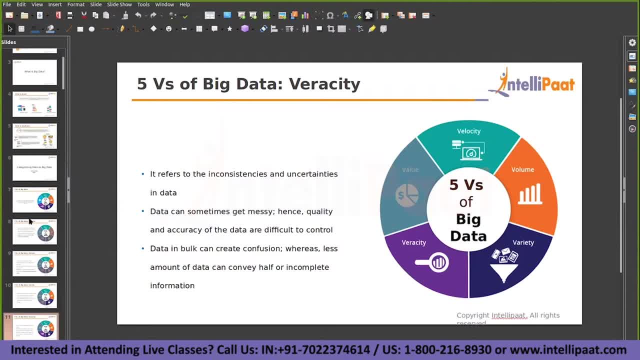 what my- uh, most important thing see when i'm getting the data in a so-and-so file. if i have to store that data in a so-and-so table, i should be creating an id column with some primary key element and that's what my identifier i can say, right? so when i dump, 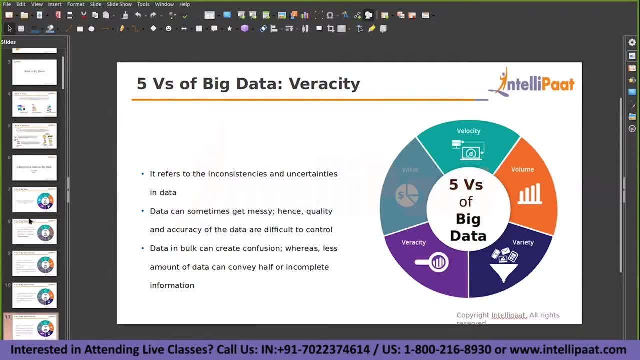 these 10 million records into the so-and-so table. it's gonna fail because some of the records have null as an id. you cannot definitely have a null as an id, right? it's not. it's not even pointing to any uh user, so that itself is a dummy record, right. so these are some of the examples that i'm saying. 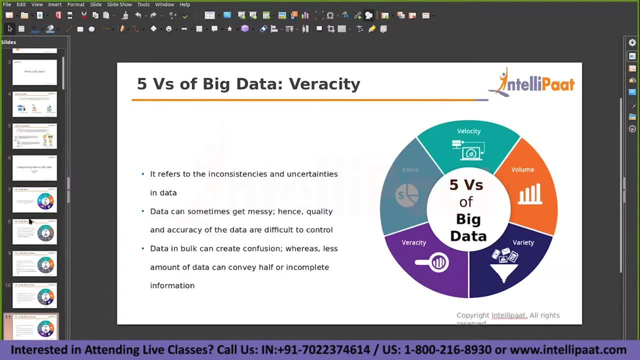 duplication is one, uh, null records are some one and, uh, some of the records does not even exist or does not even come from this specific source. so you have to do this: data validation or data filtering or data deduplication. so all this terminology we are going to use- 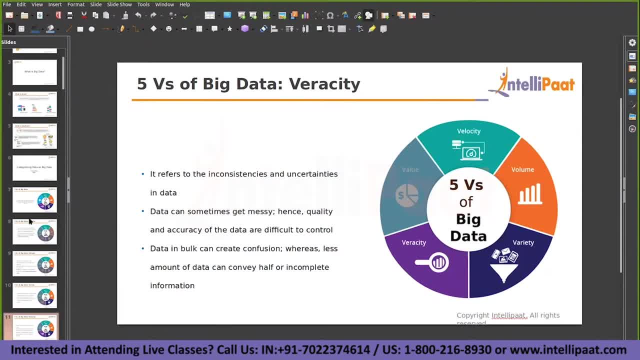 in real-time scenarios. so you have to first make the data accurate and then store it right. so all these things come under this veracity component. so make the data trustworthy, make the data accurate and all the procedures that you're going to do prior to giving it some kind. 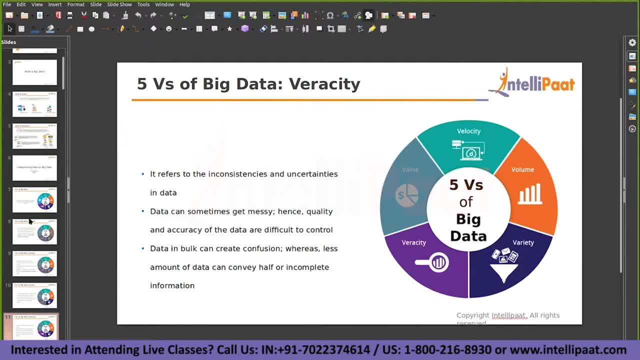 of a story is what this activities is going to talk about, right? so veracity is pretty much the trustworthiness of the data, how much you can trust it, or what, what tools, or what tools you can do to filter the data, remove all the unwanted records, or pretty much make it accurate. 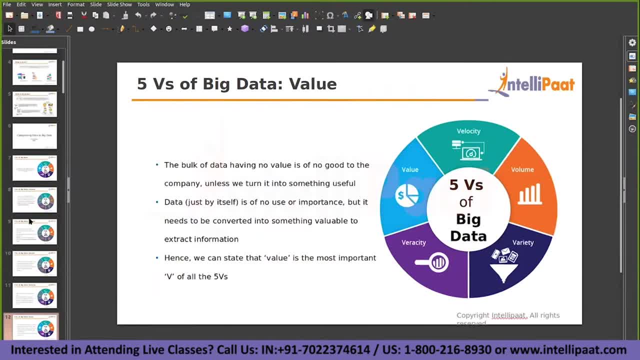 okay. and then the value. what do you mean by value? okay, i'm loading some petabytes of data. two petabytes of data data, three petabytes of data. i'm loading the unstructured data- great. i'm loading the data which is coming at so and so speed. that's very great. but what am i doing with that data? what is? 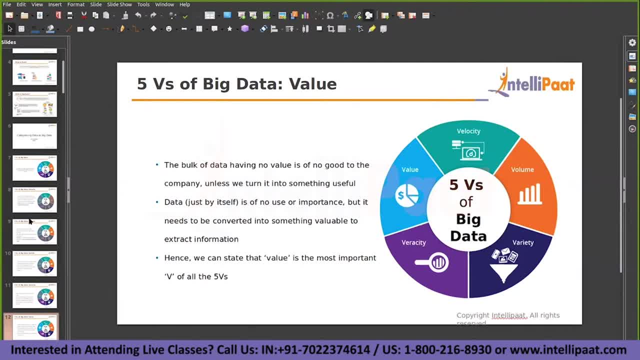 the need for you to store that data. so ultimately- for example, you are working for an organization- you extracted the data from so and so source, you loaded it into a table you, you designed it, you filtered it, you transformed it into a so and so nice table. what is the use of that table? let's say 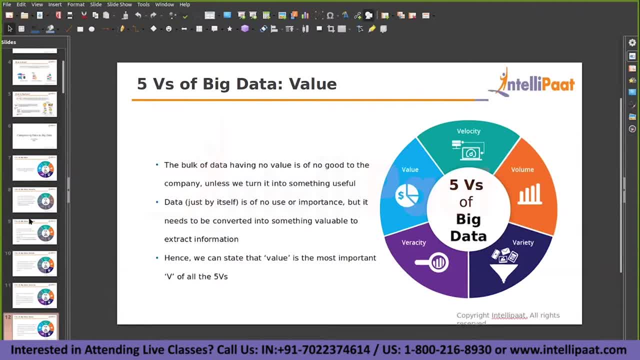 now. so if that is not giving you some amount of value for the company, what is the need for you to store that data right? so, ultimately, any data that you capture, or any data that you store, has to give some value to the company. amazon is capturing the data of a user. what is the value? 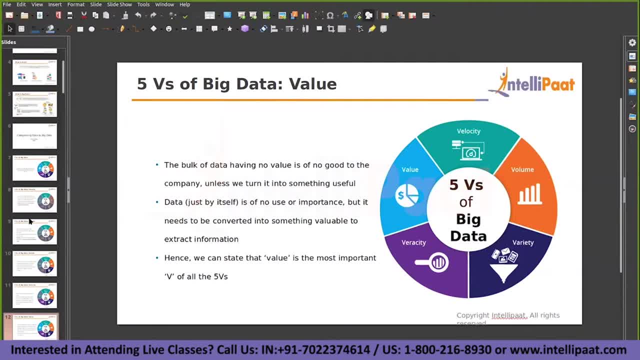 that it is generating you. it has got a large amounts of user base. what is it doing? i don't, we don't know what it is actually doing, but it's it's earning a lot of money with your data, right or better example: facebook, how many of you see in the uh discussion with uh- i mean uh, this is mark has attended some discussion. 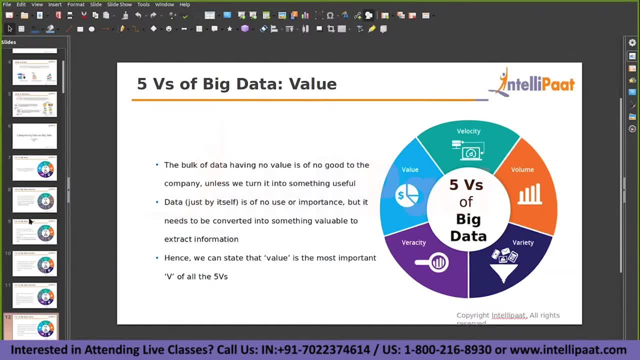 with the uh us consulate? right, it's a. it's a very nice interview actually, right. so what are they doing with that data? of course, in in simple terms, they are giving you a better user experience. it's a. it's a very nice interview actually, right. so what are they doing with that data? 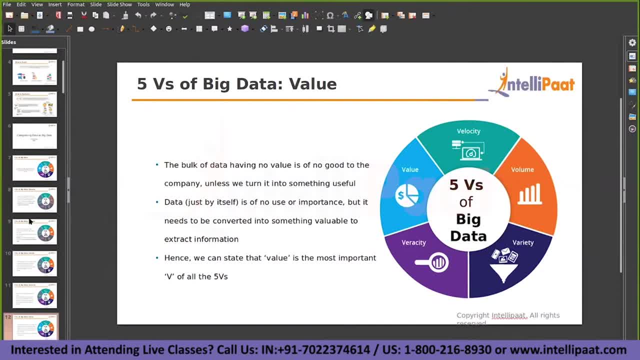 it's giving you, uh, search records, it's giving you the suggestions it's giving you it's keeping the track of all your order history. uh, they're, they're trying to build you a better user experience. okay, let's talk all about the positives. so they're trying to build you a better user experience. 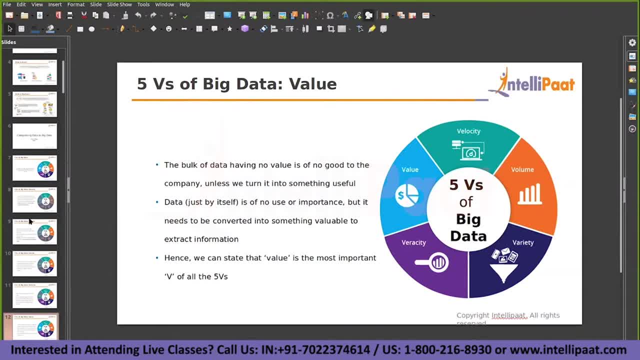 okay, they are trying to capture the data and they're trying to help you build a proper user experience. so that is one value that you are generating out of the data that they are storing, right? so, similarly, a similar example, like you can say, so, every company are when, when you are dealing with such large amounts of data sets, ultimately they have to. 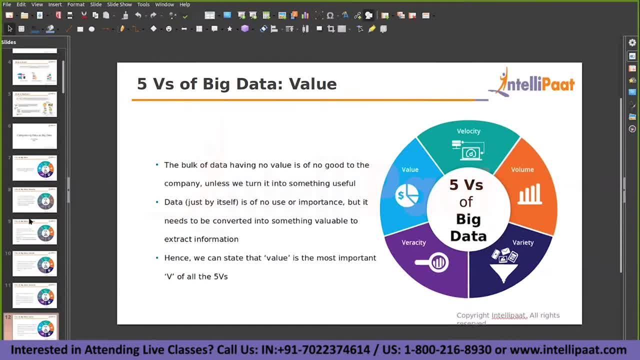 turn into some kind of a value. if they don't have a value, there is no use in storing such amounts of data sets. so the major characteristics for any data it can be- i mean need not be a big data, it's going to be a major characteristics, is it? should it should tune into a so and so value. 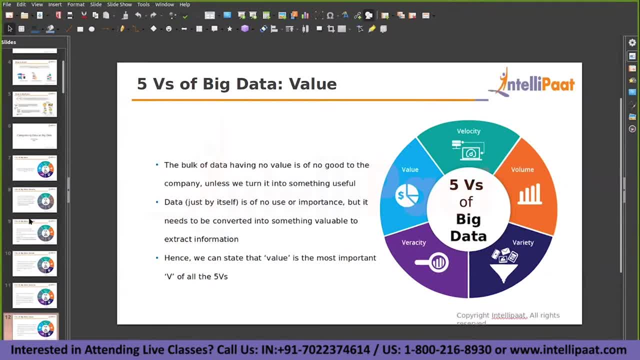 some, some recognized value for the company, some useful information for the company, right? so that is the most important characteristic of a company, right? so that is the most important characteristic of any data that you're going to store, agree? are we clear with the five v's now? 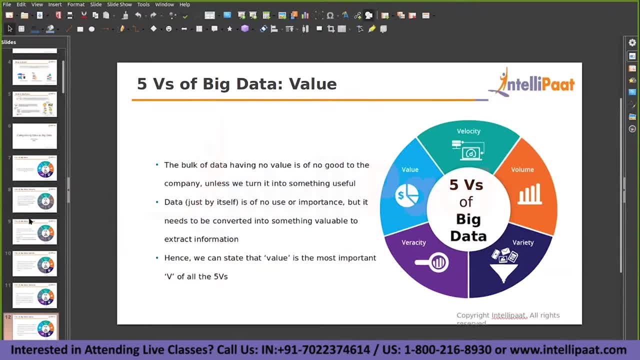 any questions? so we are not, we are not, we have not got into the technical related stuff, all this right. so it's it's only theoretical. it's kind of a nice story that we are discussing, okay. so nothing technical, it's very generic, very basic. so any questions do we have? shall we continue? 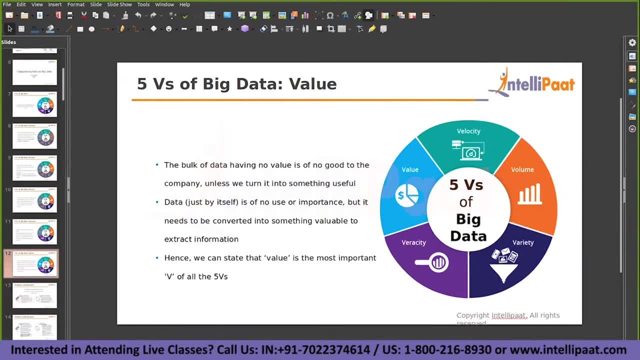 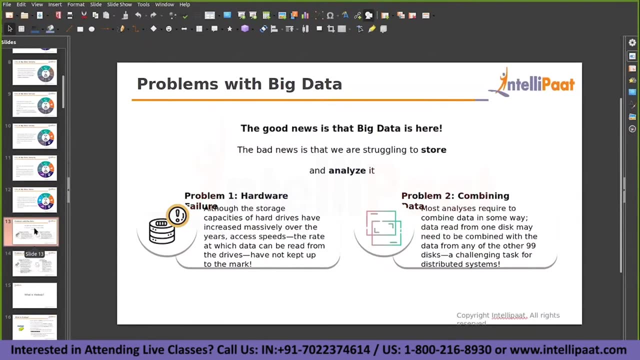 no, fine, right, so we are getting into the concepts slowly. so we have discussed about the characteristics. we have seen what, uh, what are the characteristics, uh for it, uh, for a data should have, i mean, whatever the data that we are able to store, it should have so and so characteristics. 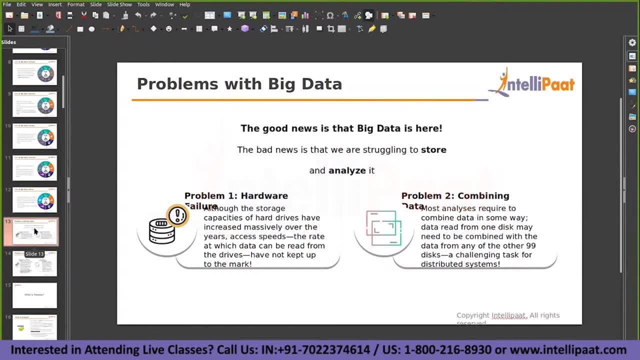 for it to term it as a big data. now, what are the problems that we are gonna face with with such, uh, kind of data sets? so we've already seen the problem with the storage, we've already seen the problem with the speed, uh, or the different types. right, so they are, they are the need. okay, i can say that's, that's. 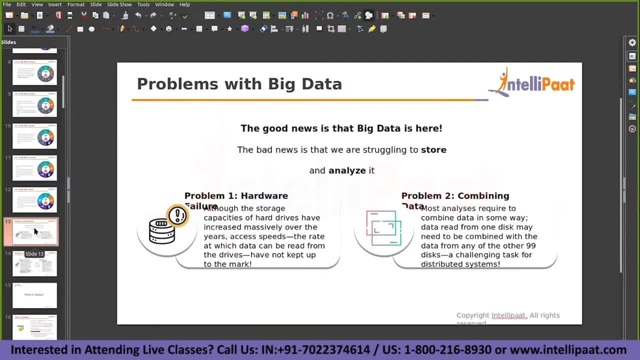 a pretty much the need for your uh new platform. so they should definitely have storage, they should definitely have speed, they should definitely have the uh uh capability to store any of the data and all that right. so the categorization of problems with b2b and b2b are very different from the. 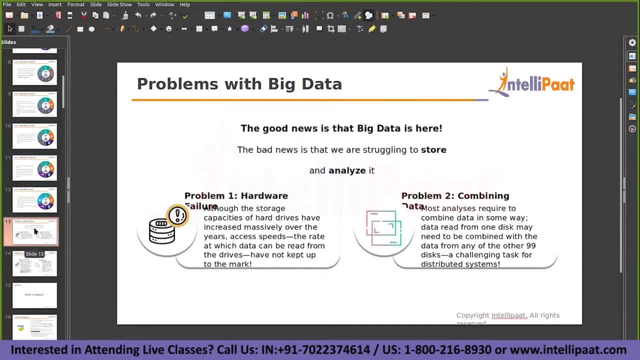 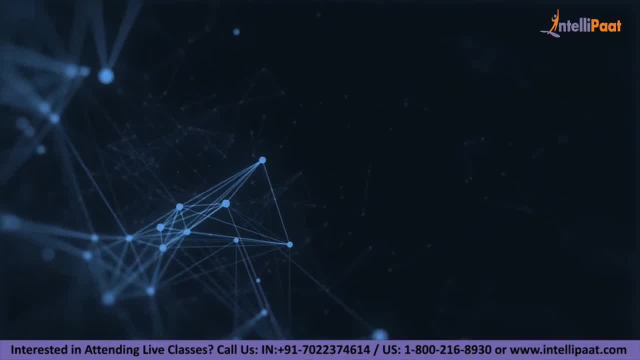 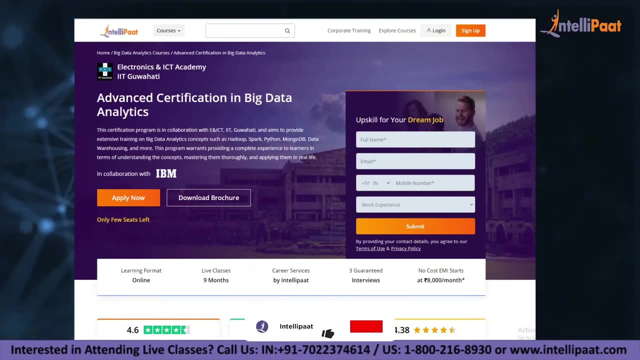 previous ones, we have seen that all of the data is being stored over the region. so that means we went from the content, which is what should be stored over the region, to what should be stored over the region, by which the data is stored by. so we have to think about what are the 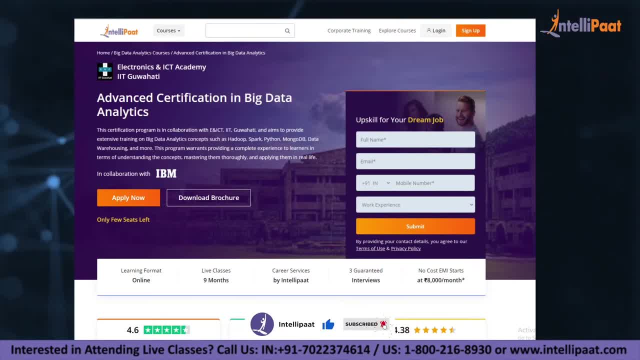 possibilities for the medium, which here is the computer software or the software, and then we give a picture. so if we have a uhh, if we have a data set, we have to. yes, we have tos and your dream job. now let's continue with the session. so, ultimately, the problem is with the storage and 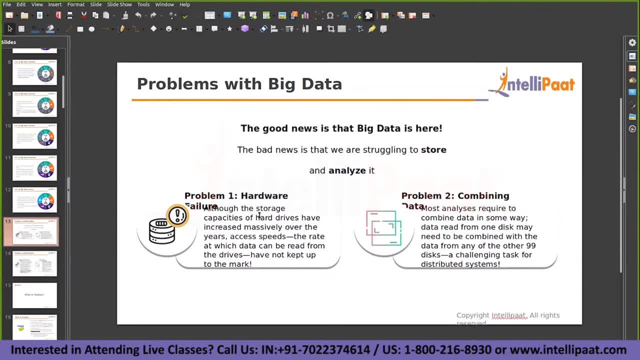 with analysis part. okay, so just to name it. so, although the storage capability capacities of hard drives have increased massively over the years, access speeds, the rate at which the data can be read from the drives, have not kept up to the mark. agree so earlier when, when we were 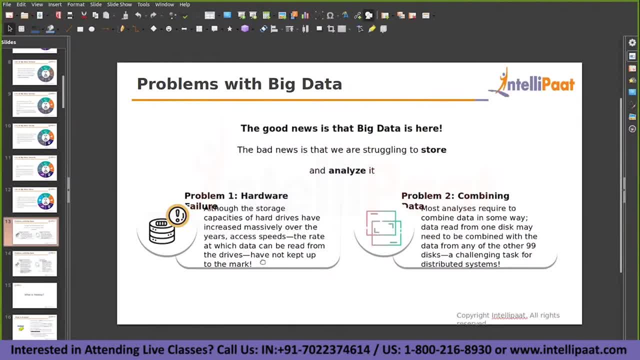 i mean 10 years back, let's say, there were systems with 250 gb, 500 gb. now we have systems with one terabyte hard disk, right? so the hard disk storage has definitely increased. i can say: right, we have already seen that. so the size of the data that you can store is kind of increasing, and you also 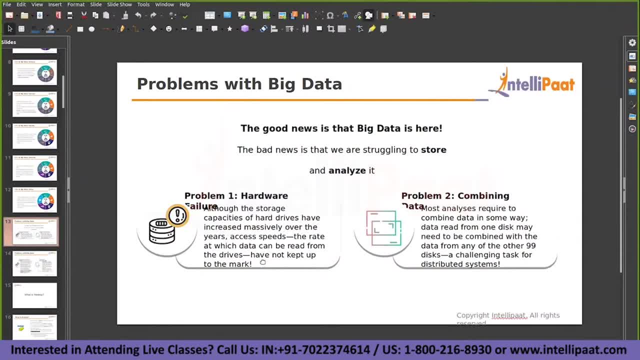 have the hardware problems that i mean you. you, you are having the necessary hardware to to store the data, but the problem is with the speed with which you access. so, in general, for example, which example do we have to take? not get into the technicals of it. okay, fine, let's, let's, let's get. 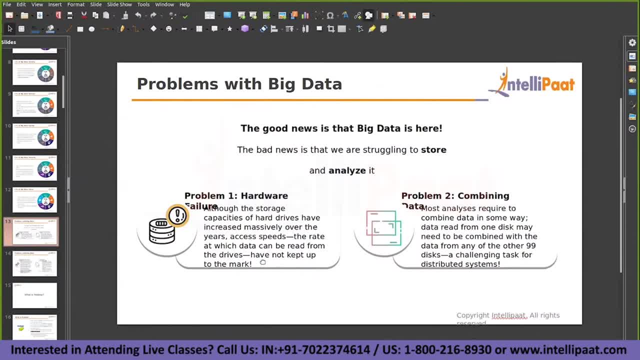 into the details of it a little later, but in simple terms, see, uh, it's definitely gonna take some time for you to store the data and for you to read the data from a specific hard disk. so how many of you have seen this memory uh processing in memory processing? how many of you heard about this in memory processing term? 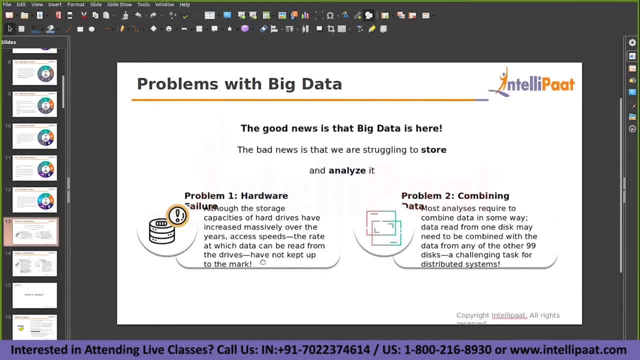 it's very early to use this term, but that's okay. okay, um, have you guys used uh, the uh- transfer of data between one system to the other system, from one hard disk to the other hard disk? how much time is it gonna take? let's say you're you're having some storage in a hard disk. 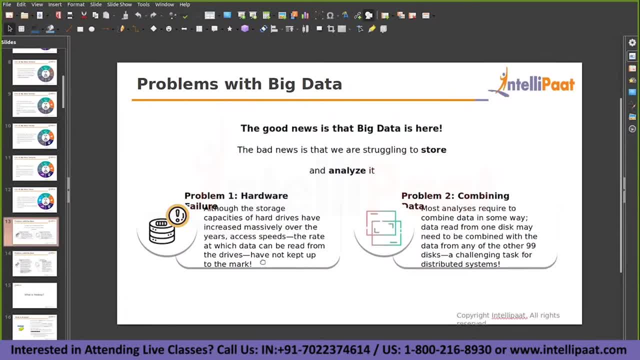 okay, external hard disk. you're trying to transfer everything into your local machine, right? this is one scenario, and the other scenario is you have some data within the d drive and you're transferring the data to a different folder in the d drive. which one is going to be faster within the within? 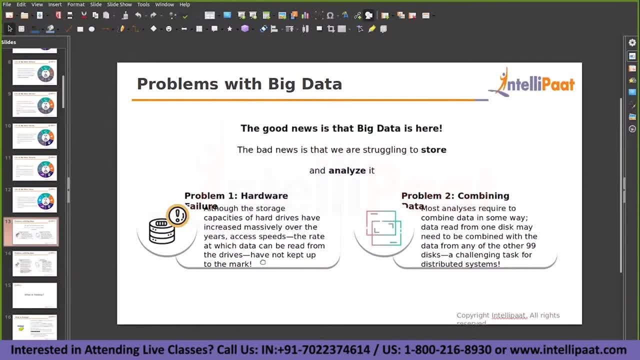 the local machine. okay, so this is not a proper example, but a very known example i can say: right, but when you are accessing the external hard disk, you, your transfer rate has been reduced drastically. right, so you, it definitely takes some time for you to read the data from an. 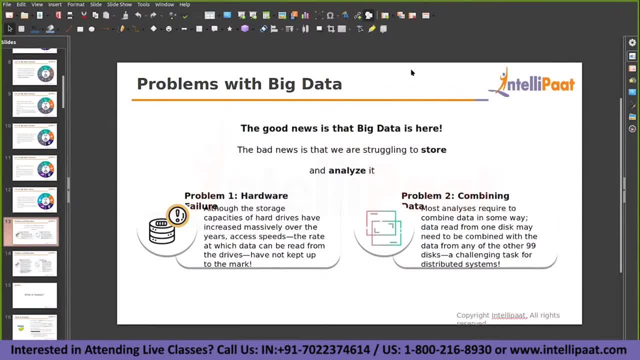 external hard disk. so that is what the problem is. so when you have the data on a hard disk, when you have the data on a, on a storage, uh, the time taken for you to read the data or even write the data into that hard disk case is kind of a problem. now, right, so you, you have a storage. fine, that's fine. 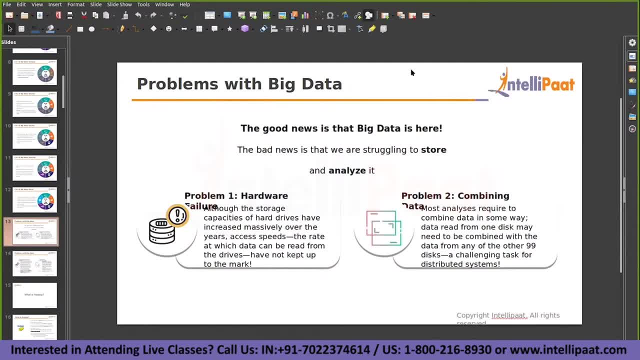 you have one terabytes of hard disk, you have two terabytes, you have three terabytes of hard disk. storage is available, but the problem is with with the read and write space. right, so you, you can just speeds, right, so you're not able to store the data with a with a faster rate and, moreover, you're not. 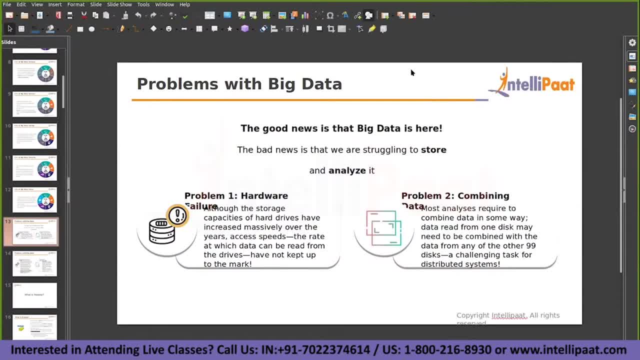 able to store everything in a single data in a single machine, let's say, right, it has to be across different machines. so that is one problem. and combining data. so what do you mean by combining this data? so most analysis requires to combining data in some way. data read from one disk may need. 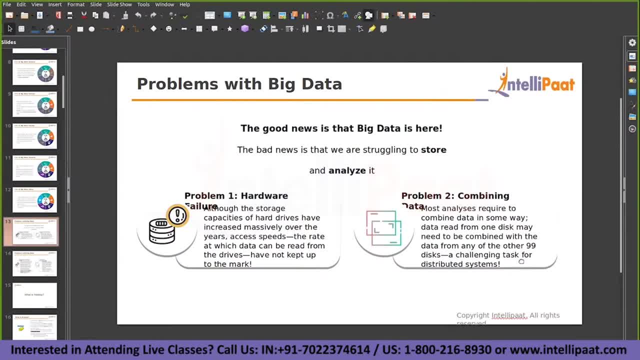 to be combined with the data from an any other 99 disks, challenging task for the distributed systems. so, as we have come across the term distributed system, so how many of you know what is a distributed system? so, uh, in the previous problem that i was discussing about, i was, i was telling. 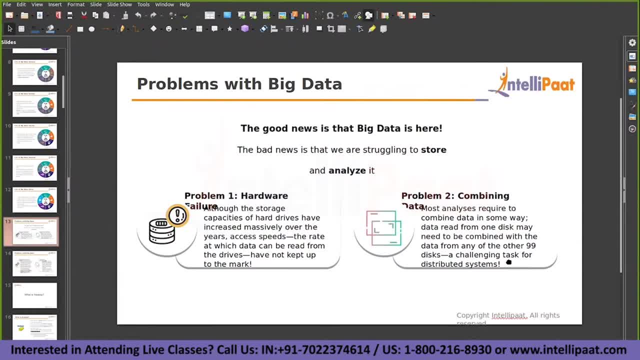 that the storage problem problem has been solved. okay, so we have the uh capability of the hard disks that they are increasing. right, the size of the hard disk is being increased and we don't have a problem with the storage now. but but the problem is with the data write and read speeds. so why am 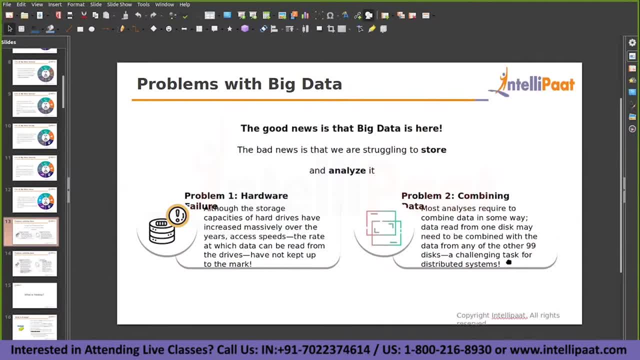 i saying is saying that is, we have a, we have a hard disk of one terabyte. now, okay, so, for example, if i, if i have a data which has to be uh, which, which, with the store which has, with the size of three terabytes, let's say what i'll do. i'll take three machines with one terabyte each and i'll divide my three. 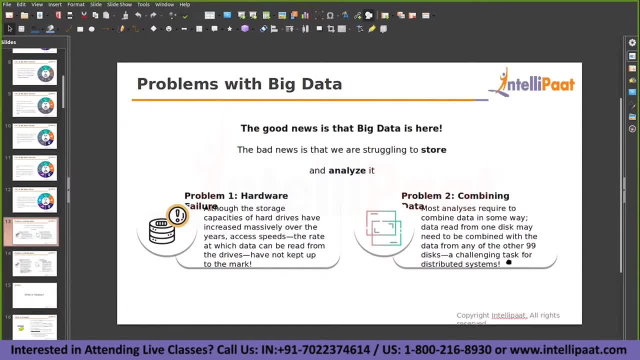 terabytes of data into these three different machines. that is my distributed storage, instead of storing the entire data on single machine, which is not possible. what am i doing? i'm dividing the data into multiple chunks of data and i'm storing it on different, different machines, right? so what i'll do if i get four? 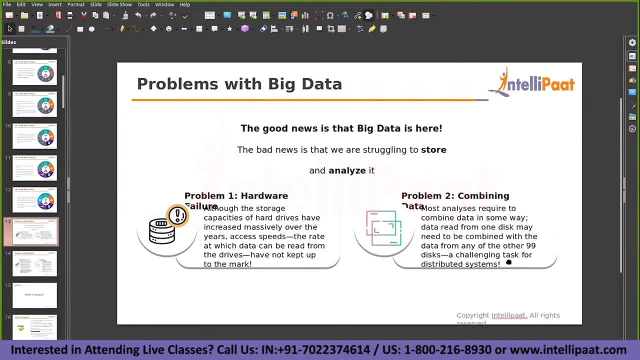 terabytes of data. next time i'll add one more machine. if i get five terabytes of data, i'll add one more machine to it. so what am i doing? i'm just increasing the number of machines in the network. what do we call this? we call this as a cluster. 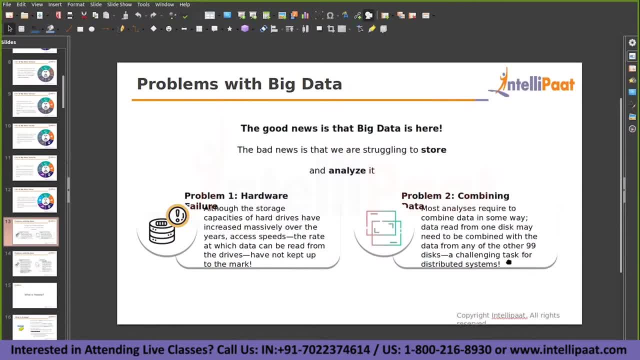 so what do you mean by a cluster? when two or more- no more number- of machines are integrated in a in a specific network, let's say, okay, so both are connected to each other. when two machines are connected to each other, or when two or more machines are connected to each other. 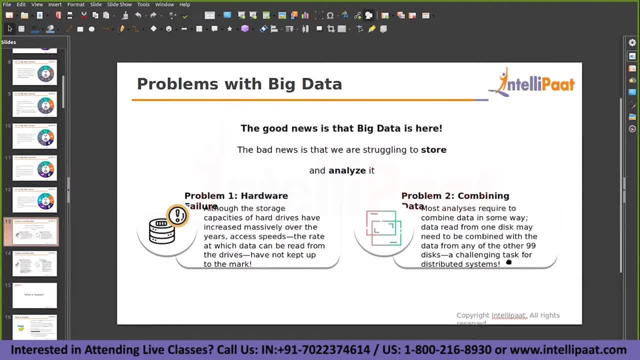 we call that as a cluster. okay, so when i when i have five terabytes of data to be stored, it's not possible for you to store the entire data in a single machine. you cannot, you cannot have a hard disk which is of five terabytes alone, right? so you will find hard disks which are 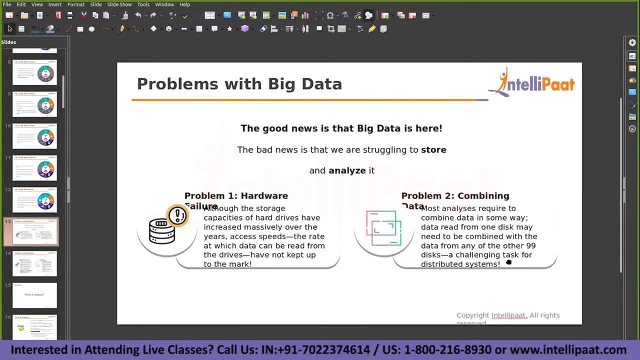 5, 1 terabytes or 2 terabytes. what do you do you? you purchase different hard disks, you integrate them on a network, right? you put them on a same network, you connect with them with each other and you distribute the data of five terabytes on this network. so now i have five. 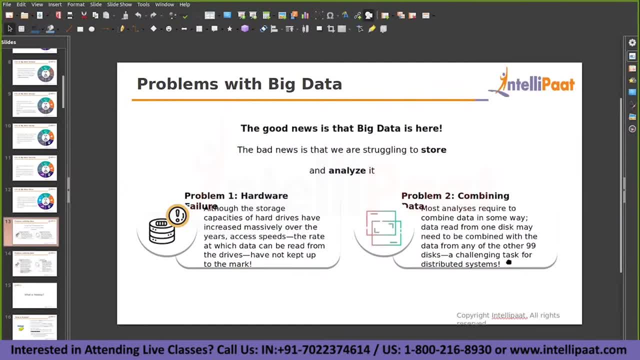 machines with one terabyte each. i can store five terabytes okay data. tomorrow i get two more terabytes, i'll add two more machines to the network. so whenever my size of the data is increasing, whenever i am running out of storage, i'll keep on adding. 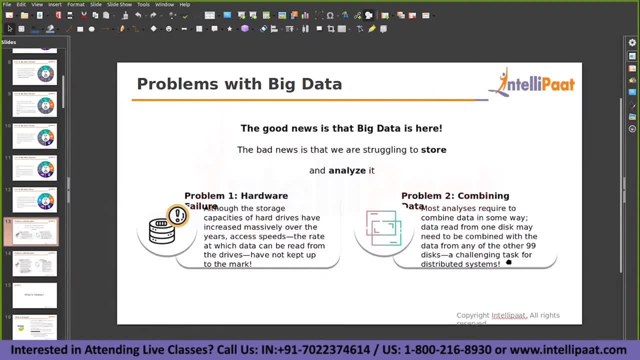 new networks, new machines to the network. are we clear with this right? so this is my distributed storage. so that is the reason why i said the storage is not a problem now, but the rate at which the speed at which your data is being transferred from one machine to 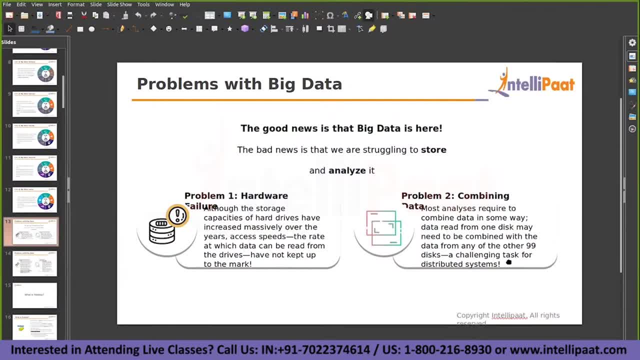 the other machine, or the speed at which you can read the data from the network and write the data to the network is is kind of becoming a problem. so that is the reason why the second problem has come, the combining data. what do you have to do? let's say, let's take this example, we have the 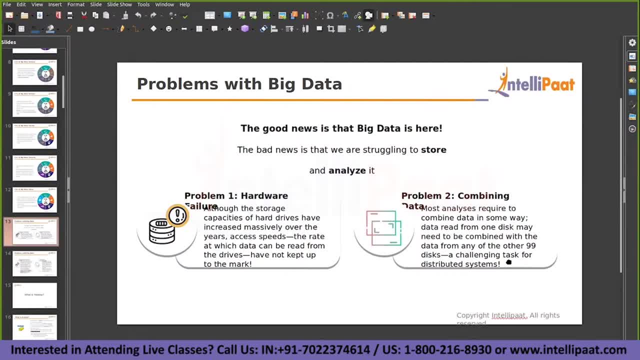 voters list from five districts. let's say, okay, right, we have the voters output and whatever the votes they have pulled, we have the results from five different districts, right? so, on the whole, it is around 10 terabytes of storage. okay, whatever the data i received is, 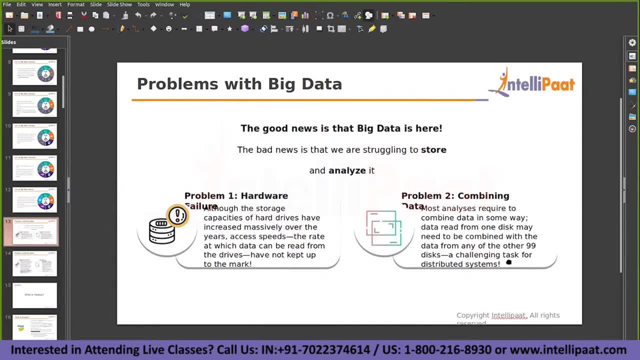 around 10 terabytes, which consists of all the five districts related information. so now when i'm distributing the data across uh 10 machines, i'm distributed this so and so number of records into 10 different machines. so now when i have to calculate the winner, i mean if i have to 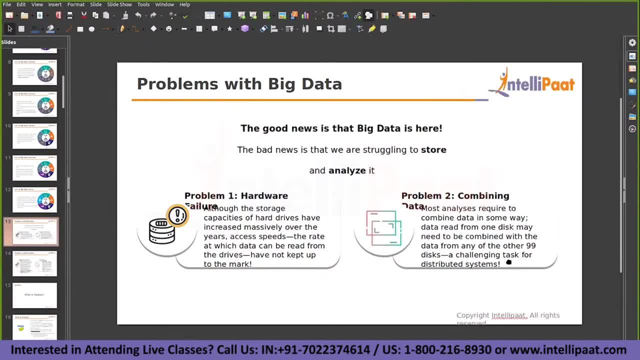 calculate the number of votes polled for each and every party. let's say i've got three parties right. so, for example, if i have to calculate it, what do i have to do? i have to read through each and every machine, read through each and every district, so which district have received which number of how? 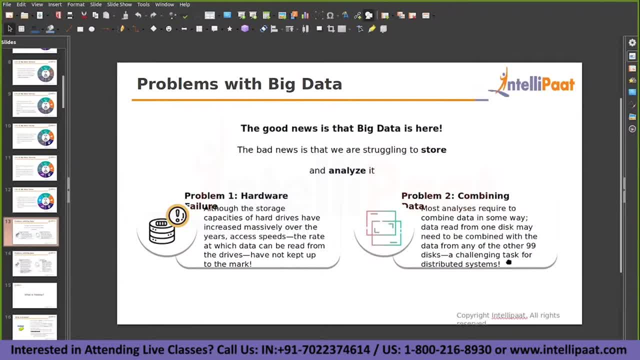 many number of votes and how many number of votes have been pulled for each, and number each and every party. three parties were there. five districts were there. so you just have to segregate the data on each and every machine, then go to another machine, then go to another machine, extract the. 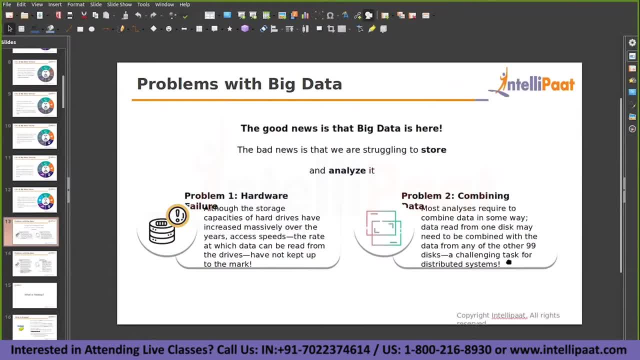 data, and then you have to combine the data and find the final output. this is what i have to do, but how challenging is it? that is what the problem is right. so when i am, when i'm i'm, i'm not having a problem with the storage. now, with the help of the distributed network, i'm able to store the data, but 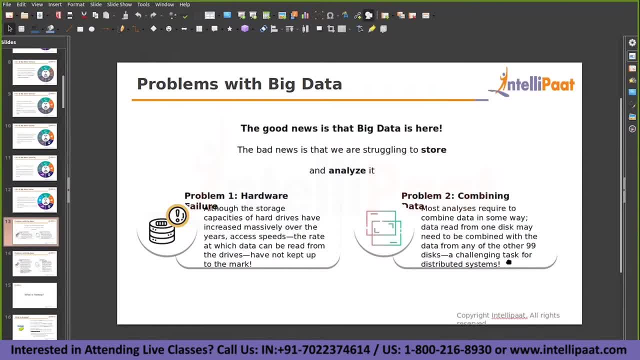 how do you combine the data from one machine to the other machine? that is what the problem is. if i have to do this use case, what i'll do? i'll collect the information from all the five machines query on top of it. i am, i have written some program, i've run some. uh, i'll run the program. 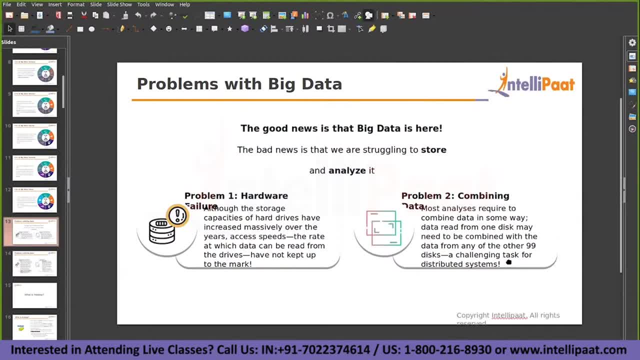 on that data, extract the output and then store the data back to the existing machines. so this is what i'm gonna do. that is what the problem is right. so it's taking a lot of time for you to read the data from the machines and write the data to the machines. the read- write time is what 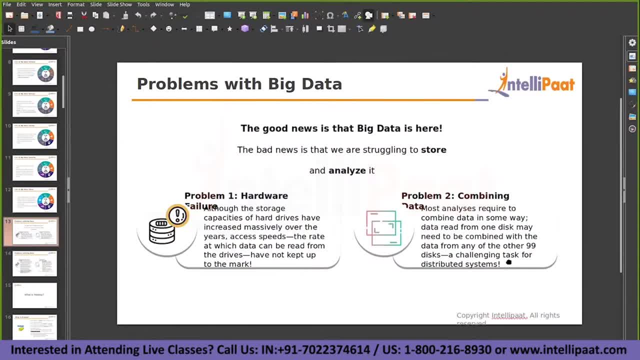 taking the uh time right so as, as we have solved one problem, it has it has brought us into another problem, as we have solved the problem of storage. okay, let's say i'm, i'm using this distributed thing, but what it is it? what is it doing when you have data, when you have the same file on different? 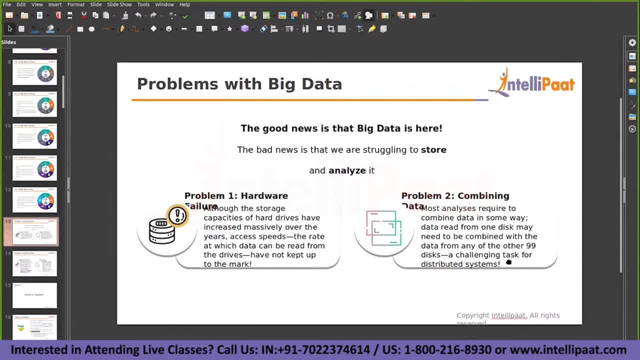 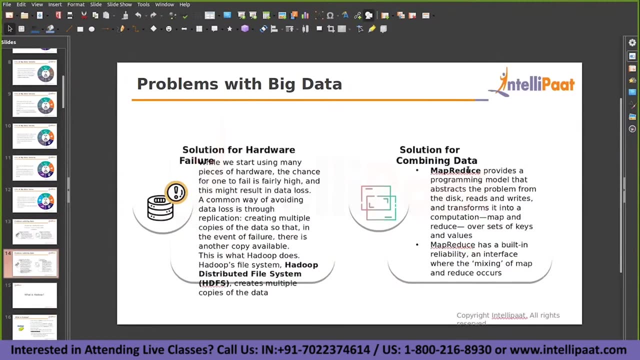 different machines, which is which is broken into different machines. then you have to combine the data to do some processing that that's going to take some time. agree with the uh challenges. do you have any questions? are we deviating anything? so let's go back to the uh solutions, whatever the 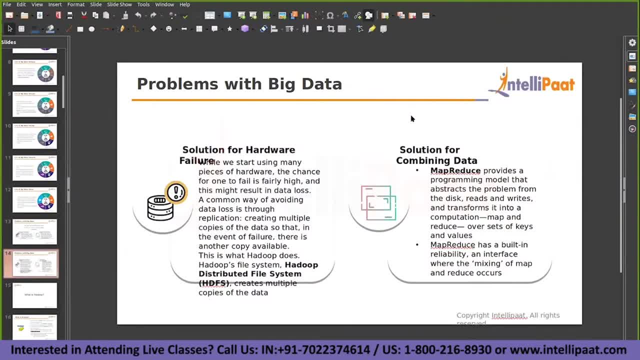 uh, problems. have we discussed what are the solutions we are gonna have? so the first thing: while we start using many pieces of hardware, the chance for one to fail is fairly high and this might result in a data loss. a common way of avoiding data loss is through replication. 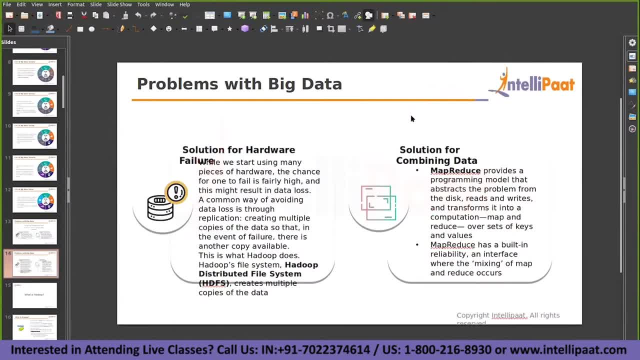 creating multiple copies of data so that in the event of failure, there is another copy available. so this, ultimately, is coming to a solution named hadoop- distributed file system, which is called as HDFS. most of them call it HDFC, but it's not HDFC. we are more used to the HDFC term. 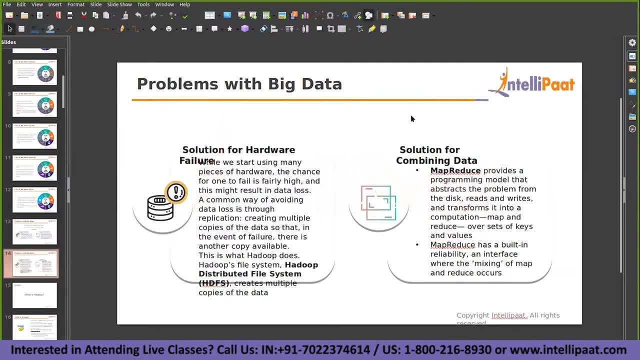 but it's going to be a HDFS. even now i still hear people saying HDFC, but that's kind of funny, but it is. it is going to be HDFS. right, hadoop, distributed file system. so we discussed about the storage problem right the first in in the previous slide. what is the problem that we had? what is the? 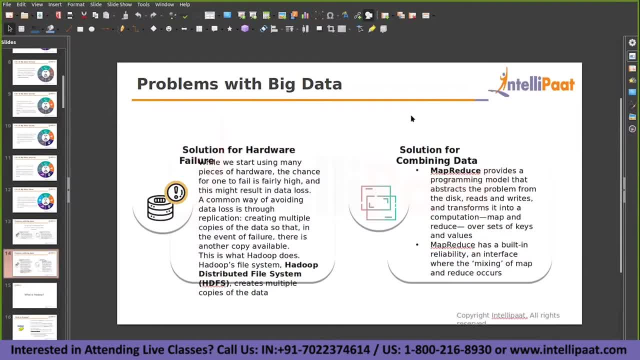 what is at least the solution that we gave? we were storing the data in different machines right in a network, so like five terabytes of data which is being distributed across five different machines. but in that case, what are the problems? it can have one simple problem which i can identify now, at this moment. 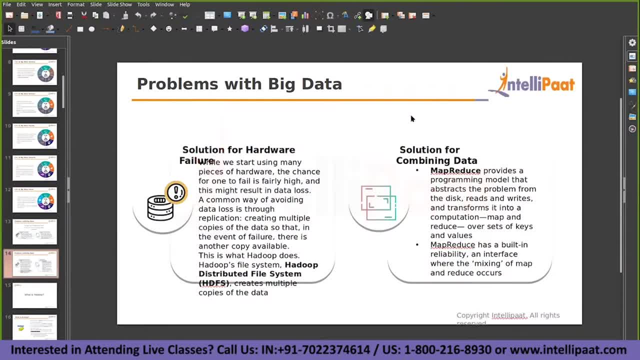 so there are other problems also, but one simple problem which we have identified in this case is is loss of data. if one machine is lost, what happens to the data on it? the entire data of one terabyte is lost, right? so what are we doing with hdfs? in hdfs there is a, there is a concept. 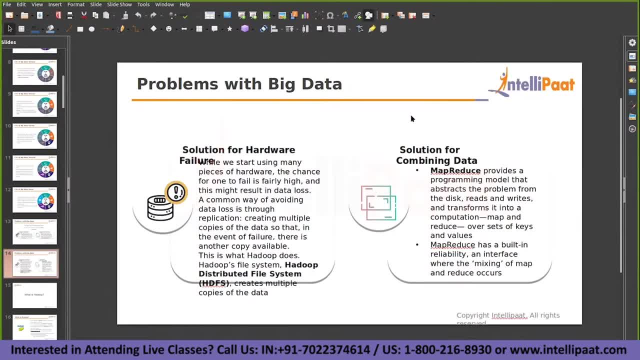 called as replication- replication factor. what does this do is every data that you store in a machine, every block of data, i can say every block of data that you store in a machine is duplicated and and stored in other machine also. that means five terabytes has been divided. 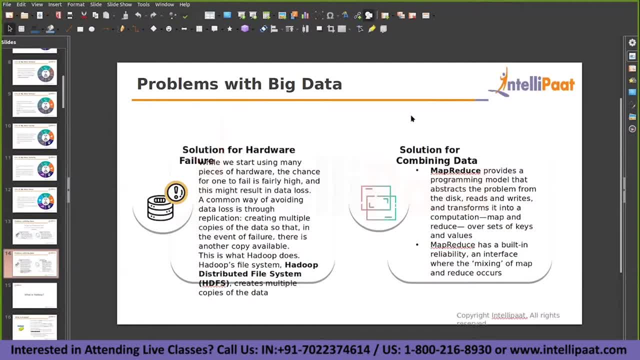 into five different machines. every machine will have some blocks of data inside it, so one terabyte will be broken into multiple, multiple, small blocks of data, small boxes of data. so each block of data, when you are storing it in one machine, you will duplicate it and store it in another machine. 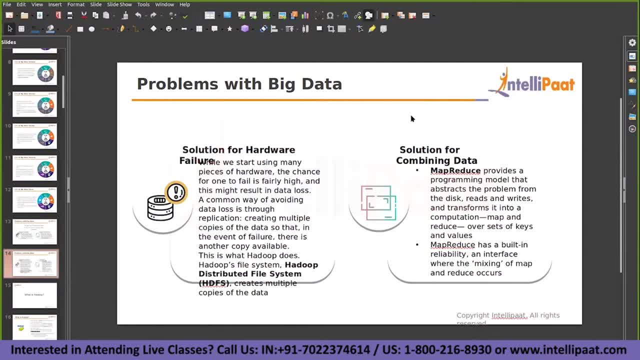 so the the. the question is how many times you will be duplicating that. for any single human storage case that you are storing, essentially likerás, there is a provision for you to duplicate it once, or you can also duplicate it twice. that means the first scenario is you. 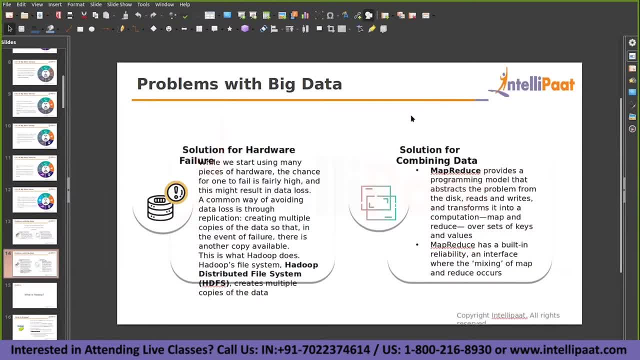 will not maintain any duplicates. the second scenario is you will maintain one duplicate property and the third scenario is you are maintaining two duplicates of it. in the first scenario, if i'm having five terabytes of data, you're only using five terabytes of data, five terabytes of storage. 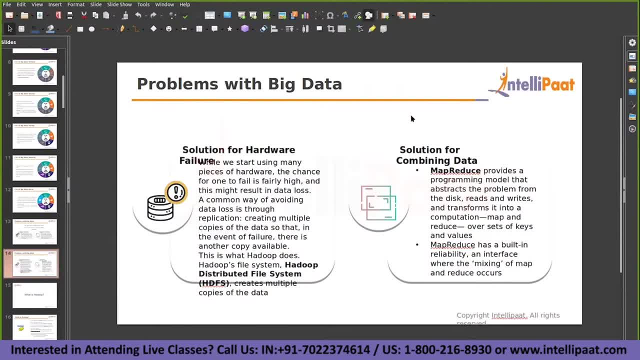 15 terabytes of storage. agree with this point, because you're duplicating it, you're, you're triplicating it. i mean you're, you're, you're maintaining three copies of same data. in the second scenario, you're maintaining two copies of same data. in the first scenario, you are not. 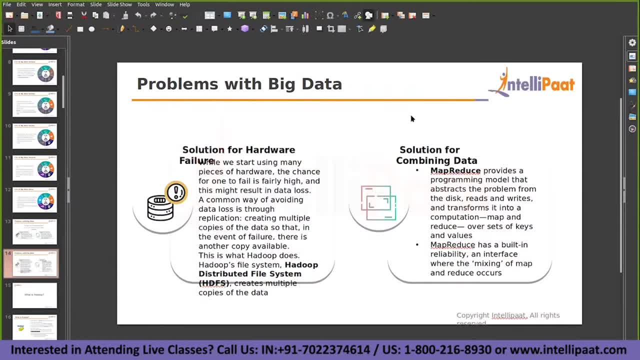 maintaining any copy right. so this is what your replication is going to tell you. in hadoop hdfs scenarios, the replication factor can be one, two or three. if there is one. if you set the parameter as one, that means it won't maintain any duplicates. if you set the parameter to two, it will maintain. 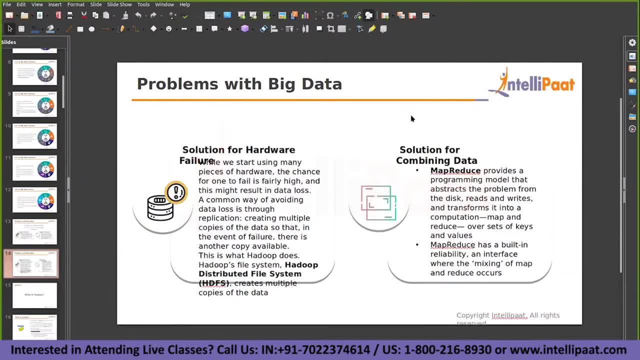 two copies of it. if you set the parameter to three, you will maintain three copies of it. so by doing this, as you have the same data available on some other machine, also in one machine or in two machines, okay, if it is two machines it is more secure. so let's say, if it is stored in one more, 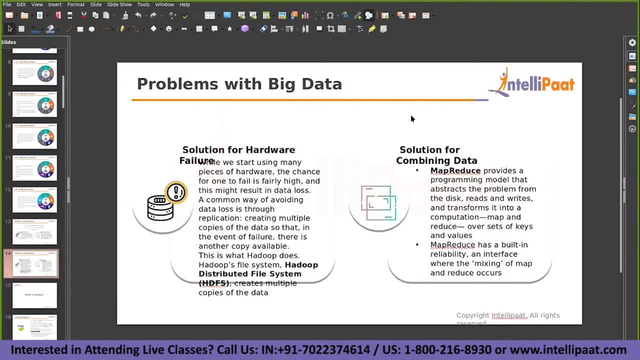 machine. even if this machine is lost, you still can retrieve the same data from the other machine, agree, right so if the replication factor is three, let's say, if you have lost it in one machine, if you have lost it in two machines also, you still have it in the third machine. it's more secure, right so? but 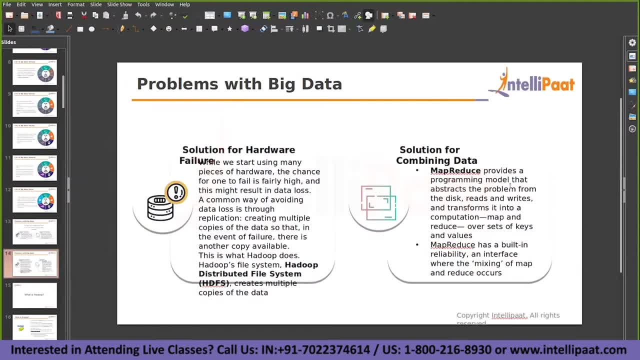 ultimately, what are we compromising on? we are getting safety. that's fine, but what are we compromising on? we are compromising on the storage right. so, instead of using only five terabytes of storage, we are now using 10 terabytes of storage for the same five terabyte of file. 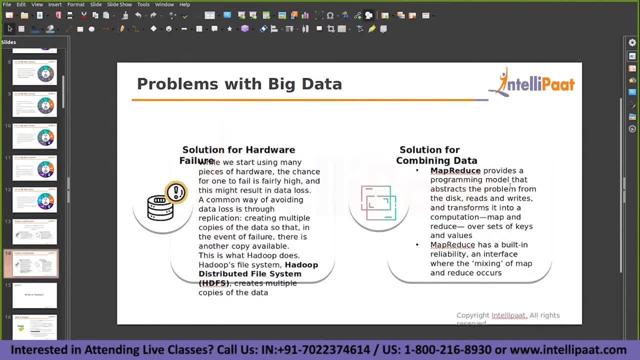 we are now using 15 terabytes of storage for the same five terabyte file. that means we are using more storage than what we actually need. but what are we getting? we are getting the security. we are getting the fault tolerance. that's what the term we are going to use. 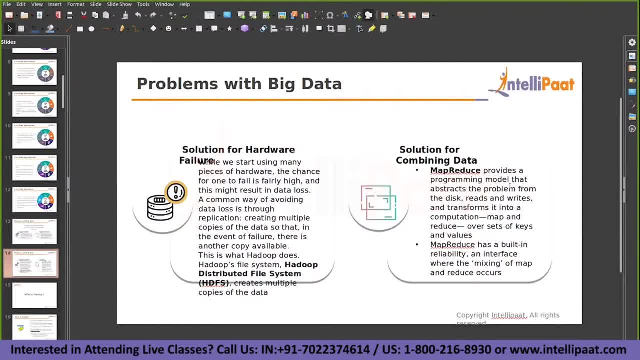 even though the machines are lost in the network, we still have the capability of retrieving it. we still don't have any problem of losing the data, losing the actual data. so now, if you look at, we've actually out the storage related thing. so now there is no problem at all with the 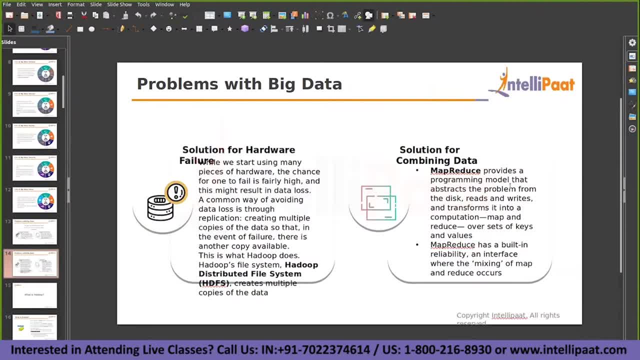 storage. I can use any amount of storage I can. I can generate any amount of storage. now I am more focusing on the security of the data. right, so that is what my HDFS is gonna give it's. it has taken the storage out of picture. it is. 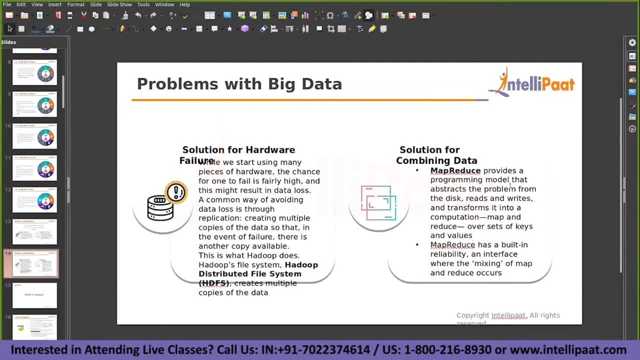 more concentrating on the the quality of the data or the fault tolerance of the data. right? so that's what the challenge I mean. that's that's what your solution is gonna be. so all your storage related solution of problems will have one single solution. that will be HDFS, Hadoop, distributed file system. so that's not it. 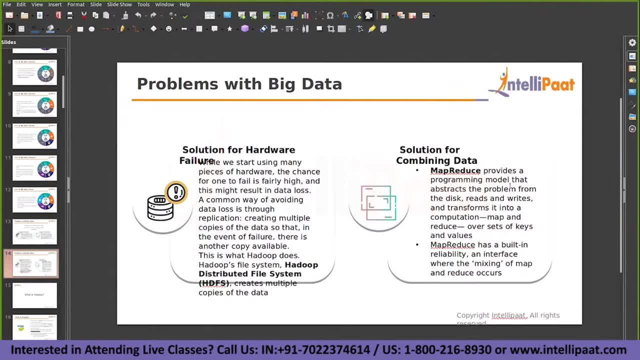 guys, there are. there are other features also for HDFS. we will get into the details. this is just to show you some kind of introduction. I can say: okay, so this is one of the feature that we have in HDFS. okay, so all your storage related problems, whatever the problems that we have, 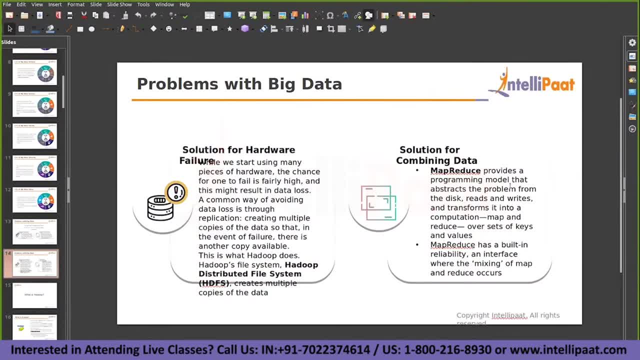 discussed in this video is all about storage related problems that we have about in terms of storing the data, storing the huge amounts of data, losing the data when you have data across multiple machines. everything will be solved in your HDFS related components. now, coming to the MapReduce, what do we have? there is some problem with the combining of the data. 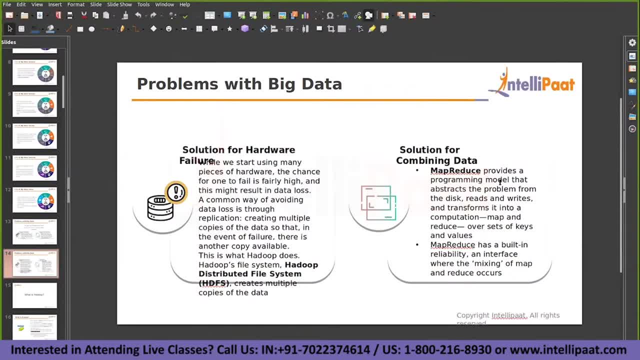 that we discussed right. so it provides a programming model that abstracts a problem from the disks, reads and writes and transforms it into a computation map and reduce over set of key values. map reduce has a built-in reliability and interface where the mixing of map and reduce occurs. okay, so there is a lot of technical terms in it. so, in simple, 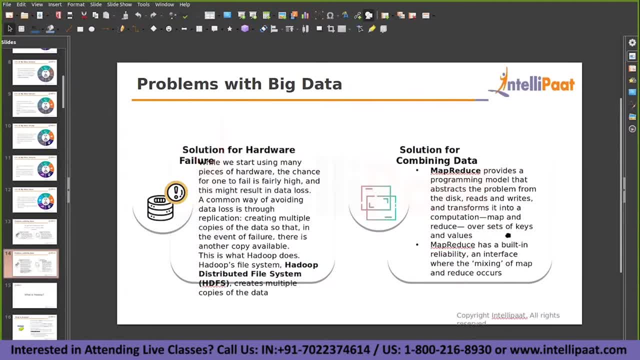 terms. i'll tell you this. so what is the actual problem that we had? we were having problem with the data that is residing on different machines. the same data. you have it on multiple machines now, right. so when you have to combine, you have to extract the data from the machine. 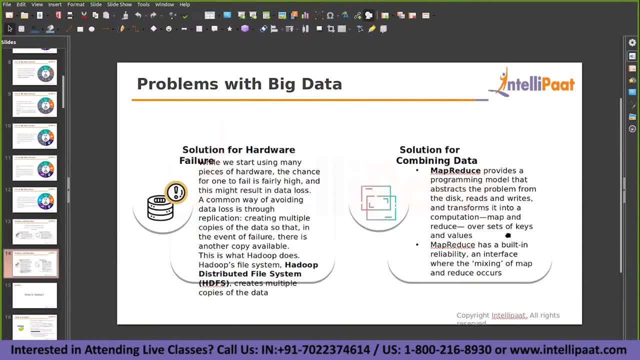 combine it, do a computation, do whatever the outer calculation and you generate the results and store it back to the nodes, to the machines. so what MapReduce has done here is you're not moving the data anymore. the data is gonna sit wherever it is. what you will do is you will 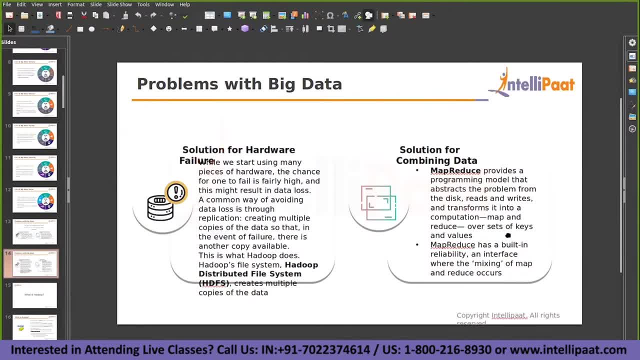 move your computation logic. so earlier, what did i do? i have written one program. so you gathered all the data from five different machines. you gathered all the five terabytes of data. you ran that program on that five terabytes of data, you extracted the output and then you distributed the data again to those five machines. but now what i'm doing is: 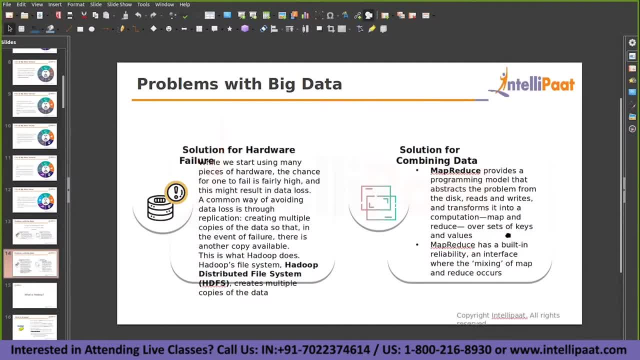 i'm not gathering the data from any machine here. the five terabytes of data- one terabyte of data on each machine- will sit wherever it is, but instead i'll move my program, whatever the code that i've written, i'll duplicate this program and i'll submit this program to five different 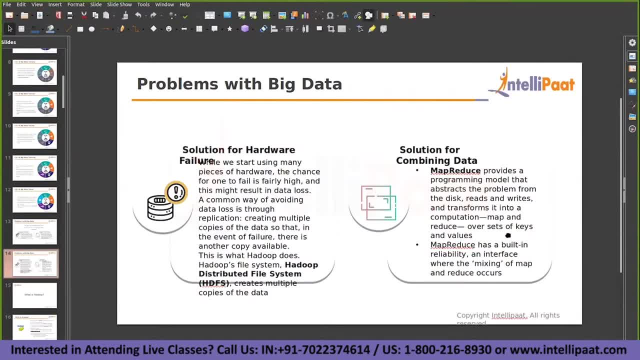 machines individually. that means the computation is happening inside the machine where the data is actually residing. you're not moving the data anywhere. the program itself is moving to the data. data is not coming to your code. code is coming to your data, agree, that's a difference. so the 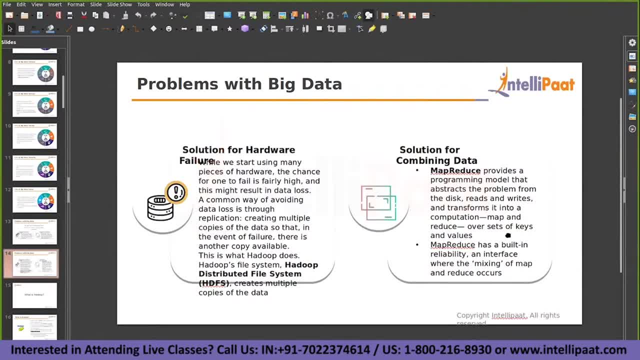 computation has been moved to the data location. you do all the transformations or computations, whatever you have. you extract the result, only the result, right? instead of extracting the entire one terabyte of data, you're only extracting the result of that one terabyte data of data. it's hardly going to be in kbs, right? so you extract the data, you result from all the five. 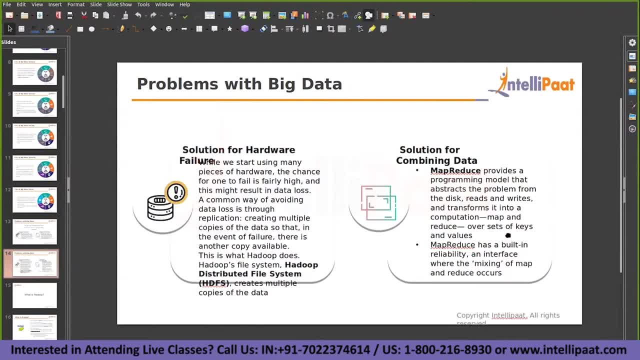 machines and you combine the result and generate one final output. so how you're going to do that, how effectively you're going to do that, what are the different processes involved in it? we will discuss that later, but have you understood the core concept of it? so, instead of moving the data from the storage, 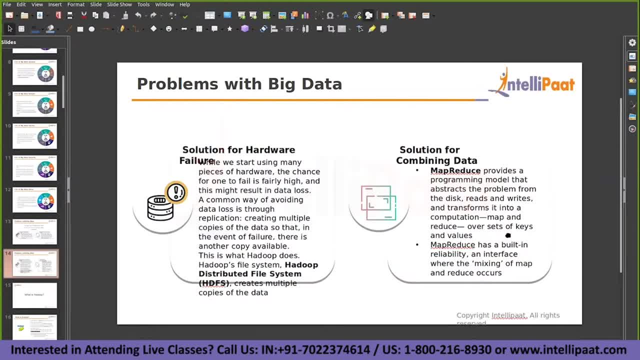 locations. you are moving the code. the problem why we are moving the code is, say, data is five kbs only, right. so instead of moving some terabytes of data, why do i have to move such amounts of data when i have, when i can move a simple kb of data to the uh machines individually? 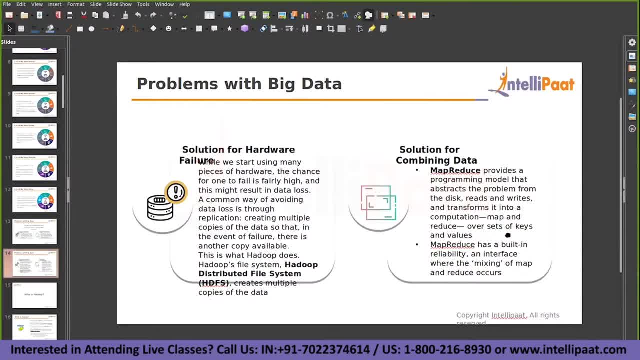 that's what i'm gonna do here, right, so now the problem of combining the data has been lost, have been avoided, right so how am i gonna do it? we will discuss that in detail, but this is what we're gonna do. this is what we're gonna do with the map reduce. so your ultimate solutions will: 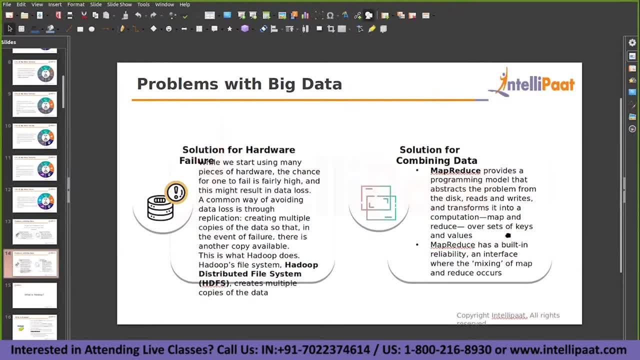 be guys. for all the storage related problems, your hdfs is gonna be a solution. for all the processing, or for all the analysis analytical related problems, your map reduce will be a solution. okay, so ultimately we have two components: one is hdfs and map reduce, so these two will 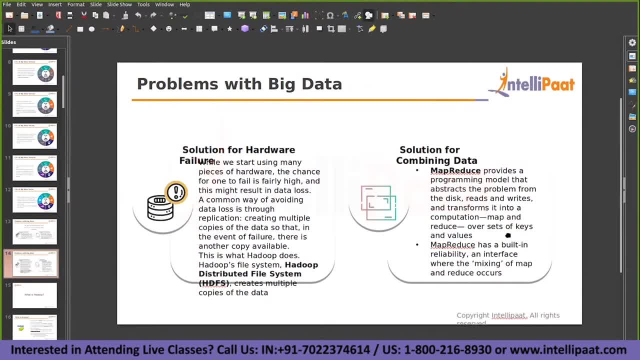 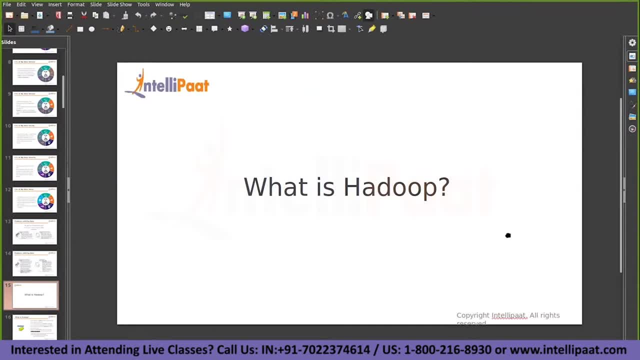 remain the core concepts of the platform that we are gonna discuss is hadoop. so hadoop is gonna have two core components. one is hdfs- hadoop, distributed file system. the other is map reduce. are we clear? okay, so we've seen the challenges, we've seen the solutions for storage, for 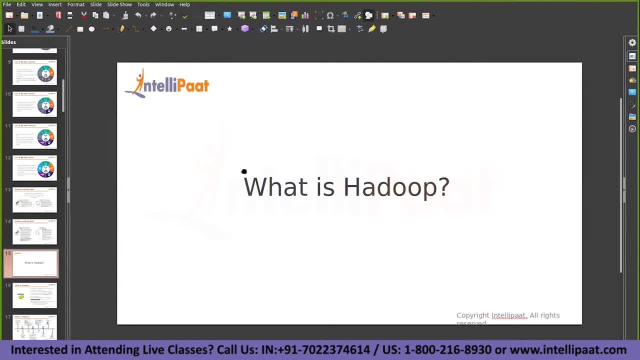 analysis, analytical related problems. we've seen the challenges, we've seen the solutions for analysis. and then what else we've seen. the hdfs and this map reduce what they are used for. all right, so those two remain the core components. we also, in the initial sessions, we have seen the 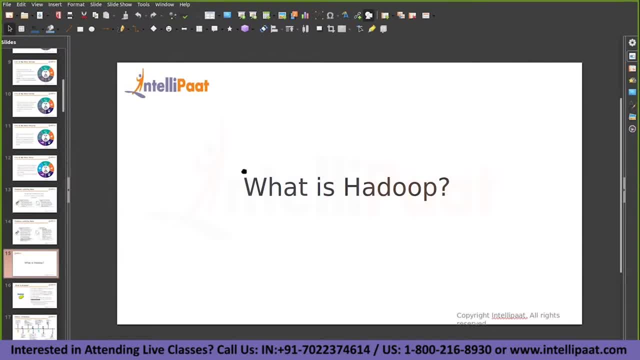 characteristics of the five v's of the big data. right. so now to start with. this is where uh we end up like. this is gonna be the platform to resolve or to to take care of all the uh challenges that we have been facing with big data. had to big data. 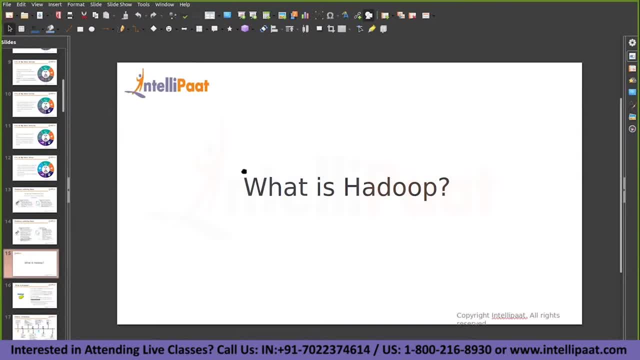 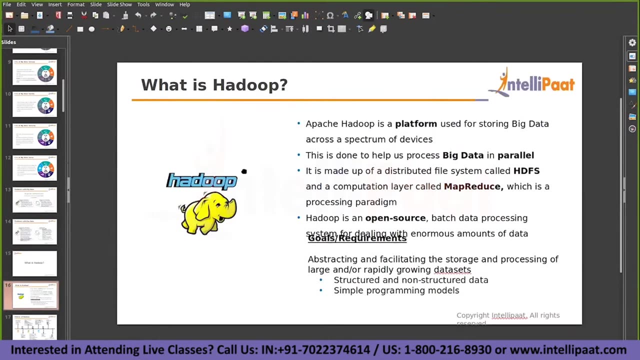 when it comes of speed storage types, all that. so how hadoop is solving all the uh challenges that we discussed. we are going to discuss further. okay, so to get a background, uh, apache, hadoop, it's now. it's now open source platform. it's. it's under the license of apache. 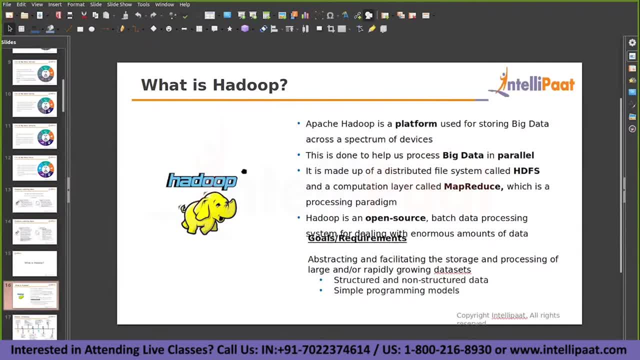 so anyone is free to use. so apache hadoop is a platform used for storing big data across a spectrum of psi devices. this is done to help us process big data in parallel. this it is made up of a distributed file system called hdfs and a computation layer called map reduce, which is 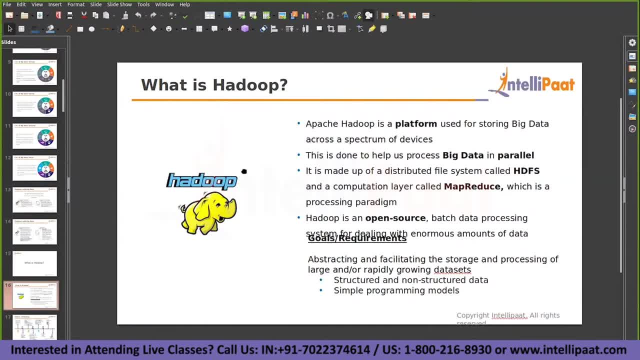 taking care of processing. it is an open source big data processing system for dealing with enormous amounts of data and abstraction and physicalization of the data and facilitating the storage and processing its structured, non-structured, simple programming model. so anything new from this slide, anything that we need to discuss? 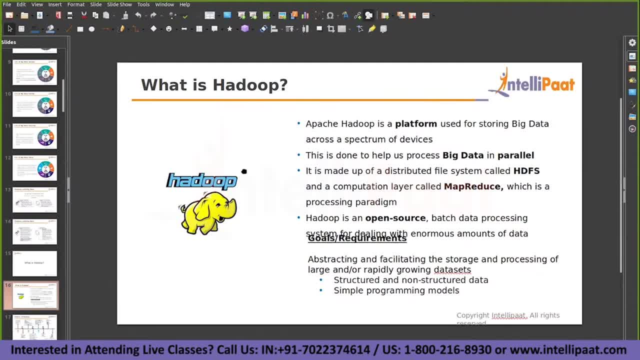 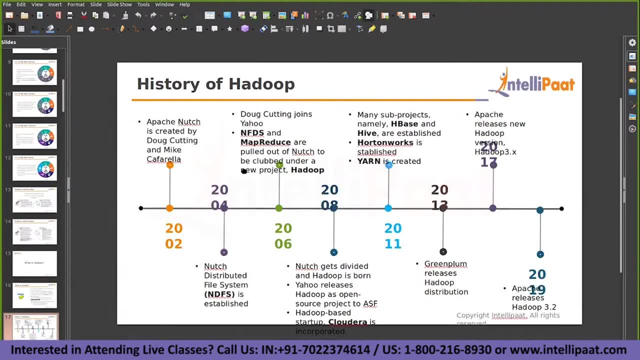 i don't think so right, are we clear? shall we move on to the next one? we pretty much discussed about everything, and that is available in this right. so so this is for you to just go through. uh, the history of hadoop, okay, started at 2002. 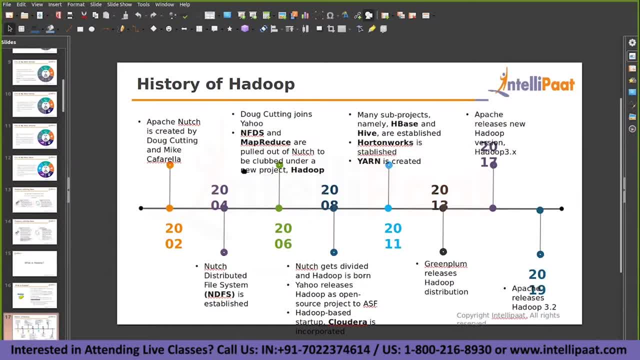 how it has evolved, what licenses it has gone into. it was with hot and works cloud era mapper and everything got merged to cloud era then and now it is available through the open source license of apache, and there were two people of cutting and mike caffrell are the people who have. 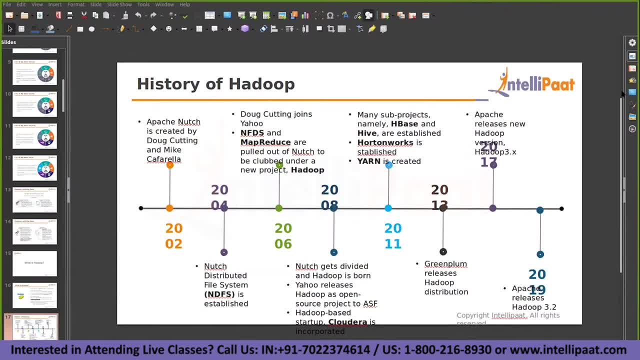 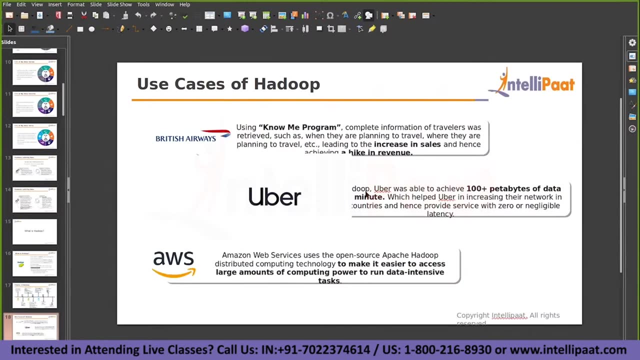 started it. okay, fine, thank you. so this is the history, guys, just for the information. so nothing, nothing in detail here, right? so then the use cases: hadoop: uh, we've listed some of the use cases- real-time use cases- where people use hadoop. what are the scenarios they use hadoop in? so british airways, we know. 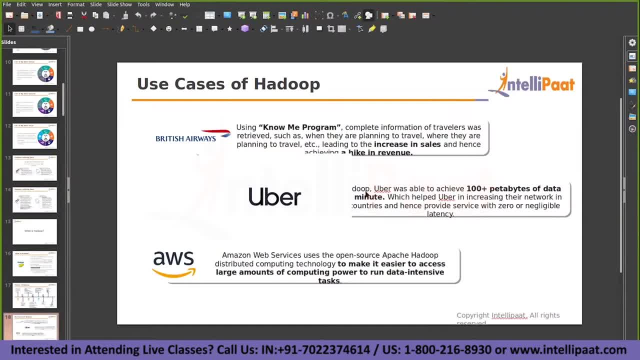 what, what, that, what they are into. so, using nomi program, complete information of travelers was retrieved, such as when they are planning to travel, where they are planning to travel and which is leading to the increase in sales and hence and achieving the hike in revenue. so, using big data, hadoop, they have, they have gathered that information and, um, they have. 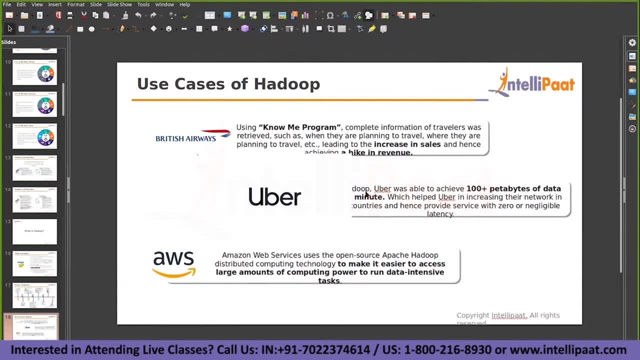 they have some of increased their revenues by by gathering all the travel information and that has used them in in in sales, pre-sales activities, and with uber, with some 100 plus petabytes of data, um, which helped over in increasing the network to the countries, hence providing service with zero or. 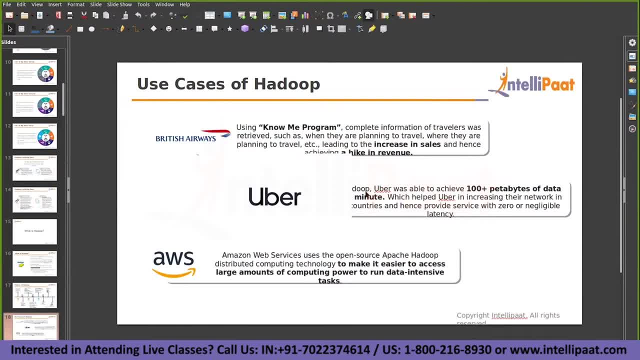 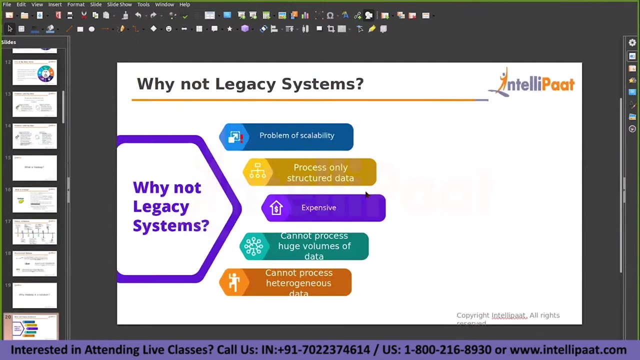 negligible latency and aws. using hadoop, distributed computing technology, it has made access to large amounts of computing power to run data intensive tasks. okay, so these are some of the use cases and why hadoop is a solution. what does it provide? what are the different features of hadoop? the first thing is the problem. 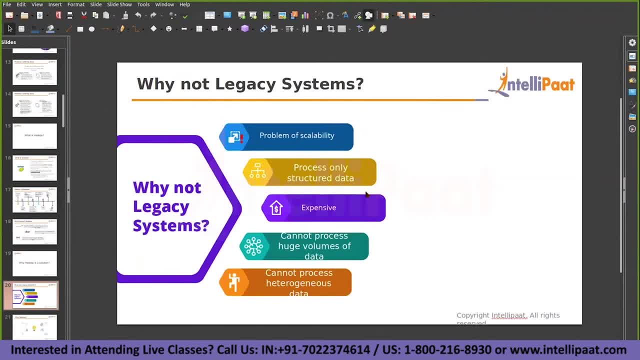 of scalability. so what is this problem of scalability mean? what do you mean by scalability factor? anyone scalability? what do you mean by this stuff? yes, no, not heard about it. what is it? scalability is um the easiness of increasing or decreasing the number of machines in your cluster. 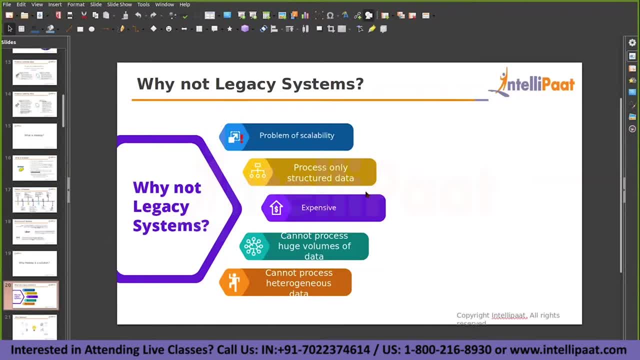 so if i'm, if i'm saying i'm scaling up thenyyyyyyyyyyy, that means i'm increasing the number of nodes in the cluster. so i'm, i keep, i keep, i keep calling them nodes, guys, because we may have to quickly move on to this terminology. so all this while 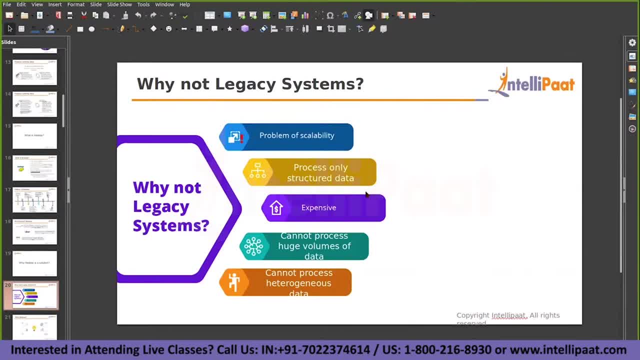 we have been terming each and every system or computer as a machine. but uh, from now on we'll be calling them as a node. so every machine inside a cluster is termed as a node. okay, so node n-o-d-e. so so when i'm saying that i'm scaling up, that means i'm increasing the number of nodes in a 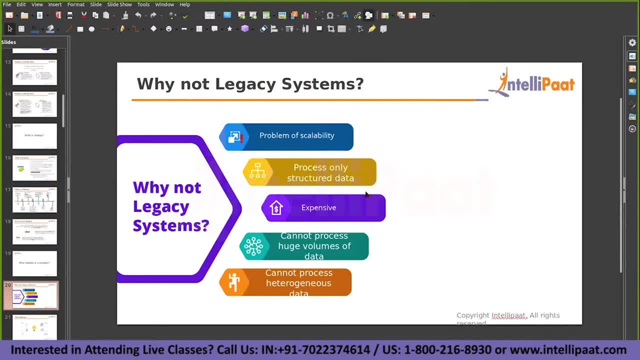 machine. i'm scaling down. that means i'm reducing the number of nodes in a machine. so this is the scalability. so these are. these are some of the problems with the legacy systems, so the pre-hadoop systems, whatever the existing systems that we have, these are some of the problems that we have. 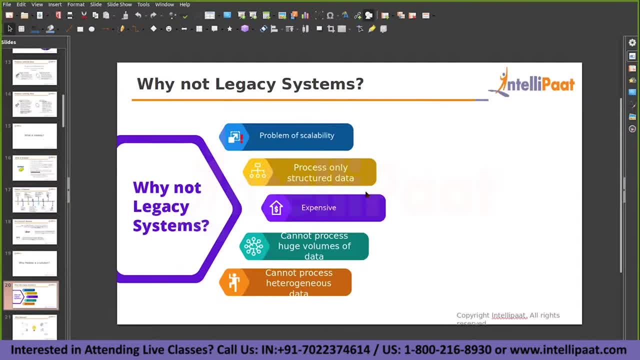 which hadoop has properly overcome. so what does this scalability mean? like they were not properly tuned for the scalability. they are not. the scalability feature is kind of complex in such scenarios, in in such systems, which hadoop has made it very easy. so what is the next one process? only structured data. 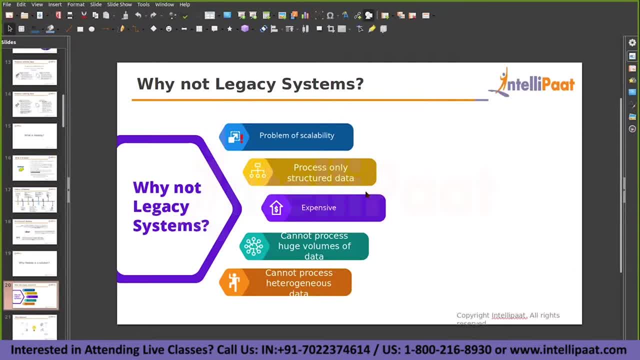 what do you mean by this? earlier systems were only processing structured data, right? so the problem is like the size of the unstructured data kept increasing, and that is the reason why we were. we were not able to handle the unstructured data with the existing systems, so that's the reason why we were. we were migrating. 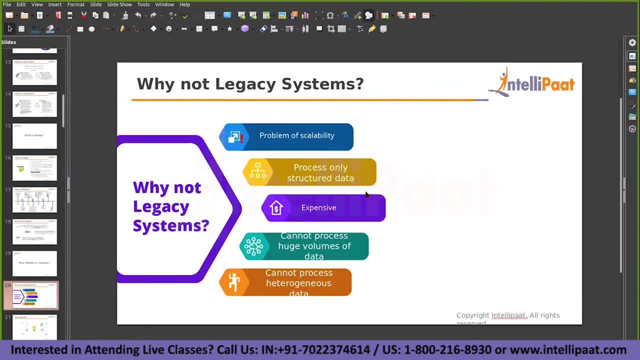 it into the latest machines. and the third problem is expensive. so why do we call this expensive? anyone? you know nothing. so when we talk about expensive, so we can categorize them into two different uh sections. okay, so we will keep comparing it with hadoop solutions and we'll 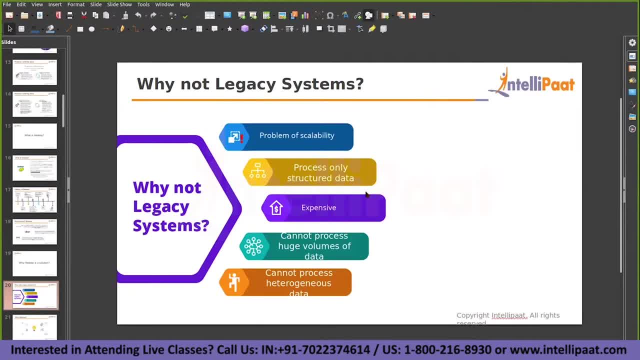 see how, how it is different. so we know mysql, we know oracle, we know postgres, we know teradata. all these, all these systems are, uh, the relational database processing systems, the legacy systems that we call it right. so are they free to use? some of them are the. ms mysql is free, it's. 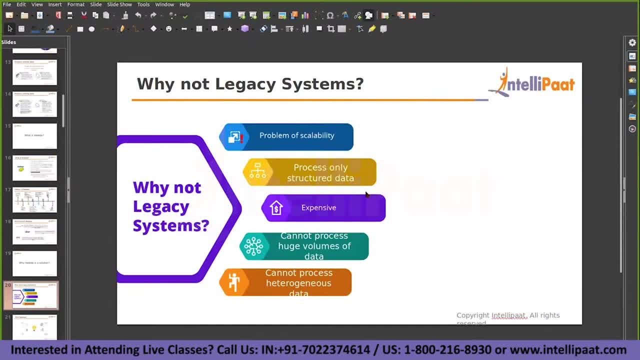 an open source. but when you talk about oracle- the most used platform, oracle postgres, these are not a free, open source tools. right, they come with a license, so you are supposed to pay for whatever the services that you are using for. but on the other side, hadoop is free of cost, you don't have to. 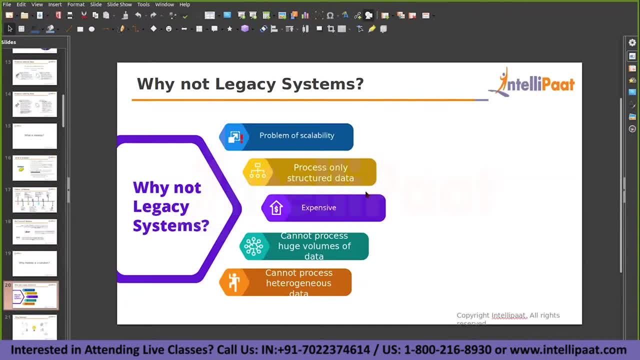 take care of any licensing costs. it's an open source solution. now, when you talk about the other systems, we know there is a distributed mechanism available, right so, for storing the data you are supposed to process, you are supposed to maintain, uh, the distributed structure. so when you have some five terabytes of data, you are dividing. 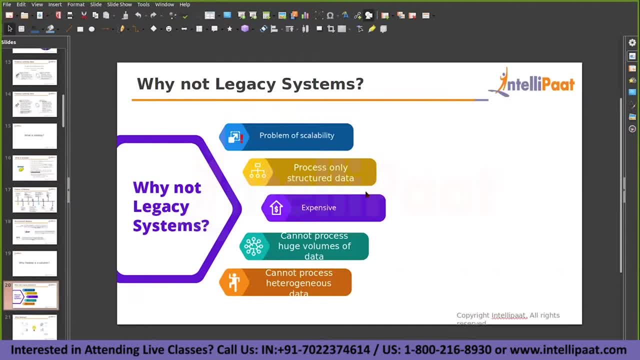 it into five different machines and you are distributing the data into five different machines here. so when there is new data coming in, you keep on adding the new nodes to the machines, to new nodes to the cluster, right? so this is what we have been discussing, so this system is available. 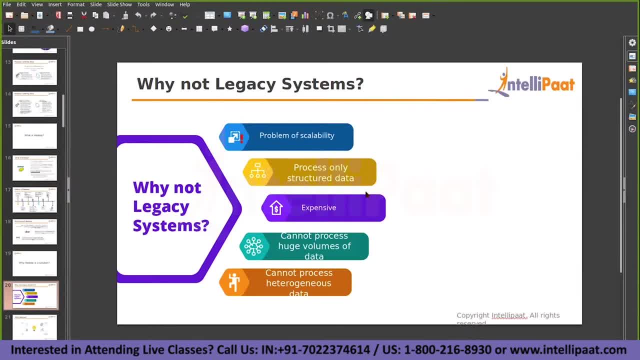 in earlier days also in in legacy systems also. this is a procedure we are going to handle and hadoop also. we were maintaining the same distributed mechanism, but how hadoop is different. so when i'm storing five terabytes of data, that's fine. i'm maintaining it in five machines. 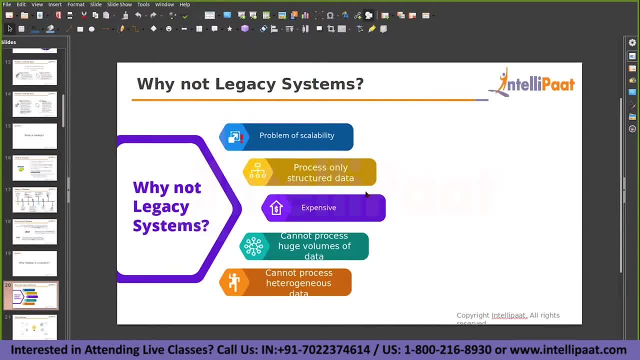 when i receive two more terabytes, i'll add two more machines. when i receive two more, i'll add. i'll keep on adding more and more machines. so what happens? the number of nodes in a cluster are in increasing. yes, so when the number of nodes in a cluster are increasing, the size, are the the price? 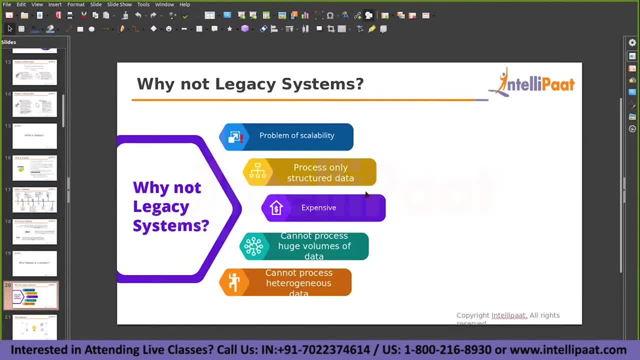 of each and every node in a machine is gonna accumulate, right, so the entire price of the cluster is kind of increasing. so the cost that is incurred for um maintaining a single node inside a cluster is: is what we consider this as a the entire cluster price, right, so every node comes. 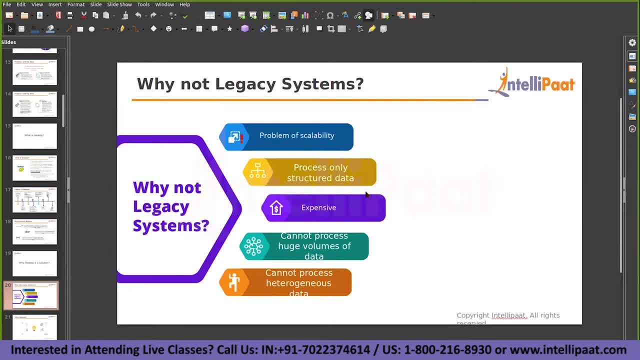 with a price. so, for example, if you have to add some cluster item to a cluster or say, let's say a dog is going to have a dog model, add a new node to the existing cluster. if there are 10 class 10 nodes in a cluster, it's, let's say: 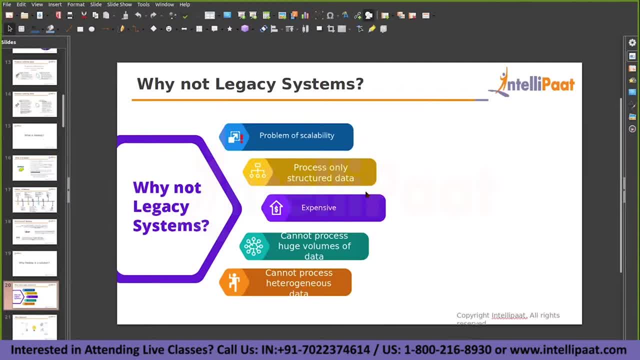 it's around 10 000 each node, so 10, 10 into 10, like it's accumulating to one lakh, for example. there is another node that is being added. right you, you keep on increasing the price, right? so adding more and more nodes to the existing cluster will keep on increasing the price, and 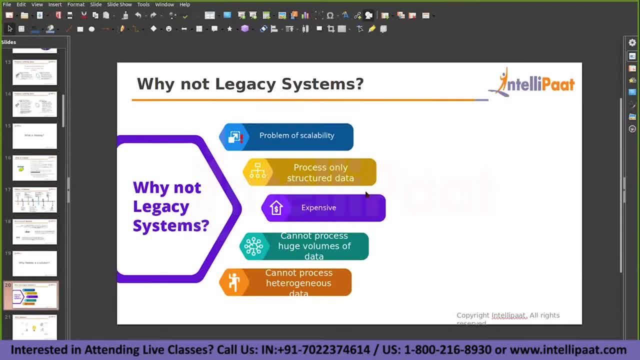 that is why it is becoming expensive. but you may question me that- because in in hadoop also use the same technology. in hadoop also use the same distributed mechanism. in hadoop we are kind of maintaining large amounts of data sets and we are also maintaining the replicated copies right in 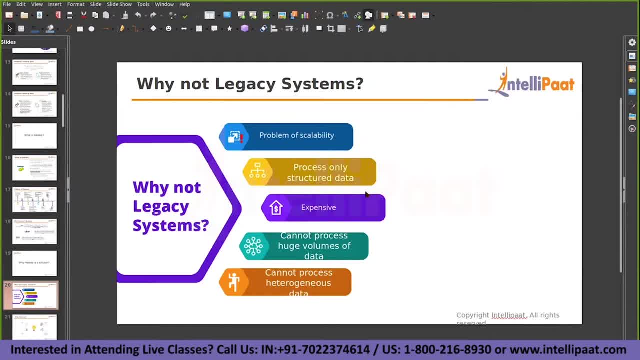 the legacy systems what we used to do. if five terabytes is my data, i used to maintain only five terabytes of storage. but in hadoop, what are we doing? we are maintaining 10 terabytes of storage, 15 terabytes of storage. why is it? because of the replication factor. i agree when the replication 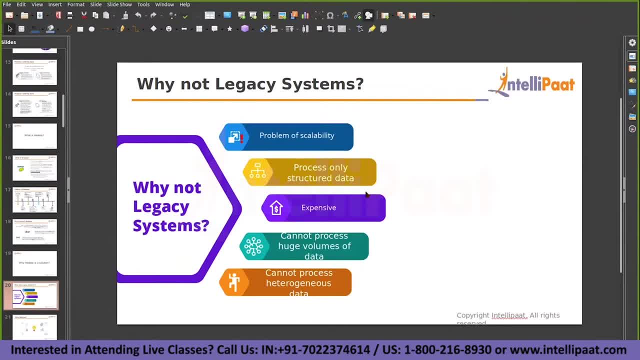 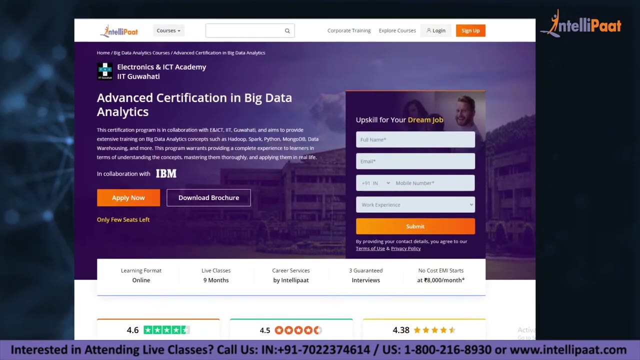 factor is set to two, set to three for storing you. just a quick info, guys. if you want to make a career in big data, then intellipaat provides an advanced certification in big data analytics by enict council, iit, guwahati. it is taught by iit professors and industry experts with 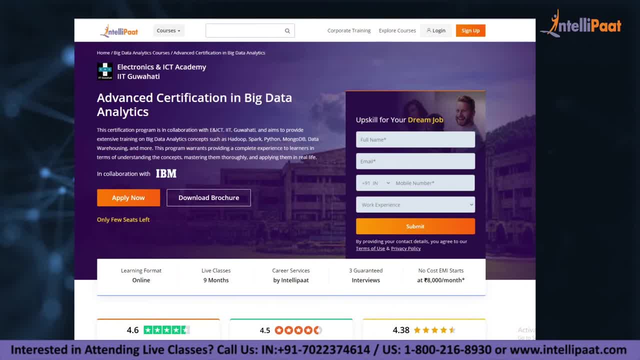 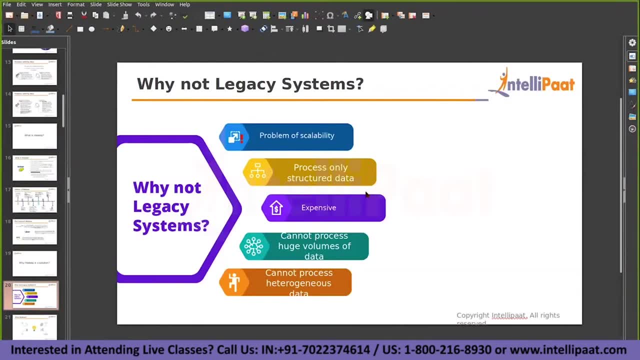 me. i am actually using five terabytes of data. i'm actually using five, 10, 15 terabytes of storage, more than 10 years of experience. this course is designed to upskill and land your dream job. now let's continue with the session. you understand the problem, that that we are discussing the, the 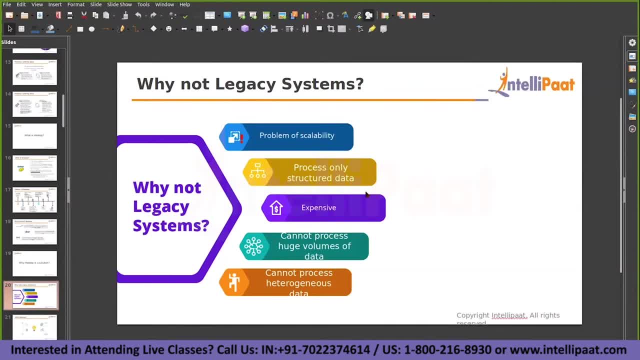 question that we are discussing. even with the distributed mechanism, even with the replication, we are still able to store it with less amount of cost. any guesses right? so the reason is there is something called as a commodity hardware in hadoop. okay, so hadoop is designed in such a way that it can also work with 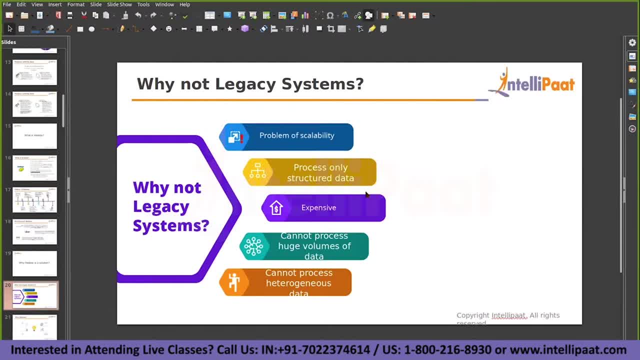 a commodity hardware. so what does this commodity hardware mean? so it's the cheapest hardware that is available in the market, right? so, for example, in your existing systems for for designing your existing nodes in a cluster, you would need some high-end software, but whereas in hadoop you are. 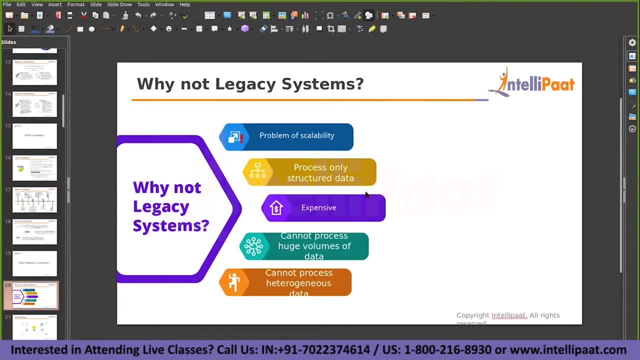 not going to use any high-end software. the only need, the only component that we would need for your hadoop cluster node to be is the, the, the size, the hard disk size, right? so if i'm, if i'm configuring a cluster, if i'm configuring a node in a hadoop cluster, you just need a hard disk. 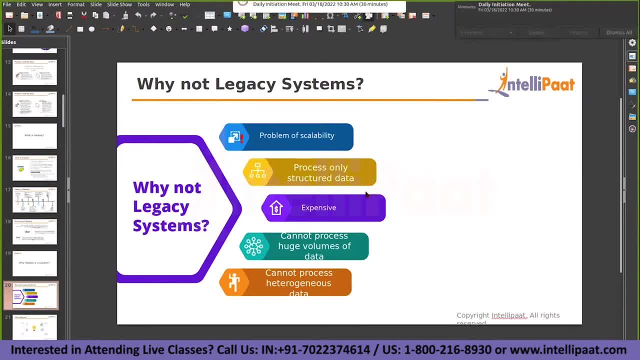 for it. you don't need any software allocated to it. there is some amount of minimum ram that is required, of course, but no other additional software. it is- it is the the least- that the cheapest hardware available in in the market is what we call it as a commodity hardware. so by, by using the 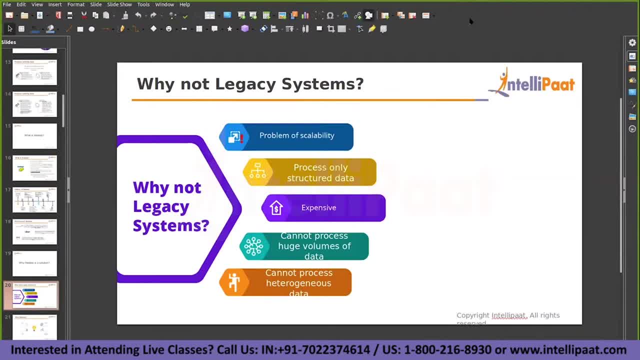 such kind of machines, we were able to reduce the cost drastically in the cluster. so if other clusters were having a node which is of around ten thousand uh per per node, if my cluster, my hadoop cluster, can have it only for five thousand or three thousand, four thousand, i mean these are 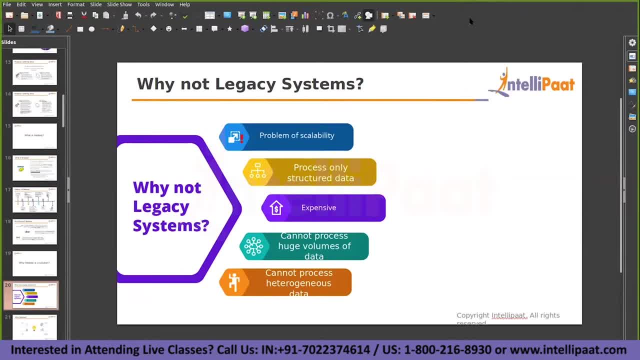 not the numbers, but i'm just trying to show you the actual uh comparisons. okay, so that is how, by by using the commodity hardware, we were able to reduce the cost of the entire cluster in your hadoop system. so one thing is: it is open source. that itself is reducing a lot of price. 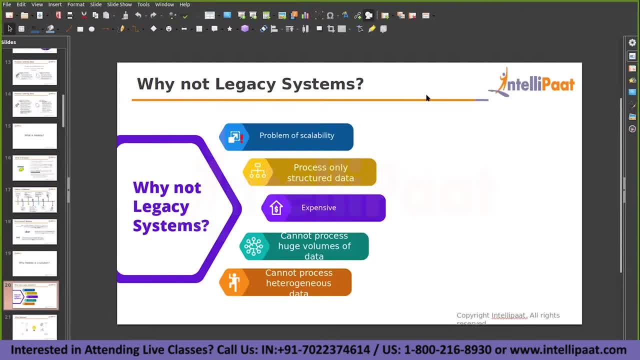 in maintenance. and the second thing is by using the commodity hardware. you need not, you need not spend amounts on uh high-end commodity high-end machines. you just need a basic hard, uh hardware that that can store some amount of data in it, right? so by using this commodity hardware, you 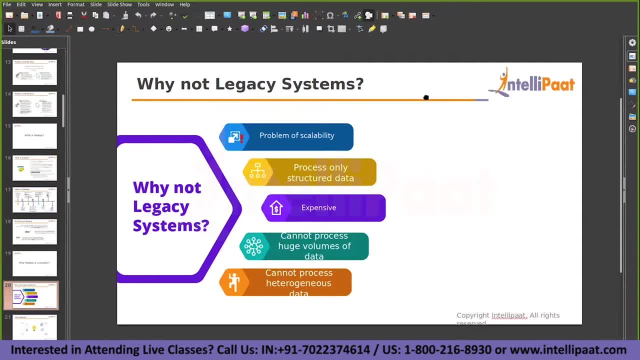 were able to accumulate more and more number of machines and and that is why that is the reason why you're able to um maintain this storage. i mean, you are able to uh negotiate or uh, it's almost negligible. the price that you are considering for storage is is negligible, and that is the reason we were able to. 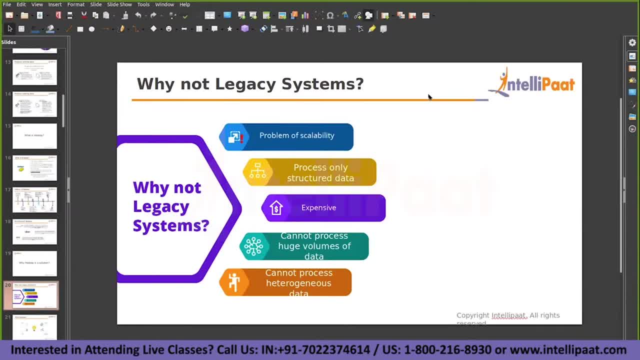 accumulate this replication as well. so we are not even worried about the storage. now, with the help of commodity hardware, you are not even considering the price of the hardware. your storage is coming at a very low cost and you are able to replicate the data and you are maintaining the security. 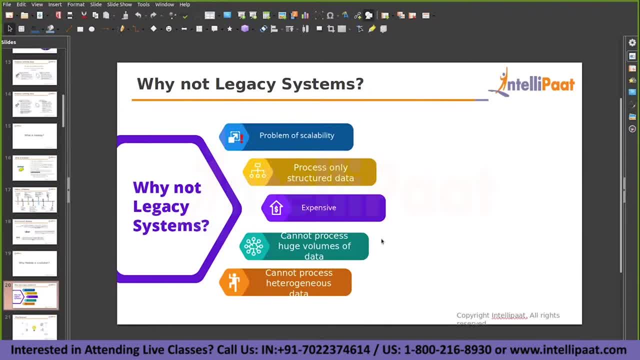 feature of it, you are maintaining the fault tolerance software. okay, so that is the reason we call it, as the other systems were called, as an expensive, so cannot process huge volumes of data. that is one reason. the existing one and uh cannot process heterogeneous data. so what do you mean by heterogeneous data? 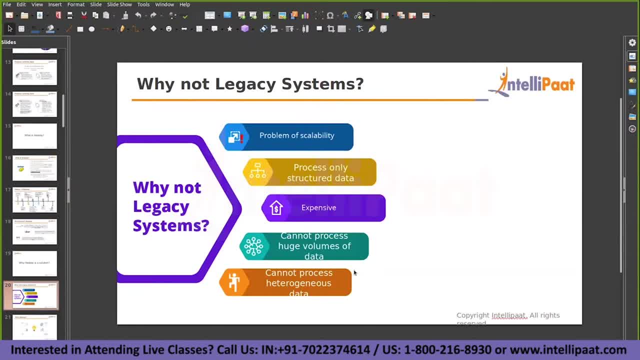 any idea. different types of data: yeah, so with high variability or different types of formats. right, we call it as a different, heterogeneous data. so how do i mean? existing legacy systems were not capable of handling such, such veritings or such variability of data sets or different types of. 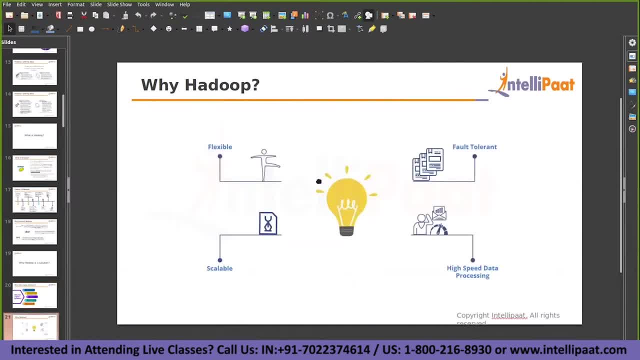 data sets. right, then, why hadoop? it is flexible. what in? what is what is flexible in terms of user friendly? someone said it's user friendly. okay, you can consider it as user friendly. right, it's flexible to use and fault tolerant. uh, what is the reason? first, fault tolerancy. how did we? 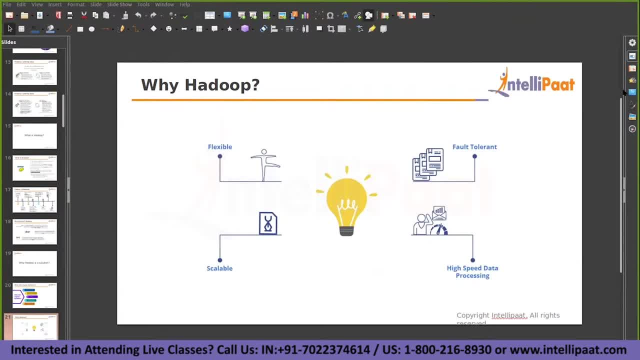 achieve this fault tolerancy right. so through replication comp concept, we were able to achieve this fault tolerance by maintaining multiple copies of uh data- the same data. the third thing is scalability. you can scale up to any number of nodes and you can scale down to any number of nodes, depending on the requirements. so scalability is not a problem. you can, you can keep. 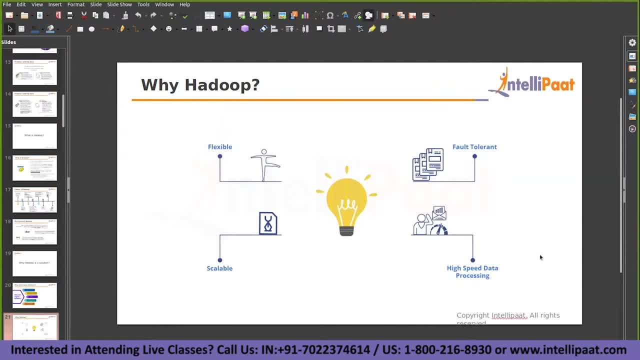 on adding more and more missions to the cluster high speed data processing. so how this high speed data processing is achieved, what are the tools comprising, are, which is, which are which are contributing for this high speed data processing? we will discuss like it is meant for high speed data processing. map reduce is one of the concepts. 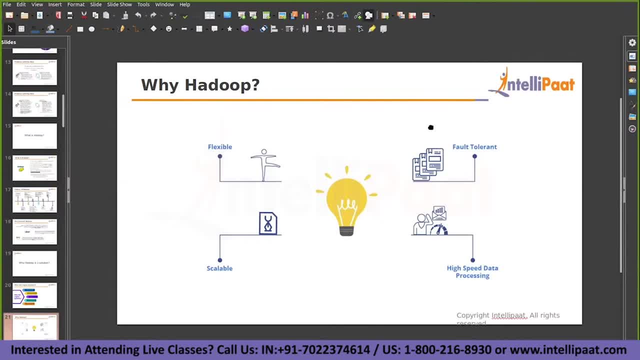 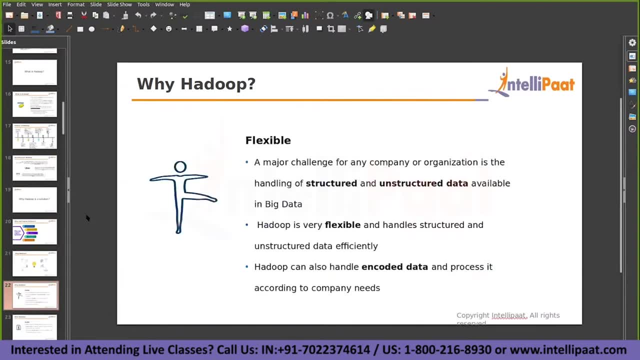 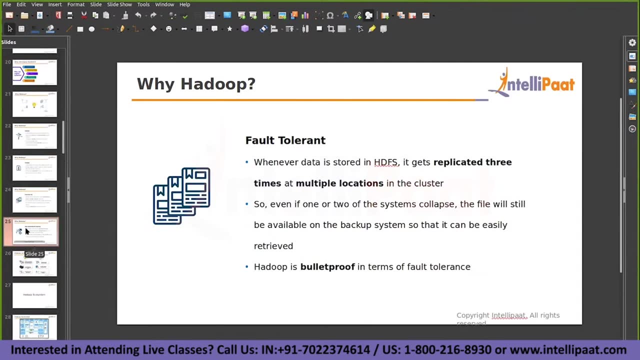 like it is. it is uh processing the data with uh with huge speed compared to the legacy systems, then. so flexibility- we have seen the structured, unstructured data, uh differentiation and scalability- we know uh fault tolerancy- that is a replication- and high speed data processing- that is achieved. 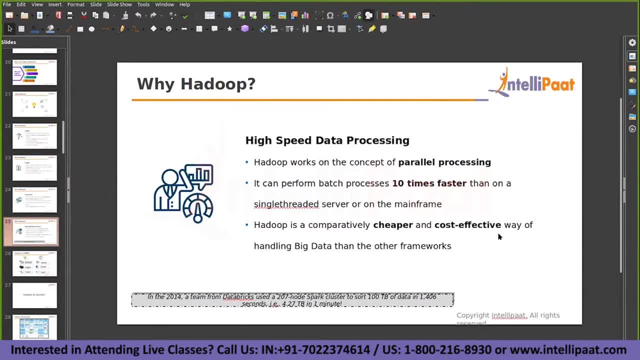 using this parallel processing system, it's almost like 10 times faster than the existing process. uh, that is how we do this, using the map reduce. so we will discuss about these things in detail. the high speed data processing: that is the reason why we will. we will move to the next one. okay, so how this high speed? 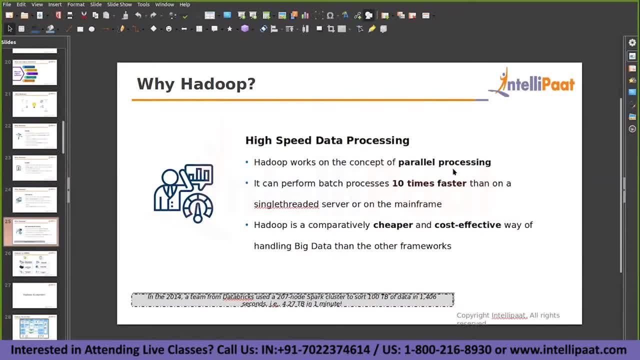 is achieved. i mean in in general terms. you can also think about it: if, if, uh, the legacy systems were handling, uh, you can take the same voters example. let's say: right, so the data, the time that is consumed for you to retrieve the data from data, and the rate of processing the system, the rate of 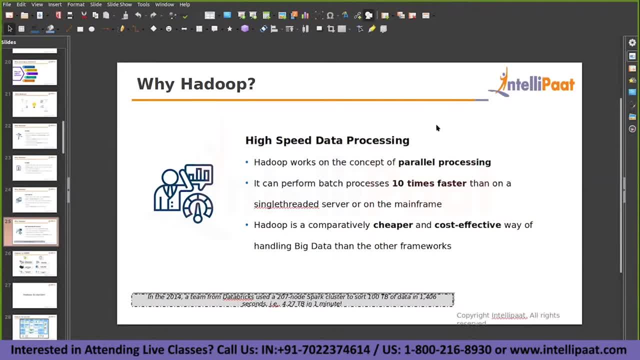 from different nodes, gather them, combine them and do the processing, do the computation and retrieve or restore the data in the so-and-so storage systems is kind of delayed process right, It's taking a lot of time for you to combine. But whereas in MapReduce way of processing 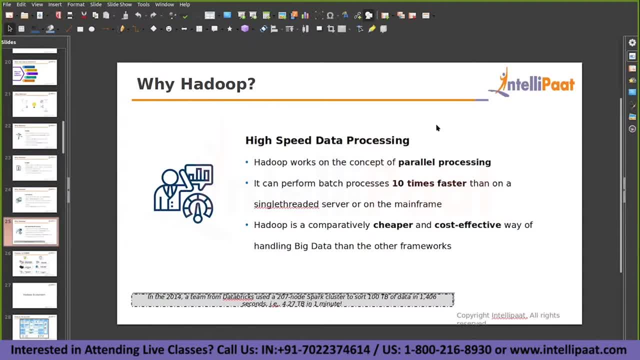 what do you do? You, instead of moving the data, you move the code to the data. You move the program to where the data is available. That is, avoiding the data reads and writes. So you're not moving the data anywhere. that because of which your time 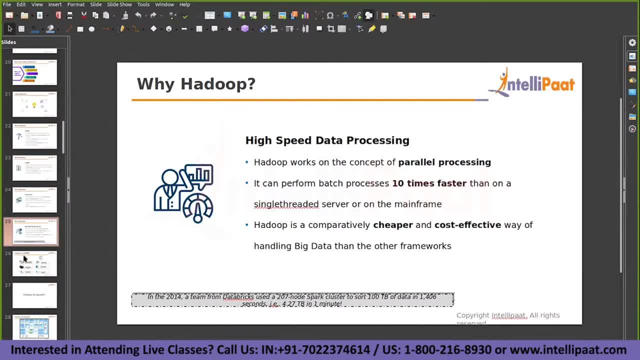 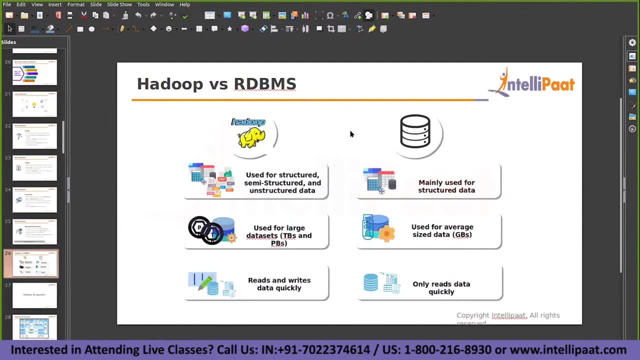 has been reduced drastically. okay, Then we have the comparisons with the Hadoop versus the relational databases. We've already seen some of them. So Hadoop is mainly used for it can handle structured, semi-structured and unstructured data sites. 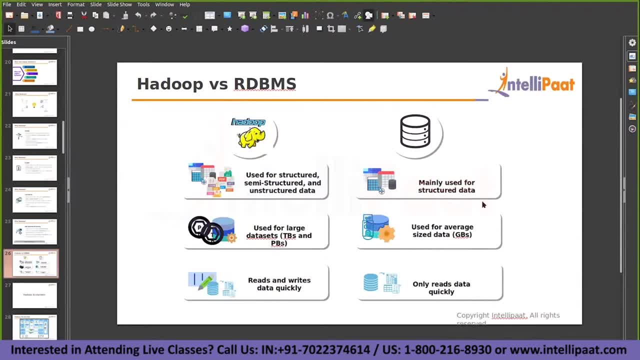 Whereas RDBMS is the relational database management systems. All the structured data processing tools- Oracle, Postgres, MySQL- will come out of this RDBMS- okay, If you're not aware of it. So it's only mainly used for structured data. 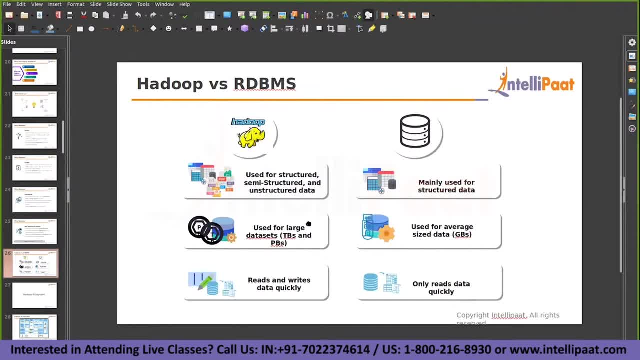 And the data size it can handle is in terms of TBs and PBs. We are not gonna talk in terms of GVs anyways, here And but, whereas in relational databases it was only restricted to GVs- And reads and writes data quickly. 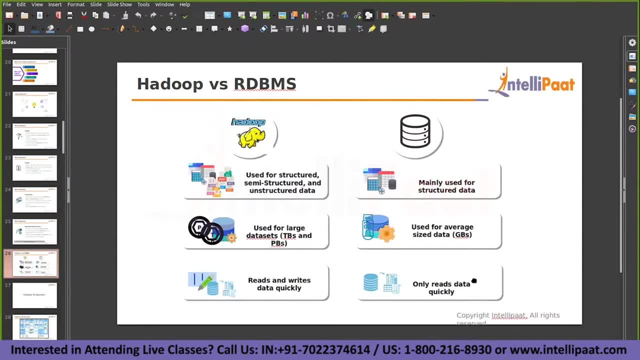 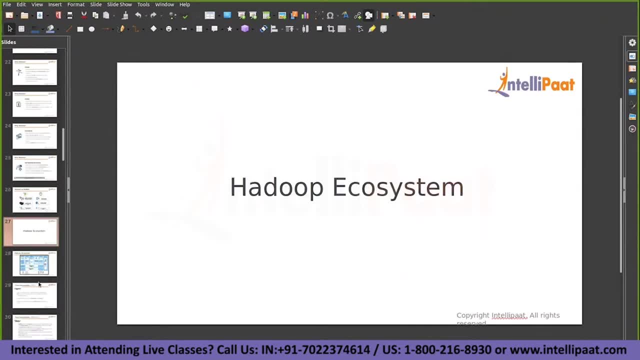 only reads the data quickly. The insert operation is gonna take definitely some amount of time for you, But right then. Hadoop ecosystem. So when I say Hadoop, there were so many other tools which come along with it. right, It's not just a single platform. 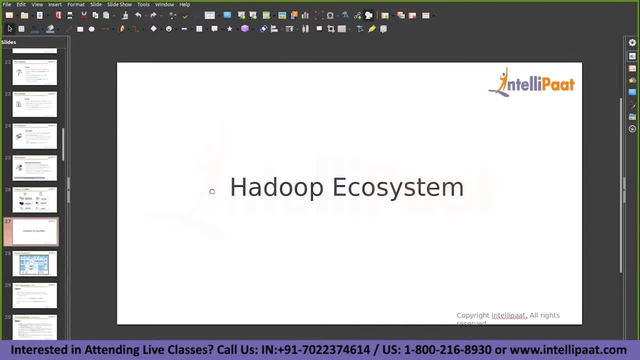 The ultimate component is gonna be the HDFS for storage and MapReduce for processing, And there is some advanced processing mechanism. But in addition to that, on top of it, I can say on top of these existing components, we built a different set of tools. 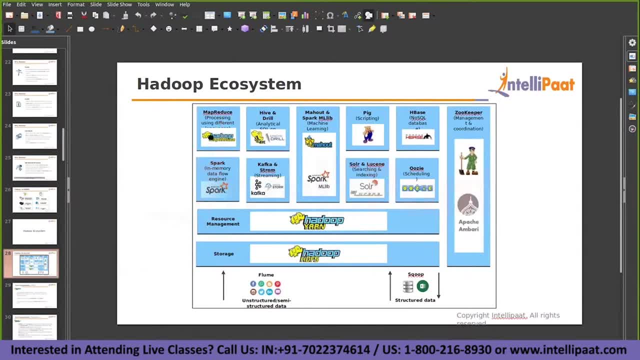 So we will. We will name some of them. So there is MapReduce, Spark, Kafka, Hive, Mahout, Pig, HBase, Zookeeper, Uzi, Solr and Luzine, And there is Flume, there is Coop. 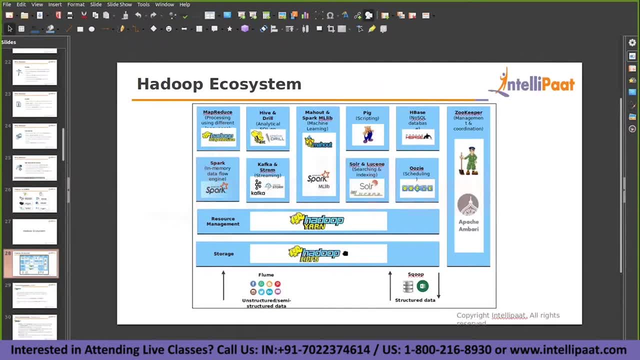 So the core mechanism is what The storage Hadoop, HDFS, right, So this is not changing for anything And there is something called as YARN. This is the advanced version of MapReduce. okay, So we will discuss about it. 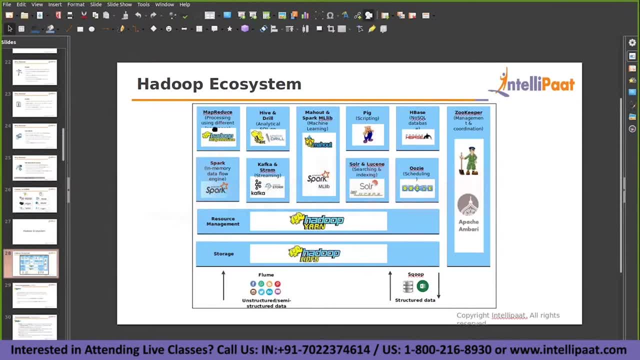 So after we discuss about MapReduce, how this MapReduce works, then we will move on to the Hadoop YARN concepts: how Hadoop YARN has overcome or has improved- or we can say it has enhanced- the functionalities of MapReduce. how it has made some difference. 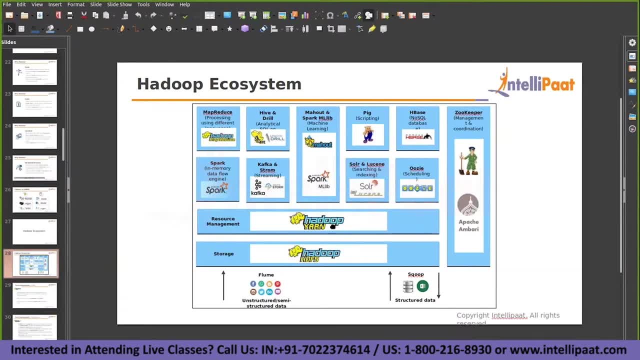 So it is the latest version of MapReduce. we can call, or the Hadoop 3.x, I guess right. So Hadoop HDFS, Hadoop YARN is gonna be the same. This is for storage, This is for map processing. 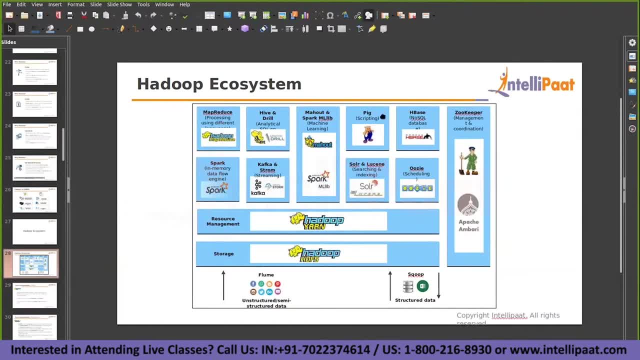 On top of which you have PIG. PIG is mainly for unstructured data processing. It has its own scripting language. PIG is kind of completely moved out of the market. now. There are very limited, very, very limited companies which are using PIG in their projects. 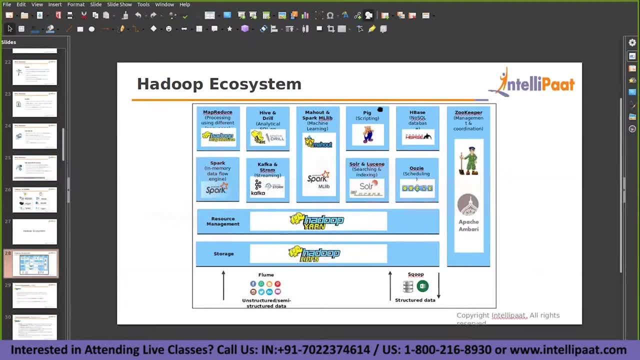 So you can assume it is gone. And the most important thing is Hive, which is still in the market, which has been used by many, many, many organizations. Hive is some kind of a tool which is similar to your relational databases. 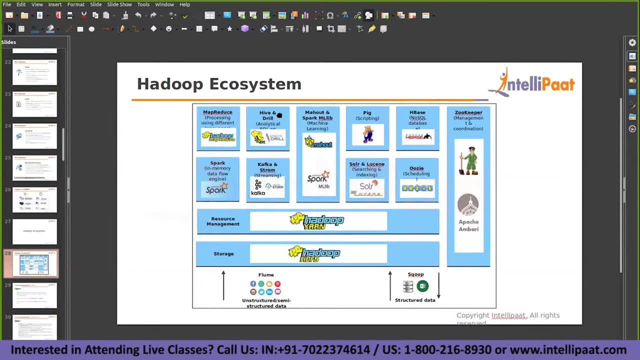 So, like we have Oracle and all that outside the Hadoop ecosystem, you have Hive inside the Hadoop ecosystem which are gonna do the same thing, which is gonna do the same thing as the other RDBMS. okay, So the problem is: 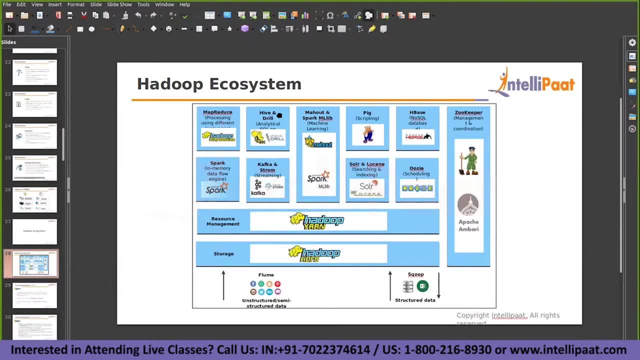 for example, I have the data, I can have any kinds of data right, I can have structured, I can have semi-structured, I can have unstructured. So when you have a Hadoop platform available, that means you're supposed to migrate. 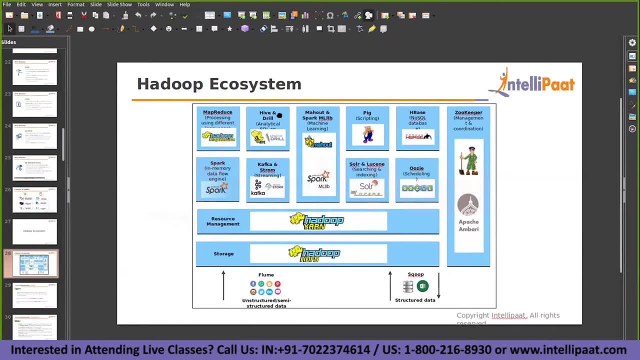 the entire existing ecosystem into your Hadoop platform. That means, for example, if you have some data in Oracle, okay, it has reached its maximum capacity, It has got its limitations. Now what you're saying? you're saying that you'll be migrating it. 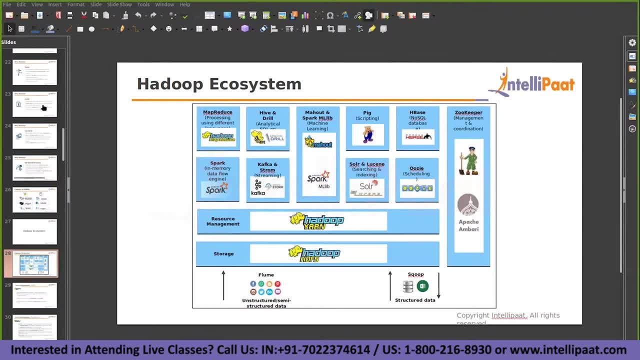 into Hadoop ecosystem. So when you say you're migrating it into Hadoop ecosystem, what is the first thing that you're gonna do? You're supposed to migrate all the existing data into Hadoop platform. Agree, right. So whatever the data you already have, 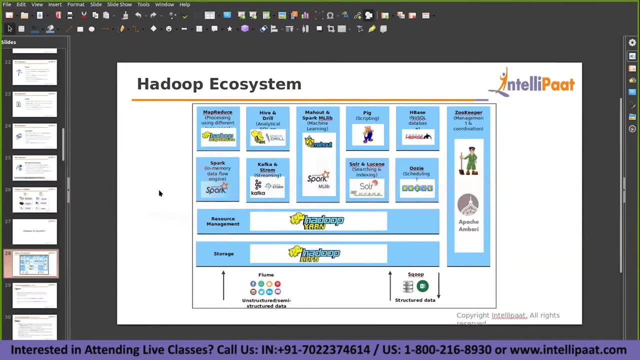 in this database or in these tables, has to be first migrated into the Hadoop ecosystem. That means you have to migrate it into HTFS. Then you think about the later stages, I mean whatever the data is coming in future, you know. 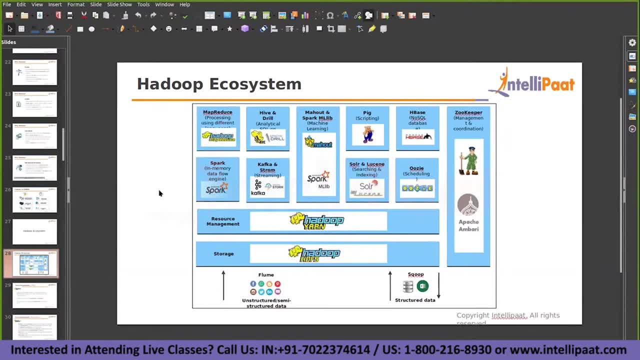 be tagging it to, you'll be pulling it into your Hadoop ecosystem. that's fine, but the existing data has to be migrated. so when the data is coming from an oracle database, you should have a similar framework, such as oracle or such as any relational database, inside your Hadoop ecosystem also for you. 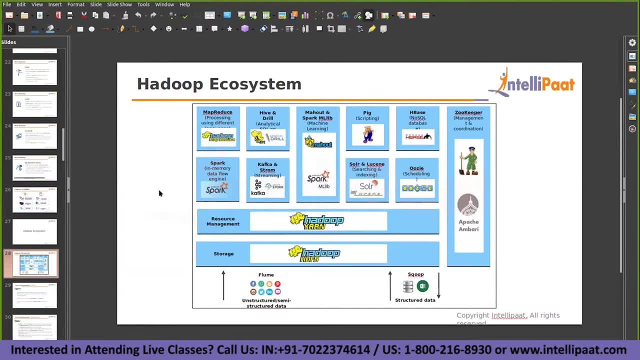 to be able to process it. so so, so easily see if the data is available in a table. let's say: okay, so there is a database db, there is a table sample. okay, so you do select star from dbsample. what do you get? you get the results. you get only one column, so you do, you do select id from sample. 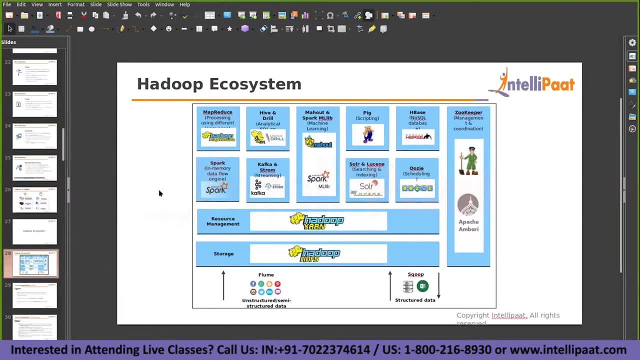 select id from sample where id is greater than 10. that means i only get ids which are greater than 10. so how easy is it? how familiar are we with this kind of reading and writing the data right? so any one of us, or most of us, are pretty sure about what a 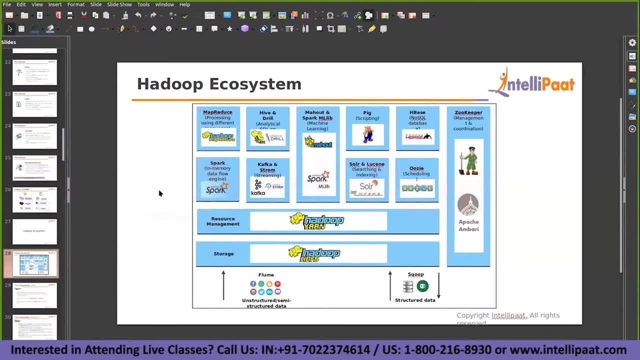 selection is going to look like. so you do select star from dbsample. so you do select star from emp. we do right, or some of us are even aware of some advanced concepts of sql, but pretty much all of us will have some or the other knowledge on the sql commands right. so this is the most easiest and 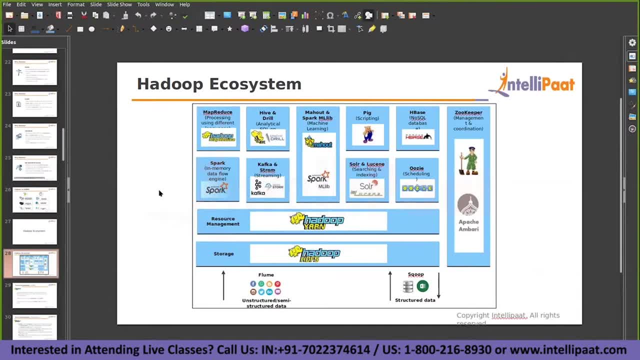 the most used way of handling the structured data, so why change it then? if this is very, very, very famous tool, if it is a very famous way of dealing with the data, dealing with the structured data, why can't we have a similar framework inside the adobe ecosystem? that's what has brought into this hype. 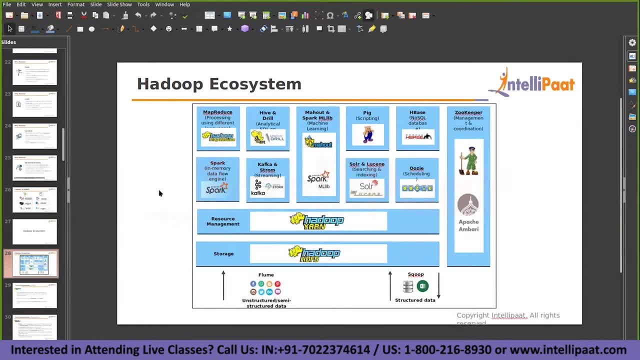 so the same command, the same select star from, or whatever the insert commands, the create table commands, or group by commands or order by anything, everything, the joins, everything you kind of import from all the relational databases. you, you build your own platform in the hadoop ecosystem- that's what is called as hype, with some advanced features, with all the additional. 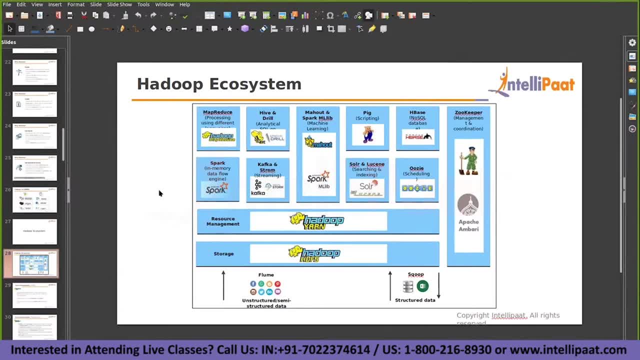 capabilities of hadoop. you kind of give the same look and feel for your data. for the structured data, mainly right. so you have hive to handle the structured data inside the adobe ecosystem like you have done with the other relational databases. you bring the hive to the adobe ecosystem. 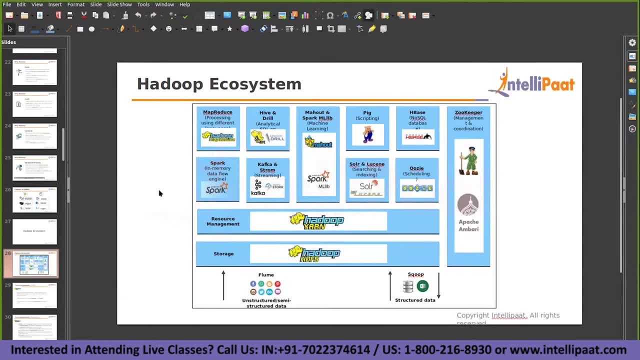 agree, clear, right. so similarly, you have other tools also. kafka and storm are mainly for streaming. we discussed about the data which is a generating with some amount of speed and you are able to capture the data on the destination system near real-time way, right? so all this? Kafka and Storm will take care of all this kind of 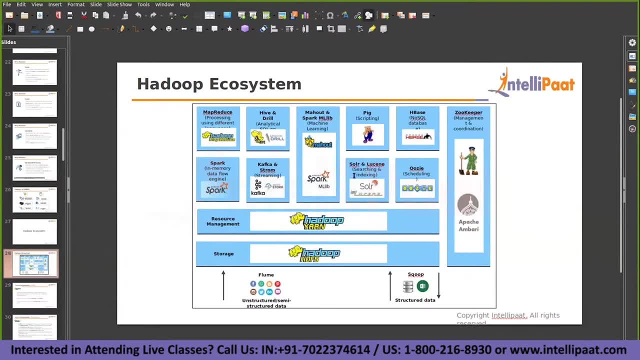 functionalities, and Solr and Lucene and which is for searching, and Uzi is for scheduling, and HBase is the no SQL way of handling, the unstructured way of handling the data, and ZooKeeper is maintaining the nodes, the management and coordination between different nodes, and there is Spark. we will anyway discuss about this in detail. so the in-memory processing and 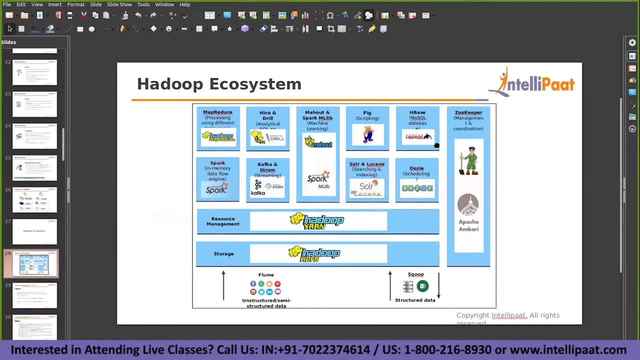 all that, so these are all combining together for your Hadoop ecosystem. there is Flume and there is also okay, so Scoop is basically used for integrating or connecting your relational database to your Hadoop ecosystem. so what it basically does is beat any kind of relational 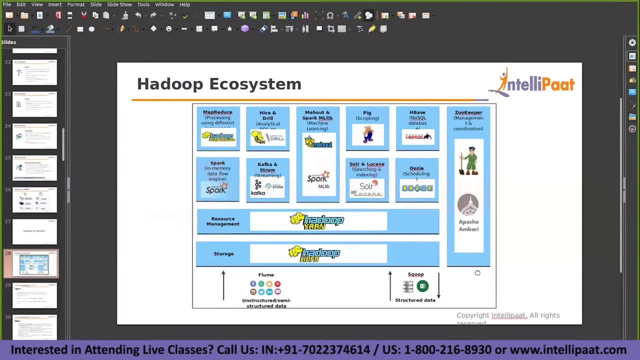 database. it is used to dump the data from source to the destination. so source can be a relational database or HDFS, destination can also be HDFS or relational database. okay, so it's basically kind of interacting with a relational database either via source or a destination. okay, so in most of the migration projects we'll be using Scoop. this is the best. 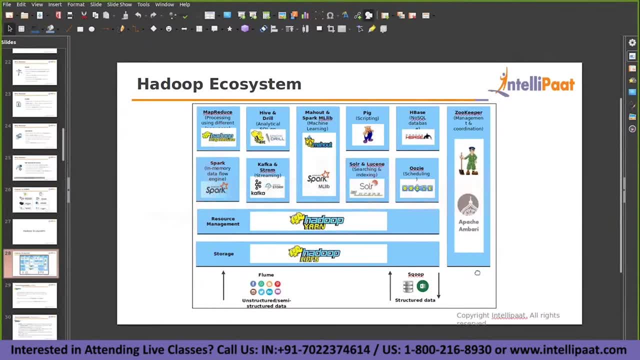 way of importing the data from the existing relational databases into your Hadoop ecosystem. any questions on this slide? Paul, clear, okay, so we are not going to get into the details of each and every component in this session, guys. what we only discussed is the core concepts of what Hadoop ecosystem is built on. Hadoop HDFS. 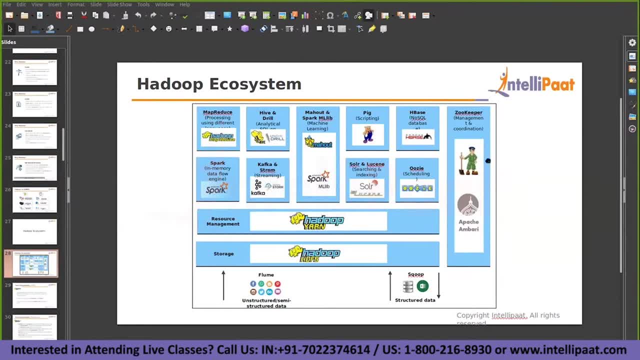 MapReduce and YARN. okay, so other concepts we may have to get into the detailed discussions of Hadoop sessions and, as we have signed up for we will only discuss for Hadoop core concepts, just to give you some kind of an flavor or kind of an introduction to what Hadoop is all about. 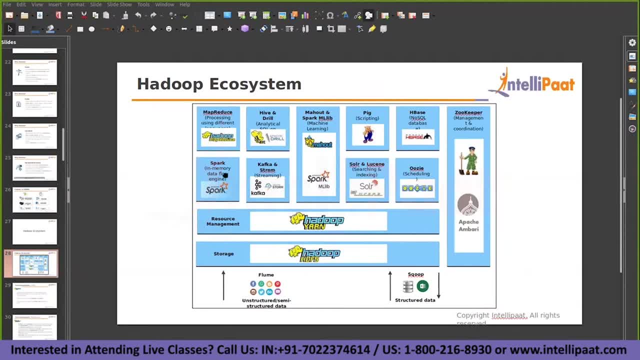 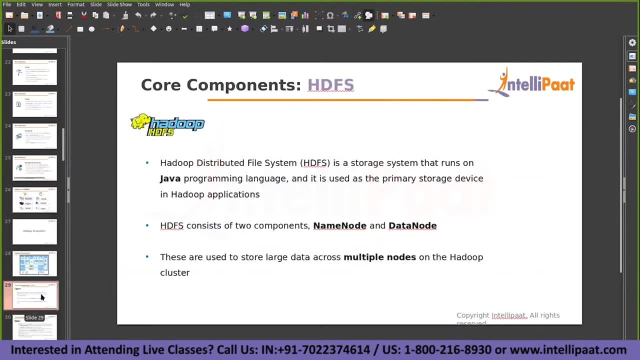 and then later on we will move on to this Spark. so Spark will get into the details, in-depth concepts of each and every component inside your Spark. okay, then, now going on to the moving on to the HDFS. so we will discuss with the core components. the first core component is: HDFS is a storage system, that's. 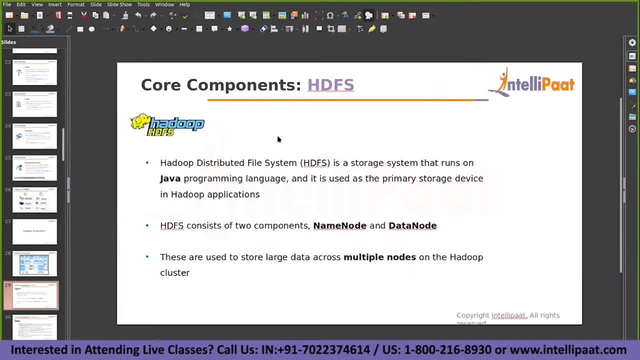 running on a java programming language and it is used for a used as a primary storage device in hadoop application. so it is built on top of a java. so we are not we are not worried about, let's not worry about what it is built upon, how we can access. so what we do need to understand is: 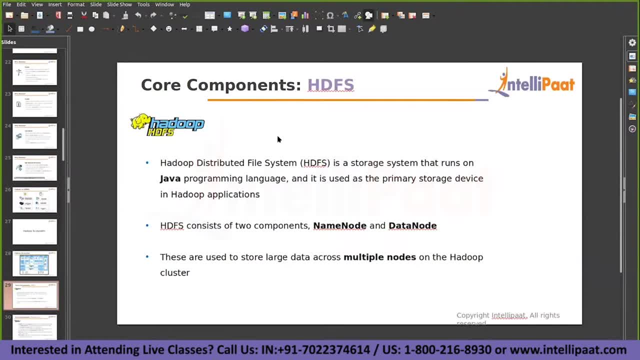 what, what are its features or what is what is its architecture, how it is working and what does it do? basically, what is it going to do? in each hadoop, it is going to take care of all your storage related needs. so in a hadoop ecosystem, in the hadoop platform, hdfs is gonna be your ultimate. 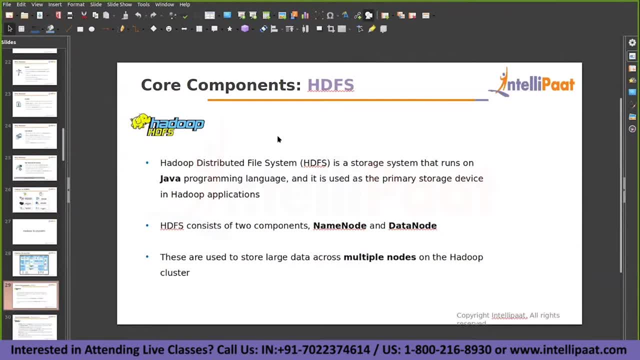 storage. okay, so, regardless of what your hdfs will be your primary source for your storage of data. okay, so it. it has two components. so, like we have in hadoop, hdfs and map review, so inside hdfs you have two more components. one is name node and the other one is the data node. so we will discuss about, uh, what is name node? 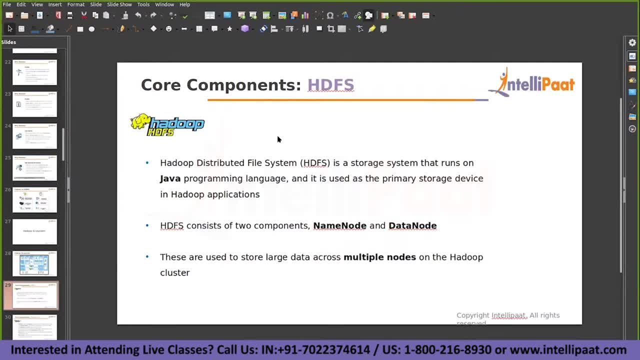 what is data node in detail? we will get into these concepts, but, just to let you know, there is name node and a data node, two nodes inside your hdfs. there is one more secondary name node, but we will get into the details later. okay, and this is used for storing large amounts of data across multiple 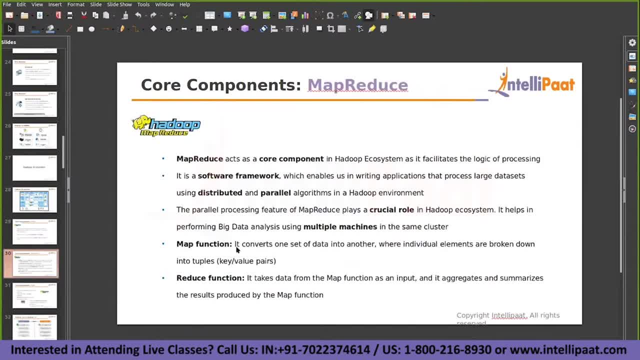 nodes on hadoop cluster. yes, you know. then map reduce, like we know we have um, this map reduce for all the processing related needs, how the data can be processed on the hadoop ecosystem. uh, all the executions, all the computations, all the processings can, can only be done through a map reduce program. so 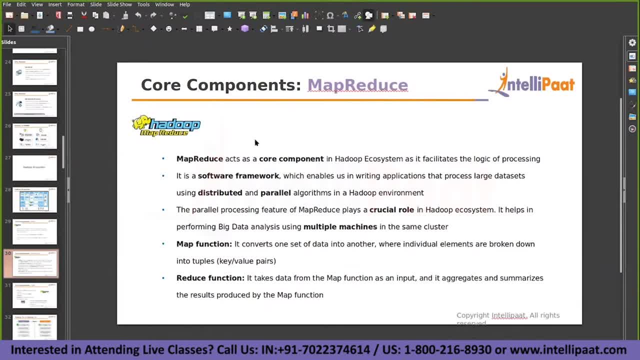 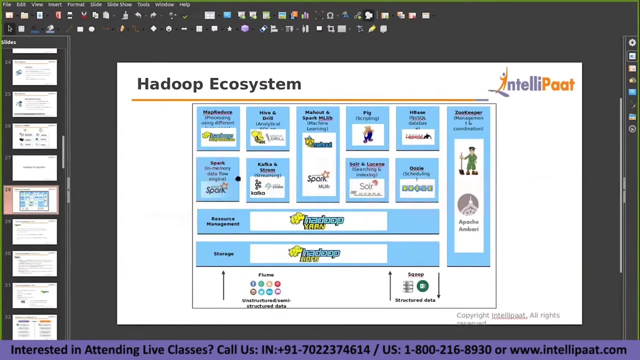 now it is being replaced by or, or it has been over or upgraded to yarn. i can say: but earlier it was map reduce, in the initial versions of hadoop it was map reduce. so, if i can go back here, see for all this, for hive, for pig, for spark built on hadoop, for zookeeper, for hbs uzi and 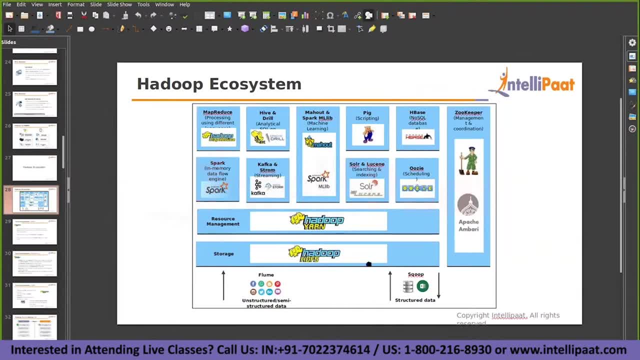 everything, the source for your storage will be hdfs, ultimately. okay. so there is no other layer or there is no other place where you're gonna store the data. i'll, it's only going to be hdfs. let's say i, i downloaded or i transferred some data from a relational database, emp table. 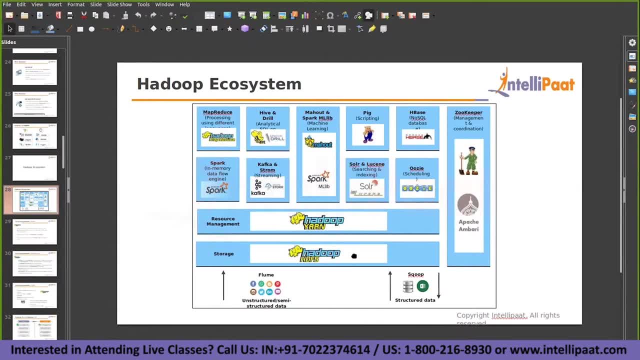 and i migrated it into the hadoop framework. now what i'll do? i'll do a select star from emp on hive right. so where is this file available? where is this data available that is available in hdfs? fine, okay, clear. the storage is available in hdfs. the emp related data in the table is available in. 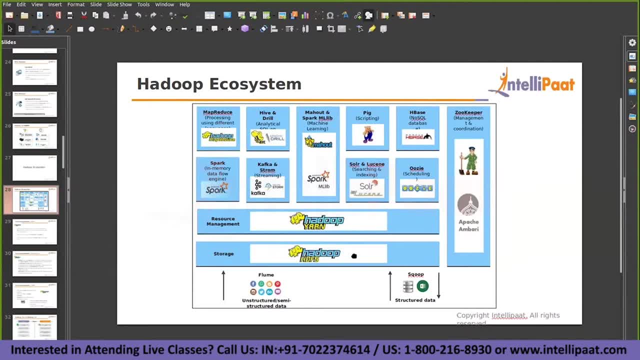 hdfs. but when i run a select star from emp, what i'm going to do is i'm going to do a select star. so what are we writing? we are actually writing a similar sql query and very known sql query- select star from emp. but internally what it is going to happen is it's going to convert this select star. 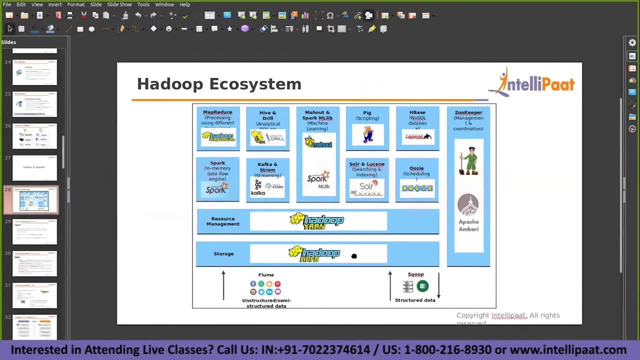 from emp query into a map reduce program. okay, so that is the reason why i'm saying so: the only way you can interact with the hadoop ecosystem is the way with map reduce. okay, so map reduce is with the Hadoop ecosystem, with the Hadoop components, with the Hadoop framework. what we 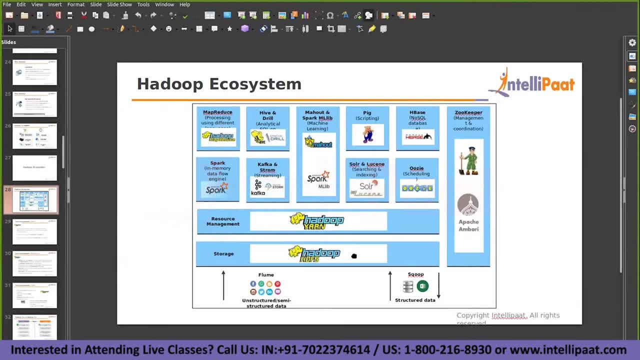 are writing. select star from EMP is for user convenience. okay, so internally it has to run via a MapReduce program only. okay, so ultimately the storage is HDFS. the processing is gonna be MapReduce, regardless of what. you write a hive query, you write a pig script, you write some. 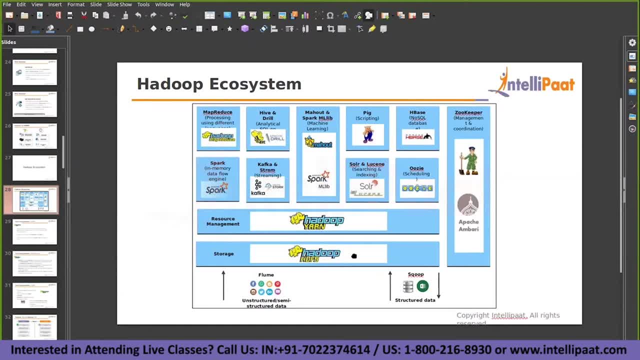 HPS to HPS query. you write some Uzi script, whatever right. so it has to be a MapReduce processing only. so whatever the query you write might change depending on the user, depending on the feasibility, flexibility of the users, but ultimately it's going to get converted into a 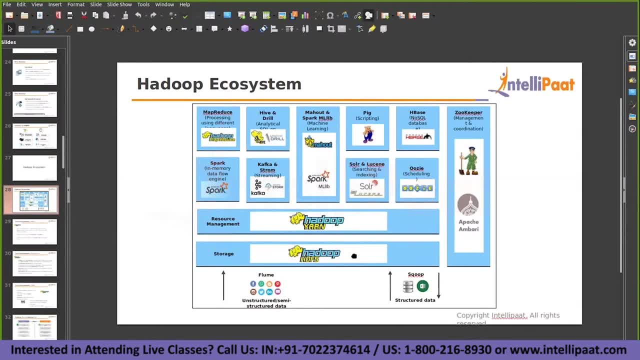 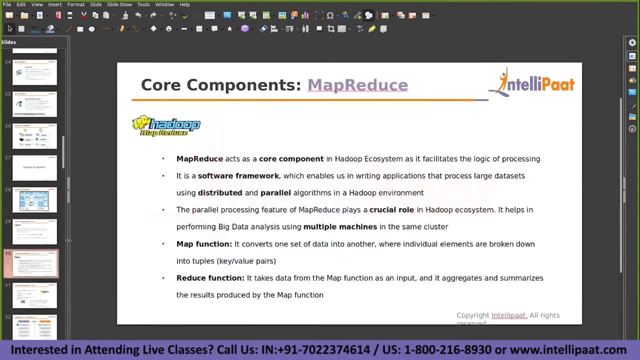 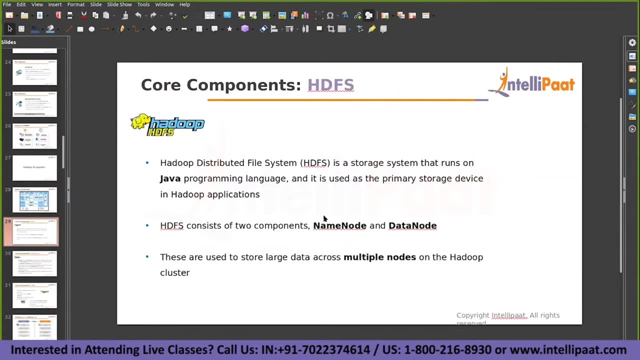 MapReduce program and it's going to execute on the MapReduce engine. there is a processing framework and all that, right. so that is what I wanted to tell. so the ultimate processing component is going to be MapReduce. it has to. it has two components again. like we have a name node and data node in in MapReduce. 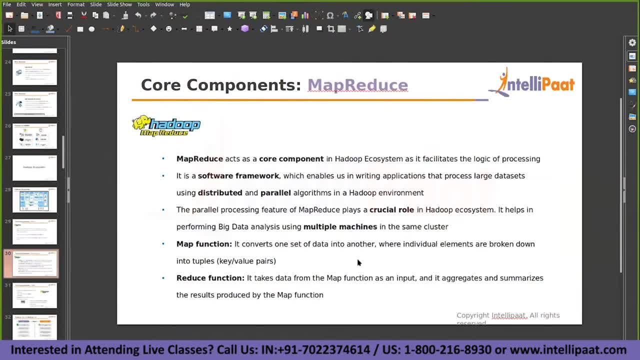 also, it has got two more components. one is the job tracker and the other one is a task tracker. so I don't think it is listed here, but the two more components, two more nodes, are job tracker and the task tracker. okay, so basically your MapReduce functionality is divided into two core. 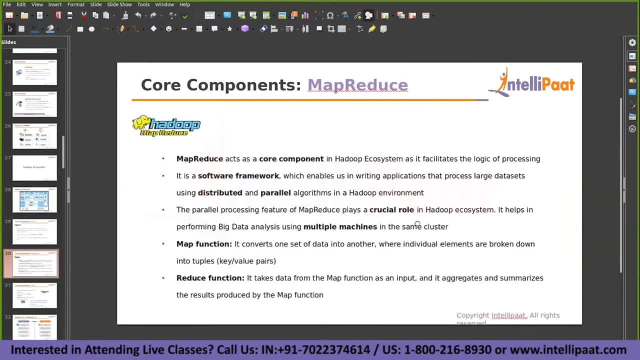 functionalities. one is the map function as well as a reduce function. okay, so we'll anyway discuss the architecture and the actual understanding of MapReduce. so let's not, let's not complicate it at this moment. so it's going to be a bit complicated for us to understand at the initial stages. okay, we. 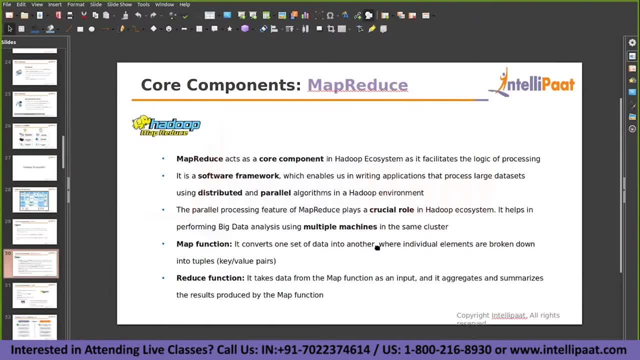 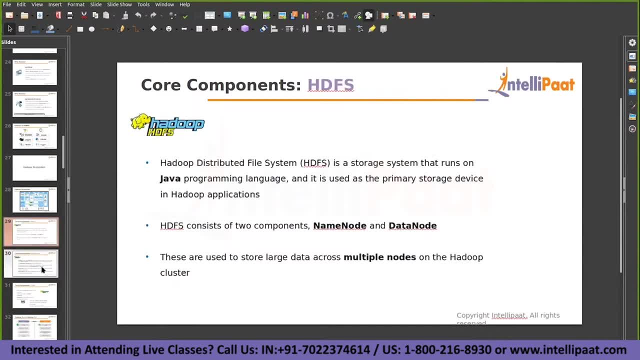 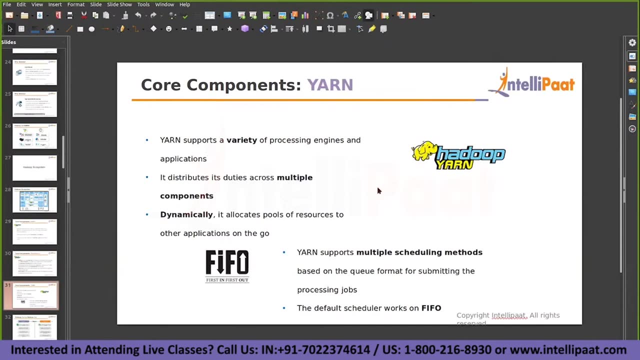 will discuss that. we will take this discussion a little later. okay, when we get into the core concepts. now are we clear with HDFS. there are two nodes: name node and the data node and uh, similar to similarly in yarn, you have resource manager and the node manager. there were two more. 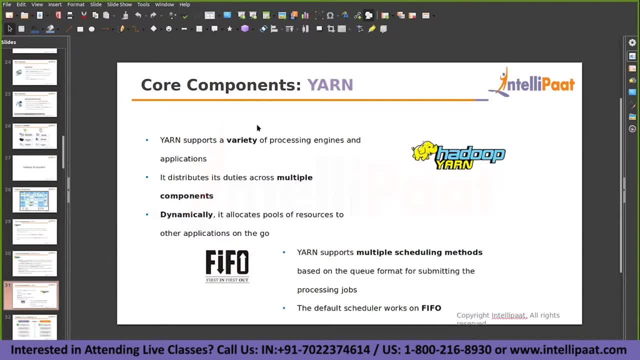 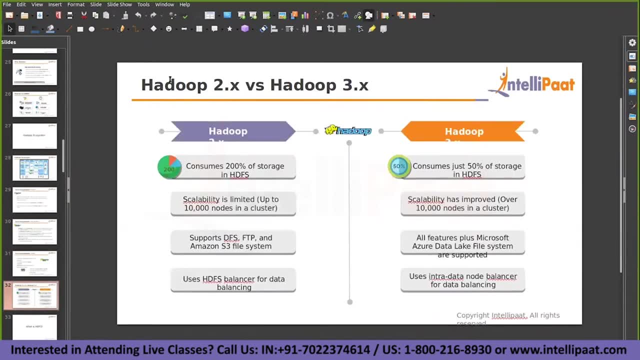 components. okay, so we will discuss about it. how yarn has got its importance, how is it different from MapReduce and all that? we will discuss about it in detail. okay then, so how do 2.x version versus hadoop 3.x version? so the the latest version that is running is hadoop 3.2, I guess. okay, earlier we. 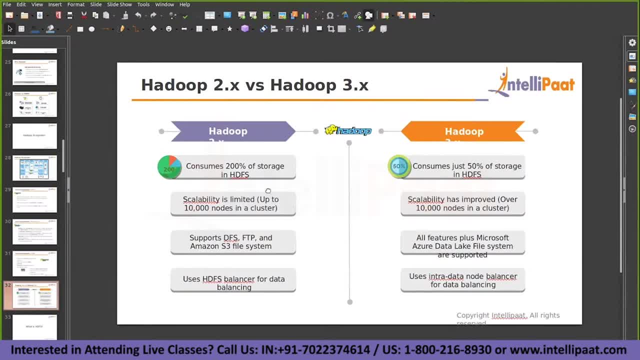 were working on hadoop 2.x versions and how is it different with the existing 2.x and 3.x? it consumes 200% of storage in HDFS. it only consumes 50% of storage in HDFS in terms of consumption of data and scalability is maximum. we can have 10 000 nodes. 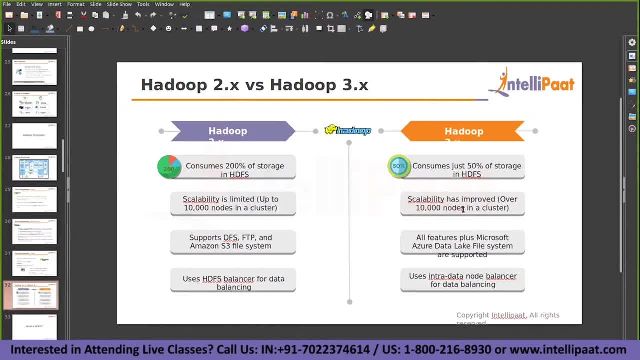 in a cluster and it has. it has gone beyond uh 10 000 nodes. you can have more number of nodes inside a cluster. see, in real-time scenarios, for us there is to be to be where we hardly work with systems which are around uh 100, 200 nodes at max, 200 nodes per cluster at max. but I mean, if you are, if you are lucky enough, you 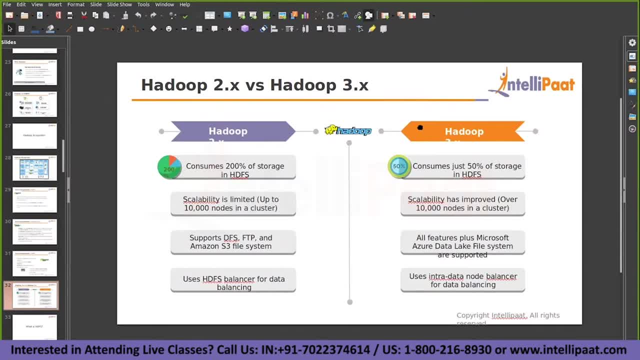 can deal with uh more, more number of nodes also, but you, being a developer, you will. you will nowhere see. I mean uh, you'll nowhere get access to see that, okay, these many nodes are available, these many uh nodes are configured in my cluster and all that information will not be shared to you. 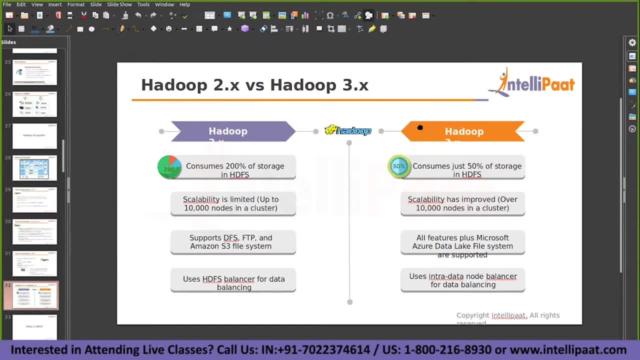 that's the admin job. uh, if you yourself is are setting the uh environment of hadoop, then you will be able to get a hands-on to it. okay, so the one which is installed on our local systems is a single node. hadoop, which is your local system, which is your local machine, it's running on a single node. 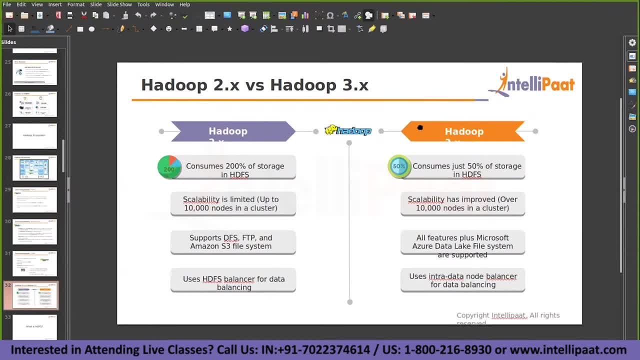 and the number of nodes can go up to 10 000 in hadoop 2.x versions and 3.x it. it has gone beyond. that's an additional feature that we've got right. so this is supporting um, uh, dfs, ftp, uh, s3 file system and all features, plus microsoft azure data lake file system are also supported. 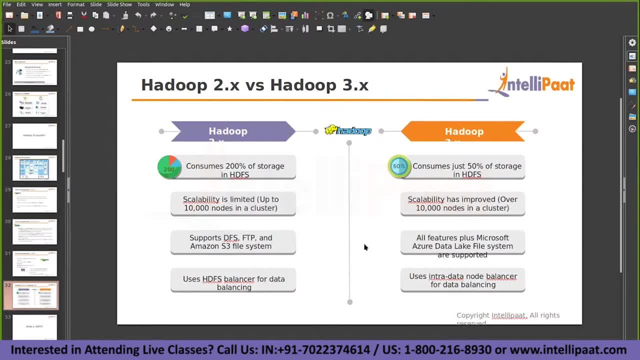 so why am I saying this? amazon s3 file system and azure data lake file system and all that is like- see um earlier. everything is an on-premise storage, agree, you know what is the difference between an on-premise and cloud? yes, right, so everything was within the 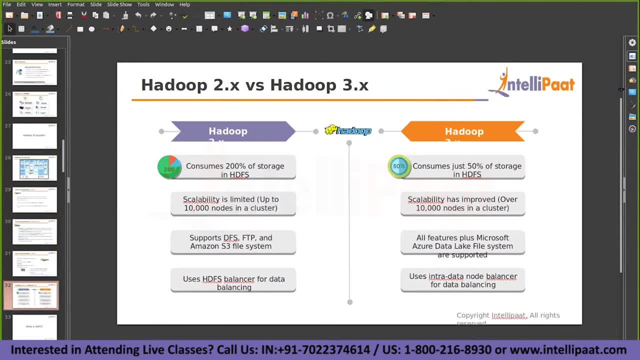 um, i mean, everything was physical storage that we had earlier. i mean, you yourself configure uh different nodes on on your uh work premises, right, you configure some 10 nodes, 20 nodes, 30 nodes and you can see this network drives and all that things. that is on-premise network. 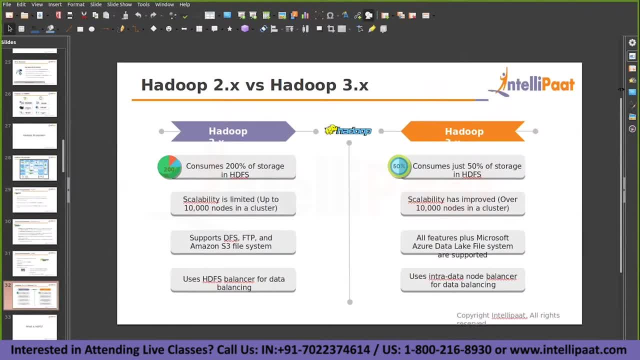 and compared compared to the cloud systems. like everything is a cloud storage now. so instead of you maintaining all this uh hardware at office premises, now you're going to be able to, everything is being migrated to cloud, so you you tell the cloud provider that you need some. 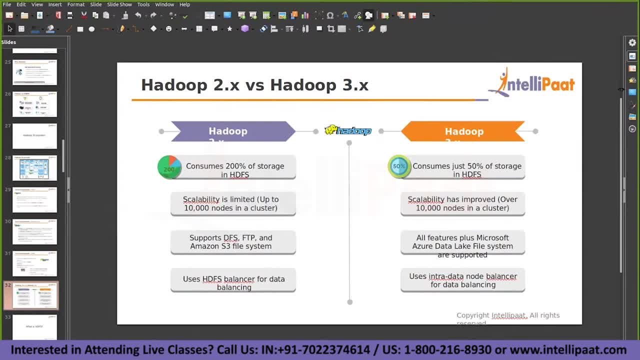 100 terabytes of storage and you would need some uh 100 to 200 cores to interact uh to the systems and they will charge you some amount and they'll give you the storage. you just need to use the uh host name or the ip address of those machines and you'll just interact with it, okay. 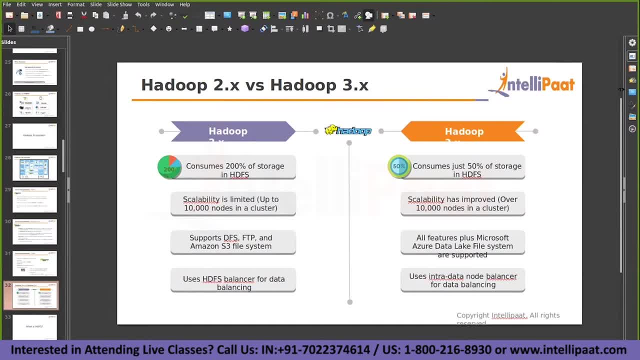 so there is no storage available at your premises here, so everything is cloud based. so that is the advantage we get using the cloud- this amazon or azure or google cloud like, for that matter- that everything is cloud-based storage now. so how your hadoop can interact with those cloud storages is what is is being provided, i mean in 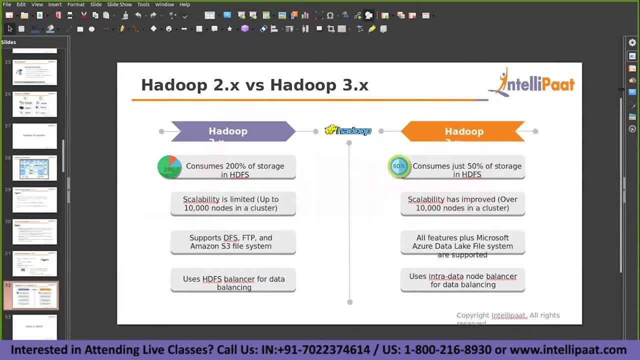 in the latest versions of hadoop you got this feature of interacting or using an amazon s3 as your hdfs or using hadoop azure data lake adls storages as your hdfs, right. so earlier it was all on-premise storage. you configured your hdfs, but now you can use the existing s3 buckets as your. 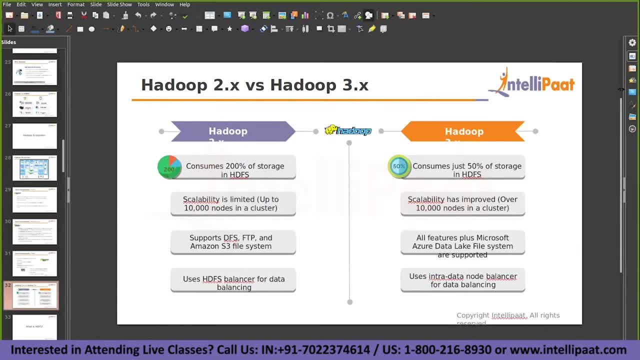 hdfs storage, so that feature is kind of added on top of the existing versions of 2.x and 3.x. okay, so in in latest versions you are, we are having the support for azure data lake storages as well. right, and in the earlier versions you are using hadoop hdfs as a load balancer- data balancing. 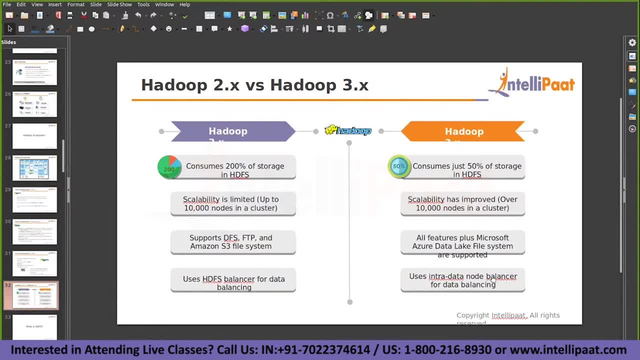 and now in the 3.x version, intradata node balancing for, uh, the data balance. so we will discuss about this concept in detail in the map. reduce architecture- pretty much okay, so let's not complicate it at this moment. so are we clear. so this is something which is out of context, guys, as the 2.x and 3.x, as we have not completely discussed. 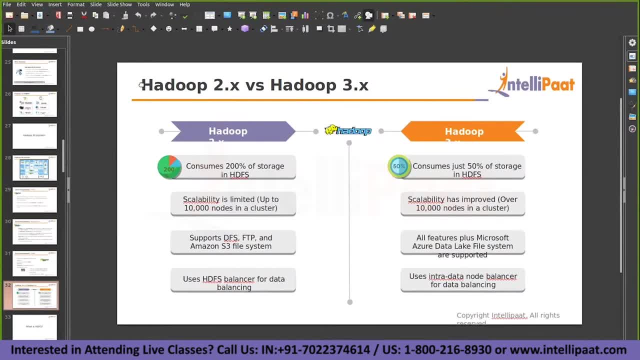 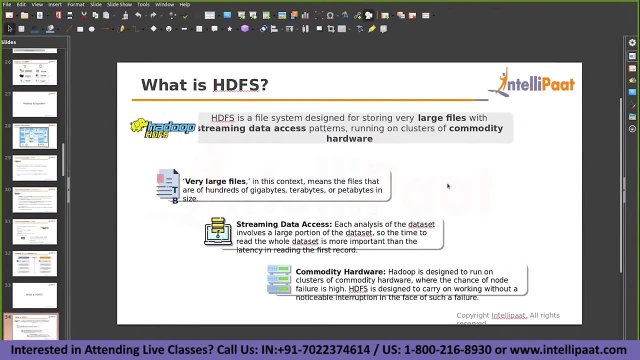 about the actual components of hadoop. we have not discussed about the core components of hadoop. we will discuss about it. then we will have a better understanding of what is available now and what is available in the later stages of it. okay now. so now going back to hdfs. so we will discuss the um core concepts of hdfs in this particular. 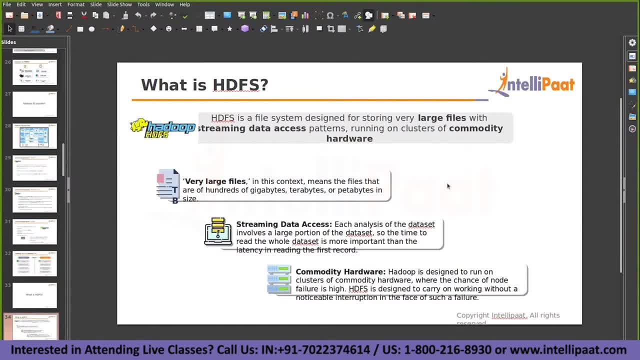 uh, slides for the next five to six slides. what hdfs is gonna do, what are its features and how is it being done? i mean, in terms of architecture, how do you, how do you take care of it? right? so we know it is mainly used for storing the data. so let's, let's just read. 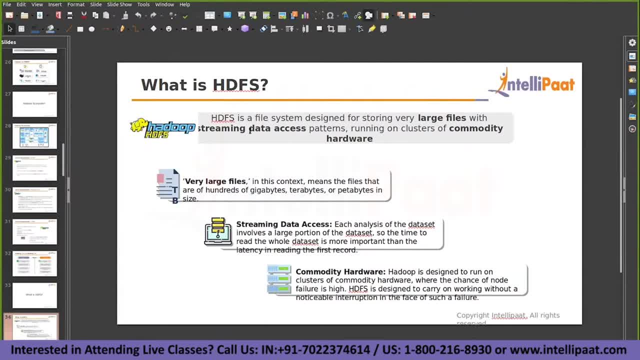 through the data definition that we have. hdfs is a file system designed for storing very large files with streaming data access patterns running on clusters of commodity hardware. so there were some terms that have been highlighted: large files is one, streaming data access and commodity hardware- okay, what does that mean? what is large files? so hdfs is primarily meant for. 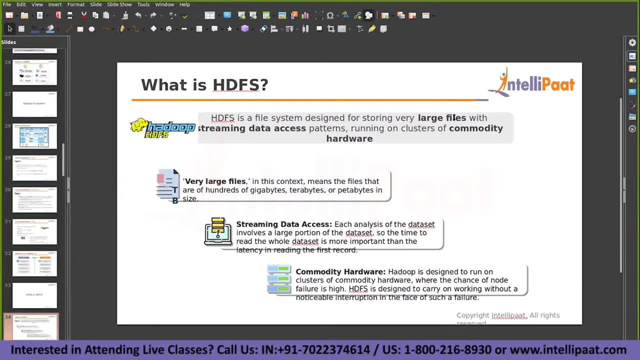 dealing with the large amounts of data set. so why am i saying? this is so? for example, there is a- uh, there is a storage requirement. okay, there is a 500 gb of storage requirement. on the first scenario, i have a one single file which is having some 500 gb of. 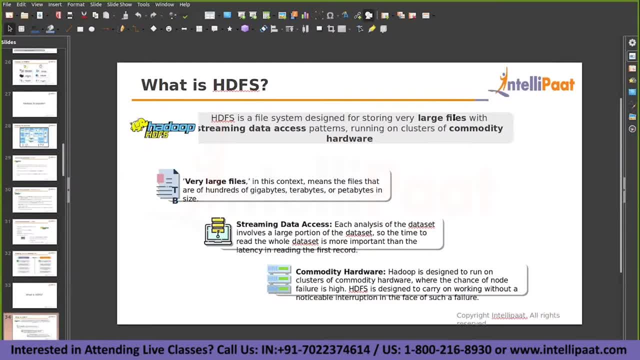 data: one single file. on the second scenario, i have some thousand individual files which are of 500 mb, each agree 516 or 508 or 512 or whatever the accurate numbers. okay, one scenario is, i have one single file which is of 500 gb or in terms of less number of storages. 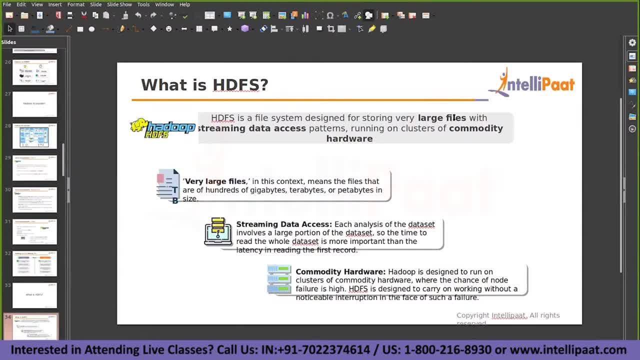 you have one single file of 500 mb and you have 1000 single files of 512 kb each. okay, so ultimately, both the scenarios. what am i using? which storage? i mean how much storage i'm supposed to allocate in both the scenarios. i have to allocate 500 mb of storage in both the scenarios, regardless of 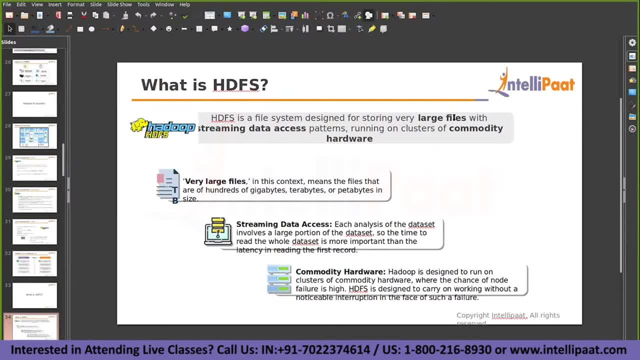 how many files i have. but the most preferred layer for storage is the first scenario, which is having the one single file, which is of 500 mb. so the reason why i'm i'm going with the first scenario is i'm not going with the second scenario. is huddup is meant or huddup is designed in such a 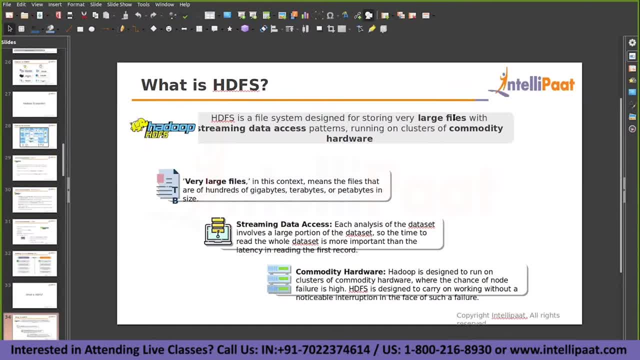 way that for each and every file you you load, you you write into the hdfs, there is some amount of metadata that is getting generated. so we will talk about it in detail in the architecture. but you know what is metadata? have you heard about this term? metadata? yes, no. so what is it gonna be? 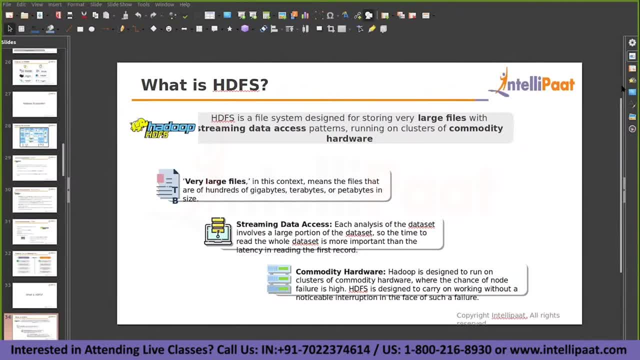 what is metadata data about data? okay, so it can be any information, right so, for example, in, in simple terms, as we are at the beginning sessions, right? so, in simple terms, for example, i'm loading one gb of one file of 500 gb, 500 mb. so what is it going to be? what is the source file? what is a? where is it? 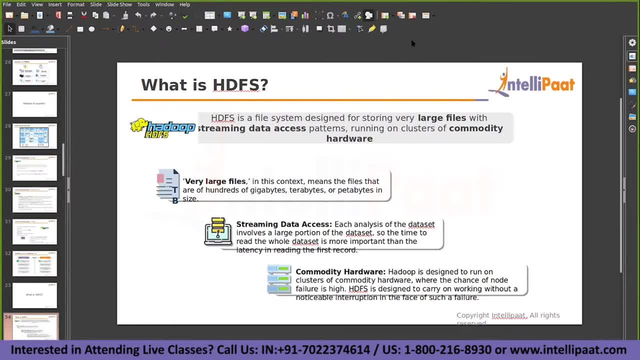 coming from, what are the number of blocks it has got, what is the information that it has got and how many number of records that it has got. so some information can be anything okay. so depending on framework, the framework it might vary. so some information about this file is called as a metadata. 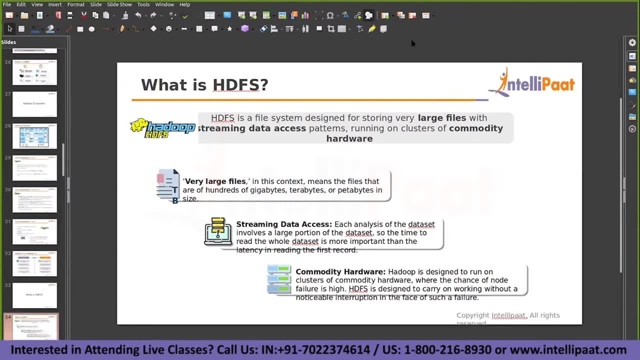 so hdfs, while you're writing, it's going to be a metadata, so you're going to have to write a metadata data into hdfs. it will create some information about this file. so that's going to be in some kbs. let's say, okay, so some information about this file it's going to create and it's going to store it. 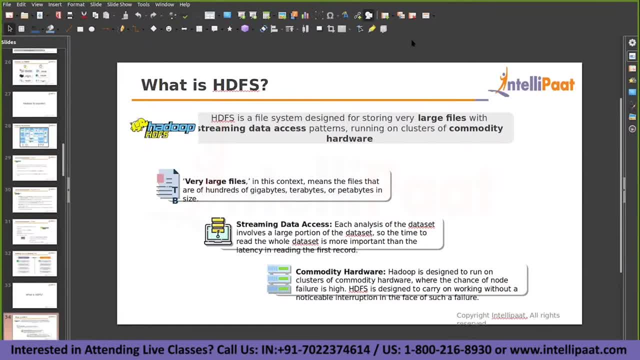 within the hdfs only. so okay, so if you are trying to access this file, this is the metadata information for it. so similarly, on the other scenario, when you have multiple such files, when you have 1000 such files, you are creating 1000 such metadata information. right, so that itself is actually. 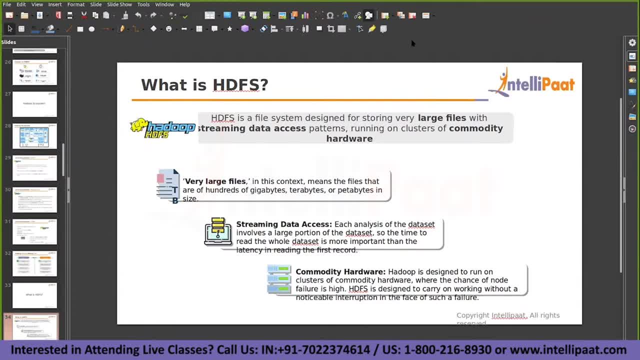 increasing the storage over a condition, right? if we are maintaining 1000 metadata information, 1000 metadata files, if am having around 500 kb of file and i'm generating some 100 kb of metadata, Touch, that doesn't make any sense for us, right? so if i'm storing some 100 kb of metadata for some 100 gb, 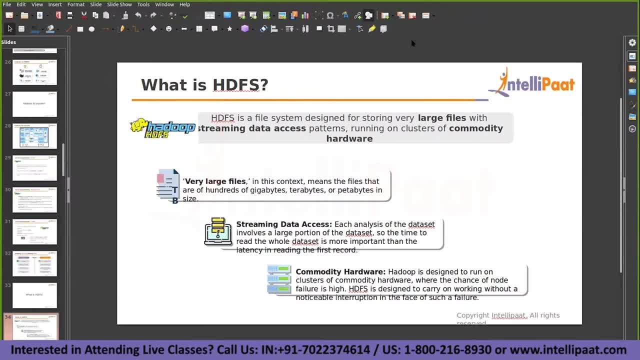 of data file, that's okay to handle. but if i'm only having 100 to 200 kb of file and i'm generating a 100 kb of metadata, that does not make any difference. that doesn't make any sense for us. so that is the understanding it needs to have. richt IDятьсяFile Metadata Vists offado a individual. 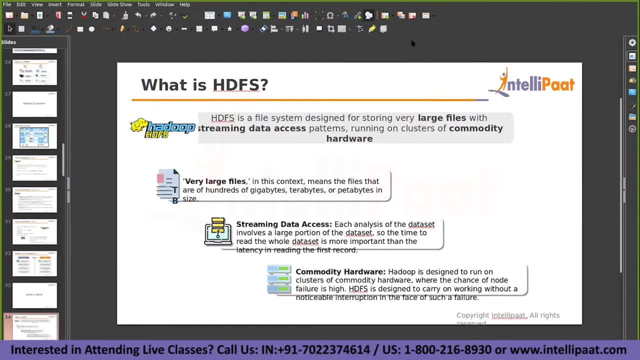 That is the reason. as it is generating this metadata for each and every file, it's preferable, it's mostly used. I mean preferably, you better use it for large amounts of data files rather than using it for small files. So that is the reason why we say that it's preferred to use large files. 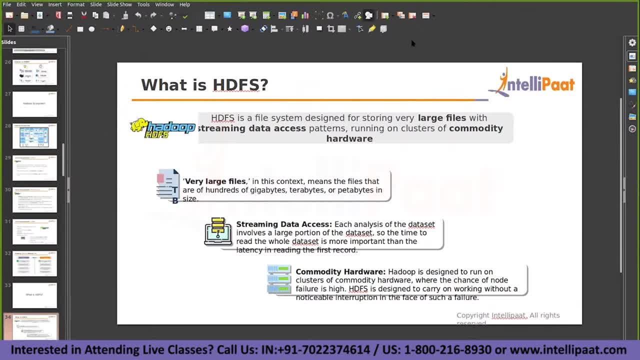 And there is something called as the streaming data access pattern, So we will discuss about it. I mean, this has to be when, how you actually write the data, how actually you read the data. the data is being written once and read as many number of times. 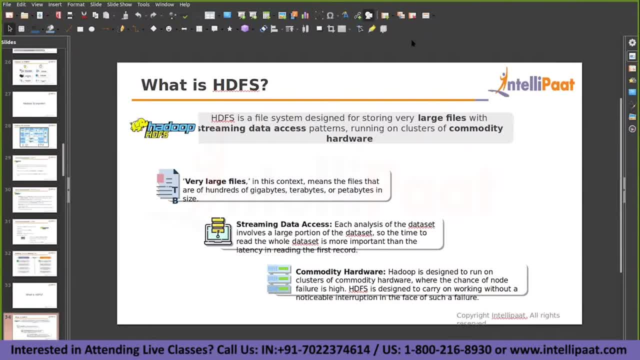 So this is how we write once and read many is the approach that we are going to follow. That means you only write once and you scan the entire data and you kind of read any number of times after that. So that is the advantage we get with the HDFS. 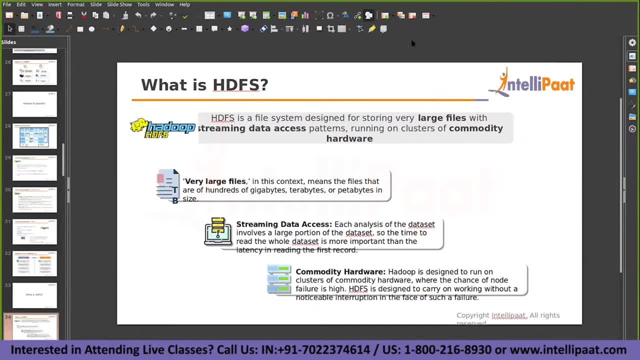 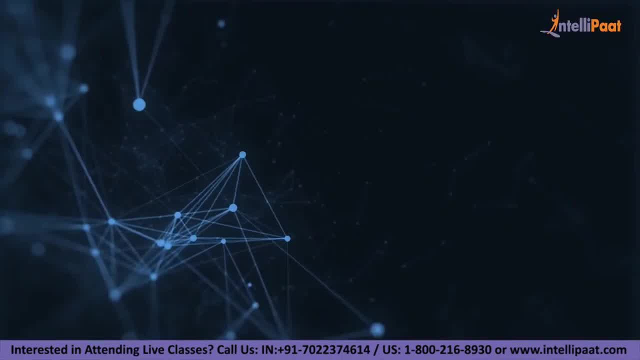 So this piece? we will discuss that in detail when we discuss about the architecture, how you write it and how you read it- And commodity hardware. did we discuss about this? Just a quick info, guys: If you want to make a career in big data, then Intellipaat provides an advanced certification. 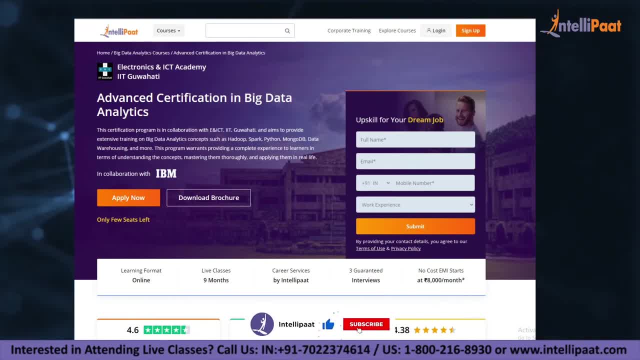 in big data analytics by ENICT council, IIT Guwahati. It is taught by IIT professors and industry experts with more than 10 years of experience. This course is designed to upskill and land your dream job. Now let's continue with the session. 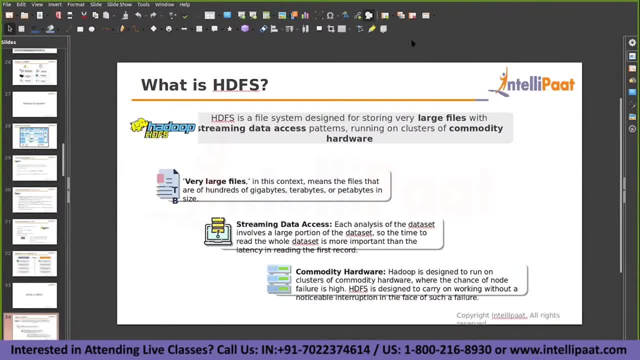 We know, we know what is this commodity hardware, right? So with the help of this commodity hardware, you are actually able to reduce the price of the entire cluster. Agree, So when we discuss about the legacy systems, the expensive component, using this commodity? 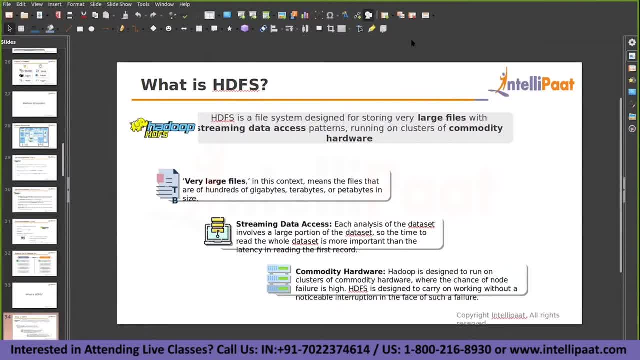 hardware. you are kind of taking away all the advanced features of your hardware. You're not even installing any high-end software on top of it. You just need a basic hard disk to store some information. That is what we call it as a commodity hardware. 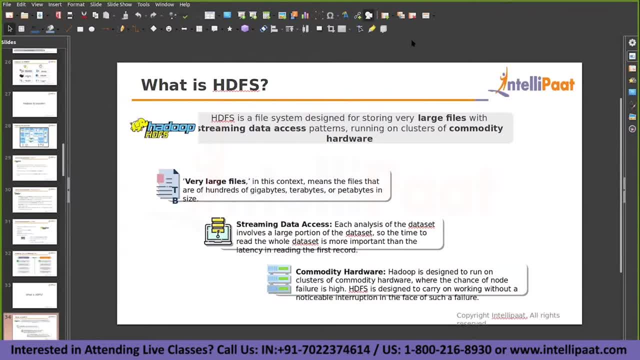 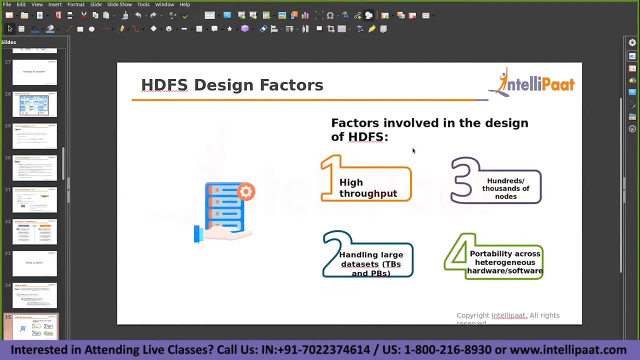 And how is it helping us? We are able to reduce the price of the entire cluster using this commodity, hardware. Okay, So these are the three components, or three main features of your HDFS And when you're designing your HDFS here. okay, 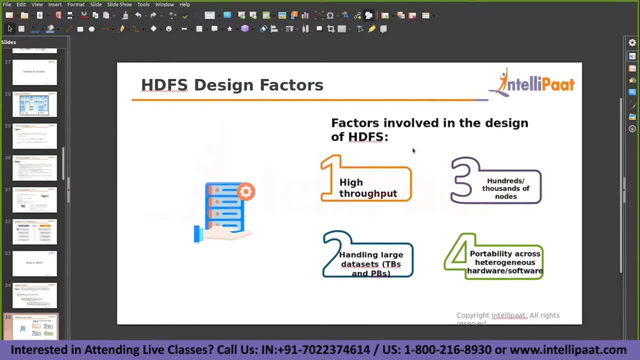 So, for example, you are setting up your own HDFS component. What are the things that you're supposed to look into or take care of? is what this design factors is going to let you know. So: high throughput, hundreds and thousands of nodes and handling large data sets. portability. 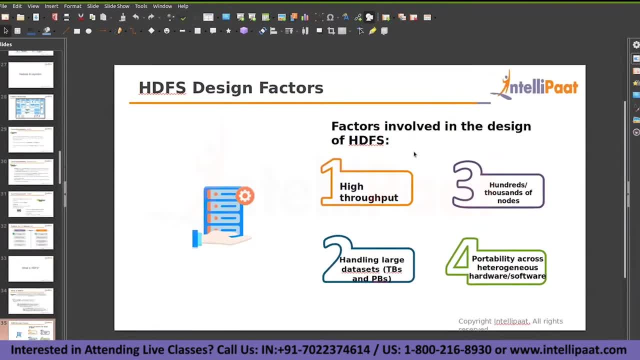 across heterogeneous hardware or software. Okay, So what does this throughput mean? Anyone, What do you mean by throughput? Okay, Yeah, So the amount of data in simple terms, the amount of data that we read or write at a specific instance of time. I can say in simple terms, right. 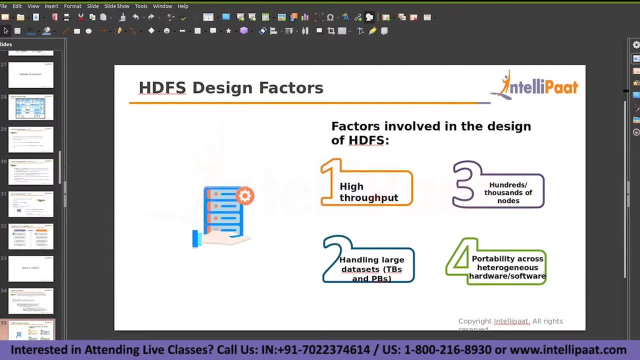 So right. So, for example, I have a single node, I have a one single input output port, right, So I maximum I can read 10 MBs per second. Okay, So that is what my throughput I call it. 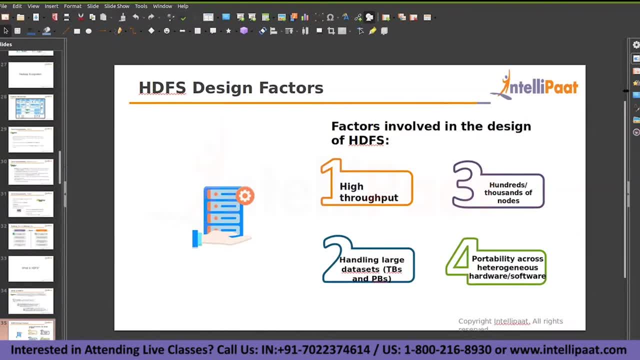 So when I have two nodes, that means I can read 10 MBs from one node. 10 MBs from two nodes, What is it going to be? 20 MBs on a whole is my throughput. So when I have multiple nodes like this, so the throughput with which I can read the data, 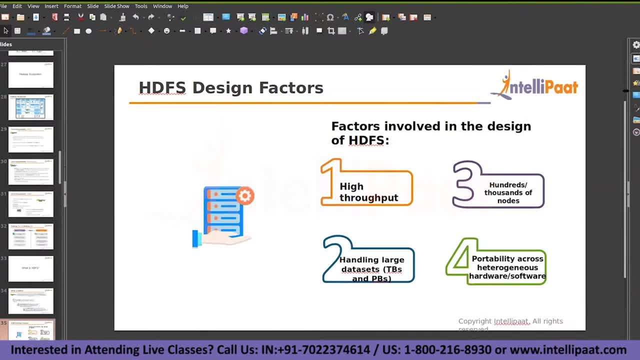 from these nodes is very, very high. That is one of the advantages that we get here. So write is not going to be faster, but read is definitely going to be faster, because when you have multiple nodes, the write is happening in a sequential order, but the read is happening. 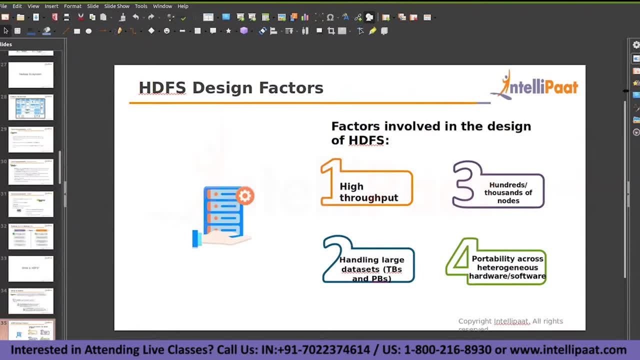 in a parallel order. Okay, So sequentially, as in like: you write the data one after the other one node, you write it, Then, after filling the entire node, you move on to the next node and then move on to the next node. But when you're reading the data, you can read the data across all the nodes at a single. 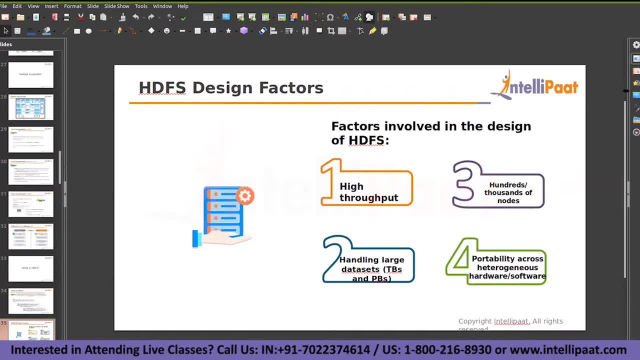 point of time. So you, you have a very high throughput here, very high read throughput, I can say Okay. And you have the feature of you have the capability of handling Hundreds of thousands of nodes, as just a while ago we've seen the slide, uh, the 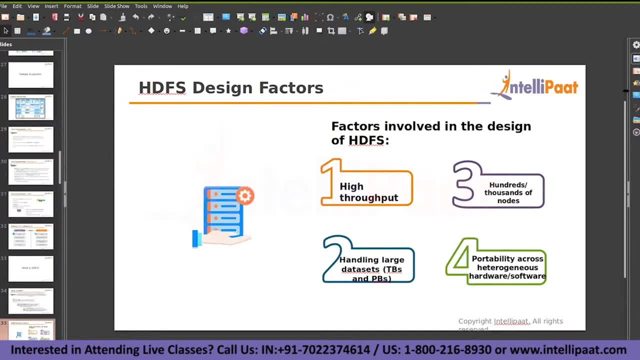 the version two dot X has the capability of storing up to 10,000 nodes, configuring up to 10,000 nodes in the cluster, whereas in three dot X it has gone beyond the 10,000. So that is the number of nodes that we have and handling handling large datasets in. 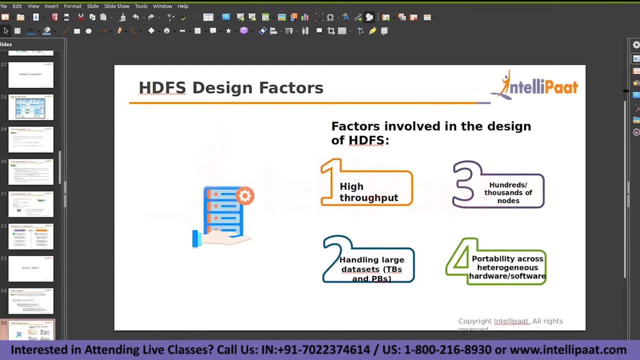 in terms of TVs and PBS. That is the advantage we get right. Just a while ago, we discussed about the advantage of reading large data files. correct, We we hardly Uh generate a very small amounts of metadata for it, and it's it's um feasible or it's. 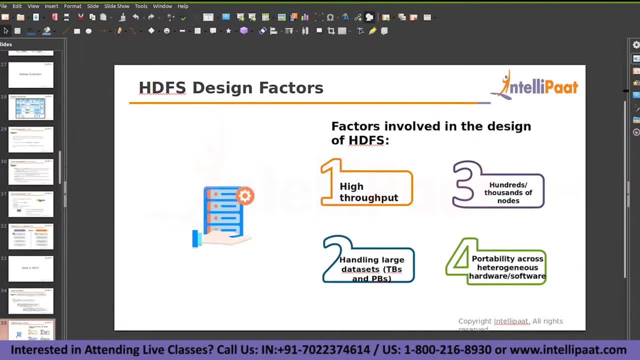 preferable to to deal with a large amounts of datasets and portability across heterogeneous hardware solutions. We know what is this: heterogeneous systems. we discussed about it, uh, a while ago in the features Um, the, the effective way of reading with the heterogeneous data sets is also available. 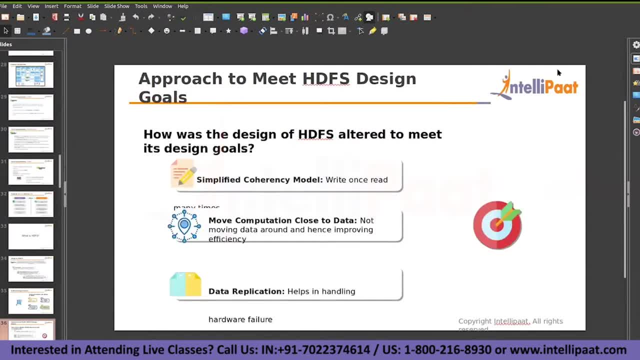 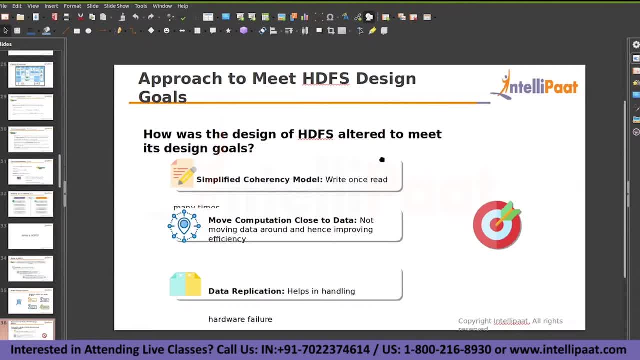 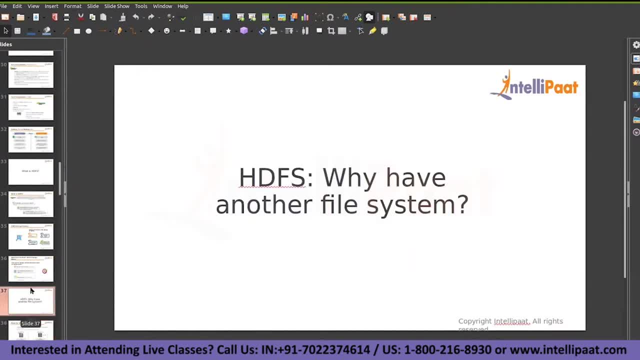 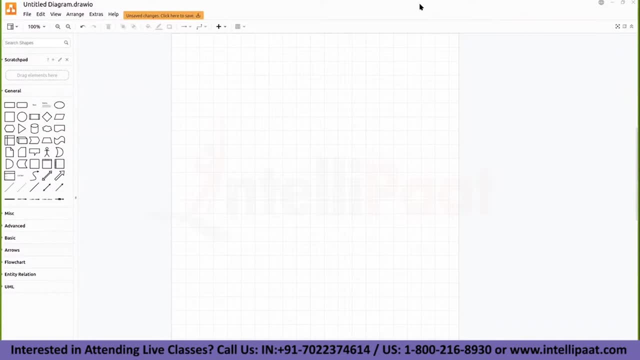 that we discussed. OK, So any questions, guys? so far Architecture of HDFS. So at least we know initially, I mean, at least, with whatever understanding we have- we know that there is, this is used for storage and the entire data that we terus storages. 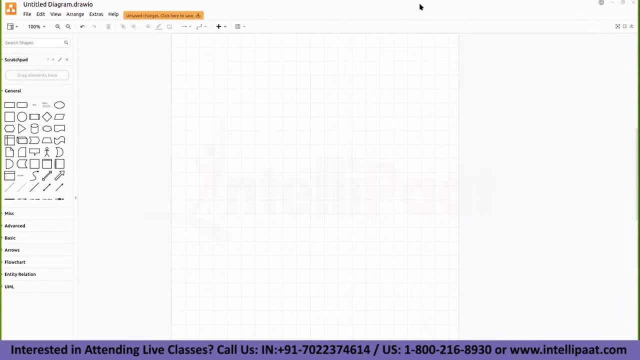 is available in the hadoop platform is supposed to be stored in htfs. so how the data is stored, how it is being accessed, and everything we will discuss. we will see that so fine. so, uh, we have discussed about two components, right? what are those two components, right? so, first one is the. 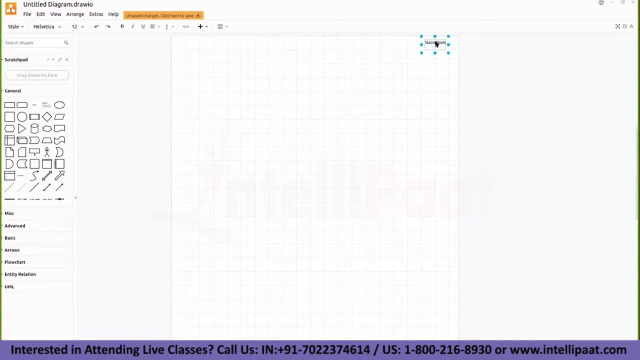 name, node and data. no, these are the two components in my hdfs, the major components in my hdfs. right? so the architecture of hdfs is a master slave architecture. so what do you mean by this master slave architecture? there is going to be one master and rest. 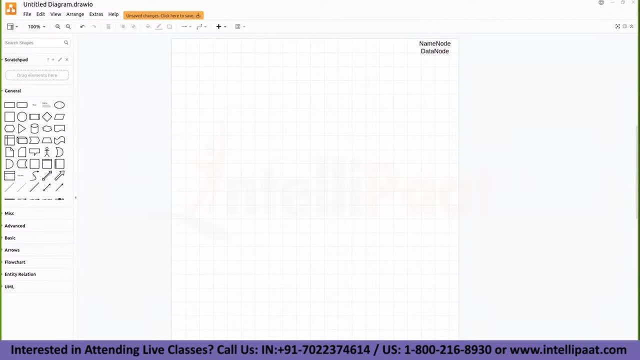 all will be slaves. okay, so when you are writing the data or reading the data, see, we know that there are some hundreds of nodes available inside your hdfs, right, so it's a distributed platform. we have a cluster. inside the cluster, we have some hundreds of nodes. 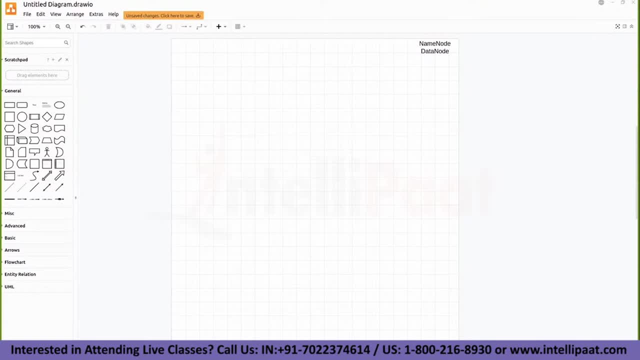 some thousands of nodes, right? so when we have so many number of nodes, how do you maintain the configuration or are managing managing of all these nodes? see, when i'm supposed to load the data, how do i decide that in which node i have to load the data? 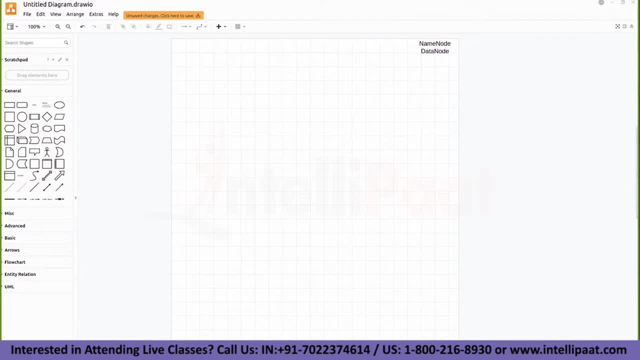 when i'm supposed to read the data. how do i know that which node has so and so information? right, so there has to be one system which actually has to take care of all the admin related activities. i can say: okay, if you are writing the data, okay, you go and write on so and so number of 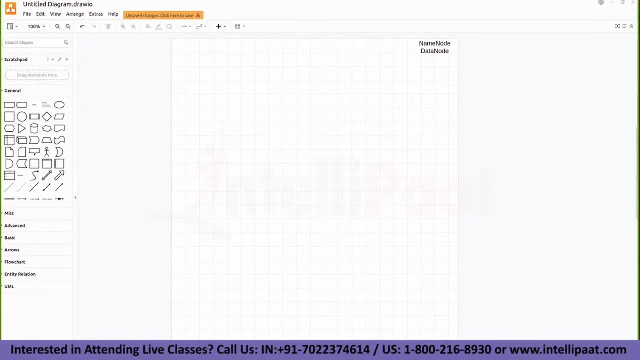 nodes. if you are reading the data, if you are looking for this information, you can go and read from so and so number of nodes. right, so there has to be one machine, one master inside your cluster, which which pretty much has to own all the operations, all the read and write related. 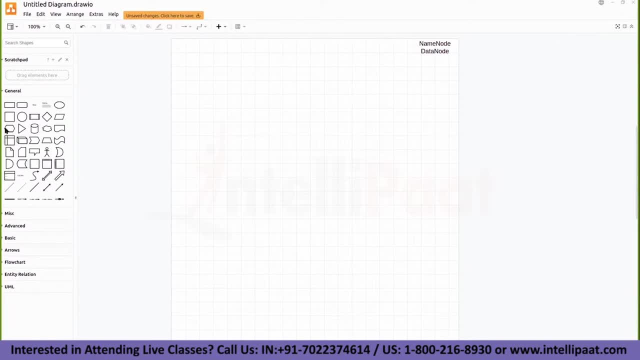 operations. so that is why this hdfs has been designed in such a way that it it it is going to have a master and it's going to have a slave as well- these number of sleeves. so this is my slave node and this is a another slave node. 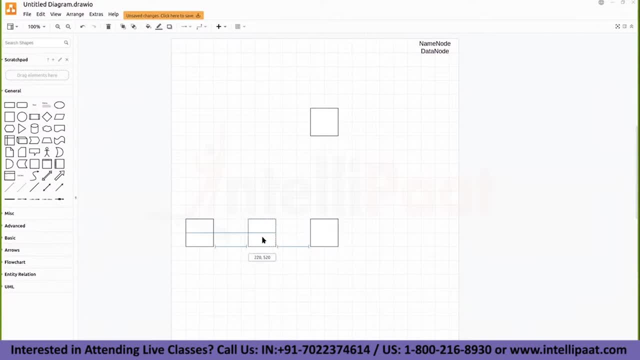 this is my third slave node and this is gonna be my fourth slave node. this is gonna be my fifth slave node, so i have one master. uh, i can increase the size. it's better, because we are going to supposed to write some blocks, we are going to supposed to draw some blocks inside it, so it's better we increase the size. 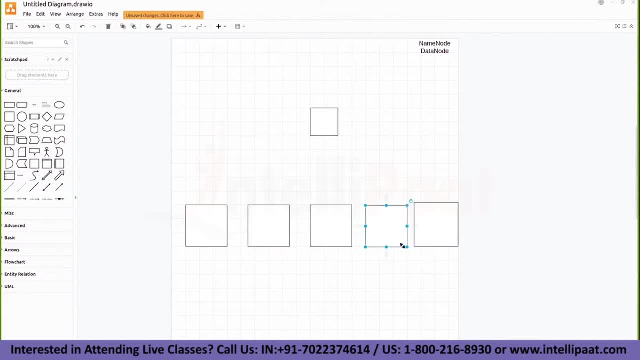 okay, so these are the nodes that we have, so i'm gonna name this the master, which is my name, node right, all the other nodes are the data nodes. okay, so all these are the data nodes. fine, so now i have to have some connectivity between these nodes. 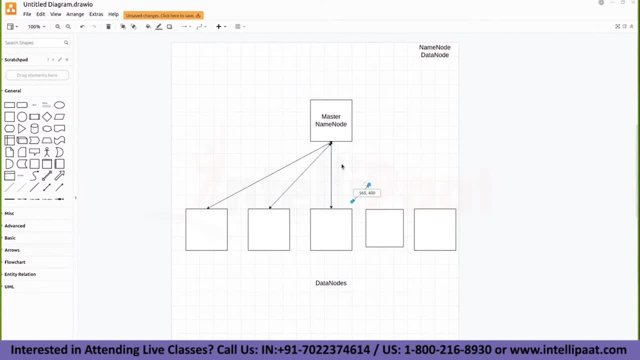 each and every node should have. everything is connected to the master, all the data nodes. so this is my master and slave architecture, right? one master is connected to all the slave nodes. so now my, what is my cluster size? so if i have to write some text here, 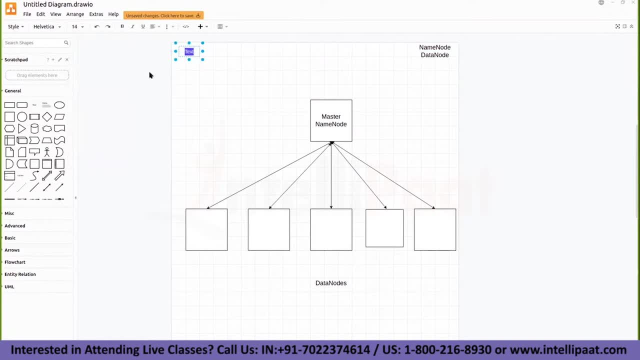 let's say, i'm writing some text, so this is my cluster. are you able to see this? my cluster size is um six nodes right: one, two, three, four, five and six nodes. this is my six node cluster size. six nodes and what else? what else? let's say the uh storage. 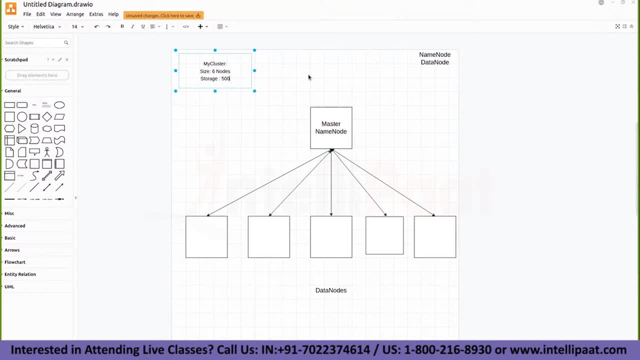 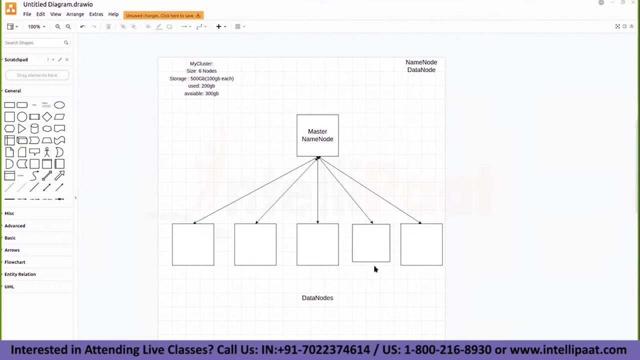 storage is around 500 gb and 100 gb each, and used is, let's say, some 200 gb, available is some 300 gb. are we clear? this is my statistics for your cluster. are we clear? this is my cluster, hdfs cluster, which has six nodes. uh, one is the master, all the other five nodes are slaves. 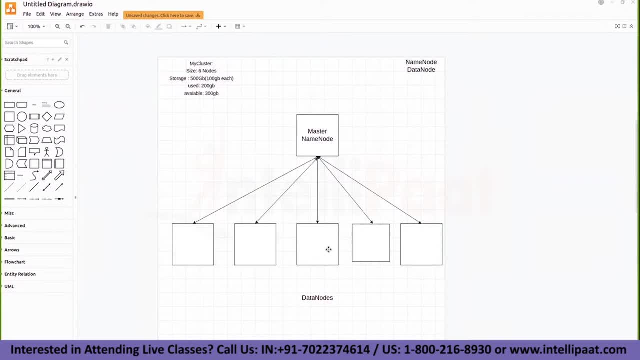 and we are only going to consider the storage available on the slave nodes, on the data nodes, as the capacity. okay, so 100 gb each. i have 500 gb of storage capacity available and out of which 200 gb is already used. okay, so my cluster is already in use and 300 gb is the available storage. clear now. 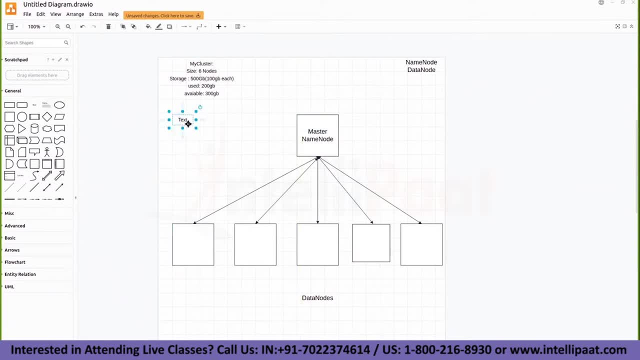 there is one more scenario. so here i have hellotxt file, which is of 100 gb, which is supposed to be written into my htfs. okay, so this hellotxt file has to be written into, has to be loaded into my hdfs. that means, whenever i am trying to 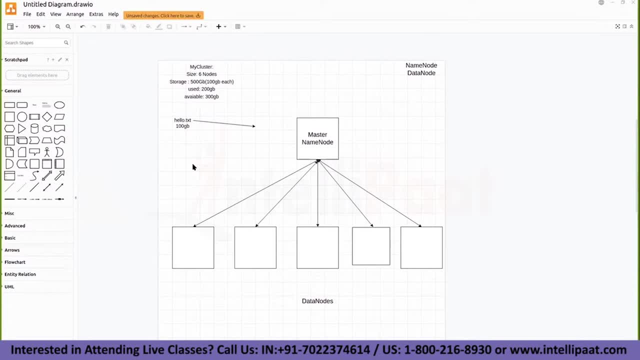 write some data into htfs or read some data into htfs, the requests which are supposed to be sent will ultimately reach my name node, the master. So when you're saying that you're sending a request to write some data into HDFS, that means you're sending a request to the name node. 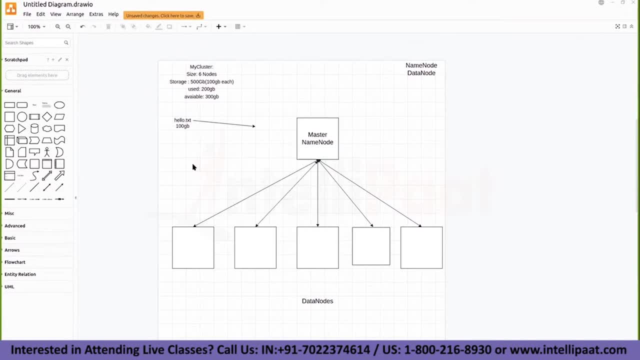 Or when you say you're sending some request to the HDFS, that means you're sending a request to the name node ultimately. So I have a request to load some 100 GB of data in your HDFS. So first, when I send this request to the HDFS, 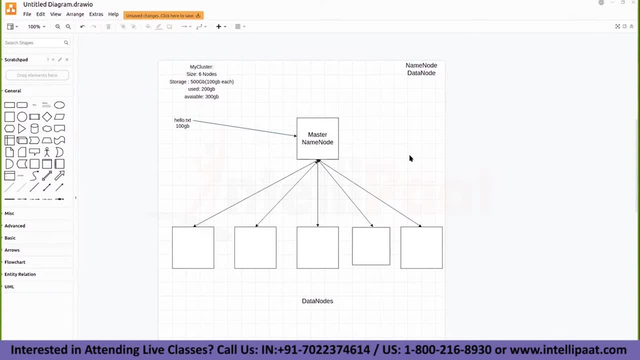 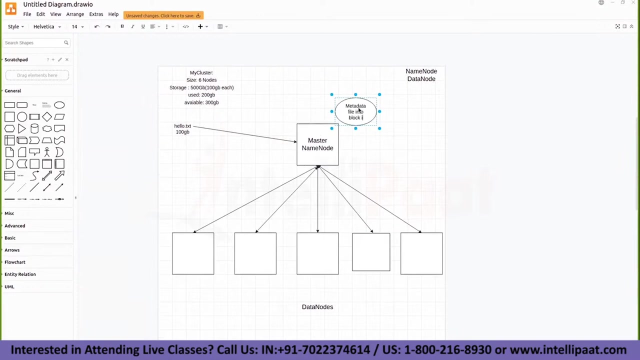 it's gonna come and hit your name node ultimately. So what is your name node gonna do? So name node internally will have this is internal to name node. okay, Will have metadata. So what does this metadata consist of? Metadata consists of file info, block info. 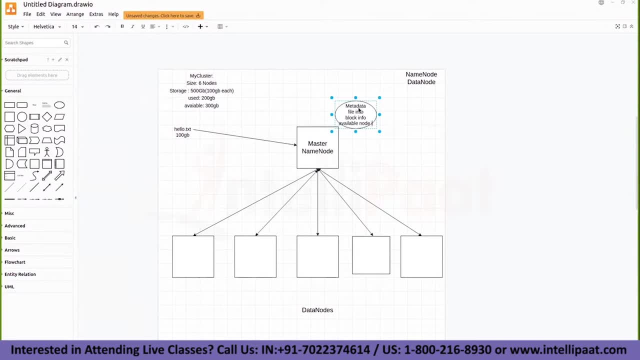 available node info. So what does this mean? So it's going to hold the information related to whatever the number of files that are written to your HDFS. what data is written to your HDFS? what are the number of nodes that are available? 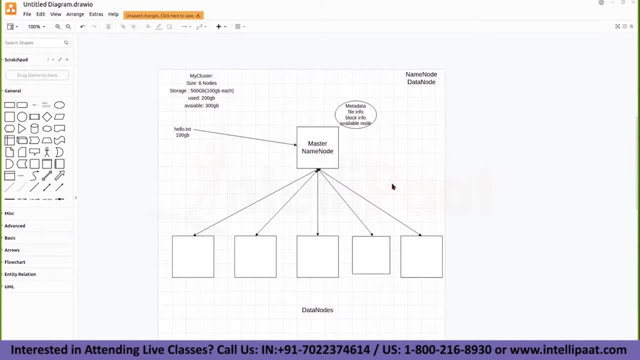 just to be stored, and in each and every node, how much amount of data is being, how much amount of storage, how much data is being used. All this information will be available inside your metadata, agreed? So when I say that I'm supposed to write some hollowtxt. 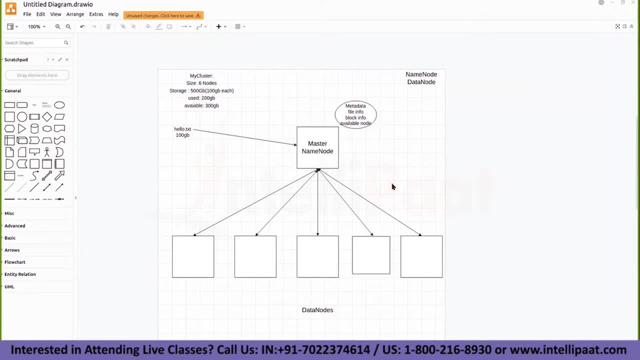 which is a 100 GB into your HDFS. what my name node will have to do is it will first internally read the metadata for the available storage, So it will check whether the data is, whether we can accumulate this 100 GB of data in your HDFS. 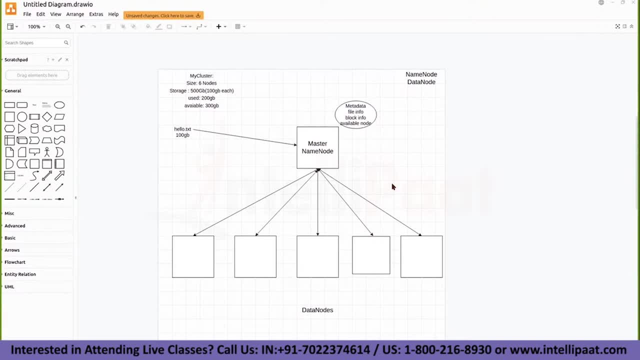 So what is it gonna do? My cluster information is going to be. information says that it is available. it is available. storage is around 300 GB, So I have 300 GB of storage. then I can definitely store 100 GB of data. 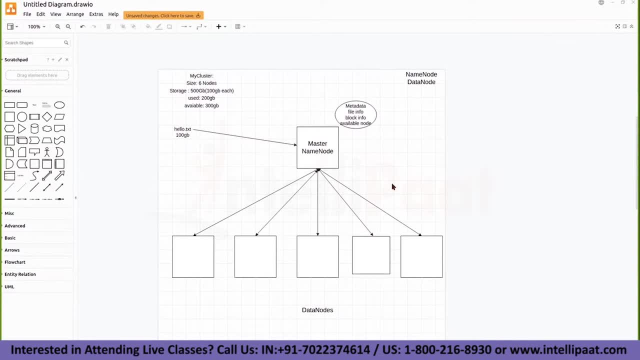 So I can definitely store 100 GB of data, but in which node I have to store it? Yes, Which node has the availability to store 100 GB of data? So now, with by looking at the metadata information, I'll identify: okay, node one, two and three. 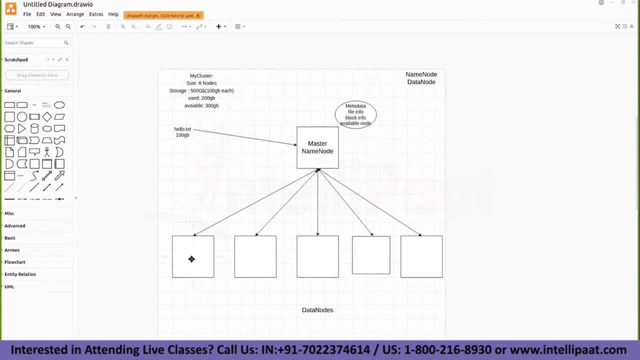 have the necessary storage to load this 100 GB of data. All right data. so now i'm selecting node 1, 2 and 3 to store 100 gb of data, hellotxt file. so now what it will do: your master will grant access to your hellotxt file to the writer, to the writer to go and write. 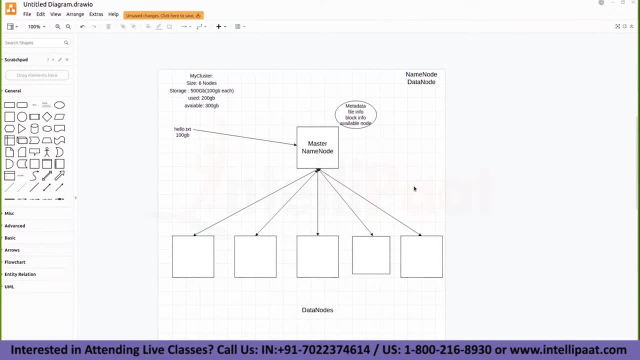 on these three nodes. so how is the data going to be written? the data will be broken into multiple blocks. so every blog, every data file in hdfs will have to be written in the form of blocks, individual blocks. so each block consists of 64 mb or 128 mb of block size. that means when i have 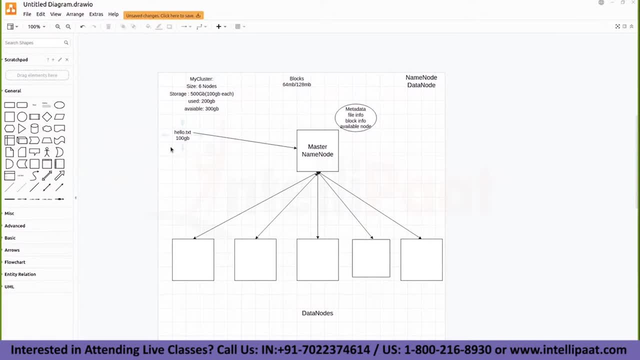 100 gb of data. i'll break that into multiple blocks of 64 mb or 128 mb. so this is the default block size of your hdfs, So you can upgrade it to 128 mb. i don't think it's. it's going beyond 128 now at this moment. 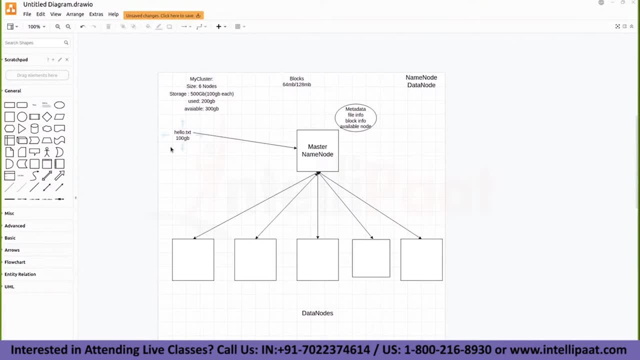 so earlier it was only 64 mb, now it has got the uh, uh privilege, the uh feature, to upgrade it to 128 mb. so now, whatever the data you have, you will divide that into 128 mb of blocks. so how do you, where do you configure it? you will be configuring the cluster information. okay, you will be configuring. 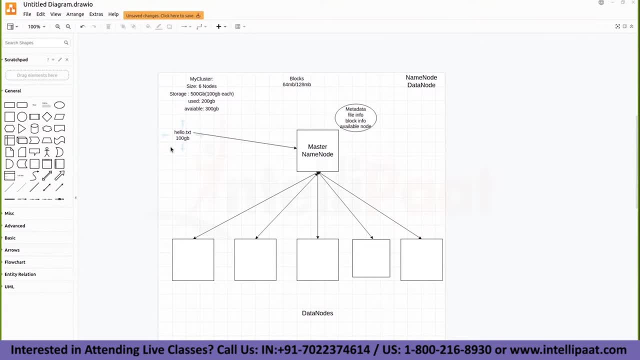 it there and? um well, depending on the configurations of your hdfs cluster, if it is 128 mb, your data will be divided into multiple 128 mb of blocks. so where are they going to be written? now? each and every block of data will be loaded into your data node one, two and three. okay, so let's say i have this one. 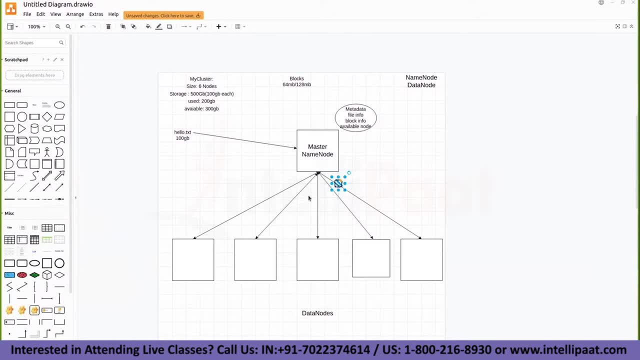 i'll take small blocks. this is one getting it. what i'm trying to do? i'm just dividing this data into multiple blocks and i'm just trying to write them into your hdfs storages. okay, it's difficult to create so many blocks here, so just just um. just let's assume that i have written some 100- 128 mb blocks of data into these. 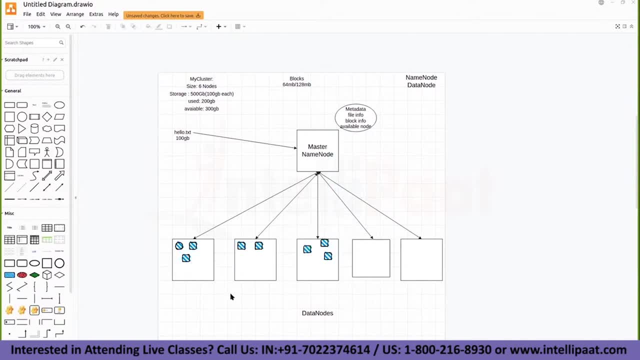 nodes. okay, right, so now i have, uh, uh, loaded this data into the data node and i'm just trying to data into these three data nodes. hollow dot txt. after you load this data, you are supposed to load the replicas also. when and as and when you, as and when you write this: 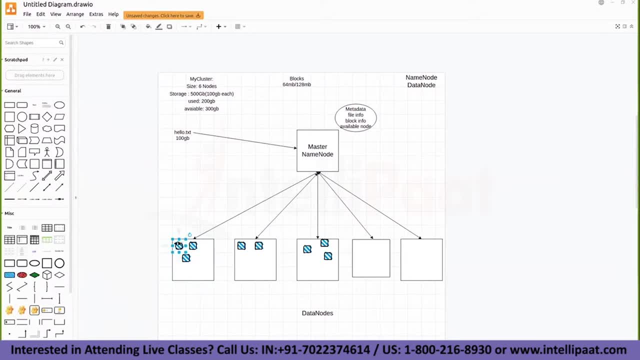 data block into so and so data node. the replica of it will be written on the other data nodes, so this is block one. i have written that into this data node. now i'll load this replica on the other data node and, as and when i write this block, i'll load that replica on some other data node as and. 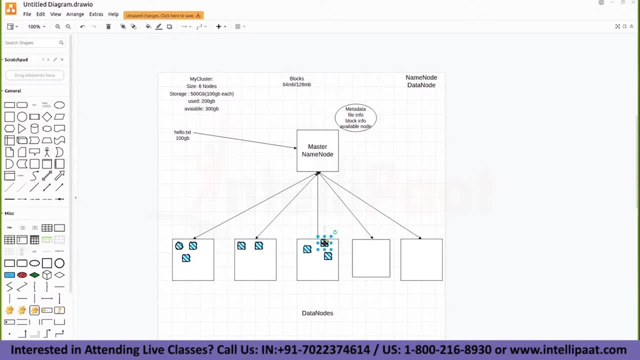 when i write this block, i'll be loading it on some other data node. so as and when you are writing the blocks into your htfs data nodes, the same time your replicas also will get created on the other data nodes. so depending on the replication factor again. so here we have. we might have missed that. 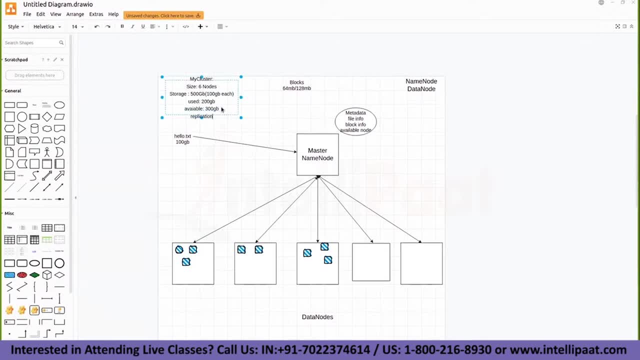 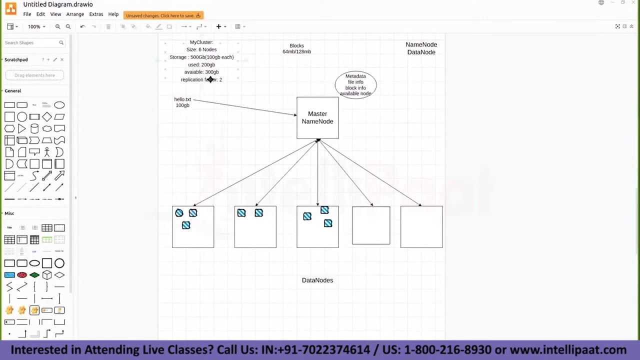 replication. so let's say, replication factor is what? two- this is my cluster information, right? so my replication factor says that i have, i. i have written the data. i have to replicate the data twice. so after i write the data on one particular node, i'll be replicating it into other data node. simple, okay. so like this, i have written all the 100 gb of data. 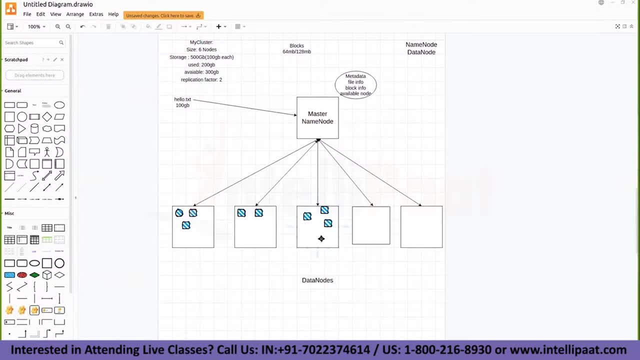 on all these three data nodes and i have replicated in on so and so data nodes. okay, so now my cluster information will change. so now my metadata information will change. so this entire thing is your metadata, let's assume. okay, so my cluster information will change something like: 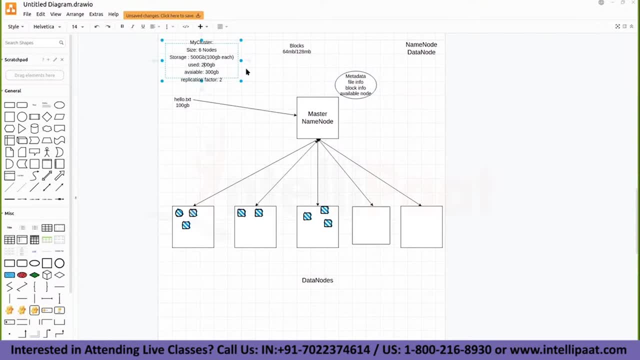 this. so your availability is around used is around 300 gb and your availability is around 200 gb. is it 200, 300, no right, 400 and 100, because it is replicated. 100 gb is the original copy, 100 gb is the duplicate copy. so now you have almost used 200 gb of storage. 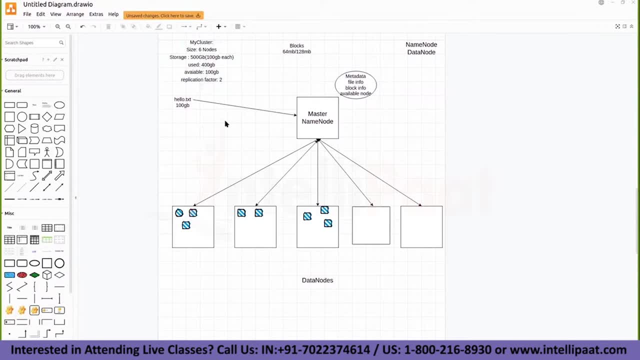 in this. so your used will be 400, availability will be 100 gb getting it. so now you have written the data, you have performed a right operation, okay. so now, when you are supposed to read the data, same hollowtxt. now, when you are supposed to read it, i'm. i'm coming now to read the data. so what do you do? you again send a request to 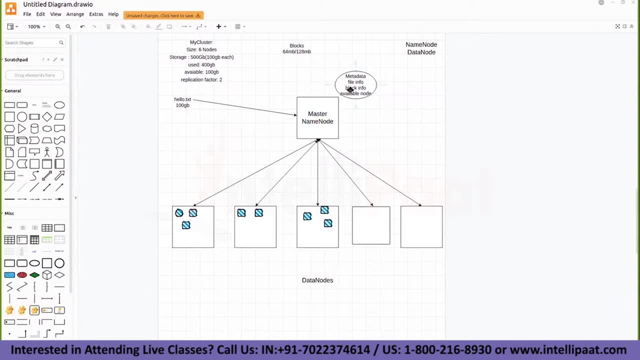 the master name node. again, name node will look into the metadata uh. look into the uh name node metadata information and it will identify that. okay, this hollowtxt is written on data node one, two and three so that your read request will go and read the data on top of this. 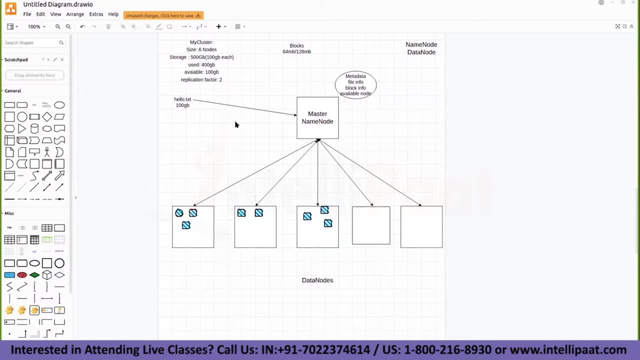 three data nodes. so your hollowtxt will be read from these three data nodes parallely. okay, earlier it was sequential, now you read it parallely. okay, this is how your data write and read operation will be happening. in addition to this, there is also this health kind of health check signal. so at regular intervals, let's say around. 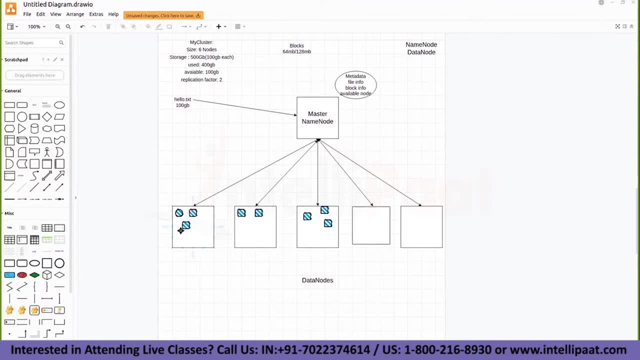 for 10 minutes once, or 20 minutes, uh once. at 10 minutes interval or 20 minute interval, your data nodes are supposed to send a heartbeat signal to your name node saying that they are alive. i mean, if the data node does not send a heartbeat signal, that will assume this data node to be dead. 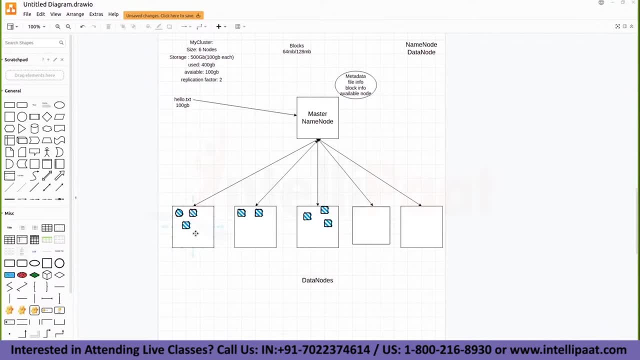 and it will not consider this data node for any further write or reader. so it's kind of a heartbeat signal which is being sent to the master at regular intervals. all the data nodes are supposed to be sending that signal. so if a data node has been failed, this data node 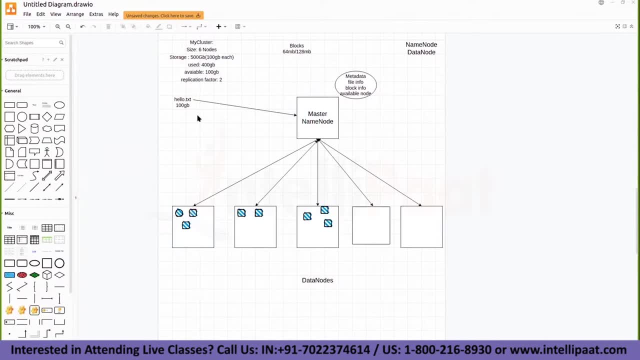 is notified that it it is not available. so now, when there is a hollowtxt read request coming in, it will look into the metadata. it will. it will read that. okay, this hollowtxt is written on one, two and three and the data node one has not sent any heartbeat signal. in that case, what happens? 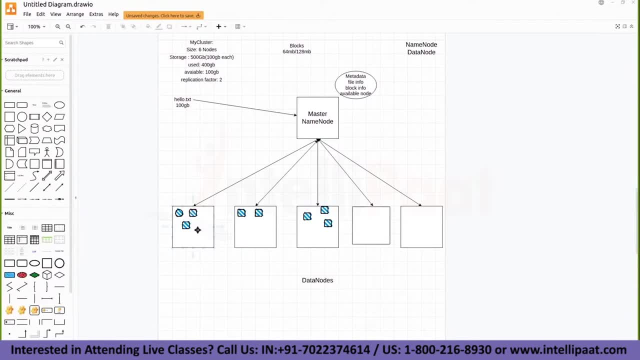 what are the blocks written on this data node and which blocks have been replicated on which data node. so when the primary block is not available, it's going to look into the replicated blocks and read those blocks. okay, so ultimately the first read operation has to be on the primary node if the data node which is holding the primary block 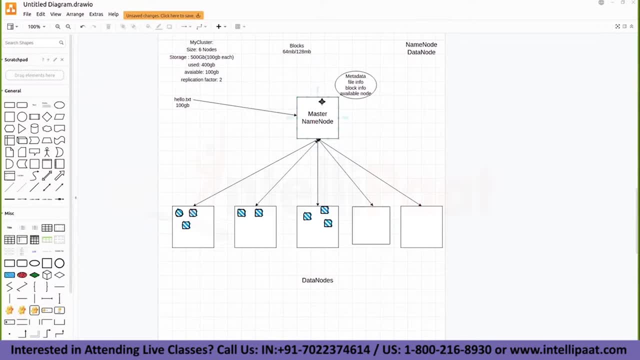 is not available, then it will look for the replicas. so where exactly it is being replicated, that also will be available in the metadata information. it's going to look for the replicas and it's going to read. it's going to process the read request from the replica. 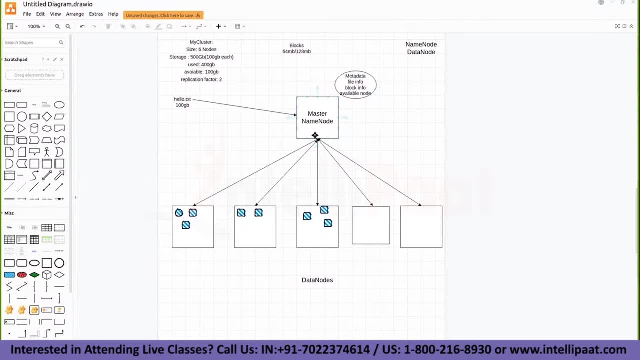 nodes right: primary block first. so replicas are always the secondary read operations. replica information will will not be the primary read operation. okay, so they. we cannot say that, okay, this block is available here and this block is our same block is available here. it can't be a. 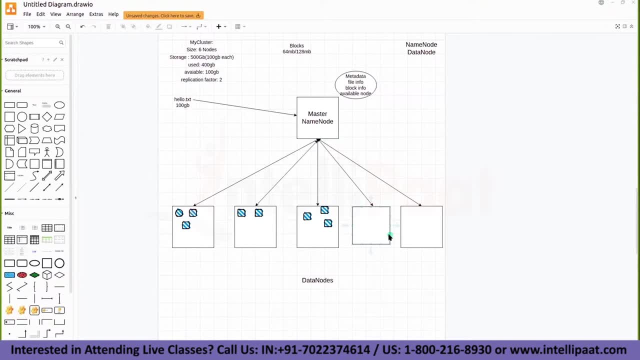 duplicated. all right, we are maintaining the duplicates intentionally. we wanted to make sure that the safety of the data is primary and we are maintaining two copies of it. first copy will be read first. if the first copy data node is not available, only the bulk data node is first copy is only available, so data node is not available properly. primary block again is available directly for read. you can go to the duplicated κα riplica ša. 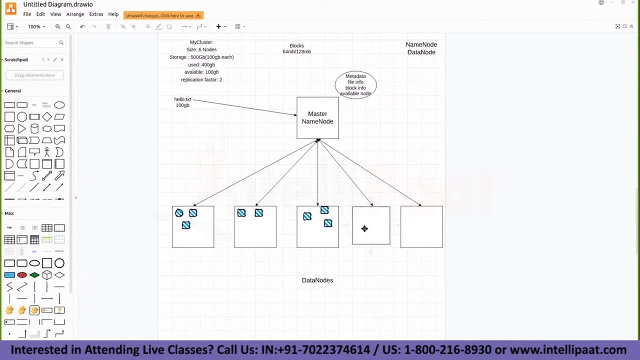 then the second copy will be ready, getting it now. so happens when you have to read the data. what happens when you have to write the data? everything is being controlled by your master node. if there is no master, you definitely don't know where to write the data, or you definitely don't know. 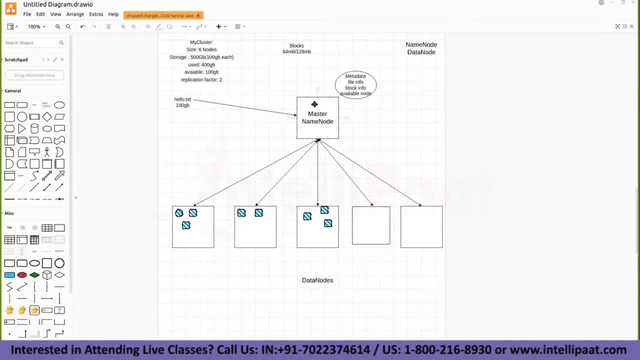 where to read the data from right. so it's basically the heart of your entire heartbeat. uh, help the hdfs cluster. okay, so now let's let's look at some of the failure mechanisms. so now that we know, uh, when a data node is lost, there is a duplicate copy available with the help. 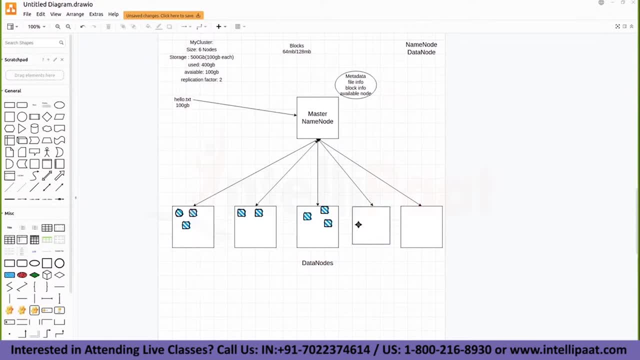 of replication factor. what we will do? we will maintain two copies, of a duplicate copy of it. so if this is not available, we will read it from the other duplicate copy. so how do you set this? replication factor is depending on the sensitivity of the data. so if the data is very sensitive, you're not supposed, you're not afforded to. 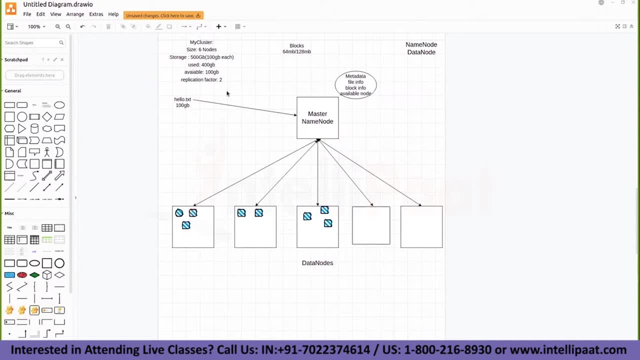 lose the data, if just this. if the case is like you have the production data, let's say, okay, the data is coming from some client, you're not supposed to lose the data at any cost. you maintain the replication factor to be three or two if it is a dev internal- uh, a dev environment. 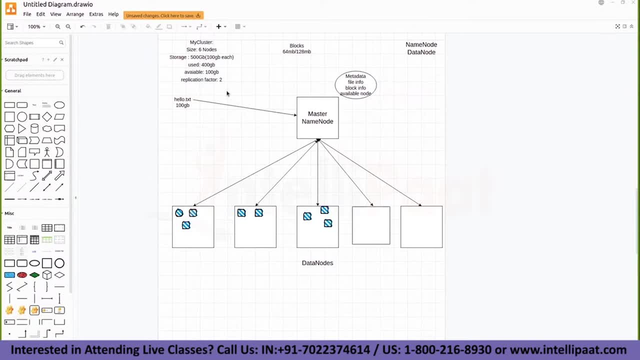 where the data is all duplicate, or i mean a dummy, or all the test data, for let's assume you don't have to maintain two copies of it. it's okay if we, even if you lose it right, so you don't have to maintain in such cases the replication. so only when. 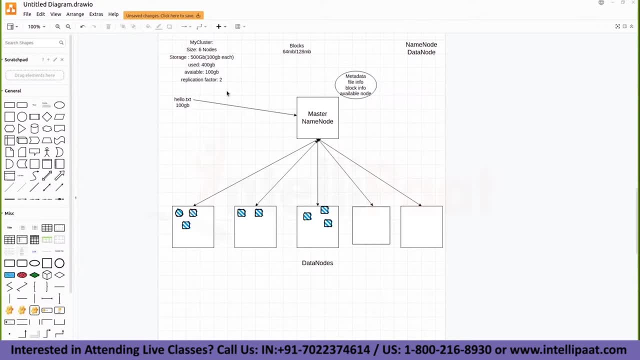 the data is sensitive and you are not afforded to lose it, then we will maintain the replication factor to two or three, okay. so in in unnecessary scenarios, we are not going to maintain duplicate copies of it. we will only maintain one copy of it as a replication factor. one, okay, so now. 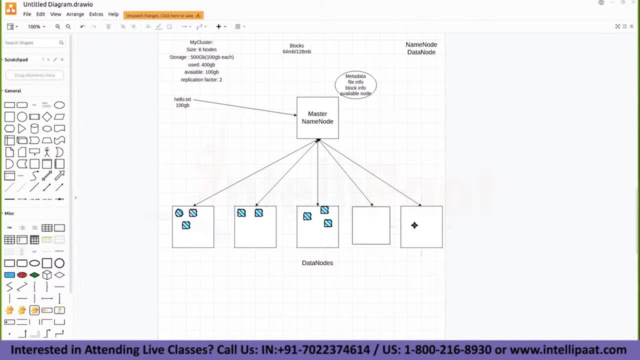 when we, when we lose a data node, there is, there is no harm, or there is no damage to the cluster. at least i can say the read and write operations can can go on, uh and the same pace. but what happens when the name node is down? see, data nodes are down, we are 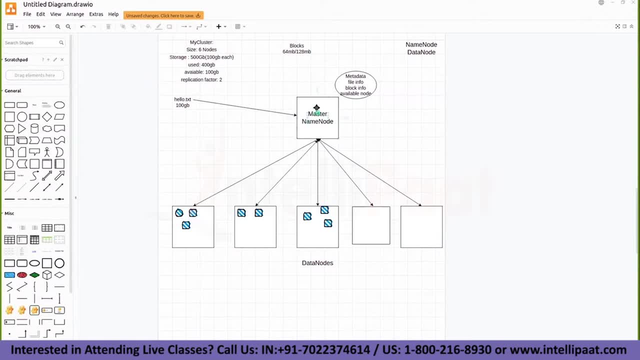 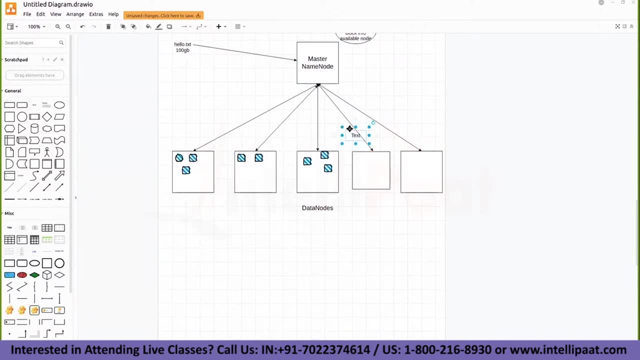 okay, we will, will continue with the operations. but what if the name node is down? so here we can consider, we can, we can um categorize this name node down into multiple scenarios. let's say: name node down. see, your name node can go down in two different scenarios. one is the scheduled or restart. okay, there is some restarts going to. 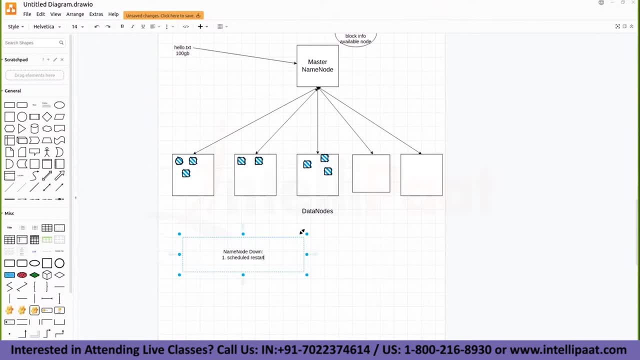 happen at regular intervals, right on weekdays or weekends. there is some scheduled activity you restart on so and so after 10 days or after 15 days you restart this machine. so there is one scenario and uh, unplanned outage or downtime, these are the two scenarios. so what happens at the scheduled uh? 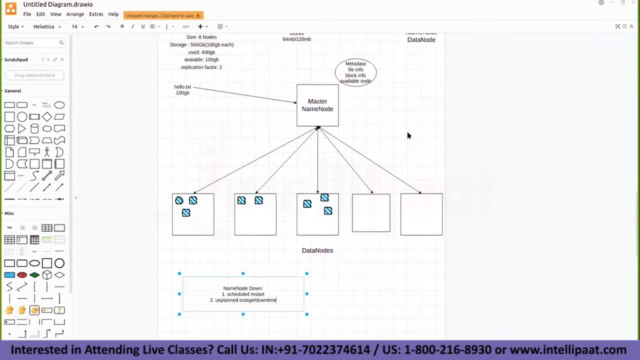 restarts. this is this is a known activity, right, so we all know that there is a restart happening on the name node and your hdfs will not be available from so and so time. there is a schedule email sent. there is a notification sent to all the users who are accessing it. 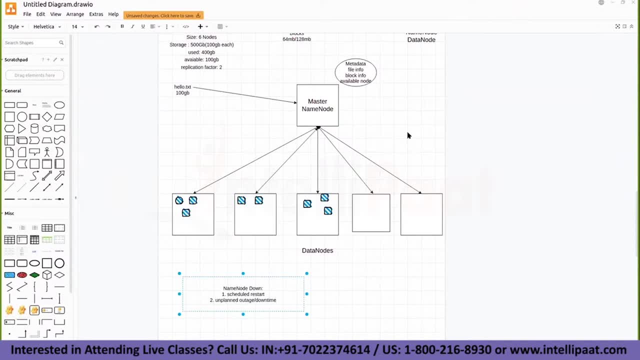 and it is properly planned. okay, when the systems are down and when there is not much traffic- on weekends or on late sundays- you do this scheduled activity. there is no harm or there is no problem with this kind of an activity. but what happens with an unplanned outage? what happens if? 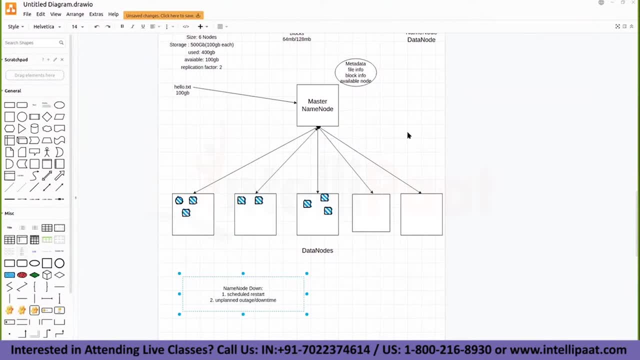 there is some issue with the master node hardware and some issue, some problem, and it has gone down. what happens in that case? the entire hdfs cluster will not be accessible, right, because this itself is going to be the point of contact for all the read and write operations of your hdfs cluster. 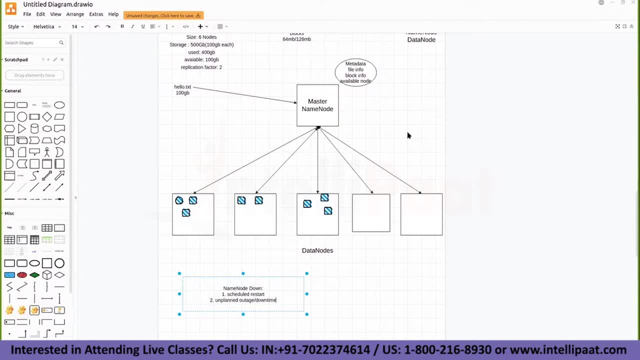 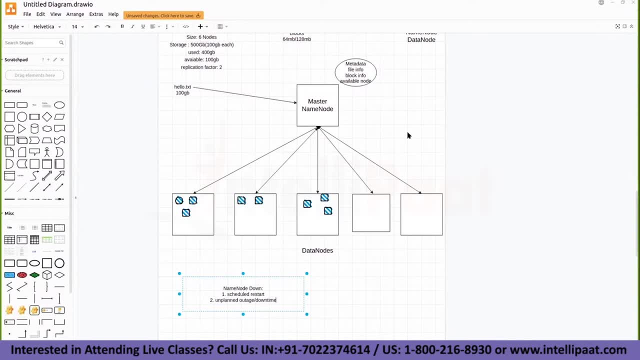 have to. i mean we. we don't matter if the hdfs is active or not, right, so master itself is going to be the single point of contact for all your read and write operations. if the master is down, then the hdfs, entire hdfs, is going to be down regardless of all. okay now. okay, you have done some. 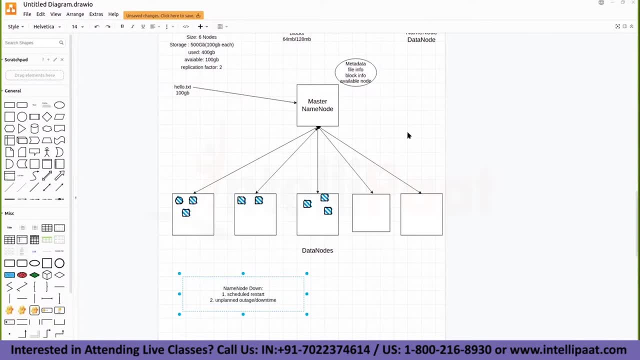 maintenance. you have resolved the issue of the master and you have somehow brought it back up again. okay, so after one hour you brought the name node back back into action. so you done the maintenance. what if the data which is available inside the master node- i'm talking about this metadata- okay, the metadata inside the master node, while you are doing the? 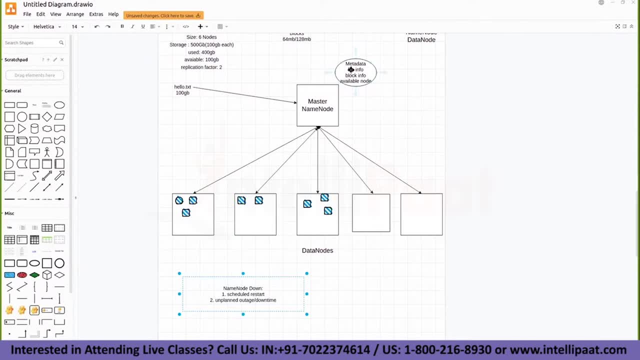 maintenance or, depending on the impact of the issue, your metadata can also be lost. some cases, right. if there is a hardware corruption, the entire data that is available inside the metadata, inside the master node hard disk will be corrupted, right? so in your unplanned down times, there are two scenarios. 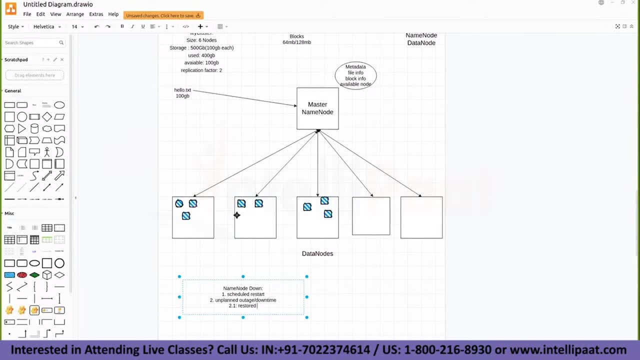 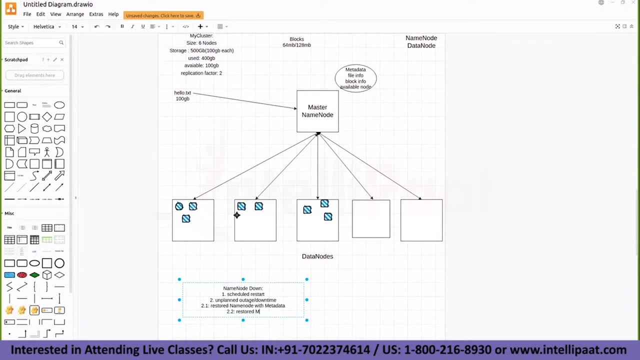 restored master, let's say name node with metadata- then 2.2 will be restored name node without metadata. now so first scenario is restoring the name node after one hour. whatever the time you have taken, after one hour you have restored the metadata name node with the metadata. so there, 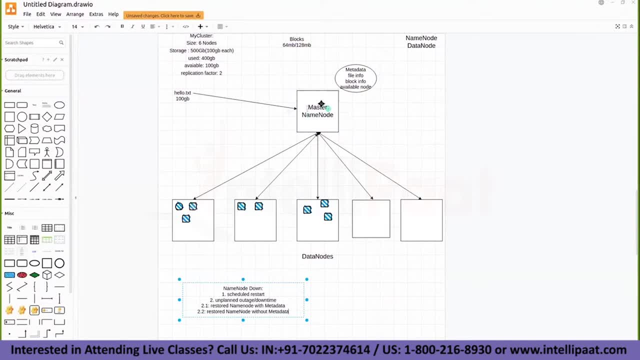 is no loss in the metadata also. so after one hour you brought the system back up again and your metadata is also active. so now what happens after this is brought back up again? you continue with the operations. there is, there is no problem with it, right? so the only downtime will be the one hour. 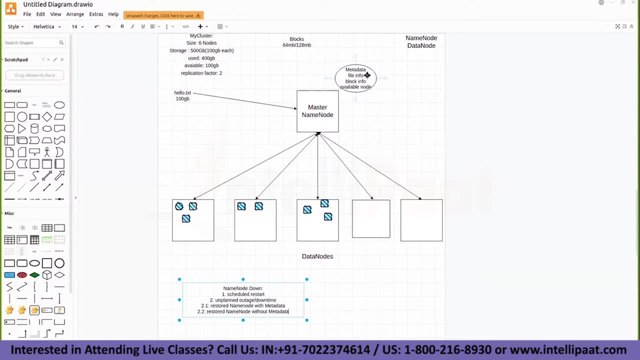 which you have lost in in doing the maintenance activity. so this is not having any problem. but what happens if the restoration of name node is down is done without actually restoring the name metadata? what happens? you have the name node available but there is no metadata. how do you? 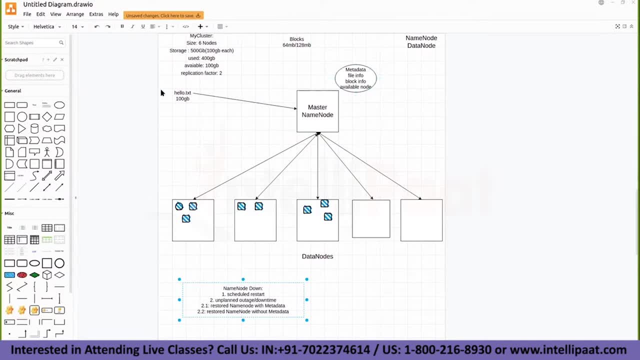 interact with the data nodes. no, for example, there is a write request. how do you actually write the data without the information of your metadata? yes, so in this cases also, your name node is considered to be inactive. there is no recovery for this kind of a scenario. that means your entire htfs cluster. 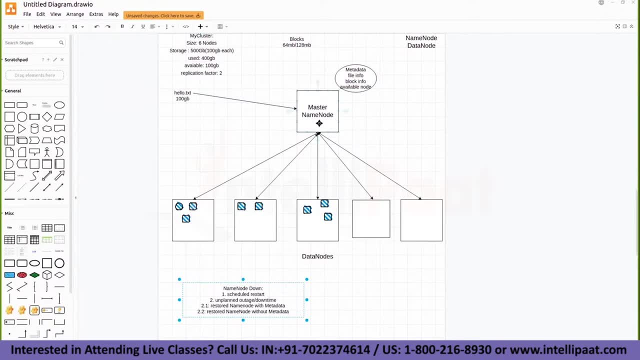 is supposed to be crashed. okay, so there is no backup. i can say your name node is is is not gonna restore to the existing functionality. your entire htfs cluster is considered to be down, crashed, okay. so to avoid these kind of scenarios they have, they have done some changes. so before, before. 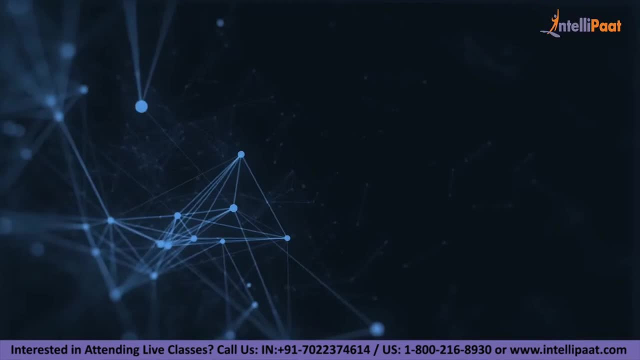 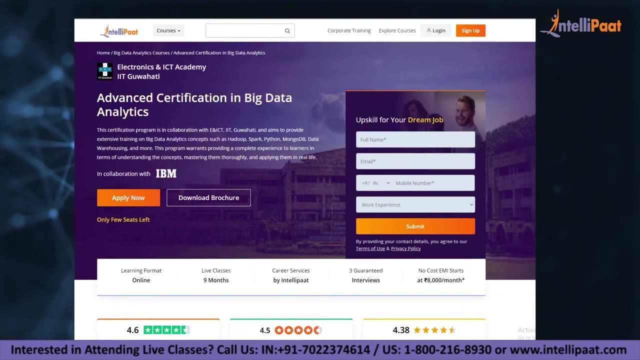 we get into it. i think i missed out on some points here. just a quick info, guys: if you want to make a career in big data, then intellipaat provides an advanced certification in big data analytics by enict council, iit, guwahati. it is taught by iit professors and industry experts. 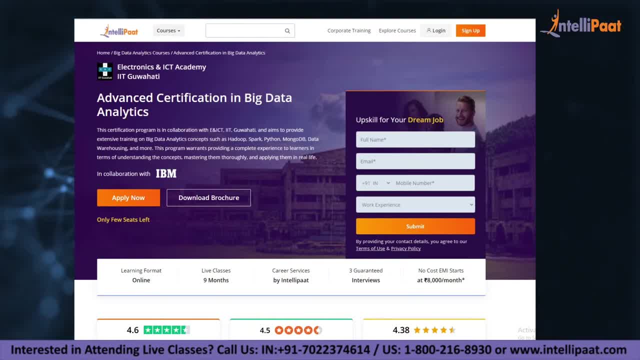 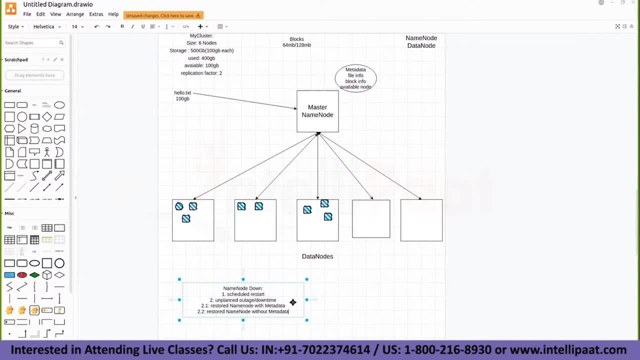 with more than 10 years of experience. this course is designed to upskill and land your dream job. now let's continue with the session. are we clear guys with the failures? i missed out on the metadata information. there is some data that has to be updated, so inside the metadata guys, uh, sorry, i. 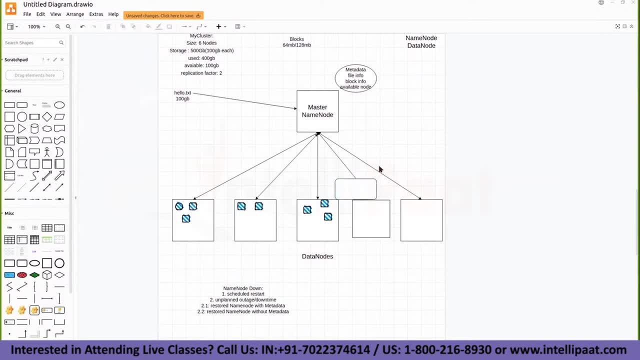 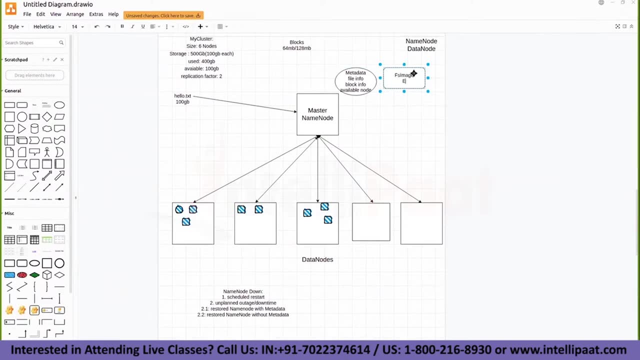 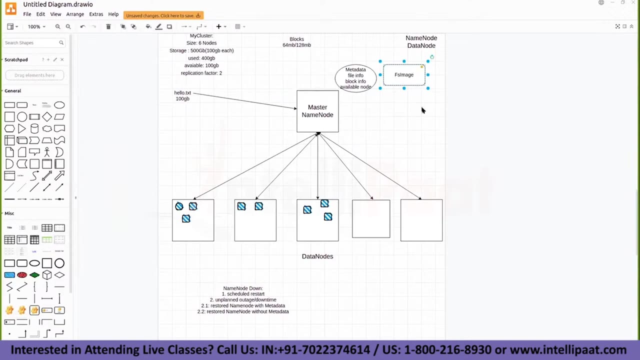 forgot to include one point. there is inside the metadata. there is something called as fs image and edit logs, but there is something called the read logs, let's say not fs image. so what does this fs image mean? so this is all inside the metadata, only inside this. 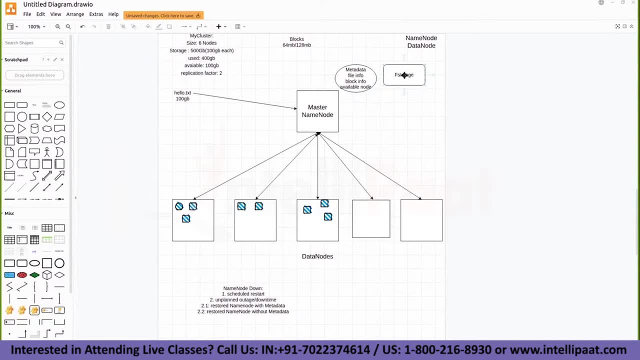 metadata information. so what does this fs image mean? so fs image is something which is going to have the image of the entire file systems. that itself is the term right file system image. that means it's having the information of all the data that you have inside the right. you have the data. 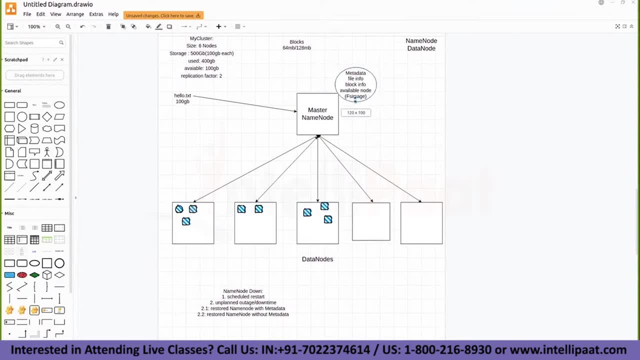 of all the. you have the information of all the data that you have included in the hdfs cluster. that is what we call it as an fs image. okay, and for every right operation in the previous scenario we have done some 100 gb, right, right, so you have updated something on data node. 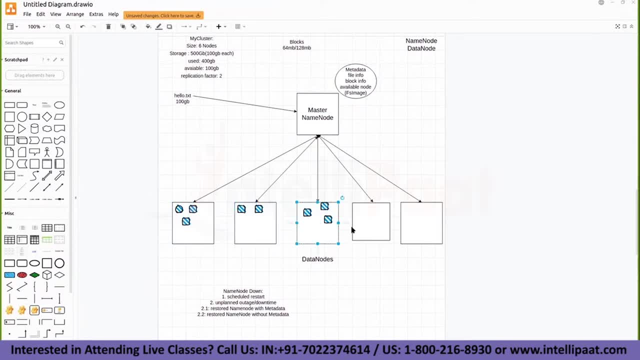 one updated something on data node two, you have updated something on data node three and there is no update happening on data node four and five. so for every right operation or for every change in hdfs data node operations, for every write or a read operation, there is something called as. 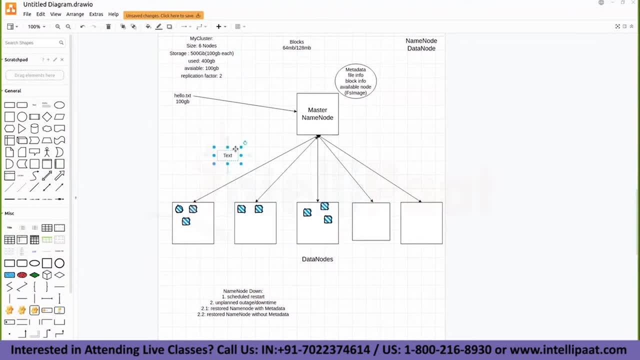 edit logs that is getting generated. we call it as edit logs. that means for every edit happening, for every write operation, there is an edit log that is generated which reads the changes happened across all the data nodes and it will append this edit log to the actual fs image. 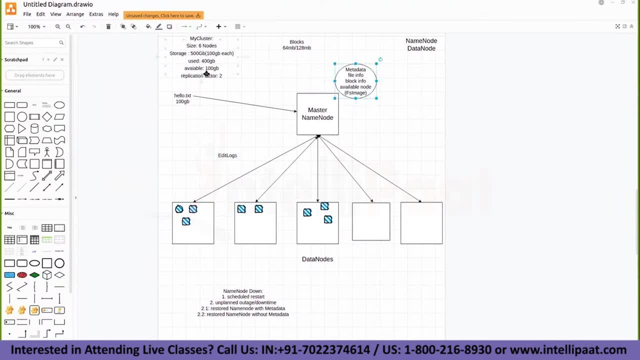 that means in the previous fs image my cluster capacity was around 300 gb used and to 200 gb used and 300 gb available. but now, with the edit log information that i have updated, i updated it to 400 gb used and had to be available. that means whatever the changes that have happened in this particular 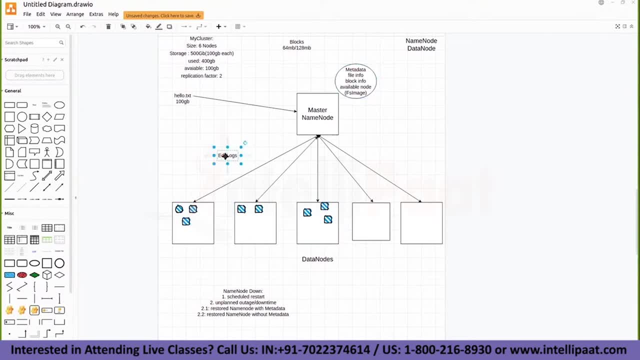 right operation have been captured in the form of an edit log and they are going to get appended to the core fs image. whatever the entire information that you have, you just keep appending this edit logs to the existing fs image so that your fs image is latest. every time now when you get a read operation, your 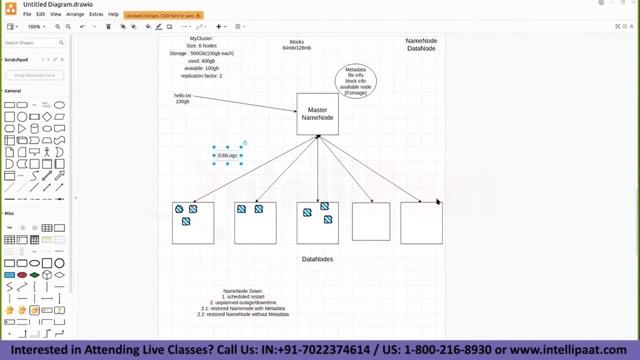 fs image will be latest and it will be able to process the actual information, getting it, getting this understood, this concept of edit log and fs image: yes guys. so edit log is for every right operation. you generate some metadata and append it with the existing metadata of your master. 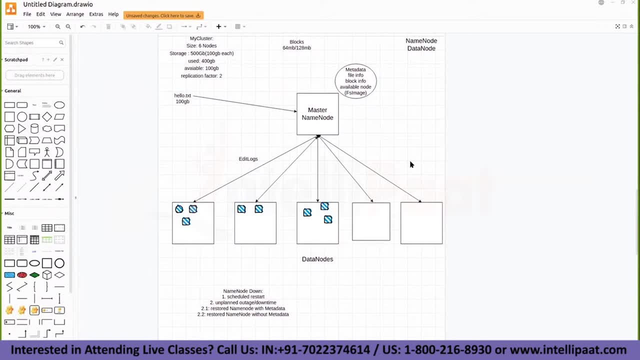 your master name node. so the, the core, the entire metadata, is called as fs image and for every edit, whatever you capture, is called as an edit log, the log for each and every edit. that is what the edit log fs image is: the file system image, the entire image of the file system. okay, you take the edit. 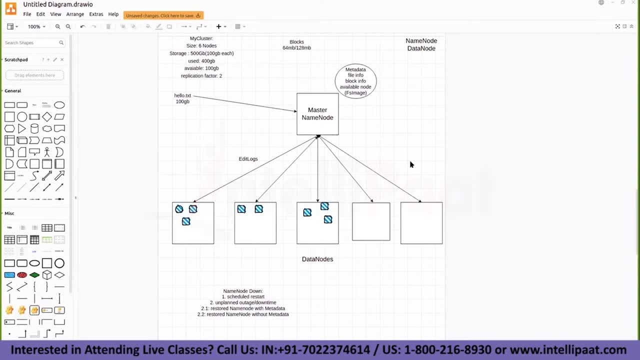 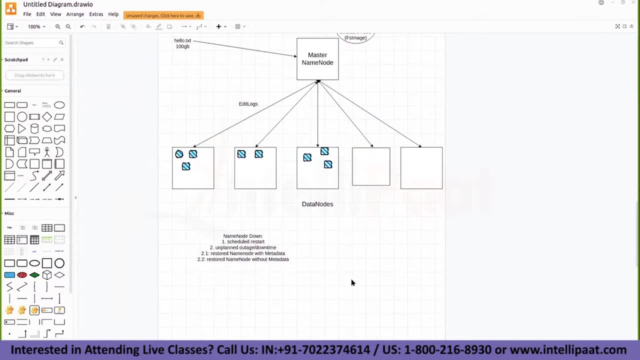 log and you go and update in the fs image. this is one thing that i missed in the previous discussion. okay, all right. so now going back to the downtime scenario. so now you understood, guys, how many ways the downtime will be. one is the scheduled downtime: on some weekdays, weekends, you will be scheduling. 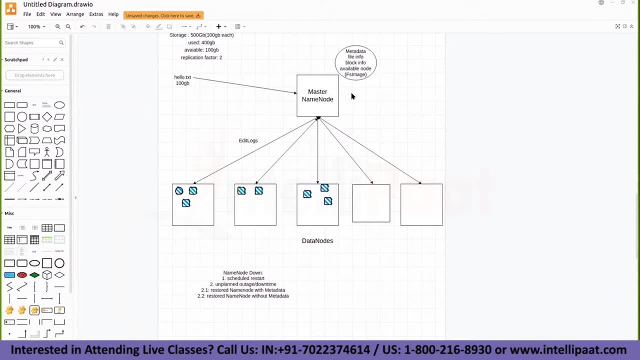 uh, your name, now to restart and whatever the time it is taking to restart, your name node will be down and after the proper activity your name node will be brought back up again and your entire processor will continue as planned. this is a planned downtime, i can say. but whereas for 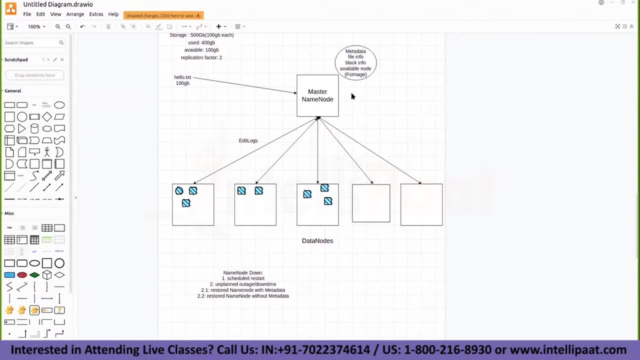 unplanned downtime. there is some issue with the uh name node and it has crashed. now you take some time to repair it. you brought back again and when you do that you will be able to go back to the. when you have brought it back again. there is there are chances that your name node can. metadata can. 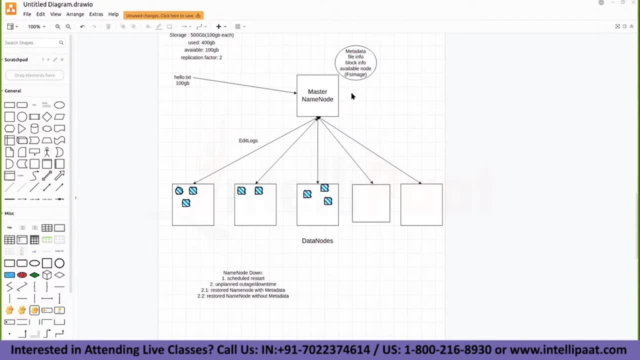 can be restored completely or your metadata can also be crashed in some scenarios. if your metadata is restored, there is no downtime. i mean, whatever the time it has taken for you to repair the system, is is actually the downtime. after that, you can continue with the rest of. 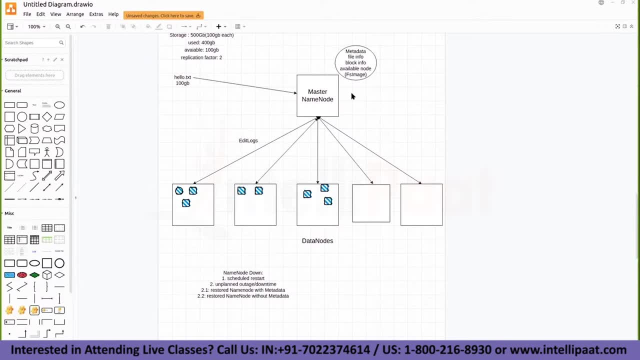 the activities. but when there is no metadata, when the metadata restore is not done, this is the entire system failure. we consider it as okay. there is no restoration, there is no uh resolution for this kind of a issue, right? so this is considered to be the entire cluster failure. okay, if your name node is down along with the metadata, then your cluster entire. 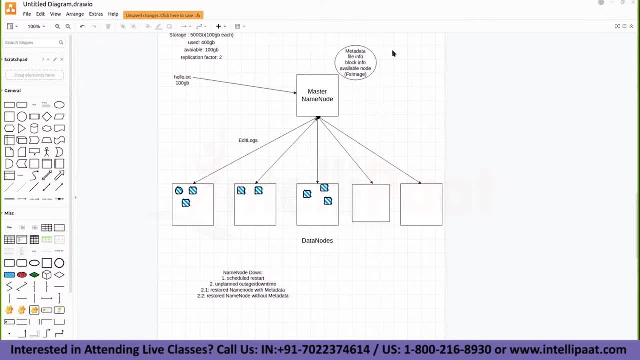 cluster will be down. so to avoid this scenario, this is the earlier versions of adobe in the. in the earlier days, this is the scenario. we had only one name node and we don't have a backup. so to avoid this scenario, what they have done is they have included something called as a secondary name. 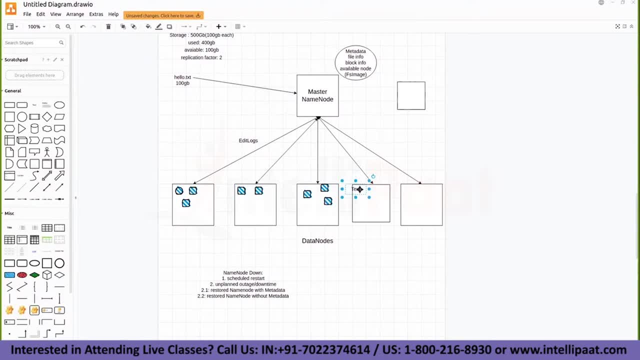 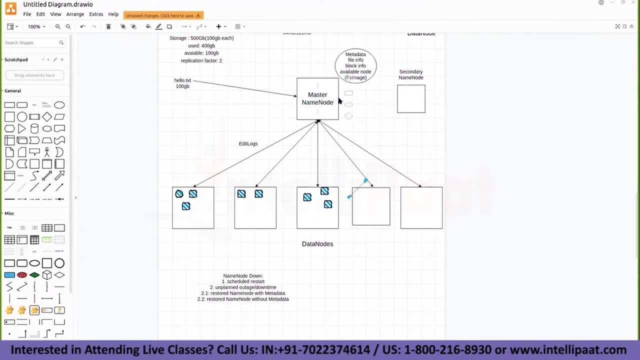 node. i call this as a secondary name node. what does the secondary name node do? it is a backup of name. yes, it's a backup of your name node. uh, it's, it does not. let me tell you that this is here. this is here, so what it only holds is right. so this secondary name node is considered to be the. 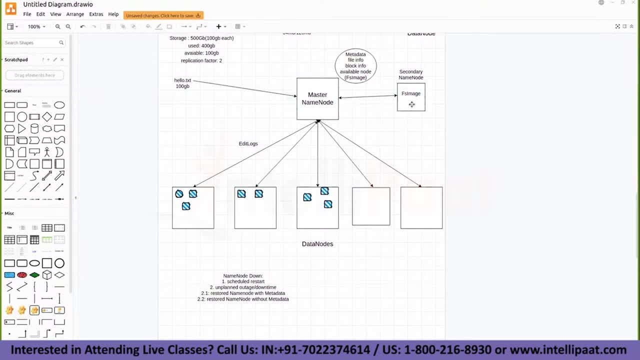 name node metadata only. okay, so it's not a backup of your name node. that means see when your name node is down. your secondary name node cannot take up the process and it cannot run, uh, the htfs cluster in the absence of your name node. okay, what it will only do is at regular intervals it will. 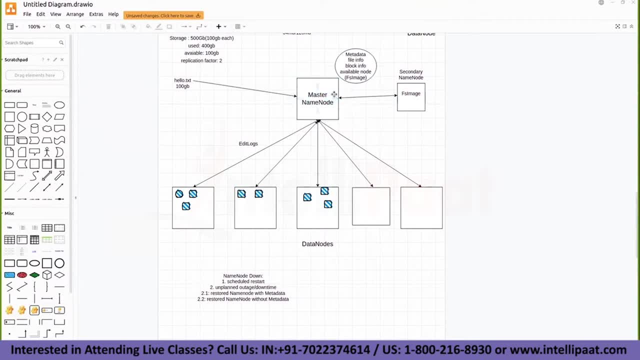 just take the fs image which is available on the master name node. it will take a copy of it, store it inside the secondary name node and then send it back to the master name node. that's the only activity it's going to do. that means we are only maintaining a backup for your metadata. fs image. 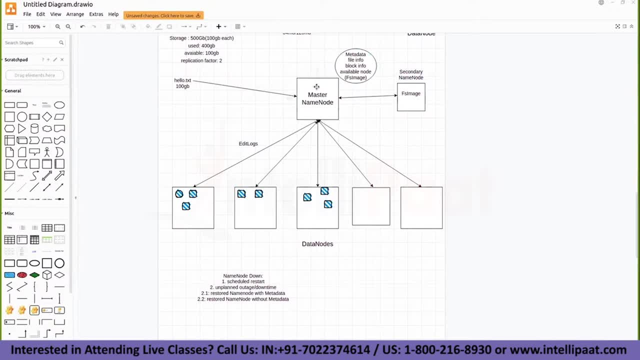 apart from that, we are not doing any other activity which your master name node does. secondary name node does not- does not take care of any other activities which your master name node is going to do. it is only meant to maintain a backup copy of your fs image. 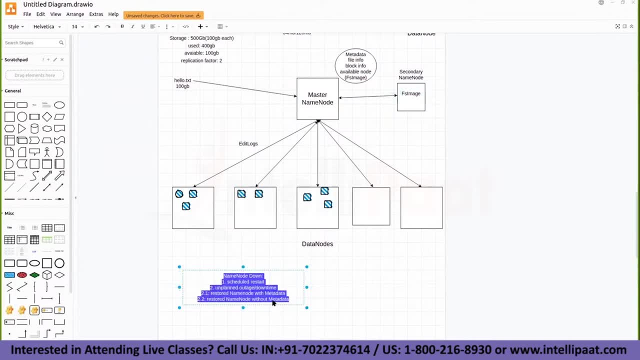 just to avoid this last scenario. what is that last scenario? when your name node is crashed along with your metadata, you restore your name node and you take the latest fs image copy from the secondary name node and you continue the process. in the last scenario there is, there is: 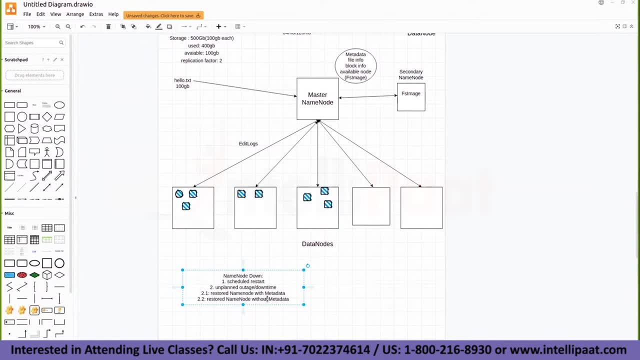 an irreplaceable issue, right it. it cannot be restored again. that is what we discussed. so to avoid that entire crash zone of the system, we included something called as the secondary name node. okay, just to maintain a backup for your fs image. so this is a very important question, guys. you, you might get even in. even now you are getting. 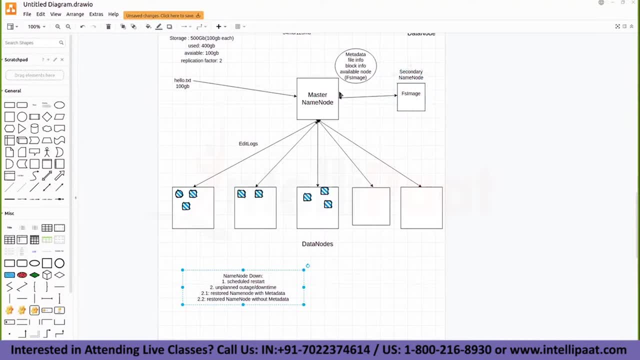 these questions in the interviews. so your secondary name node can not cannot take up your activities of your master name node. it is only meant to maintain a backup of your fs image clear at regular intervals. it just takes out a copy of fs image, stores it within itself and it's 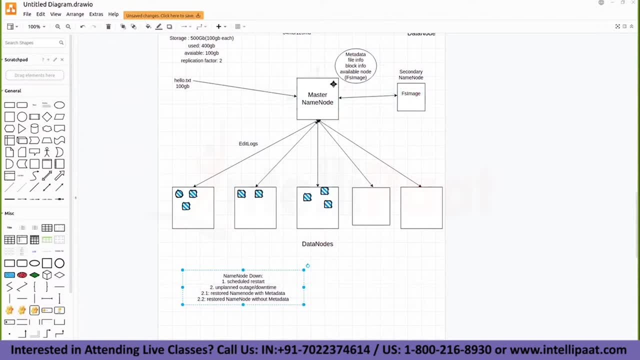 going to be soon realized. ok, so well, guys, I hope you have used enough data. hundred percent. we can conclude this part right before we start uh youtube today with you guys, and you are Estáo Byur. Thank you, sorry. We understand the technical operation. we intentionally discussed this first part and 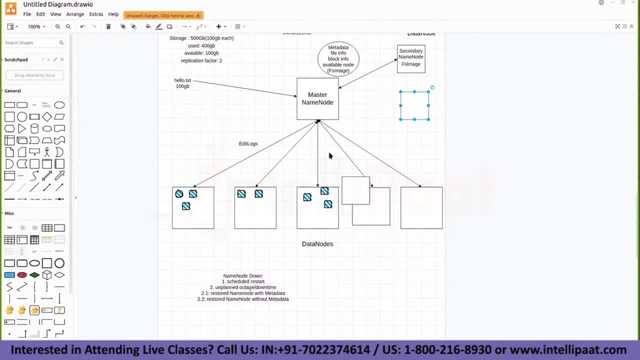 But the result of our metadata is positive, according to the user, to this node network lead into a all isolate version, doesn't work itself and sends it back to the master. name node okay, heart okay of hadoop, first generation of hadoop okay, which still has a problem of name node failure, right. 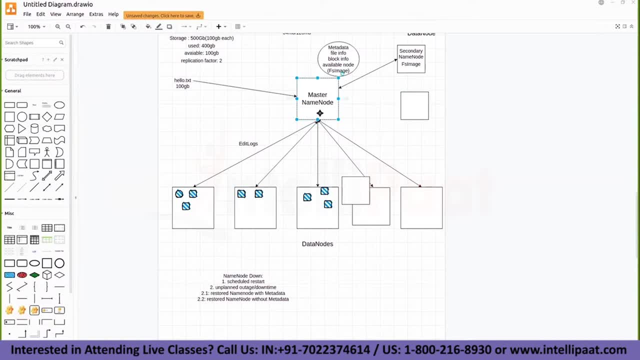 so when the name node is down, the entire cluster is down. there is no recovery for it, right? only when the name node is brought back up again you can continue with the rest of the process. so, whatever the time the name node is down, that time you, in that particular time, you cannot access any. 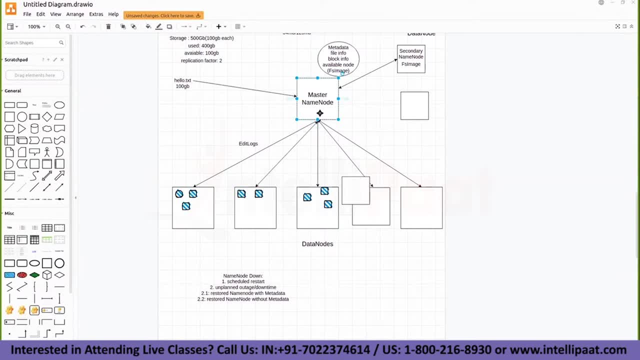 read or write request. okay, that downtime is always there. but in the second generation of hadoop what they have done is they have included some concept called as active and passive name node. so in second generation of hadoop, or else shall i write it in a different diagram? shall i put it in a 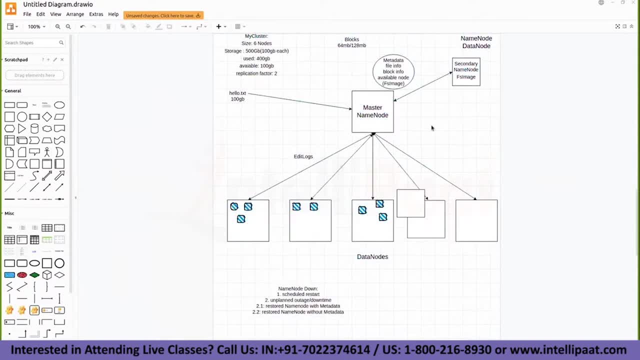 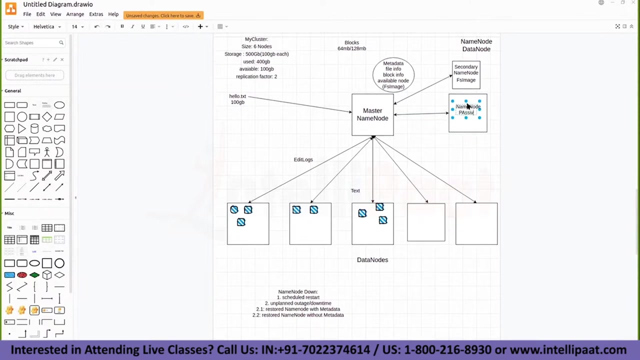 different file altogether. right, so in second generation of hadoop, the only change is gonna be here. everything else will remain the same, but i call this. oh, there is also an option to draw like this, is it okay? super, how do i make it bi-directional? right, so this is your what name? node, i can call it passive and this is: 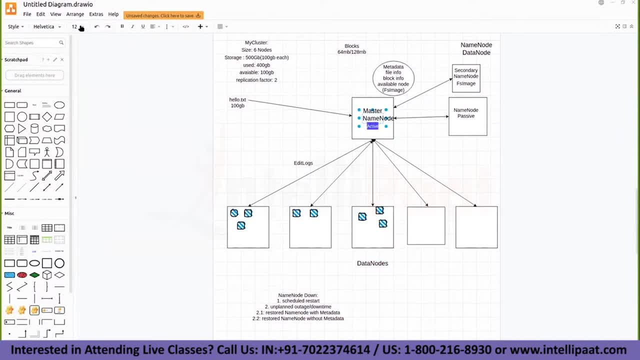 active. so there's a concept of active name node and a passive name node here. okay, that means rest, all concepts will remain the same. okay, that means there are two name nodes. one is going to be active, whichever is running, the other one is going to be passive, so the same connectivities will be connect, will be having a similar. 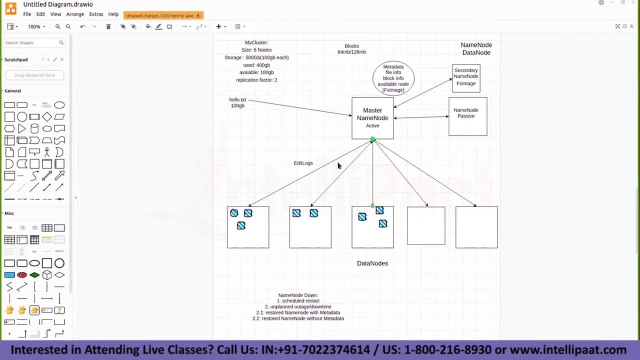 connection with passive name nodes also, um, how do i make this? i think i'm gonna become expert in draw. if my manager knows this, then he's gonna make me draw all of these nodes and then i will just call all these diagrams, all the architecture related diagrams. is gonna make me do okay, super. 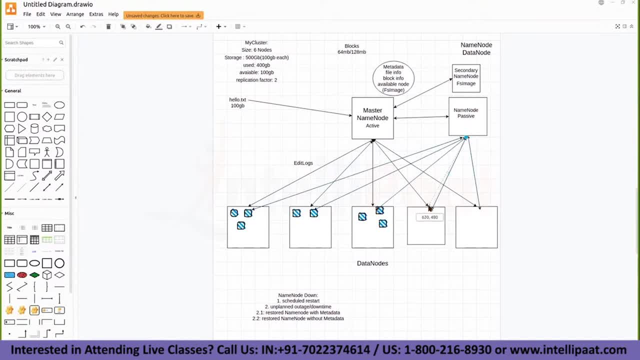 this is how it's going to be understood. so that means there is a backup. there is a backup for your name node actually here. okay, so even when the uh name node is is gonna go down, you still can uh continue the operations using the passive name node. so whenever your active name node is. 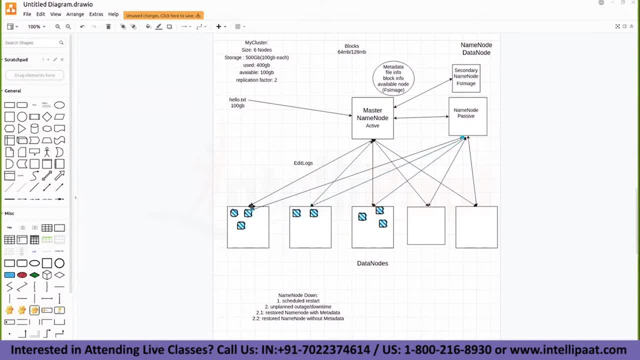 down, your passive name node will take care of it right. so this is how it's going to be, so that you are maintaining 24 by 7 availability of your name node. the only reason why we get this is you maintain 24 by 7 availability of your name node, so we are just trying to make sure. 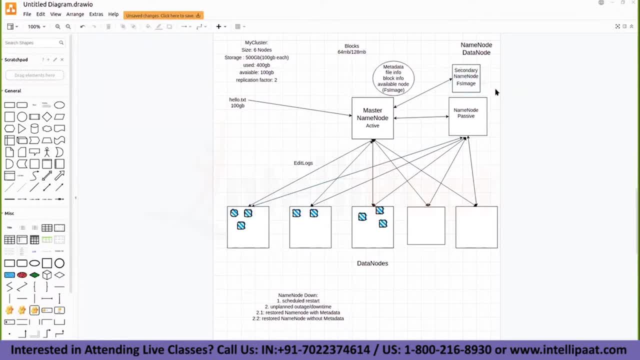 your name node is available all the time, so let me just take this out for some other place. so i'll move this here. and there has to be a connection between these two as well, because the fs image can come from any place. right, it can come from. 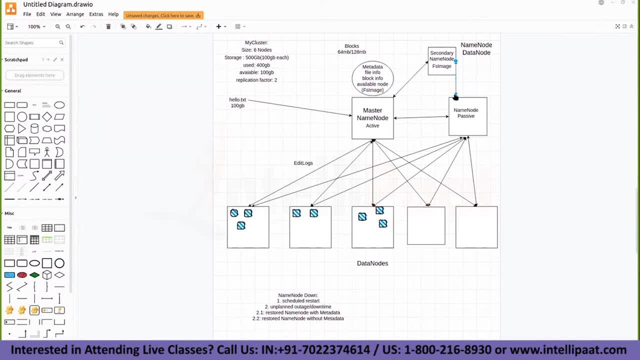 name node, active name node, or it can also come from passive name node. this is how it's going to be. so your secondary name node is going to be in the middle and your fs image can come from any place. understood so many arrows. so your secondary name node is again only maintaining the fs image. 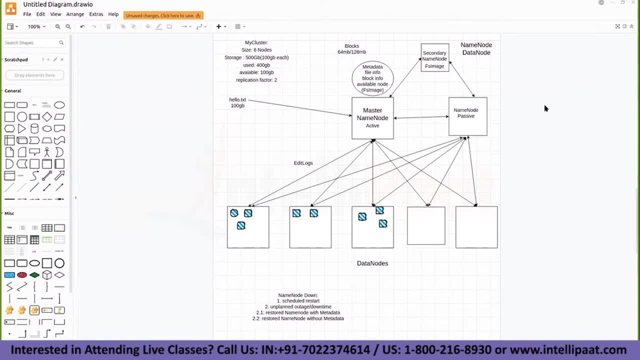 but your master name node active and the master name node passive, is something which is going to act as a duplicate, a backup, actual backup of your name. so when your master name node is down, all the controls will go to your passive name node. right, so it will. continue with the read and write operation. so when this is brought back up again, it will come. it will come back to the controls of your active name, right? so every time you make sure any one of the name nodes is running again, don't ask me if both the name nodes are down. that depends on your. 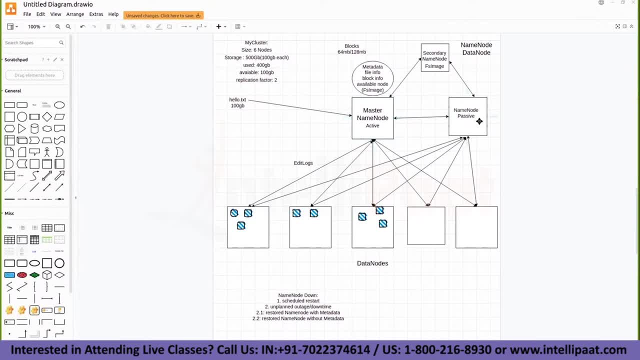 luck entirely. i'm calling this active and calling this passive because this is running currently. this is going to be active. if this is running, this is going to be active and this is going to be passive. that's it, okay. so don't, don't get, uh, misdirected about this, misdirected about this. 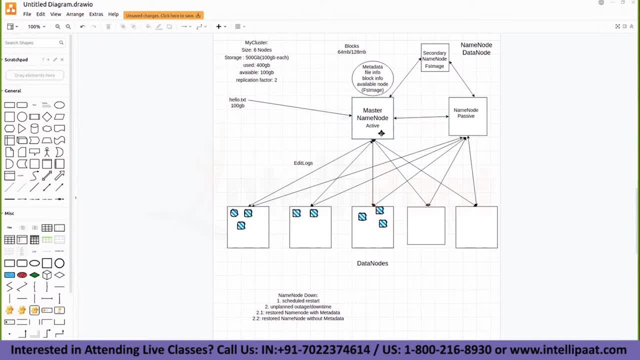 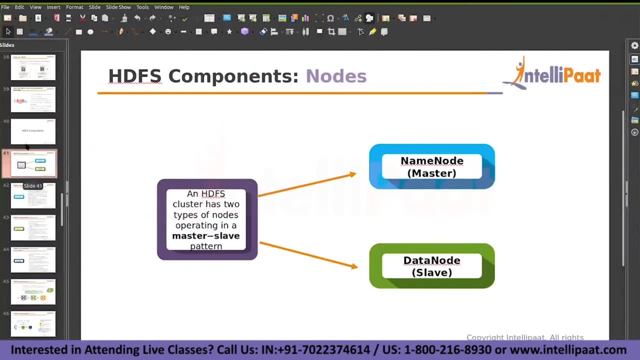 active and passive terminology. whichever is running will be active and the other one will be passive. okay, simple. so any questions on this? yeah so, uh, we know that hdfs has two components. hdfs cluster, uh. one is a master and one is a slave. master is a name node and slaves are all the data nodes. so whatever the number of uh nodes you have inside, 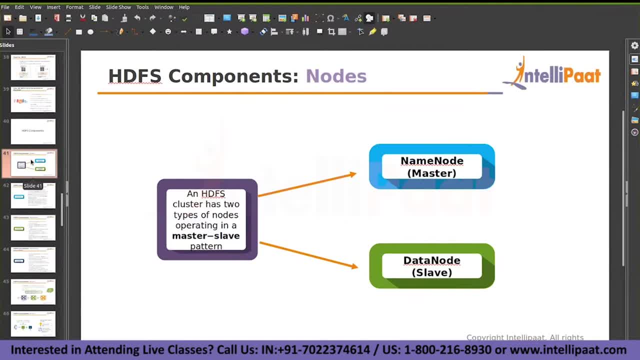 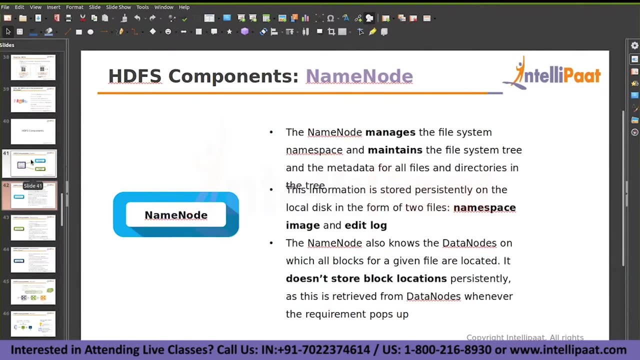 the cluster. so one will be allocated as a, one will be considered as a dedicated master, and the other rest of the nodes will be the slave nodes, right? so we know what's the functionality of a master and a slave. so let's, let's, let's just read through some of the operations. 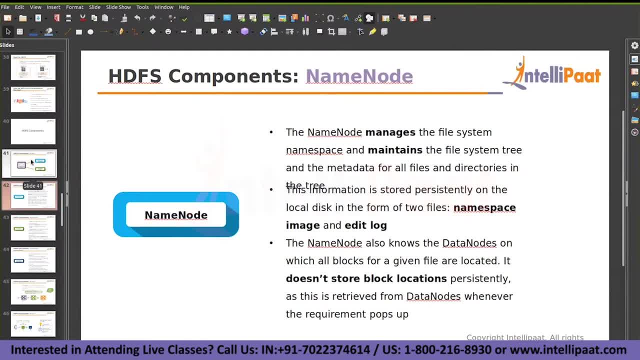 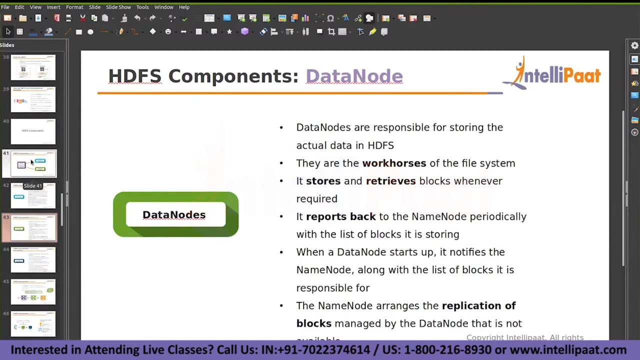 uh, the name node manages the file system namespace and maintains the file system tree and metadata of all the files, and it also maintains the namespace and edit logs- and we've seen what this namespace is all about, okay. and the data nodes? these are actually the workhorses. it stores and retrieves the data. so, whatever the activity which is related to the 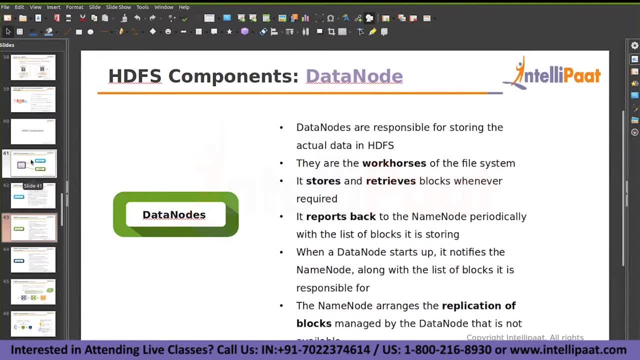 read and write operations. is is going to happen on top of the data nodes, so name node is only just managing the resources or the the flow of the data. name data node, uh, is is something which stores the data and you've also seen the replication, how the data node replication is done. 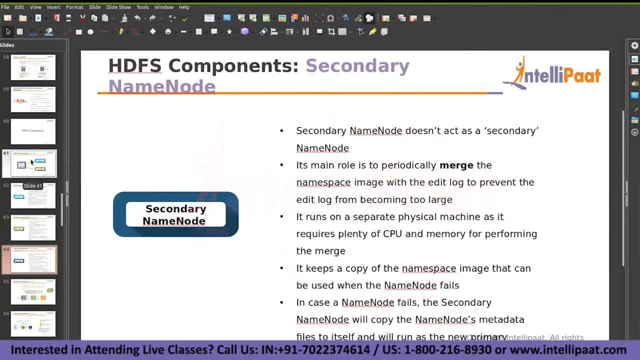 and the secondary name node doesn't act as a secondary name node, so it's not a secondary, it's not a backup to the name node. that's what it means. its main role is to periodically merge the namespace image with the edit log to to prevent the edit log from becoming too large, right? so it just. 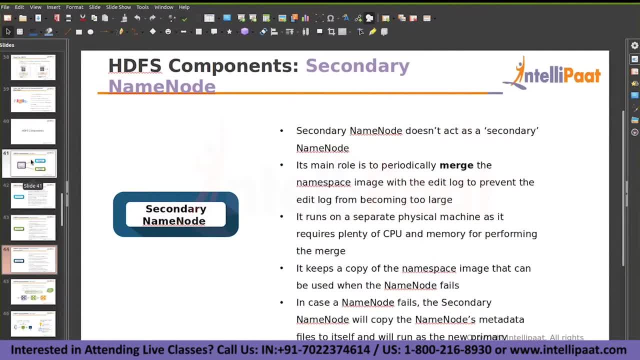 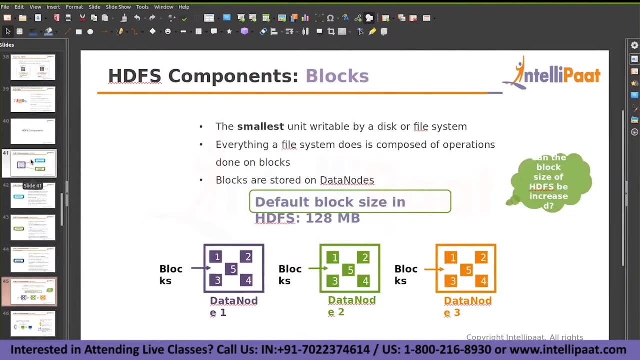 runs on a separate physical machine as it is requiring plenty of cpu and will perform in this much right and only just in case if the name node fails, the secondary name node will copy the existing existing metadata to the primary name and we have also seen the blocks how the data node 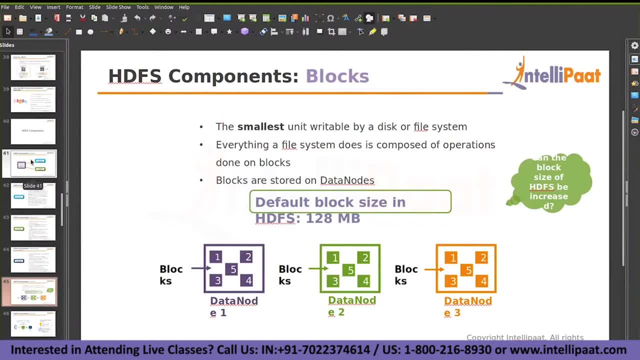 blocks are divided. whatever the data size can be, your data is always going to be stored in the form of individual 128 mb blocks. okay, so each block is uh around 128 mb. this is configurable. earlier it was it was allowed. the maximum was allowed: uh only 64 mb of block size. now, in the latest versions of hadoop, it is now. 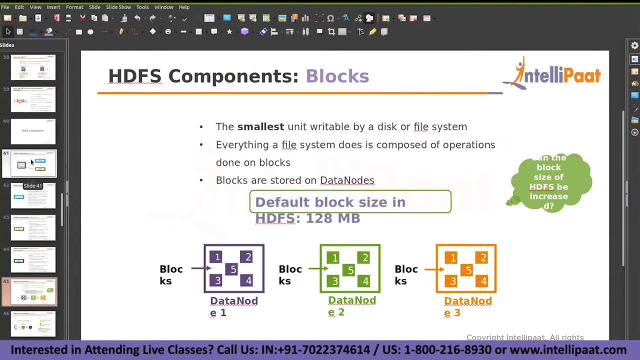 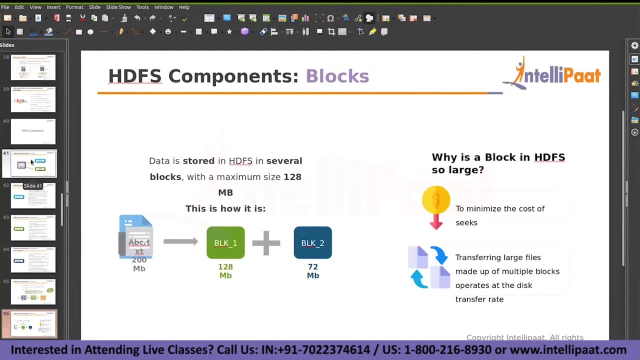 moved to 128 mb. so any data, any data, any data file has to be split into multiple blocks of 128 mb each, and these blocks will be stored on the uh hdfs data nodes, right? so this is some uh representation of how the data can be divided. so there is a data file of abctxt. 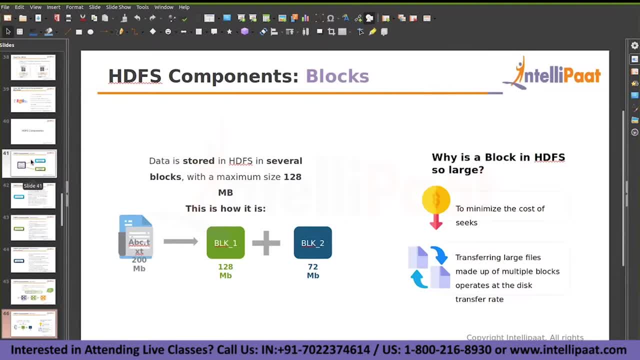 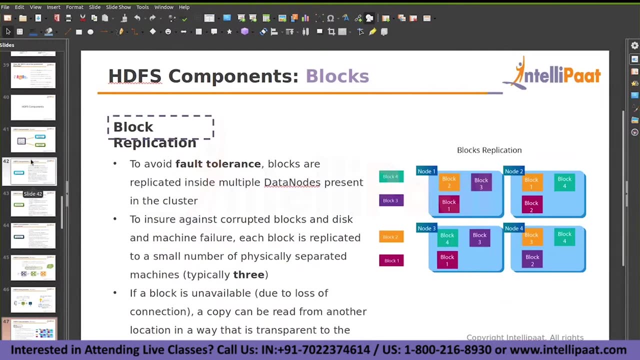 it's. it's supposed to be divided into two blocks, considering one block sizes of 128 mb. so 128 mb is block one and the rest 72 mb will be block two. right and the block: replication. we know what's the replication, the maximum, the default replication factor. 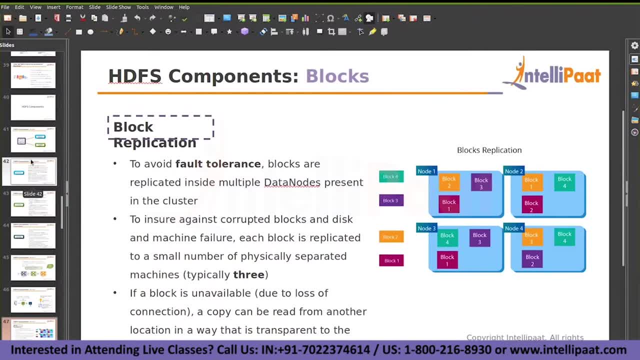 when you configure the system would be one, but you can. you can take it up to uh three. you can have three copies of the same data maintained so that you don't lose the data even when the data node fails, right? so there's also something related to the 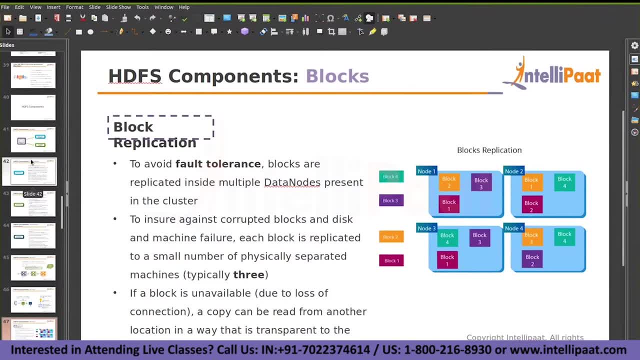 um, off these replicated blocks, see for example. if you see, so this is just a theoretical saying. I mean, I don't know how do we can, how we can prove this practically. but in general, i've gone through some documentation where it says, for example, we have three replication factor, right, so that means three. 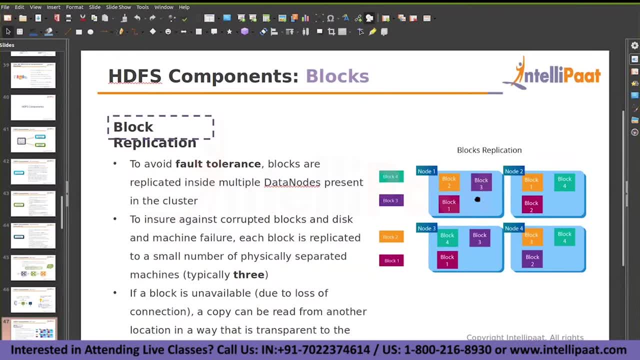 copies of my data has to be maintained. so the primary data block, you store it in this data node. okay, in whatever the data node you are supposed to write the data, you will be storing it in that particular data node. so that's the first block, that's a primary block. 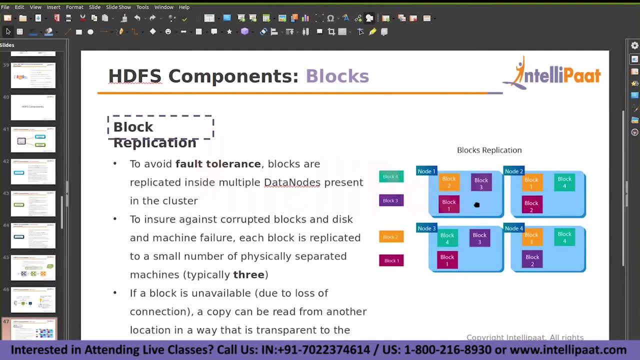 and the next block of data will be stored in the closest possible data node, right? so, for example, i have some 10 data nodes. so whichever is near to the data node one, the first primary block, i have written on the data node one. okay, so whichever is nearer, nearer to the data node one, we will. 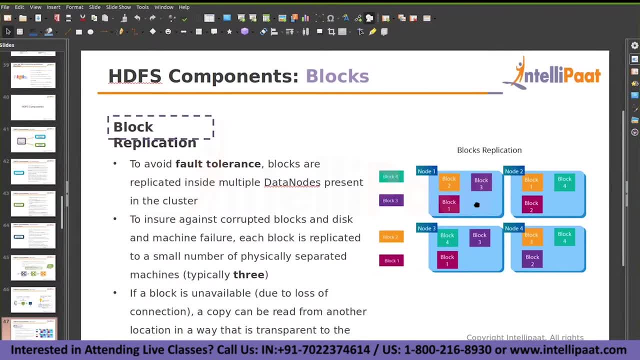 consider that data node two or three, whichever has got the availability of storage. so we will consider that as the slide second copy. okay, so you'll store the second copy of it on the nearest data node possible and the third copy of it is is being stored on a different rack altogether. 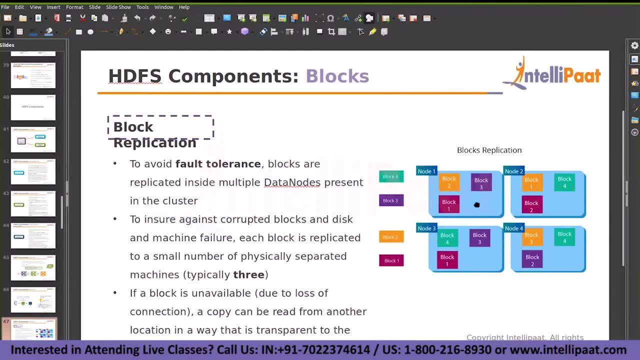 so what does this rack mean? so, has anyone, have you, have you heard about this concept? rack, so some group of data nodes, you you consider them in the form of a rack. so let's say i have 100 data nodes. so 10 data nodes, i'll place it in some location. 10 data nodes, i'll. 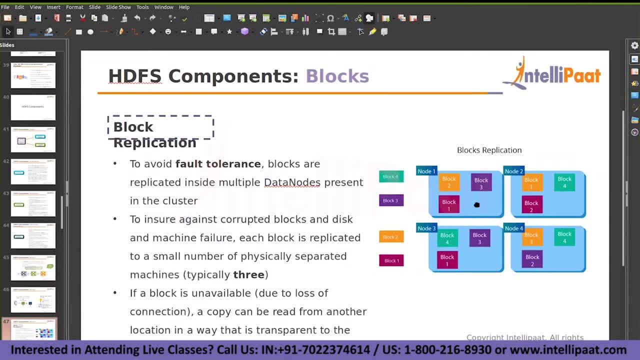 place it in some other location. 10 data nodes: i'll place it in some other location. so virtually when, when the physical location of the data nodes is in different regions, so one is in us, one is in some india, one is in some canada, so different locations. so we call them as a data. 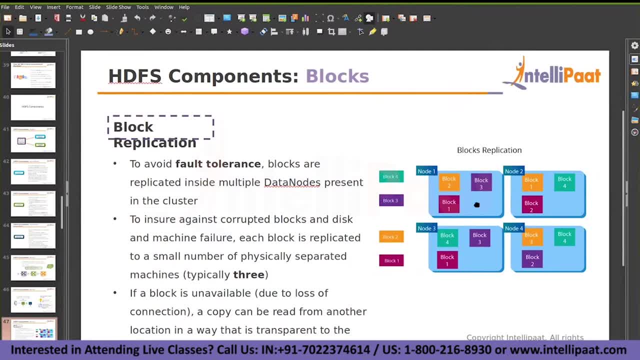 centers. right, you must have heard about this term. data centers can be at different locations, but but when, when you log into the masternode, or when, when you are looking at a particular htfs cluster, you you take to see them on the same, i mean on the same network. i mean, that's what we are trying to do, right, so it? 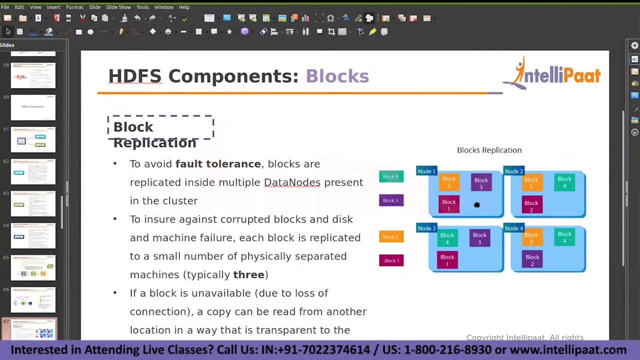 doesn't make any difference whether they are available on different regions also. so you you tend to see them available on on the same network, which which can be accessible easily. so the third block is is said to be located on a different region or a different track altogether. so that's. the reason being: when the first copy of the data is lost, the first first copy of the block is lost- the master node- it has to look out for the next copy of it right. so when it is looking for a next copy of it it does not have to traverse through multiple data nodes. it has to be available in. 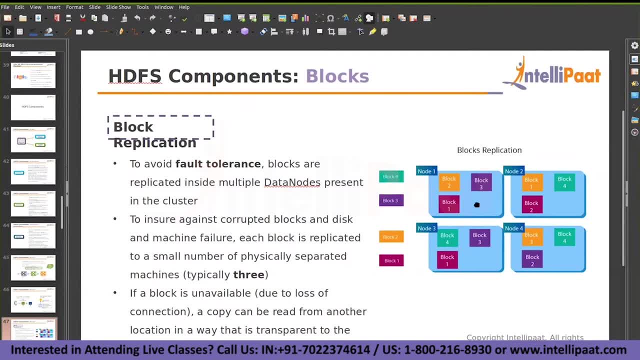 the next data node in the closest possible premises of the primary data node. right, so that is one. and when the entire region is also lost. i mean where, for some reason, when the data nodes available in so and so region or in so and so rack have all been uh, uh down, let's say for. 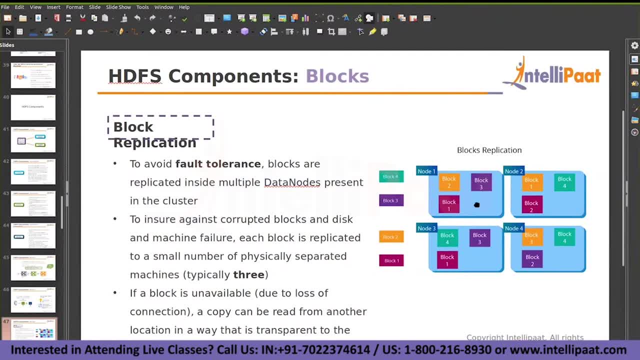 some reason, okay, some, some, some natural reasons. so in that case you still have a backup in a different region. okay, so that's what is. is is being done. i mean in, in general, in real time scenarios you will definitely are. in most of the scenarios you will not have data node blocks from different regions. 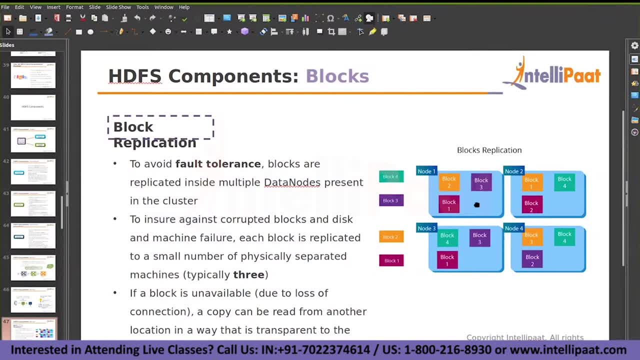 everything will be in single region. but when there is a feasibility of your data node- i'm talking in terms of a high level, high scale architecture- so when there are, the data nodes are being spread across multiple regions, and so on and so forth. so that's what is being done. okay, so that's what is. 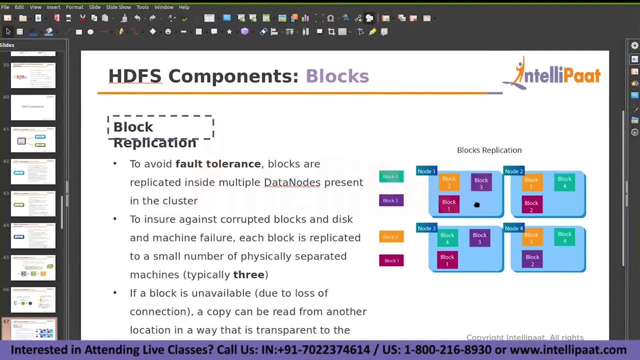 being understood. right, and yes, so use with blank space. so it happens. okay, there is one way to particularize this script: ahora sim indulge efforts in reality. okay, this is how the replication is going to happen. just just keep in mind, that's it. you don't have to explain it to anyone else. okay, right, so block replication. that is how it's it's going to. 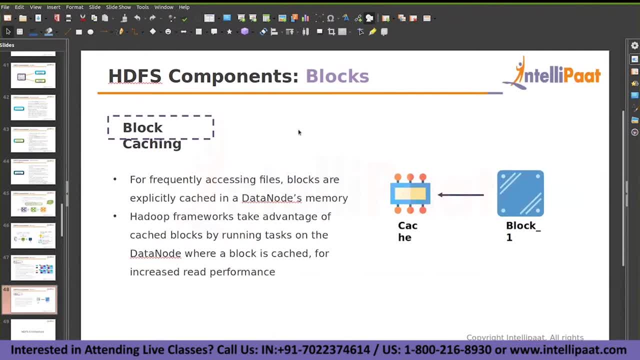 take care of. and then we have this block caching. so we know what's the caching mechanism, right? so for frequently used information, you, you keep it in in a specific location. so for the same reason when, when the specific block is being accessed multiple times, when it is being accessed, 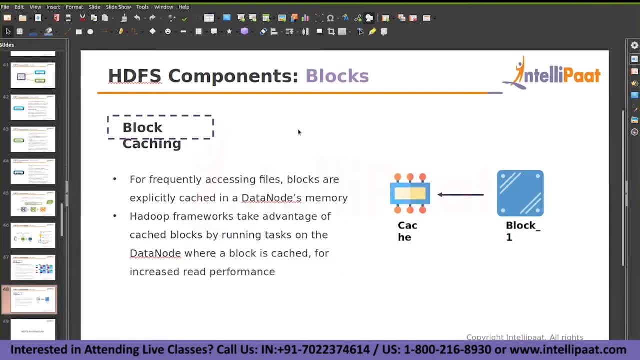 frequently you, you store this particular block of data in the data node memory. okay, so that's that's what we call it- as a caching, so that it's going to be easily retrievable. so definitely, if you, if you compare the differences, the data available within the memory is easily accessible. 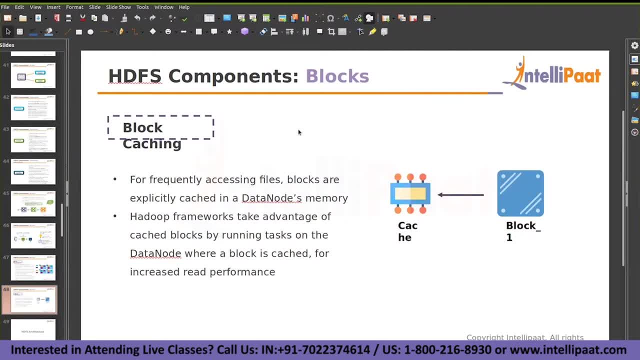 or quickly accessible than the data available in the hard disk of the same machine. right? so that is why we we store within the memory, and even even with spark, that's the advantage we get, right? so when, when the data is uh, when the data node block is frequently accessed, then you, you kind of uh. 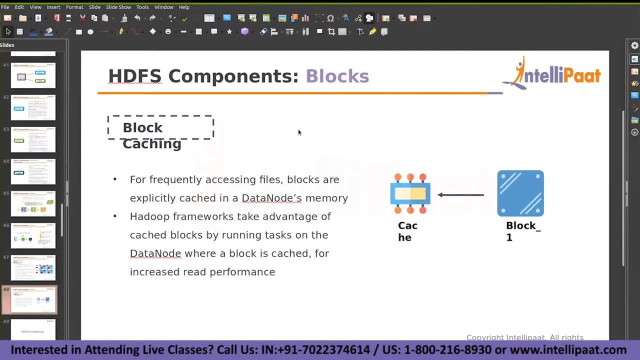 put, put them, put that particular particular block in the uh data node memory and you kind of access them easily. i mean it's going to be faster compared to the hard disk read and write, okay. and there is again some parameters how long it has to be in the memory. if that is not, 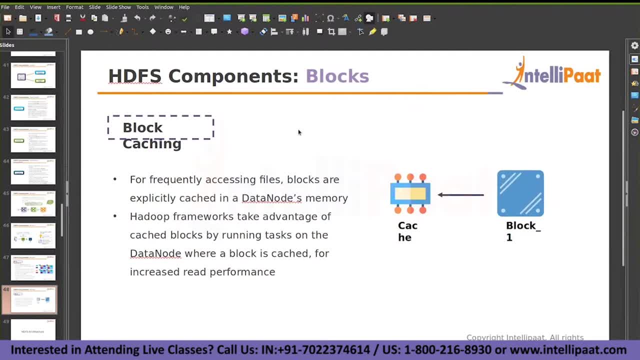 accessible per se, for for 10 minutes or for five minutes. it has to go back to the, it has to go back to the memory and it has to be removed from the memory, right? so we call it as persisting, persisting in the memory, and then you, you, you kind of remove it from the memory and it has to be in. 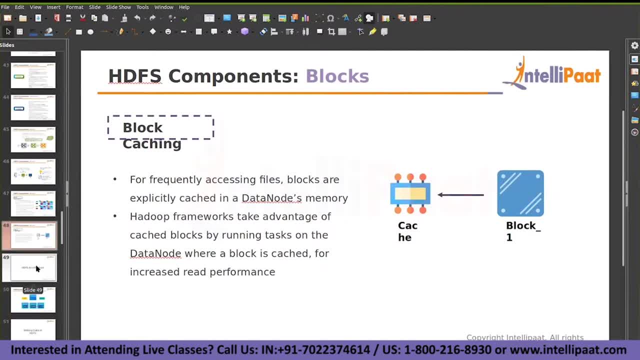 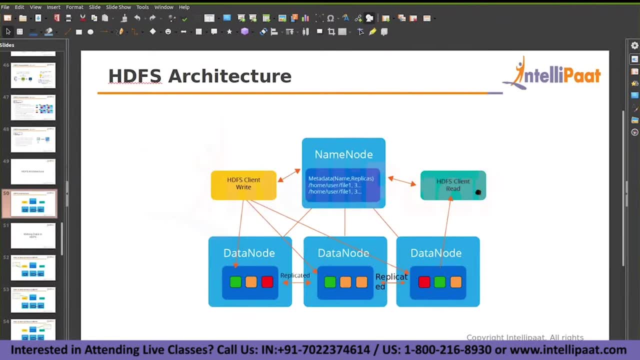 the hard disk of it. understood, yes, see hdfs. uh, client, right, and client read is something. uh, who? who is sending the request? okay, so whoever is sending the request to the hdfs cluster, it can be you as well, right? so you log into a specific machine which has access to the hdfs cluster. 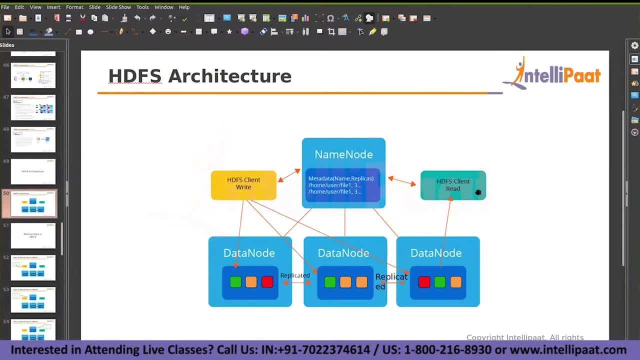 you submit a request or cps from so and so location, so and so file. i'm trying, i'm trying to write it to your hdfs after you into the hard disk hdfs. so whoever submits the request, we consider them as a client. okay, so hdfs client- right, and hdfs client read. so it's a write client. 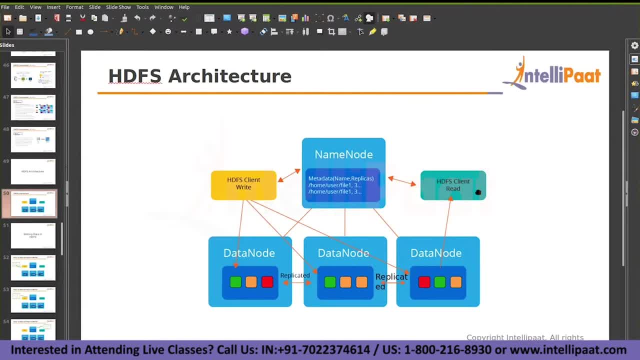 and a read client. that's, that's the only difference. apart from that, do you? do you find anything new or anything that we need to discuss? then we have the procedure for writing to the hdfs. there's a step-by-step procedure. okay, so client requests to create a file. 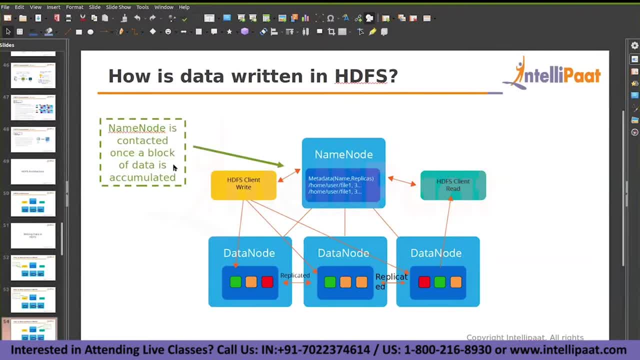 and name node is contacted once a block of data is accumulated and name node responds with the list of data nodes. so, list of data nodes as in whatever the available data nodes it has got with with so and so amount of space, with available space you will. you'll let the client know that these are. 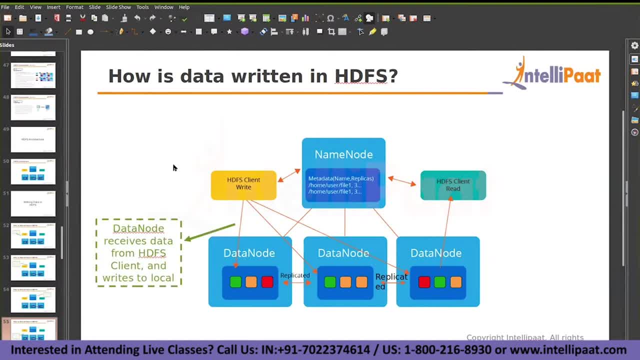 the data nodes that are available to be written. and data node receives data from hdfs client. and after you receive the data node uh list from the name node, the client will go to the data nodes and it will start writing it. and data nodes forwards a file to a second data node for replication. and 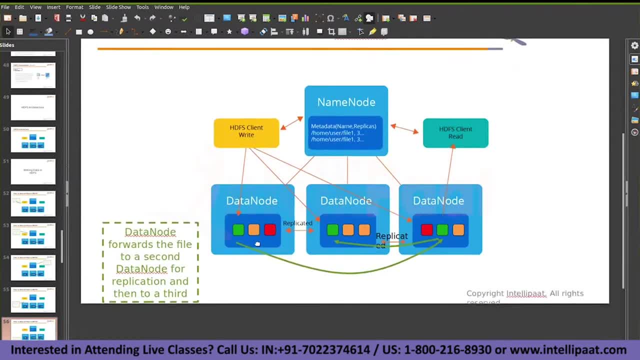 then to the third data node. so as and when a particular block of data is written, so as and when a block is written, that has to be replicated. okay, so it's not that the entire data will be written and then, uh, replicated on the block. this too, we discussed about it. so yeah, as. 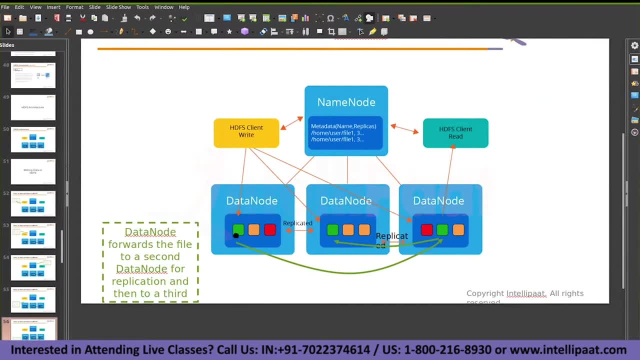 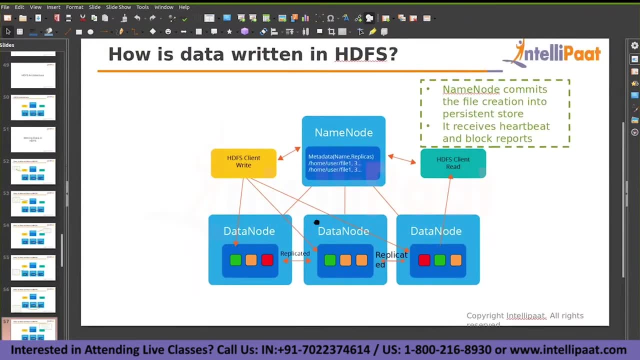 in when you you write a single block, this step- it has to be forwarded to the uh other data nodes where it has to be replicated then and name node commits the file creation and into persistent store. it receives heartbeat and block reports. so heartbeat signal. we have seen what is a heartbeat. 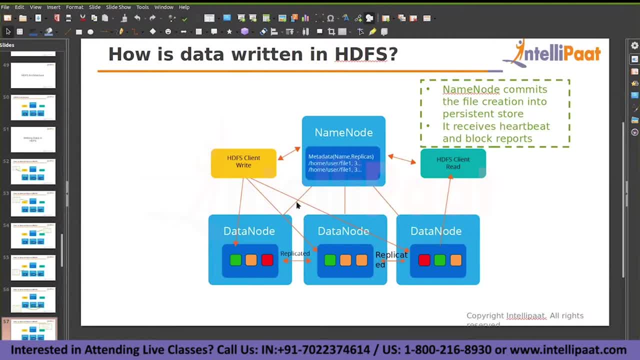 signal just to make sure that the data node is active or data node is alive, so it keeps data node. every data node keeps sending this heartbeat signal to the name node just to make sure the data node is available. similarly, there is also another signal that keeps on sending is the block report. 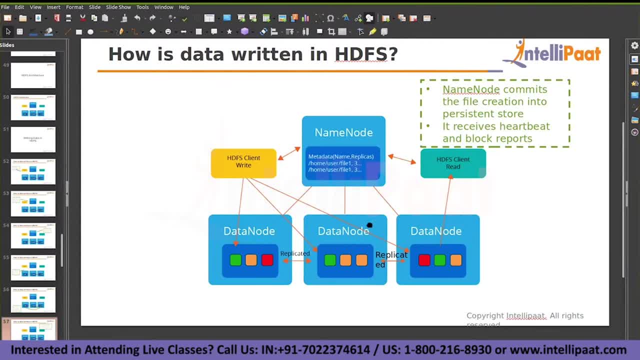 so every data node has to send the block report at specific intervals. so just to keep the data name node updated, so how many blocks it is holding, holding just the info of how many blocks it is holding and which data node block or which file it is related to, all that information will be sent. 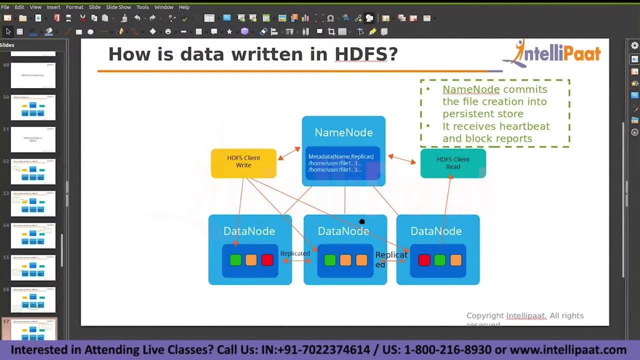 in the block report. so there is two heartbeat signal as well as a block report which the data node keeps sending at regular intervals. and then, yeah, we have a client gets the data node list from the name node. this is for the read again. okay, so this is for the same read again, like: uh it, you, you, your. 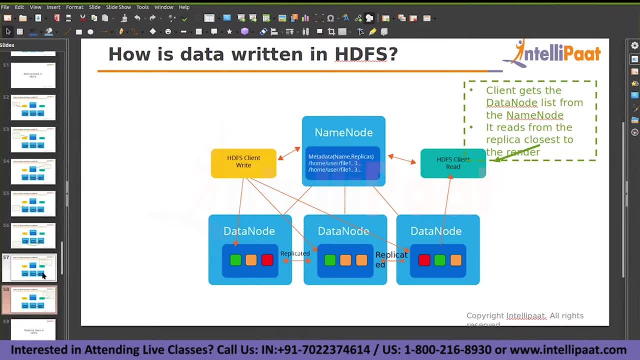 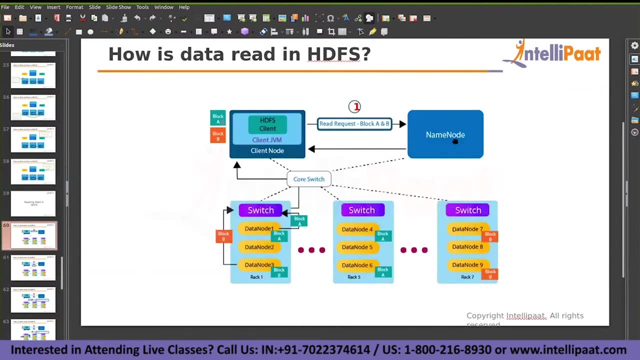 hdfs client read will, uh, will, will go to the name node and it will uh request for the information where this particular data is being written. okay, then we have reading the data in hdfs, so this has a lot of information yet. so this is your um client, hdfs client and you have a read. 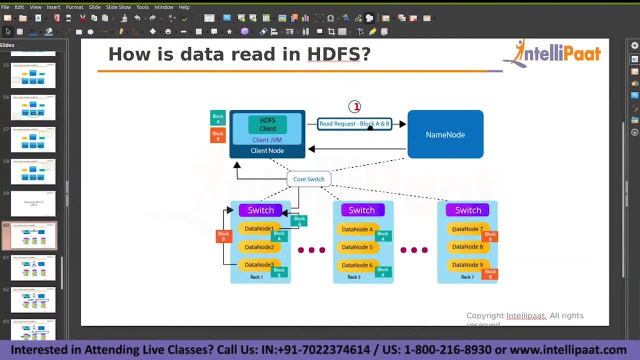 request that is being sent to the name node. so what is what does this read request consist of? read request consists of information that is related to block a and block p, so i'm trying to read the block a and then the name node will send the ip addresses of data node one and data. 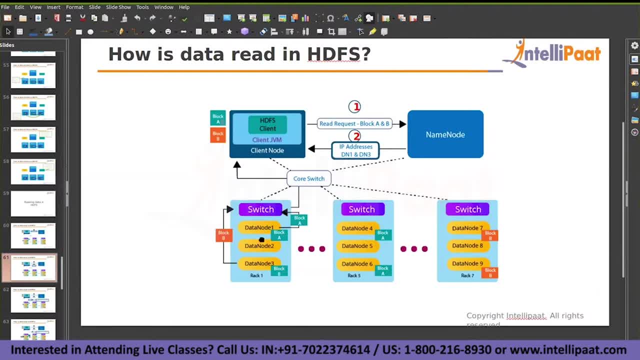 three. so where is block a and b available? block a is available on data node one. block b is available on data node three. right, so this information is being sent to the client. similar, similar information. so don't get, don't get scared or don't get uh, deviated by the diagrams. i'll tell. 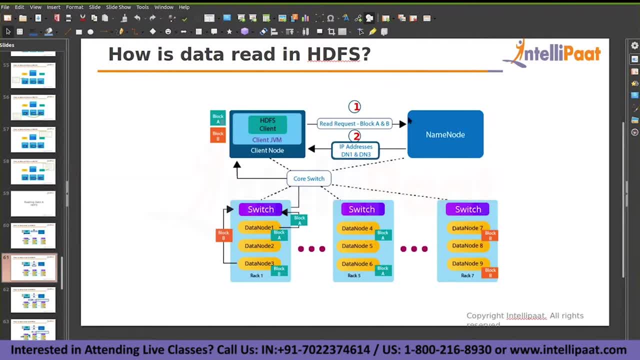 you what is the switch and all that. so read requests sent to name node. name node will send the data node information. it's just the list of data nodes, so forget about ip address of dn1- dn2. so you are. you're getting the information of the data nodes where this block a and block b are. 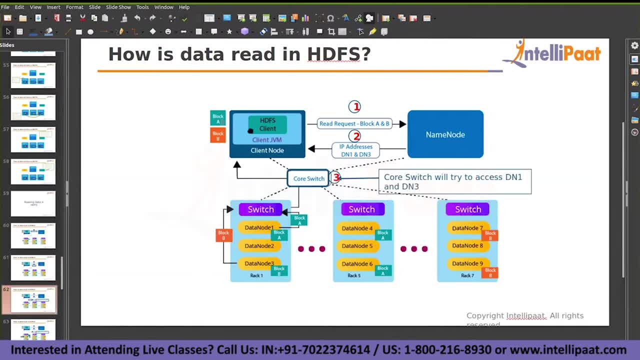 available. so now it's a. it's a job of this particular client to go and read through the data nodes. so why is this core switch available so earlier? in the right operation? it was not available because this core switch is something which is going to read the data across all the data. so 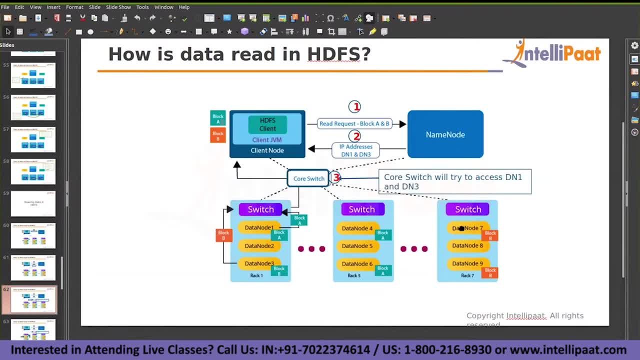 forget about this course, which so read operation. how is it going to happen? it will happen on all parallel right. you, you kind of read the data across all the data nodes. so there has to be some kind of a mechanism where it has to access, it has to control, it has to, it has to- uh, read it. 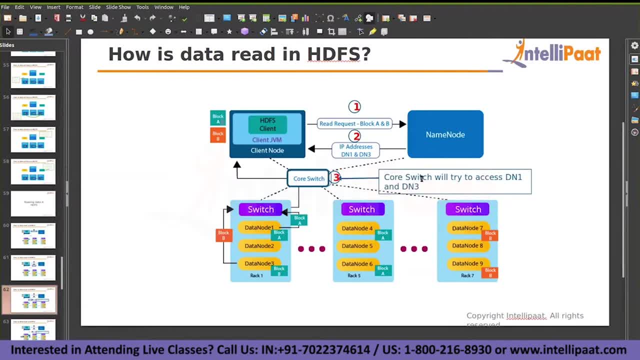 from different data nodes. so this course, which is helping you to read the data from data node one and data node three, it's it's kind of uh try to access both data node one and data node three. so earlier in right operation what has happened is like your date uh client has gone to the data node. 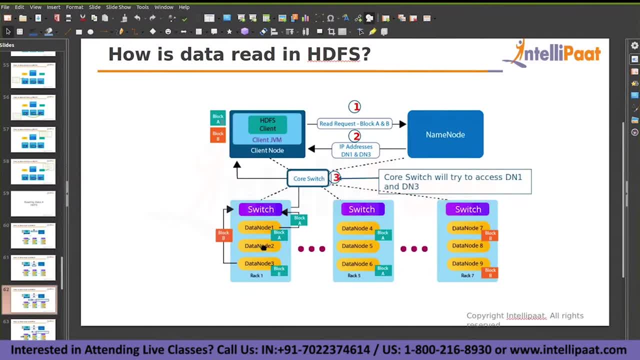 one finished all the right operation and then gone to the next data node. so it's all serial, it's all sequential. so, you, you do the right operation one after the other data node, but whereas the read operation can be done across all data data, all the data nodes, then what is? 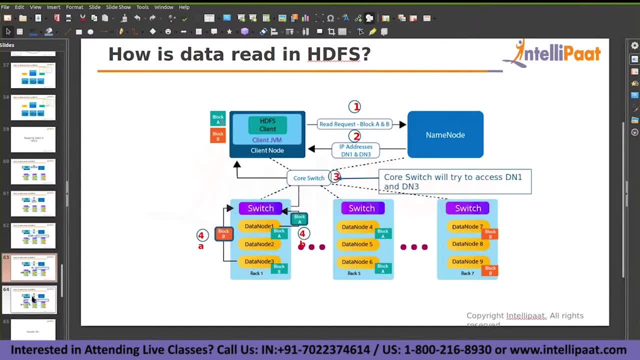 the next one. so this block a is being uh retrieved and then you have a block b is being retrieved. so both the information of this block a and block b is sent to the uh uh actual client from the from course, which okay. so block a is here, block b is here and there is also block a in data node four. 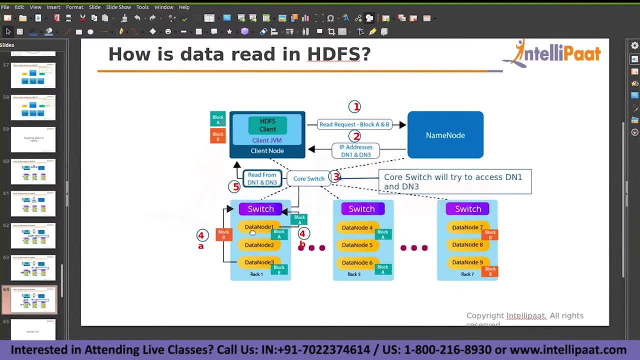 and six that they are not being shared because this is this primary data block is available. these are all the replicated blocks you can consider, okay, so, uh, yeah, so any questions on this? the diagram seem to be a bit complicated, but but keep it simple. what you are trying to do is you are trying to read the data from name node. 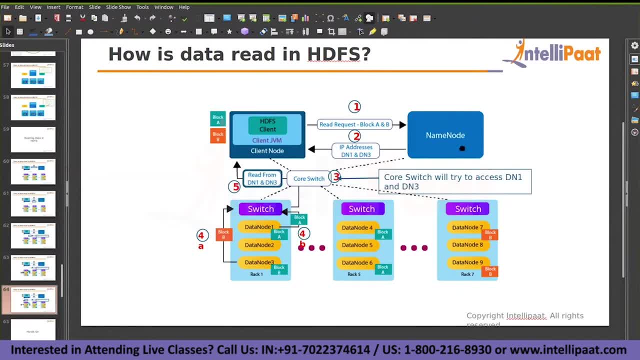 it will give you the information. it will access the internal metadata and it will identify which data nodes have the blocks a and b. it will give the information of these data nodes where to read from. so hdfs client will go and read on top of those data nodes and retrieve the data and send. 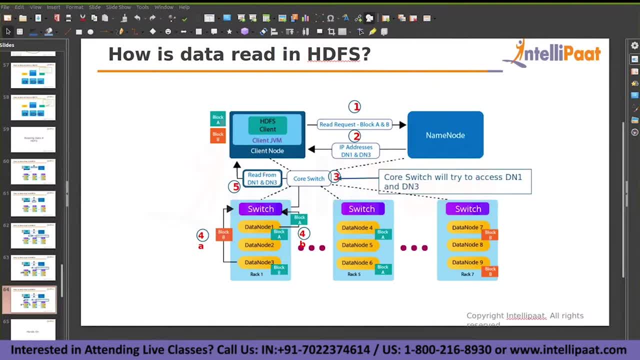 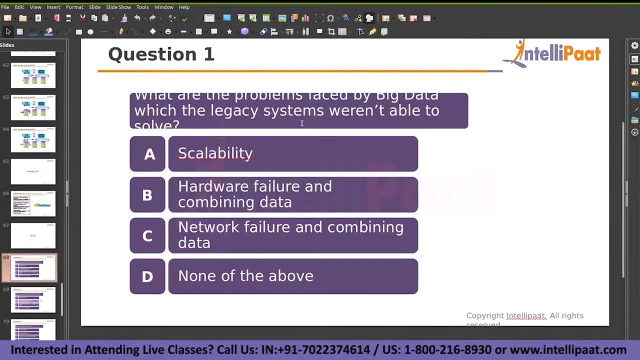 it to the client, whoever has requested it. okay then. so all right. so what are the problems faced by? there are some questions around five questions, i guess. yeah, and there are some five questions. so what are the problems faced by big data which the legacy systems weren't able to solve? so what is it? yes, what's the problem that? 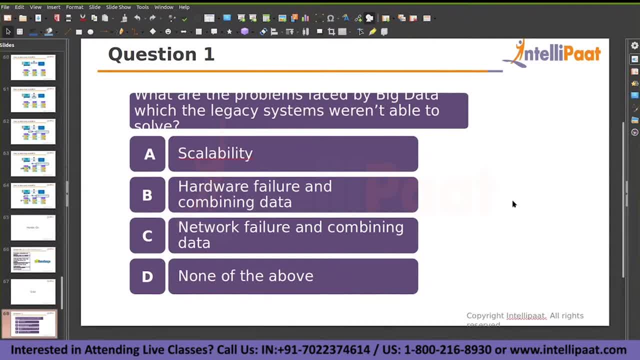 are faced by the big data systems which the legacy systems were solved, able to solve. there are two problems that will be listed. yes, anyone. what is scalability? increasing the number of nodes or decreasing the number of nodes? scale up, scale down and all that right. so in earlier, 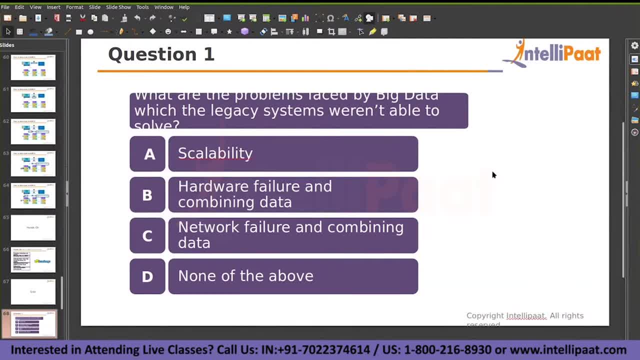 systems in existing systems? do we have a provision to scale the systems, to scale the number of nodes? we had we had, we have we can increase the systems. yes, we can increase the systems as and when it is required, but it's not something which has come into big data only, right. so 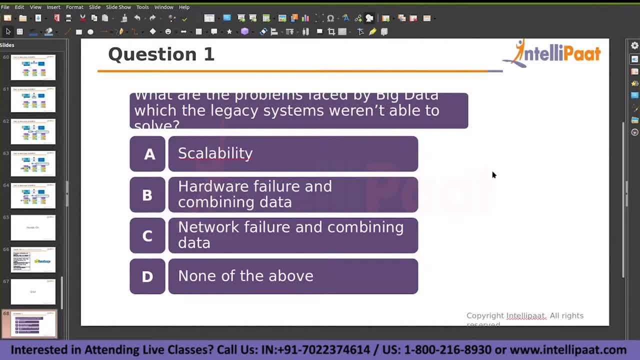 hardware failure and combining data. so in existing systems also. um, when we, when we are, we deal about some deal, deal with some hundred gbs of data, it's, it's not available in a single system. you remember even the oracle databases or whatever the sql databases you handle, they 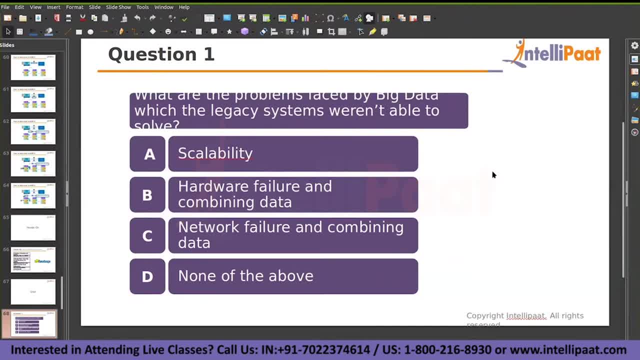 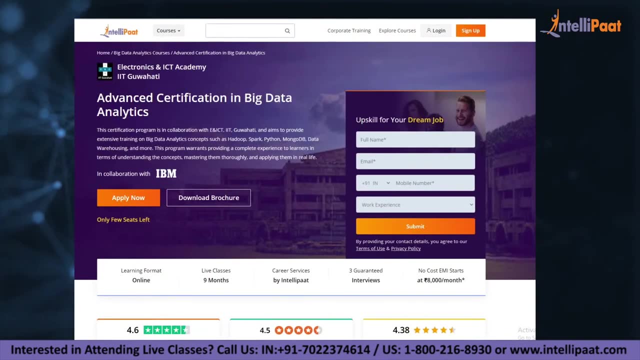 are not on a single machine, they are also distributed. but the problem is handling the failures. how are we handling the failures in hdfs in in big data? just a quick info: guys, if you want to make a career in big data, then intellipad provides some kind of a job for you as a data developer. 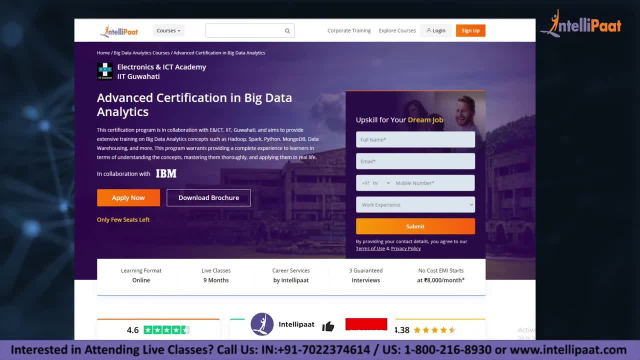 provides an advanced certification in Big Data Analytics by ENICT Council, IIT Guwahati. It is taught by IIT professors and industry experts With more than 10 years of experience. this course is designed to upskill and land your dream job. 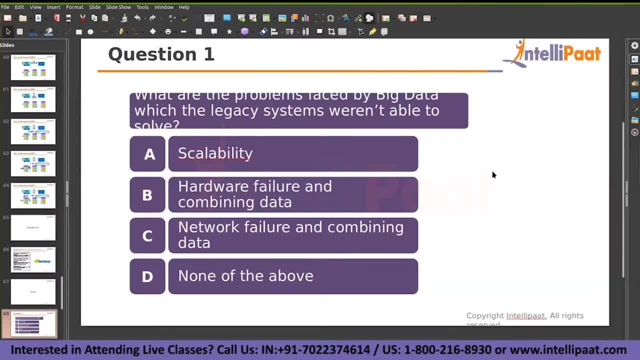 Now let's continue with the session. Why you have replications. So that is one solution we provided. And combining data. how are we combining the data Earlier? what is the problem? The problem with combining data is when you have to retrieve the data from multiple machines: 1GB on different machines. 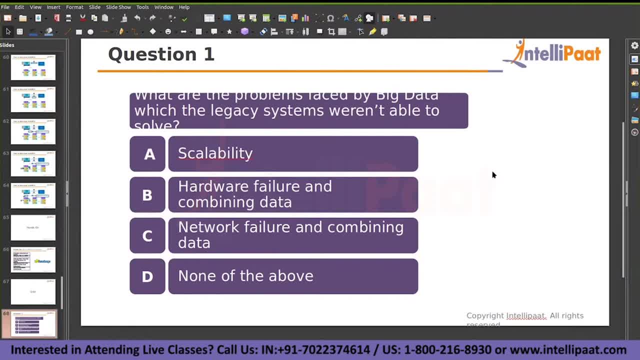 For example, I have 1GB on a single machine. I have 5 machines available. That means 1GB on each and 5GB overall. So if I have to run some query on this 5GB of data file, what am I supposed to do? 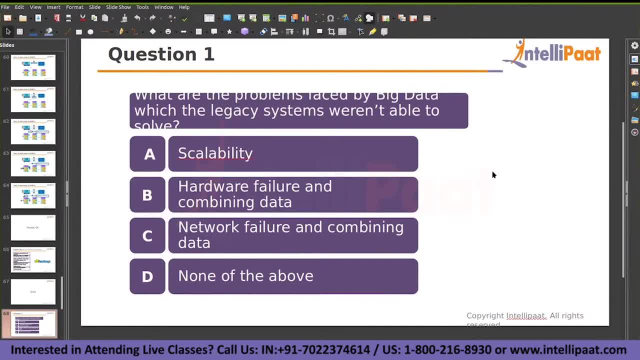 I'm supposed to extract the data from all these 5 machines, gather it at one place and then run the query. But with Hadoop, what are we doing? We are not moving the data anywhere. Data is going to reside wherever it is. 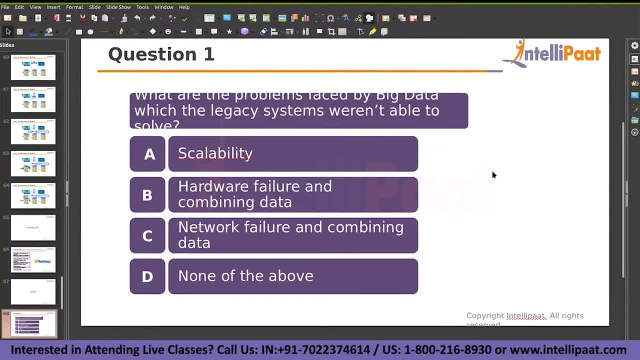 But we'll be moving the code to the data. So you send code to wherever the data is available and that will retrieve the results. So instead of moving the data, which is a very complicated task, you're just moving the code. 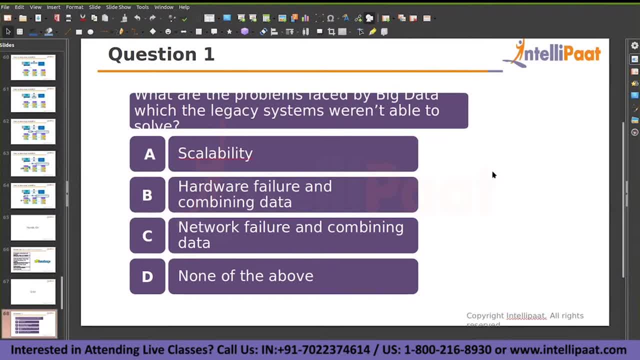 That is the problem we had and that is the solution we have provided. So network failure and combining data, Network failure: we have not discussed anything about the network failure So far. none of the airbow is also not the answer. 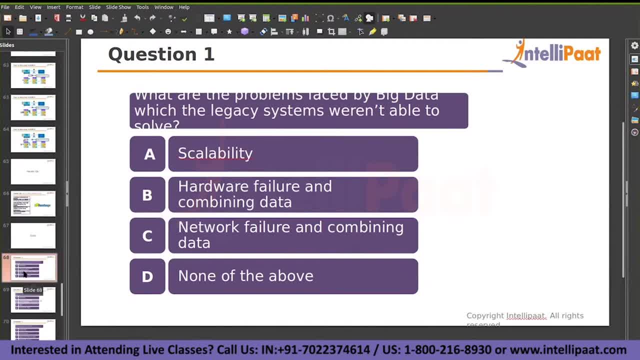 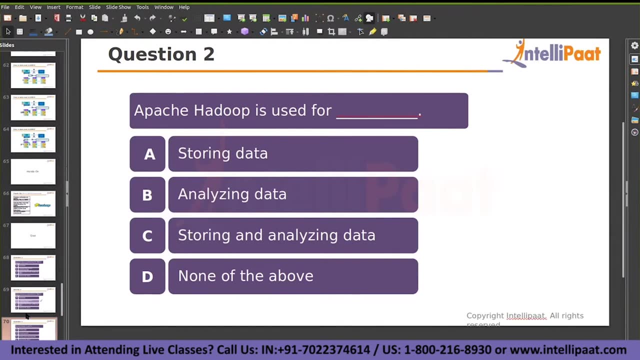 So the answer would be B, So hardware failure, and the combining data. So Apache Hadoop is used for what? Storing and analyzing data. analyzing data and storing data. So storing data. how are we doing? Which component is doing it? 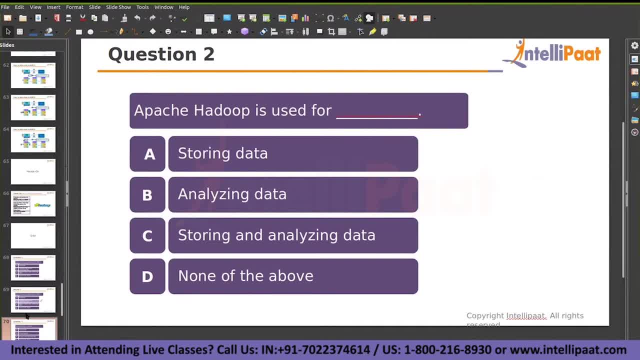 HTFS is doing the storage part And who is analyzing the data, Which module, Which component Method use? So the core components of the core functionalities of your HTFS is: one is storing, it which takes care of, which is being taken care by HTFS. 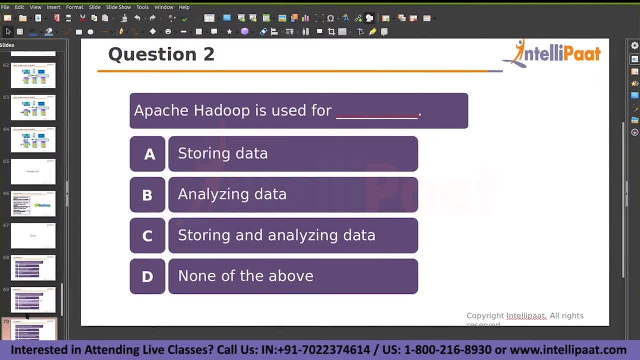 And the second part is the analyzing, which is being taken care by the MapReduce component. Then which command would you use for creating a directory in HTFS? So forget about HTFS or wherever we are creating. So what is the command that we use to create? 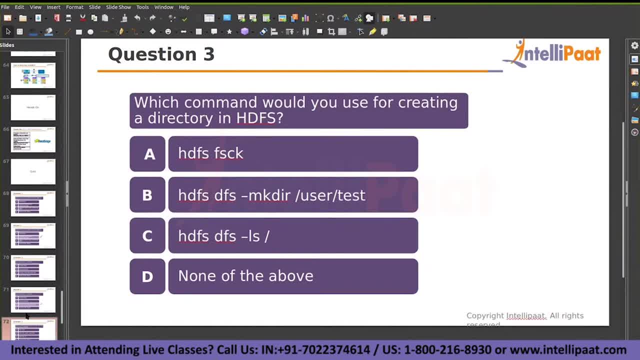 I mean in general, what is the command that you use to Make a directory? Use to create a directory? Yes. what's the answer? MKDIR. So forget about where we are creating it. In general, the command used to create a directory is MKDIR, right. 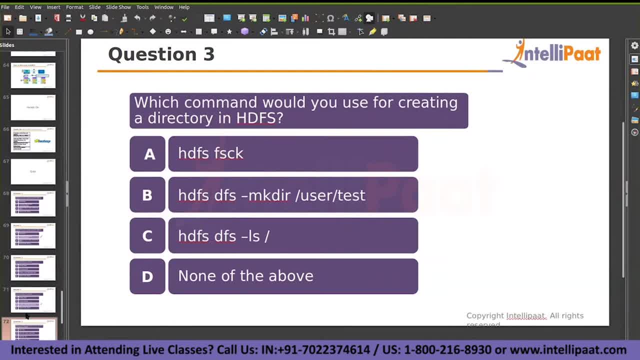 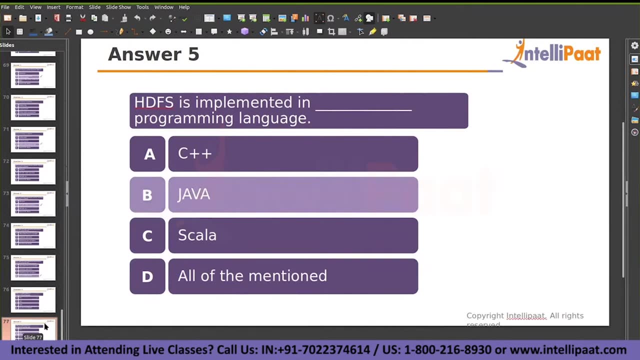 So how many of you are comfortable with the Unix commands, Linux Unix commands. So then, what next? HTFS is implemented in programming language. what, Oh my God? it failed in the first attempt, only is it Okay. 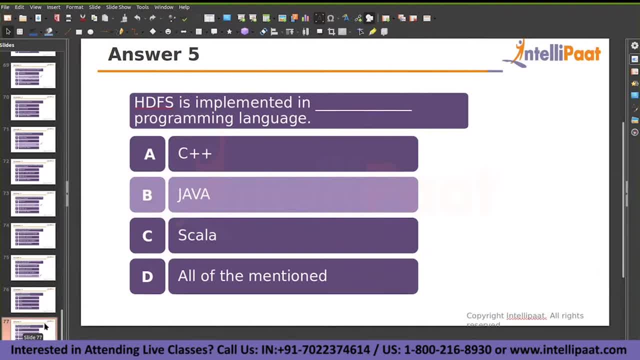 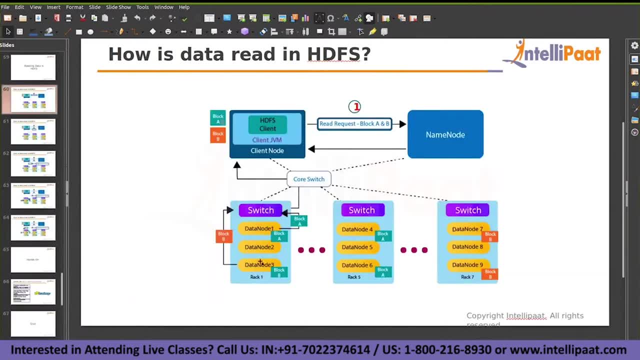 It's built on Java, Scala and Python and all that will come in Spark. Okay, fine, There is something called as a RAC written here, like we discussed about this RAC concept. So RAC is something where you have some multiple data nodes- whatever you say multiple data. 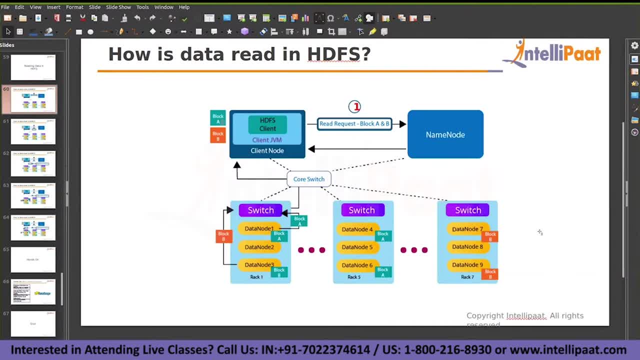 some groups. So you have a group of data nodes assembled together. okay, So data node 1,, 2, and 3 have been assembled as RAC 1, let's say Physical separation. I mean manually, as in if you're doing it on cloud, you definitely 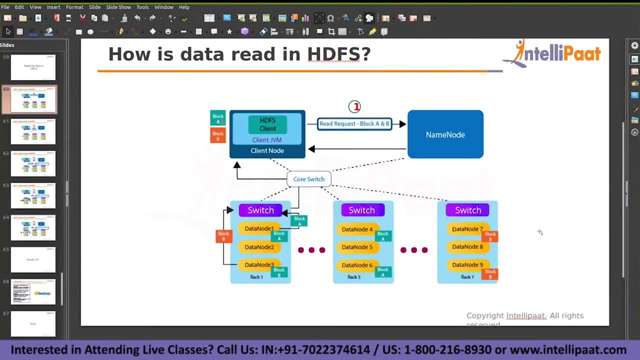 cannot do it, but that's the reason I was comparing it with the regions. Okay, So let's say, if you're doing it on, I mean see, when we have to give a justification, it has to work for all the scenarios, right? 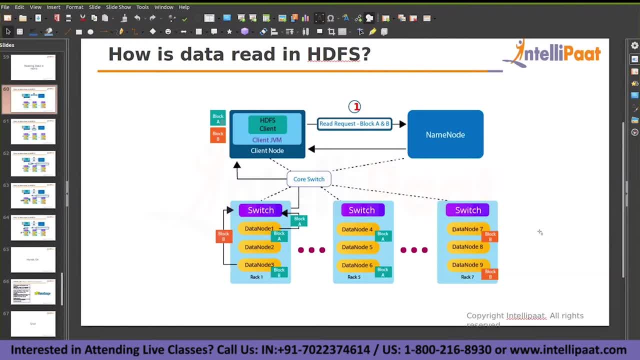 So, if I say in general, in other scenarios, for example, you yourself are configuring some kind of machines to the customer. So five machines have put it on one single network, one single RAC, and second, five machines have put it on another RAC. 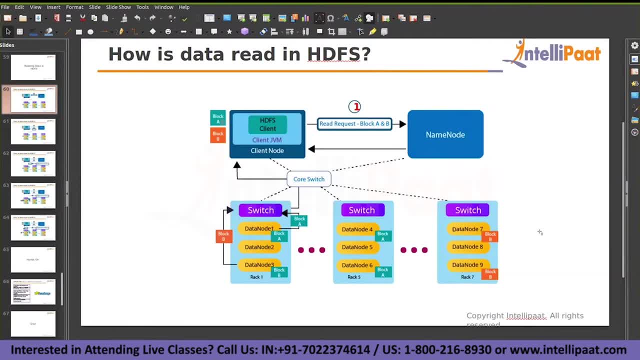 So that is something which you can do. This is a physical separation, or grouping the five data nodes together, but when you are configuring it on a cloud, so you cannot do that separation. So RAC is definitely a physical separation. It's nothing to do with the internals of Hadoop. 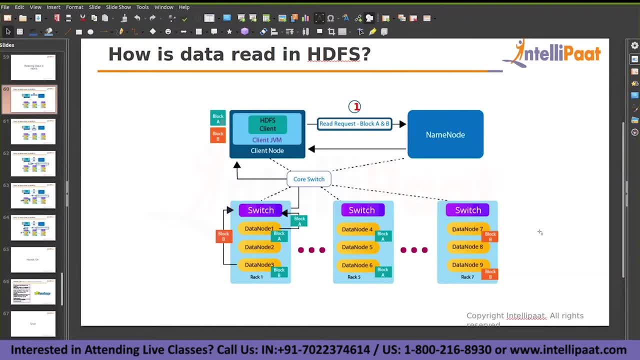 So when you're configuring it on a cloud machine, cloud network, so it's definitely impossible for you to configure, configure this rack systems right, so you definitely don't know which system is available in which particular rack. so in that case, uh, what i was comparing is i'm comparing it with them, with 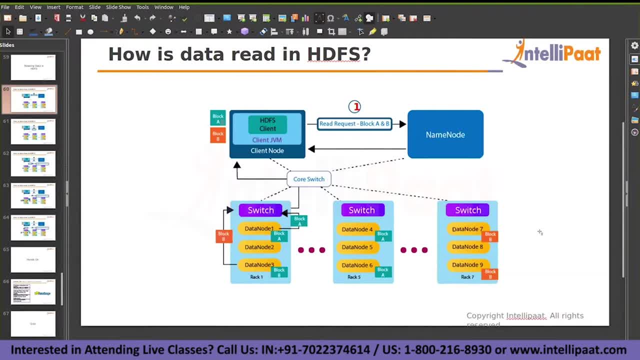 them with the regions. so us east is one region, us west is one region and mumbai is one region and you have other regions also. you create some 10 data nodes in us east, another 10 data nodes in us west and other 10 data nodes in mumbai region. so these are all the data centers i was 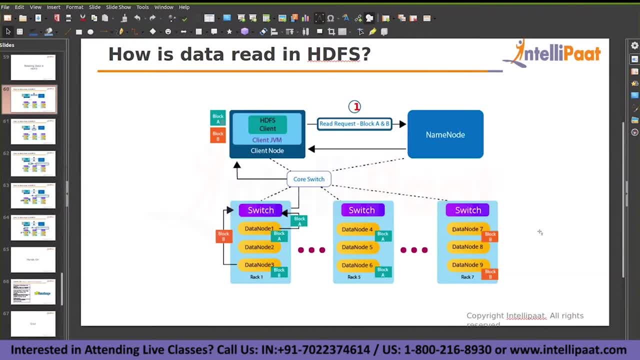 comparing it to right. so when you have this separation of these data nodes, a physical separation of these data nodes done, i mean, ultimately all the data nodes will will comprise to the cluster, but there is some kind of a physical separation that is happening. so there is a switch that is being uh, that that you are seeing there. so when you are trying to read the 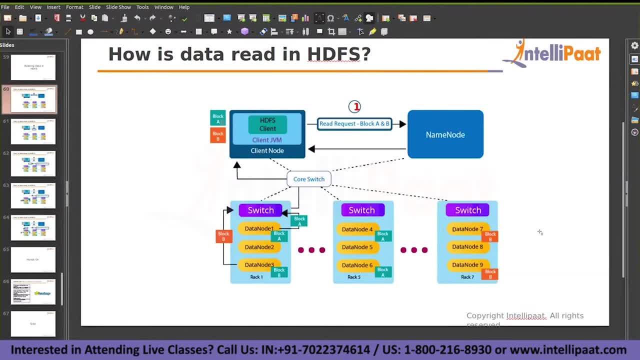 data from multiple data nodes together at a specific point of time, so read is going to happen parallelly. so when you are reading the data from multiple data nodes, there is a switch which is being switching from data node one and data node. in this scenario, this, which is switching from data node one and data node three, data node one. it is reading the. 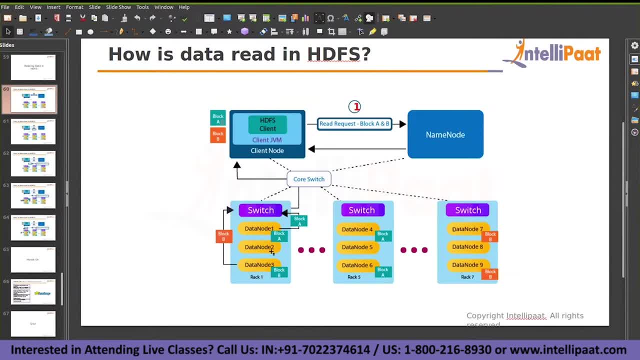 data for block a, data node 3. it is reading the data from block b. okay, so there is only one connection, there is only one single line of operation which is reading the data from multiple data nodes. okay, so your client is not directly accessing data node 1- 1s and data node 3- 1s again. 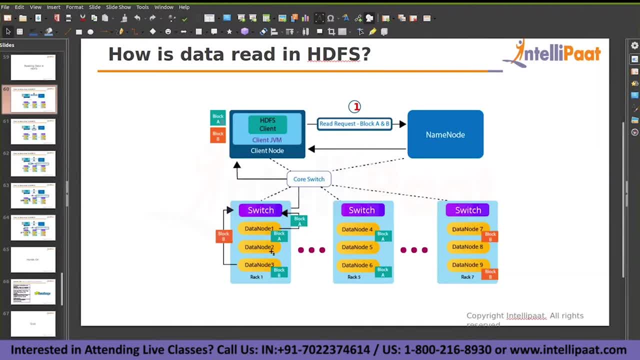 so, using a single switch mechanism, you are reading the data from data node one and three simultaneously and the output you are sending it to the client together. i mean whatever the data node, block one, block a and block b- you are sending them together to the client. that is the reason i. 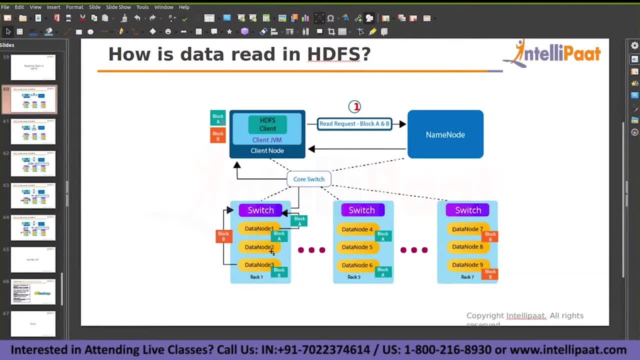 was saying the parallel parallel read operation, but whereas in the write operation you will not do it parallelly, you will not write the data using a switch on data node one and data node three. you will finish writing the process of data node one first and then the client will send the request. 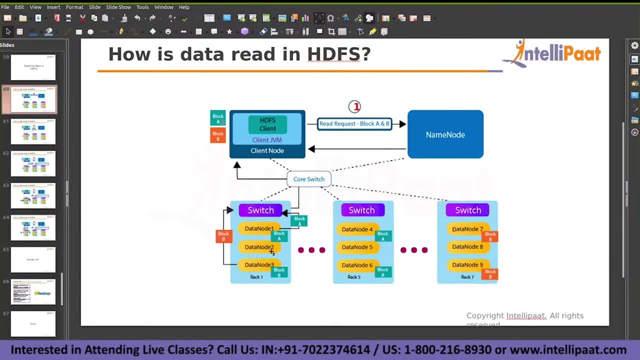 to write the data node three again. okay, so after finishing one data node, you will move on to the next data node and write the data. but read can be done parallelly, the reason being the data is already available, you just have to know where to read it from. the data is already stored and it is 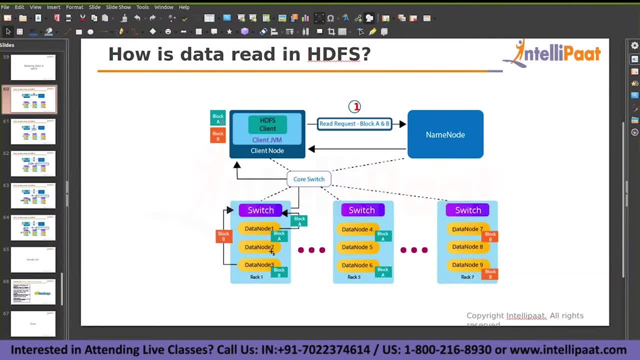 available. so why? why waste time in reading one after the other, right so, the reason also being, for example, there is a file, hollowtxt, let's say, which is available in the data node one and three hollowtxt. okay, so when you are writing it, you will break, you'll be. 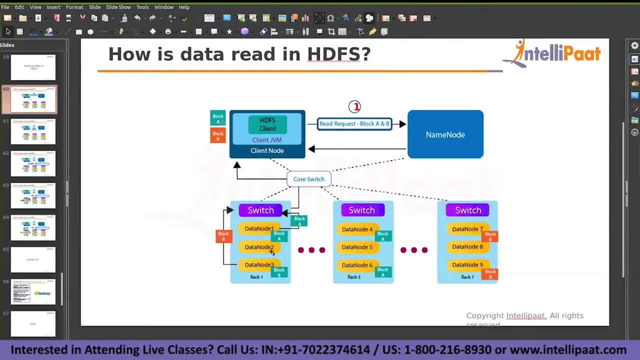 breaking that hollowtxt into, say some 10 blocks. okay, 10 blocks, you have broken it into and you are writing them into data node one, two, three, four, five and six. okay, so let's say, five data nodes i have written. that's fine. i mean, i'm breaking that into some 10 blocks and i'm writing it into. 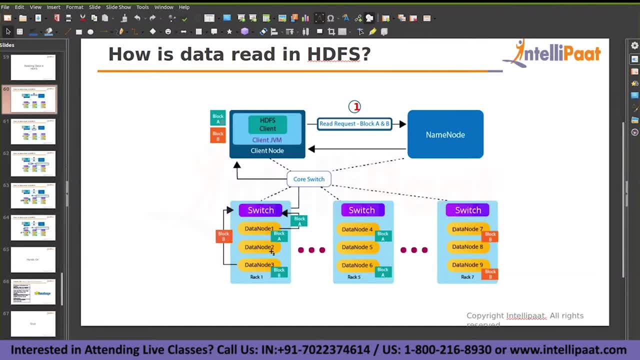 different, different data nodes. but when you are reading it, what is the expected outcome? when i say: how do you read the data is hdfs, dfs, hyphen, cat, hollowtxt. this will get you the contents of your hollowtxt. how am i supposed to get the data? should i get in something like: uh, first, block data. 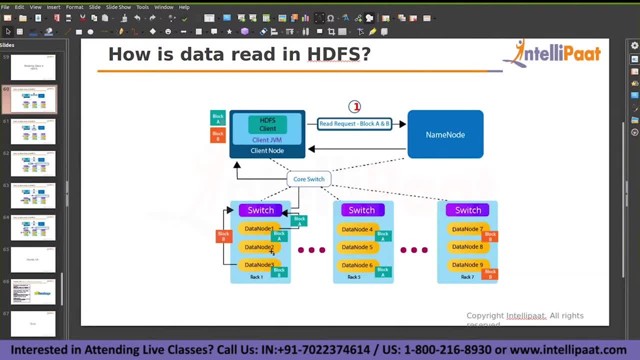 i'll get in line one first. second block data. i should get in line two. third block data. i should get in line three. it shouldn't be the case right when i do a cat. i should get the whole hollowtxt file. that means i have to read all the data nodes together. i'll have to join them or i'll have to. 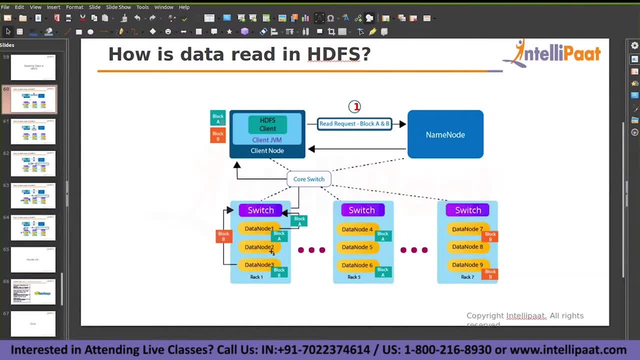 touch them and i have to present the read request together in whatever the format i've stored it right. so now, if you're, if you're, let's say you're, you're reading it with a form of a switch. so the first block, a first data node, has got the 10th block. the second data node has got the fourth. 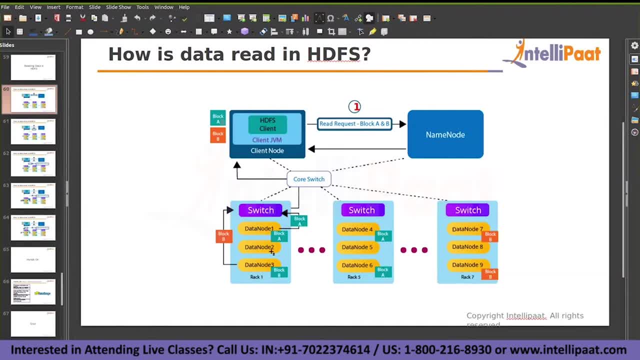 block. the third data node has got the seventh block. let's say something like that: so your switch is reading across through different data node blocks. and let's say you're you're arranging the in the in the form of a proper format to the client hollowtxt. the entire file is being read. 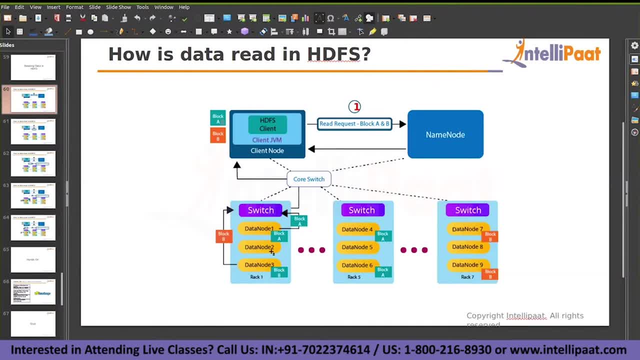 and will be sent. when your client is going to the data node one and data node three separately, are reading the data, the first output you get is from data node one. then after that you will get an output from data node three. but that's not what i'm looking at. i should get the data in the form: 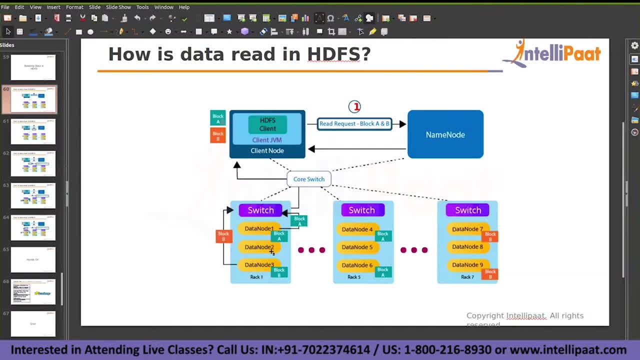 of a hollowtxt file where you have all the contents together. right, that is the reason we do a parallel read using a switch. okay, so there is no component such as a core switch that is being sent to the client at once, which are something like this: inside your, inside your. 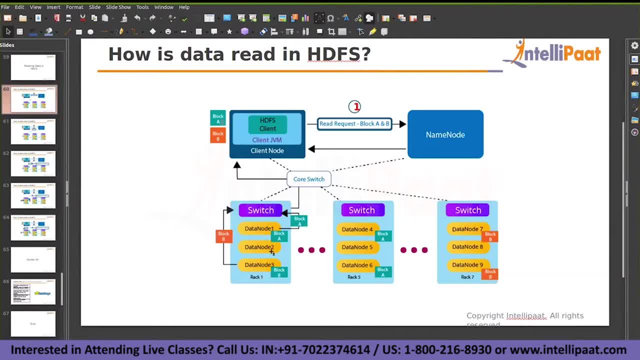 client or inside your adobe cluster. but your your name node will make sure you you read from so and so blocks together and your, your client will be able to. your client will be able to see the data all together as a one single file getting it. so it is some kind of a threshold where all the data 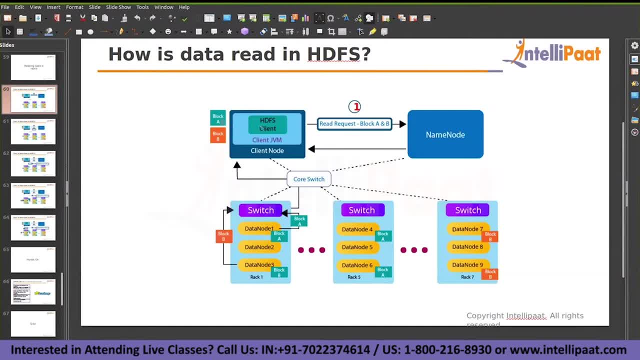 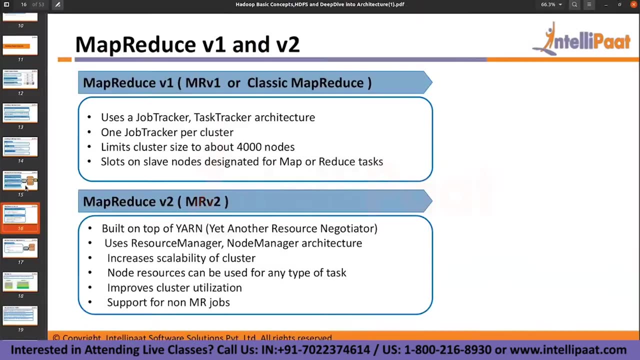 is being pulled in here and is being sent to the client at once as a single file, not in the form of a block, the course which is kind of accumulating the data from all the other switches, and one single output will be sent to the client. okay, so this is. this is having some bits, and 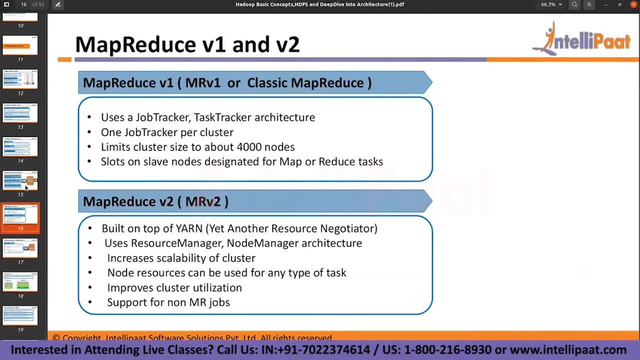 pieces of it, i'll come to the proper diagram, okay, so, like we have done using the draw io, we'll, we'll also do some apparatus architecture diagram in detail, but let's, let's just try to understand what is being listed here. so, uh, we, we have seen as the 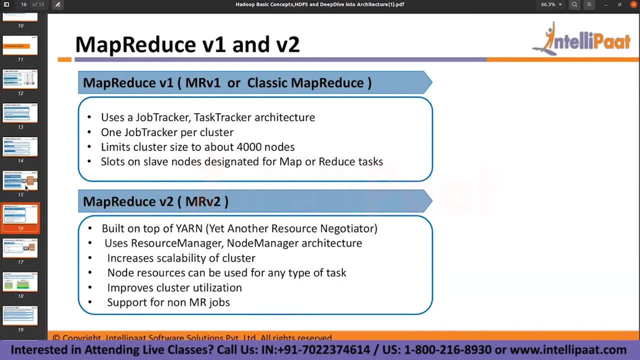 hadoop, generation one and generation two. did you, did you remember the discussion that we had as architecture? what is generation one? what do you have in generation one? name node, data node is is paka? it's gonna be there, but do we have secondary name node in generation one? 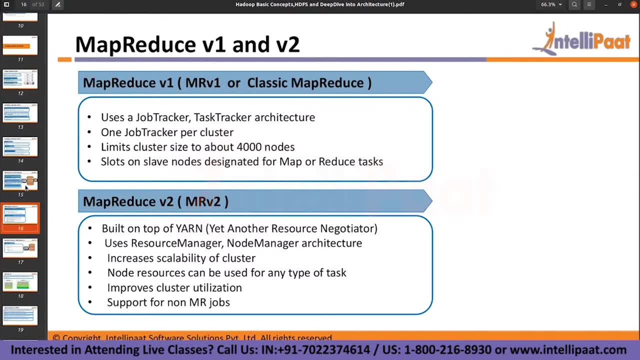 and generation two. what did we add? what do we have in addition in generation two? okay, that's one, the number of clusters is increased. okay, some active and passive name nodes, but yeah, so in generation one you have a name, secondary name node, guys. so name node, data node and the secondary name node will be part of your. 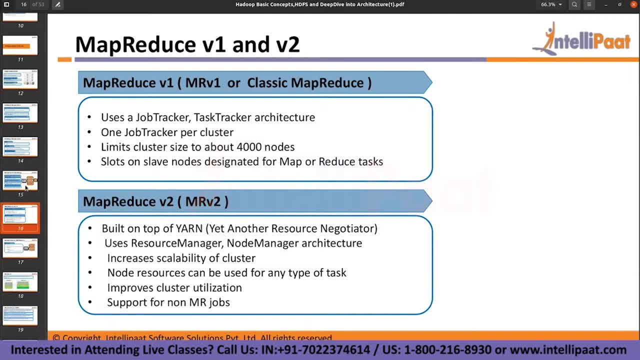 generation one and in generation two the addition that we have made is only the active and passive name node. so just to avoid the single point of failure on the name node, you kind of created a backup name node, actual backup name node, right? so hadoop one is holding name node, data node, and second, in name node, hadoop two is having active, passive name. 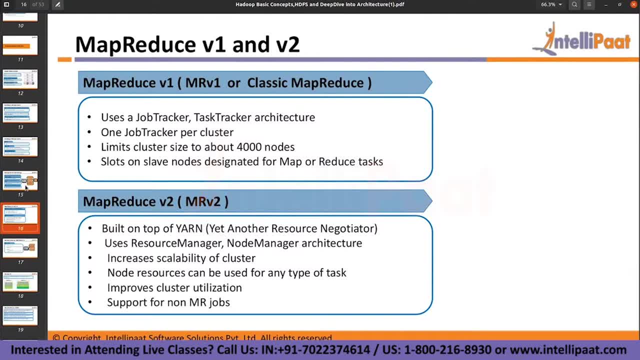 secondary name node and in the data node. okay, so similarly, a MapReduce also has two versions of it. okay, version 1 and version 2. generation 1 and generation 2. so MapReduce version 1 is considered as the classic MapReduce and MapReduce 2 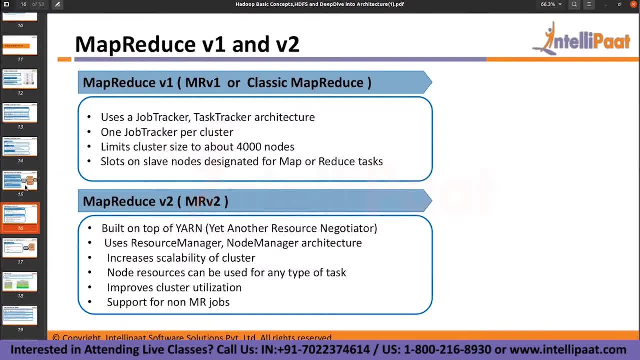 is considered to be a YARN- yet another resource negotiator. okay, so YARN is a different architecture altogether, so it's not something like your HDFS where you have made some minor changes to it, but the entire architecture flow. the data flow is has been changed in the MapReduce 1 to 2. okay, so we will first. 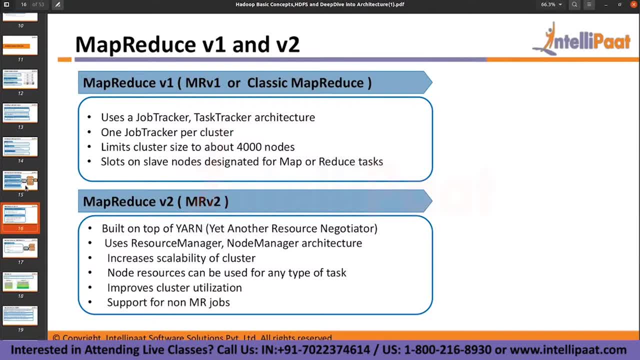 understand what is the basic core concepts of MapReduce, how it is actually being developed and what is the main purpose of it, and then we'll move on to the architecture of MapReduce 1 and then we'll understand the MapReduce 2 architecture. so with that we will, we will have to close the Hadoop. 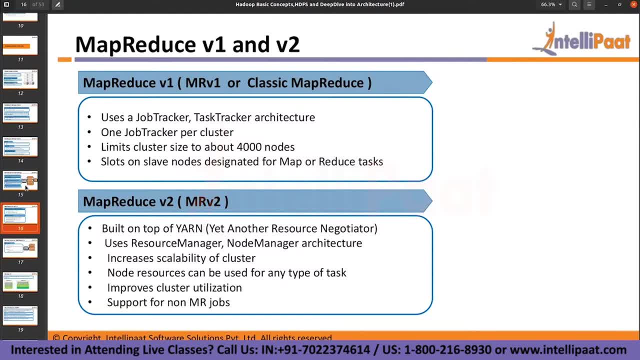 introduction. so Hadoop, HDFS, MapReduce 1, MapReduce 2, and we will be will be coming under your basic introductory course. okay, all the other ecosystem tools were not part of this particular discussion, so after we complete this, we'll move on to the Spark, right then? so MapReduce, what is it? 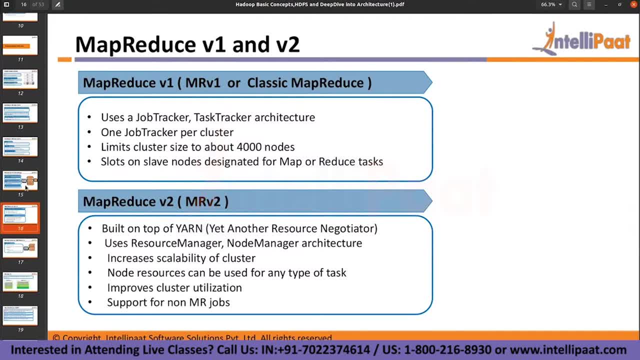 used for MapReduce is some kind of a data processing tool. so after you store the data in Hadoop HDFS location, you have to do something with it. right, you have to do some kind of processing, do some joins, do some aggregations, filters or whatever. whatever the processing. 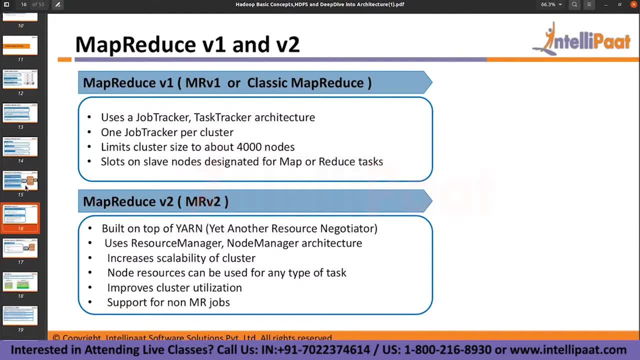 go nuts other. so all these basic things will be explained by third wheel. tenho thatших actions. the next day you go and you write. you write these data from your USB. is this method of Gmail that is called notice, so you will have a list of all the methods you have using the map reviews. so map reduce is. 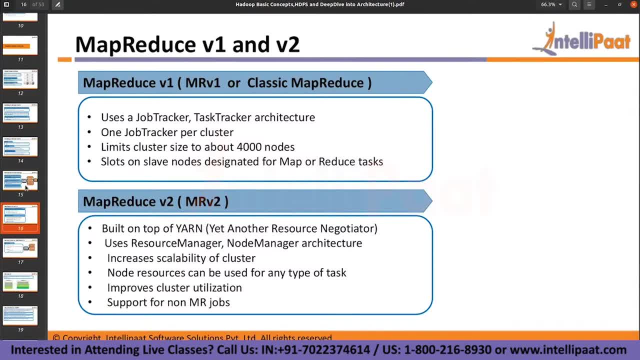 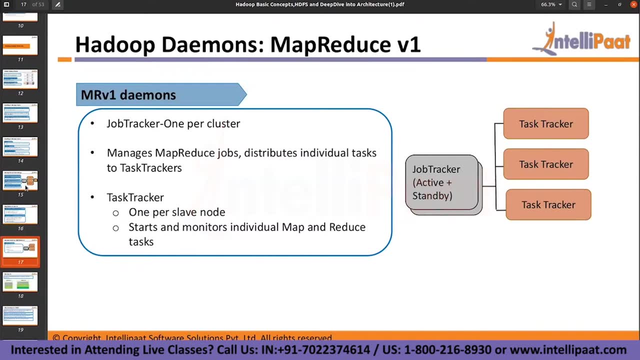 basically built on Java. using a specific Java program, you're gonna do the transformations. you write some logic, insert the MapReduce program and you submit that jar file to the map reduce engine. it will. it will execute and do all. two more uh components: one is the job tracker and the other one is the task tracker. okay, so job. 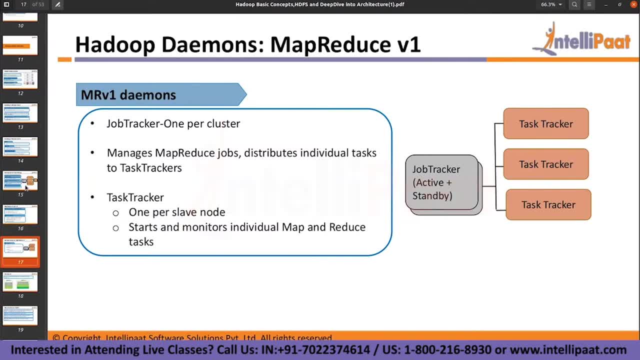 tracker is the master again and task tracker is the slave. okay, so like we had name node and data node in in hdfs, uh, mapper reduce has job tracker and the task tracker. okay, so these are all called as the demons guys services. i can say so. hadoop has five demons, the generation one hadoop has. 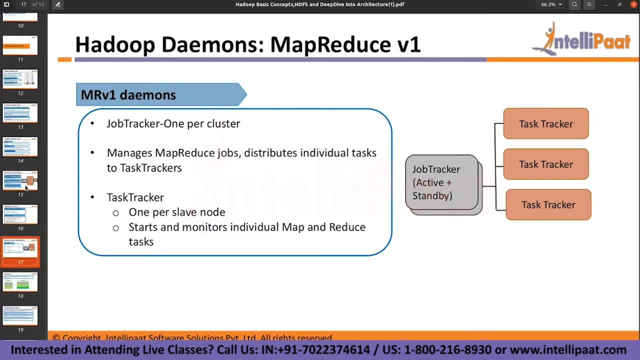 five demons. one is name node, data node, secondary name node, job tracker and task tracker. these are the five demons available in your hadoop cluster. okay, demons, as in the services. so you, when, when you run these services, you, your hadoop cluster is said to be available, right, so map master is. 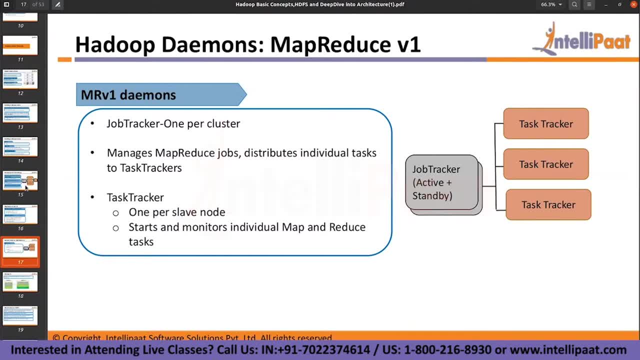 the job tracker. slave is the task tracker. so whenever you are supposed to submit some kind of a job, when you are trying to execute some query, you are supposed to send it to the job tracker. that will identify the job and that will run that job using the slave machines, using the task tracker machines. okay then? uh, we've seen this hdfs hadoop. 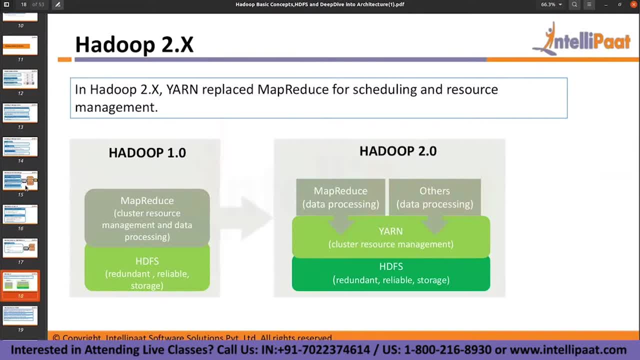 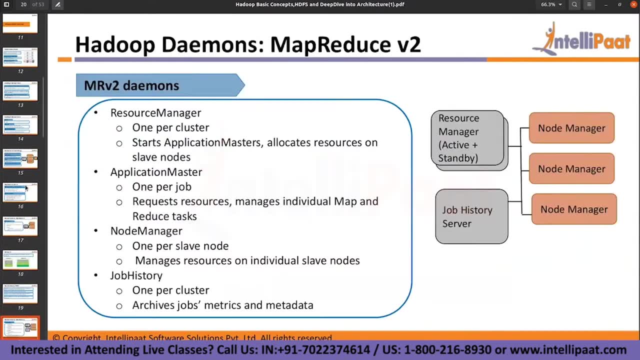 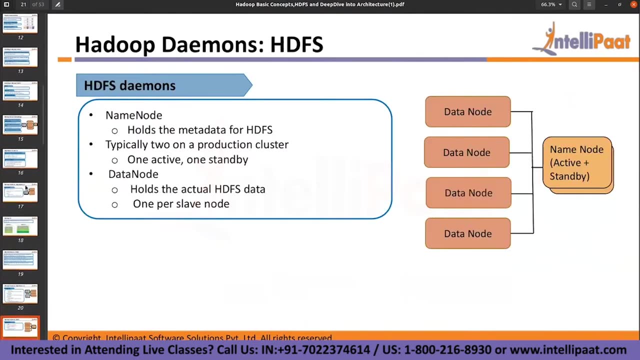 one. uh, how is it different? we will. we will come back to the 2.x version. what? what's the change that we have done? but forget about all this yarn things. now there is another document, altogether yarn. so don't worry about all this now at this moment. okay, so i'm just quickly moving to the 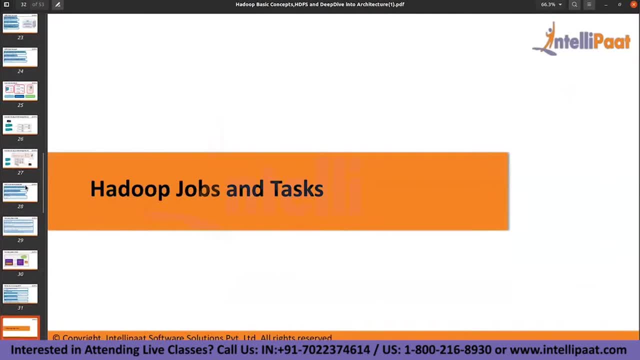 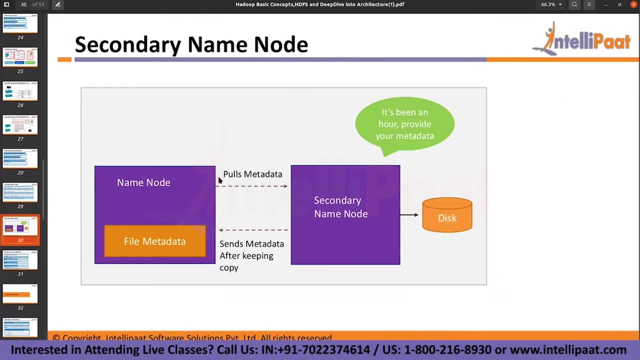 this hdfs is done and yeah. so this is some diagram for the secondary name node. guys, if you just just look at it, this is your name node and this is your secondary name node. so there is a metadata available in the name node. so it's going to pull the metadata. it's going to keep a copy. 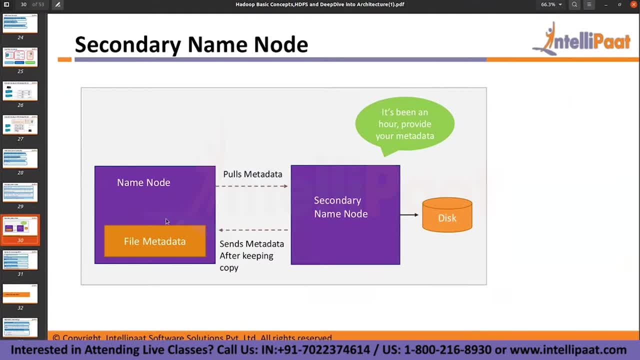 and sends a metadata after keeping a copy. okay, so it's just pulling the data, keeping it in the disk. back to the name node. this is the functionality of your secondary name node. so someone was asking for a diagram, the secondary name node diagram. right, so this is how it's going to interact with. 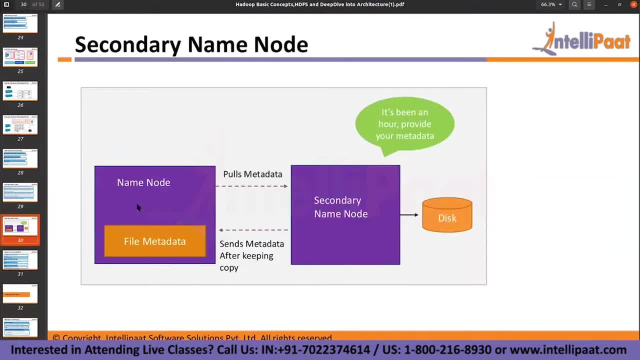 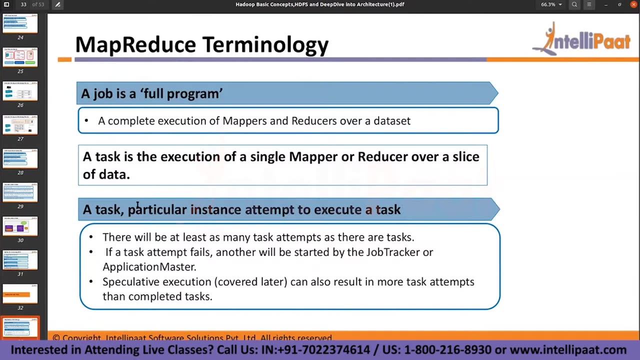 the secondary name node, then that only accesses the master name node. i mean that own. that's only going to interact with the master. it's not going to interact with any of the data nodes. so we are coming back to the again. we are getting confused again. okay, so a job is a full program map. 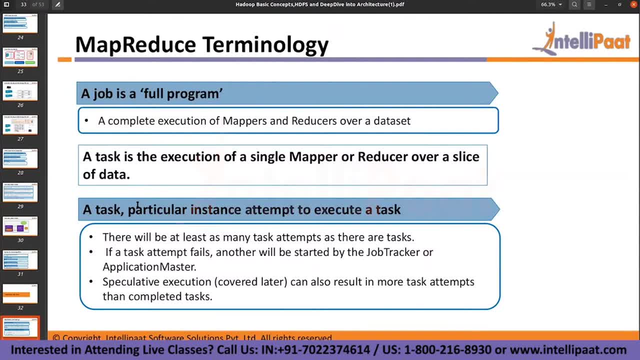 reduce terminology. we have something called as a job and a task. so job is a complete set of job, a program that we have written, the entire execution, is called as a job, and when you break that job into multiple chunks of activities, you call them as task. okay, right, so a client is. 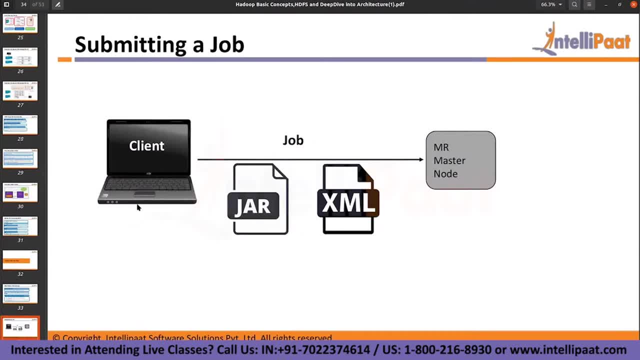 submitting a job to the map reduce engine. that means there is a, a jar file, or there is an xml file, uh, in- using which you will be submitting the data. you'll be submitting the data, you'll be submitting the program. okay, so, along with the jar file, you will be writing, you'll be providing the. 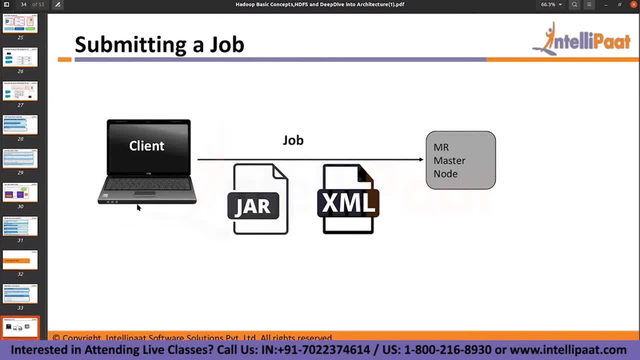 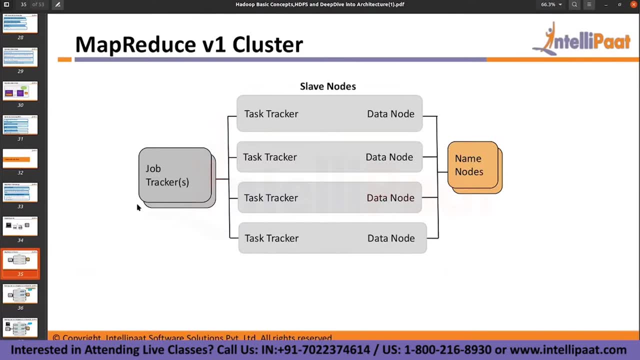 input location of the data and you will be submitting it to the master, to the job director. so this is a difference, guys. on the left hand side you have this map reduce. on the right hand side, you have this hdfs related information right. so when you are supposed to load the data, 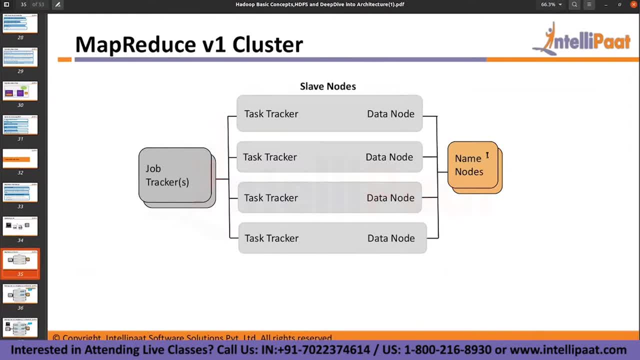 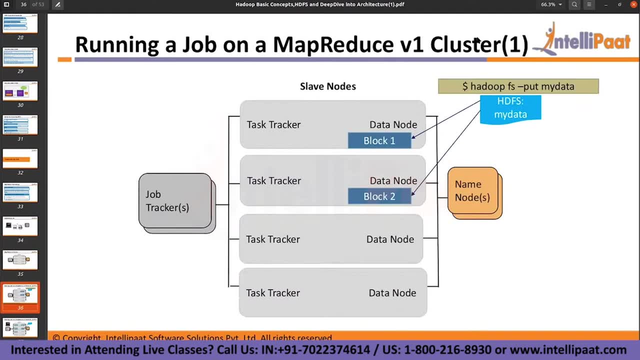 whom are you going to connect to? you are connecting to a name node, right, you are sending a request to the name node and you are storing the data on the data nodes. so this is this right. block one, block two: what is my data? this is my. my data is my file. i'm trying to load it into. 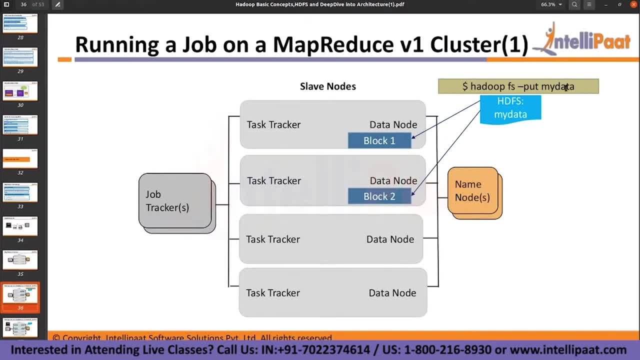 so, and so blocks. now, after loading this my data, you are trying to run some queries on this my data. you are trying to write some program and evaluate some data on the my data file. so whom are you going to submit this request? soon you'll be submitting that program to the job tracker, so 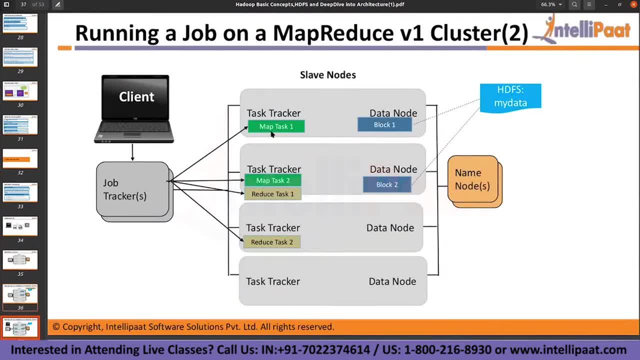 now the job tracker is running the task crackers on top of the data nodes, where the data is available, getting it. so there is a data available on your hdfs, on some so and so data nodes, so as and when you receive a program, as and when you receive a job to execute. 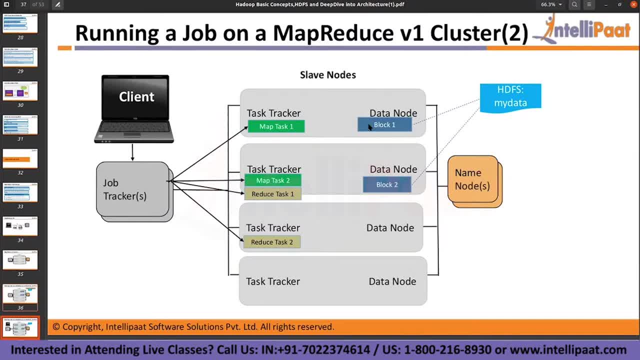 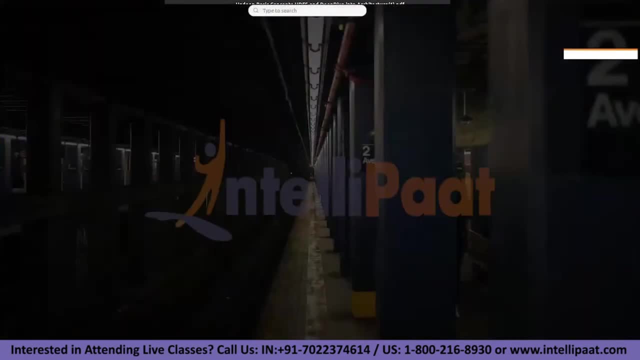 it will interact with the name node and identify which location the data is available. right, so after you interact with it, after you find the data nodes, the task trackers will run on top of that data nodes to execute that program. okay, so now going back to the actual 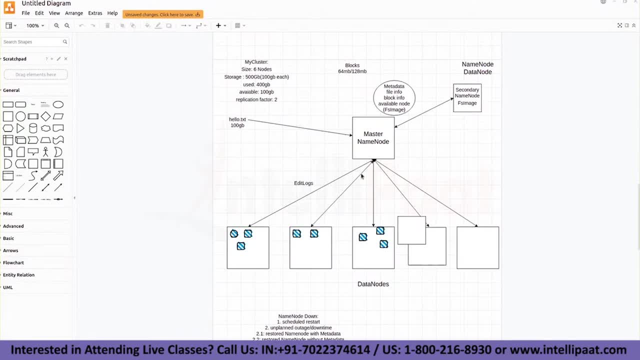 diagrams, right? so this is your master, which is going to be your job tracker, this one and these are all your task trackers, right? these are all your task trackers. on the other hand, there is hdfs. let's say: this is your hdfs, right? so now i'm i'm writing a program. let's say i have a, i have some, so the file is. 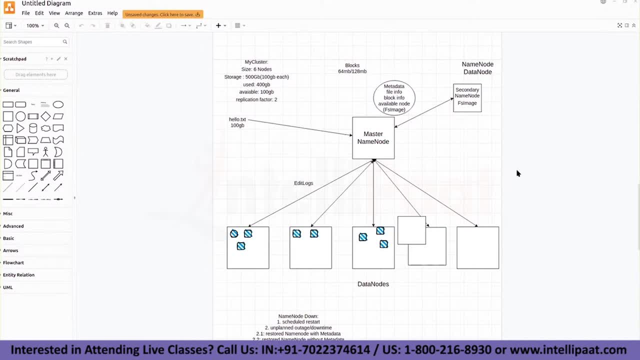 you know, i want say let's have the data哈哈, okay. so the first thing they need to do is go to the css. so if we go to css file and you see there is theтакit, um, user, um, voter championship, uh, data and c you have some data. so voterscsv consists of some 10 lakh records. let's say, are we clear? 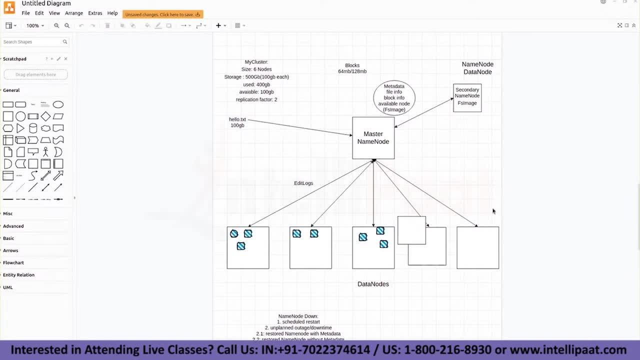 with this scenario. voterscsv is my file which consists of some 10 lakh records, and this 10 lakh records are available in the hdfs in the form of a voterscsv file which is consisting of the parties a, b and c votes list. okay, so for each and every candidate, whichever party they have. 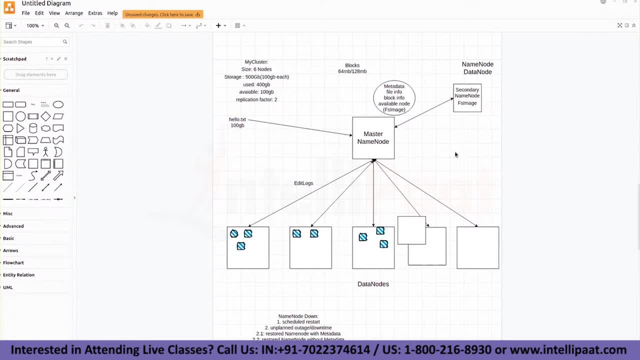 voted for that. that particular number is. that particular information is available in that csv file. so now i store this voterscsv file in hdfs. i sent a right request to the hdfs cluster. that means i'm sending a right request to the name node and i have written this voterscsv into. 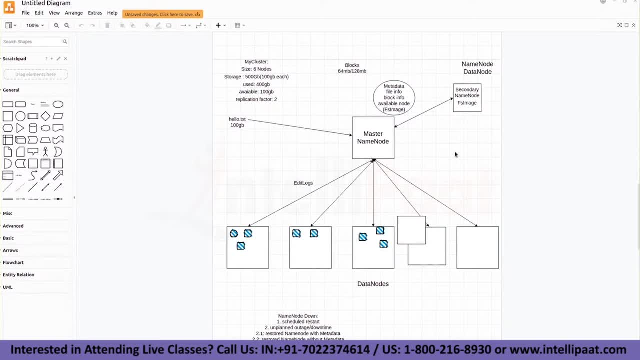 let's say four data nodes. agree, please? i have written this data into four different data nodes for our convenience. let's say i'm dividing the data equally accordingly, across four data nodes. okay, so there is no need of dividing it. but let's say i am dividing it into: 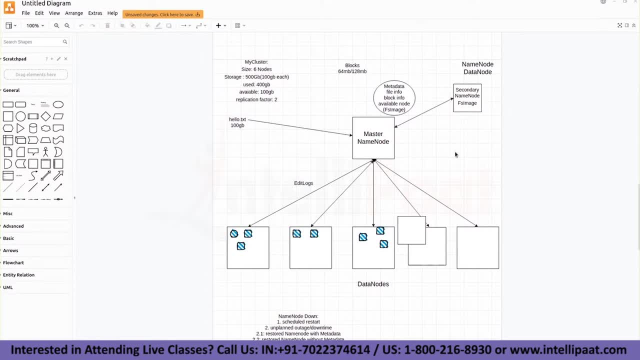 four data nodes equally. that means, each data node has how many records? 25 000 records. no, sorry, two point two point five lakh records, agree, so two point five lakhs each on each data node. i am dividing it into four data nodes in your hdfs cluster. this is my scenario, got it? so now i loaded. 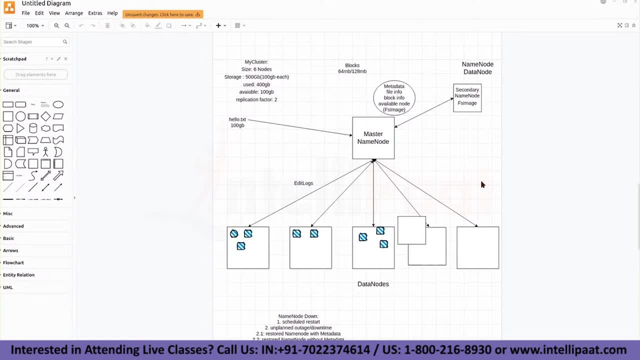 the data. i have the data ready, so now i am supposed to calculate the winner. the final winner- whoever is is receiving more number of votes, will be will be the ultimate final winner, right. so now i have to calculate whoever has got got the more number of votes. so i'll write a program here. so i'm gonna write a. 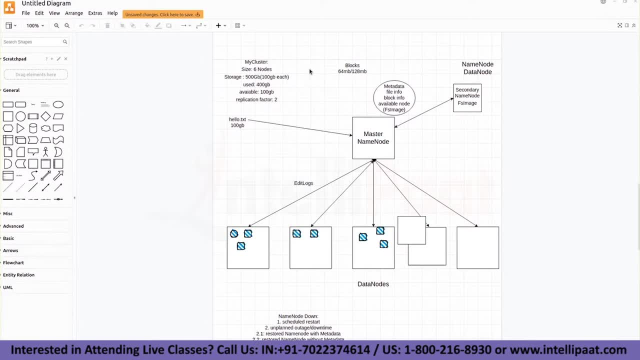 program somewhere here. map reduce program- see map reduce program- is a java program generally, so map reduce program. you have written a logic. MapReduce program consists of two classes. how many of you are comfortable with java, or at least have some basic knowledge of java? you know what is a class, what is a method. everyone right, you know. 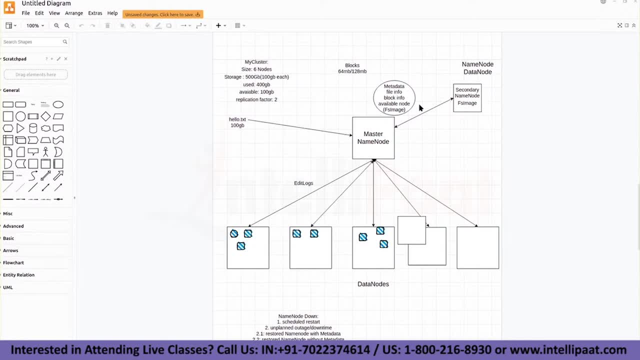 at least you know what is a class, what is the network. so a java program, a map reduced java program, always, always consists of two classes. one is a map class, one is a reduced class. okaya, mapper method as well as a mapper class as well as a reduced class. so you have to write some logic in this. 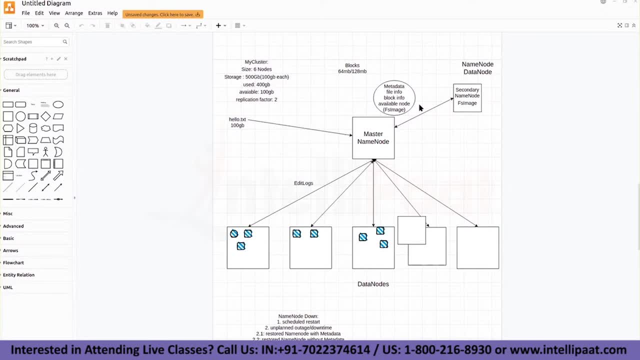 mapper, you have to write some logic in the red user. so that is why, uh, we call it as a map reduce program. so by default it's going to be mapper and a red user. so what happens inside that? on all that, we will discuss that later. so i have written some program, i have written some mapper. 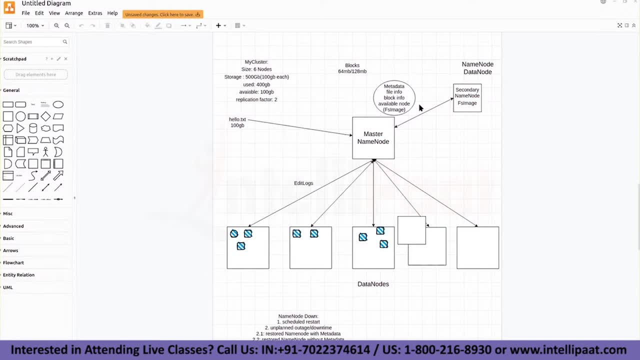 logic: uh, i have written some logic. one here in red user. i have written some logic, uh. two here: i have written some program and i have converted this into a uh pinner dot jar file. this is the jar file that i created out of this map radius program. 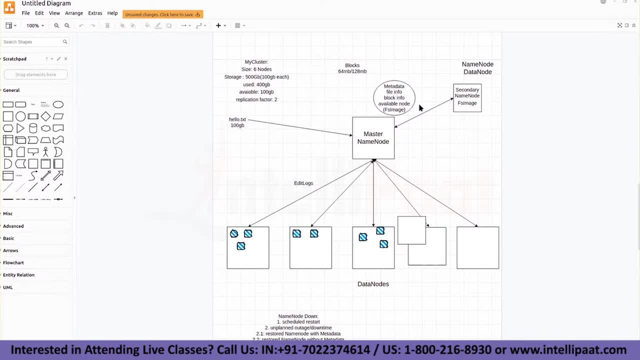 okay. so i submitted this jar file along with- along with the location of the data, home training. so here this voterscsv is loaded in. see if you are writing it into hdfs, you will find some location elected to it, so home training, and then you will find some directory where you will be. 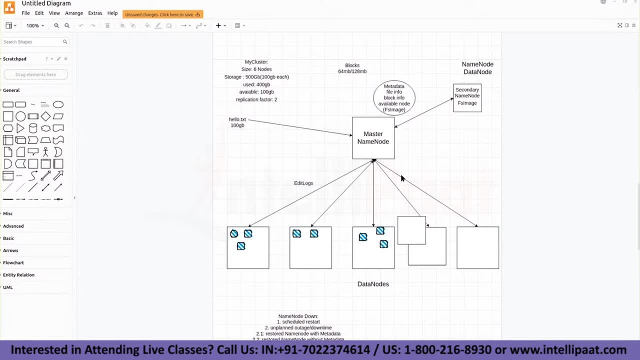 storing this data: data slash voters dot csv. this is the location of the file in hdfs, so similar location. i'll have to provide that in the jar, also in the jar file, along with the jar file: data slash voters dot csv. this is my input, this is my program, and the input for the program is the location of the data. 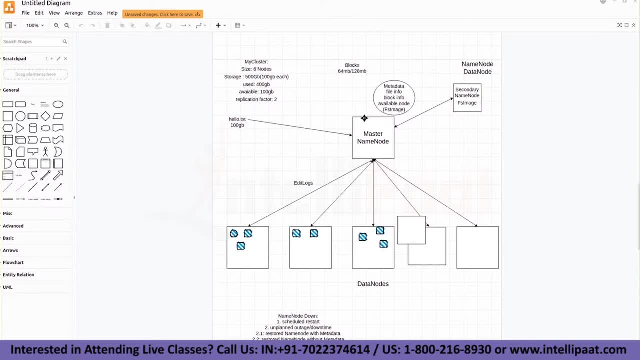 you submit this to your job tracker or the map reduce engine, for example. so what has to happen now? you submitted the program, you submitted the input file location also. so first my map reduce engine. i mean when you are submitting a request to the map reduce, that means you are submitting a request to the job tracker only. that is again the master right. 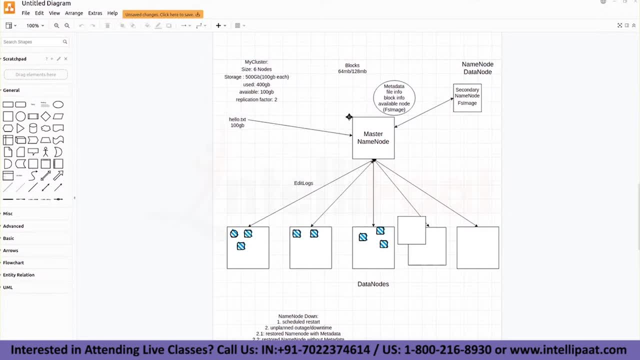 so your job tracker will analyze the program and will also look at the input data so it has to validate whether this particular data is available in hdfs or not. so job tracker is interacting with your hdfs first as and when a job is submitted, it is interacting with your hdfs whether this voterscsv file is. 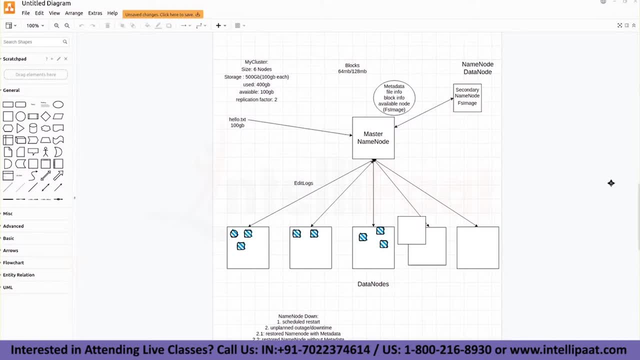 available? yes, it is available. if it is available, in which data nodes it is being written into? understood. so the input is there. information will consist of list of data nodes. list of data nodes holding voterscsv. agree, so it is available in hdfs, but in which data nodes it is available? 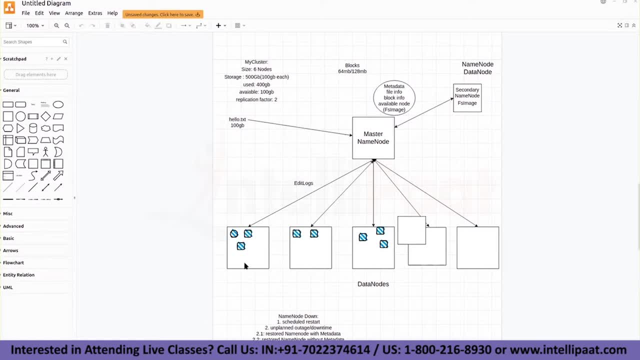 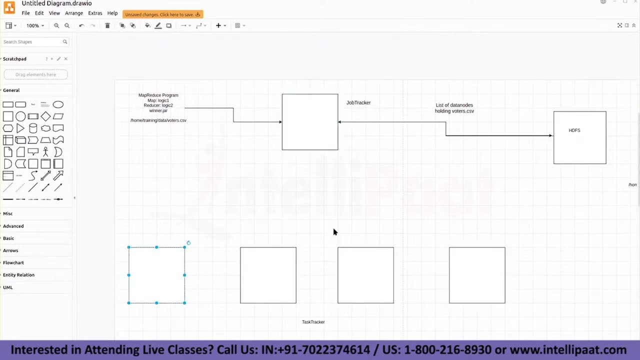 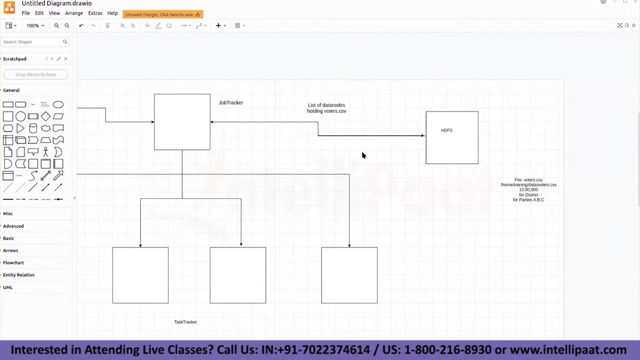 only then, if i, if i, if i know which data nodes, only then i'll go and run that query: right, job tracker and the task trackers agree, master and the slaves clear now. tracker and the task tracker. and on the other side, forget about these lines now. at least now you can forget about this. let's say, forget about all this content. 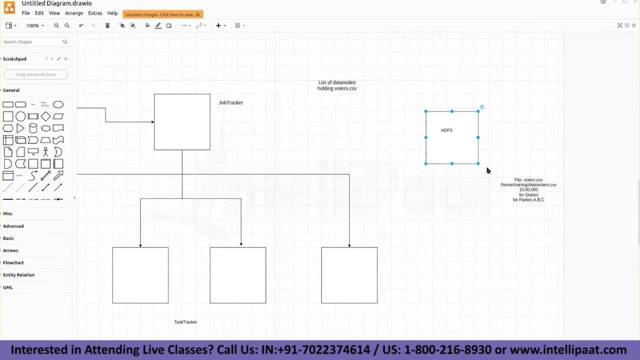 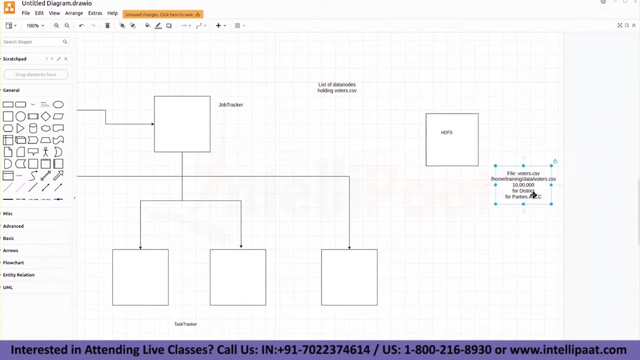 there is hdfs on the other side. okay, in hdfs, what did you do? you have, uh, written some data, okay, so what is the data that you have written? you have written the voters data, uh, which is voterscsv, so you have written voterscsv file. and when you write some data, you 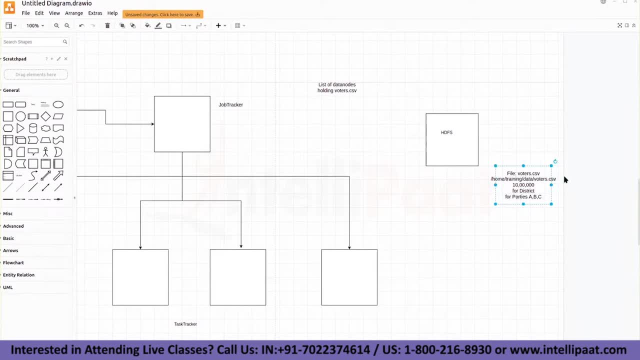 will have some location allocated to it. so home training data voterscsv is the location in hdfs where this voterscsv is written. so this voterscsv consists of some 10 lakh records for a so-and-so district, for parties a, b and c. so a, b and c votes have been pulled and 10 000 uh. 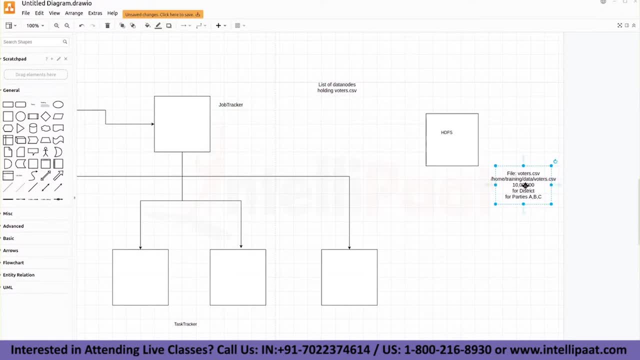 people have called this record, hold this votes, and the data is stored in the form of a csv file. now this csv in hdfs, i have divided it into four data nodes. i have to write it into data nodes, right? so i have broken that into four data nodes and and. 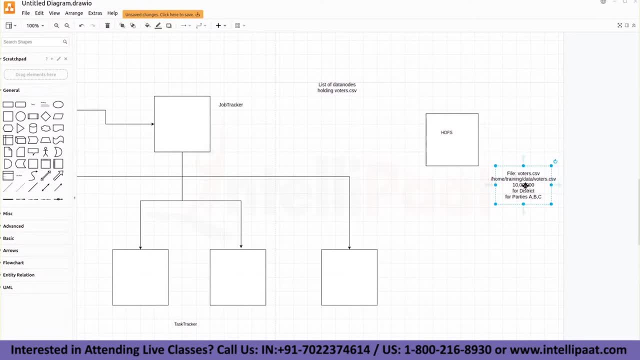 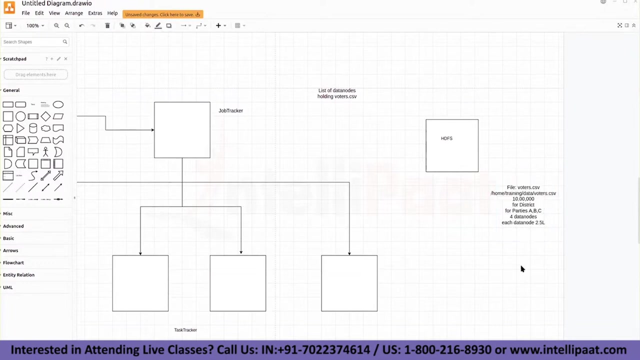 for our convenience, for simple use case, we are breaking it into four different data nodes equally, so each data node will have 2.5 lakhs of records. are we clear so far? four data nodes, each data node 2.5. okay, now the data is stored here. this is done and dusted now. 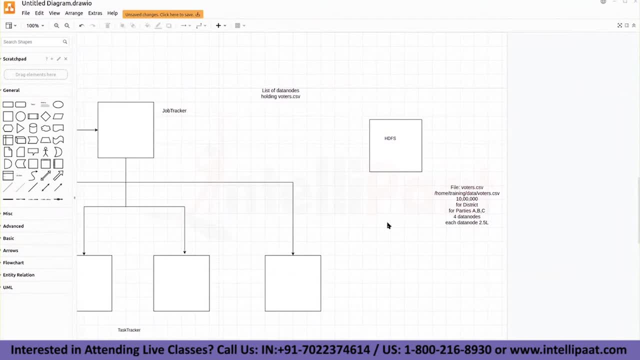 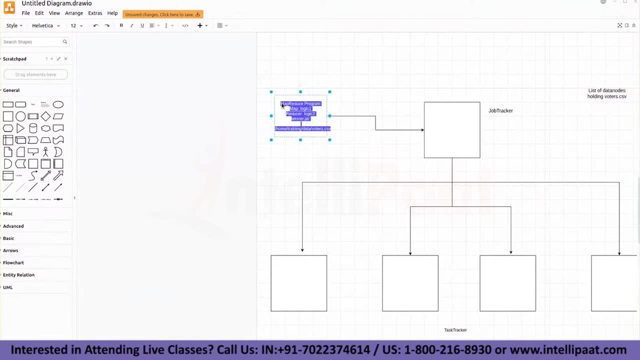 now we will have to run a program. so after you load the data, what you need to do? you need to write some program for it, agree. so you are writing a program. you are writing a map reduce program with two classes: one is map class and a reduced class in it. so that's the reason we call it as 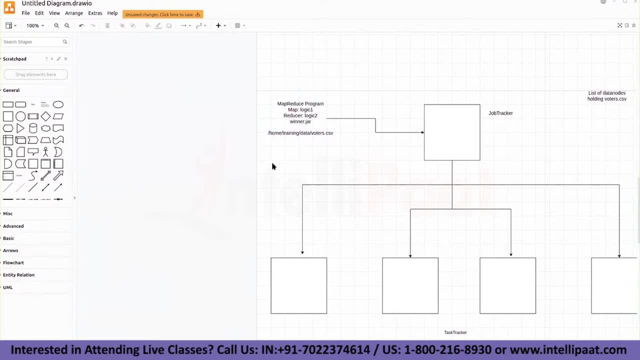 a map, reduce programs, which is, which is having a mapper class and a reducer class. so what do you write inside the mapper? and reducer. let's not worry about it now. okay, i'll tell you what. what we need to write, how, the, how we can define the logic. 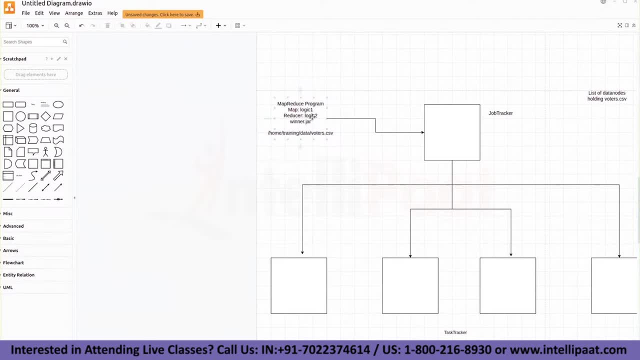 so i have written a mapper logic- this is logic one, reducer logic, logic two- and i have converted this into a jar file, that is winnerjar file. along with that jar file i'm sending the location of the data in hdfs right. so this details, i'm submitting it into the job. map reduce engine. so map reduce. 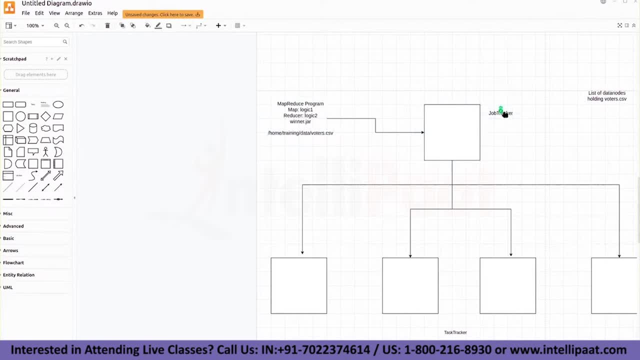 engine as in, you are submitting it into the job tracker only ultimately right. so job tracker itself is going to be the master right for us. so you're submitting it into the job tracker. so after your job tracker receives the jar file as well as the voters, dot csv location. 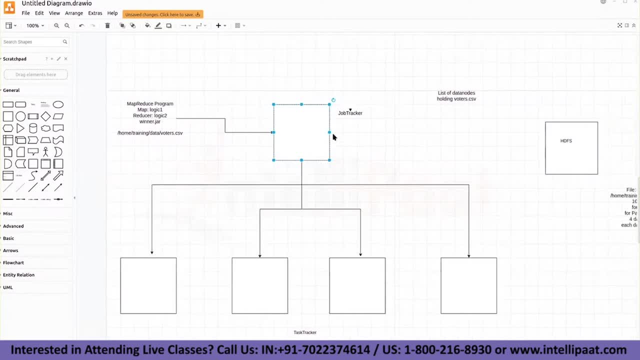 what it has to do initially is it has to validate whether the specified location is available in hdfs or not. okay, whether this specified location is available in hdfs or not. so my job tracker is: what is it doing? it is interacting with the hdfs, that means, with the name node, to validate whether. 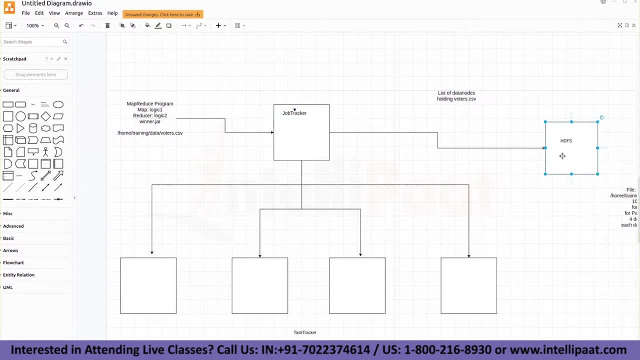 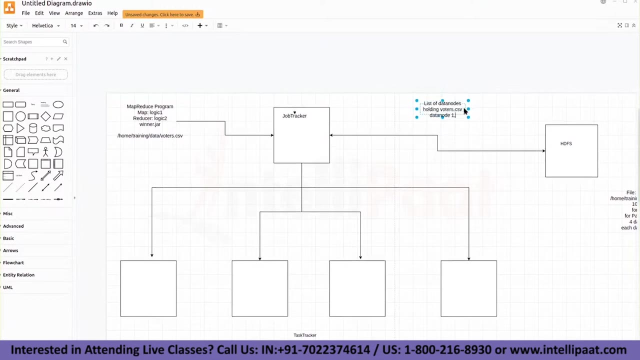 or not. if it is available, in which data nodes it is available. so what is it going to get in return? it is going to get- is going to get, the list of data nodes which are holding the voterscsv file. agree, data node one, two, three and four are having this data of voterscsv file. this information has. 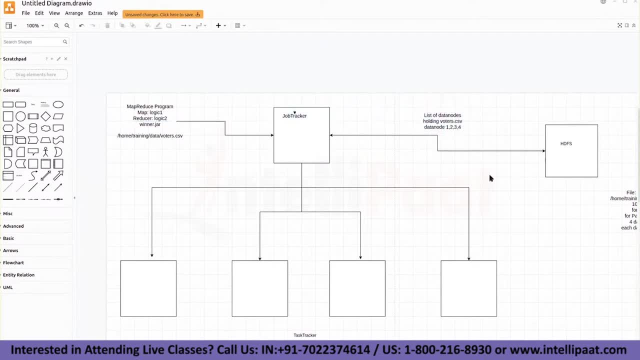 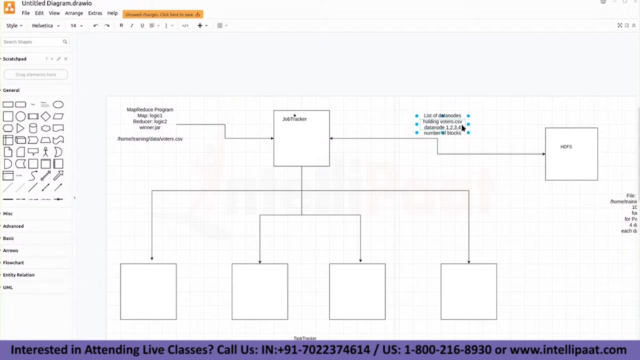 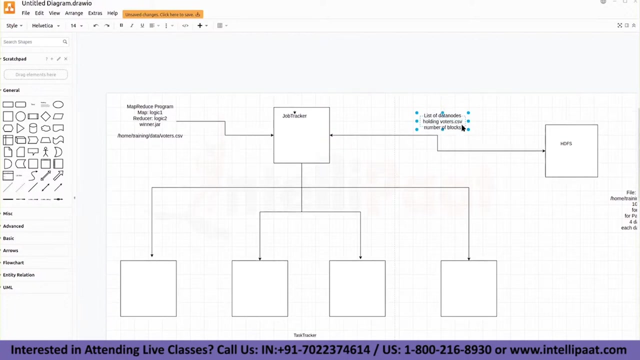 been shared with the job tracker. agree, any questions? so, depending on the number of data nodes or, if i can get into the details, number of blocks, so forget about number of data nodes at least. so how many blocks this particular data node, this particular data has been written. 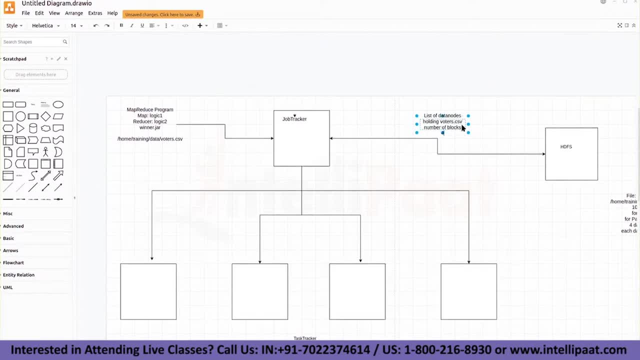 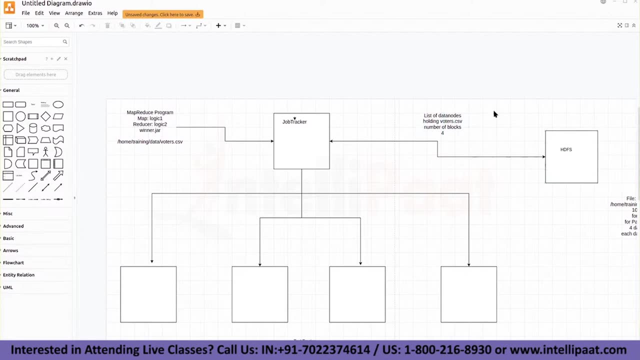 let's say i'm writing it into four different blocks. right, that is what we discussed. so i have written the data in hdfs into four different blocks. four blocks of data is available, so, depending on the number of blocks of data in in hdfs, your job tracker will split so many map. 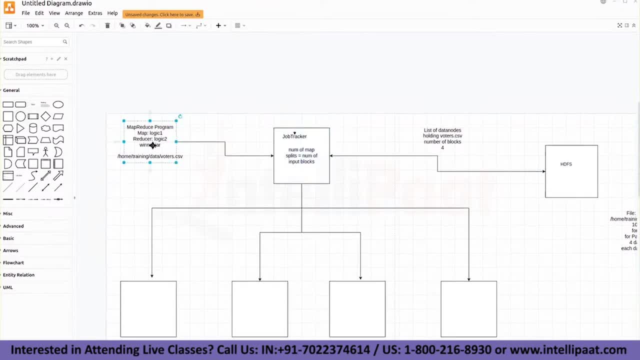 tasks. so this entire winnerjar is a job. right, i'm submitting a job under this job. there is a task called as map, there is a task called as a reduce. so these two are the individual tasks. so i have written the data in hdfs into four different blocks. four blocks of data is available. 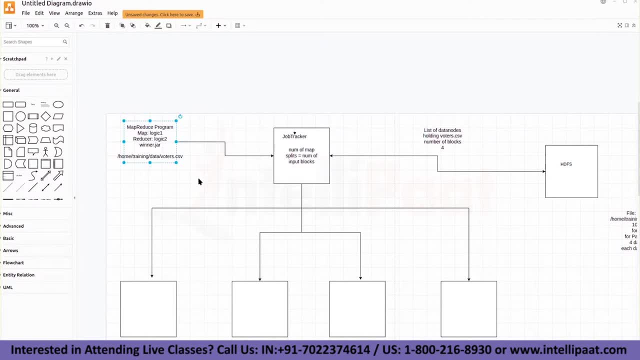 okay, map task and a reduced task together called as a winnerjar. so whatever the program that you have written in logic one, whatever the program you have written in mapper, that is being split into the number of input blocks. so how many input blocks are available? four input blocks are there. 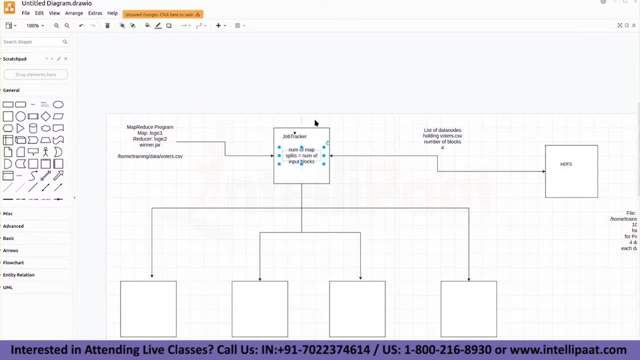 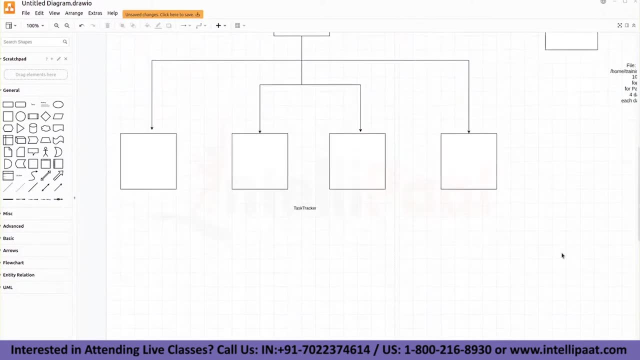 so how many map splits will be divided? four map splits will be divided. that means in simple terms: let's say so, i have written a program. let's assume this is what i've written in the mapper. okay, it's a simple use case. what is it going to write? it is: 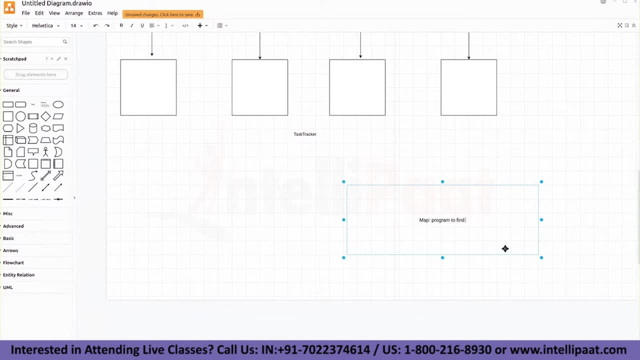 having a program to find votes for each party. this is what i've written in the program. given an input, with whatever the input you have, whatever the input you're running in, it just identifies how many votes are for party a, how many votes are for party b, how many votes are for party c. 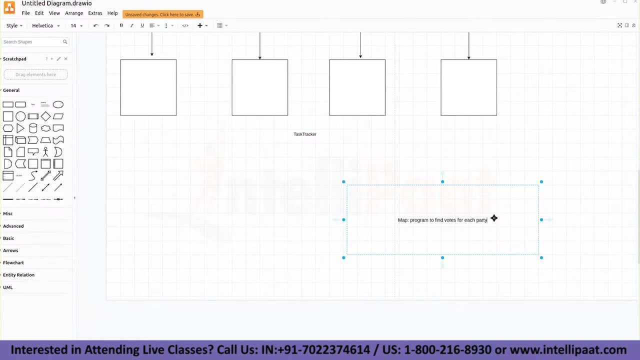 this is what i've written in mapper. this is the logic i've written in mapper. okay, so you have to run this logic and it you will generate. you will, you will generate an output saying: uh, map a, party a has received so many, party b has received so many votes and party c has. 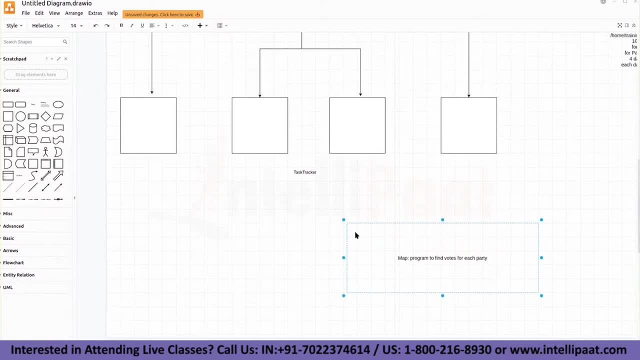 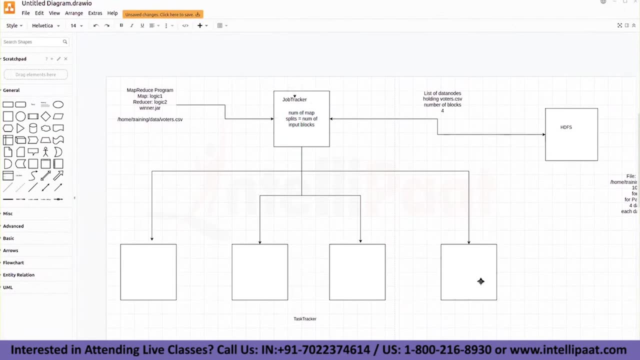 received so many votes. so this is the program that i have written. so now this program: i'm dividing it into four splits. four splits, as in, i'm duplicating it into four splits. so the same program you will duplicate into four splits. why, sports, four splits? because i have four blocks written in hdfs. so for 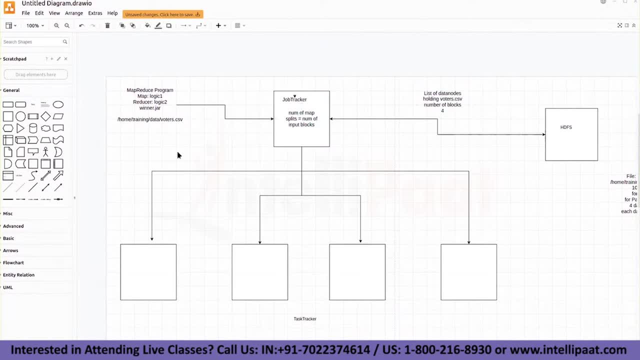 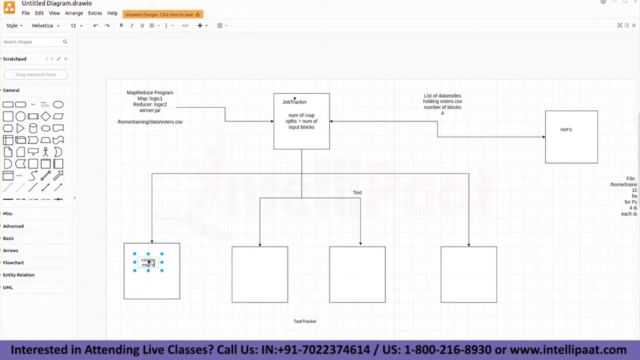 each block of data, your map split will go and run on top of it. so number of blocks: depending on the number of blocks, your number of map splits will be defined so that each map split will be assigned to each block of data. so here this task tracker, this task tracker running map split one on. 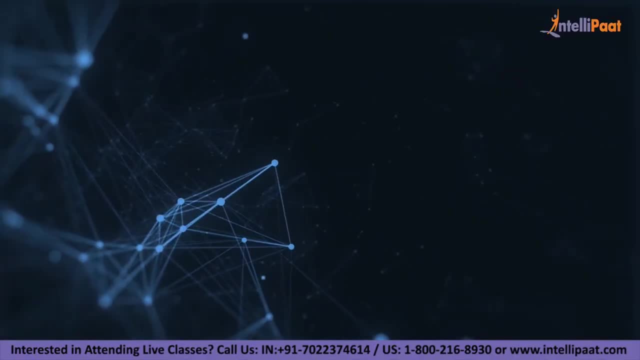 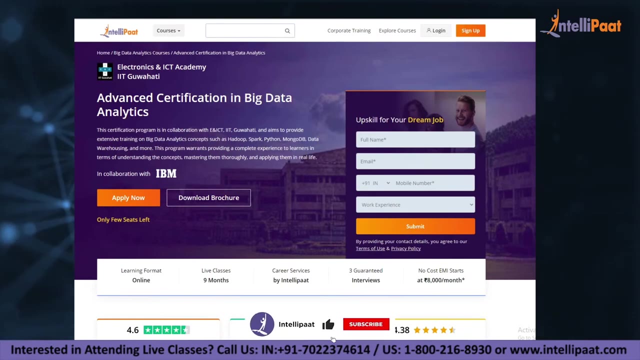 input. just a quick info, guys. if you want to make a career in big data, then intellipaat provides an advanced certification in big data analytics by enict council iit guwahati. it is taught by iit professors and industry experts with more than 10 years of experience. this course is designed. 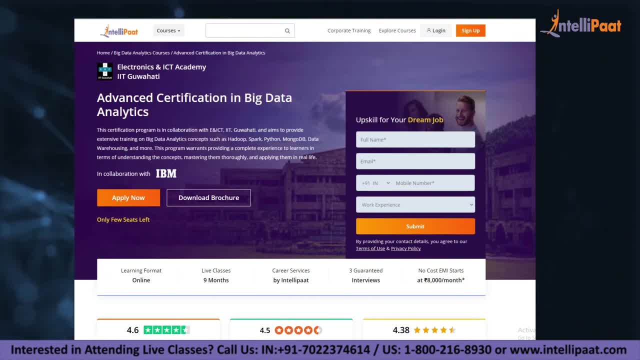 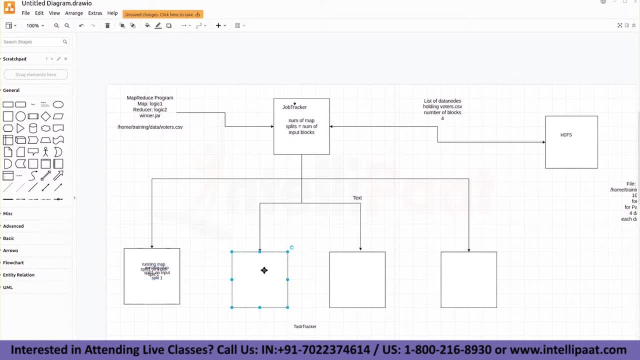 to upskill and land your dream job. now let's continue with the session. and the same one, same other task tracker is running here, which is of it's running map split 2 on input, split 2.. so what are they supposed to do? they have to execute some tasks. task trackers are meant to execute some task. so out of the given job, your. 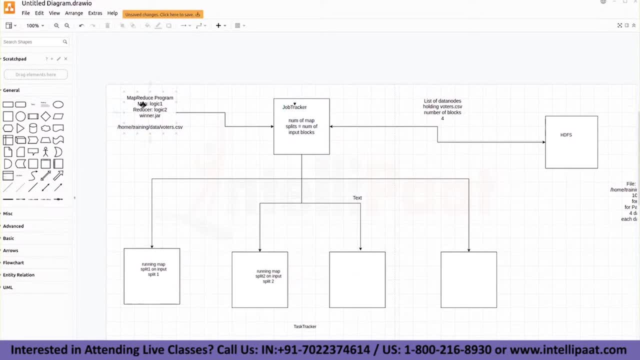 job tracker has divided mapper into four duplicates, four duplicate code and each. each piece of code has been submitted to each task tracker. so what they have to do, they have to go and run on top of the data block that they are available wherever the data is available, in whichever data node. 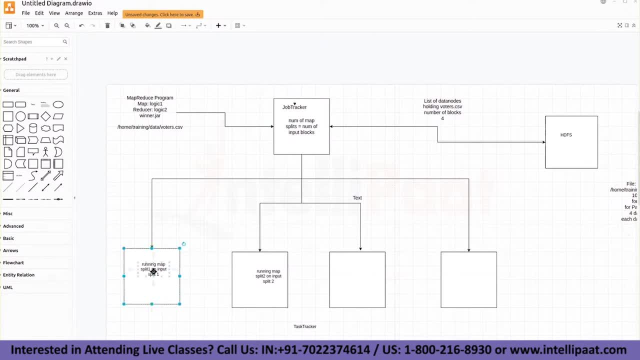 so this task tracker will run this map split, one piece of code, on top of the first block of data in htls. are we clear so far? this is a bit confusing, but but when we, when we get into the details we will, we'll have some better clarity. so, uh, number of map splits is what? 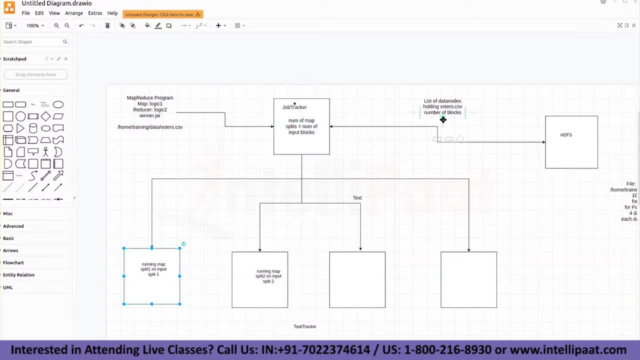 number of input blocks. so input blocks are four. so i divided my mappers logic into whatever the program i got. i duplicated the program into four copies. each copy i'm sending it to each and every task tracker. so each and every task tracker has to go and run on top of the data blocks where the 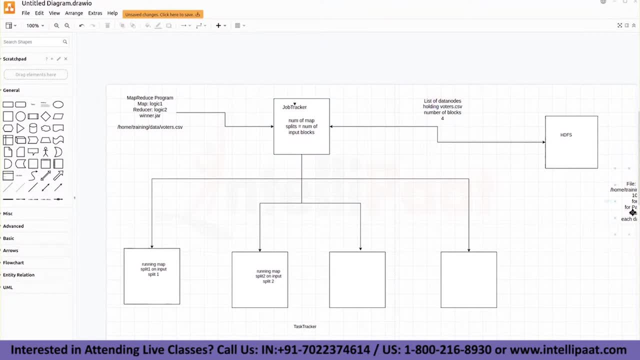 data, where the data is available, on on top of each data block. uh, i'll have to run this, execute this map, split one so what i might get the out. what am i going to get as an output? what is my task tracker? one output going to be. 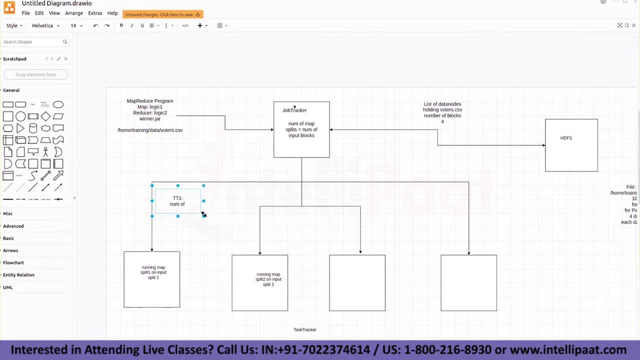 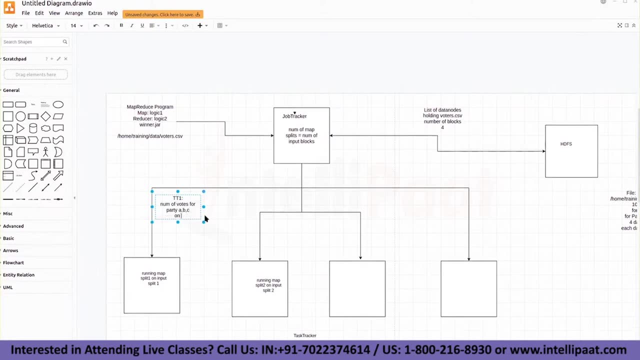 task tracker one output is number of votes per party- a, comma, b, comma, c- on how many records? by lakhs of records. so this is task tracker one. similarly, task tracker 2 output will be same on the other 2.5 set of records. agree, guys? are we clear? 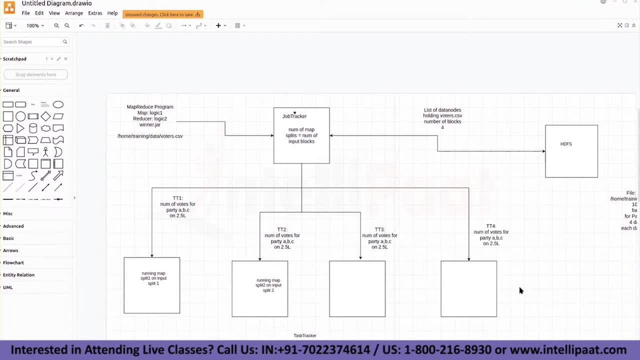 this is task tracker three. so are we um agreeing with the concept of moving computation to the data? so the data is available in hdfs? we are not moving the data anywhere. we are moving the code. whatever the code you have written in the form of a mapper. 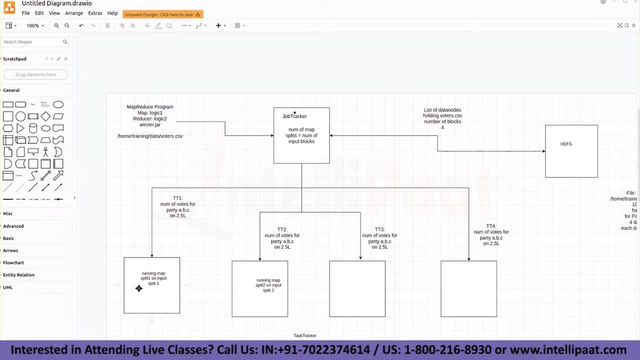 you are moving the code using the task tracker. you are running the code on top of the data wherever it is available. you are going to the data node, you are going to the specific block and you are running this task tracker and you are extracting the result. you are only getting. 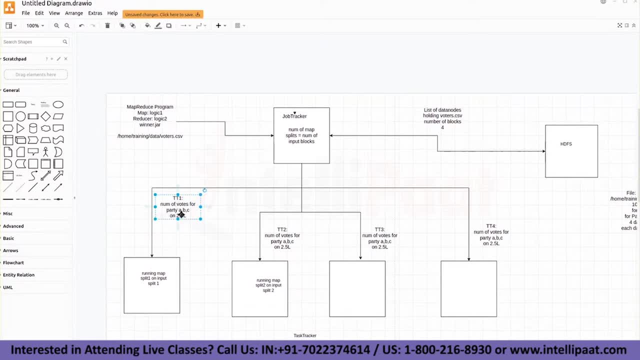 the result here. so now you have got the output from task tracker one, task tracker two, task tracker three and task tracker four. what is the output you got? you only got three records, that is, party a, how many votes, party b, how many votes, and party c, how many votes. that's it. so now you have to send this output of. 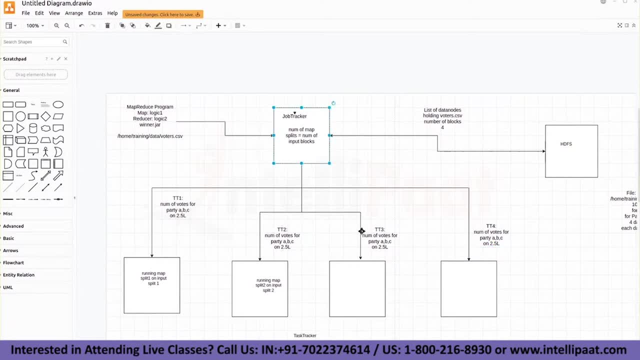 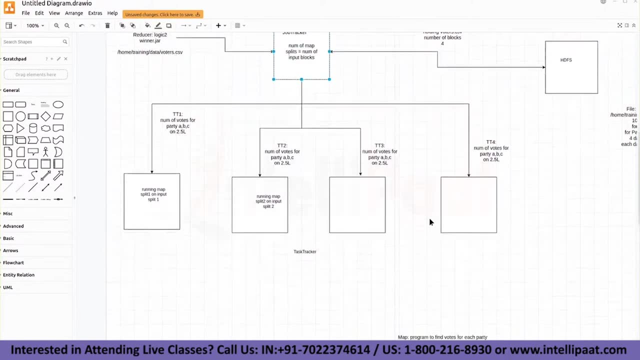 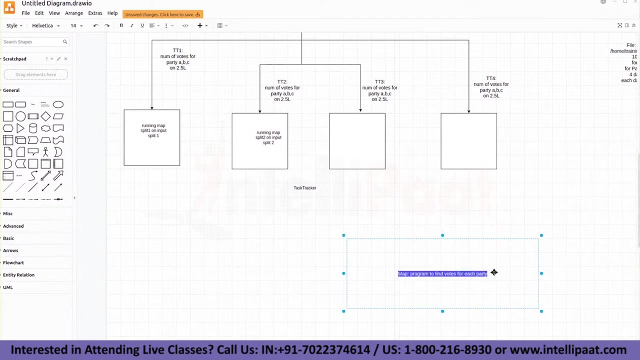 all these task trackers to your job tracker. your job tracker will accumulate the output from all the four task trackers. now what it has to do. so that is going to be written in the radio, right. so at the end of this material, the mapper is the individual activity that is happening. 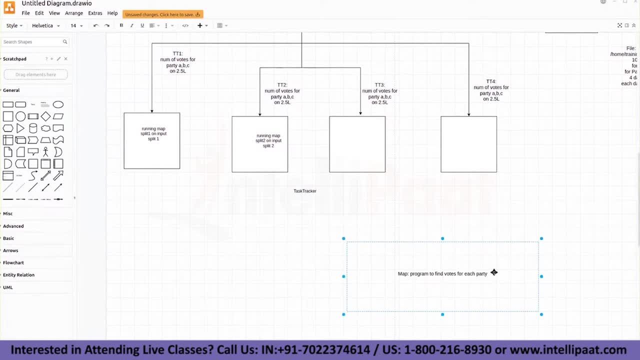 and red user is the summation. i mean the, the, the activity that is applied on top of the outputs of the mappers. so your red user logic will look like this: um, accumulate results for each party and find maximum right. so that's what i'm going to do. 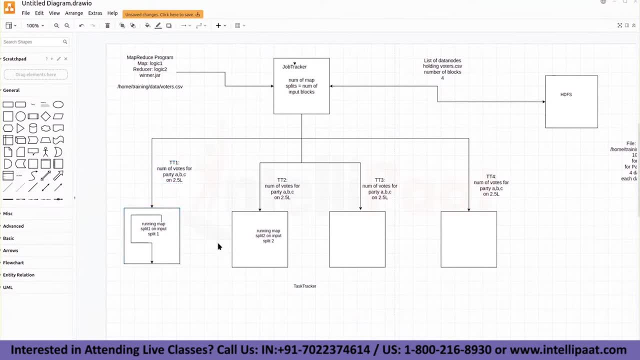 the results to. after you submit the results to all the uh from all the map task trackers to the job tracker, your job tracker will run the reducer logic on top of it. what it is going to do, it's going to add the votes for each and every value from each and every task and it's going to 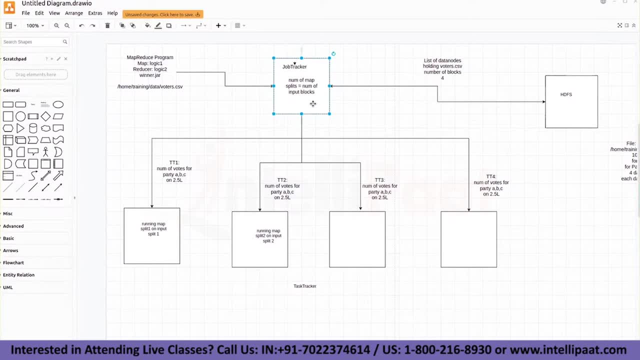 accumulate the data and it's going to find out the maximum, which, whether party a has received maximum, party b has received maximum or c has received maximum. so that is going to be the. that output will be sent to the client, so it only depends on what you write in the program. 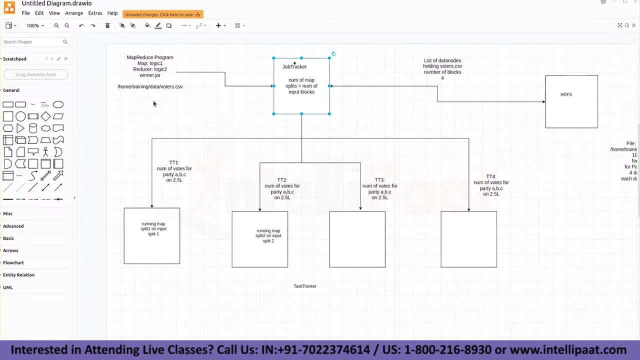 what you write for the mapper or what you write for the reducer. so, depending on the use case, depending on the requirement, you are defining the logic as okay. finding the votes is the mapper and accumulating the votes is a reducer. for a different use case, there can be a different logic. 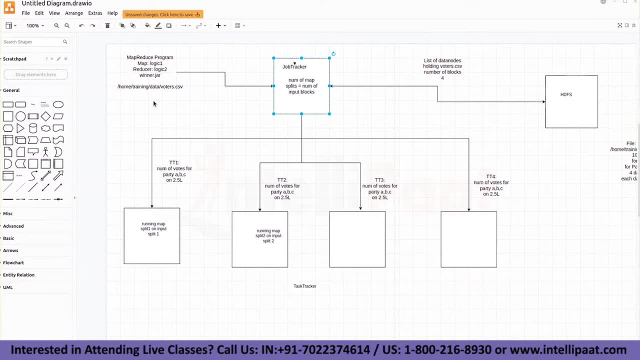 all together, okay, see, always mappers are going to get submitted to the task trackers and they're going to get executed first. so whatever the program you're writing for the mapper or what you're writing for the reducer, you right, you can, you can tweak and make the changes and um and execute it. but again, like 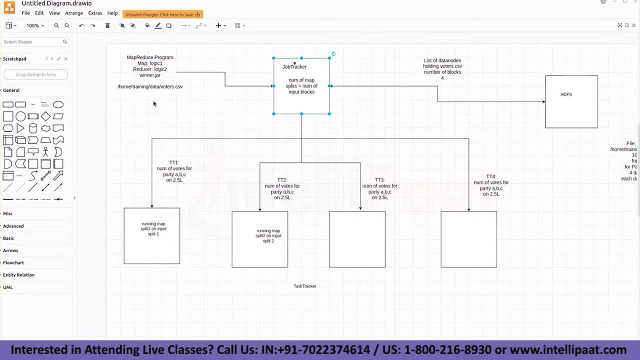 when you want to change it to red user and mapper, then the entire logic of operations will change right. one map class, one red user class. yes, there is only one map class and there is only one red user class. but, um, yeah, i can also come to that. you can have multiple map classes, depending on. 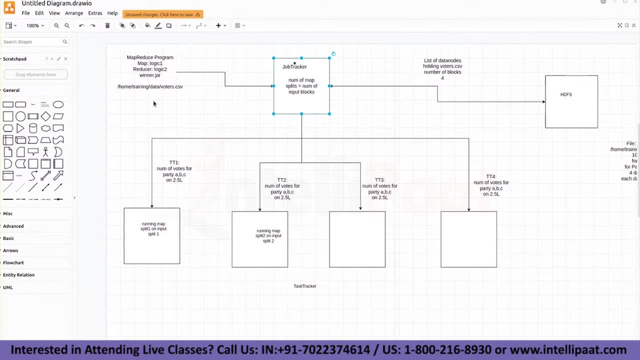 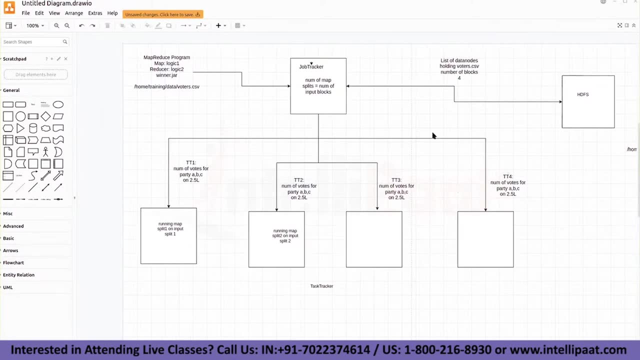 the scenario that again we have to discuss. yeah, i'll come to that, but let's not complicate it at this moment. are we clear? so we have been discussing about the map reduce architecture. map reduce has two demons, again internally: one is the job tracker, the other one is the task tracker. 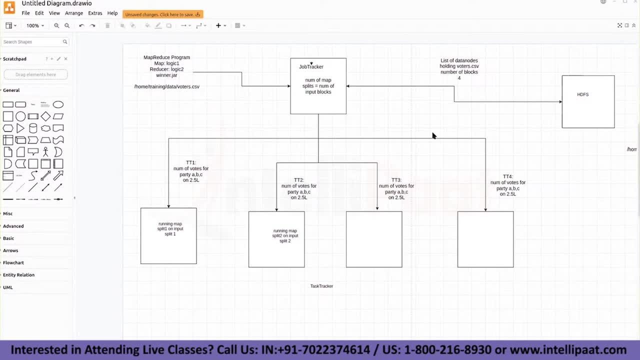 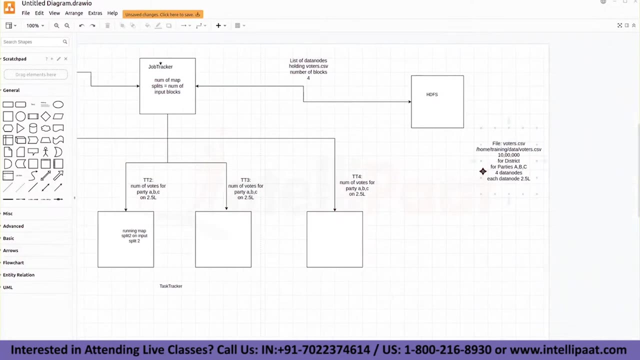 job tracker is considered to be the master and all the other task factors will be. uh will be the slave machines. so after you write the data into html- so we have considered an example of uh voterscsv file- you have written into htfs, you have sent a. 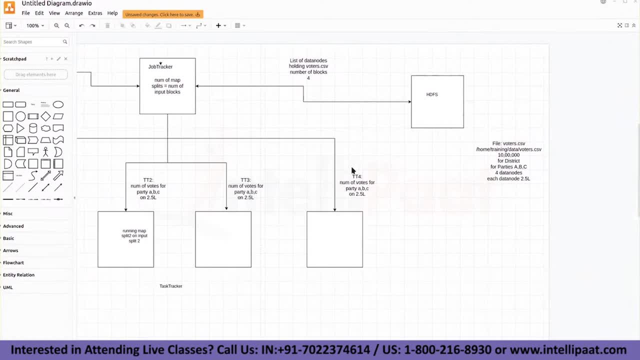 request with the name node that uh, and and the data node have stored the data and the data location is home training data- voterscsv. and we've divided this into four uh data blocks: uh, 10 lakhs. uh data is: uh, are you seeing my screen? 10 lakh records, each divided into 2.5 lakhs, and uh, we are dividing it into four different blocks. 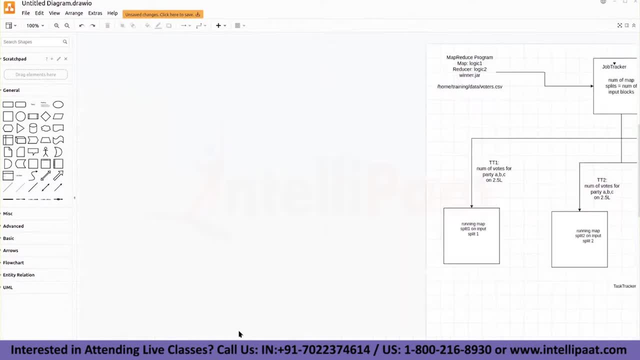 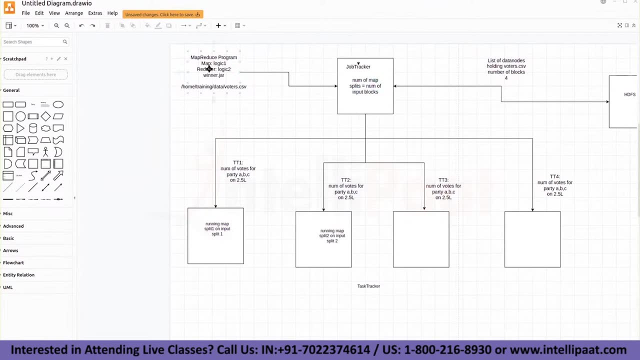 and after you submit a request, after you create a job, you have written a program and you've also given the input file location to the job tracker. this will analyze the map reduce program and it will interact with the hdfs name node to identify whether this voterscsv file is available in hdfs. 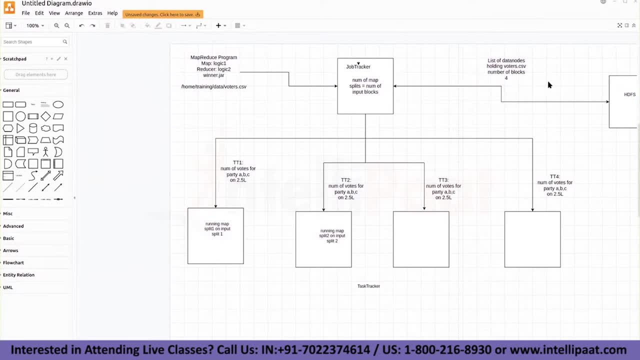 if it is available and how many blocks it is loaded into. after you retrieve the number of blocks, your job tracker will divide the number of map tasks into so many input blocks, okay, and then each map task will be allocated to the available task trackers. this task trackers will go and run. 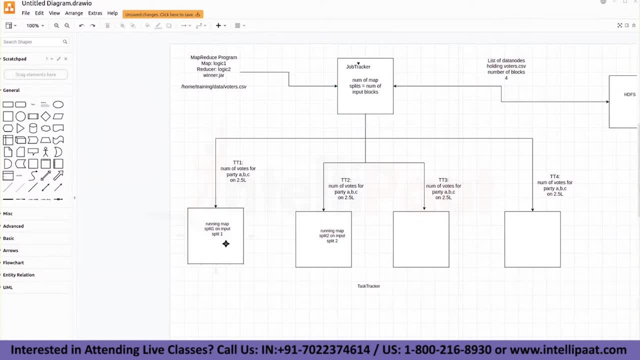 this job on the data blocks where the data is available. okay, so you retrieve the results from each and every task tracker and then you do a reduce task which will collect the output from all the map tasks and we'll we'll do an aggregation and find out the final winner of the lot. 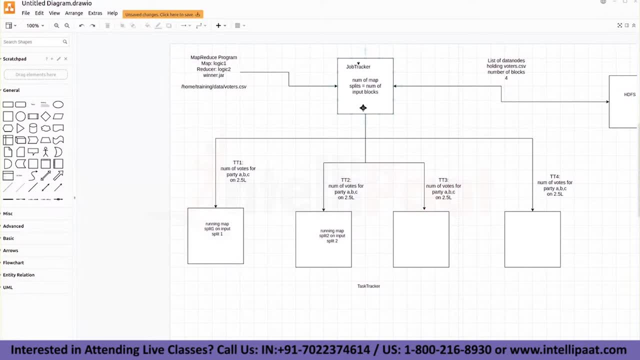 okay, this is the flow. then let's move on to the next one. we'll have to do a theoretical programming of how a MapReduce program can be written and how the execution flow is going to happen. okay, so for that we'll take an example of word count program. you must have heard about word. 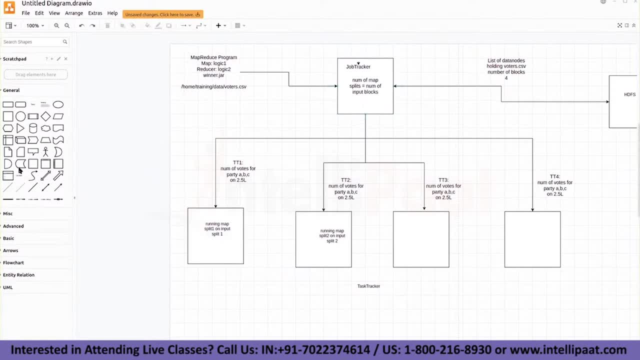 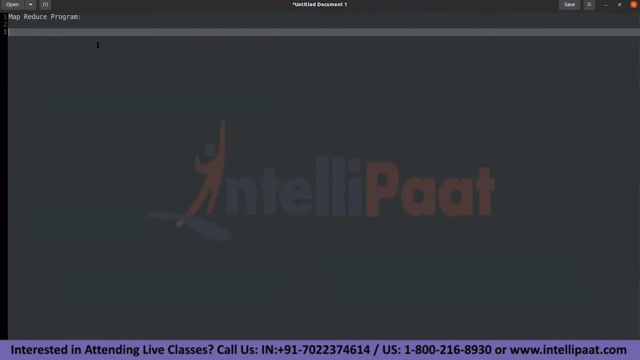 count right. okay, let me open a notepad. yes, are you seeing the notepad window right? so we'll have to consider an input. input will be hellotxt file. okay, so this hellotxt is having a data, something like this: okay, so this is the content of 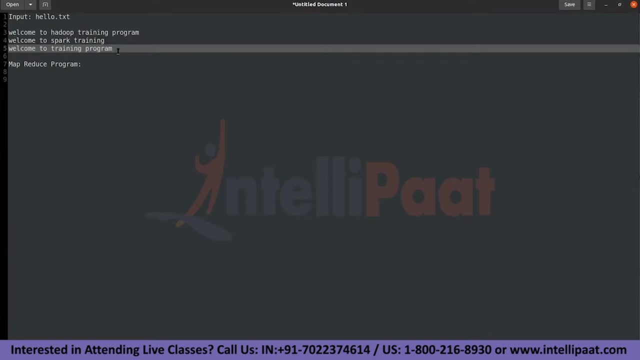 your hellotxt. some text content, okay. and what am i supposed to do? i'm supposed to find out the word count, that means how many times each and every word is being repeating. okay, so how many times welcome has been repeated? how many times hadoop has been repeated? this is my simple task. 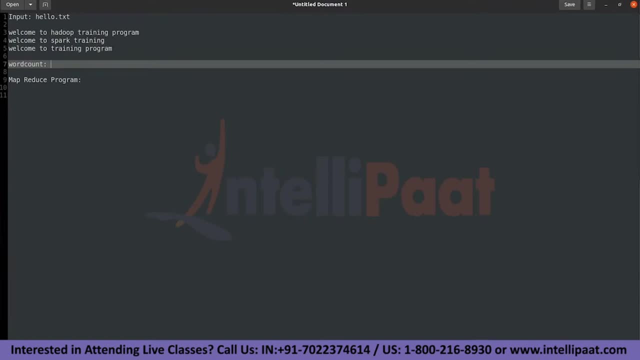 okay, so every MapReduce program, i mean everything, has to start with a word count program, only generally. so we we start with the word count program and try to understand, uh, the different features of it. okay, you understood the question. hellotxt is my file and, um, this is the data available in hellotxt. 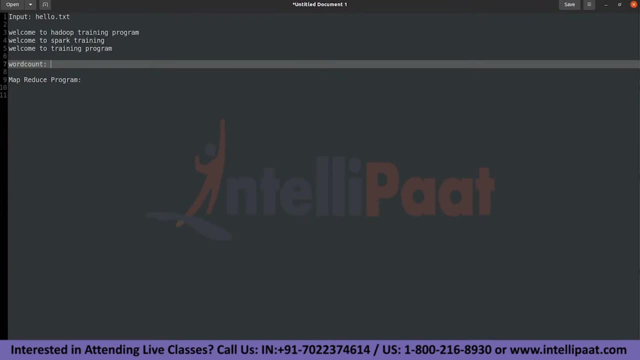 and you're supposed to find out how many times each and every word has been repeated. got it now. firstly, you're supposed to write a MapReduce program for this right. so one thing you need to understand is: if you want to write a MapReduce program, you need to write a MapReduce program for this. 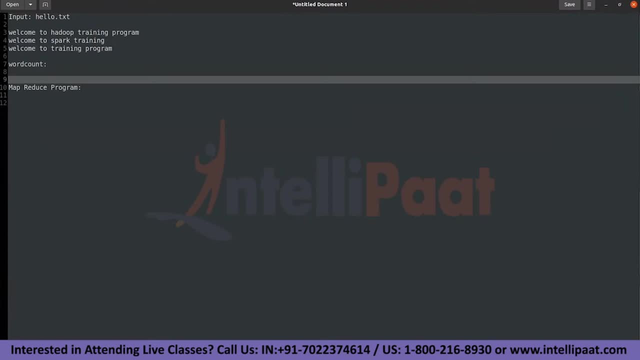 right. so one thing you need to understand is if you want to write a MapReduce program for this, every MapReduce program, for that matter, any, any MapReduce program that you write, or MapReduce engine will, will only understand the data in the format of a key and a value pair. 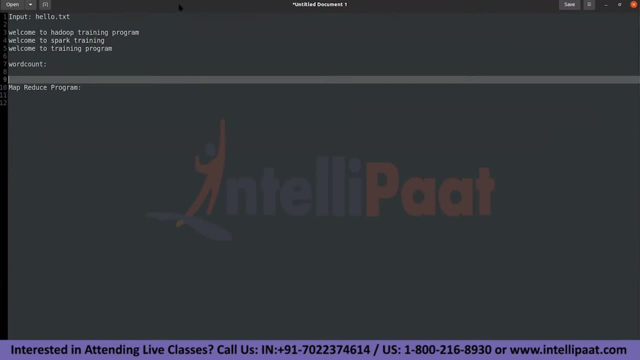 okay, just sorry guys, just just a minute. i have to take a risk like this. so this is a scenario: um, hellotxt is a file and we are supposed to find out the word count uh of the hellotxt file. so initially, so before, before we get into the MapReduce program, your uh MapReduce program mapper, as well as reduce, 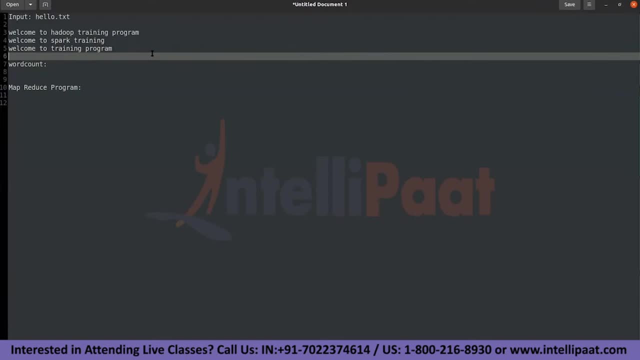 or whatever the phases you have. um it's, it's only going to understand the data that is in the format of a key and a value pair. so we have something called as a MapReduce engine, engine, as in, something which is which is facilitating or which is executing the MapReduce programs. okay, so 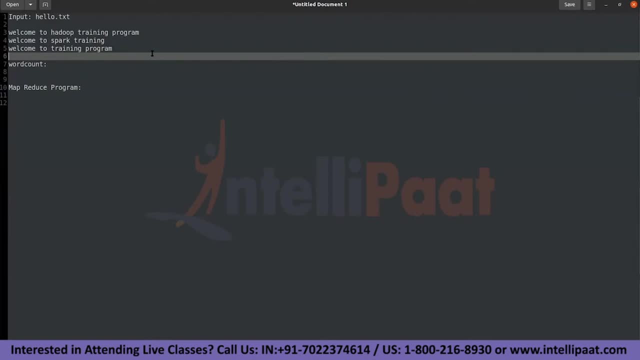 whatever, the core functionality of the map read is architecture that we've seen right. so that's the MapReduce engine that we've got about. so mapper reduce engine will will make sure your data is converted into the key and value pair before it is being submitted to the mapper reduce program, the mapper class, the reducer. 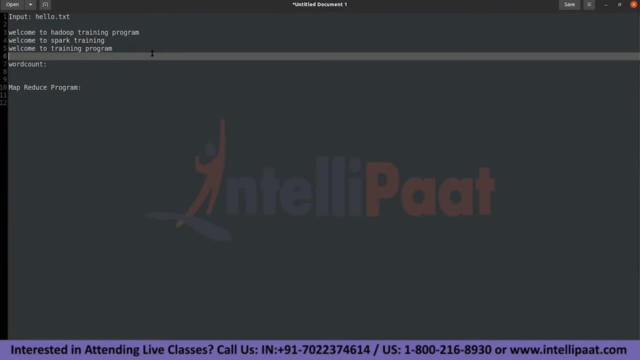 class or the main method, everything will will have the parameters in the format of a key and a value pair. okay, so that means your input has to be in the format of a key and a value pair for your mapper reduce program to read it and to evaluate it. okay, so what you need to do? you need to convert. 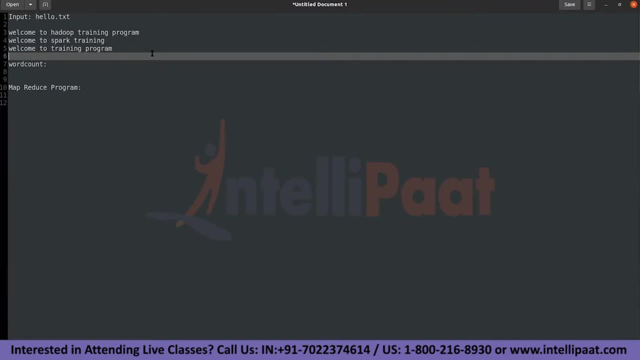 this data. even in the previous example, the voterscsv file we have taken right, so that also has to be converted. that is, that is everything being done internally. i mean, you're, you're not doing anything in this particular case. okay, you, you not define or you'll not write any. 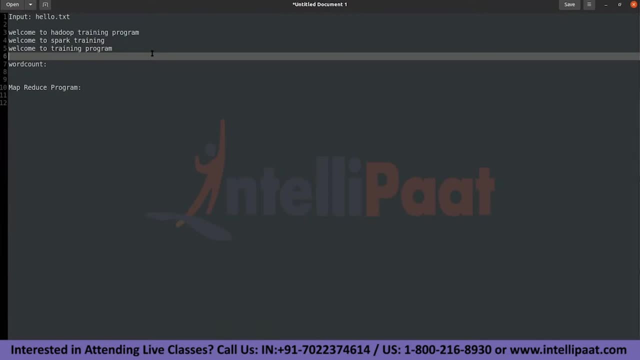 uh logic for the conversion also. so mapper reduce engine itself will convert the data and it will make sure the data in the format of a key and a value pair. so now this is your input file and i'm dividing this input file. i'm loading this input file in. 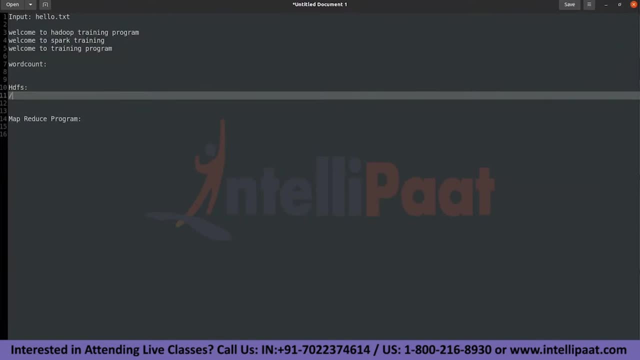 hdfs into this location, home. okay, so this is how the directory structures will be in hdfs: home, training data and hollow dot txt, and the data is divided into three blocks. okay, block one, block two, block three. let's assume this is my first block. simple line by line separation. okay, i'm breaking this into. 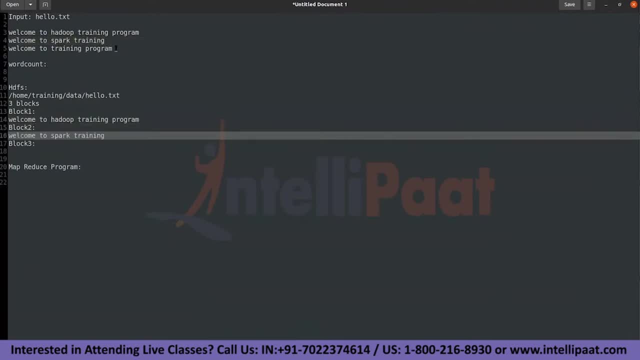 three blocks. it can be anything, i mean, it can break into different numbers of blocks also, but let's, let's, let's understand. this is being divided into three blocks and it is loaded in: hello dot, uh, home dot, training, uh, slash, data, slash location. so now, um, i have written a mapper: reduce program. 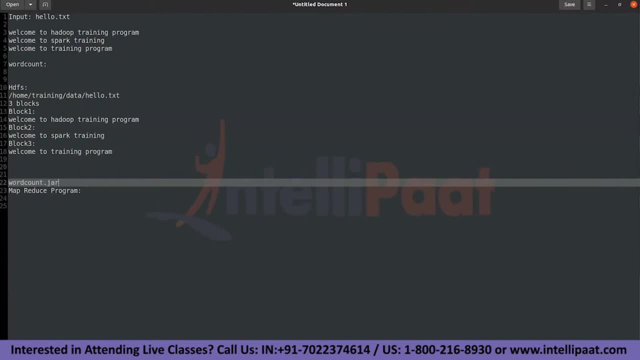 my mapper reduce program is word count dot jar. okay, work on dot jar is my mapper reduce program. along with it, you have given a file name called quote input. file name is input. file path is slash home. you have this path already right, so as and when you submit this, 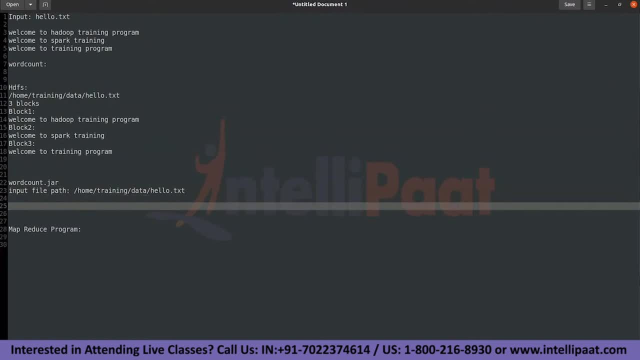 what, what, what is going to happen? your job tracker will will go to the will receive this request. word count request and the input file location. it will receive. and your job tracker will go to the uh uh. input file request. will receive this request. word count request. word count will receive and the input file location. it will receive: growth and your job tracker. 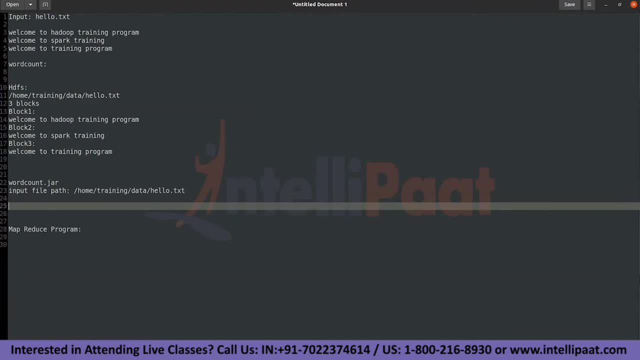 go and hit the name node to identify whether this hellotxt is available in so and so location. if this is available, how many blocks it is it is being divided into. that's what the information we get from the name node, right? so the reply will be yes, available, something like this acknowledgement: 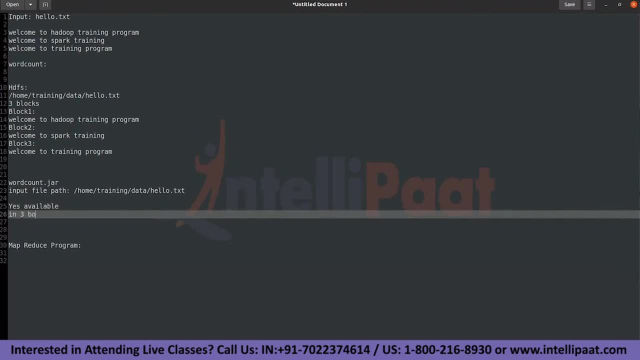 and in three blocks. so it's available in three blocks and you also have the data available with this, this particular location, this is the data block that is available. so now, after your data, the job tracker receives this information from the name node, so this has to make the data readily. 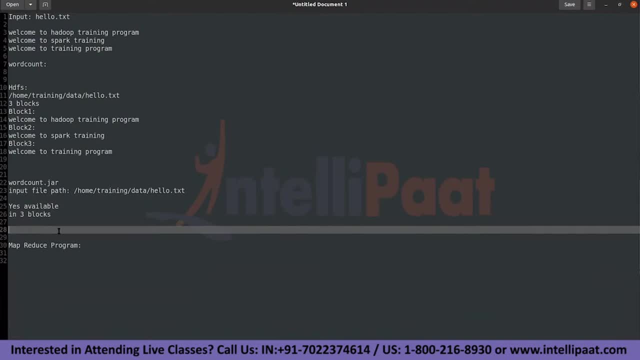 available, or this has to make the data. this has to convert the data in the format of a key and a value pair, right. so for your program to run, your data has to be in the format of a key and a value pair, right. so what it will do? it will take the block one. it will convert into a key and a value. 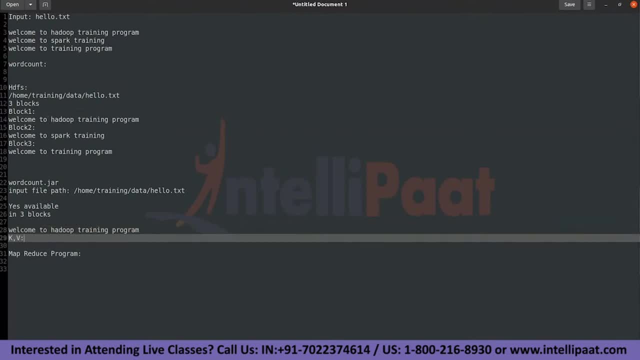 to a key comma value. so how is it going to convert? is the key comma value pair for this data block is the data comma t will be the offset. what do you mean by an offset? offset is some kind of an address location you can consider, okay, some address location of of this particular block, so wherever it is available, one zero, zero. 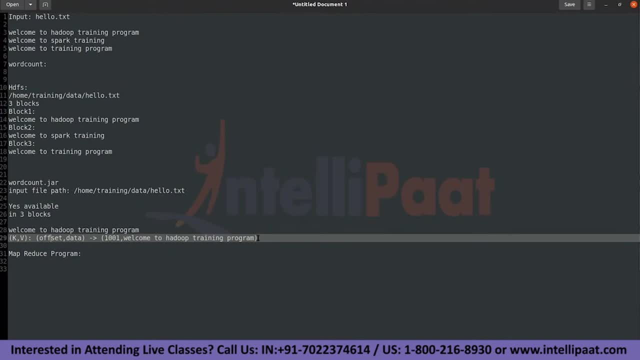 one or whatever some, some dummy address location. so this is my first key comma value pair. so key is by default being considered as an offset and value is the data. okay, the entire, whatever the data you have here in the block will be considered as a value, similarly for other um blocks, also your. 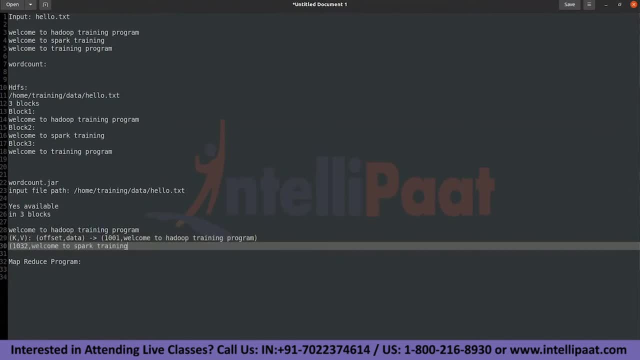 key comma value pair will look something like this: one zero, three, two comma, this one, and something like one zero, six zero, the address. so this is the three key comma value pairs available for you. this, this offset allocation, is, is dynamic. i mean, we are not, we are not being involved in this. 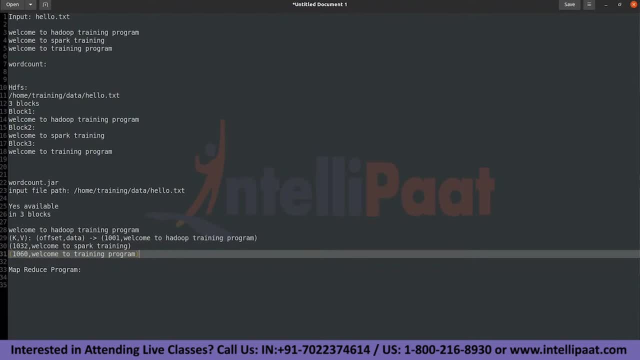 offset allocation. so your map reduce engine will convert the data into a key and a value pair, whereas key will be an offset. okay, so whichever offset it is available, maybe the location of the first character will be the offset and the location of the next line first character. 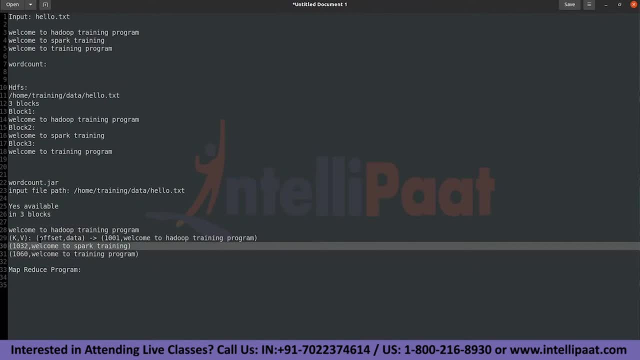 will be an offset, right? so you're not being allowed, or, yeah, we are not even being involved in the offset allocation here. okay, so it's just an offset and some uh address of that particular file location or for that particular block location will be considered as an key here. 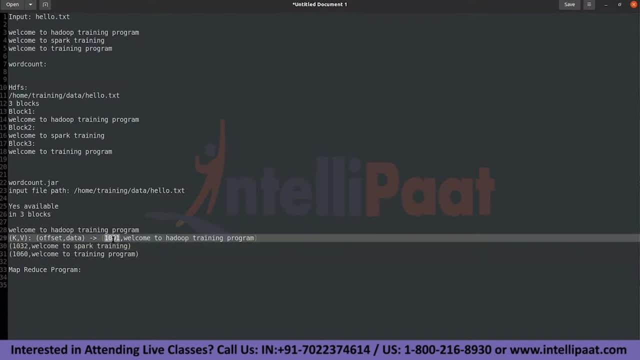 anything, anything. this one, zero, zero one is something which i gave just to, just to show that. okay, so it. it can be anything. it can it, can it. it is being allocated by the map reduce engine itself. we are not being involved anywhere here. we, as a developer, will not, will not even look. 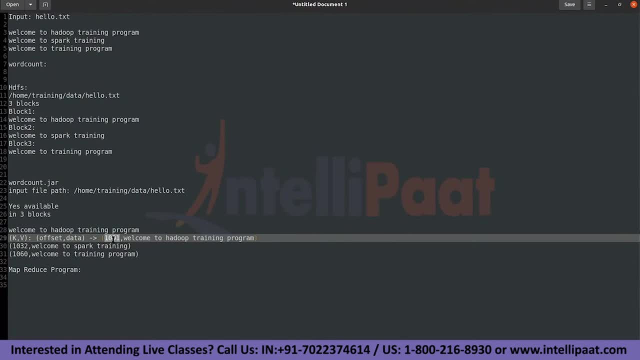 particular data. okay. what we only need to understand is it got converted into a key and a value pair. okay, and why is it supposed to be done like this? I mean, why are we actually creating this key, comma, value pair in this format? only so there is an input format available. see, when the data is in the format of a text. 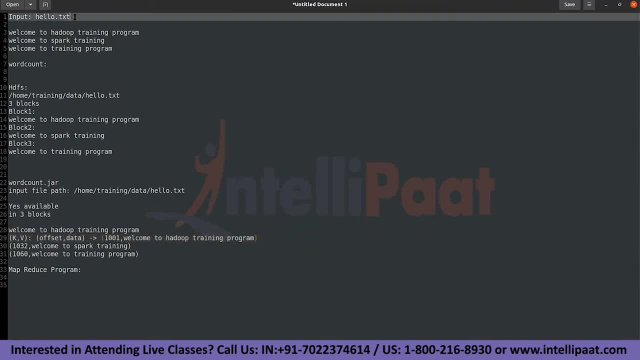 input format: text input format. as in whatever the input file that you have, or txt, or whatever the data you have- is in the form of a text input format, this is the conversion methodology. if the data format is in the format of some sequence input format or file input format or key value, text input format. 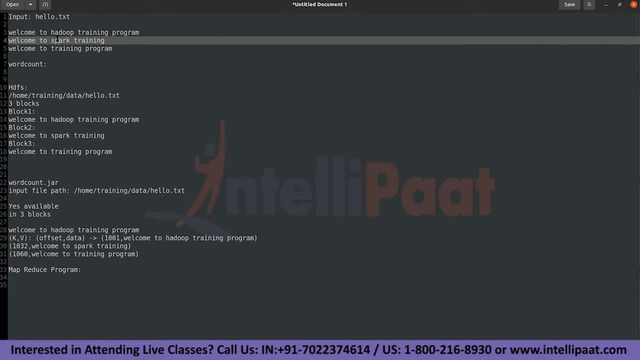 there are four different input formats available. once we get into the theoretical session we will see. one is a text input format, one is a sequence input format and one is the file text file input format, something like that. okay, there are four. so if the data is considered to, 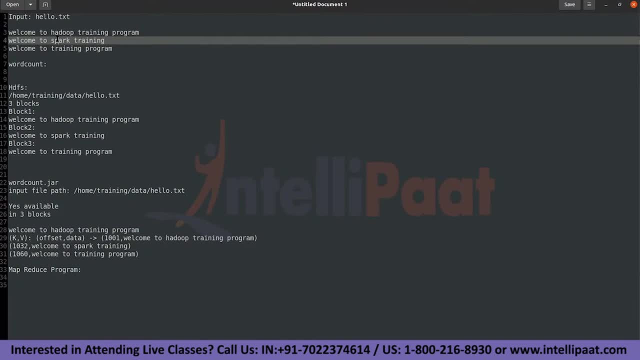 be in the format of a text input format. this is how the data key comma value pair conversion will happen. if the data is in the format of a sequence file input format, then there is a different format of conversion. okay, so most of our inputs that we deal with are going to be text input format only, generally, whether it 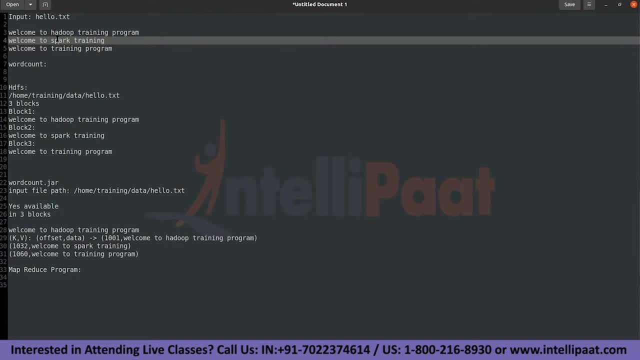 is in the CSV or whatever, the data will be in the format of a text only. okay, so your text input formats will have a default conversion methodology which is an offset will be a key and value will be the data. clear. Any questions in this Right? so, after we converted this data into a key comma value pair, what are we? 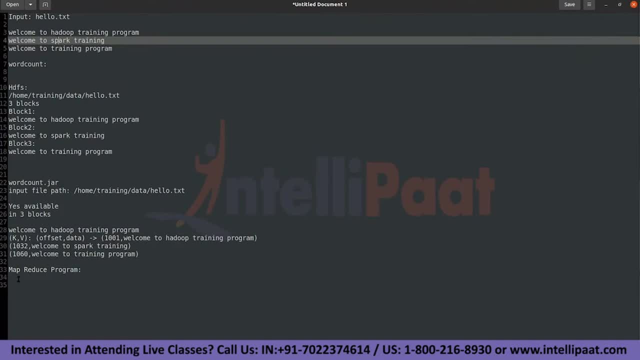 supposed to do. we were supposed to send it to the mapper first. so in mapper reduce program you have mapper class and Red user class. okay, so first mapper class will receive. okay, so before that there is also one more functionality in between. so you have three blocks of data. how many map splits have to be divided? 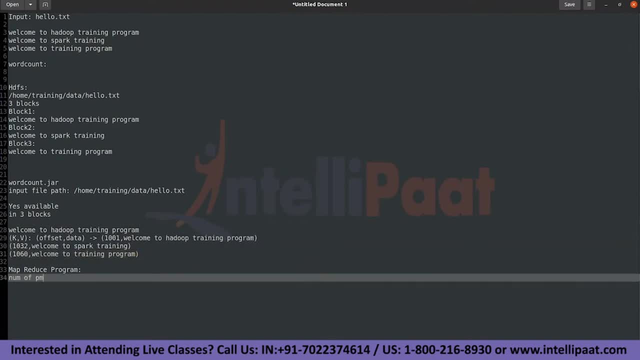 divided number of map splits equals to number of input blocks. ok, So your job tracker has divided 3 map splits. So this is your map split 1, what is it? Map split 1 will receive the input for this way. This is going to give you a. this is going to be the input for your 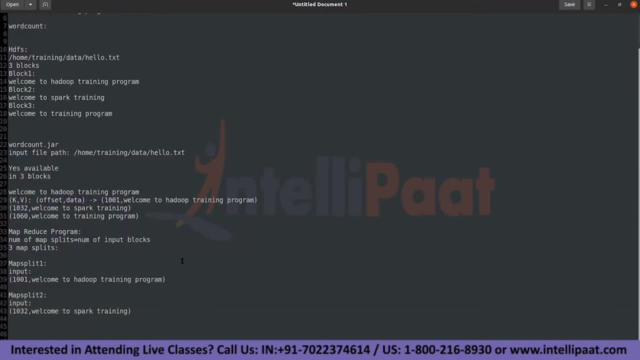 map split: 1. Agree, Agree, guys. So 3 blocks of data, you have 3 map splits you will be dividing. So your map reduce program will have 2 logics. One is map code, mapper code and reducer code. So your mapper code will be divided into 3 duplicates, 3 copies of 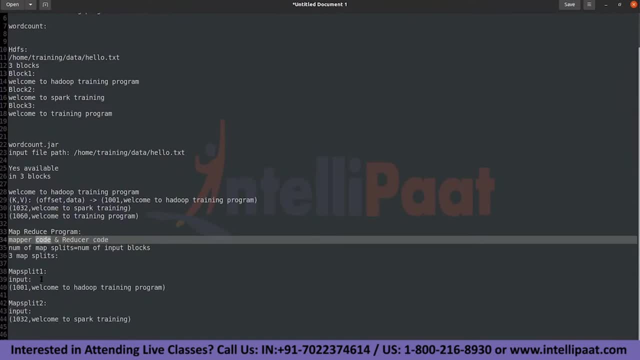 mapper code. So each mapper code will be divided into 3 duplicates. So each mapper code will be sent into this particular map split 1, map split 2 and map split 3 will get executed. Ok, So here you have mapper code execution running. So here you will be running a mapper. 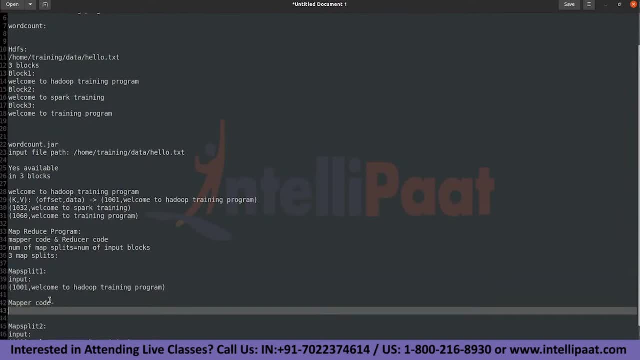 code. What do you run here? So your mapper class. whatever the program that you have written in the mapper class, that is what you are going to execute here. So mapper class will have 2 arguments: key and a value argument. So this input is in the format. 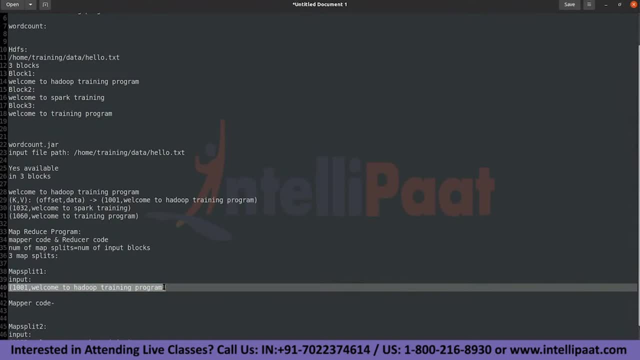 of a key and a value pair. arguments are matching and you have the data in the format of a key and a value pair and you will be reading the data. so now what I am gonna do in the mapper code: I'm reading only the value, I'm picking the value, which is this. I'm not 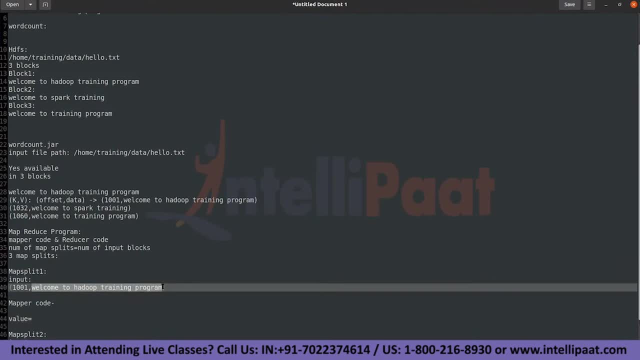 even worried about the key here, because that's just the dummy offset that it is being allocated. right, my actual data is available where in the value? only. right, I'm reading the data in the format of a value. I'm reading the value out of the key from a value pair. and what I have to do now? any any suggestions? what, what? 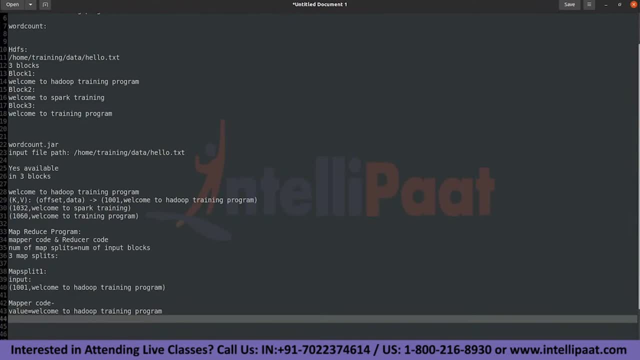 logic we are supposed to implement nothing related to MapReduce. so, in general, this is your string, right? I'm converting this into a string. I just have to find out the word count of it. how do you do it? so first operation is split by an empty space. what is it going to get? I mean what output you are gonna. 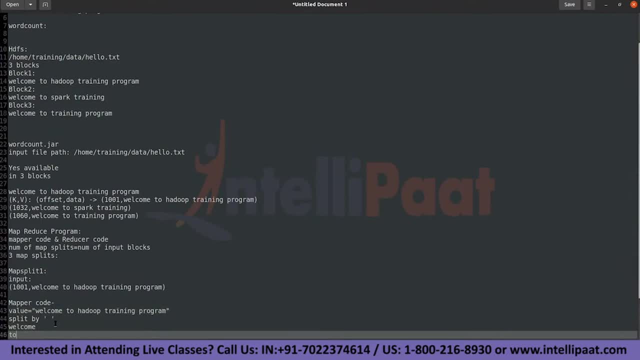 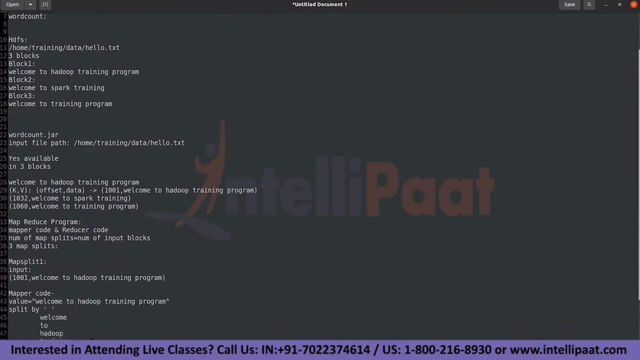 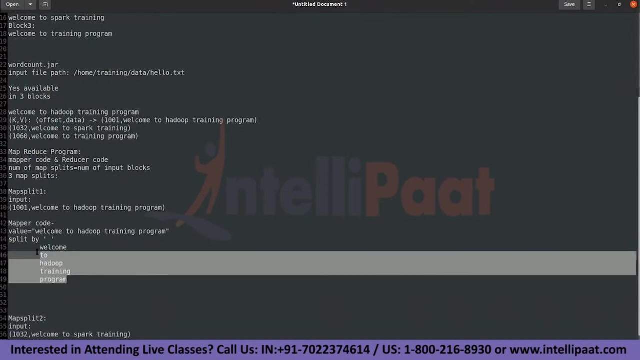 get welcome is one. your string is divided into these output pairs. this is output you got right. so after you do a split by space, this is output you got. what do you do next? I got this as an output and what do you say? what do you do to the mapper output? what? 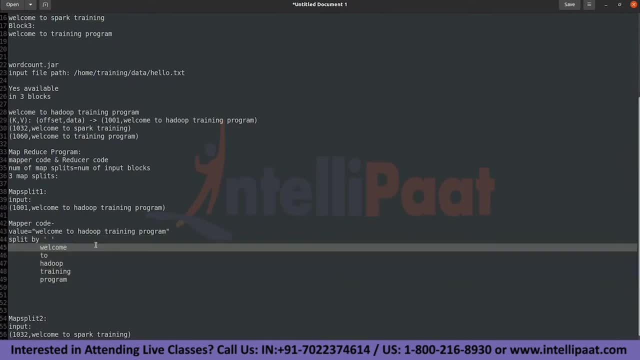 are you supposed to do with the mapper output? you are supposed to send it to the reducer, yes or no? but your reducer also will have the input parameters as a key and a value. I mean, it's only going to accept the data in the format of a key and a value. so your mapper output also. 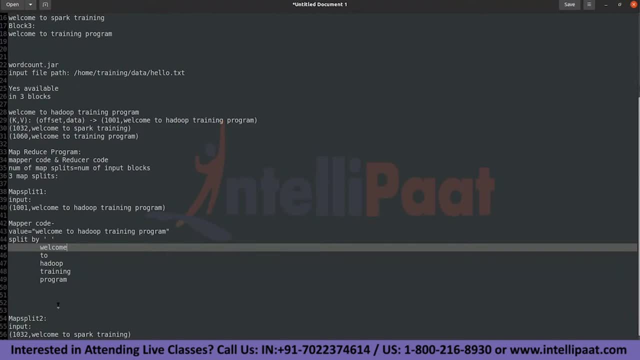 has to be converted into a key and a value pair. so what do you do to convert this mapper output to a key and a value pair? I'm doing this. I'm allocating one by default, saying that he is the data, one is the value. any harm doing it? so I 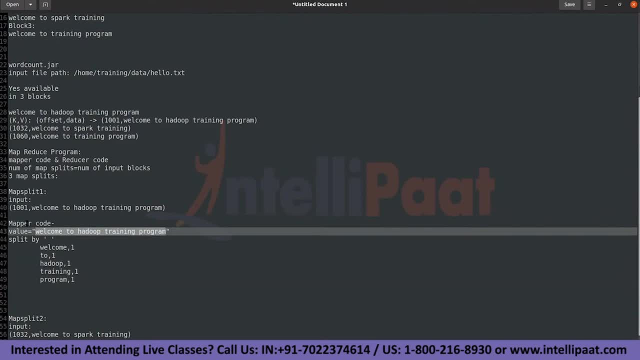 have taken the value out of the key comma value pair from the mapper arguments. i've done a split by function on the space after i receive the output in terms of individual values, individual string elements. here i'm allocating them, i'm considering them as a key and i'm 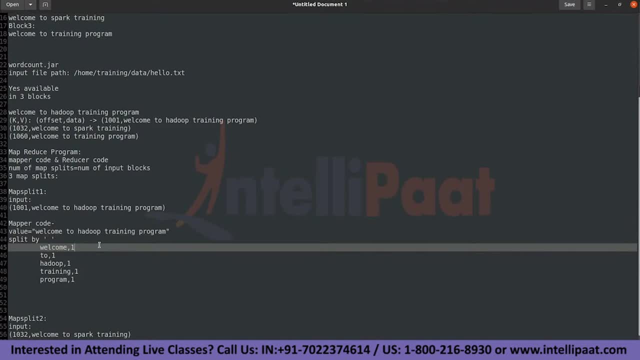 allocating one by default as a value. why are you allocating one by default- is like that's my own logic. i've written: okay, this is, this is all being written inside the mapper program. why only one? why can't i allocate something like dummy a, b or c or something like that? you can also allocate whatever. 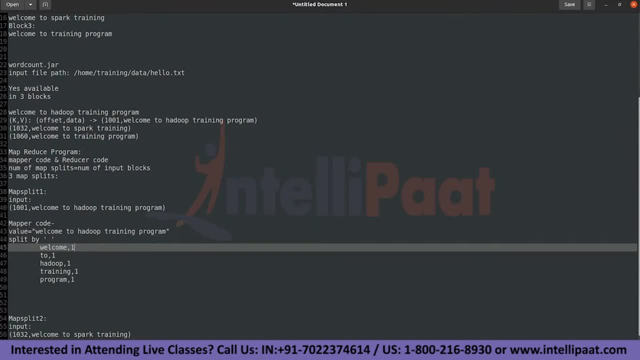 you wanted. okay, the reason why i'm allocating one is i'm telling that this is the. this is one occurrence of welcome. this is one occurrence of two. this is one occurrence of hadoop training and program. so for each and every occurrence of a value, of a string, i'm allocating some number to it. 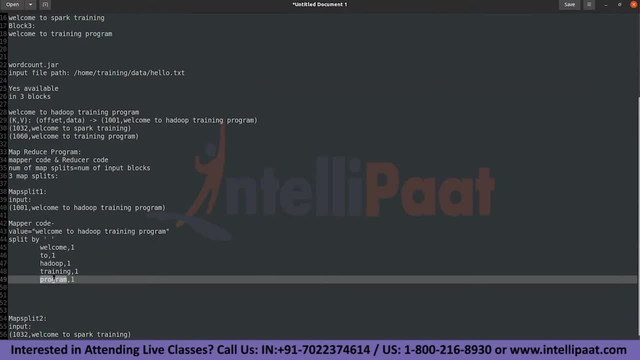 that means this is one occurrence of this particular value. ultimately, what is my goal? i have to find out how many times this value has occurred, right, so how many times this has occurred here- it has occurred once- and how many times training has come. this has come once. how many times? how? 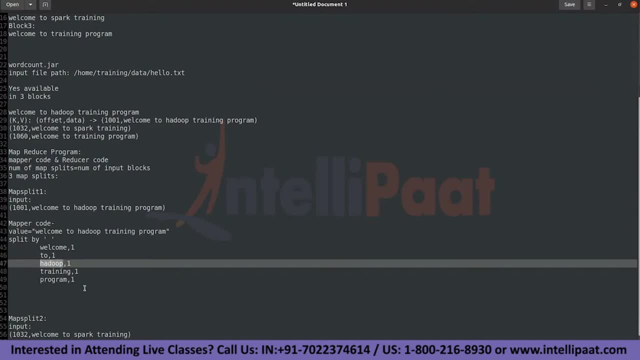 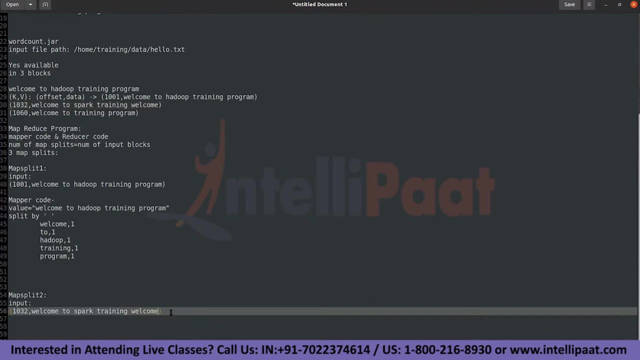 do? i have come, this has come once. something like this: three. now let's see what is it going to happen. so here we have, welcome. so what is my mapper code supposed to do? it is going to do a split first. it's going to pick value. right, pick value from the key comma value pair and apply. 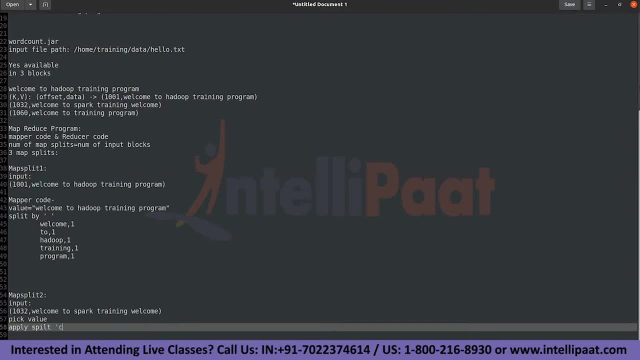 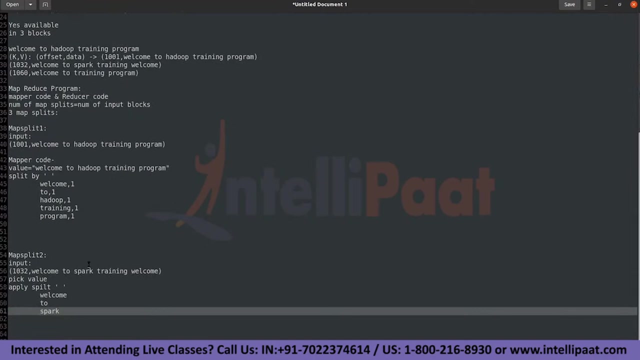 split on space, yes, and what is my output going to be in general? what is my output? welcome, and then the third line will be spark. so this is how your split output will be, if you're not aware of it. so after you do a split, it's going to break it into space. now, what am i supposed to do? 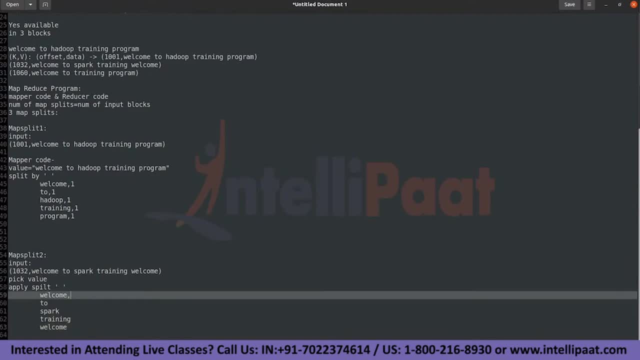 i'm supposed to allocate one by default, just to make it look like a key comma value pair. what is it going to come now? no see, this is an. this is an individual mapper output, map split, one output. which is this? okay, by default. by default, i'm allocating what i'm. 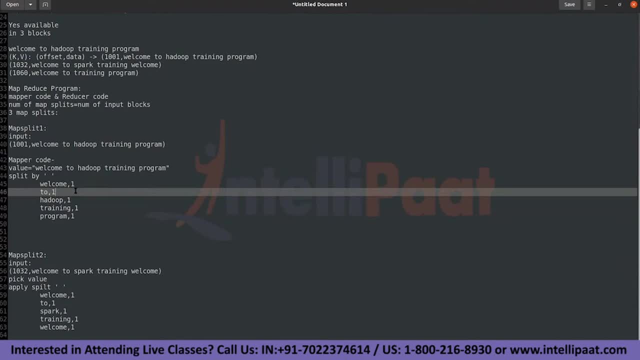 allocating one as by default value, regardless of whatever key you get. okay, the only reason why i'm allocating one in this particular scenario- at least let's assume for now- the only reason why i'm allocating one is just to make it look like a key comma value pair. 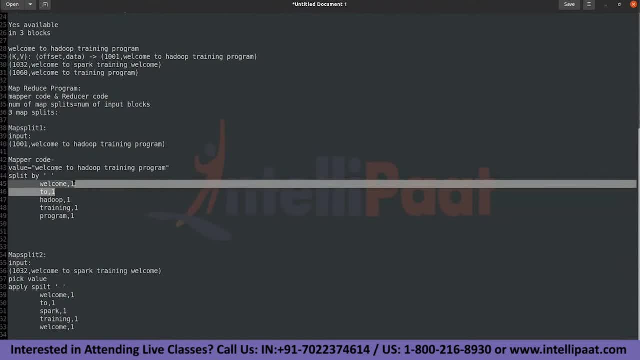 and why i'm allocating only one is to to to tell that this is the occurrence of one. one occurrence of welcome, one occurrence of two. okay, so here also, this is one occurrence of welcome, this is one occurrence of two, and even though i got another welcome, i still am allocating one. i didn't write any additional code for. 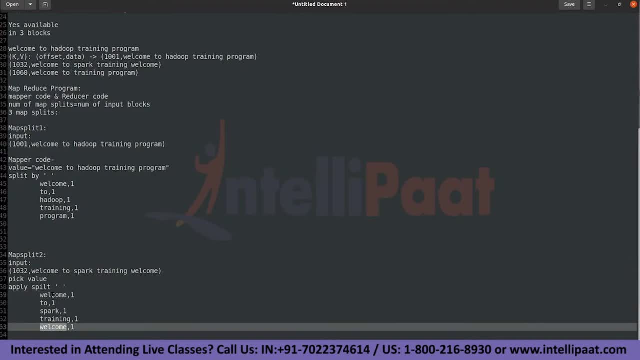 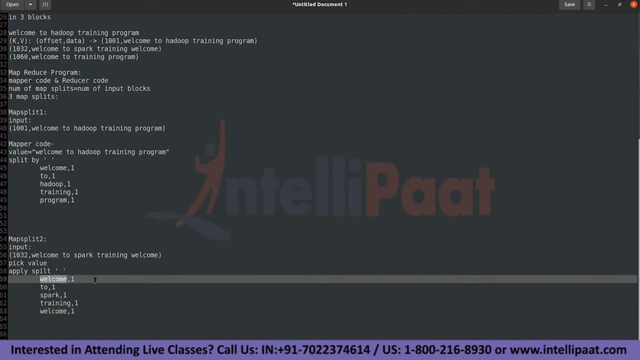 identifying whether the same key is available here. if i there is a same key, i'll have to give two for it. i didn't write all that code. regardless of what data you have in the form of a key, my only logic is to allocate one by default. agree, yeah, i mean, let's not get into that key and a. 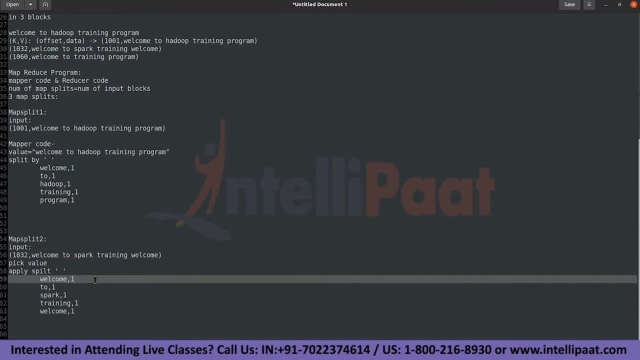 value pair. see keys are. this is just looking like a k comma, v format: okay key and a value pair: okay, so it's not a unique key that we are talking about. okay, so this is my map split two output and similarly map split three output. also i'll write, so just just tell me, i'll directly write. 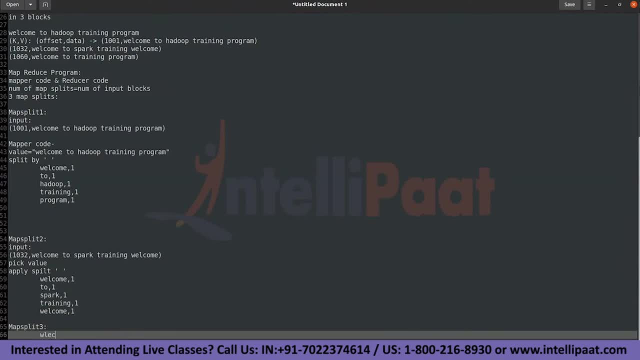 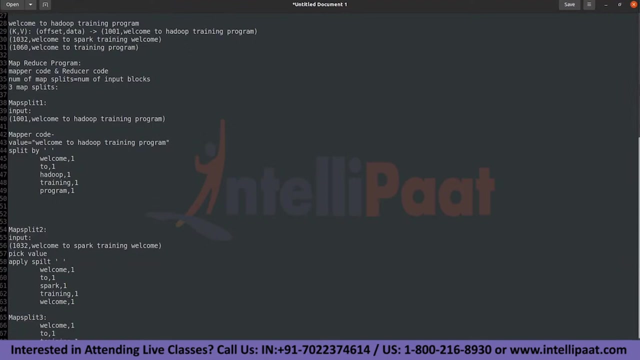 the output. so, which is going to be welcome number one, i'll give you a proper, proper under a proper reasoning. why have we have to allocate only one at the end of this discussion? but at least for now, let's look at this. welcome to training program. is it number one? program number: 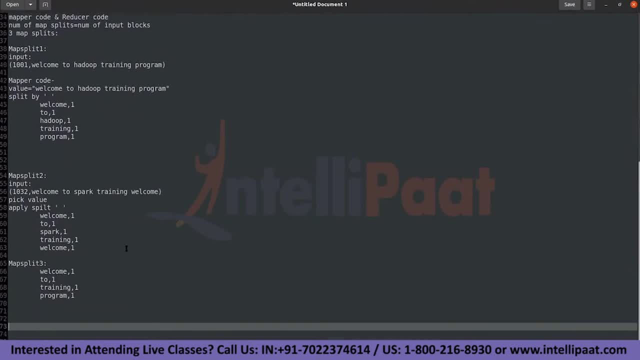 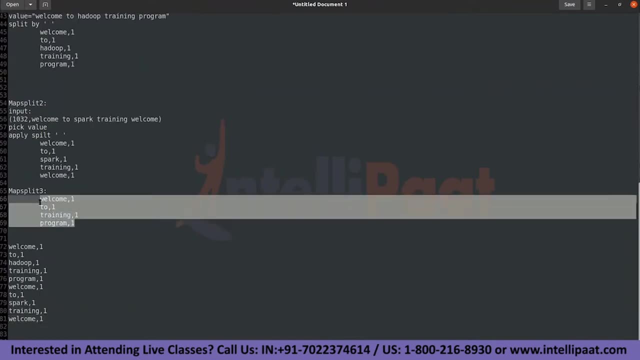 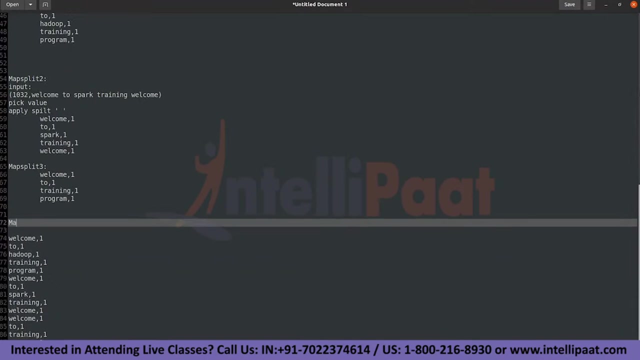 one. this is map split. three output. all right, so all these three outputs, where they have to go? they have to go to a reducer. all the three outputs of mapper, where are we supposed to send them? we are supposed to send it to a reducer. now, right, this, i can call it map output. map split: one, two, three together, everything will be a map output. 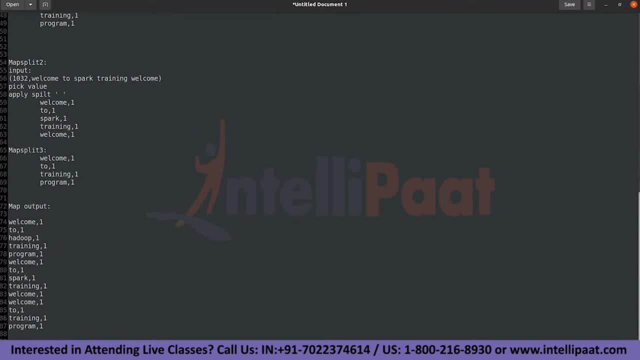 now, where am i supposed to send them? reducer? so, looking at this output, what can i write inside my reducer? what logic i can write inside my reducer? so reducer also is in the format of a key and a value pair. fine, that's okay. what do i have to write inside? 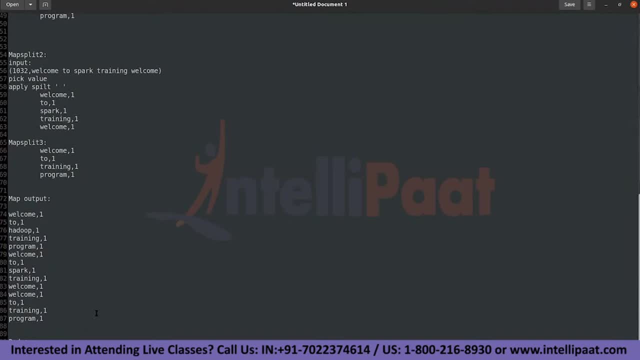 my reducer now tell me, okay, so i'll find out key find, i'm just writing it in a theoretical way. okay, find repeated keys. right, and repeat repeated keys and count them. count values: yes, this is what we are talking about, agree, right? so after the map output and before the reducer, the logic might. 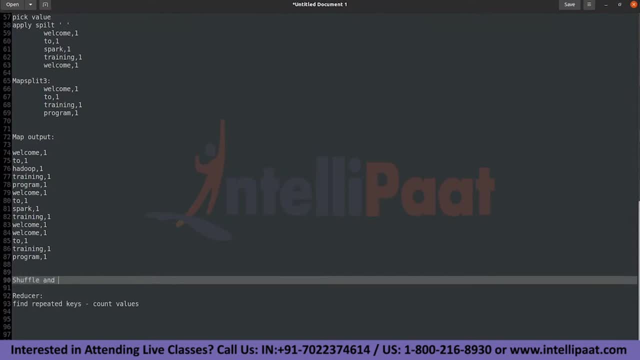 not change, but there is something called as shuffle and sort. so this is not. i mean, you're not going to write any program for shuffle and sort. your map reduce engine will take care of this shuffle and sort operation. the only logic you are going to write is for mapper and the other logic is for the reducer. so what is shuffle and 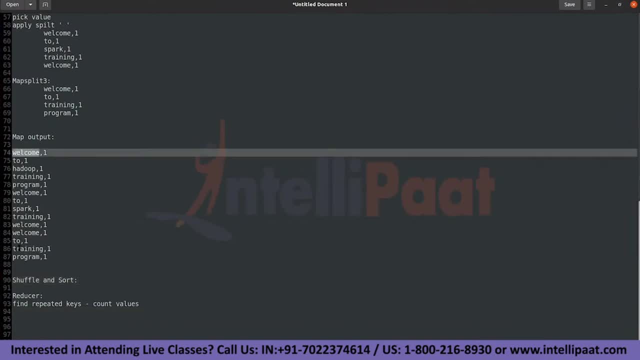 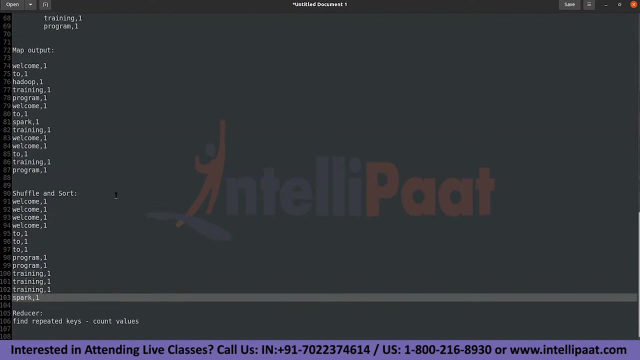 sort doing is it will shuffle the data according to the different keys, something like this. it will shuffle something like this: okay, welcome to all welcomes together, all twos together, right, twos together, and all programs together and all trainings together. just forget about, i mean, whether they are two or three. that's okay. okay, this is one. so this is what your shuffle and sort. 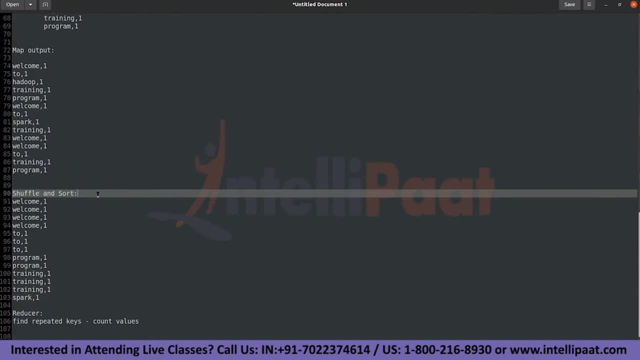 doing so. the major operation, the main operation of your shuffle and sort functionality is just to make sure whether you have received the output from all the three mappers or not. see, i received the first map split output, that's fine. i received the split output, that's fine. i received the first map split output, that's fine. i received the. 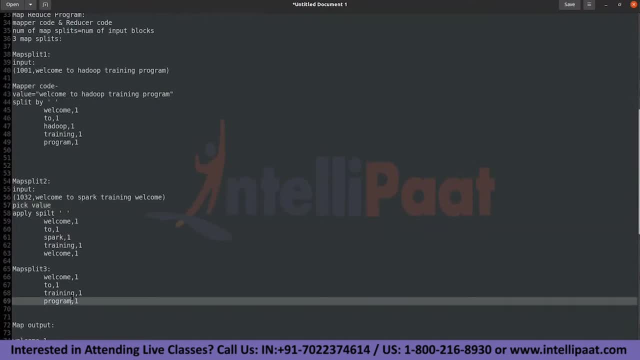 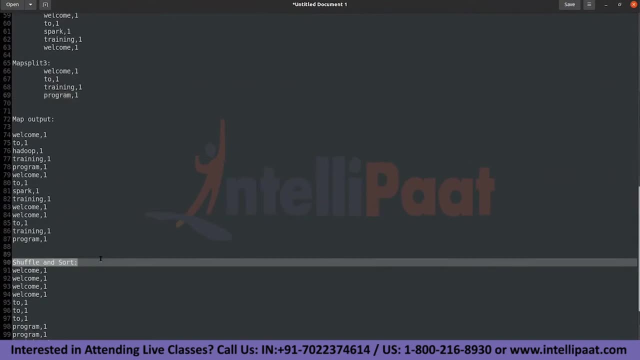 second map split output. that's fine, but i did not receive the third map split output. i cannot send it to the reducer right. so this shuffle and sort is some kind of a threshold where it will wait for all the map splits executions, all the task trackers to complete their execution and 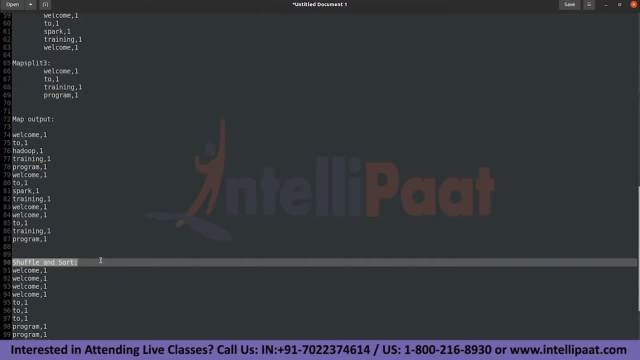 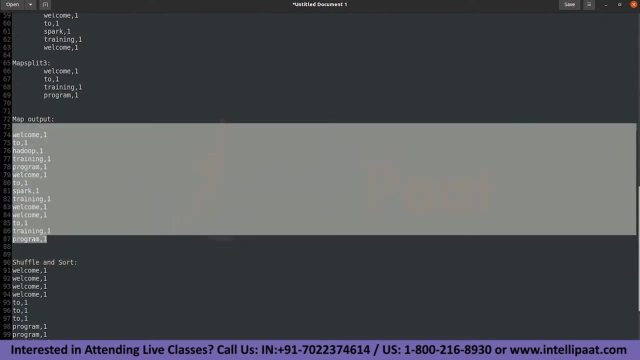 send their outputs. so i know that there are three task trackers allocated, three map splits and three task trackers allocated. so my shuffle and sort has to wait until you receive the output from all the three task trackers. this is some kind of a threshold checkpoint. i can say, okay, so after you receive from all the three, 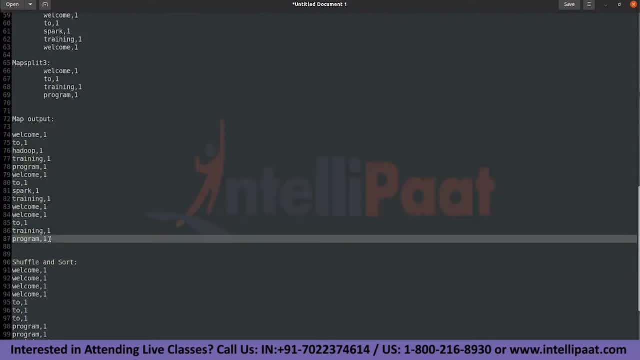 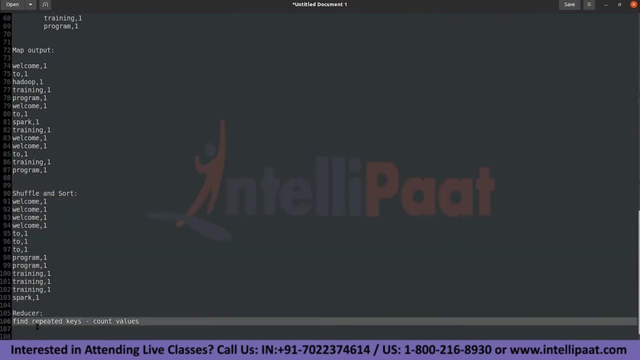 outputs: three map tasks: map tasks: i'll be doing a shuffle and sort and i'll be allocating the unique keys together. understood a simple operation. that's it. so can i write something like this? find up after that. okay, shuffle and sort. output you got this is: you are sending it to the reducer. 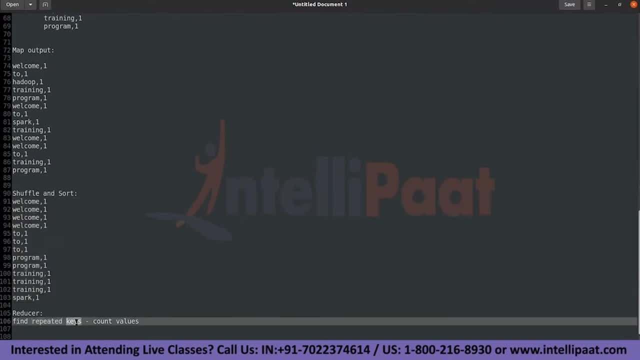 so now this is how you have the data: you are finding the repeated keys and you are finding the count of values. can i do sum of values, finding the repeated key, and i'll do some of the values? okay, so it is just waiting. it is just making sure the data is executed. i mean, all the mappers have executed the tasks. that's it okay, and 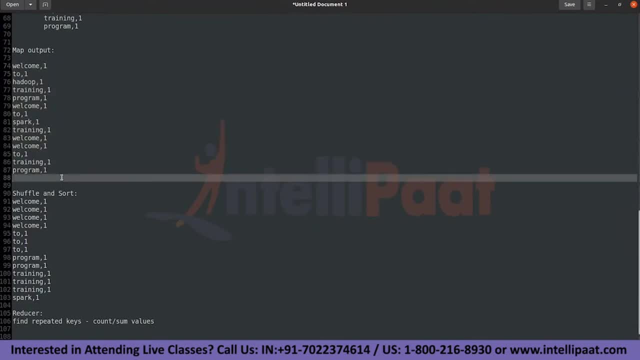 and after you receive the output from all the mappers, it is just shuffling it and sorting it. that's it, sorting it, some depending on some order. anyway, if there is no sorting, also, there is no problem. right, we are anyway doing the uh read operation on top of all the results here, right? 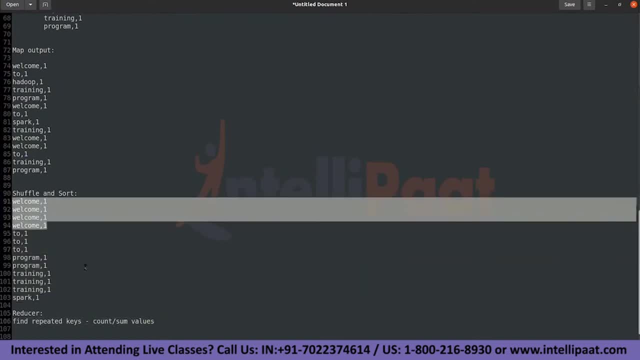 in the reducer. so you are finding the repeated keys and you are even finding the count of the values, or you can also find the sum of the values. agree with this point. you can do both. both will result to the same output. this is where the result will come into. 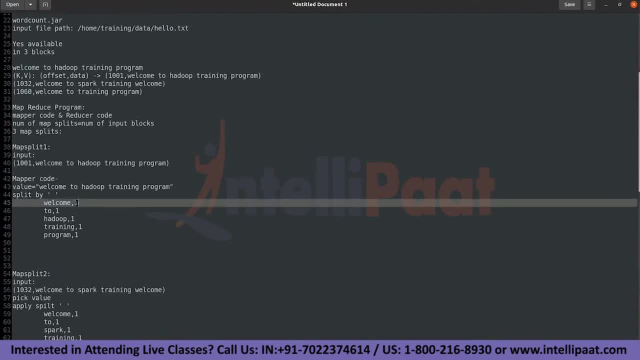 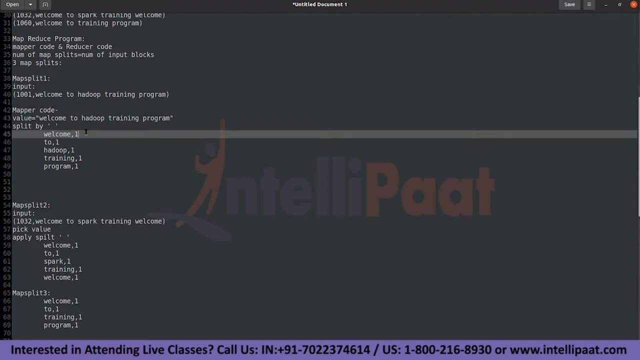 so why have i? why, why am i allocating only one by default? is this, is my code right? i'm allocating one by default. so, for example, you, you contradict to the statement and say that, okay, i can't allocate one by default, i want to allocate a here, right, some dummy value, some you write whatever you. 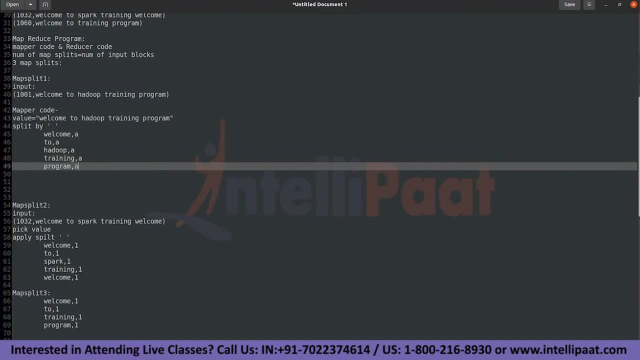 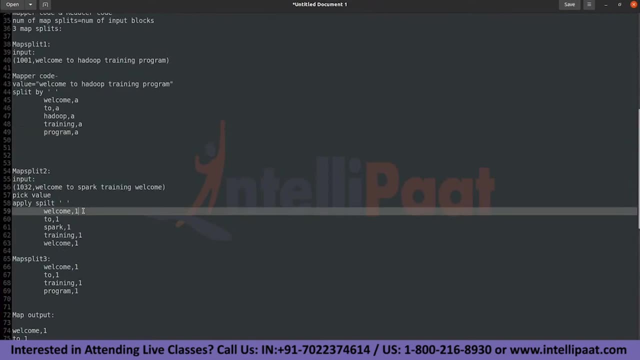 write your name also. whatever right, but some unique value. so in this case, your outputs from mapper 1, you are allocating a, and outputs from mapper 2, you are allocating b. or map outputs from mapper 3, you are allocating c, so at the end you will receive. 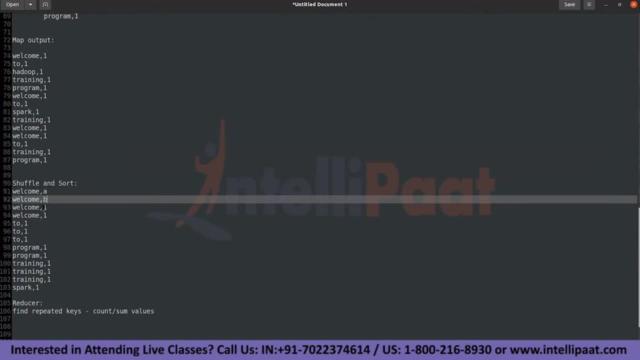 welcome comma a. welcome comma b. welcome b. welcome comma c. right, if you get like this, what is your reducer if you are allocating different outputs other than one as by default value? what you need to write? you need to find out the repeated case and you need to find out only the sum of its as a. 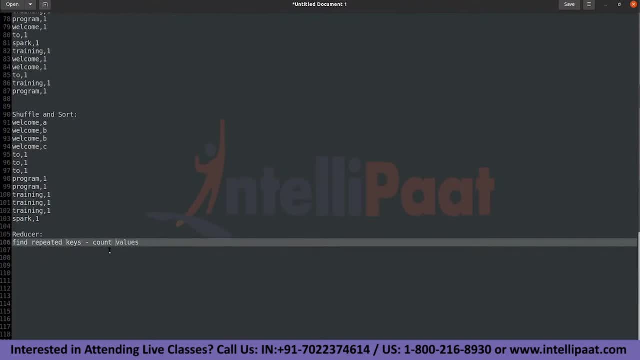 count of it. some will not work in this case. so, depending on what you write in your mapper, you are changing the logic of your reducer. that's it, okay, so there is no necessity that you are supposed to allocate one only by default. okay, you can allocate whatever you wanted to, but based on 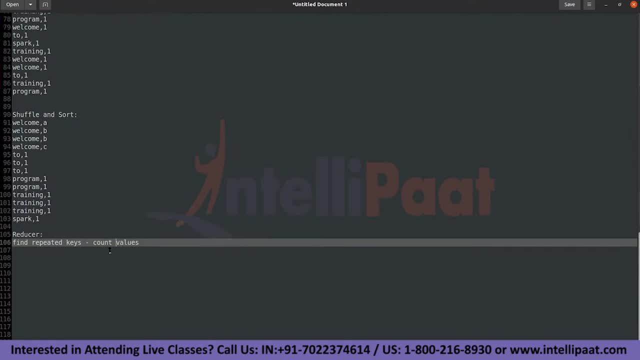 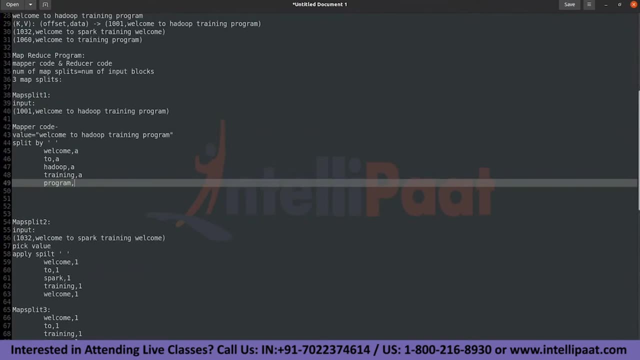 the data that you send as an output from the mapper. so what output you are you are receiving from the mapper. depending on that, your reducer code will change. okay, so now that i'm allocating one by default for all the values inside the map split, i can do whatever i wanted to. i can do a. 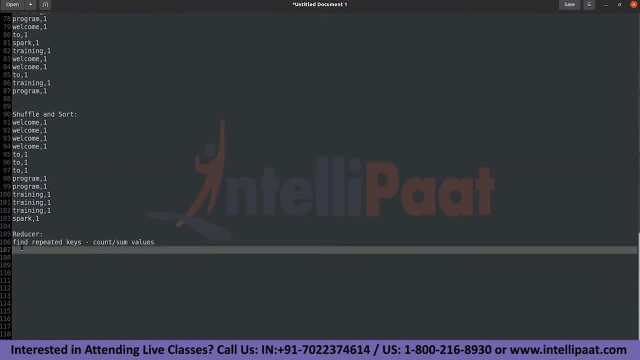 count of values, or i can do a sum of values also. so now, in this case, can i do something like this? reduce by key. this is a function that i'm going to use, using the reduce by key function on this particular input. it is going to generate me an output something like this: welcome comma four. 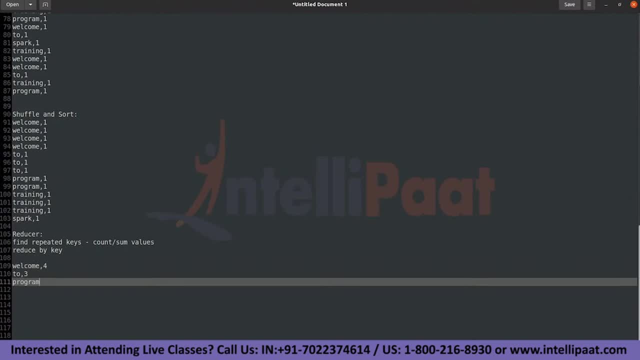 two, comma three: program comma one: you, you, this is what i get. agree with this? okay, fine, so this is how you, you execute a map reduce program. okay, so this is the logic. this is what you're gonna write. you write some code in the mapper depending on the mapper code, you, you define your reducer logic and you can find the word point. 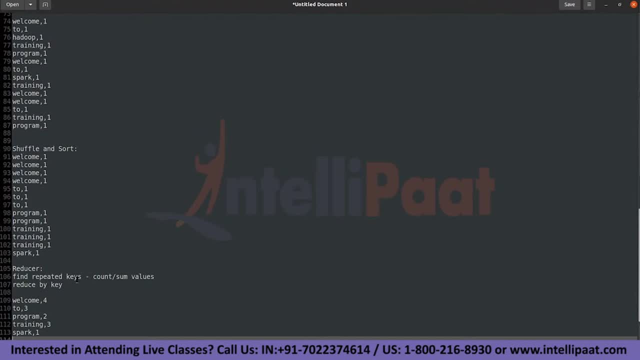 so now we will think about some enhancements in the mapper code and we will think about some enhancements in the mapper code to this. okay, so this is a core program. mapper reducer is is the core program. on top of it, what are the other enhancements that you can do? so if you look at the uh map split two. so someone was. 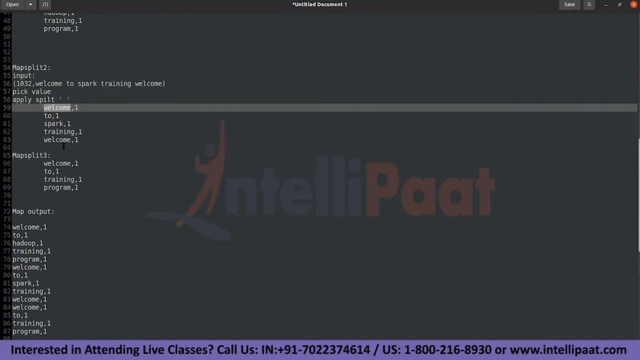 pointing out. so there is welcome comma one here and welcome comma one here. why can't we do welcome comma two here itself? rather than sending two welcomes, you can only send one. see. what i'm trying to say is see, uh, the output of map split two. how many records are there in the mapper code? 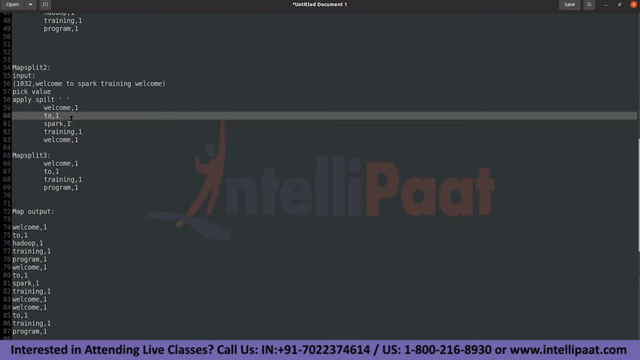 do you have one, two, three, four and five? right, but i'm sending welcome twice. so why do you have to send welcome twice? why can't i do welcome comma two? and i only can send four records there? right, it's anyway the duplicate. why can't i, why can't i do the aggregation here itself? 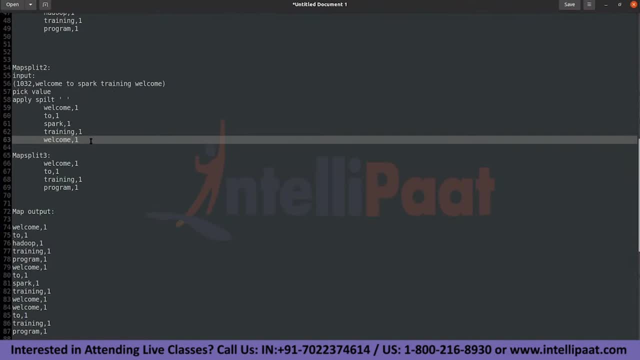 what i'm what i mean to say is so i'm converting this into this so you understood this thing. map split two output. earlier i was sending five. why can't i send only four? what is the advantage i get using this? see, i i was sending five. earlier. now i wanted to send only four. why can't i send four? 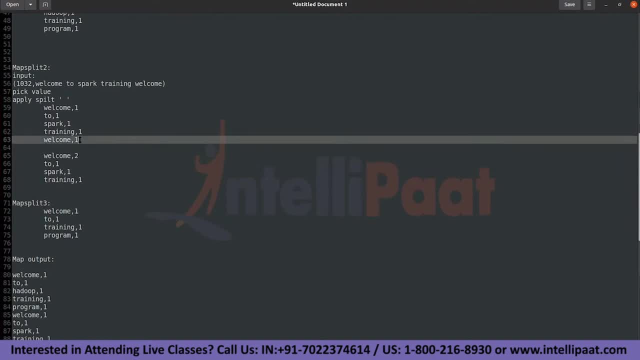 the advantage i get is i i reduce the network traffic between the tasks. okay, so map task is one, reduced task is one, right, so how many records am i sending between the map tasks to the reduced task is? is the network bandwidth i follow. so now, uh, i'm sending. let's say, 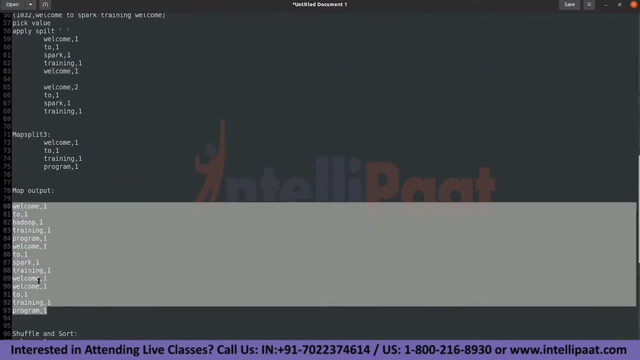 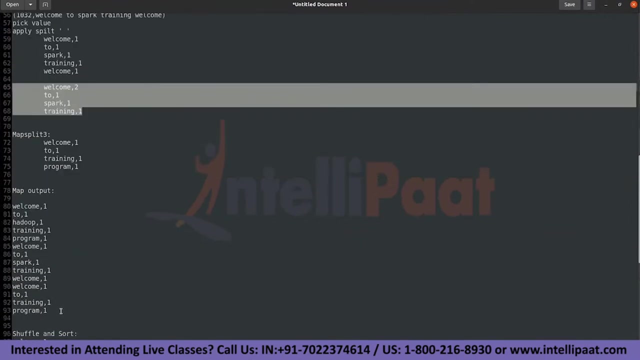 20 records. i'm setting how many are there? uh, 80 to 93, right, 13 records i have. right, so 13, 14 records i have. so i'm sending 14 records here in the previous scenario. now, by doing some aggregations within the mapper task, i'm only sending 13 records. that means i'm reducing the number of. 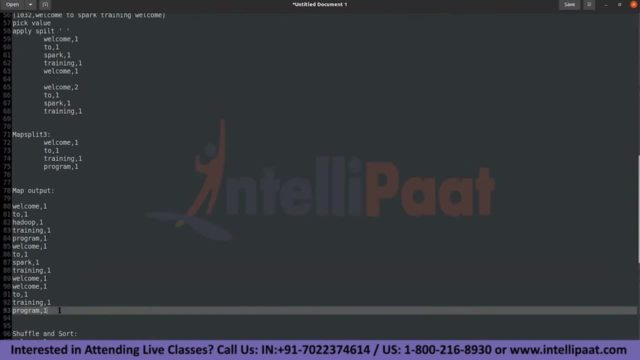 records that are supposed to be sent between mapper and a reducer. see, it does not make much of a difference. 14 and 13: right, but when you have more number of records duplicating like this within the map task, you're recording more records than you're only sending reports to the mapper task. so 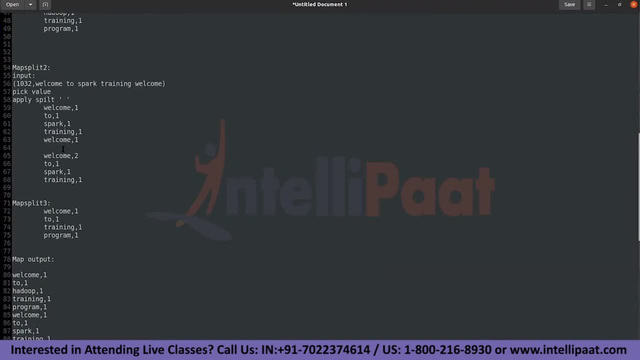 it's going to make some difference, right when you are dealing with large amounts of data sets. instead of sending the data again and again or multiple times repetitively across the same task, you can do some aggregation and filter all the repeated values and send the output to the reducer. 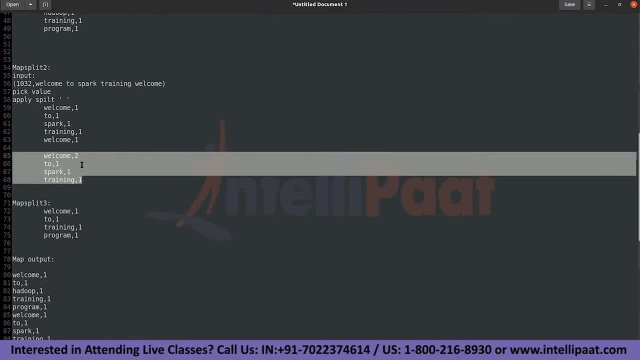 it's. it's. it's reducing some burden on this task which shuffle and sort, yeah, shuffling and sort will remain the same. i mean, that doesn't mean no, no, no, it means it will take less amount of time, less amount of uh records to process. see, in this particular scenario it's only 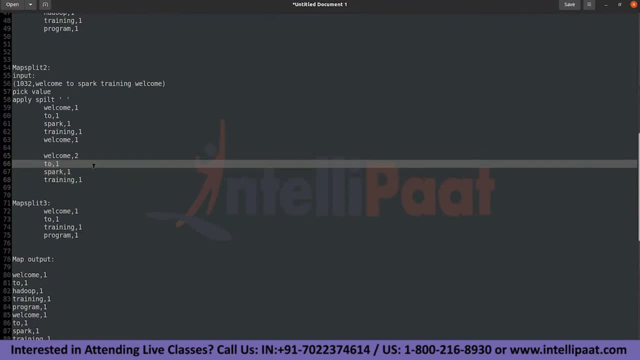 one additional record we are sending. but but in general, when you are dealing with large amounts of data sets, with duplicate values within the same splits, same task, right then, then it will definitely make some change. so, okay, there is a use. i mean, i what i'm, what i'm trying to conclude here. 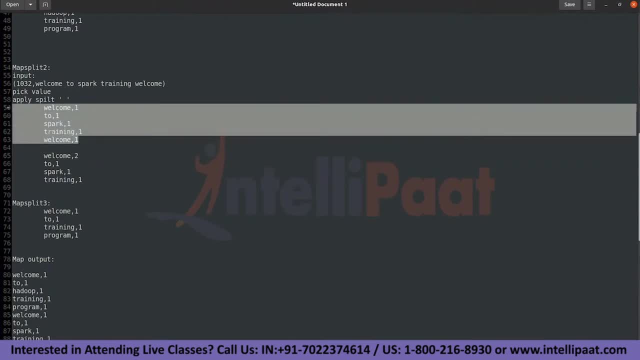 is. there is definitely some use in reducing this. duplicate values. but how do you do it? tell me, what am i supposed to do here? i'm supposed to convert this welcome comma one, welcome comma one, into welcome comma two. how am i supposed to do it? checking the duplicate keys and do what? 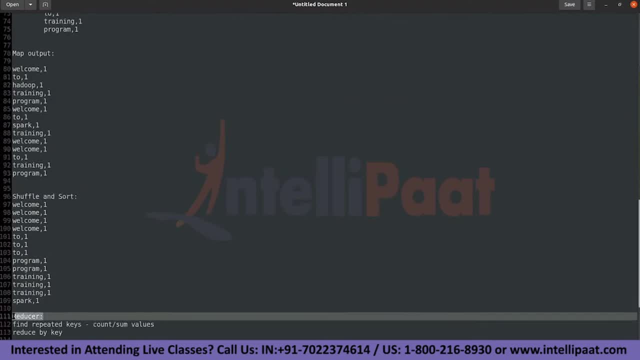 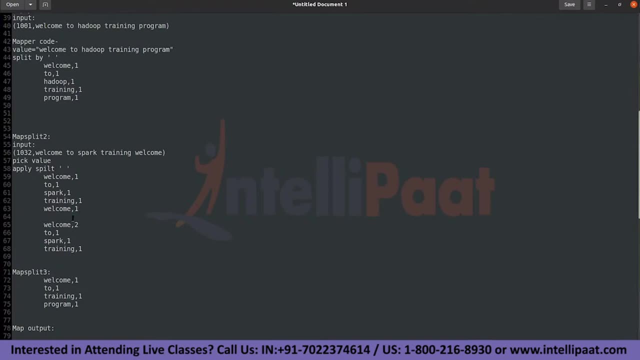 what is that logic? is it not the logic of a reducer means? before sending the output to the reducer, i'm actually executing a reducer within the mapper itself, within the map split, understood? so so inside this map split 2, i'm calling a reducer function or reducer class. why am i calling this reducer class? just to remove this, just to further. 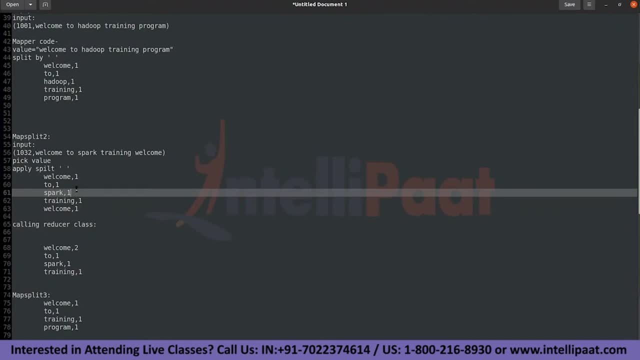 aggregate it. i'm it's not about the duplicates always, but just to further aggregate it anyway. we are supposed to do the same thing in the reducer phase, but why am i still going to the reducer and doing it? i can do it within the mapper itself, right? so by doing this, what is? 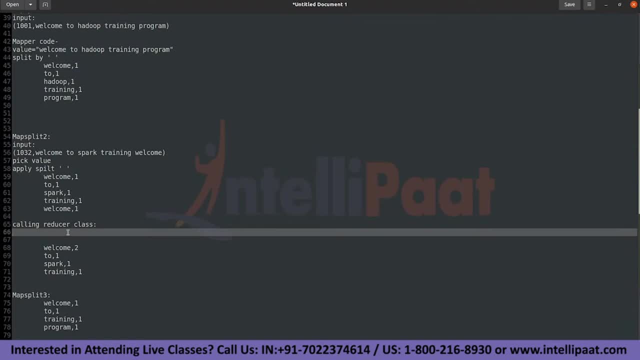 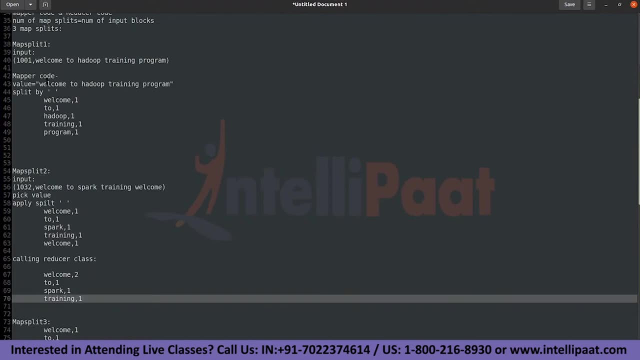 what is happening is you are executing the reducer within the individual mapper split, only within the individual mapper task, getting it so in the mapper code. what you are supposed to do is see in mapper code. inside the mapper code you have to call this reducer function. call reducer. 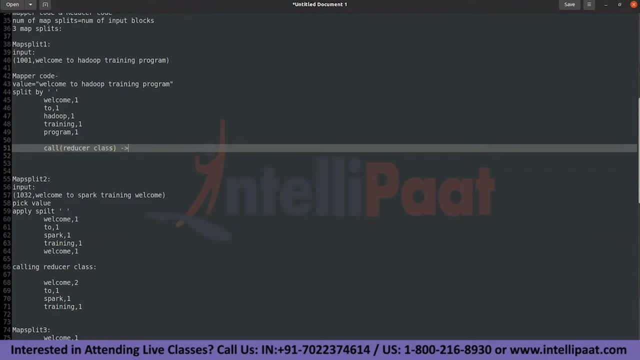 class. so calling this reducer class inside the mapper code is called as a combiner logic. so mapper is one, reducer is one. inside the mapper you will be writing a logic for the combiner which is going to in turn call the reducer function. you are not writing any additional class for the 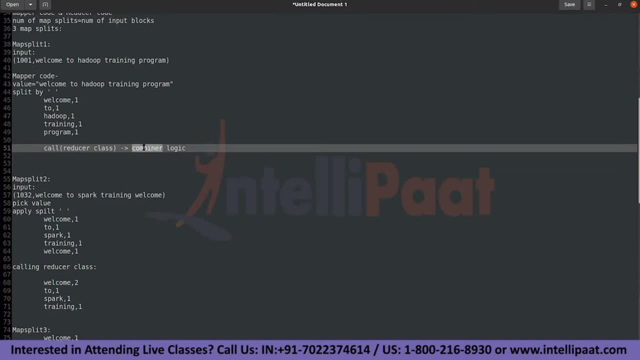 combiner. it is one single line of code that you are going to include inside the mapper class, which will, in turn, call the reducer function. agree? so instead of going to the reducer and executing those tasks, i am applying a reducer function within the individual mapper task only. 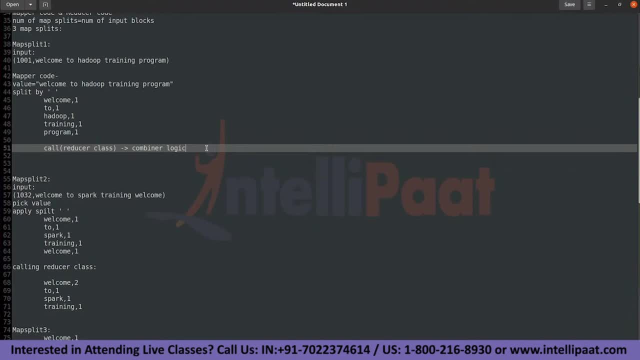 that running of reducer class within the individual mapper class is called as a combiner class. okay, so combiner is going to reduce the network traffic or the number of records that you are going to traverse through from mapper tasks to the reducer tasks or to the shuffle and sort tasks. 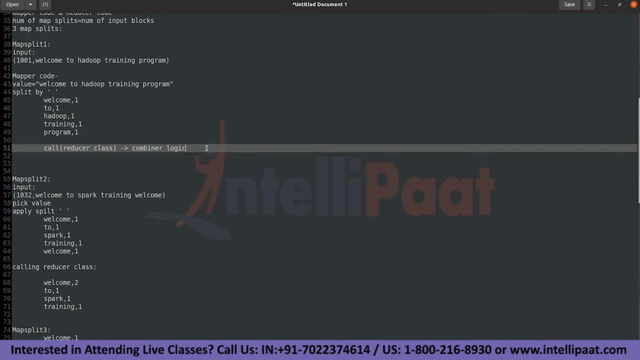 that is one way of the performance enhancement. see how am i? am i compromising on the code? no right, it's only one line of code. it may it may take some time for the execution, but if it is worth it, then it's definitely going to be helpful. we are not increasing the number of lines of the 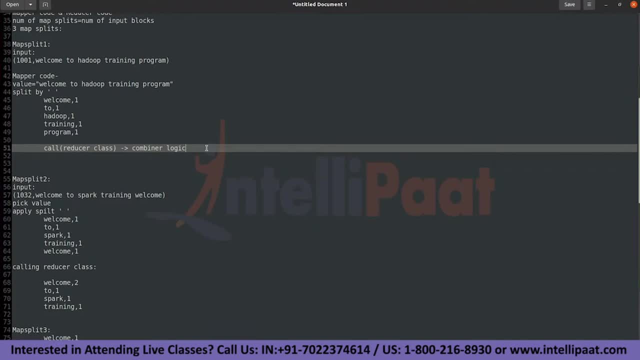 program. here we are only just adding one line of code. you are just calling the reducer class there, right? so by calling a reducer class within the mapper class itself, you are removing the aggregate, i mean you are removing the, you are combining the duplicate records or combining the repetitive records and reducing the number of outputs that you. 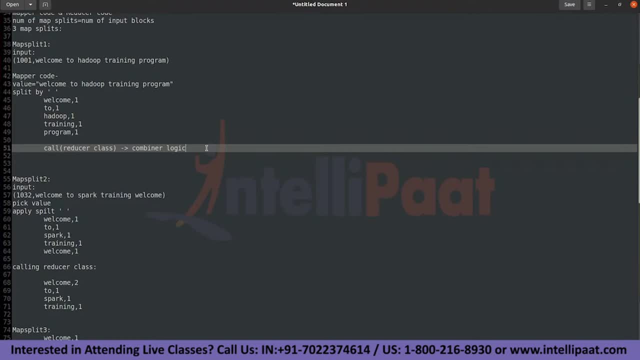 are sending it from the mapper. any questions? are we clear with this map? split map logic, reduce logic, shuffle and sort logic and a combiner class logic. so this is one of the performance enhancement that we have which is going to reduce some network traffic between or some number of records that are. 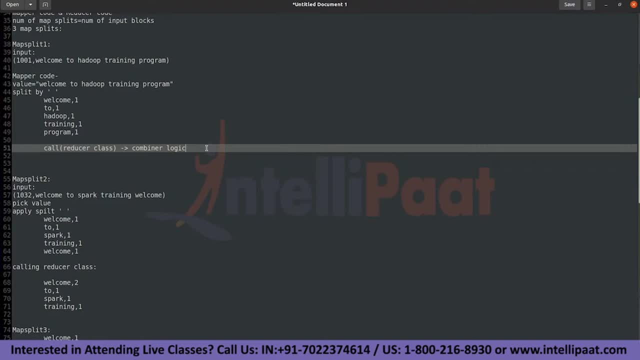 sent between the tasks, individual tasks, map to shuffle, shuffle to reduce or whatever right which is going to reduce the number of records. and there is one more performance enhancement. so we cannot call it as a actual performance enhancement, but the uh uh enhancement of the particular output. see, for example, i have this as an output right. 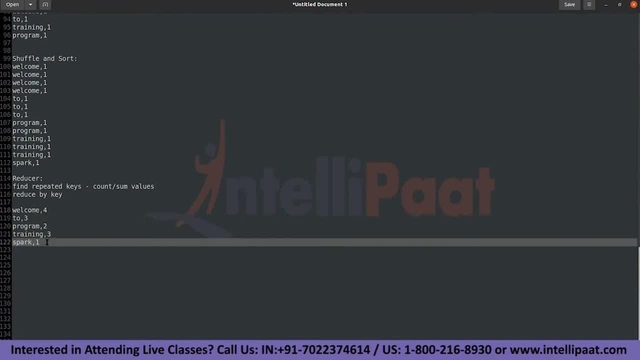 reducer class is giving me this as an output. what if i'm saying: see, when you look at the output, the output path will look something like this: in hdfs. you are saying the output again: in hdfs only. so your output will be stored in somewhere like this: home training. you give some output and 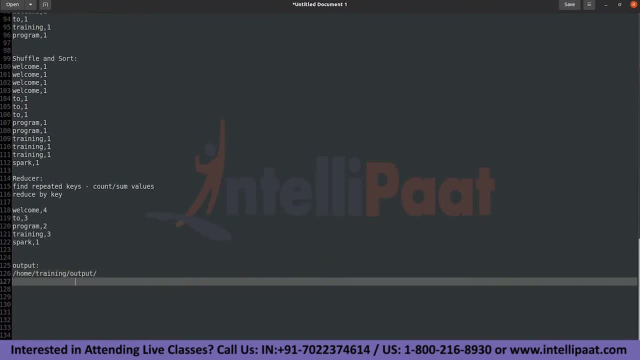 under output folder you will have part hyphen zero, zero, zero, zero, zero five. so under output folder you will have part hyphen zero, zero, zero, zero, file name and also a success file. so this is the format of the output file. okay, so don't get confused about this. so part hyphen zero, zero output file will be here. this is this is going. 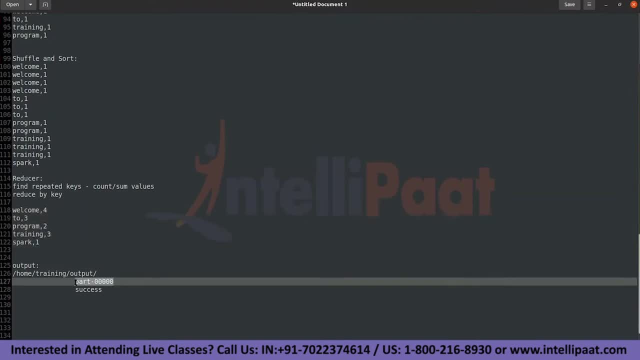 to sit in this particular location in this particular file- okay, and there is a log message that is a success message. for every successful map reduce execution, you will find a success message listed. there is nothing written in this, it's just a success. uh, uh, empty file- okay, and you will have. 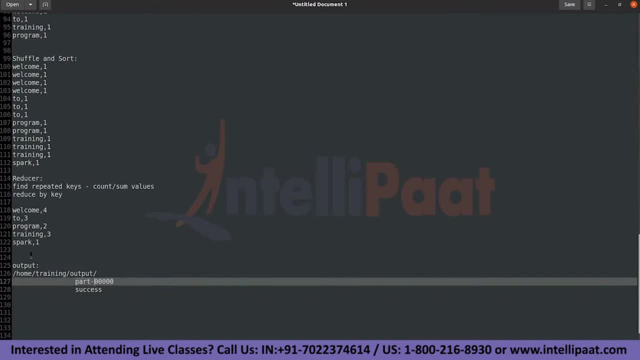 a partition file- zero, zero, zero, zero, zero- with the output in it under the output folder. okay, so now this is my output file. but what if i want to do something like this? see, our partition output file will have all these outputs. so what i wanted to do is what i want to do is i want to generate an. 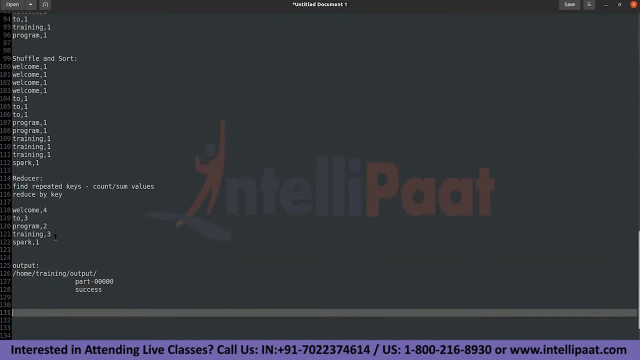 output file which can be used to generate an output file which can be used to generate an output file. so you can see, here it consists of values only which are repeating more than once. that means only which are, whatever the values are repeating more than once, only those values i need. i don't need. 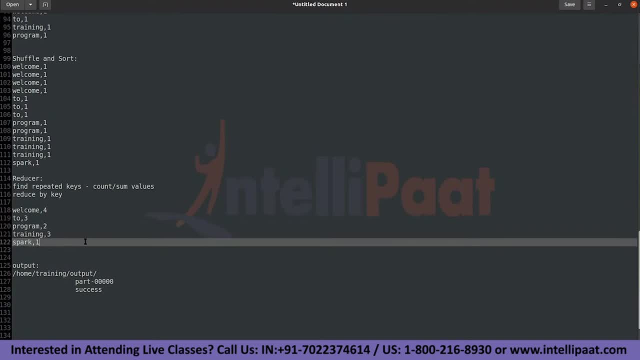 the values which are repeating once, only once. okay, i just have to segregate or i just have to partition the output into two, wherein one folder will have the output one of where, where, which are repeating more than once, and the other file will have the output which is only repeating once or otherwise. 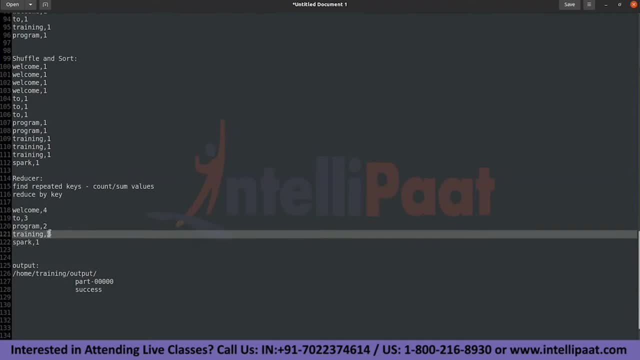 ignore these values. i just don't want to find only one output file wherein it should. it should generate only the data that is repeating more than once. right even in the earlier scenario: voterscsv. we have seen right. so output file: what does it show? party a has received so many votes, party b. 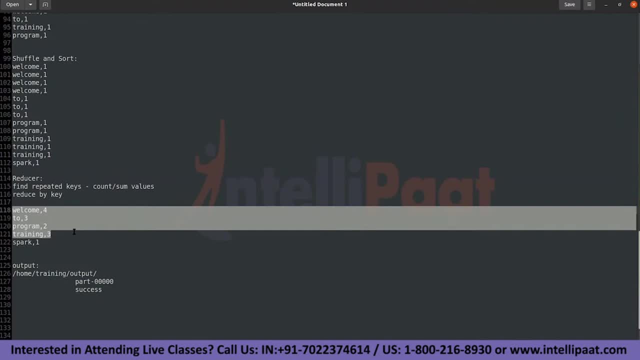 has received so many votes and party c has received so many votes. this is the output you get. yes, but why do you have to think about party b and c when you have party a as a winner? right? so my output file should filter the data according to the maximum number of votes and it should only 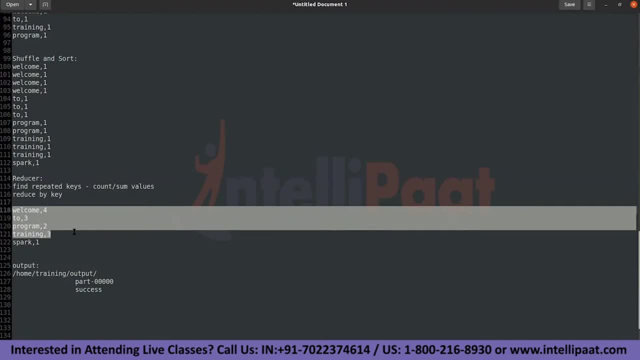 generate an output file which has got the more number of part votes right. that is, you are filtering the output and you're only receiving whatever the output. you need only filtering whatever the required output you wanted to generate. so here my required output is: whichever. whichever words have received the count more than once, i wanted to load them in one file. 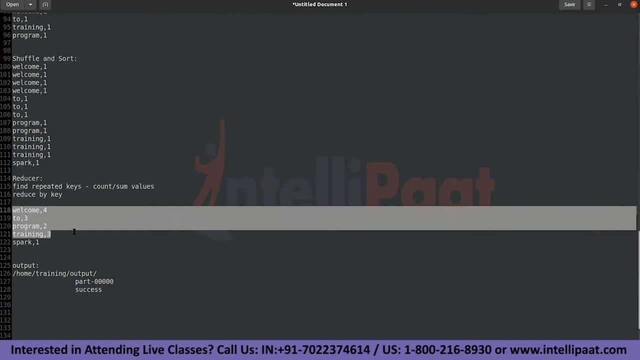 and all the other dummy values. i want to load them in the other file. more than three or four times i wanted to generate. i'll load them into one file and other values will load into another file. so this is what you call it as a partitioning. 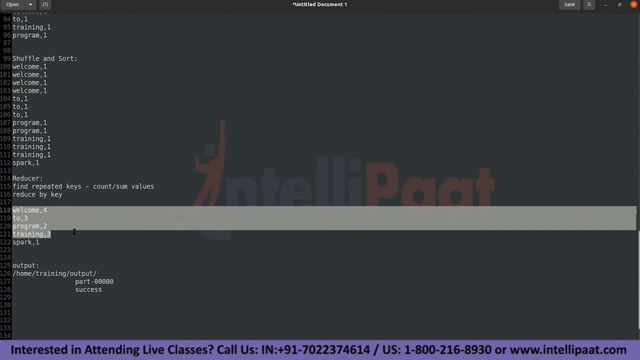 of your output. okay, so we do a partitioning of your output file depending on the user specific scenarios, depending on whether you wanted to filter them or whether you wanted to divide them into two different files. all that will be done. so there are two ways of partitioning it. so 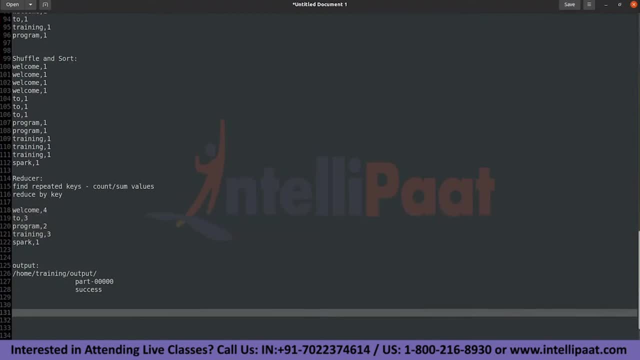 in again apart, like, like we have done in mapper and reducer, you have to write a partition class for it. so in partition class you are supposed to write some program, you are supposed to write some logic for it. okay, so there are two ways of doing it again. one is dynamic partitioning and custom. 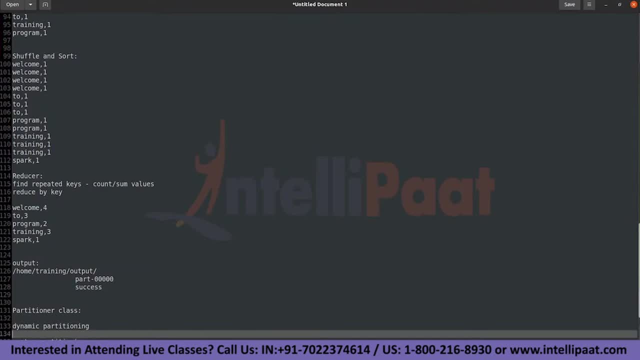 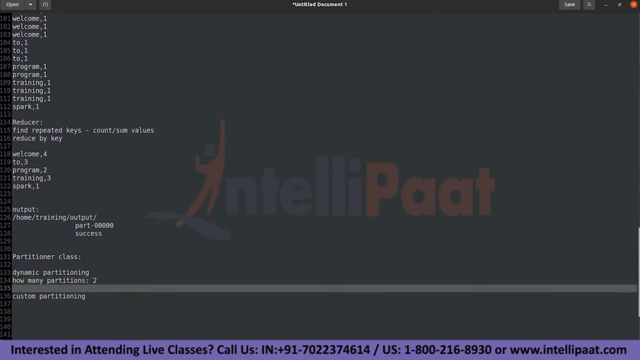 so in dynamic partitioning you just have to specify how many partitions you are supposed to divide them. let's say two. in dynamic partitioning you're not supposed to. i mean, you're not. you're not required to write any logic. see, i only wanted to divide the output into two partitions. 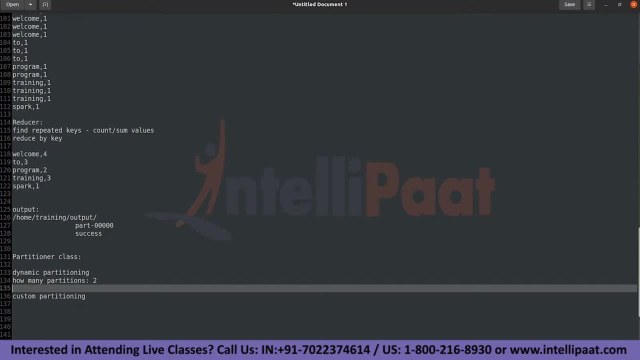 how am i going to divide? i'm not writing, i'm not defining any logic for it. the system itself will design, define it. so let's say: if i define, if i, if i tell them that i need two partitions, let's assume, uh, greater than three and four will be one partition and less than three and four will be. 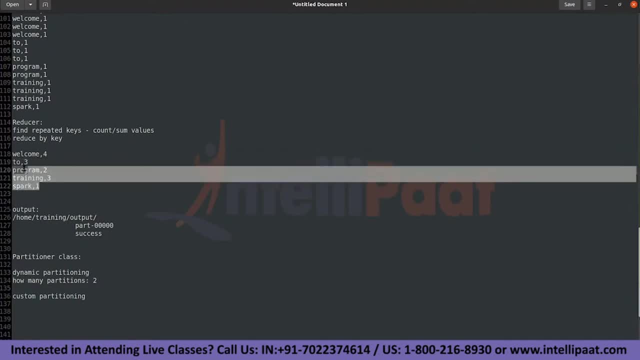 one partition divide. depending on the amount of partitioning you are supposed to write, let's say amount of output that you have- it will try and divide the output into two different partitions. it will break the output into two different partitions if there are more number of records. 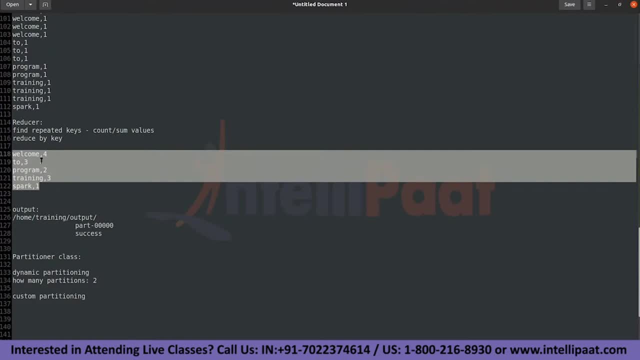 greater than four. if there are less number of records greater than three, it will find out another other, other logic. okay, some dynamic way of partitioning it. okay, we are not having any control on it. system itself will decide which data should go into which partition and which. 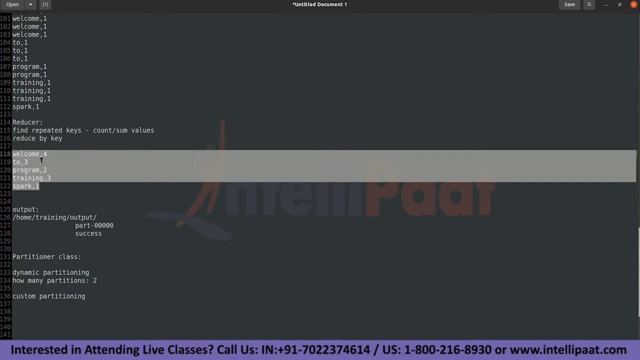 data should go into the second partition. so this is dynamic. you are not. you are not specifying any logic here. so what you tell is only the number of partitions. so set number of the, the value that the parameter that you are going to set here is. this is not written in the partitioner class, but 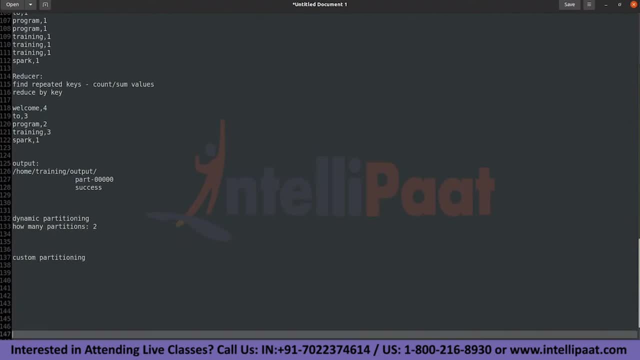 this is written inside the main method itself, so you have to write: set number of reducers is to set number of reducers to two, as in you are telling the system to create two partitions and you are not writing any logic for it. that means it is going to be collected dynamically and in custom partitioning you set 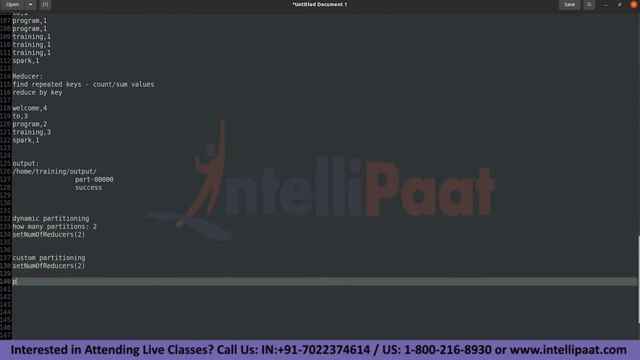 the number of partitions to two and you define the logic in the partitioner class. what logic? you are saying: okay, uh count greater than uh r equals to three will be first partition and l equals to three will be first partition and l equals to three will be first partition. 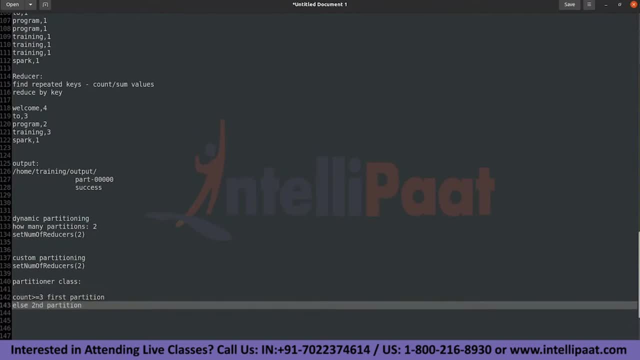 else all records will be second partition, getting the difference dynamic partition and the custom partition. so, dynamic partition, you will only tell the system that you need two partitions or three partitions or four partitions, whatever, whatever the dependent value is. but in dynamic, in custom partitioning, you are specifying the, the filter conditions also for the partitions to take place. 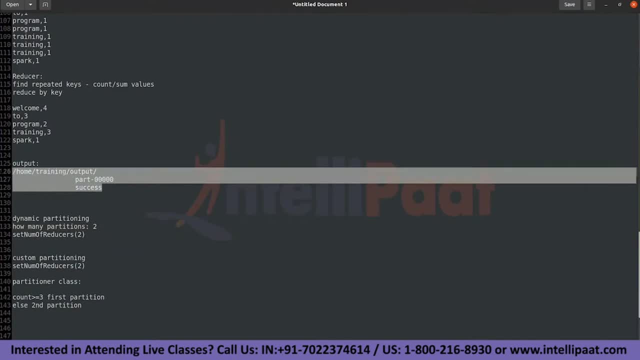 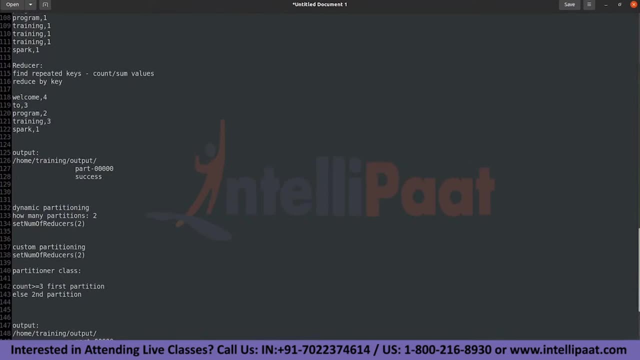 so in this case, what is your output file will look like? the output will look like something like this: in both the cases, output will look something like: part hyphen zero, zero, zero, zero. part hyphen zero, zero, zero, zero one. this is the first red user output, first partition output. this is the second partition output. 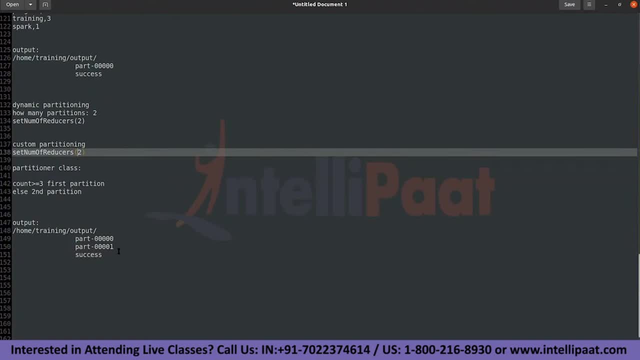 if there is three number of partitions, you will have zero, zero, zero, zero two. this is how you will be segregating the output of your red user. so where do you write this partition class? where do you execute this partition class? before reducer or after reducer? no, it has to be before reducer. 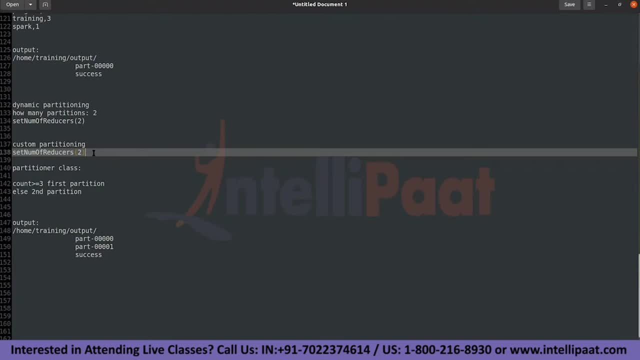 so, before the reducer itself, you're kind of segregating the data. you're kind of separating the data and executing it into two different partitions, two different reducers. okay, see, even though you are executing it before the reducer, it does not mean that you are trying to do a filter. 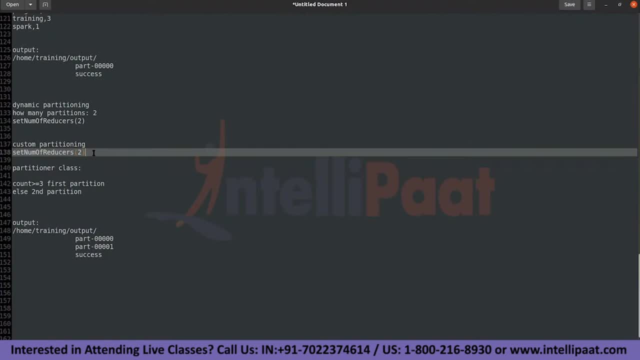 and you are trying to do and everything. so your, your, your counts and filters and everything will will happen inside the reducer only. okay, so this partitioner class and the reducer class run, run parallel. you can say, okay, both run together and the output will be segregated. so while we are, 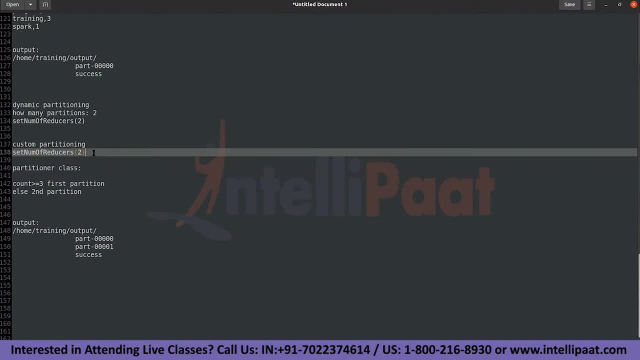 inside the reducer class. it's going to call the partition class and it's going to execute it. so are we clear with the logic partition class, what, what it's going to do, how the dynamic and custom partitioning is done. that's hash partitioning methodology. so depending on 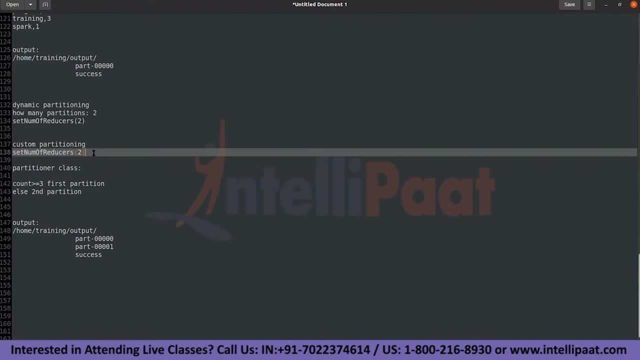 see if your output is is completely integer, is completely a number output. okay, integer output, let's say: okay, if you select two partitions, odd values will get into one partition and even values will get into one partition. so that's how it's going to divide generally, generally, very, very. 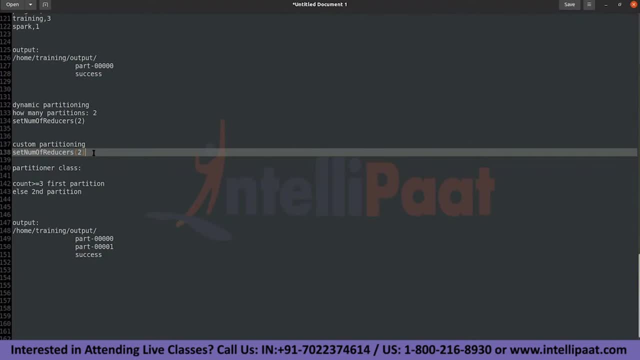 basic level partitioning. if you have 10 records, first three will be one partition, second three will be second partition and last four will be third partition, something like that. so it will just try and make sure that you equal number of records are being populated across two different partitions. that's it. 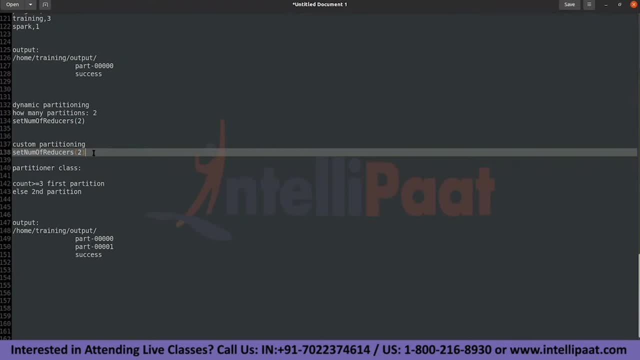 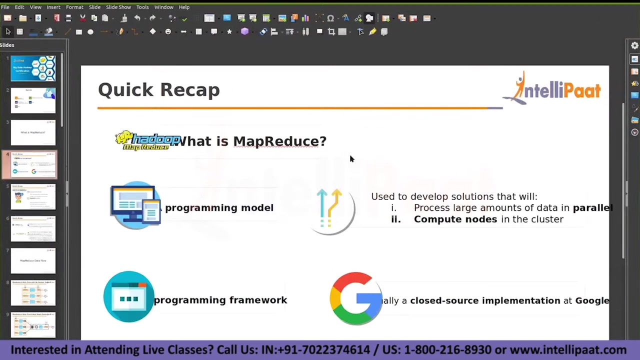 so what's the value or how it's going to partition it and all we? we don't have much of a control until and unless you specify that you, you tell the system that, okay, i want this data in partition one and this data in partition two. so map reduce is a programming model, a programming framework. 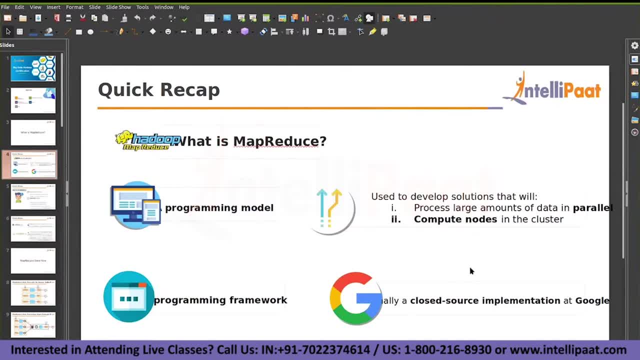 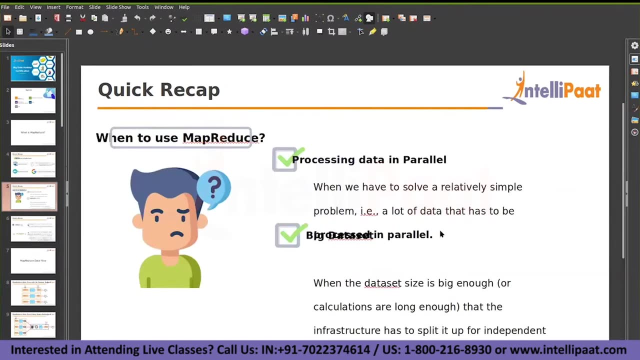 used to develop solutions that will process large amounts of data in parallel compute nodes in the cluster, generally a closed source implementation at uh, google. so this is just the technical definitions for it, right so when to use when you have um processing data in parallel and big data. 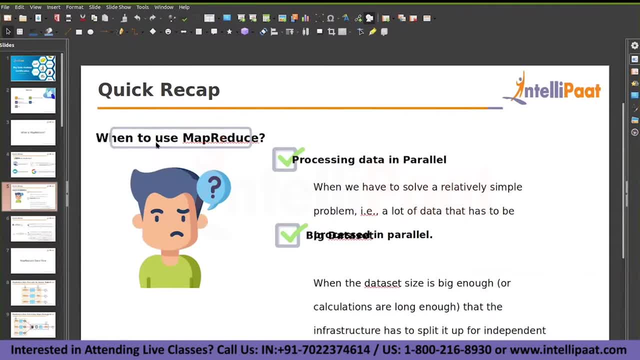 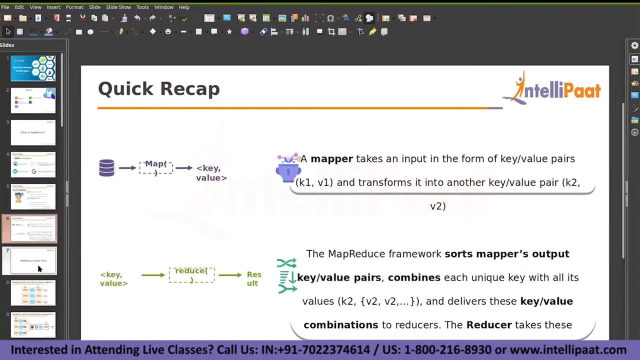 big data sets in parallel. okay, some scenarios. so there seems to be another documentation for this one, just scroll up. so there seems to be another documentation for this one, just scroll up. let's see one more documentation, right? so, uh, we know what is a mapper. a mapper takes the input in the format of a key and a value. 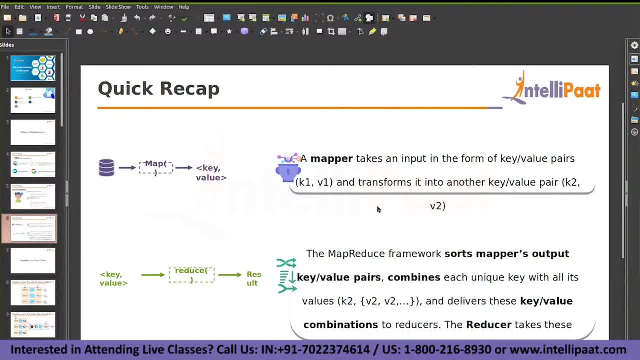 pair and transforms it into another key comma value pair. right, so that's what we have done in the mapper, right? you take the data, you convert that into a key comma value pair, apply the mapper logic and the output of it will also be a key comma value pair and a reducer, which is a sorts 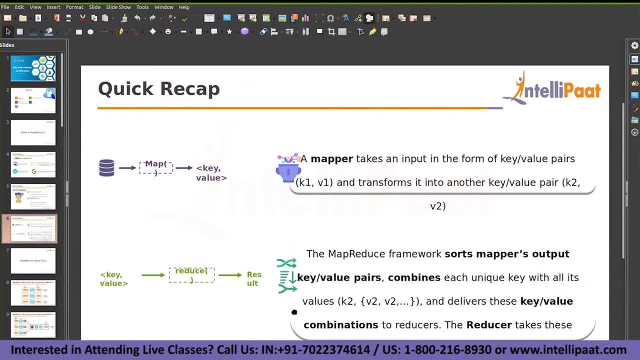 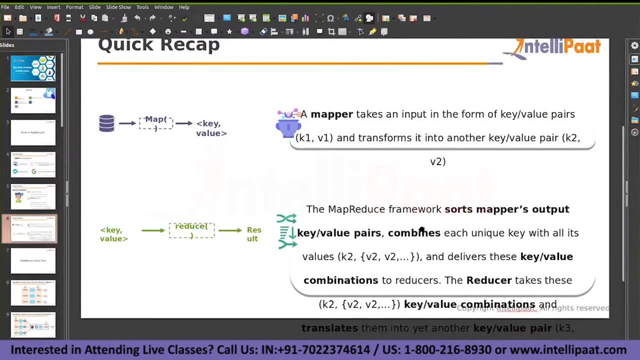 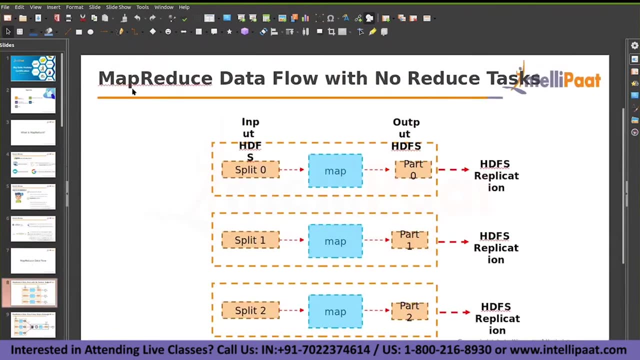 mapper output key comma value pairs, combines each unique k and all its values and delivers this to a comma value combinations to red users. right, so this is what the shuffle and sort is doing. and then, if you look at the data flow, this is a map: reduce data flow with no reduced task. okay, so the red. 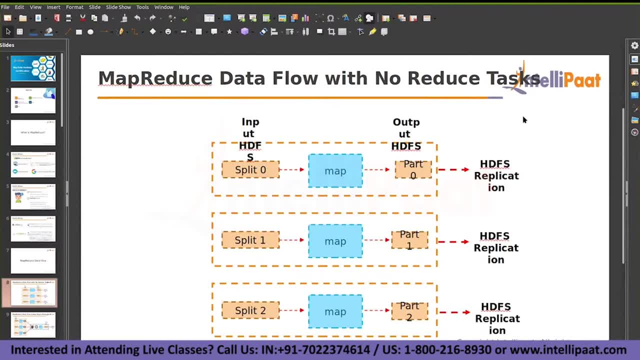 users. we have seen there is a mapper and a red user and there are multiple red users, right, so there are also operations where you don't need a reducer at all. okay, so, some functionalities, you, you pretty much write the logic in the mapper itself and and you, you don't, you don't have to. 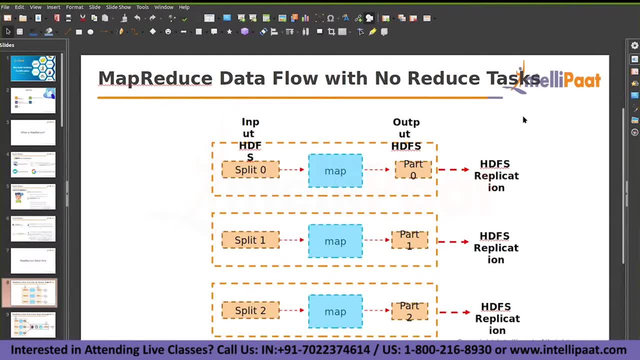 specify anything in the reducer, so reducer logic will be empty. you don't have to run any reducer logic for that, for that matter, right? so in that cases the number of set number of reduced tasks to be equals to zero. earlier we have set it to two, right? so there you can specify that to be zero. 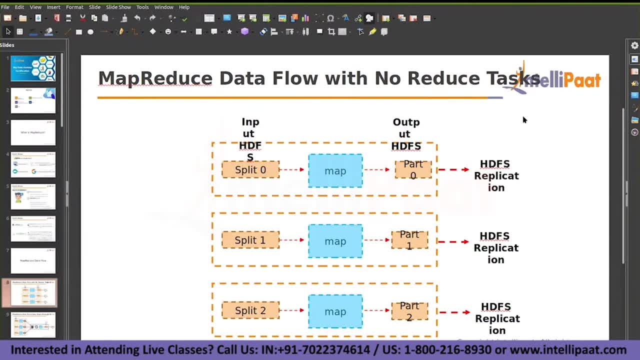 and you can ignore the reduced class implementation. so one very known example of a zero reduced task program is that we call this as a map only program. okay, so when there is no reduced task execution, we call it as a map only task, map only, map reduced program. so when you are, when you are ingesting the data, 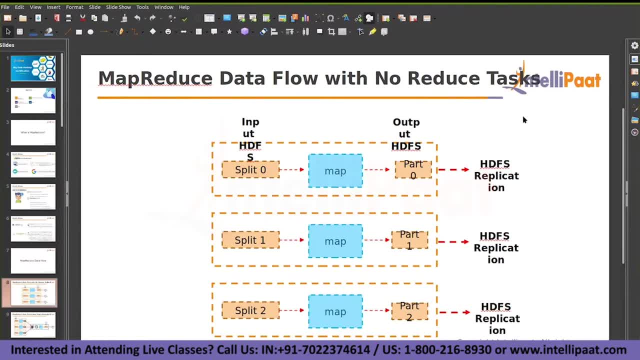 from a relational database. okay, for example, there is a source data available on some oracle database. you are writing a program or you're writing, you're using a spoof command to to ingest the data into a system- hdfs. so source is the relational database and the destination is a hdfs. that is a map only. 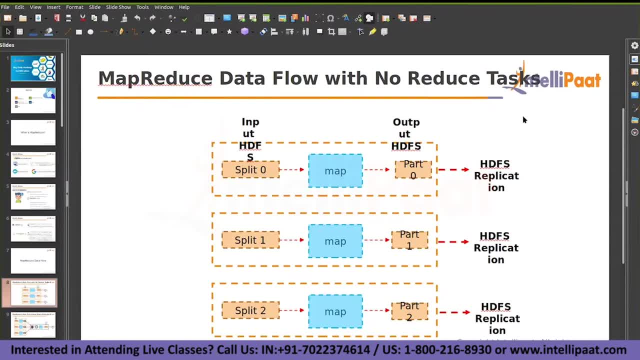 job. so all the ingestion related or the data extraction related jobs will be map only jobs. okay, so when you are executing the program itself, you can see, uh, the number of mappers are zero or one and the number of reduced number of numbers are three to four and the reducers are zero. so 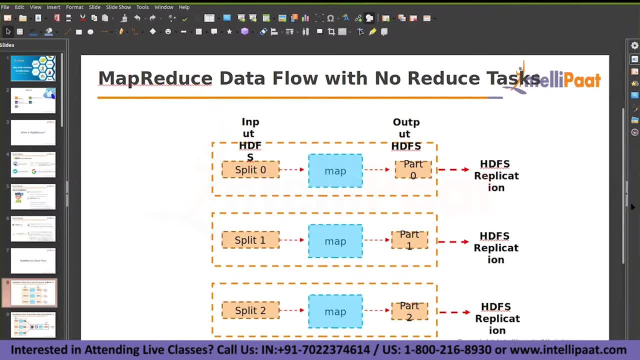 that that is also possible scenario. so in map only jobs, for each and every split you will have a output file getting created. so depending on the number of input splits available, after running a map output you will find the. in hdfs you will find the partition file getting created. so for split zero, you have a part file. for split one, you have a part. 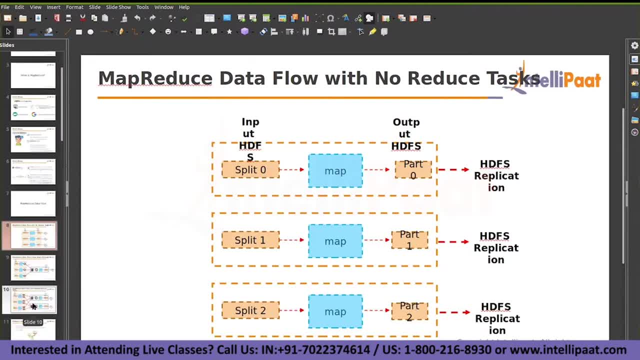 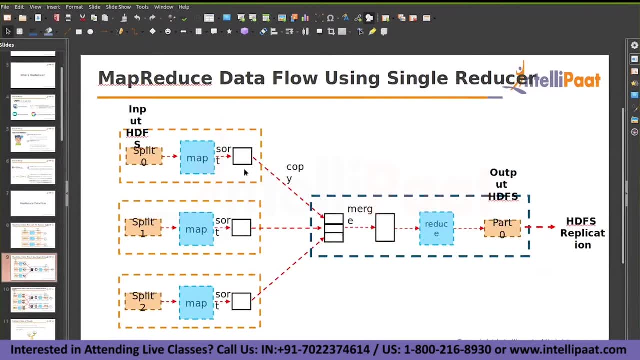 one file. for split two, you have a particle file. okay, so this is something we have. and for a single reducer, you can see there is split one, split, split, zero, split one, split two. it's running and there is a shuffle and sort operation which is going to combine and send it to the reducer and 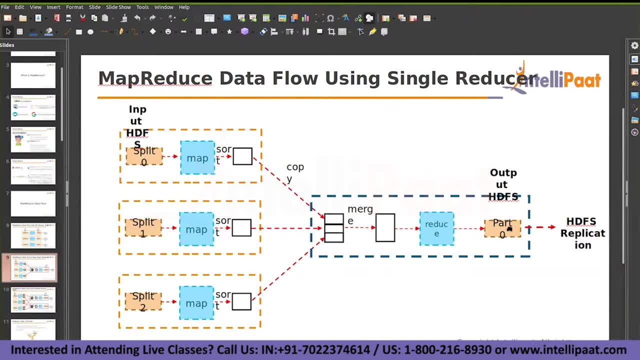 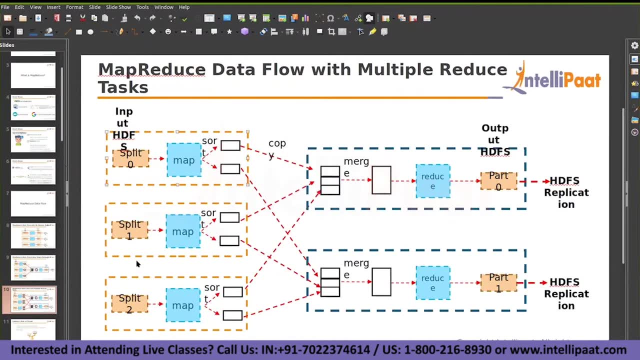 the reducer output will be sent to the part hyphen zero zero, zero zero, zero five. okay, and with multiple reducers, there is part hyphen zero file and part hyphen one file. so same split operation, split one, split two, applied to three different mappers. uh, the sort output will. 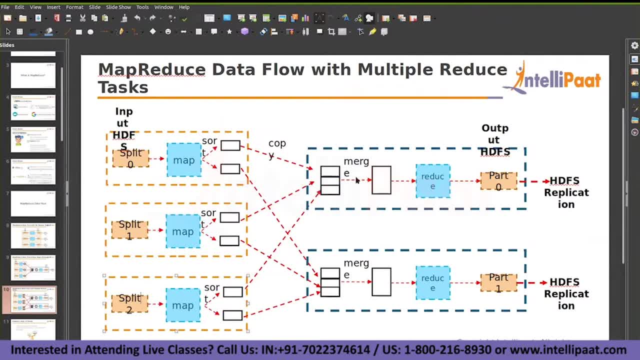 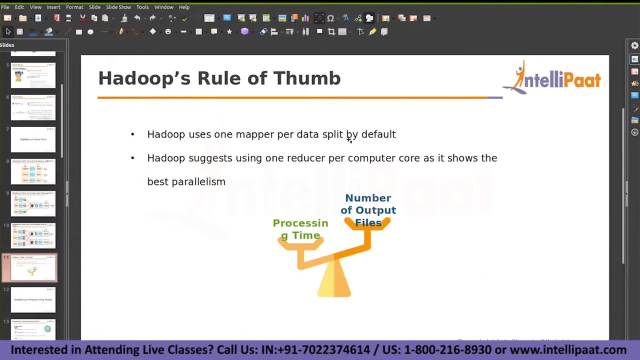 be sent to, depending on, uh, the different partitions. you'll be sending it to the reduced one and reduced, okay. so same thing, whatever we discussed. and then hadoop uses one mapper per data split. by default, hadoop suggests using one reducers for compute core, as it shows in this parameter. so there is also one more scenario, see um, we know. 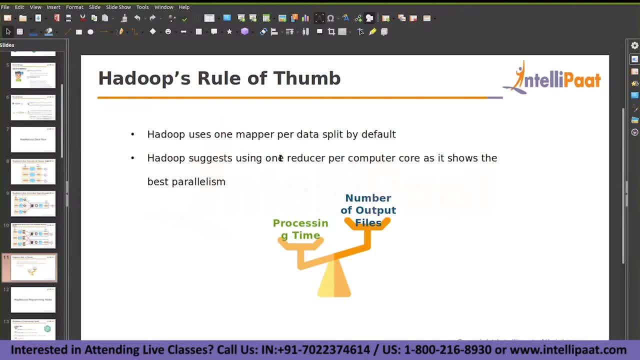 that in the earlier scenario, in the earlier example, there were four task trackers. right, there were four task trackers and you could run four mappers out of those four task trackers, four map splits. when you have a single node cluster, for example, you have defined a cluster. when you 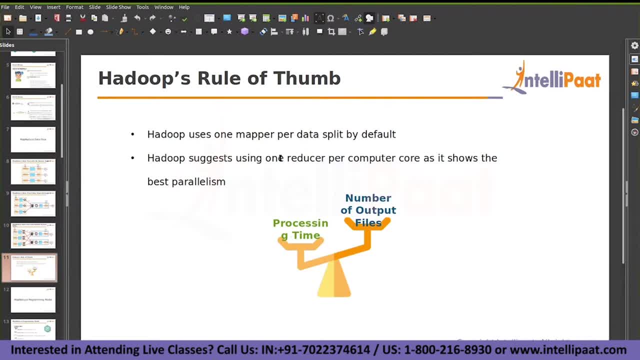 don't have any cluster at all. you have a defined a cluster which is a single node. your same mission will be map master, same mission will be slave name node, data node. the same mission will act as a job tracker and same mission will act as a task tracker. so in that case, for 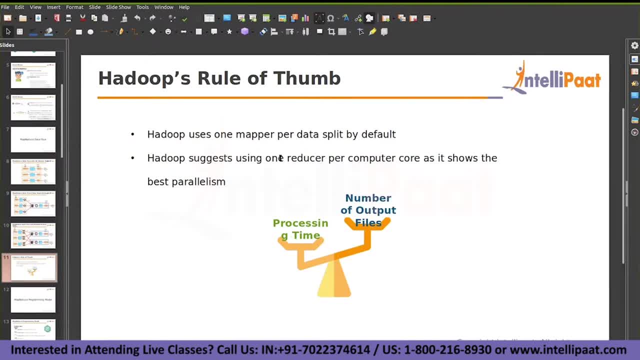 example, when the data is divided into three input splits. let's assume okay, so when the data is divided into three input splits, how many map splits? you would need three map splits. but how many task trackers? you have got only one task tracker. so in that case what happens is: 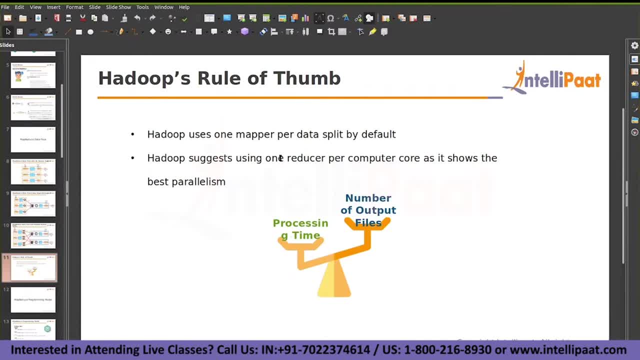 your uh single task will like. it will get executed first, the map task zero will get executed first, then the map task one will execute at second and then the map task two will be executed. okay, so same task tracker will be used to running multiple map tasks. okay, so that is one functionality we can. 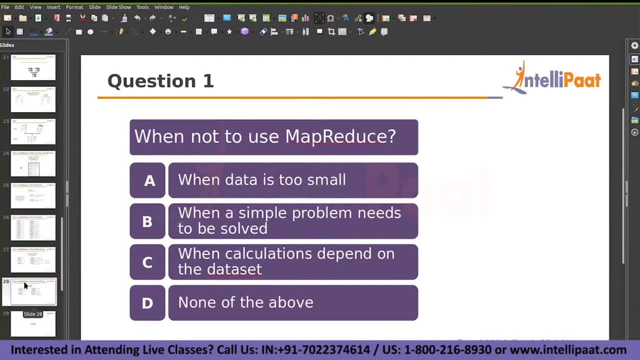 we can keep in mind. why not to use when? when? not to use map reduce, so when the data is too small, but this when a simple problem needs to be solved, when calculations depend on the data set. so when is when? is it not suitable to use a map reduce program when the data is too small? so we discussed: 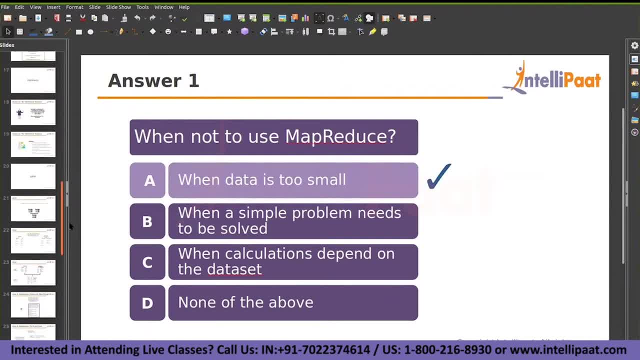 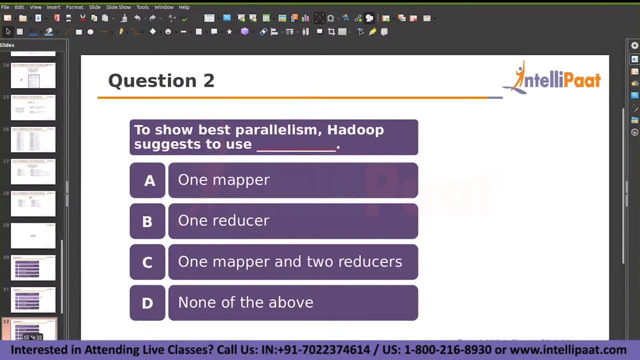 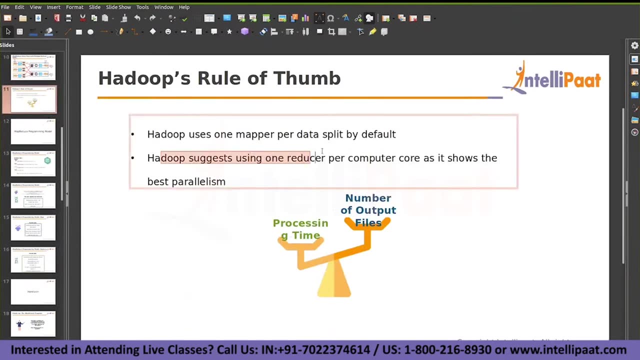 in the earlier slides. uh, the suitable scenarios are when the data is too large. okay, that's where you will be using map reduce programming and to show the best parallelism, hadoop suggests to use one right, so hadoop suggests using one reducer per compute as it shows best parallelism. so when you 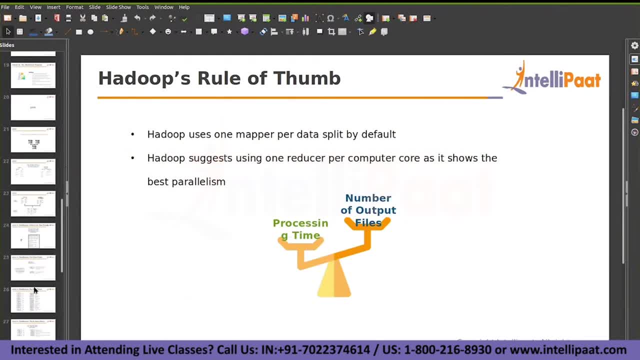 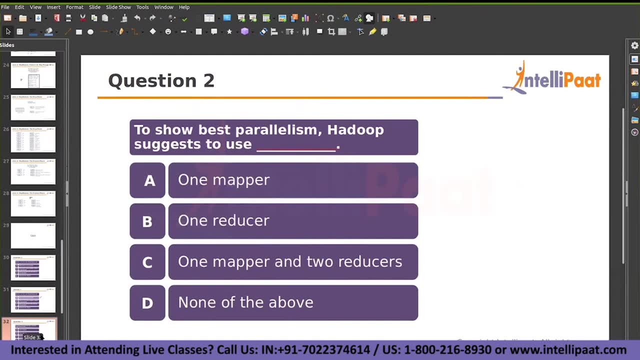 running and all the mappers shuffle out to one single reducer, right. so that's when your parallel jobs are getting executed. when you have two reducers, there are two tasks again getting executed, right, so two reducers as in. it has to run. it has to run sequentially, it cannot run parallel. 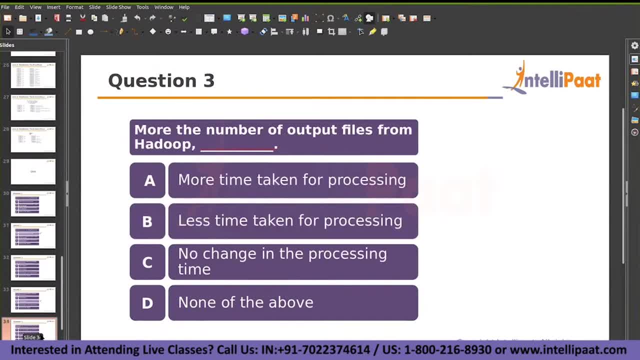 all the two reducers then, uh, more number of. more the number of output files from the hadoop. more the time taken for processing. less the time taken for processing. no change in the processing. what is it going to be? more the number of output files from hadoop. 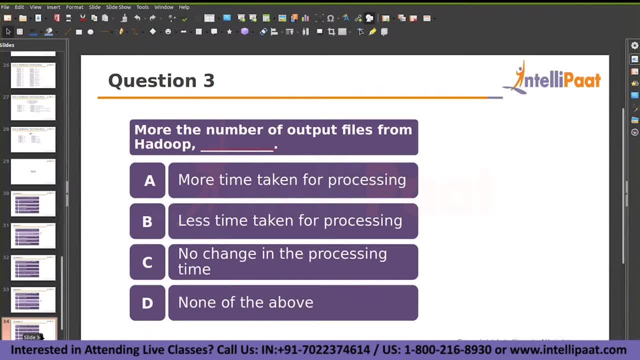 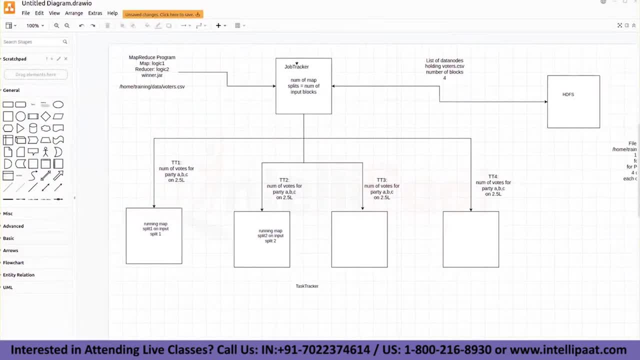 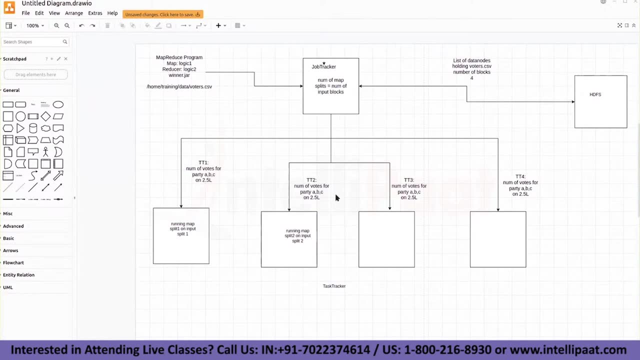 any other answers? why is it less time in the job tracker, task tracker scenarios, like we had in, like we had discussed in hdfs, what if a specific task tracker has failed. okay, so let's assume there is. there is this: task tracker 2 has failed and the task tracker 2 has failed and the task tracker 2 has failed and the task tracker. 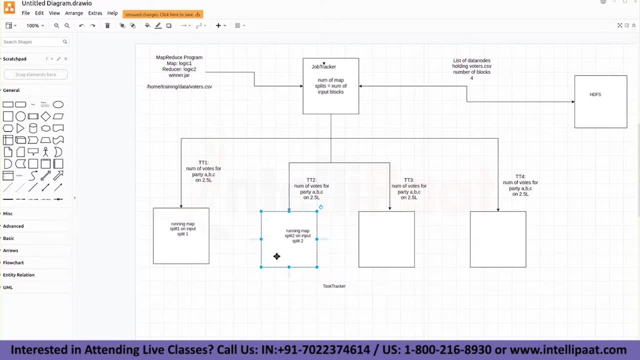 2 has failed due to some some hardware issue. what happens? what is the impact going to be? how is it going to be a loss of data, because it will be an impact on the result, but it will be an impact on a specific task alone, okay, on the task that is submitted to it. so map split: 0, 1, 2, 3. 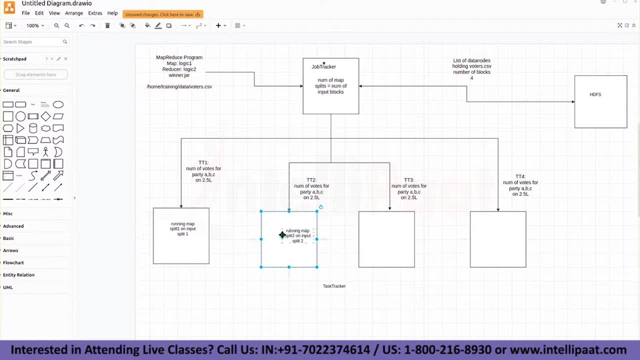 and 4 are submitted to task tracker 1, 2, 3 and 4.. if the task tracker 2 got failed, then only the task allocated to this task tracker, that is, map split 2, only will get impacted getting it. so there is also one more scenario. let me just discuss that first. so for example, I have 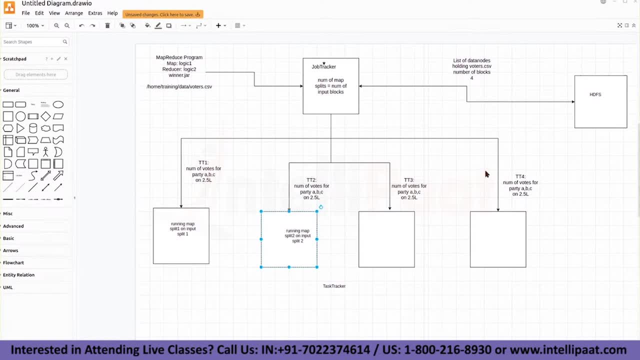 divided the data across all those task factors equally right? we we discussed about this scenario. all the task trackers have received 2.5 lakhs of records. uh, they are working on the 2.5 lakhs of data. so I'm running the same program on top of all these four task trackers. 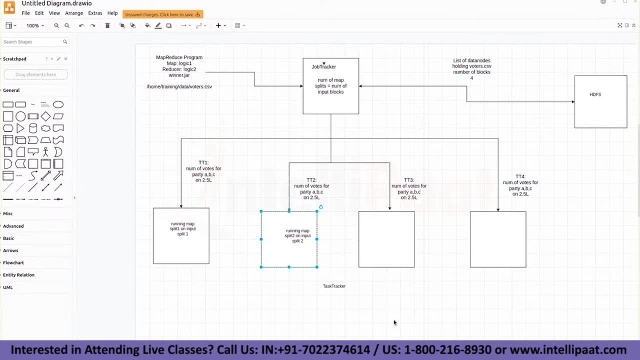 then, ideally, how much time does they take around around? equal amount of time they should be able to complete, right? so let's say, if this task tracker is completing it in two minutes, all the other task trackers are also expected to complete it in two minutes. that's the general. 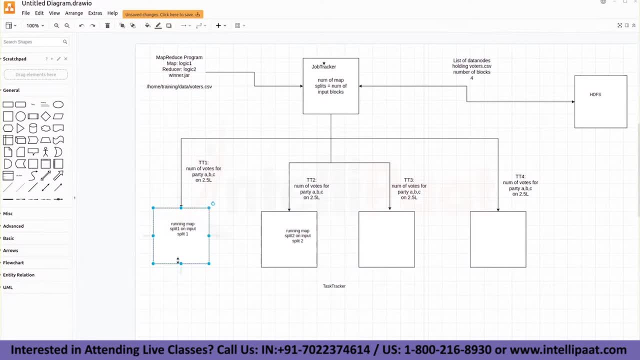 assumption. but what if? after and after the end of two minutes, if this particular task is complete? this is complete, this is complete and this is still running. so what happens in that case? so, at regular intervals, your task trackers are also going to send the intermediate task completion status to the job. 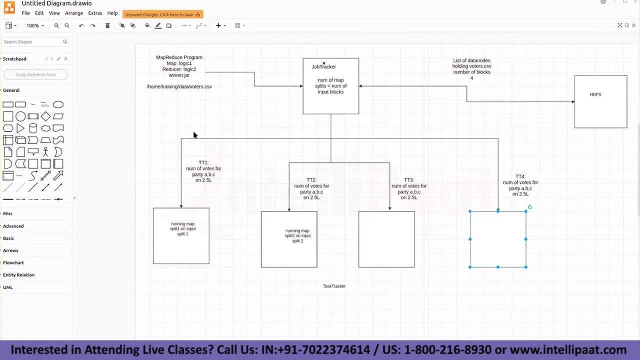 tracker. that means at: at the end of 30 seconds I'll say 25 percent of task is complete. at the end of 30 seconds I'm going to say some 20 percent of task is complete, some 20 percent, so 20 percent is complete. so this is how the intermediate status report of the tasks execution is also going to be. 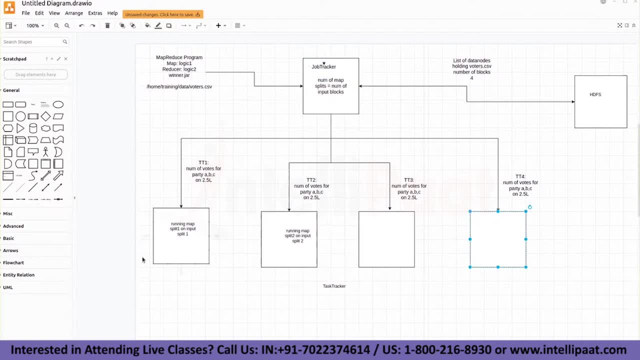 shared with the job tracker. so at the end of one minute let's say: this is completing 25 percent, this is completing 25, this is 25 and this is, let's say, two to three percent somewhere around like that. that means there is some issue going on with the task tracker code, some some some internal RAM issue or whatever. 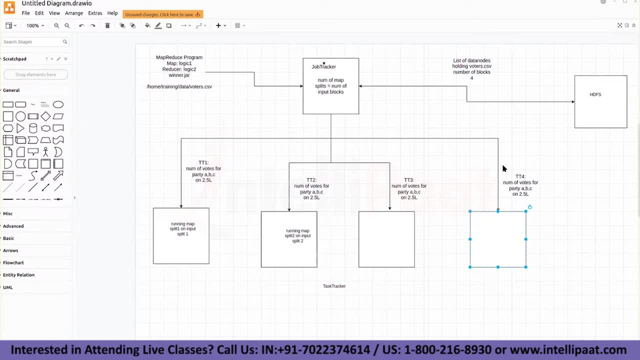 the availability of resources or whatever right. so in that case, what my job tracker is going to do is the same task, whichever is allocated. on top of this particular task tracker, there is going to be a duplicate task created and the same the. the duplicate task is going to get applied on the same. 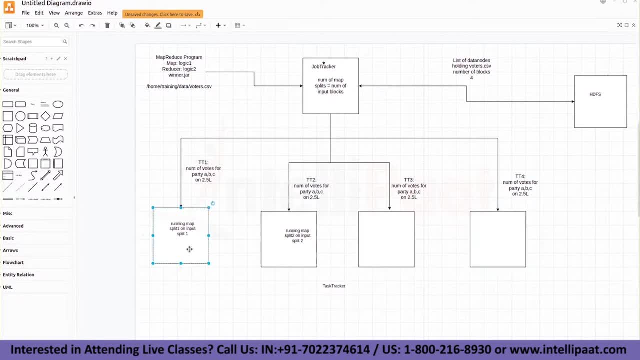 data block which this is working on. that means this is working on block one, input block two, input block three, input block four. so the task tracker four is taking more time than expected. there seems to be some issue with this particular task tracker and my job tracker will allocate another map split on top of the. 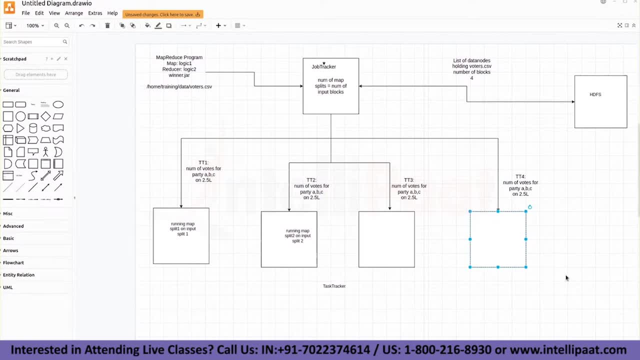 block four and it will allocate a new task tracker to run on top of this block flow. that means two task trackers are working on the same block of data and whichever completes first, whichever generates the results first, will be considered as a final copy. i mean will be considered as a 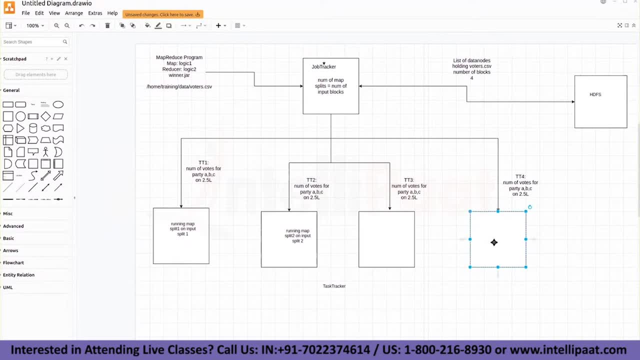 output. the other task will be will be kept on four getting it. this is a cumulative execution mode, we call it as. but that's just for the just for the theoretical understanding sake. okay, so by analyzing the intermediate status report, what is my job tracker job tracker doing? it is 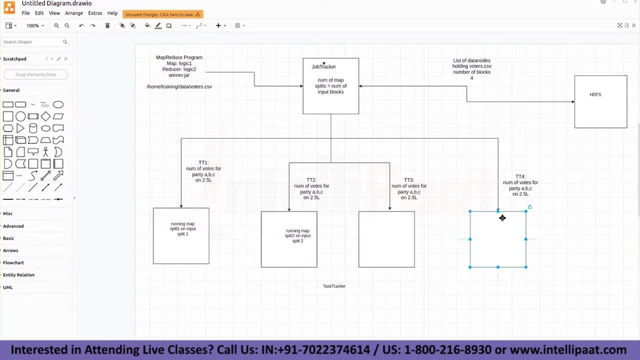 it is identifying the slowest running task tracker and it is allocating by by looking at the slowest running task tracker, it is allocating a duplicate task tracker to run on the same block of data getting it. so it's just not waiting for this task tracker to complete. but 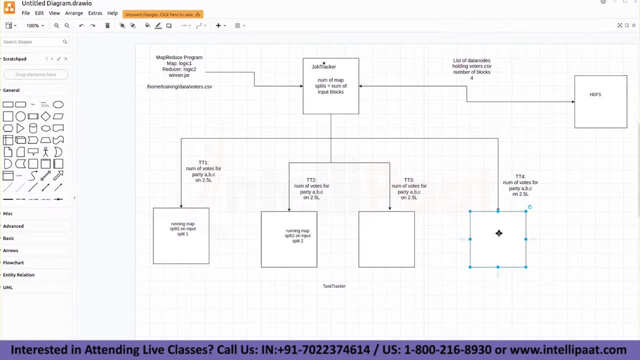 it's actually taking a proactive measure to make sure that this will not impact the final execution flow, right? so there cannot be a scenario where it will just wait for this task tracker to complete. these task trackers have completed the task in two minutes and this they are just waiting for this. 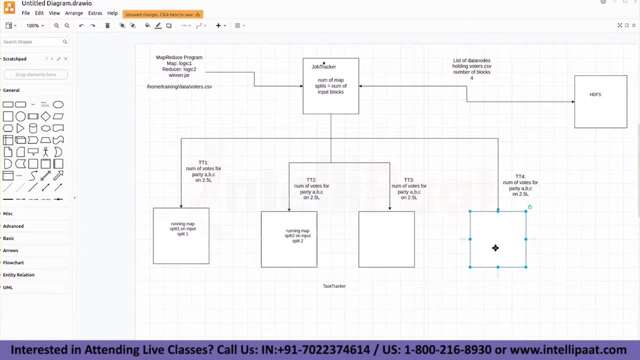 particular task to complete. this has taken 10 minutes, let's assume. so what is going to happen? the entire job execution time is going to get hold right. so, to avoid that, at intermediate stages itself, at the initial stages itself, it's going to identify the slowest running task tracker. 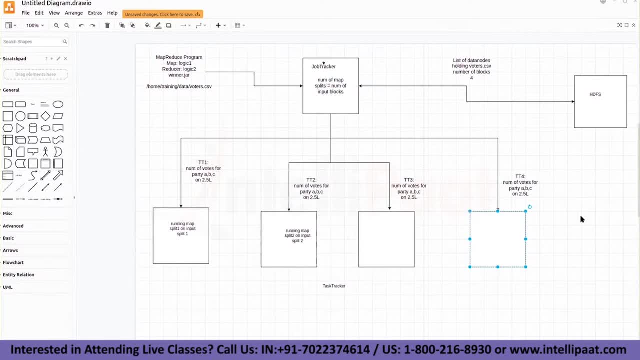 and it's going to allocate a duplicate uh task tracker to run on the same block of data and whoever results, whoever send the results first, will be considered as a final copy. the other uh task tracker activity will be terminated. okay, the other task tracker duplicate activity will be. 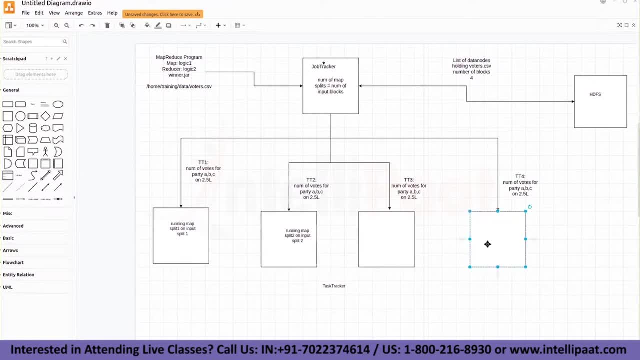 terminated. if the other task itself is sending the same uh, sending the output, uh, quickly then, then then that itself will be considered as a final copy. okay, so what if i don't have the availability of this task trackers? i don't have the task trackers available. what is going to happen? 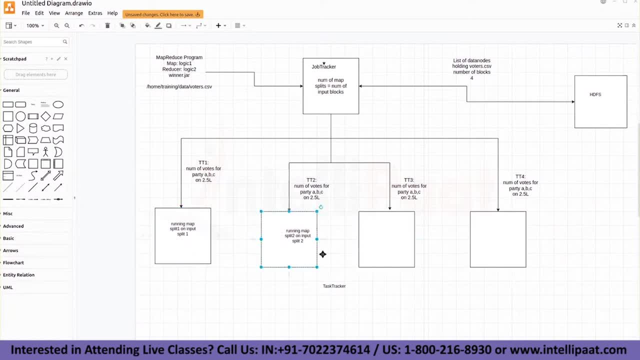 after finishing, after successful completion of all these task trackers, existing task trackers- it will pick any one of the existing task trackers to run on the same block- same block of data. it's going to parallelly run on the same block of data so this lowest running machine will at least have some backup on um on using the other machine. okay, 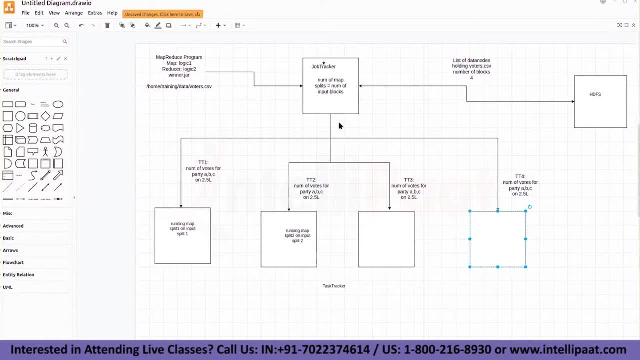 so whichever is going to complete first will will send the result as usual. it's all. it's all going to be dependent on the resources understood. so this is one way of doing it. and now you understood that when, when there is an issue with the task tracker. so the impact is. 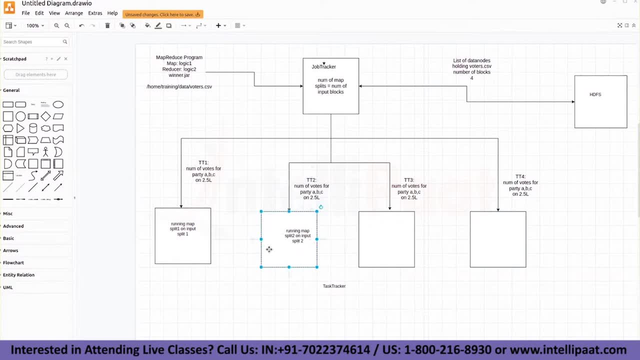 going to be only on the task that is allocated to this task tracker and your job tracker will identify this issue and it's going to run a duplicate task. it's going to run and it's going to allocate on another class tracker to work on this particular job splitter. now map splitter. 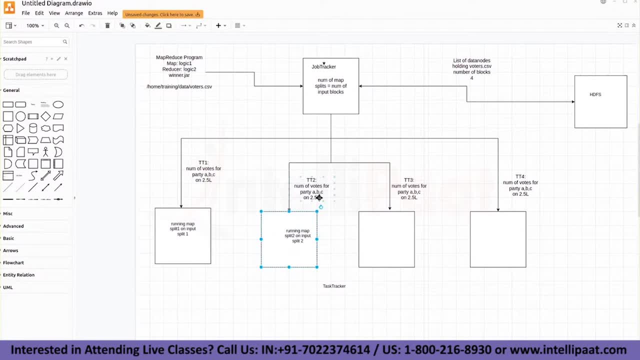 right. so that is the impact it's going to be. the impact is only going to be restricted to this particular task alone. and what if the job tracker itself has got failed? the impact is going to be for all the jobs, for the job that has been submitted now. 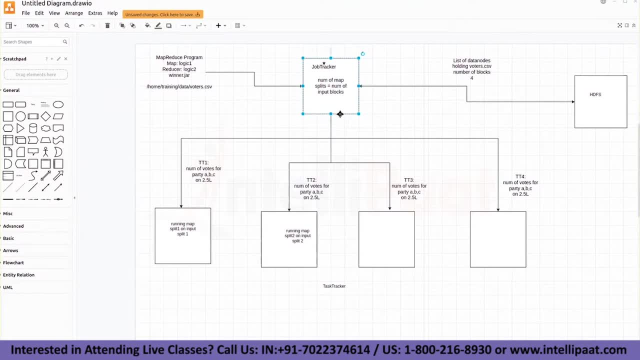 and for also the other jobs that are going to get executed right. so this also is a single point of failure. so when the task tracker or when the job tracker is down, then the map reduce engine is considered to be down, yes or no. there are no other uh backup and the entire map reduce uh. 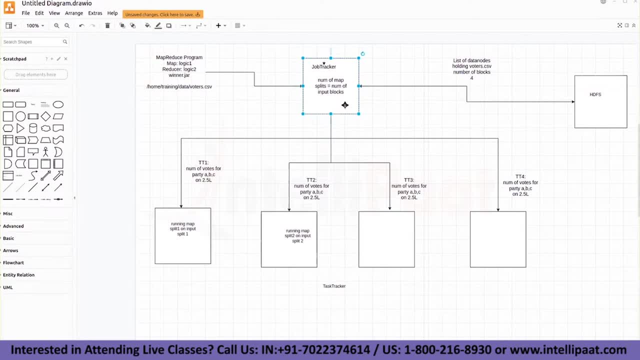 functionality is being kept on full until the job tracker is brought back up again getting it. so this is one issue, and whenever there is a map reduced program that is running in, okay, there is. there is a map reduced program that is getting executed, let's assume, and the first map reduce, 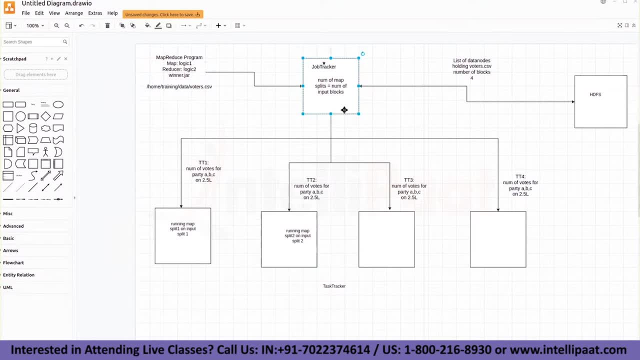 program. when i've submitted it it has identified that it would need four task trackers to run. okay, allocated four task factors. what if there is another program that got submitted at the same time getting it? so there is a map map reduce program submitted, submitted first. one MapReduce program got submitted. now the job tracker got the results. 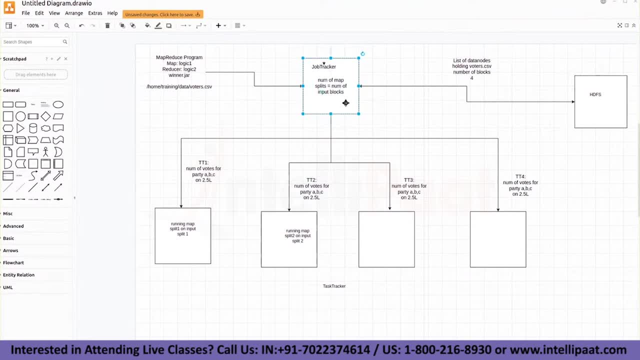 from the HDFS. it's analyzed the program and it has decided that it could need four task trackers out of the available four task trackers. I have allocated all the four task trackers to the same machine. let's say I have one more. let's assume I have five task trackers but I have 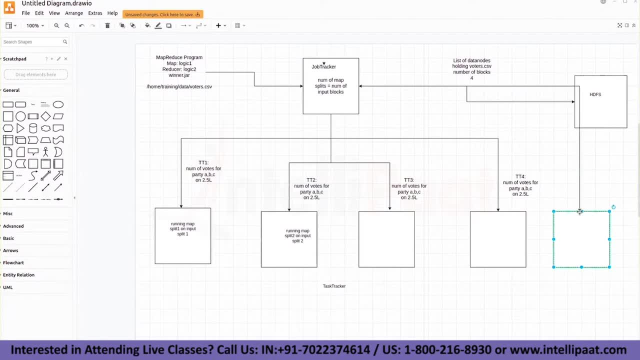 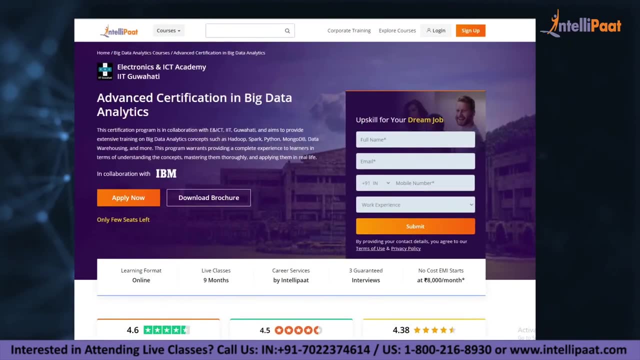 allocated four to one single machine. only just a quick info, guys. if you want to make a career in big data, then Intellipaat provides an advanced certification in big data analytics by ENICT council, IIT Guwahati. it is taught by IIT professors and industry experts with more than 10 years of. 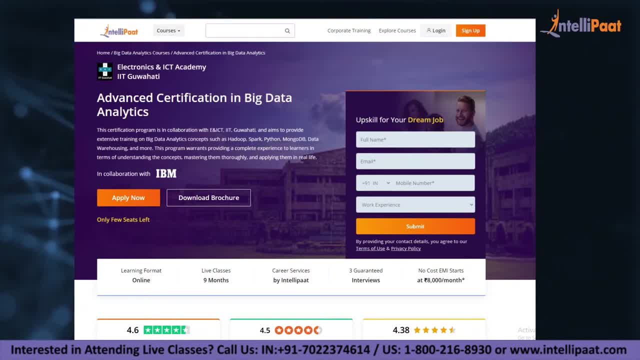 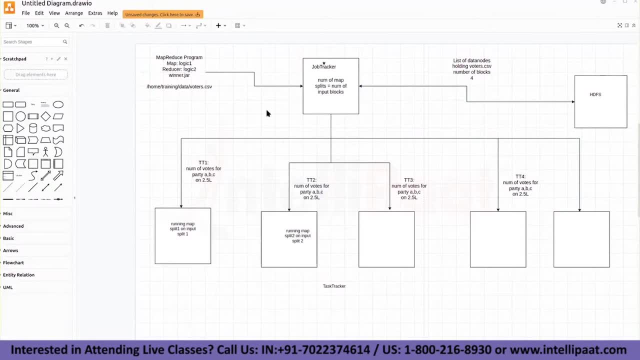 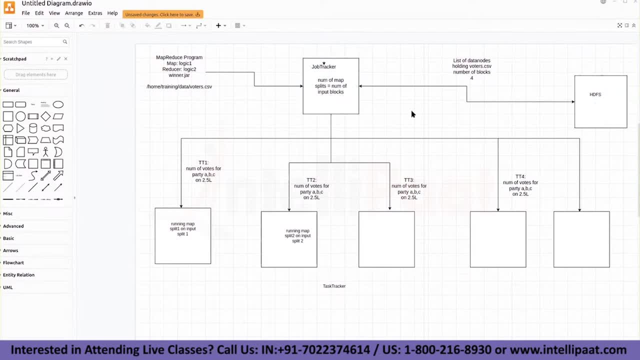 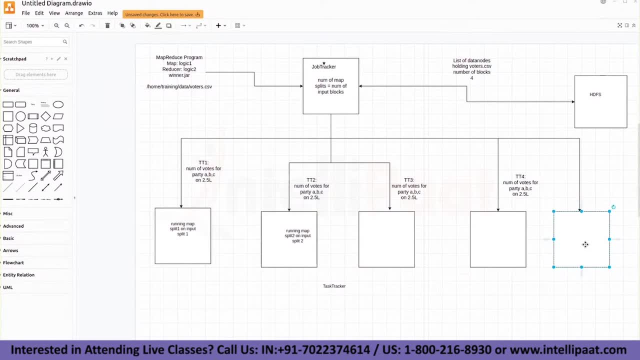 availability. I have only one task tracker available, so that means this job two has to wait for job one to complete. only then your task trackers will get freed up and then your next job can start executing. so that means ideally, uh in in. in ideal scenarios, it is only one job that is getting executed, yes or no? not more than one jobs are allowed to execute. 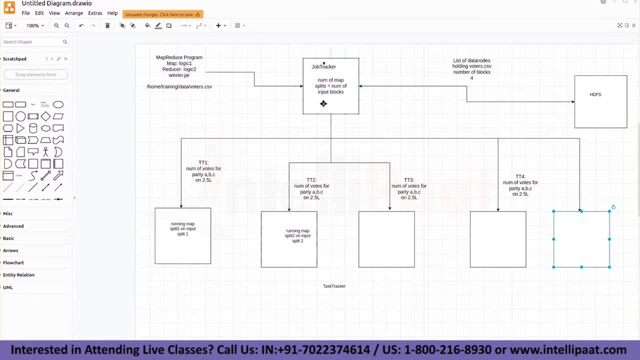 depending on the resources again. but how well is it managing the resources if? if there is a scenario where, um, the first job would have taken only three resources and the second job would have only taken two resources, okay, I could have managed. I could have managed- the first job to take only three. 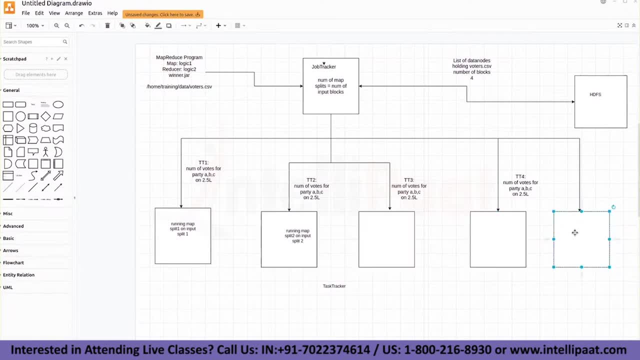 resources and the second job. I could have managed with the two resources, considering both of the jobs are running parallel. at least both of the jobs have been allocated some resources and they are. they are at least running in parallel. so that scenario would have been possible. but that feature is not available with the existing. 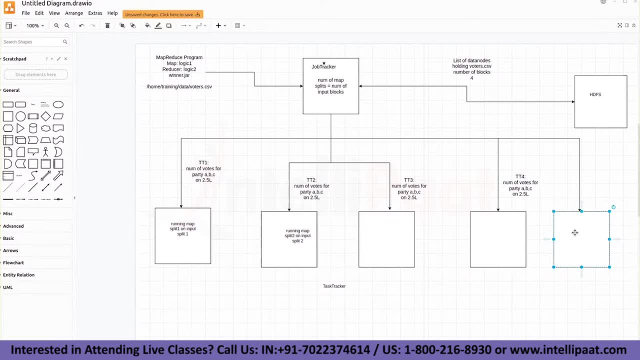 job tracker functionality. it's in the MapReduce generation one. there is no parallel job execution process or there is no dynamic allocation of resources, proper maintenance of resources- to multiple MapReduce jobs that are getting submitted. so whenever the resources are available, it is allocating them in bulk and when the new job comes in, you are just. 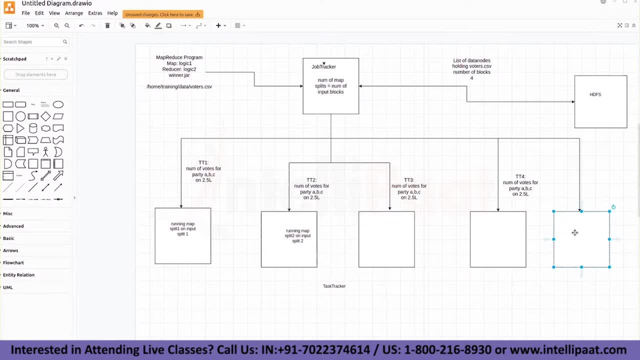 it's just just making it to wait for the other, for the previous job, to complete what I could have done if there is a better management. I could have allocated only three for the first job and kept two on spare, and when there is a new job coming in, I could have allocated 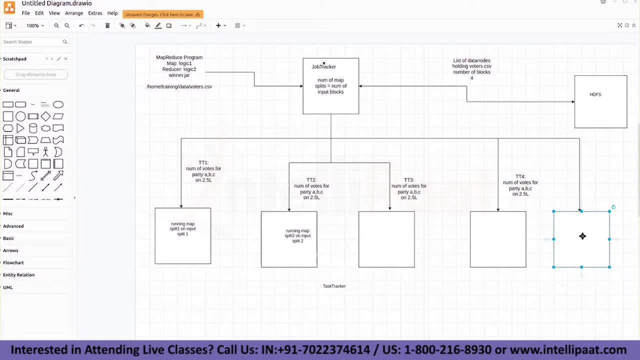 these two for the other two for the other, second job. so this resource management are the failures of the jobs. there is no recovery and all these issues have comprised for the version two of MapReduce, that's what we call it as a map. uh yeah, MapReduce version two. which is the yarn? yet another resource negotiator, the major. 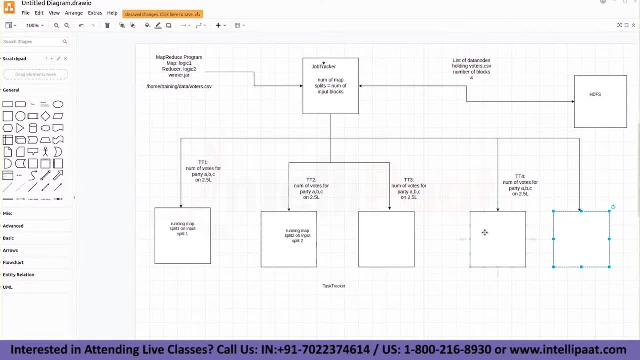 concentration of the MapReduce version two is on the resource management functionality. okay, and also whenever a job is being submitted, whenever any MapReduce job is being submitted, what is the first activity that we are doing? we are converting the input data into a key comma value pair, but what if my input is in the format which? we are converting the input data into a key comma value pair, but what if my input is in? 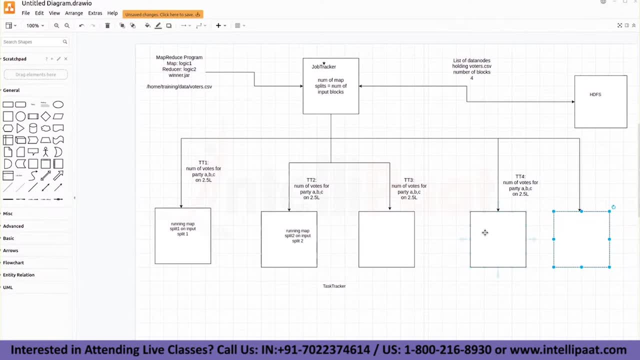 the format which which cannot be converted into a key comma value. we know there is a sequence file even though there is a text format. we know there is a file input format of different, different formats. we know, but what if the data is in in a format which you cannot convert it into a key? 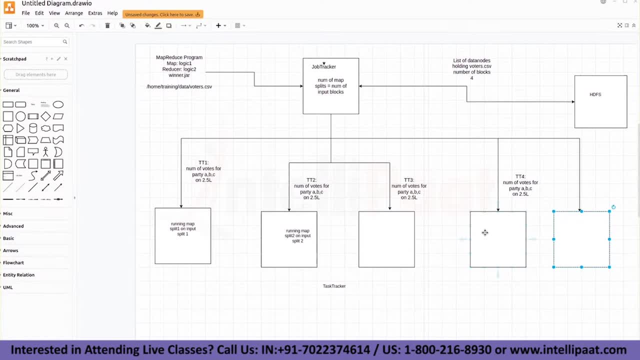 comma value, some graph data or some some, some video data or whatever, whatever the data is- is not getting converted, or if you are not able to convert the data into a key comma value pair, the is in such a format, then your MapReduce framework will not be able to work on that kind of datasets. 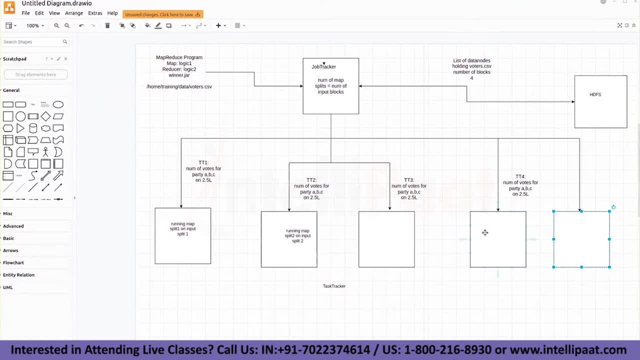 So this is also one of the drawbacks. So for your MapReduce version one to work, your data has to be converted into a key comma value pair. Your program only understands the data which is converted in the format of a key comma value pair. If the data cannot be converted, then that kind of 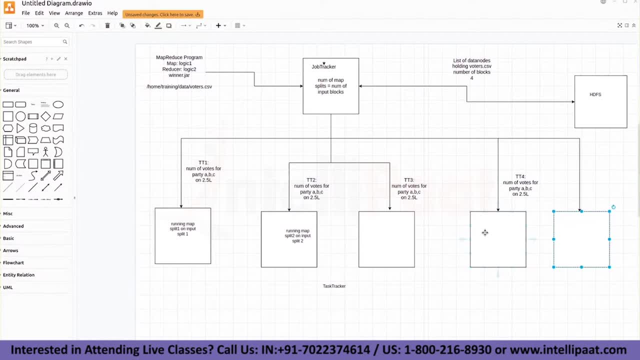 datasets would not be able to process using the MapReduce engine. So first thing is the resource management. well, resource management is not properly done. and the second thing is with the data conversion: key, comma value, pair conversions. These are all some of the challenges that we have. 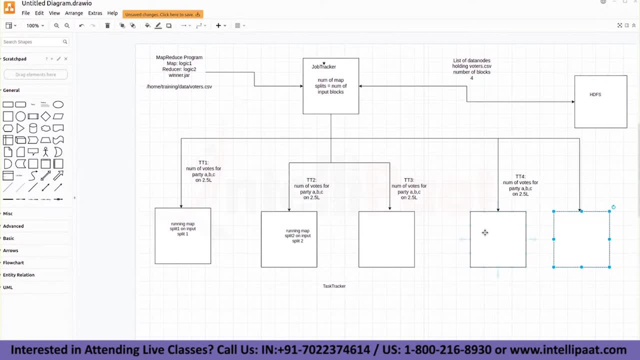 with the version one which have which have got into the version two yarn- yet another resource negotiator. So in version two we have resolved all these pending issues. So the major problem was what? like we don't have a backup for the job tracker. If the job tracker is failing, all the 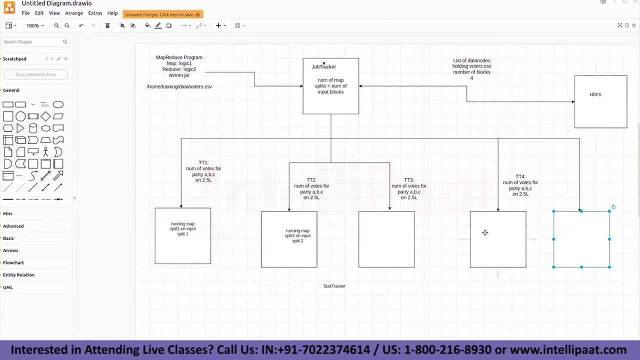 jobs running on that particular job tracker is going to get failed, right, There is no backup and the resource management or the- what else? the key comma value pair conversion. So all these, all these problems we had and that is why we are going to the next version of MapReduce engine. Clear guys, any questions? 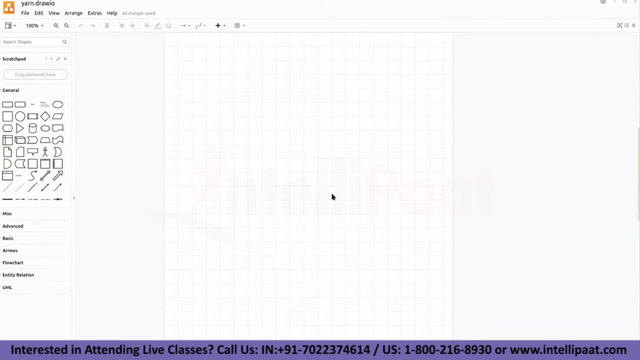 That's master slave architecture. I'll just quickly give you a recap. There's a master slave architecture. Master is going to be your job tracker. where, as the slave is, slave machines are the task trackers right. So whenever you create some MapReduce program and you you convert that into a jar file and you 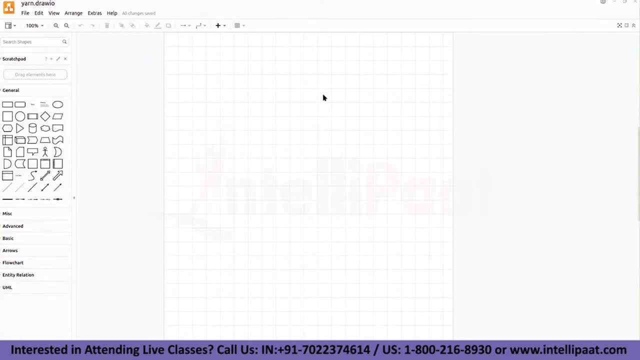 provide the input path. so all these things you'll be submitting as a job to your MapReduce engine and what your job tracker will do after you submit a job. your job tracker will receive those details like that's a master and it has. it is a point of contact for all your MapReduce. 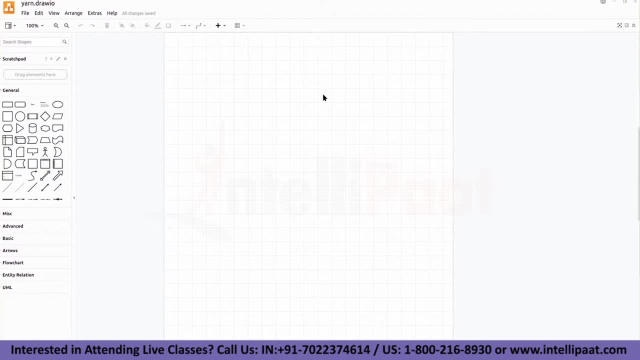 related um executions. so your job tracker will understand, will will analyze the job that you have submitted and it also will check the input path so to to check whether the input path is valid. it has to interact with the hdfs cluster, with the name node to be specific. so, job tracker, 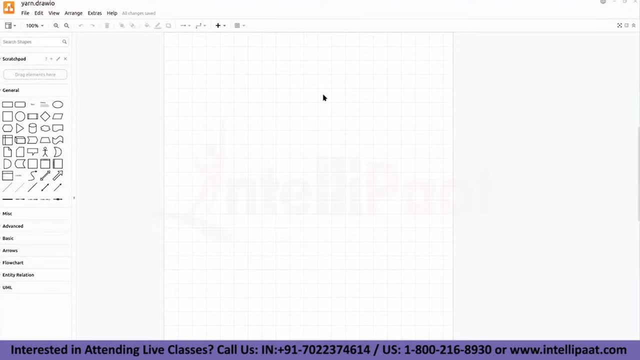 will interact with the name node to identify whether the specified input path is a valid input path. i mean, do you, do you actually have that data in the hdfs? so if the data itself is not available, that's that's going to be a failure. i mean that's going to be a written message saying: 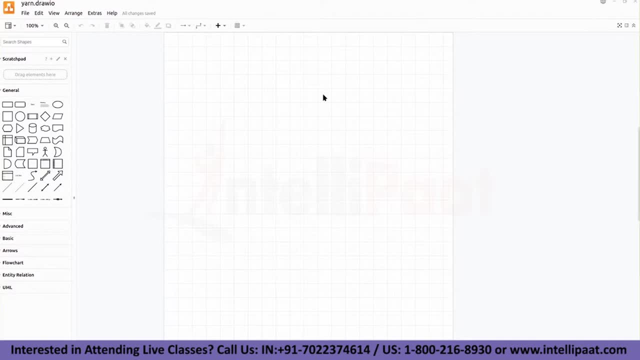 that the input data provided is not not valid. so, if you have the input data in the hdfs, what is the next step? what are we going to do? what is your name node doing after? after getting a request from the job tracker? first step, first step is to check whether the input path is valid. 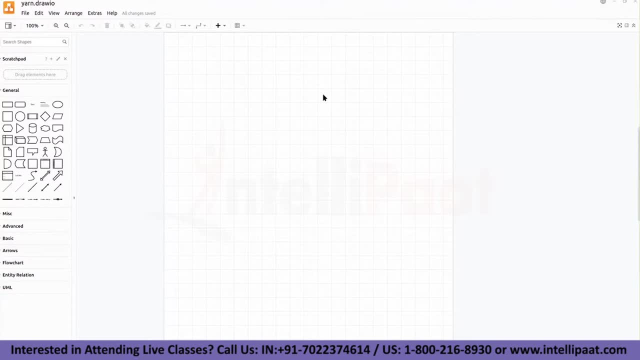 second step is to provide the number of blocks. the data has been written into right, so how many blocks it has been divided? that number of blocks will be shared with the job tracker. so, depending on that information, what is the next activity that your job tracker will do? yes, anyone. what is it? 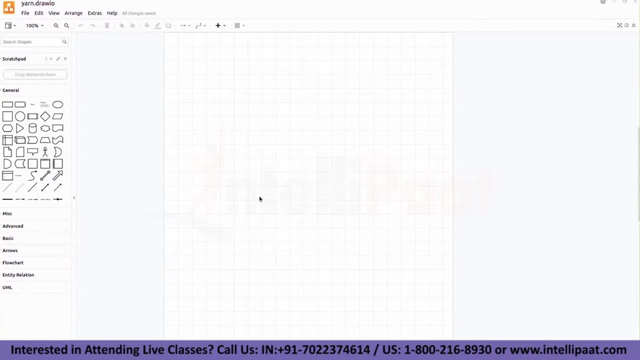 going to do so. we got the block level information: how many input blocks. the data is stored from the hdfs. so after you receive that information, your, your job tracker will divide the number of map splits right. so your map task has been submitted. your map task has been submitted. a reduced task has. 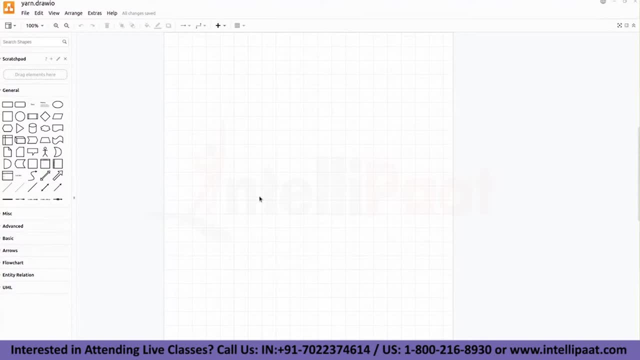 been submitted as in the form of a program. so your map task has to be duplicated, has to be split into multiple. i mean, it's not. it's not being split, but it has been. it has to create so many number of duplicates that are equal to the number of input blocks. 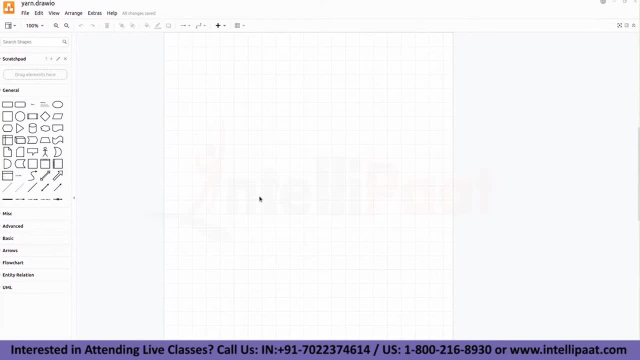 so after you create this duplicates of map tasks, multiple copies of this map task, each and every task, is going to get get allocated to the input block. okay, so your your task tracker will will pick a map task and you it will, it will start executing on so and so. block of data in hdfs. 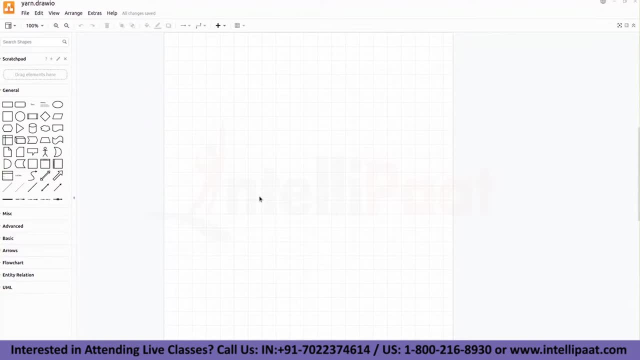 agree with this, everyone. so now i have a question. let's say i have only three task trackers available, okay, so i i designed my system. my cluster is not very huge, so i designed my system. i have only three task trackers available and on the input, block input. 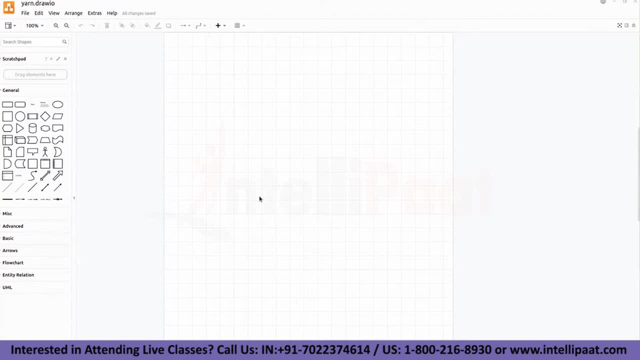 side, on the hdfs side, i have some hundred blocks of data written. okay, so my input file has been divided. i've been divided into hundred blocks of data, so, ideally, how many map tasks it has to execute and how many map tasks it has to create- hundred- it has to execute. so i have only three. 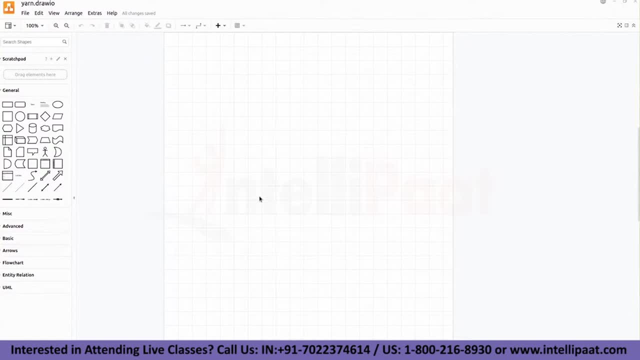 task to create and for hundred. for executing this hundred map tasks, how many job trackers do we need? we would need 100 job trackers, ideally, but how many do we have? it does not mean that we we have only three job trackers. so what's going to happen now? so how are this hundred map tasks gonna get? 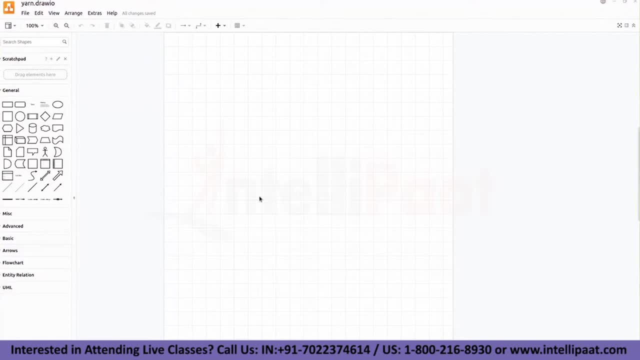 executed on top of this three job trackers. so that means the first three will get executed, then in second three the cumulative uh execution will be executed in the third set of three will be executed. right, so that's how we will be dividing uh. you, you submit these three map tasks at a time and then then uh after execution of: after. 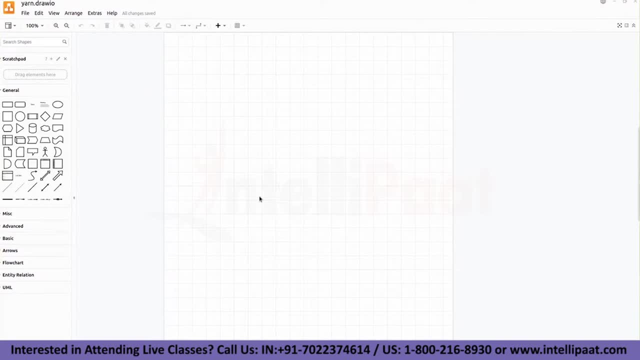 completing the execution of these three. you, you, you submit the next three slots of it. okay, so something like that, you will, you will, you will try and execute. and this number of in map splits is is not like, not exactly equal to the input blocks, but it is actually greater than or equal to the 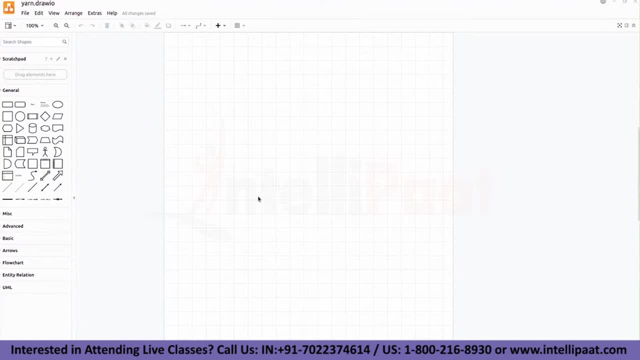 to the input blocks. okay, so it's. it's going to create some um backup copies which would be at least one or two more than the actual equal number. okay, so it's going to be greater than or equals to the number of input blocks. fine, so now we have executed it. so, after this map task has been, 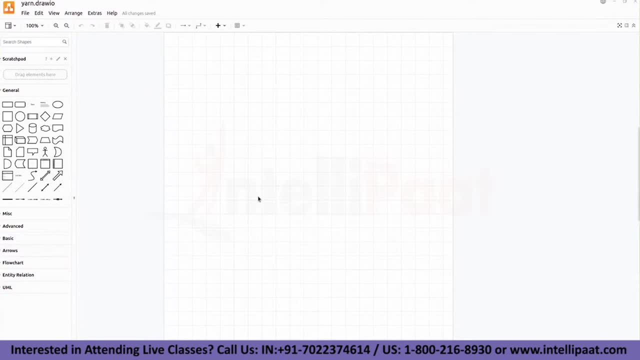 submitted to the job task trackers, they'll start running on the input blocks, they'll execute the data and they'll generate the result. so, after you generate the results, what is going to happen? there is a component called as shuffle and sort within within the map: reduce framework. 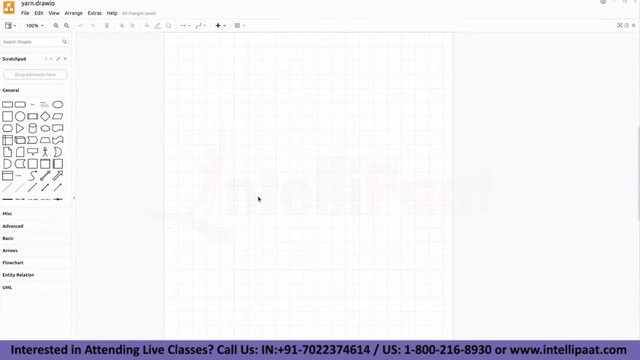 what is it going to do? it's it's going to make sure that all the map tasks- map tasks- have completed the execution and all the map tasks have provided the result right. so it will just, it will just kind of be a checkpoint where it will wait for all the map tasks to complete. 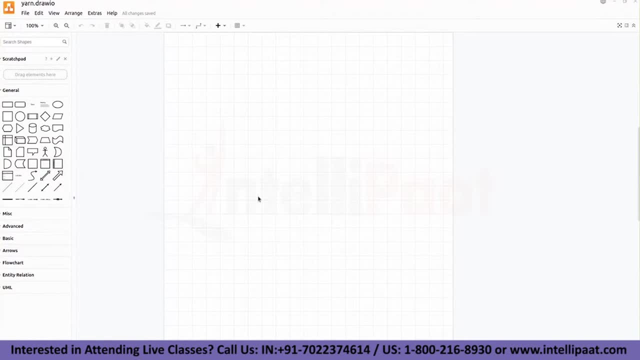 the execution. okay, so after all the results have been received, it's going to shuffle a and sort the output of all the mappers and it's going to send it to a red user for accumulation, for aggregation of the map results. So, depending on whatever the logic you write, 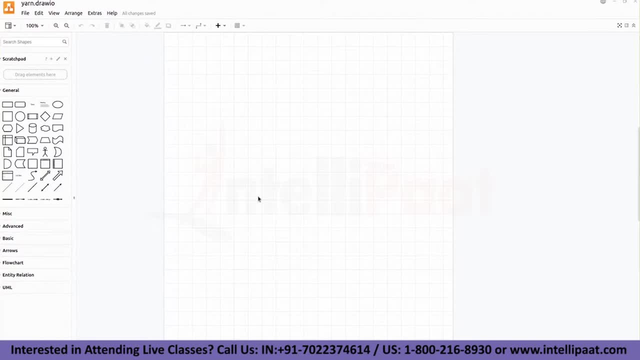 inside the mapper and inside the red user. it's going to break, it's going to execute it. Then after that, the final output will be returned to the HDFS location. again, We know how the file is being created. So now we've also seen the theoretical flow. 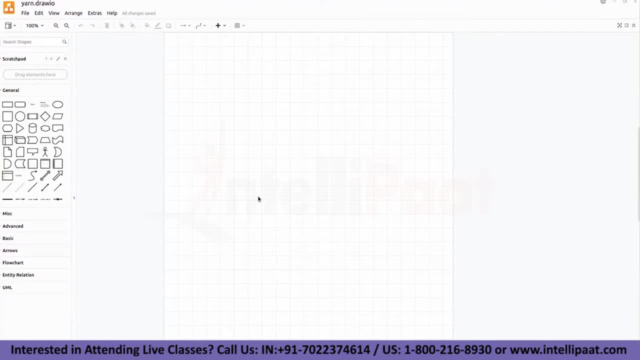 of how the word call program gets executed. We've seen the split function and default allocation of one by as a key and a value right. So every input or an output for this mapper and reduce has to be in the format of a key and a value pair. 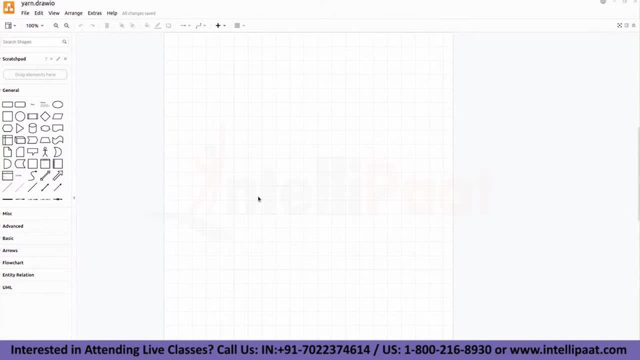 So that's why we kind of convert this into key comma value pair. So in between map and reduce you also have a component called as combiner. So what is this combiner doing? What is the operation of a combiner? Anyone? 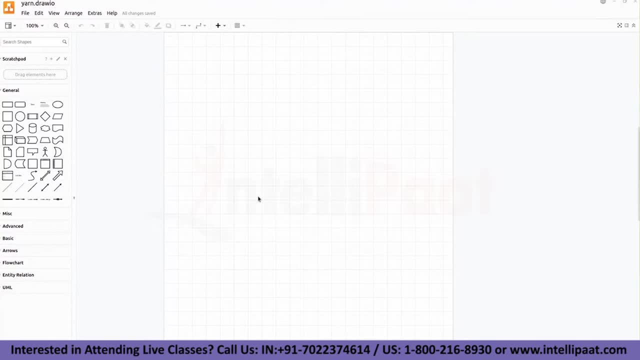 Yes, remember, okay, Yeah, so it's something which is doing a reducer operation within the mapper itself. So see, whenever we ask what is a combiner, our answer should be something like it's going to be, it's going to perform a reducer operation. 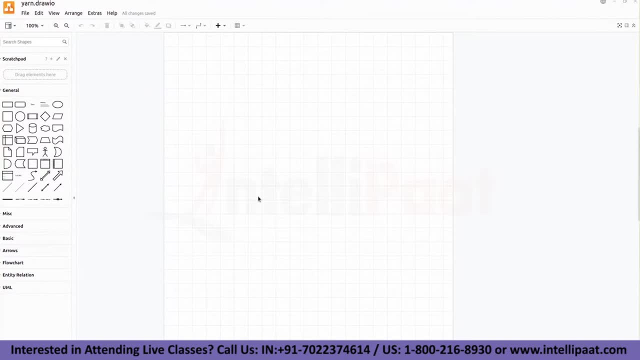 It's going to perform a reducer functionality within the mapper itself, within an individual mapper itself, right? So it's not always going to be identifying a duplicate key and merging both of them, because in word count we've identified: okay, there is welcome and welcome. 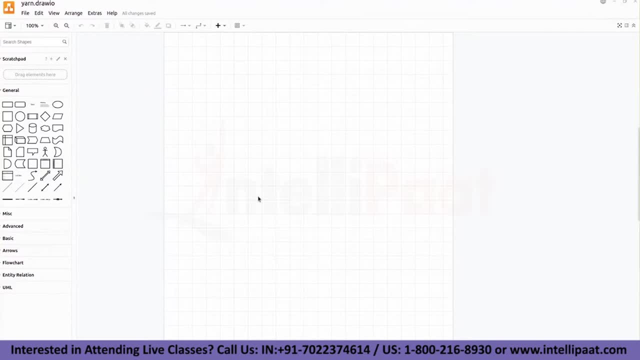 We merged both of it and we made it two, But in general, it's going to be a different functionality. It can be anything right. So what is that we are ultimately doing is we are using the reducer functionality. So, whatever is going to happen inside the reducer, 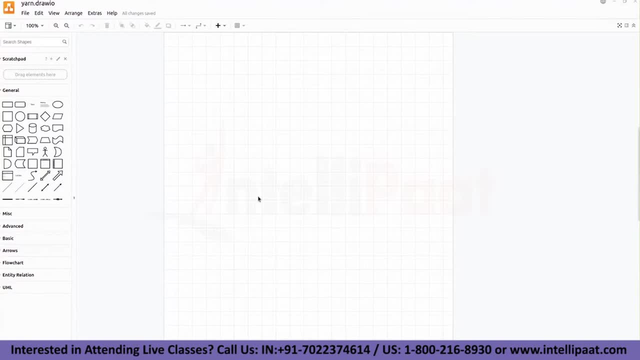 you just read that method, You just call that method and try and execute that functionality inside a mapper, Yes or no? So instead of running it on all the mapper output, we are running it on a single individual mapper output. So we are not writing any logic for combiner. actually, 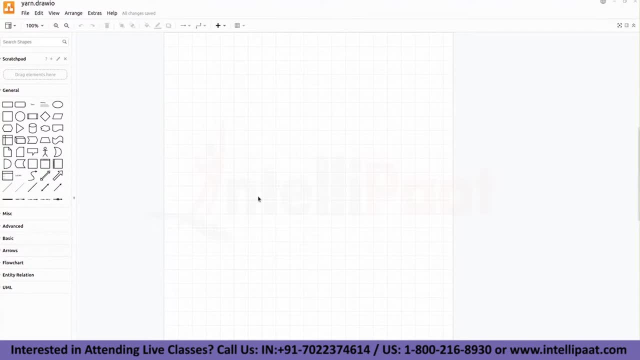 So it's the same functionality as that of a reducer, but the only difference is we're going to execute it inside a mapper, right? So your combiner is something which is a reducer which is going to run inside an individual mapper. So this is how the definition is going to be. 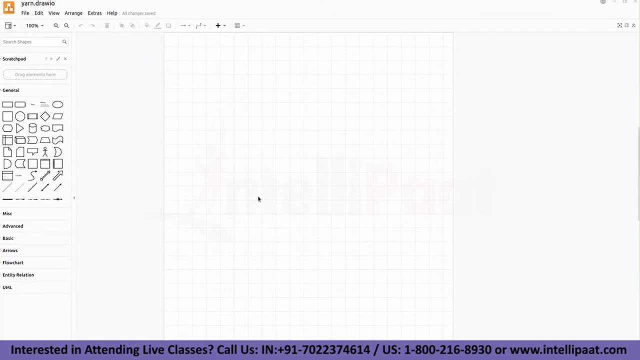 I mean, this is how the explanation has to be, So we are not going to talk anything about the duplication or anything like that. okay, So combiner is a reducer, itself is a reducer, but it's going to run on an individual mapper output. 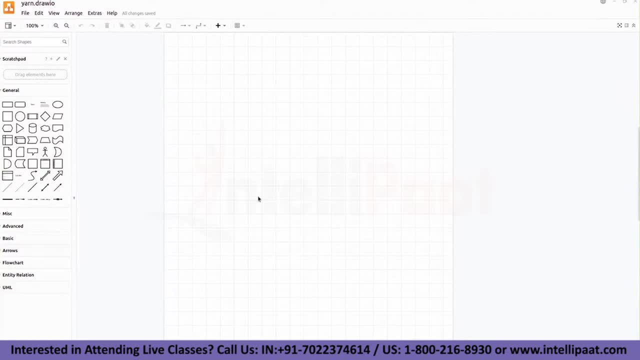 rather than running on the all the mapper outputs. okay, So then we have discussed about the partitioning, how the custom partitioning and dynamic partitioning can be done. So custom partitioning is pretty much. you don't write any logic to it. 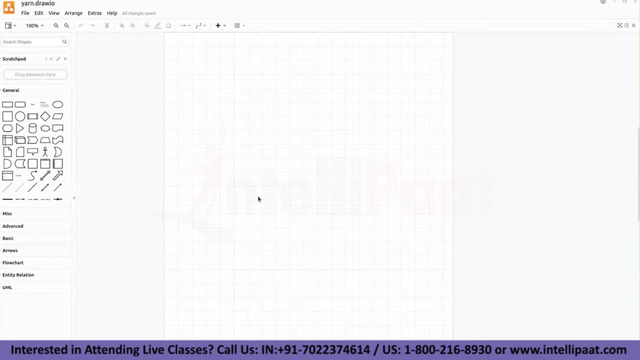 You don't define any logic to it. You just specify the number of reducers so that it will write the data onto different output files, depending on some dynamic logic. I mean it's all within the framework. Again, you don't have any control. 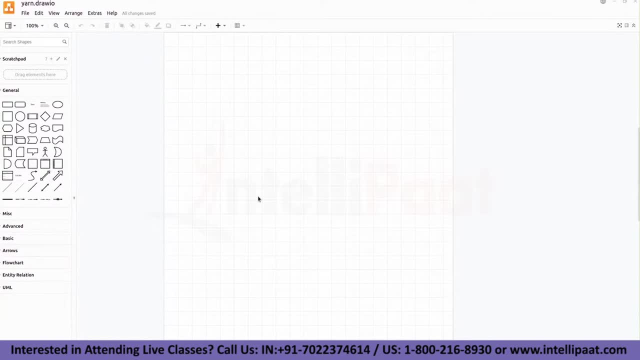 on how the data is being split and being written into multiple data files. But in custom partitioning you can specify. you can specify what is the logic for individual mapper. you can specify what is the logic for individual mapper. you can specify what is the logic for individual mapper. 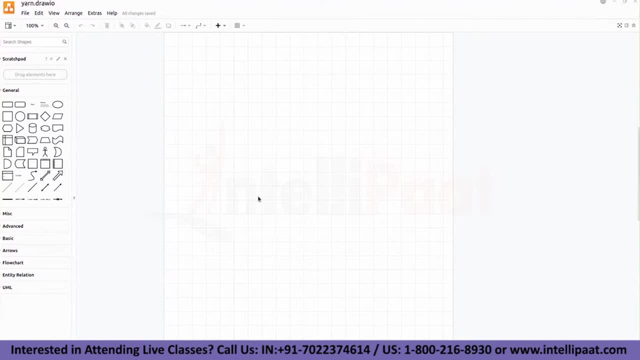 you can specify what is the logic for individual partitioner. Okay, so if this logic is satisfying, you send this output to this particular file, And if this logic is being satisfied, send this output to another file. something like that. You can specify or you can segregate. 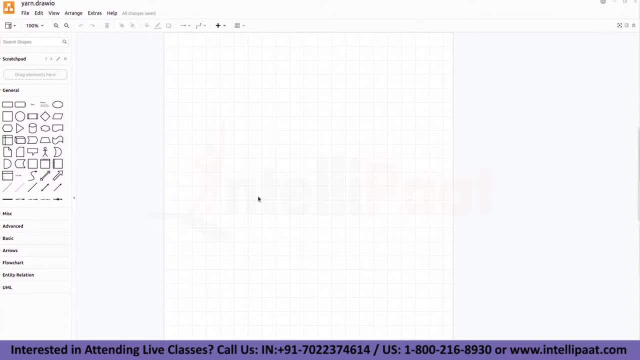 or you can aggregate the data and send it to different output files, correct? So that's the partitioner logic we've discussed, right? And also when it comes to the limitations, we have not handled anything related to the resource management, pretty much. 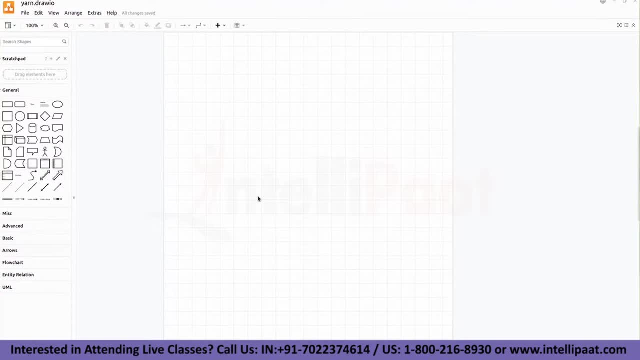 So, like we've seen, when there is already a job that is being submitted and when there is another job that is getting executed, I mean that is getting submitted to the job tracker. in that case, what happens? It will just wait for the first job to complete. 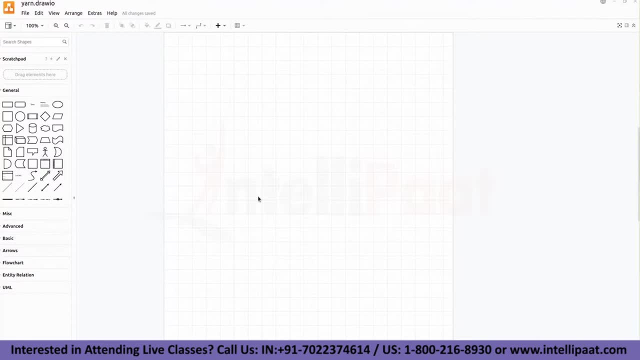 rather than try and accumulate the resources, try and properly allocate the resources. It is just waiting for the job tracker, It is just waiting for the previous job to complete. So there is no proper resource allocation done for this And, moreover, there is no backup for your job tracker. 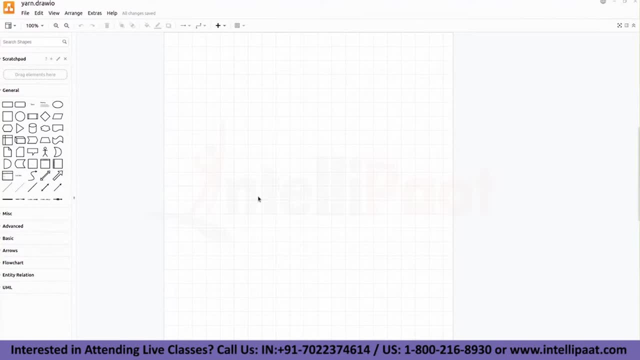 When there is a job tracker failure, it's kind of the entire system failure is maybe we're gonna consider right, So yeah. So let's see how all those limitations have been overcome on the YARN side, the latest version of MapReduce. 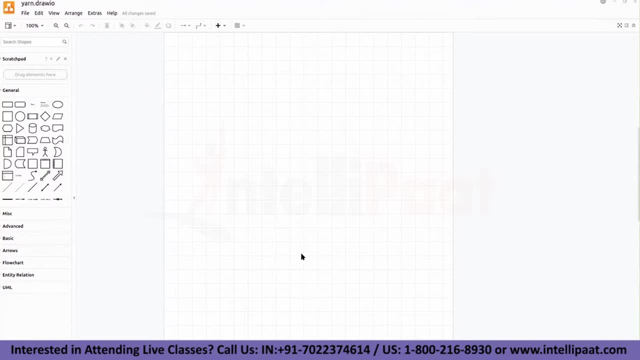 the updated version of MapReduce 2, we call it as a YARN right. So YARN is nothing but a MapReduce 2.. In HDFS, similarly, we have seen HDFS 1 version 1 and HDFS version 2, right. 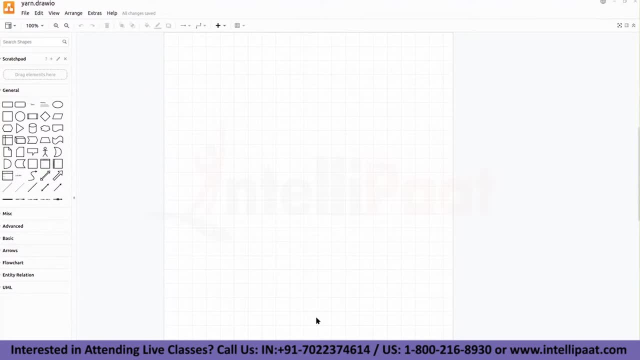 So in version 2, we had active and passive name nodes and nothing else. nothing else changed actually there, But in MapReduce there has been a lot of change in terms of the architecture. okay, So now let's start with the similar diagrams, okay. 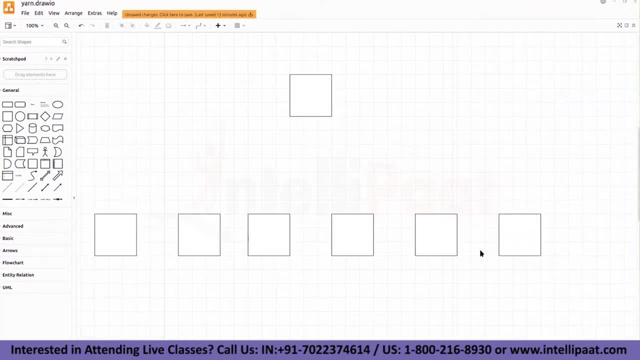 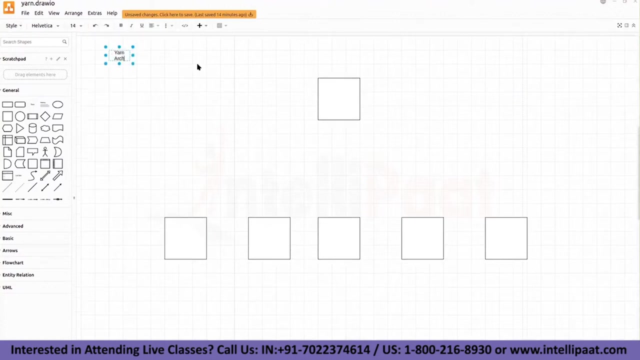 So let's put one more right. So this is your master and slave architecture again. Let's write some text to it, YARN. And there's also one more limitation that we have right. So everything inside a MapReduce application has to be converted into a key comma value pair. 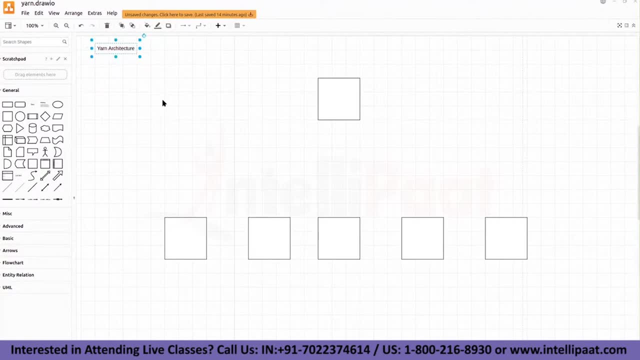 regardless of whatever the input we are dealing with, right? So there is no other way of dealing with the data. So, regardless of whatever the input, is you kind of convert that into a MapReduce program? always, right? So that is also one of the limitations that we had. 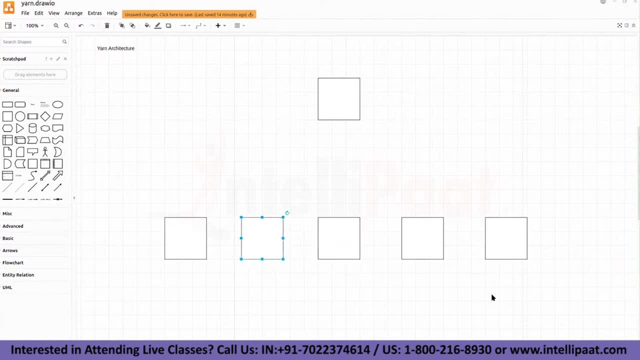 with the MapReduce functionality. So now? so inside this YARN architecture, like I said, there is going to be- this is going to be- a MapReduce- I'm sorry, master and slave architecture, whereas the master is called the resource manager. 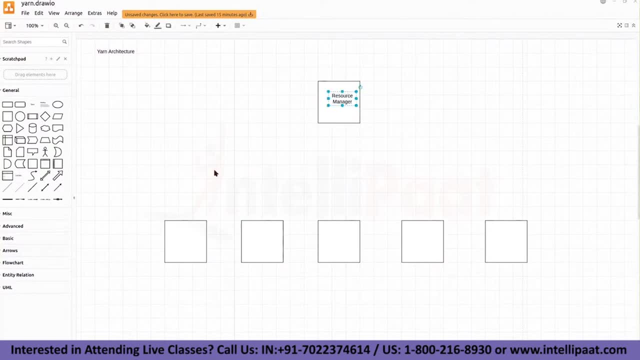 Manager and the slaves are called as the node managers. okay, So is it visible, the text, All these are the node managers. So I'll tell you the reason why I'm writing it, for all These are all the node managers: one, two, three, four. 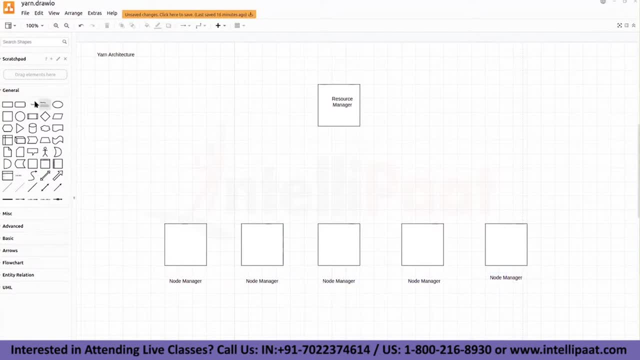 and five. So inside the node manager we have something called as an application master and container. So let's say, let me write, let me put it this way: So application master is one and there is something called as a container as well. right, 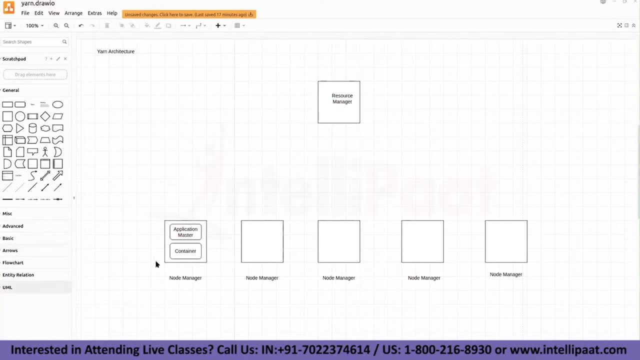 So inside every node manager, for that matter. okay, So inside every node manager we have an application master as well as a container. So now, starting with a job submission, right? So whenever there is a job that is getting submitted, 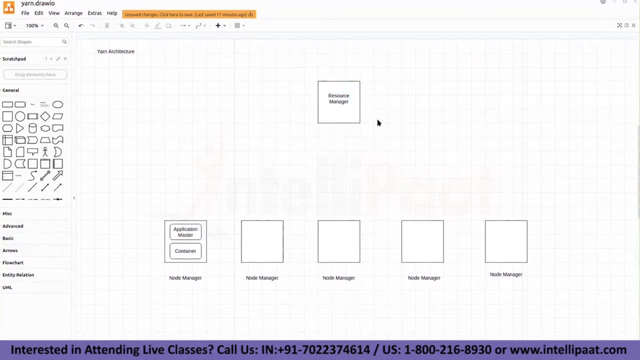 what is going to happen. So in MapReduce we have been calling them as jobs, right? So every JAR program that we submit, every set of program that we submit, we consider this as a job and we consider the individual components of it. 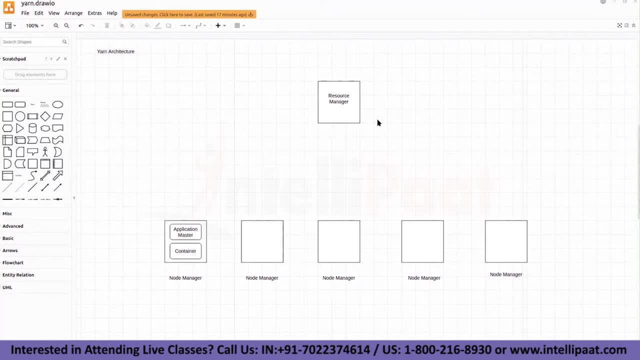 the small modules of it as the task, But in YARN architecture we call them as an application. So we say there is an application one That is getting submitted, Application two that is getting submitted free. So because the reason is like if it is a job, then it's going to be a MapReduce job, okay. 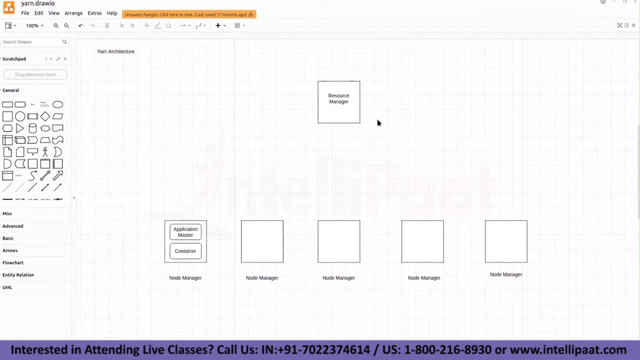 So in YARN, what are we dealing with? We are dealing with other ways of execution as well. It's not just a MapReduce way of execution, but it's also running on an other. it also deals with the other sets of execution modes or other sets of data sets. okay, 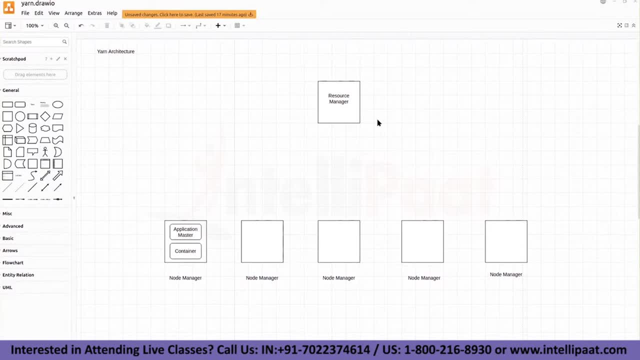 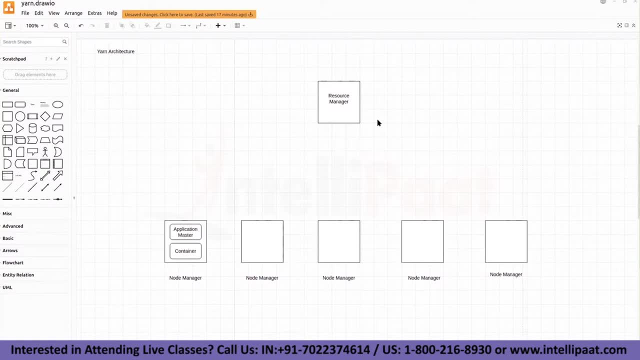 In YARN, as we are dealing with other applications also, other sets of programs also, we call this as an application. So I'll tell you the reason why. See in MapReduce: what did we discuss? We discussed about the scoop job. 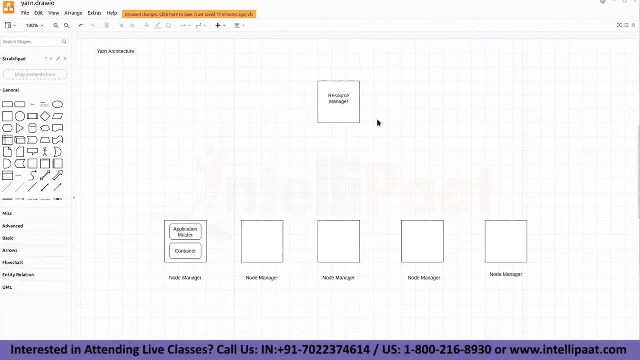 We discussed about a hive job, right? So whenever you write a select star from in hive, whenever you write a scoop import program or whenever you write a pick query, So everything, everything within the, So everything within the Hadoop ecosystem, is going to get converted into a MapReduce. 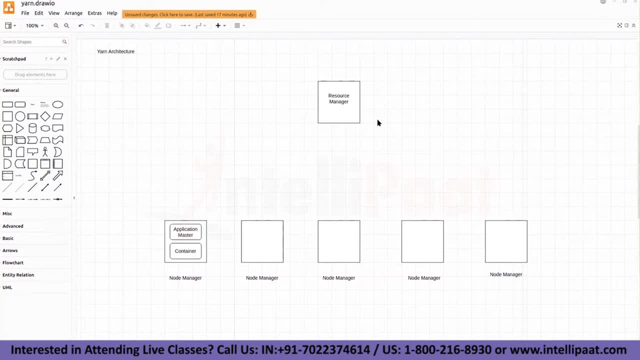 program. So it actually doesn't matter what query we are writing. okay, So what query we are writing is only for the user convenience. So in hive we have been provided with an SQL kind of a framework wherein we were able. 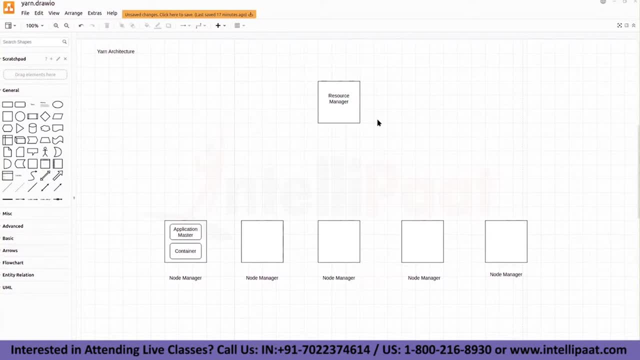 to write the SQL, simple SQL statements within terms of select, star or any joins, group, buys and all. And in pick there is another Latin script And in scoop there is another format of commands. So all this, all this, syntaxes might be different, but when? whenever you submit them, whenever. 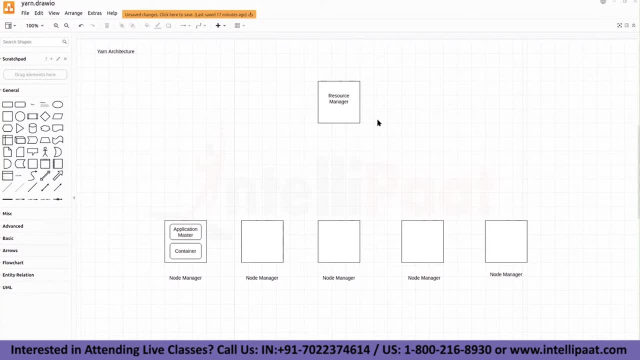 you execute them, it's again going to be a MapReduce program at the back end that is getting executed. okay, So that's the. that's the agenda in the MapReduce framework, in the earlier versions of the MapReduce framework. 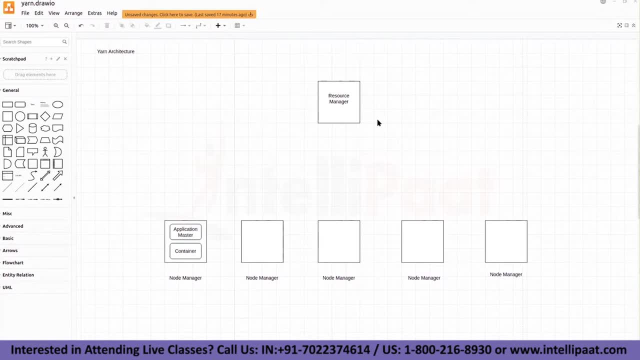 But now in YARN, everything is is kind of an individual application. So now, now you have hive, that is again a MapReduce program. But there is a Spark. let's say, okay, So there is a Spark application that is getting submitted. 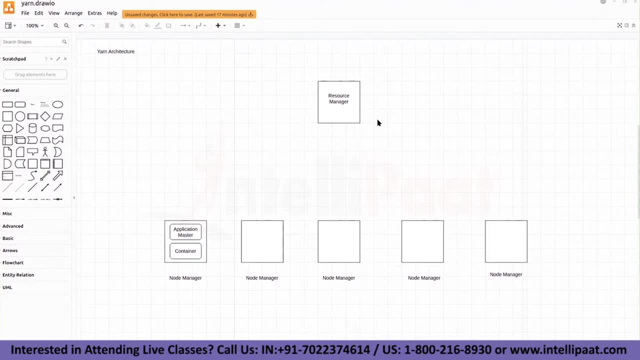 There is a Spark job that you want to submit, that you want to execute. So if Spark is built on top of YARN system, then when you submit a Spark application, that's that's actually an application It's. it's not going to convert the data into key comma value pairs. 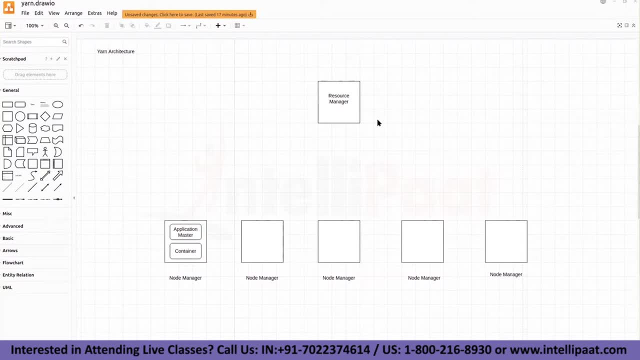 Getting it, It's. it's going to execute as a proper application. It's going to execute as a proper task. okay, So if it is related to MapReduce, Then we can call it as a job. If it is related to something else, then we have to call it as an application. 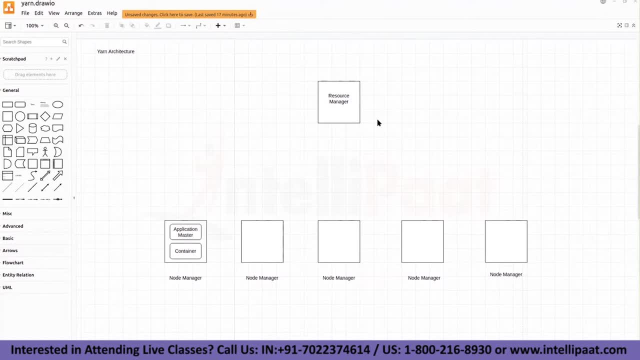 So YARN is something which is going beyond the MapReduce. I can say in simple terms: okay, So earlier it was only restricting to this MapReduce way of execution, But YARN has taken it to a next level wherein it can- it can execute other other applications also. 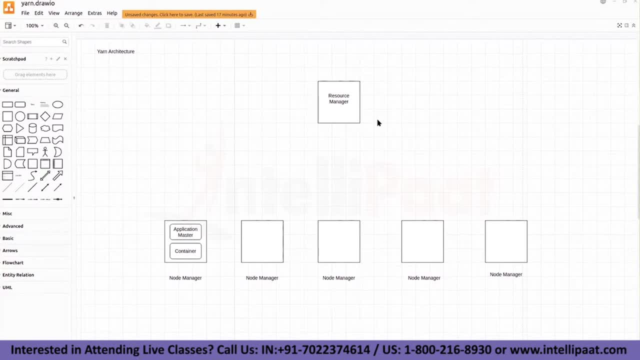 You have a Spark application that it can run And you have some kind of a Flume application that it can run Or some Flink application, It can run anything. anything other external systems beyond the Hadoop ecosystem. That's what I mean to say, okay. 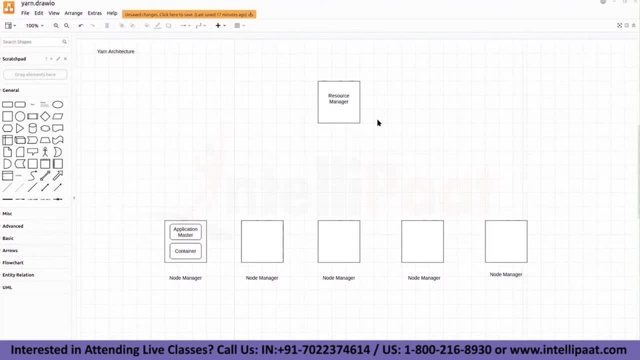 So it has got this integration. You can run a Spark application, You can run some some other, some other external applications and all that. So it's not only a MapReduce way of execution, but it can be an other way of executions also. 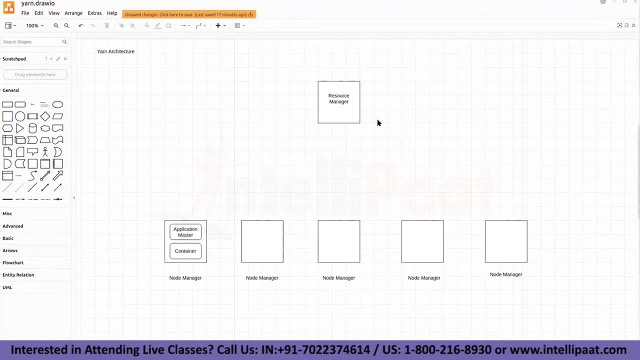 So now? so for our convenience, as we are already aware of the MapReduce functionality, let's say I've submitted a MapReduce job only for this YARN system. Guys, are we, are we confused here? Are we clear with this? 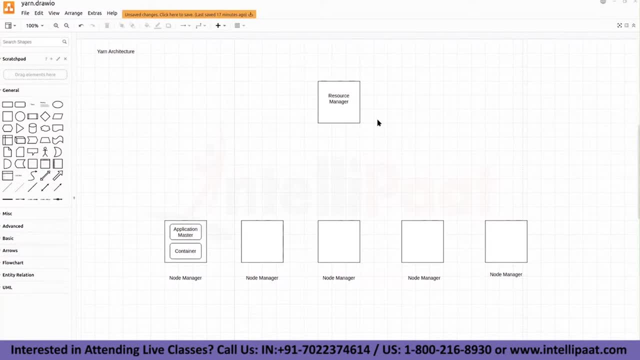 Whatever we've discussed in the last five minutes Is it? is it confusing? Are you clear with this concept? How is it different from MapReduce and how it is why it is called an application rather than calling it as a job? Yes, 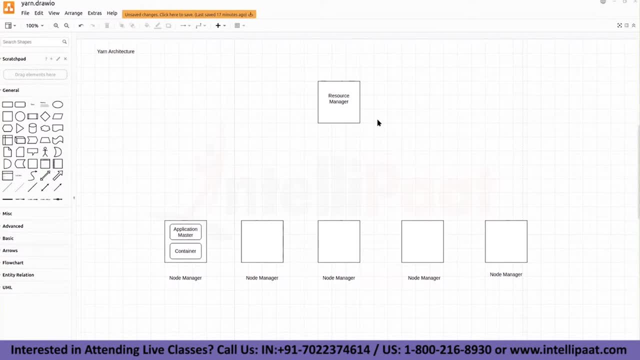 So you actually need to understand what's the main difference between a MapReduce framework and a YARN framework, right? So YARN is something going beyond, beyond the MapReduce framework, So it's not only a MapReduce, but it can also deal with other sets of other kinds of applications also. 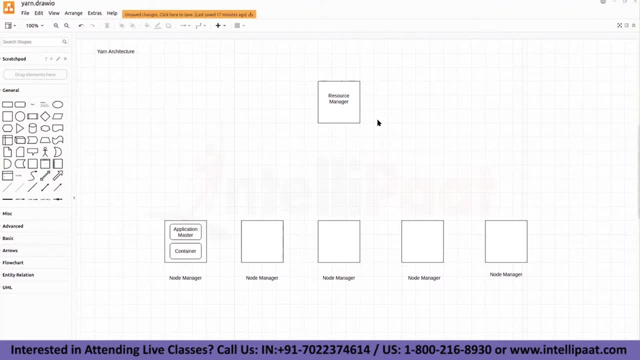 And it can also deal with MapReduce applications. right. So now for our convenience, let's say, I have submitted a MapReduce program itself for your YARN system. Okay, it can run others also. It can run a Spark application also, but I have submitted in the first place. I have submitted as a I'm submitting a MapReduce application. let's say, 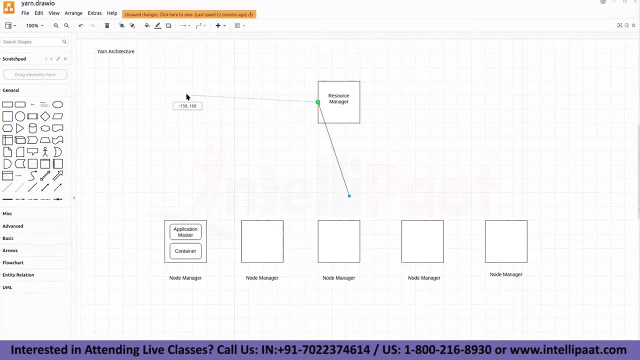 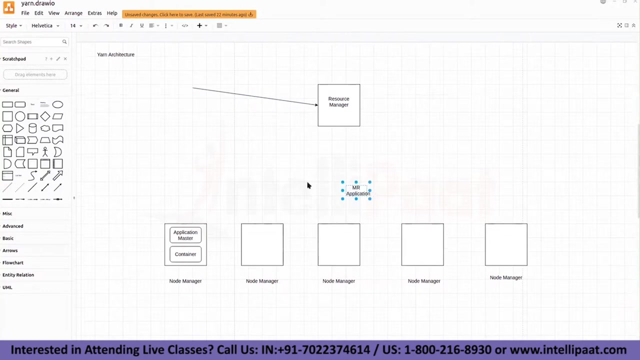 So what is going to happen? So here I have the first one as the MapReduce application. So I can call this as an application, or I can call this as a job also, because this is just a MapReduce program. Again, I can, I can simply call it as whatever I wanted to. 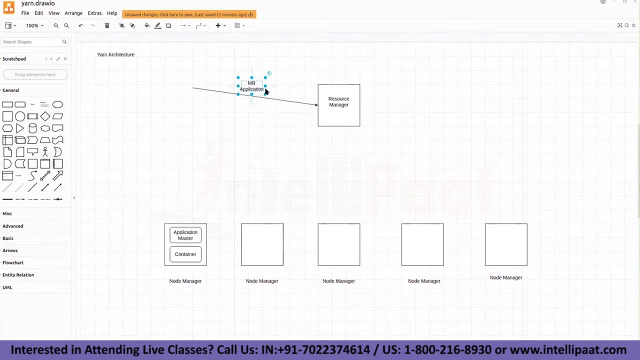 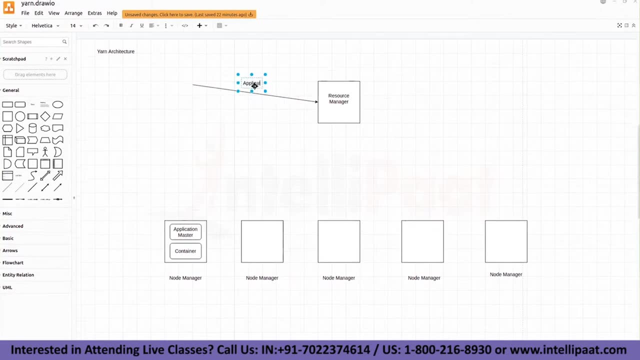 So this is your MapReduce application one. So this is, let me put it this way- Application one Which is a MapReduce right One. So this has been submitted to your YARN system. So whenever there is an application that has been submitted to a YARN system, who is going to receive it? 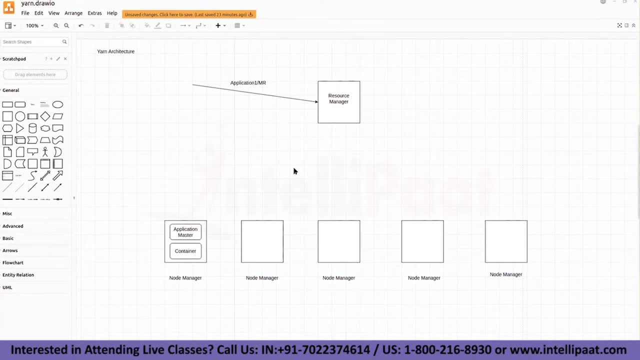 Again, it's going to come to the resource manager, right? So it's going to come to the resource manager and it's going to analyze the application. So this is a MapReduce program that I'm submitting, So it will have what. 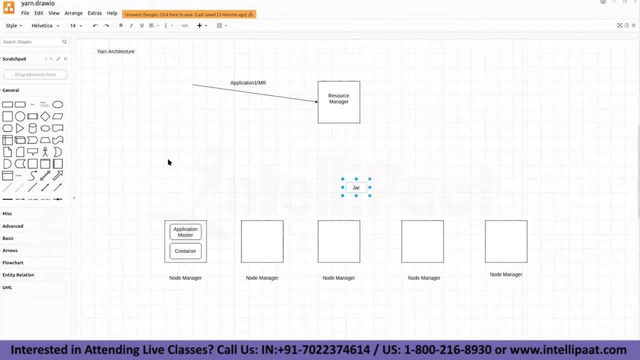 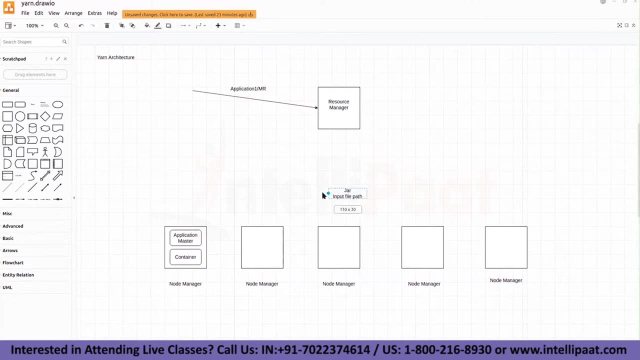 It will have two things, So a YARN and input file info. input file path. okay, It's not the block info, but it's input file path. Along with the program, you specify which YARN to execute on on which particular file. 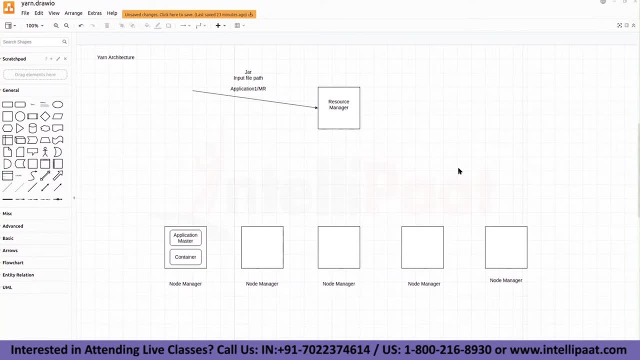 The file is in HDFS right. So the same thing I submitted to the MapReduce framework. What did it do? What did my job tracker do? It started analyzing the YARN, It started looking for the HDFS path, It interacted with the name node and received what? 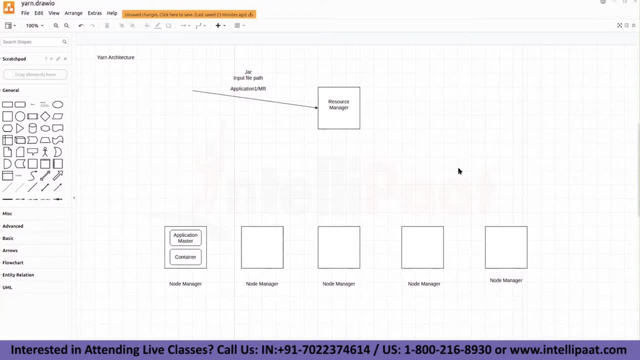 It received the number of input blocks from the HDFS name node, But now the same application has been submitted to the resource manager, to the YARN system. What is it going to do? So, regardless of what application a resource manager receives, regardless of whatever the application it can be, 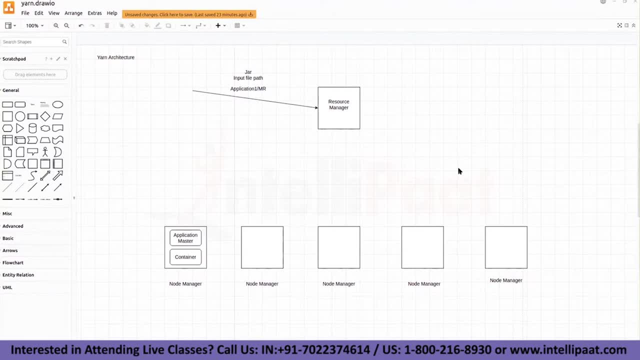 what it is going to do is it is going to allocate this application to any one of the available node managers. So see the difference. So it's not even processing it, It's not even analyzing this particular application. So straightforward: it's just going to forward the application to any one of the available node managers. 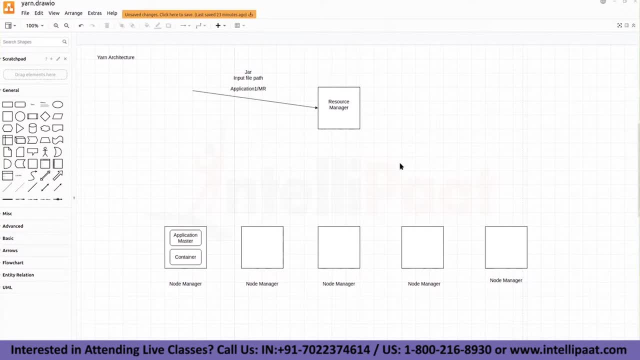 So now I have five node managers available, So it's going to allocate to, let's say, node manager one. okay, So again, it can be anything. It need not be a node manager one, but it can be anything. 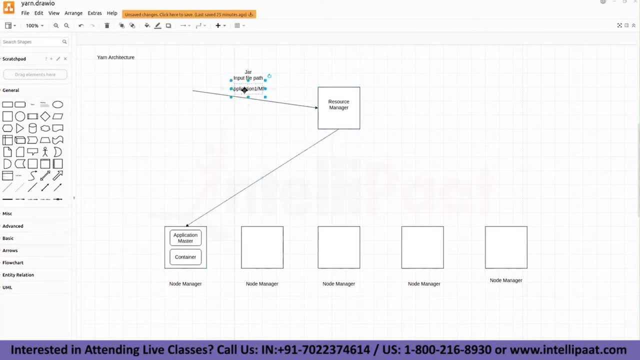 What it has done. It has forwarded the application to this node manager. So every node manager internal to every node manager, we will have an application master as well as a container, But a container will be started only when an application has been submitted to this node manager. okay, 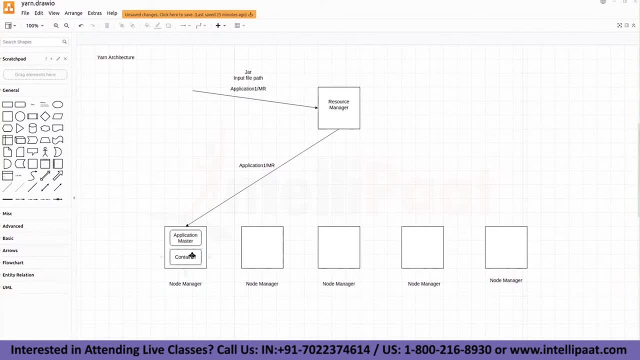 So all the node managers will have this AM and C containers. okay, We'll have these components, But they will not be triggered. I mean, they will not be this application, This container will not be. This application master will not be triggered. 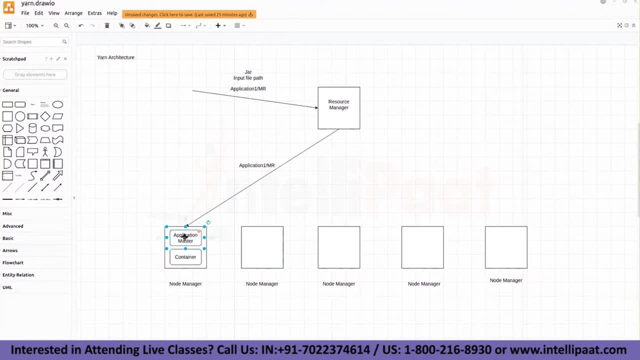 They'll all be in a disabled state. let's say, Only when an application is submitted to a node manager, that's when we will start a container and we will trigger the application master. So, for example, if this application one has been submitted to, let's say, to node manager two, what is going to happen? 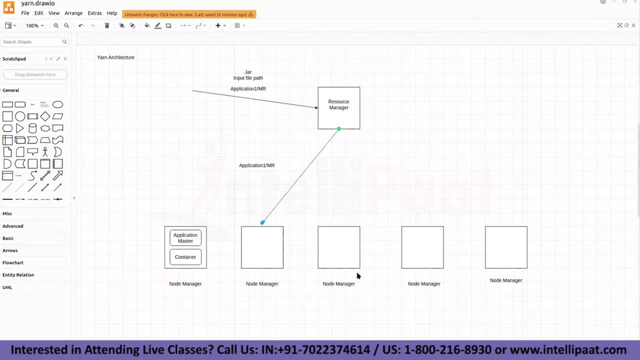 The same thing. The same application master and container will get started. So, whatever the node manager it can be, So to whichever node manager it gets submitted, that application master and container which is available on top of that node manager will get triggered, will get started. 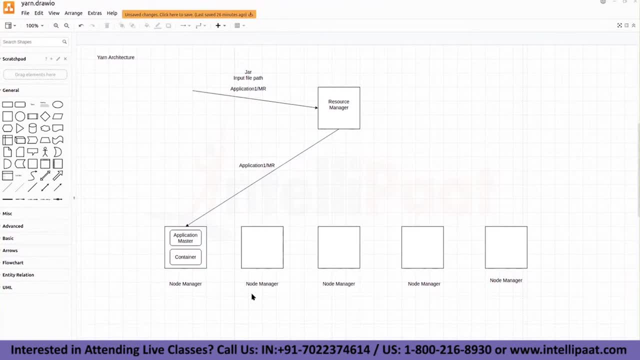 So now, what is this container? What do you mean by a container in general terms? No, I mean, forget about the blocks and everything. So container, What is a container going to do? It is going to hold something. 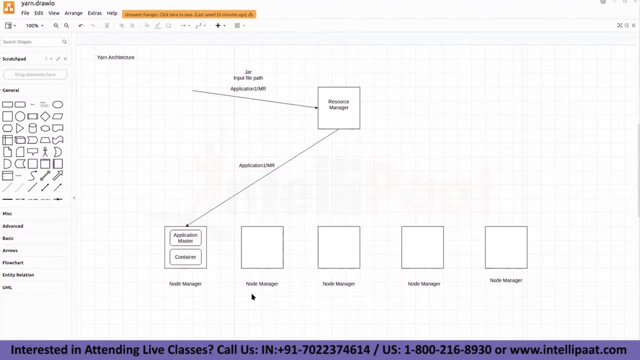 A container is generally used to hold something. What is that something? here It's going to be the resource. So this container in node manager- one now, in any node manager for that matter- is generally used to store or hold some set of resources. 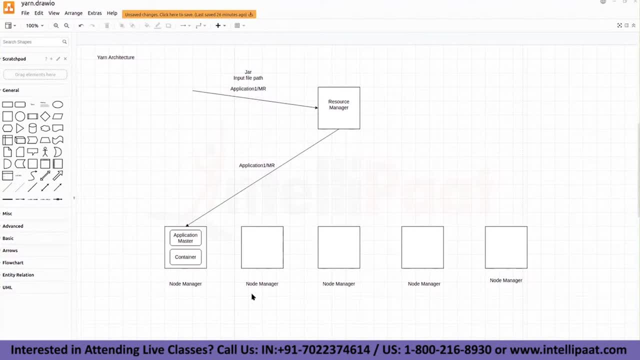 So why is that we are going to need these resources? We need these resources to execute this application one, Yes or no? So we received this application one. So now I received this application one and I need some resources to execute this application one. 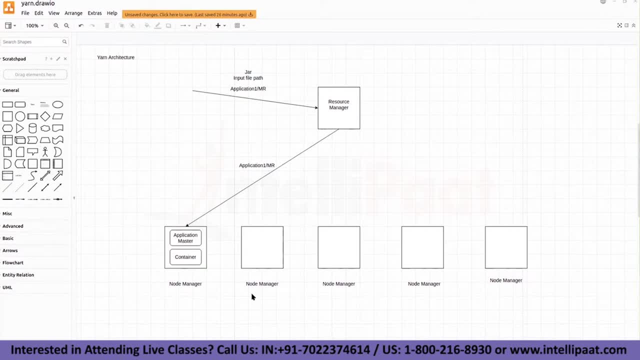 And where do I keep that resources? I'll keep that In the container. See, it's not that you will pull all the resources and put it in this particular node manager, But see, allocating a resource to a node manager is something as simple as, like you, just providing the IP address of the machine. 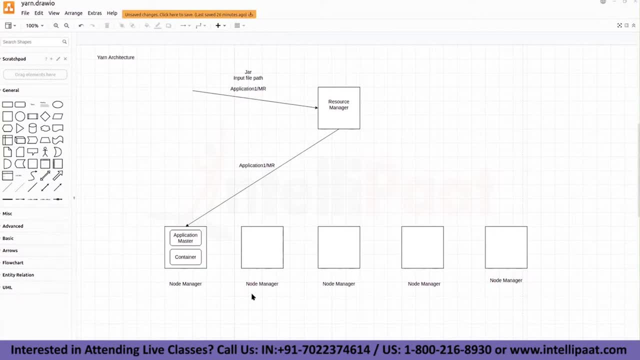 You just need to use it, That's it. Okay, So in some file the IP address IP addresses will get tagged, And as long as this IP addresses are tagged to this particular file in the node manager, that means they are all working for this node manager. 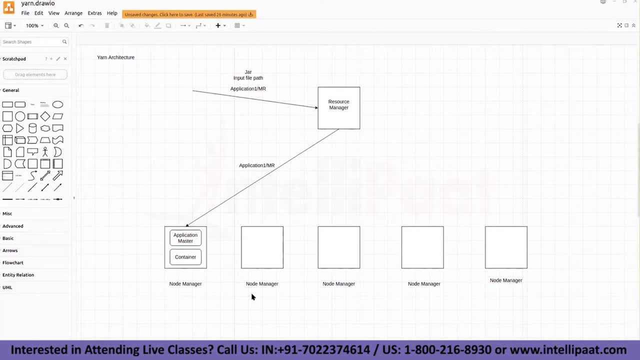 That's itself. That itself is the allocation of resources. Okay, Okay, So it's not some other thing. All right. So now we would need a container to use to hold the resources. So that is the reason why we will be using the container. 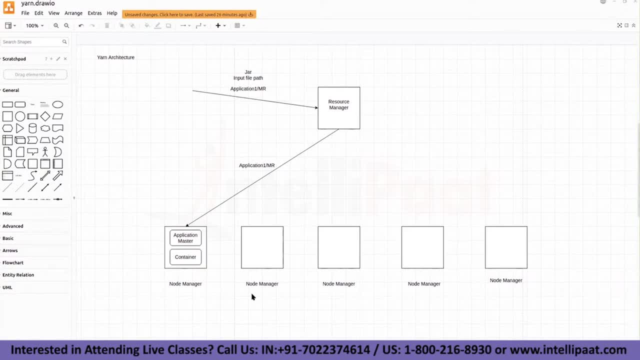 And application master. So what does this application master mean? So, for every application to run, this is an application, one that is getting executed. So, for every application to run, you would need an application master, which will take care of all the execution of the application. 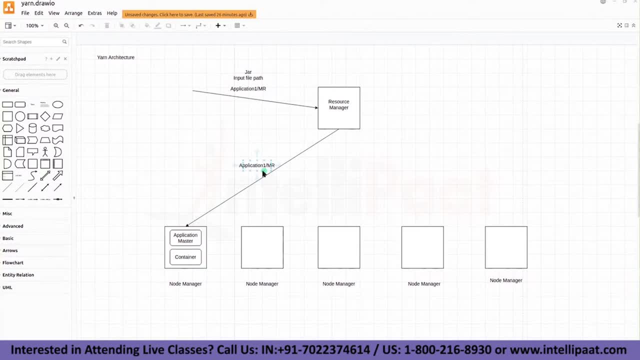 So, in simple terms, you can consider this application master as the job tracker in your MapReduce framework, Job tracker in the MapReduce framework. So I'm talking in terms of job tracker now. So now this application master is the job tracker for your application one. 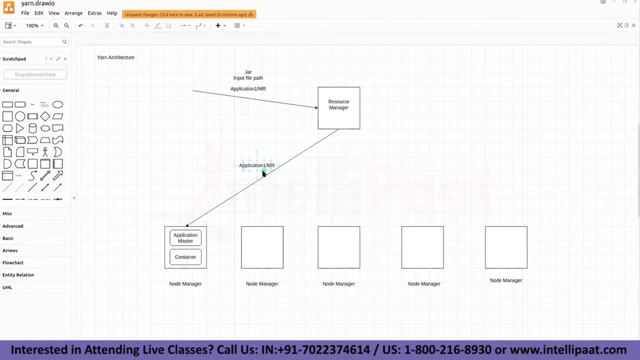 It's the sole owner, It's the whole responsible person, It's the sole person for this application, one to execute. Okay So, application master on node manager. one is the complete responsible to complete this execution of this application. one, All right. 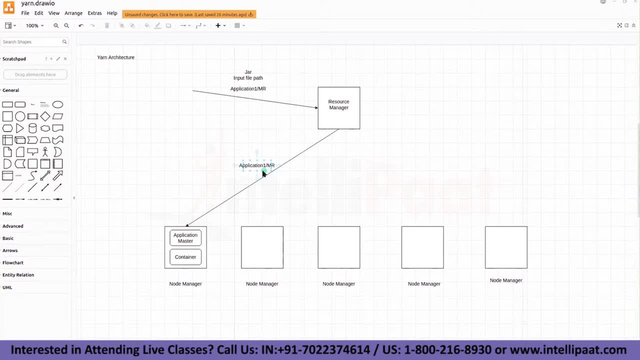 So it will now act as a job tracker for application one. So what it has to do, What is it going to do now? What did my job tracker do? as and when there is an application got submitted, It will interact with the HDFS. 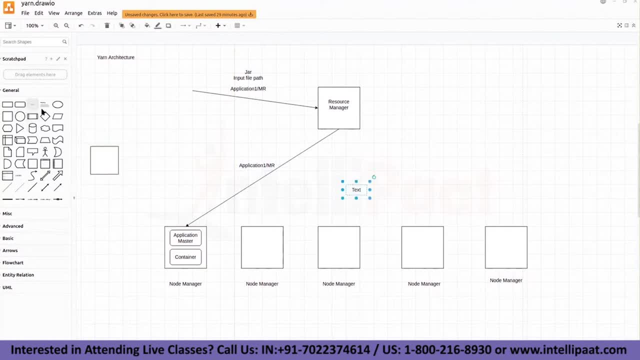 Right, So there is some HDFS. There is some HDFS here, let's say: And what is it going to do? It will interact with the HDFS to identify whether this input path is correct. If the input path is correct, what it's going to do. 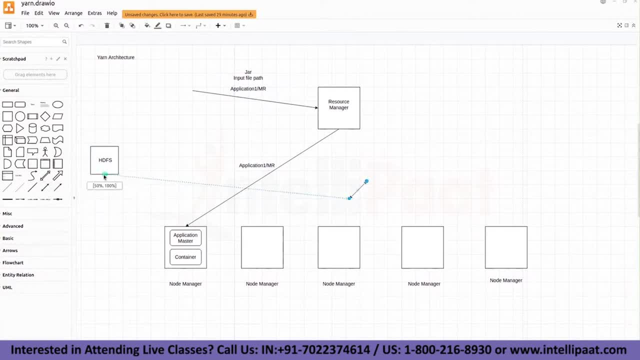 It will retrieve how many input nodes or how many input blocks it has got Right. So depending on that information, I'll point it to. So application master has interacted with the HDFS And it will identify whether the input path is correct. 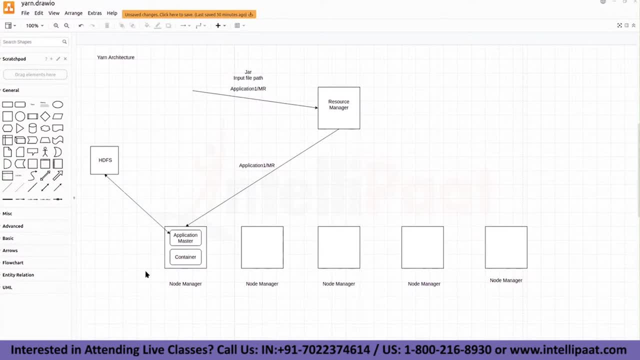 If the input path is correct, it will receive how many input blocks that it has been written into Right. So, depending on the number of input blocks, what am I going to do? I'll be dividing those many map splits Because, as this application itself is a map reduce application, 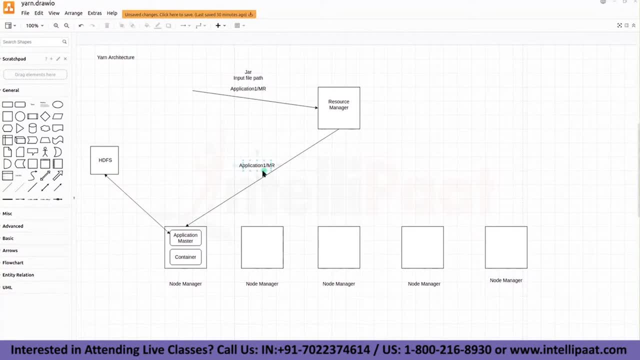 Okay, I'll have a map task and I'll have a reduce task, Right? So I'm taking this as an application- map reduce application- because we already know the procedure of the map reduce program, How it's going to execute. 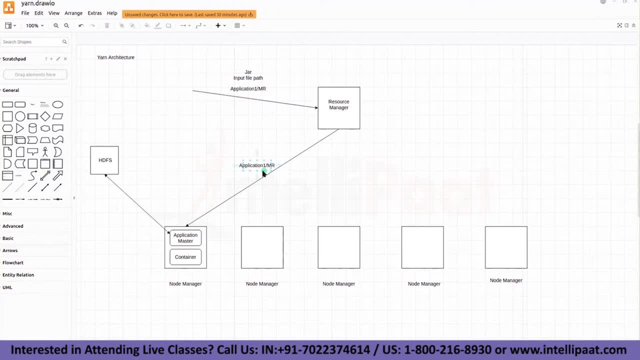 Okay, For spark program it can be a different procedure. procedure again, Right? So let's, let's talk about that a little later. But now we know that there is a map reduce application that has been map reduce job that has been submitted to it. 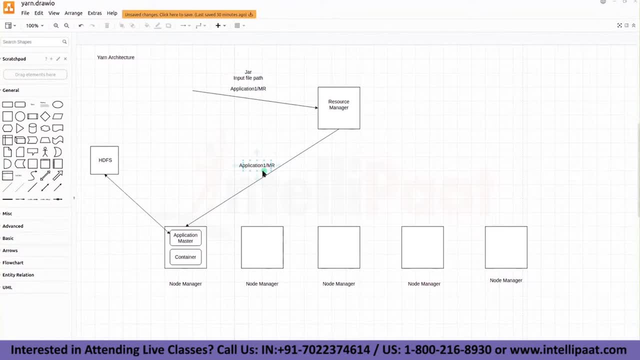 So now it will. it will send it to the application master. Now your application master will interact with the HDFS and will receive how many input blocks that particular file has been written into. Depending on that, it will divide so many map tasks. 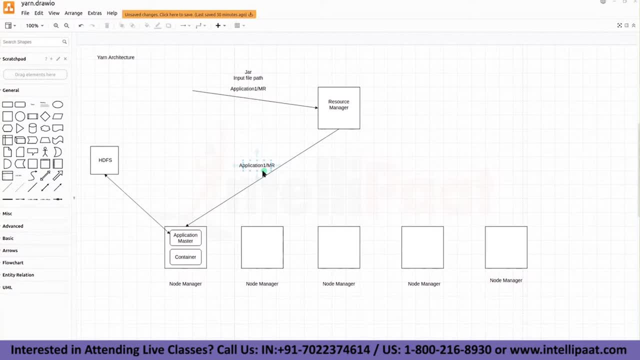 Right, So many map tasks it will divide. After dividing this map task, What is the next thing it has to do? Yes, What is the next thing that it has to do? It has to. what is the job tracker doing after dividing the map tasks? 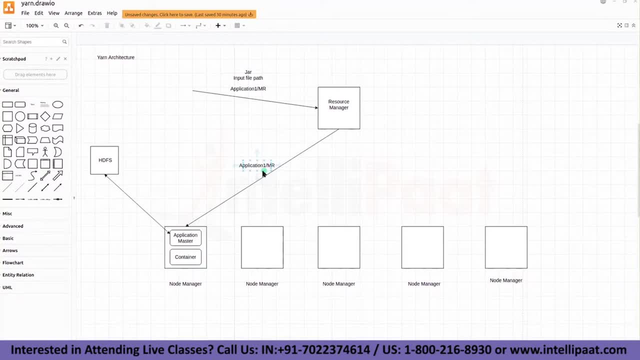 It is allocating it to a task tracker Right. Each map task has been allocated to so and so task tracker Agree, But where are the task trackers here? So now, after, after analyzing this map reduce program, after interacting with the HDFS: 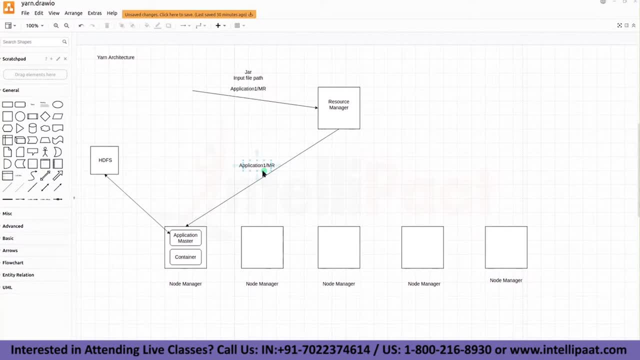 Yes, Let's say I have. I have three blocks of data on the HDFS side. Okay, So how many input splits map splits I would need? I would need three map splits. So now your application master knows that it would need three map splits. 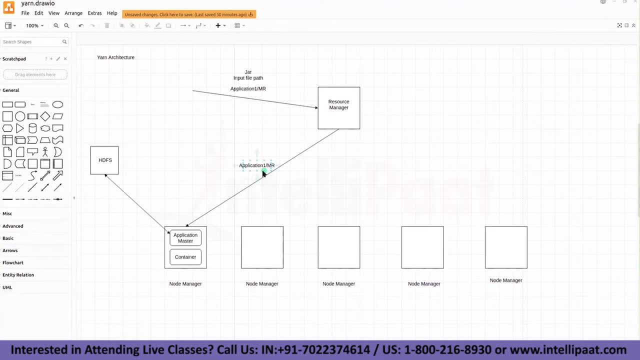 It has been divided into three particular map splits. So for executing this three map splits, I would need three resources, three task trackers to execute. So whom I have to interact? I'll have to interact with the resource manager. Now I'll be interacting with the resource manager. 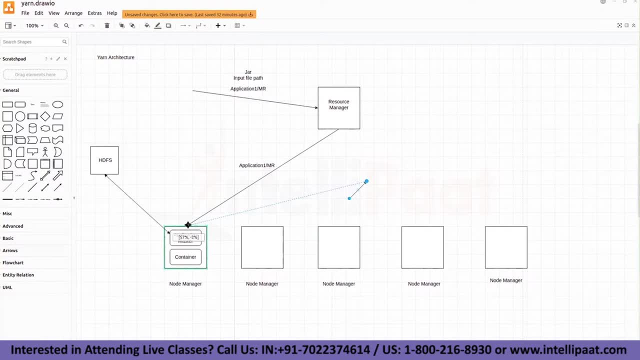 And then I'll be requesting for the resources. So interact with the resource manager saying that, okay, I would need three resources to run this particular application one. So now, when I allocate this three resources, when the resource manager agrees to this request and allocates these three resources, these three resources will under will come under the control of this container. 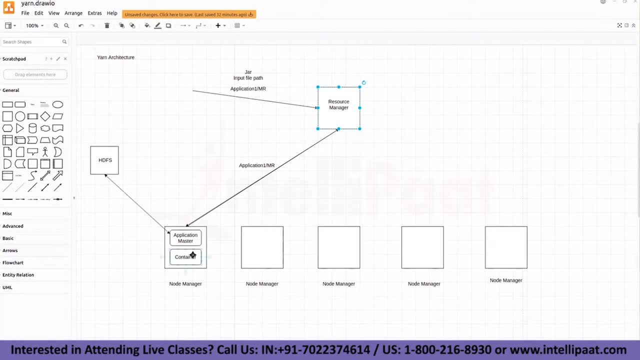 I mean it's, it's, it's under this particular container, It's under this, Okay, So now what happens? Okay, Whatever. So what is going to happen is this: application master will will get the control. 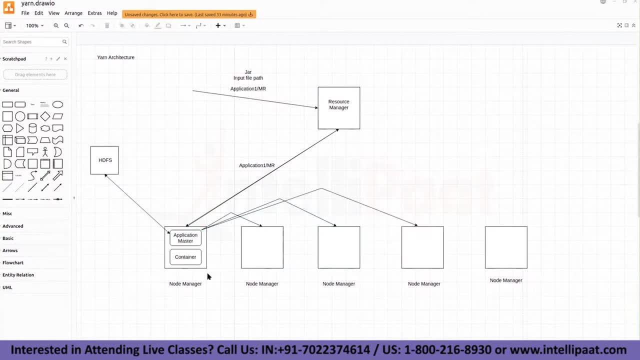 This is enough, right for us, Right. So now resource manager has allocated these three node managers to your application master, available on the node manager one. so what it has to do now: your application master has received the resources, so it will submit each. 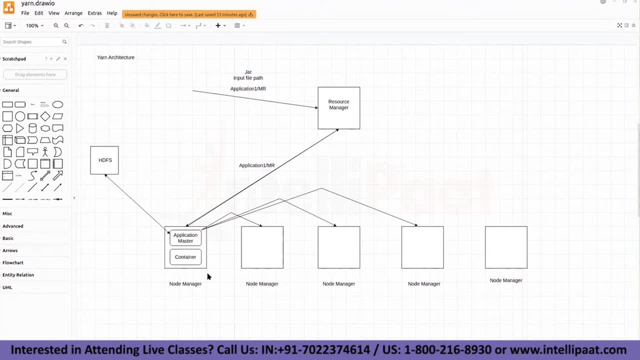 and every map split to each and every node manager and it will make sure they execute this map splits. so these node manager two, three and four now are acting as a task tracker. agree, right? so now the submission has been done. the map split submission has been done. 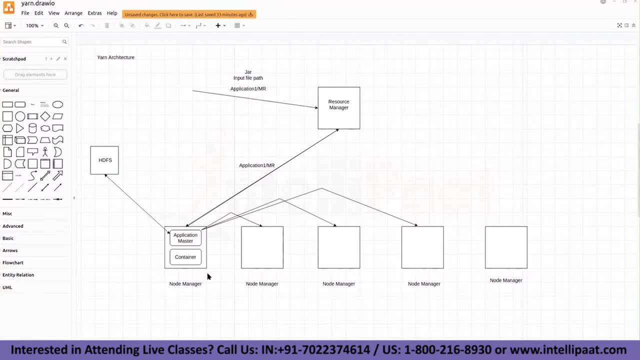 and they'll start executing the map task on top of the hdfs data block. they'll return the result and the result has been accumulated at the application master, and then, followed by it, they'll run a reducer. i mean application master itself will execute a reducer functionality. 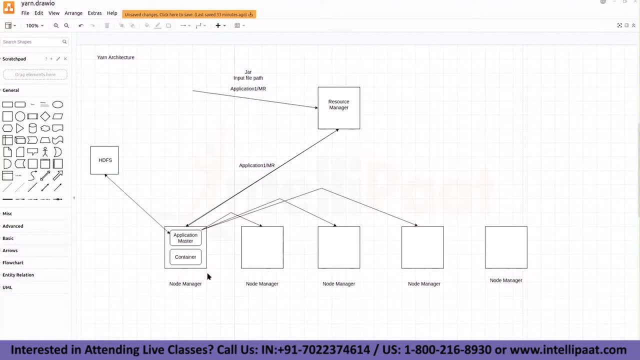 after retrieving the output, the application master will send the output to the resource manager. so after the output has been sent to the resource manager, the resources will get the untagged, i mean they get removed from this application master and this application one will get removed from this node manager one. so now, after the application one execution has been. 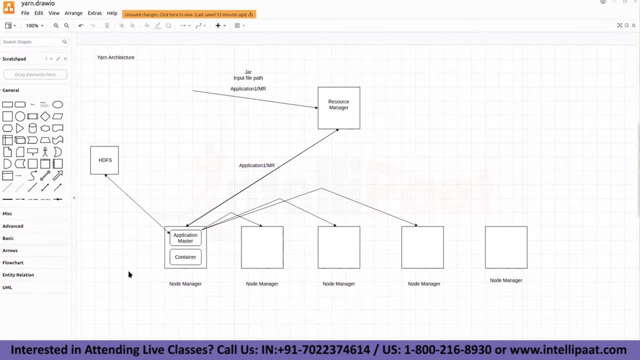 completed, all the node managers will go back to their routine state. i mean, all the node managers are now one and equal. this is not a master anymore. this is not a slave anymore. okay, getting it. so next time when an application gets submitted, it may get submitted to node manager two and this: 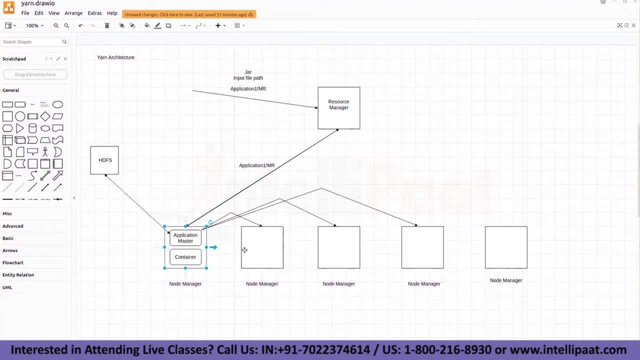 also can act as a task tracker. so this is not a master anymore, this is not a slave anymore. this will act as a master and this will act as a slave. so any node manager can can at any point of time for uh for a different application, can act as a master or as a slave. okay, so that is the uh that. 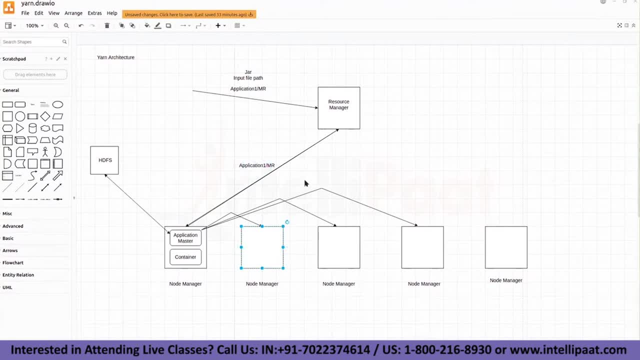 is the functionality of it now, in the mean time, let's say in the meantime, application one is running. there is an application two that got submitted. this is a spark application. let's say anything, anything it can be okay. so this just is a application to spark application anything, anything okay for that matter. so this got. 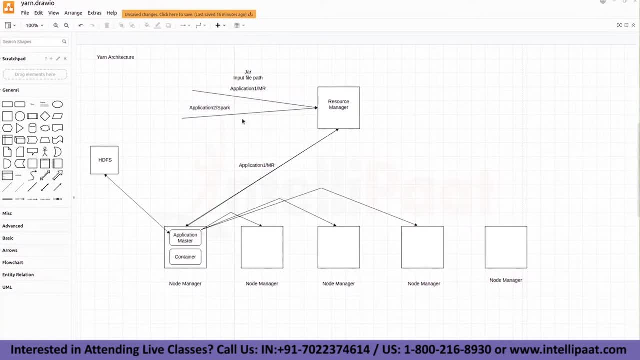 submitted in the meantime while this particular node manager one is running. so what it has to do? resource manager will send or will forward the same application to the available node manager, that is this node manager five. so what happens? it will trigger this and then application two will run, and then application three will run, and then application four will run. 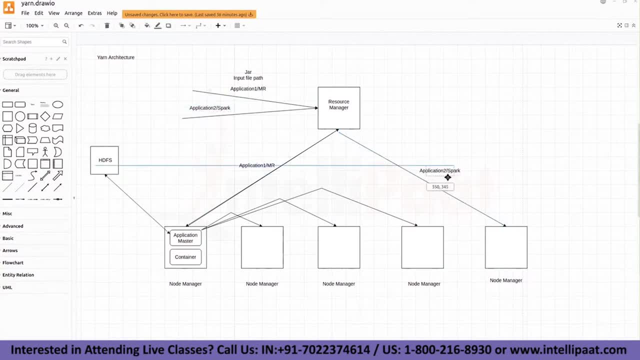 and two gets triggered to this. so this is all parallelly happening. i mean, while the application one itself is running, this particular process is being contained, continued. so you get this application master. you get this container because the application has been submitted to this node manager. pirate, so this get and this gets submitted. so next, what is the process? it can be a different. 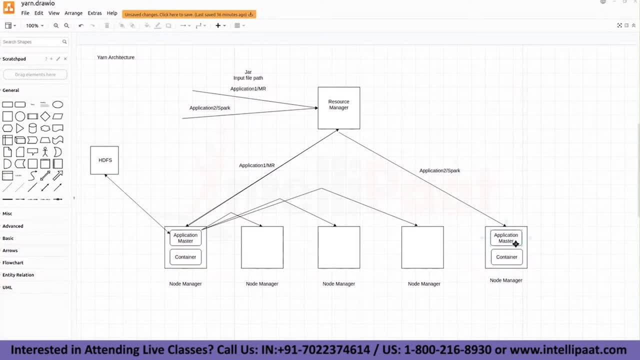 process now. so spark has been submitted, the spark application has been submitted, so everything will have some input file. so it will interact with the hdfs, first to check whether the input file is done, is correct, and then there is a. there is a different procedure altogether, there is a different functionality. 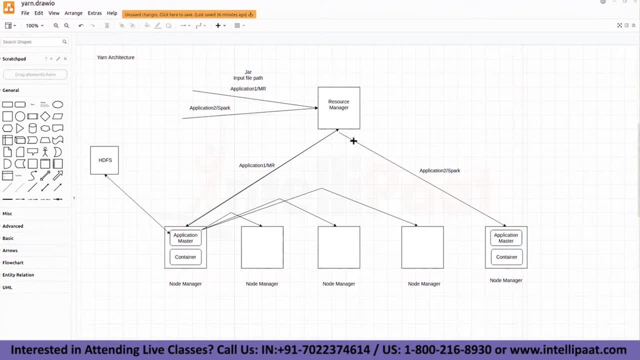 altogether. it is running right. so, depending on that, it will identify how many resources your application master available. in the node manager, phi, will identify how many resources it would need and it will interact with the resource manager to allocate those resources. so if the resources are available, it will allocate. otherwise it will be on queue or it will be on hold until the other. 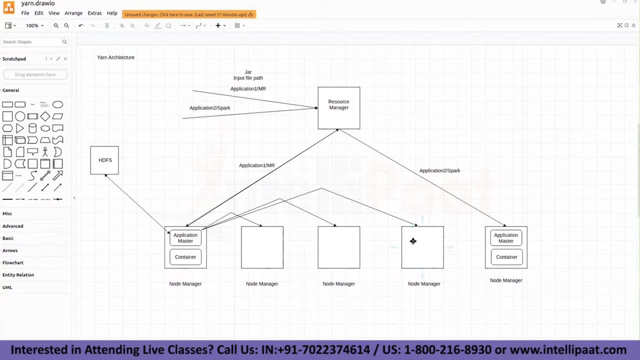 resources get freed up. getting it. are we clear guys with this procedure? okay, so what is that we are achieving from this? is we are decentralizing the master functionality, the job tracker, or the master functionality, from the actual master, from the resource manager, to the node managers. right, so that way we were able to execute multiple 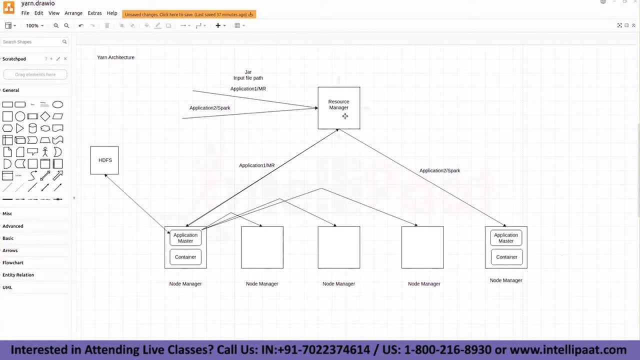 applications at the same time. so earlier, when the job tracker was running on the master, when it was processing the application it had, it had allocated most of its resources or most of its time to complete the application that it has been submitted with. until then, until the execution is complete. 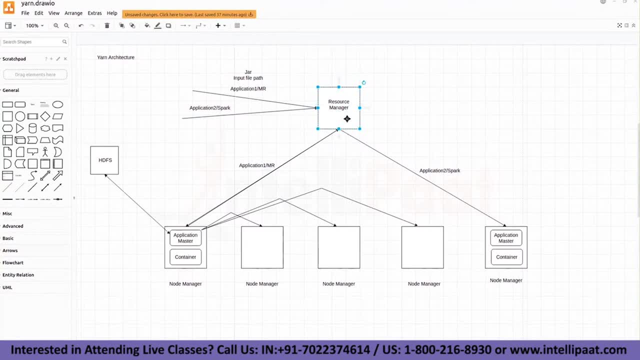 you're not in a position to submit any other application because, let's say, the ram of this resource- job tracker- is some 8gb. so you submitted application one in the in the previous versions, in the previous scenarios you submitted some application. so entire ram or entire memory is. 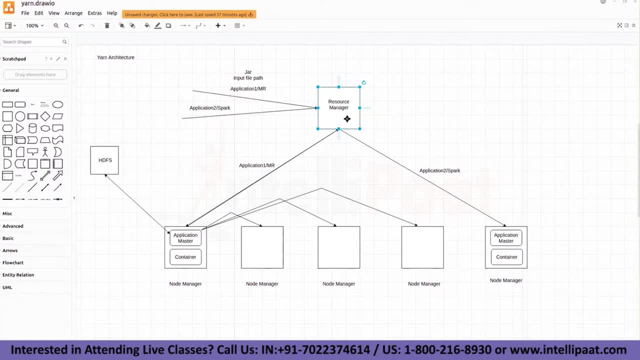 being allocated for the application one only when you submit the application two. it does not actually have the resources to process the application two because there has to be some kind of an activity happening on the job tracker also, right, so it does not have the available resources. so now what is happening is your master is kept in. this particular master is kept. 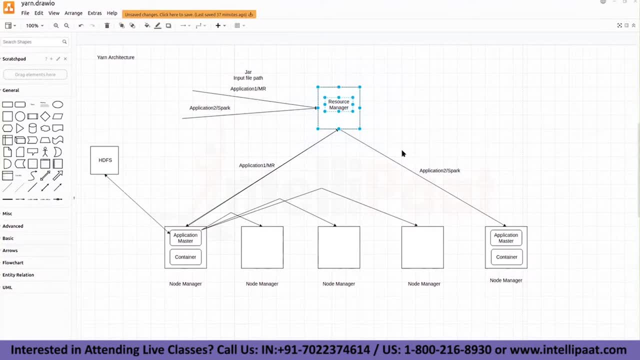 readily available always, i mean it's. it's not taking care of any execution process, it is just making sure it will receive the applications, any number of applications, for that matter. right, it will. it is it been kept idle? it has been kept open for receiving the applications and after receiving the applications. 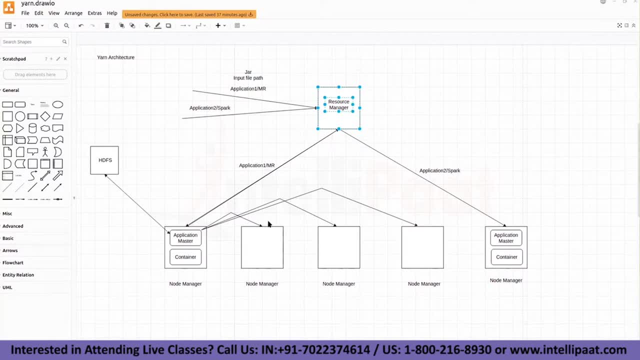 it is just identifying the available resources and it is just forwarding it. so you are decentralizing the entire core operation from this master to an actual slave machine. so you are actually making a slave machine as a master for a specific application. actually, node manager is what it's. 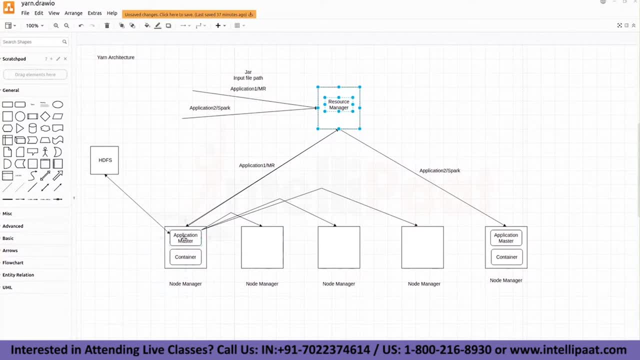 a slave machine and you are making it as a master to execute as a specific application. so that is the advantage we get here and, moreover, the resource management is is being done by a particular resource altogether and only when identifying. after identifying the resources you are, you are receiving the request, your resource manager is analyzing the request and 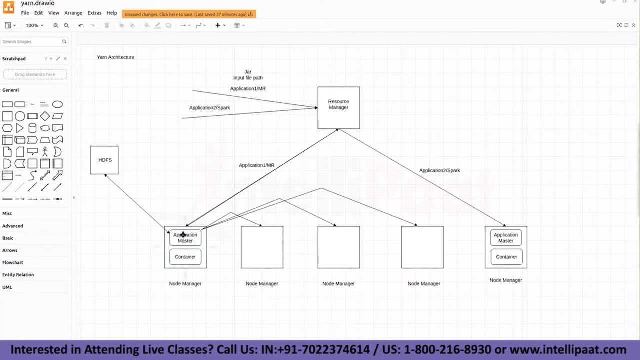 it is just allocating the resources depending on that. so it does not mean that when you need 10 resources, it will allocate 10 resources, but there is going to be a threshold and it's going to allocate the resources in a proper order or in a proper format. okay, so those are the 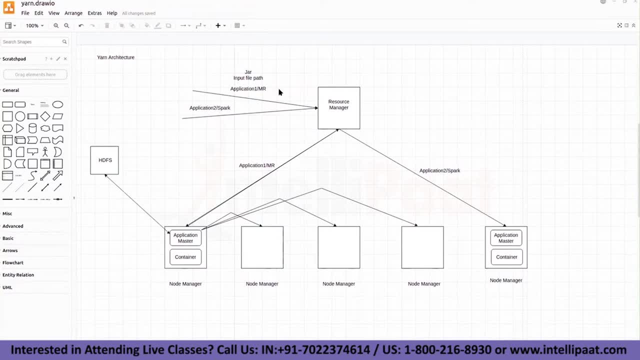 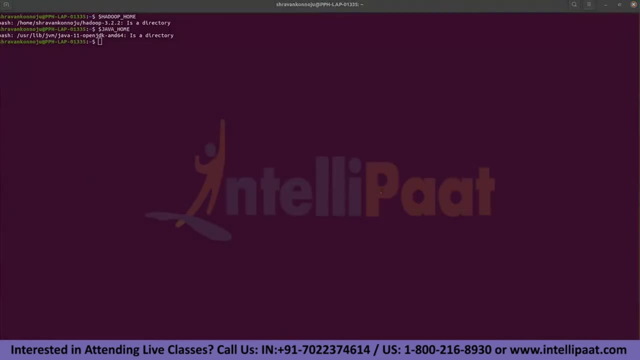 limitations we're gonna be, we're gonna solve here, guys, are we clear? okay, so this is it with the yarn architecture, guys. so, um, the change is gonna be something like this: so you have a folder named the hadoop envsh, right, so there, you will anyway update the java home and in in uh core site xml. 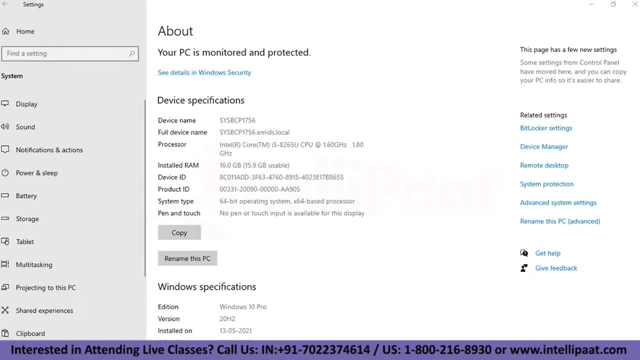 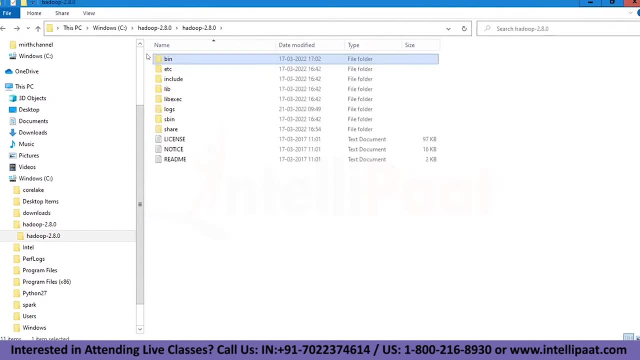 so go to the home directory, hadoop directory, and navigate to the bin path. to the bin path. uh sorry, yes, bin path has been. you have all those. so go to the ai. one second, one second: hadoop 2.8. go, come back. come back, hadoop 2.8, and here you have a etc folder. can you open that etc folder, etc. hadoop. 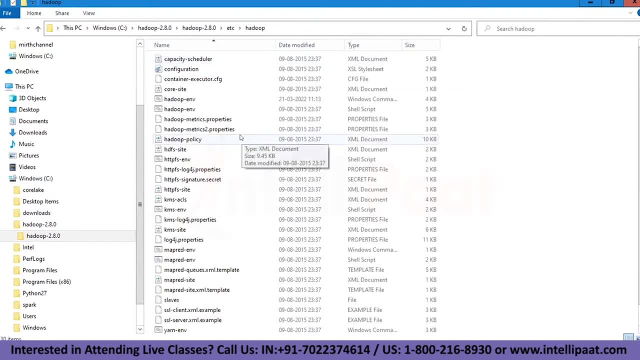 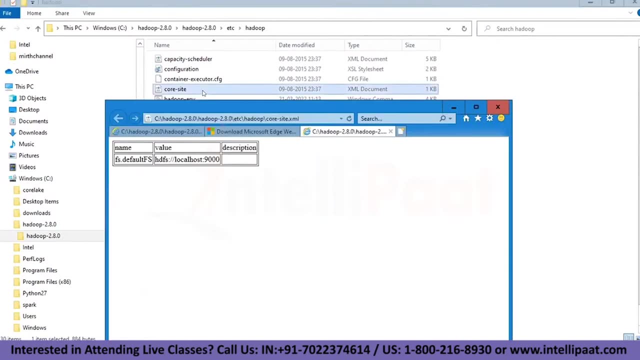 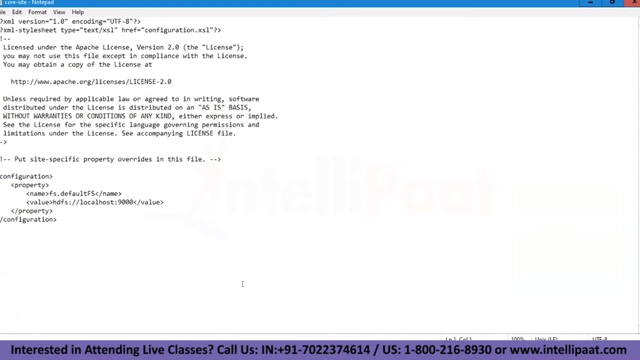 see, the first property file that we need to change is a core site xml. okay, so core set xml will will provide you the. uh yeah, open that file, right. uh no, no, edit it in notepad to open this xml. it will open up uh xml page directly. so edit it with a notepad, right? so here you can uh see uh the fsdef. 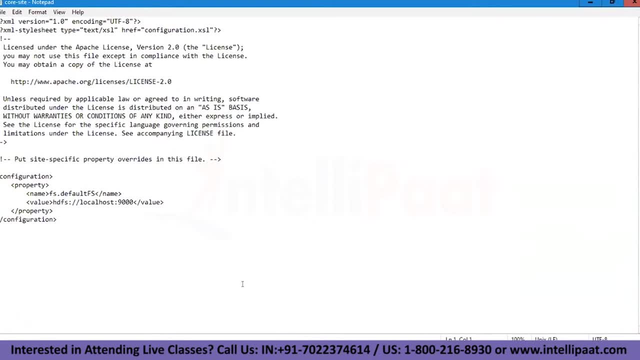 fs property is been set. right so hdfs, colon 127: whatever the local host path, and 9000 is the default path for your hdfs, right? so this properties will be set to the available hdfs and you can also come see: this is the default path for your hdfs. it will not be set to the setup policy, right? so this property? 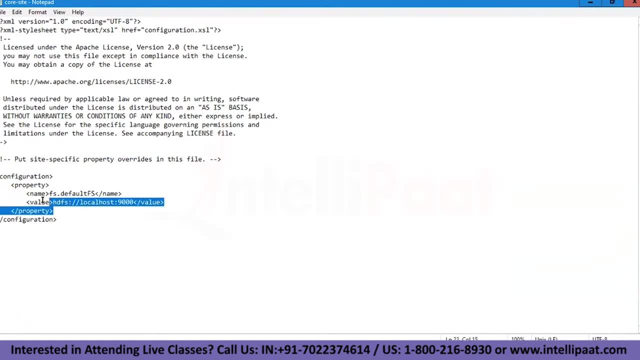 has been set and everyone might have this property value already available. this is the default port number. so what happens is, after you log into the, after you start the services, you may navigate to the localhost 9000 and you will be able to see the HDFS UI web UI. okay, so we will see that little later, and then 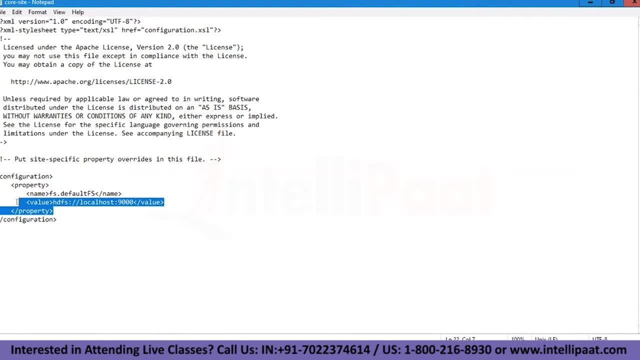 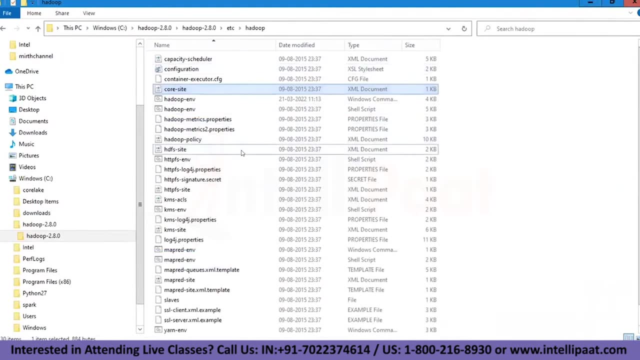 now open the HDFS site dot XML. close this. this is the only change that we need to do in the core site. so there are other properties also, guys, but those are alternative in optional. so now you can open the HDFS site dot XML. HDFS site dot. 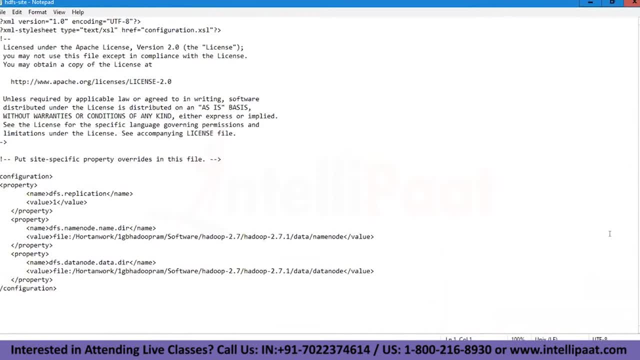 XML does has what. so there is a defaults dfsreplication, so this is a property that says that the replication factor is been set to one. so here you need to make the changes 1, 2, 3 and it will. it will accordingly update that in. 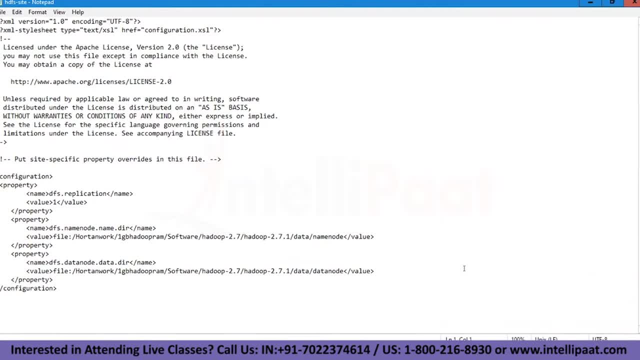 the data nodes: okay, so dfsdatadirectory. okay, so dfsdatadirectory- data node- data dot directory. and name node- data node- data dot directory. so there are two files available here. so these files are: uh, we may have to change the path. so here you have to change the. 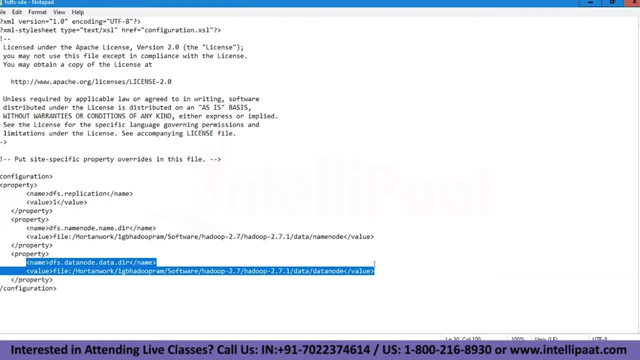 path to whatever the directory you are considering you are. you are considering it to be a um. why is it 2.7 again here? did we change? did we make these changes because it's a hadoop 2.8 file? right, if it is coming by default, it must have had 2.8 file only, others also having the same file. 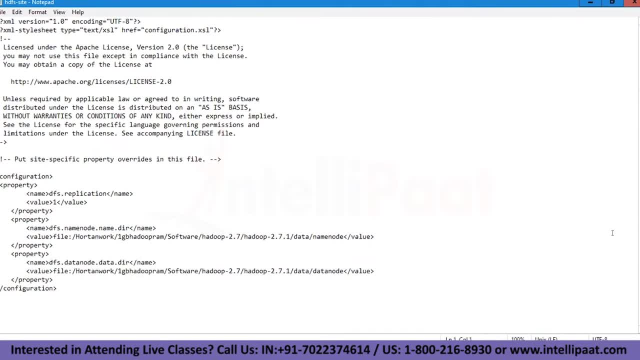 with the 2.7. what is the file name that we are reading? hdfsixml, right? yeah, let me check in mine. hdfsixml has what this is by default. uh, giving you the 2.7 path. okay, so here, what we have to update is we have to give some c drive location or any d drive location. 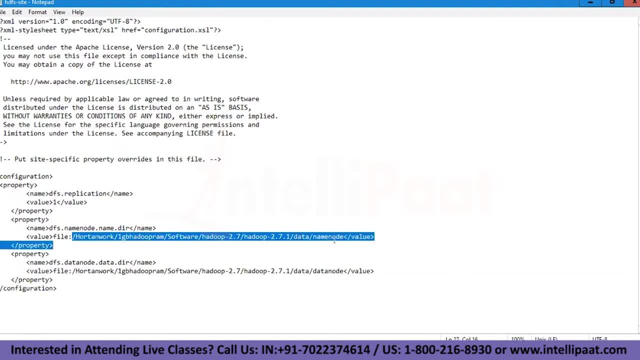 which you wanted to consider as a data node or the name node. so, whatever the data, yeah, so whatever the path you specify here will be considered as your data node location. okay, so whatever the files you store will get loaded into that particular location. so this is for your. 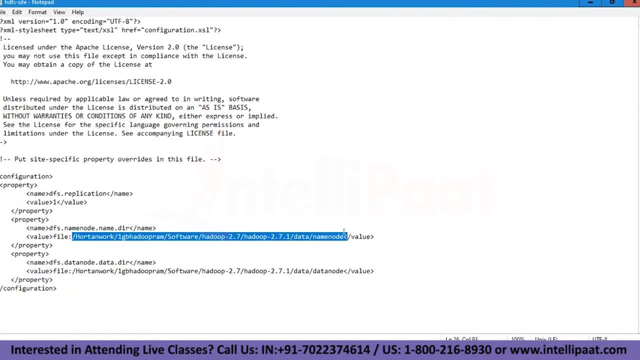 uh, name node and the down below one is your data node. so name node directory is that and the data directory is this. so you specify c, dot, whatever, whatever the file names you wanted to, and that will convert it into a data node path as well as a name node path. by default, name node path in the data node. 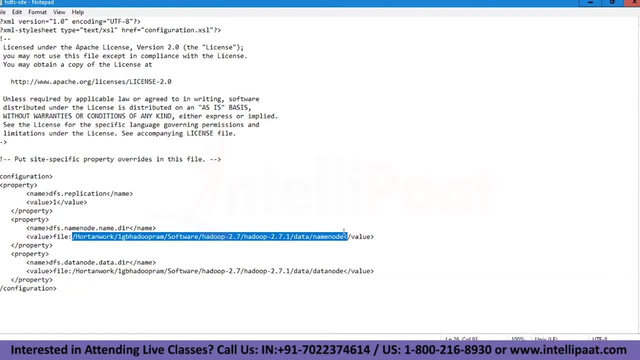 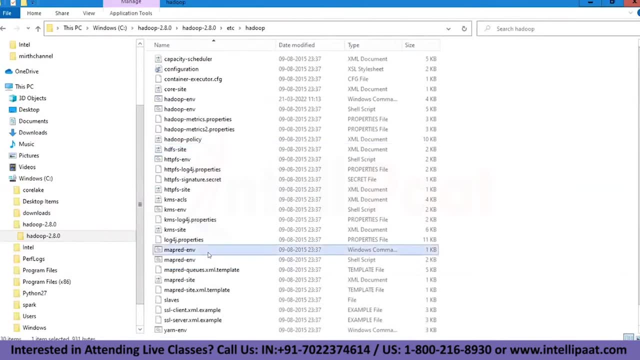 path. so this is one hdfsixml, and can you go to the mappered sitexml? there is one more mappered sitexml, that, no, no, not xml file, but xml file. next, next, next, next, next, next. yeah, here this is the xml file. edit it. so here you have only one. 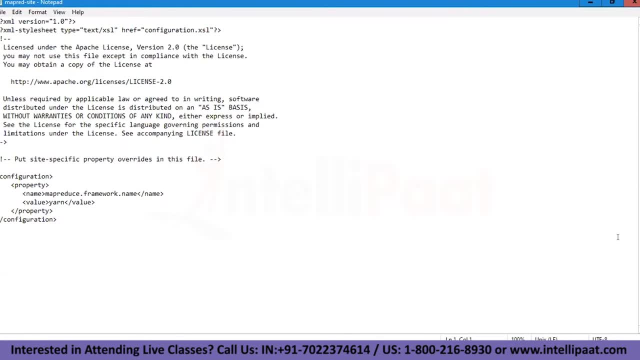 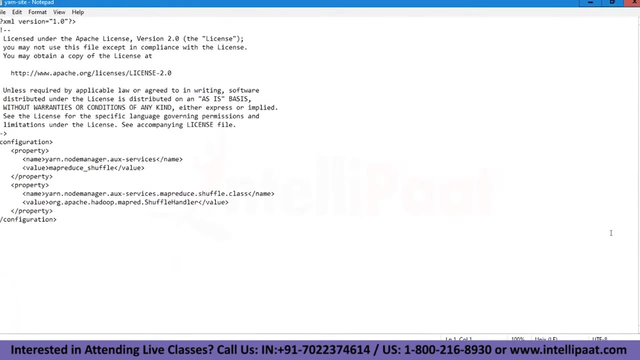 property mostly. yeah, so mappered framework name is yarn, so this is. this is anyway there. this property has already been set here. so now come back to the yarn site xml. once again. last one, and do we have a property defined? uh, services is not required, services manager is. 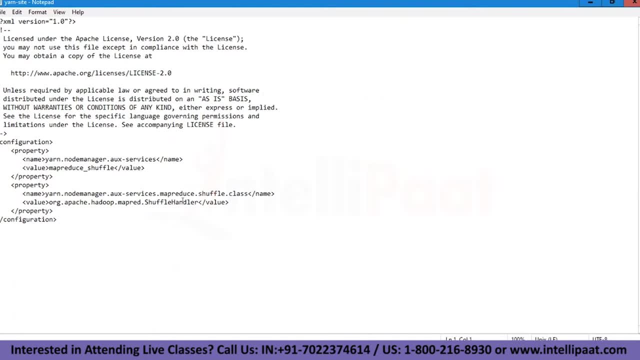 not required, but you can specify. um, i'll give you the property name. so i'm putting that in the chat so you can update these two, so you can just append these two values to the existing properties, these two tags, these two property tags. this is in the yarn site xml. no, no, no, add these two. you. these two should be there. 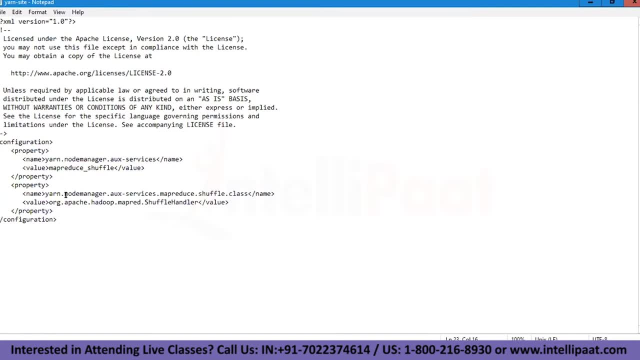 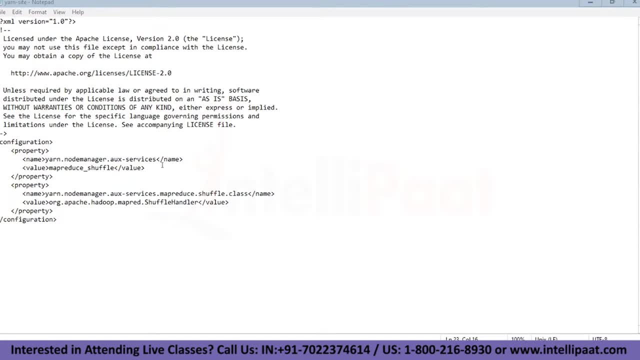 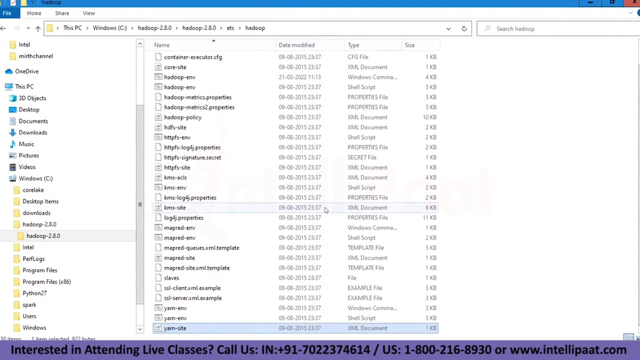 twenty seven dot zero dot one, and that will take you to the resource manager ui web. ui, right, that should be fine. yeah, and then save it and come back to the uh hdfs site xml file. we didn't update right, so that's okay. can you give some path in the hdfs sitedf, hdfs sitexml, because that's. 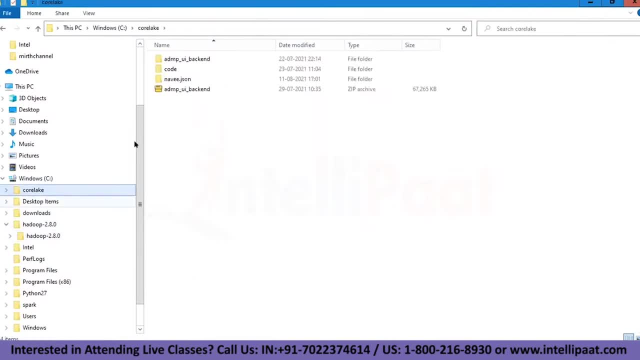 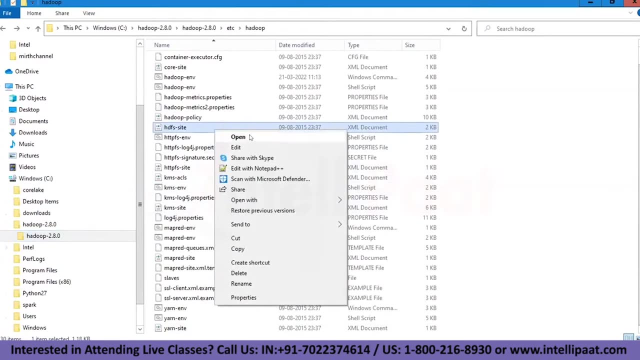 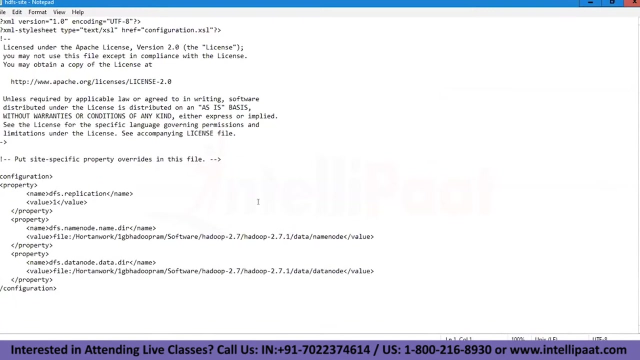 the only file we didn't specify the here here. it's up here itself. no, no, no, come back. come back in the same file: hdfs sitexml. i did that file once i did that file. what is it listed? file: colon uh carton works. so here after that, colon uh give. 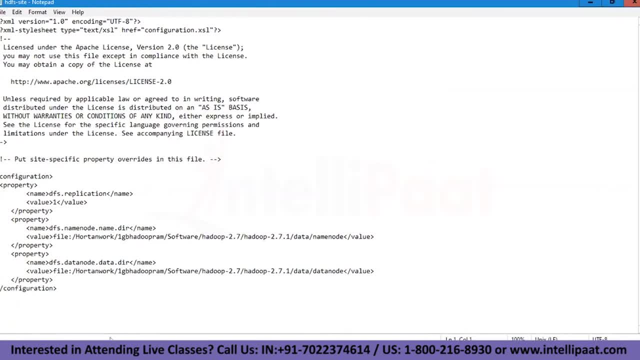 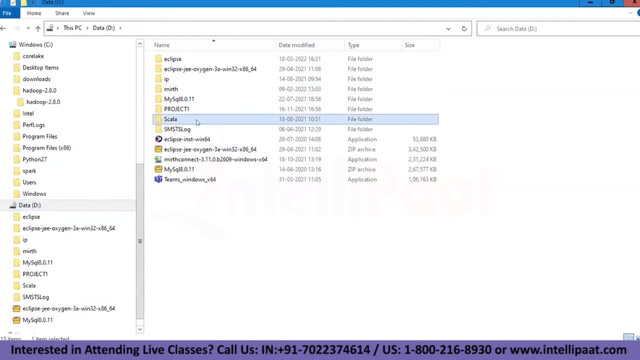 some c drive path or d drive path, whichever. whichever path you wanted to specify, that's okay. so d drive is editable, right? so better we give this: um: create one directory here, otherwise no, no, on the d drive itself: create one directory. create one directory saying that data or whatever. 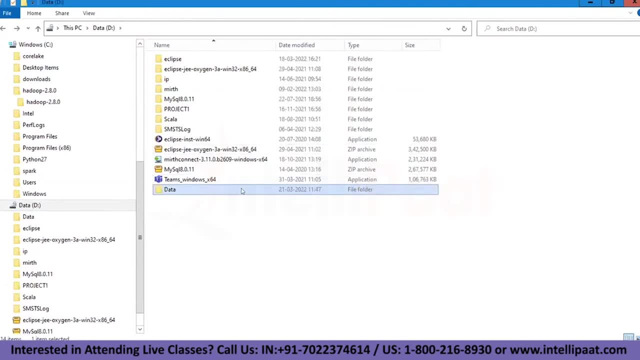 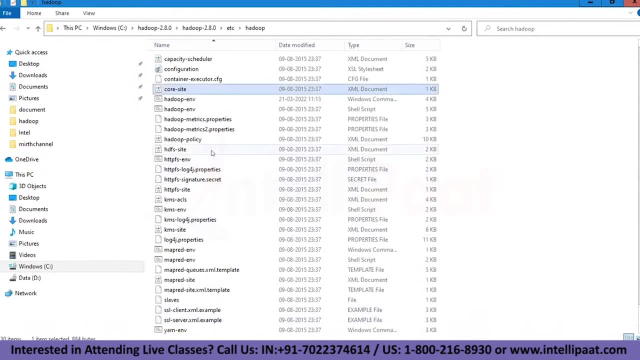 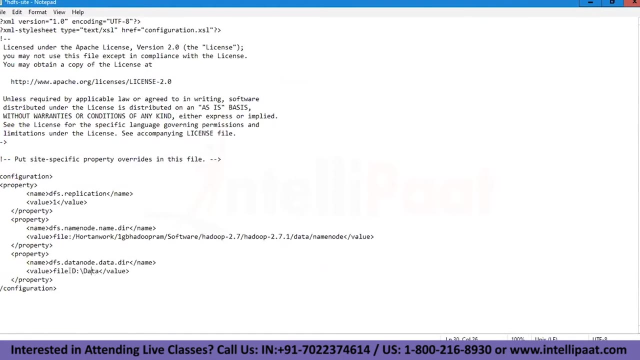 data: yeah, use this path, use this file path to give in the hdfs site. not bad, it's already open like this. yeah, data, not directly. so, but you have to specify this in the format of hdfs and remove that file as well. let's see, because this windows format. we have to see what. 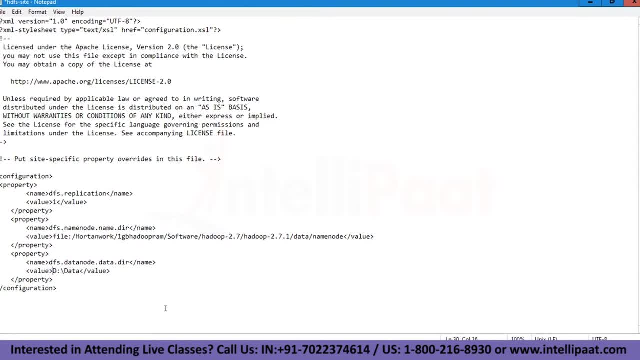 format it is going to take. yep, save it. let me see. if there is any other format specified, let's save it. that's okay. let's do one thing otherwise. um, let's create one directory inside the hadoop itself, inside the hadoop folder. that's better, because it's going to identify directly. 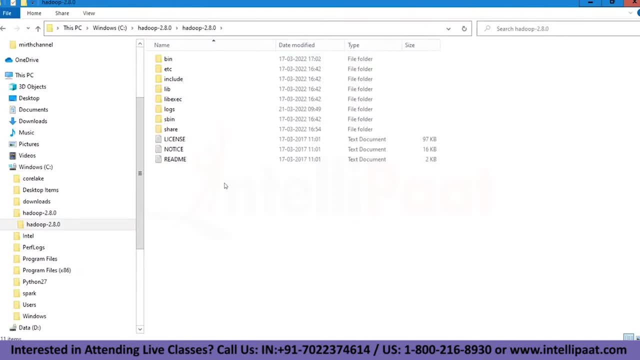 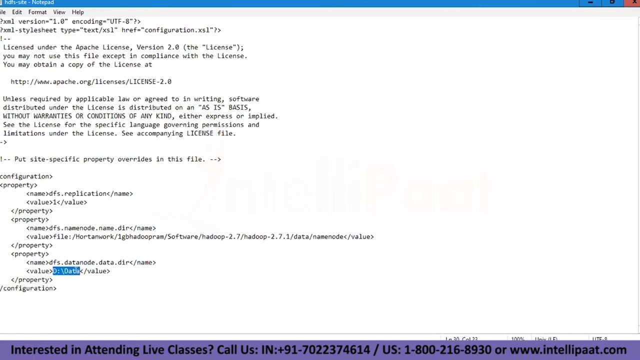 can you create one directory in the hadoop folder, inside the hadoop 2.8 folder? right, yeah, can you create one directory named data node and the name node? yeah, name, not separate. data not separated. which one? um? yeah, you can replace it um, but, but, but, what is the path that we need to give? we have to give a right path. 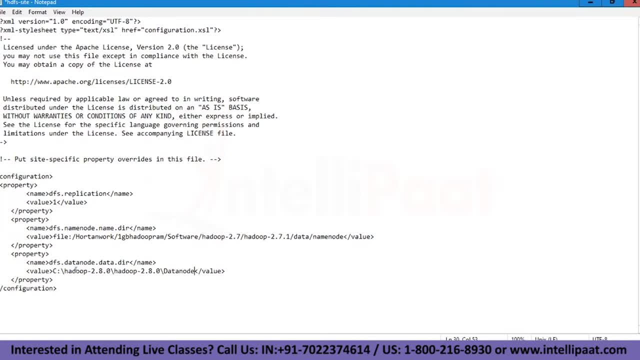 right side path, i mean left path- is not identified. actually, see, if you see the um symbol, uh, this is not a proper format of giving it. so do one thing: uh, inside the c, remove that c colon and just give hadoop 2.8 and everything in the backward slashes. 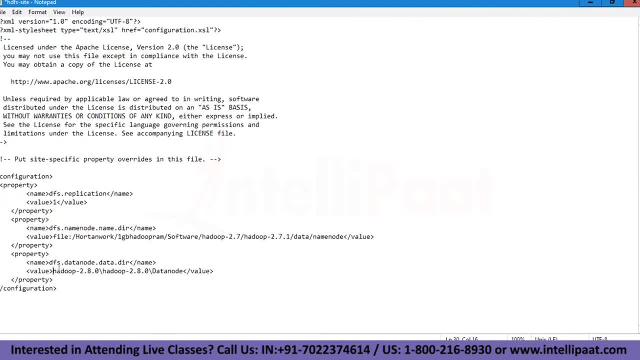 yeah, give one slash in the beginning, a backward slash. uh, this is a backward, is it then the other one forward? i keep confusing with the. and give the forward slash, then yes, and give the other slash, also here, the same thing for others. also remove and then replace it. 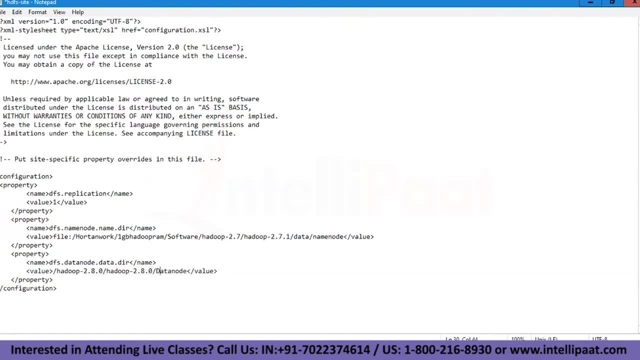 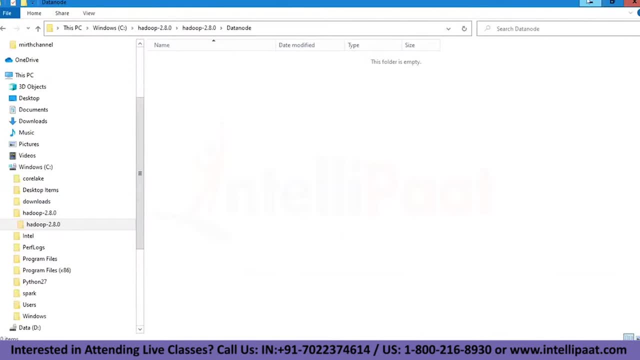 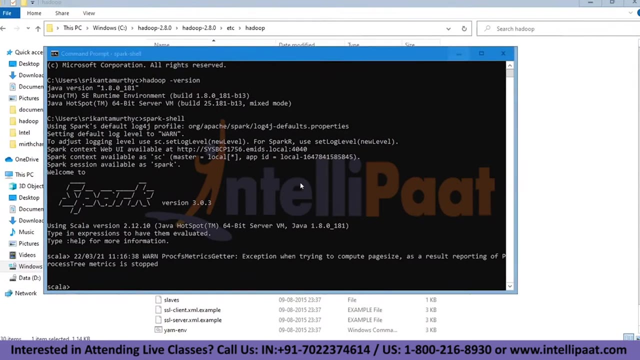 yeah, so now let's save this and then come back to the terminal, save this, save it and close, close it, close it, don't open it and close it as of when you save it. then you just have to close all those windows, no, close those notepad pages, pages. so now, uh, ctrl z. ctrl z will take you to the home page. 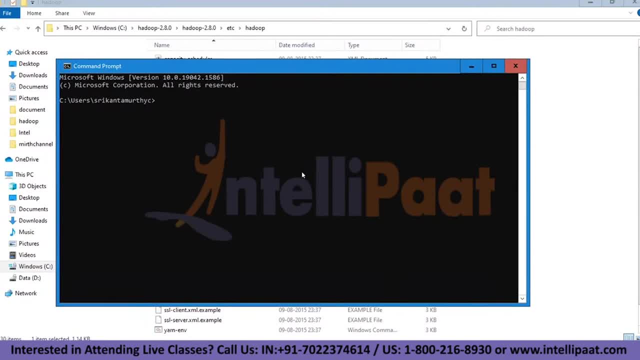 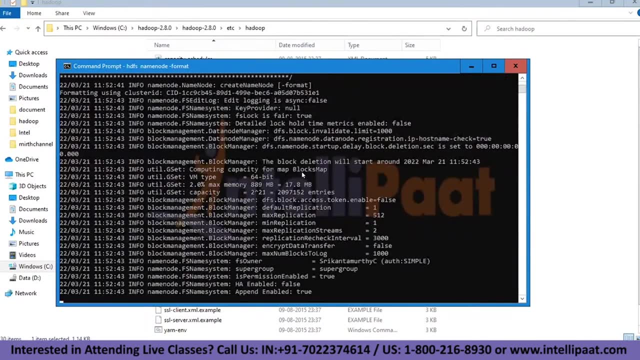 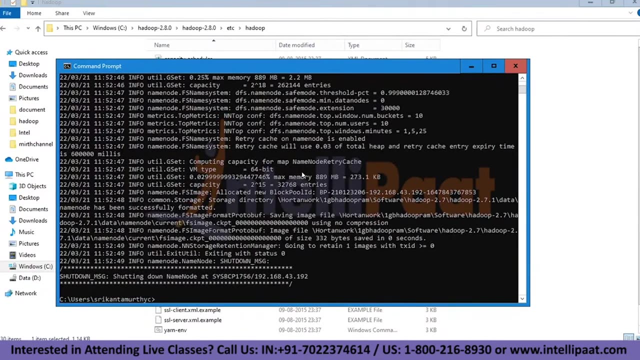 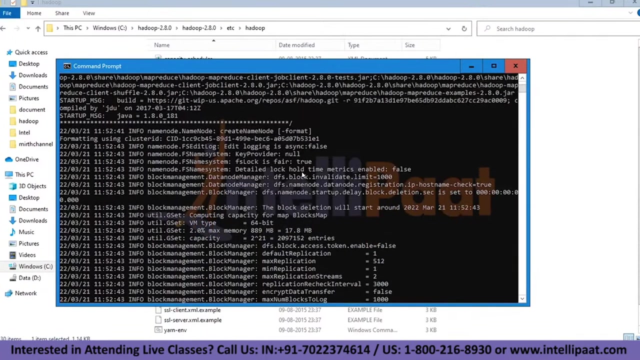 yeah, so um, hdfs space name, node space hyphen format. okay, so let's wait, let's, let's just see what is that written? anything related to the data, not block or anything. there is an error. just scroll through, scroll up, scroll up. do you see any error here? nothing, nothing, nothing, nothing. yeah, scroll down now navigate to the hadoop path. 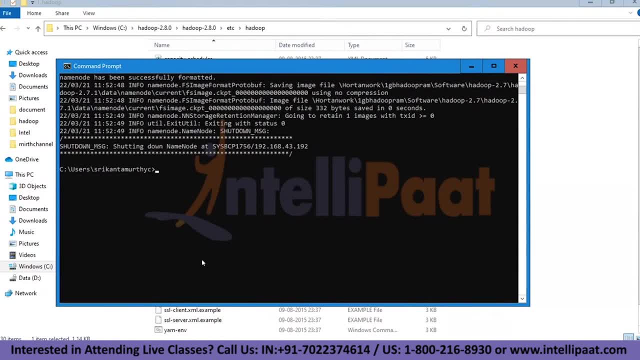 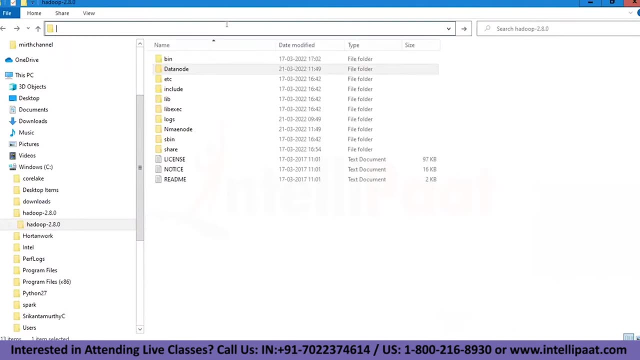 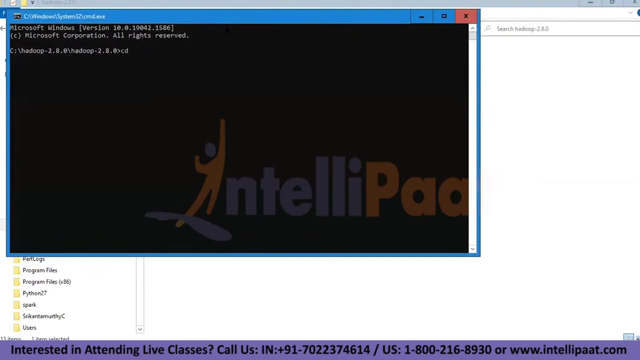 cd hadoop 2.8, wherever your hadoop is available. just do cd backslash and then come back to the home page and then do a cd hadoop. yeah, in the command line just navigate to the hadoop path. that's it. it's available on the c drive. yeah, control z, control z. yeah, do a cd sbin, yeah, sbin. 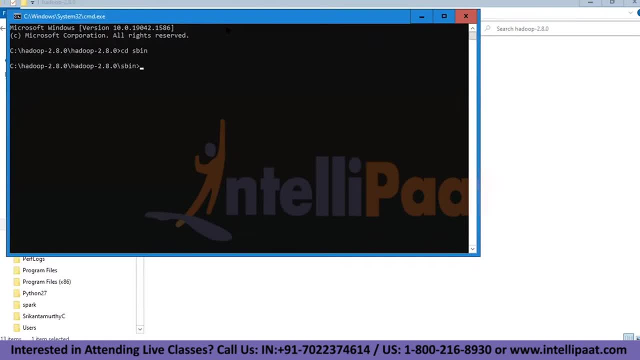 enter now: start hyphen all. uh, just put a. uh, yeah, start hyphen all. just give a tab. that's okay, just give a tab, it will give you the suggestions. it's not giving: start hyphen, all hyphen all, no spaces, no spaces. this is all single command. so that's the reason i was asking. if you give a tab, it will give you. 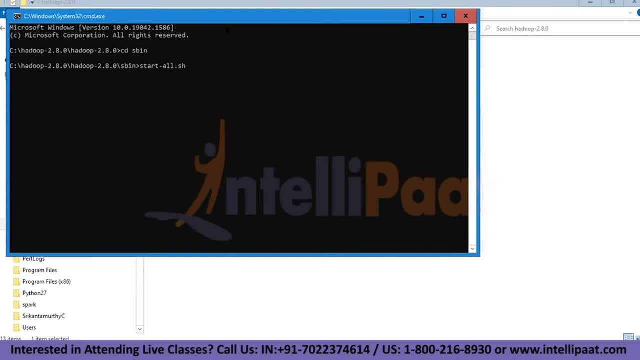 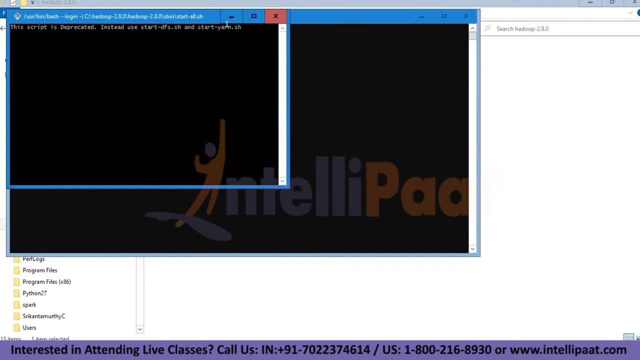 the suggestions: dot, sh. enter let's, let's wait, let's wait. this will open your terminal. so if the services are started properly, then okay. so couldn't find unload the main class org dot. apache dot tools. get configuration starting name node. connect to local host port connection refused. so this port 22. uh, can you check with them if this particular port is? 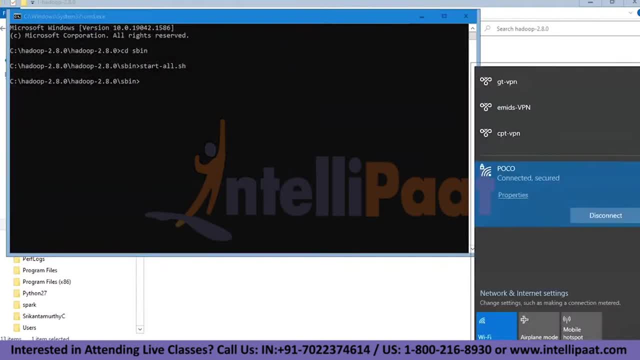 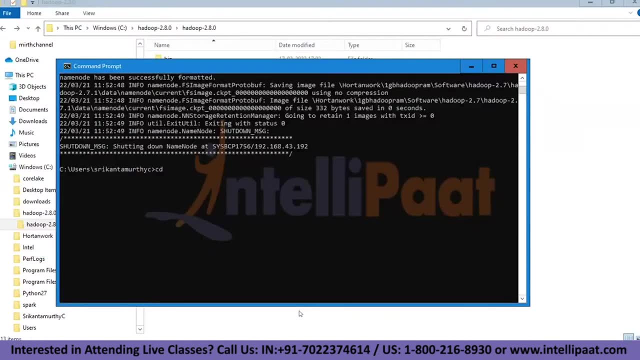 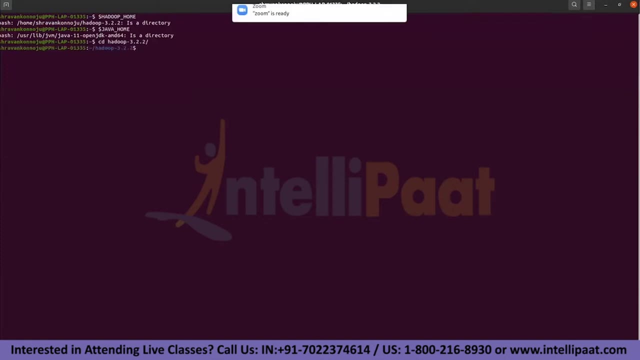 uh open or not on your machines? it's not required because this is all your local setup, right, that's required. let me share my screen for a minute. see, uh, you're seeing my screen, right? i have, uh, these folders. okay, these are files i have. so what changes i made in lset, so cd etc. and do so. you have a. 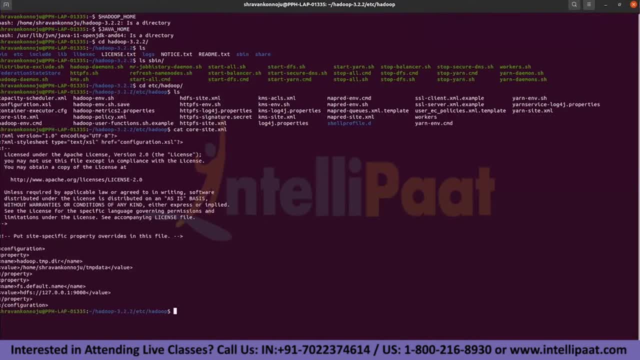 core site, right. so core sitexml. what i did is i gave the temp directory any, any. i mean that's, that's fine, i can give anything and this default name you already have with nine, nine, triple zero and the local host path and whatever the htfs. so this is same and in the htfs sitexml, what i did was i gave the path of my 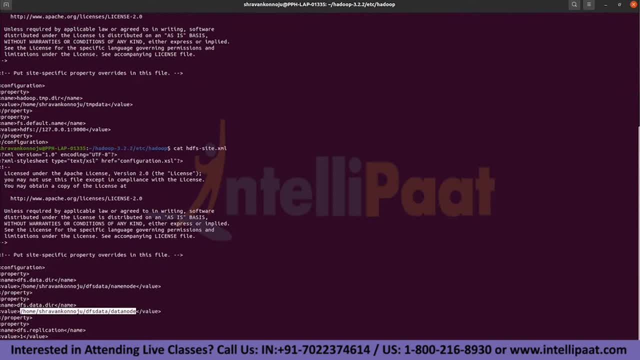 data node and i gave the path for my name node. so what is a path? some home folder in dfs data node. i created a folder named name node and dfs data node and i gave the path for my name node. so what is a data folder? i created a folder named net data node. so this is all on my home path, so whatever. 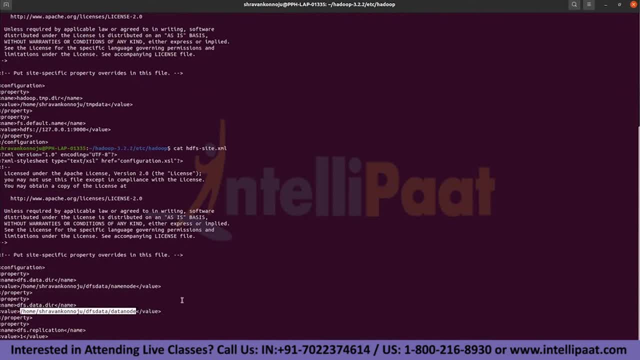 the path you give here should be an explicit path for your c drive or d drive, wherever you create these folders. okay, so in fact, you don't have to create this folder. the system itself will create it, so you just have to give this path, which you wanted to consider as a name node or the data node. 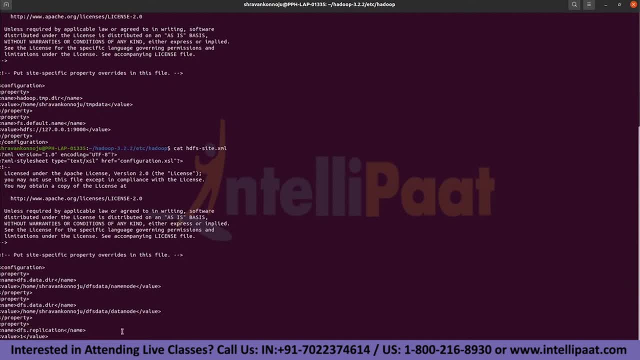 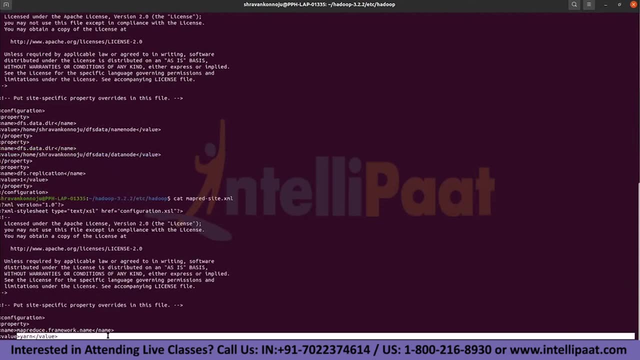 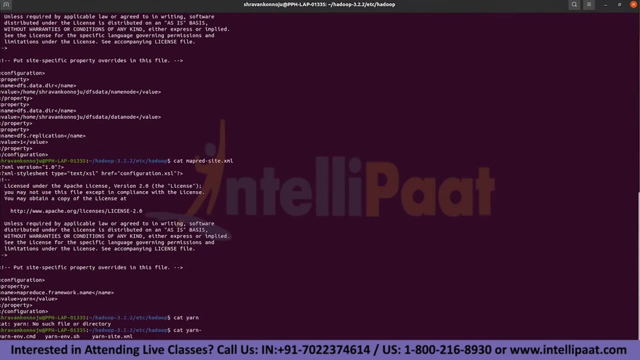 right, and the other property is the default dfsreplication- the same thing. and then i have map red sitexml, which says the same thing: map reduce framework name as the yarn. and then i have what is the other one yarn site, yarn sitexml. so here i have what this yarn resource manager. 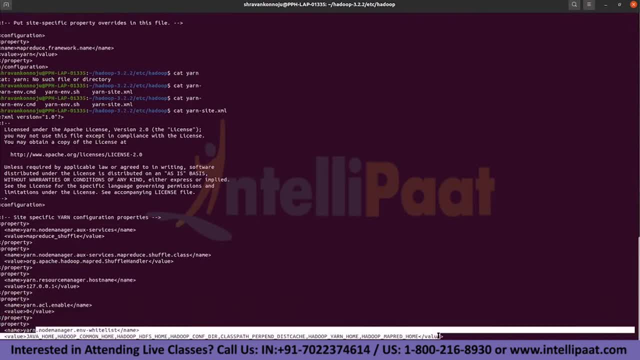 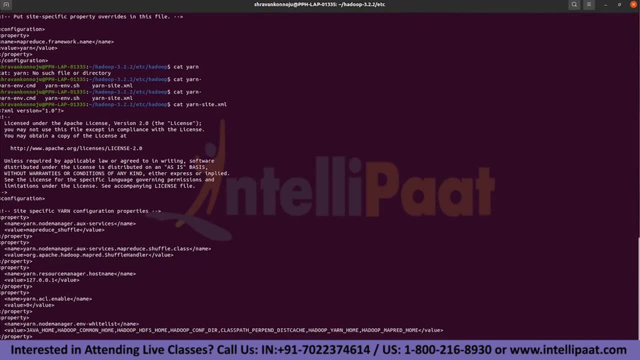 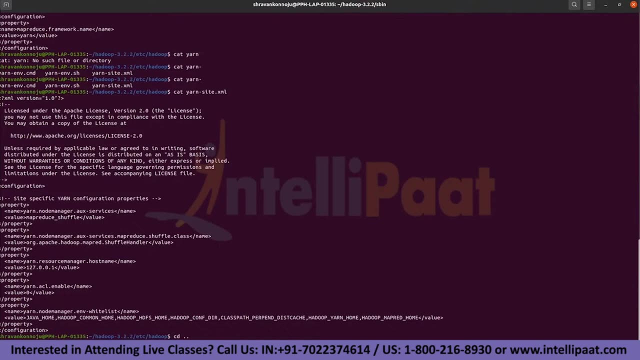 host name acl enabled and node manager whitelist or whatever. this is all fine. okay, so this is all default settings. so now what i did was, under hadoop folder, under sb bin, you just have a start hyphen: all dot sh. so this will do what. this will start all the services. 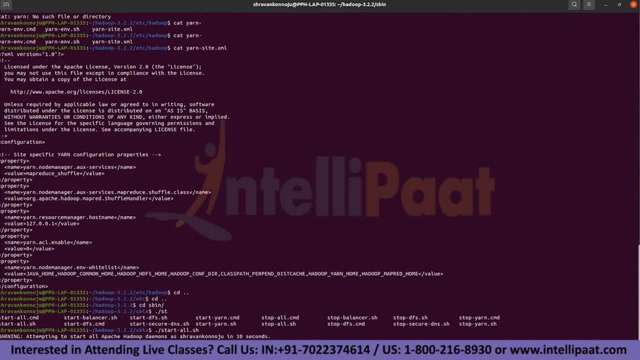 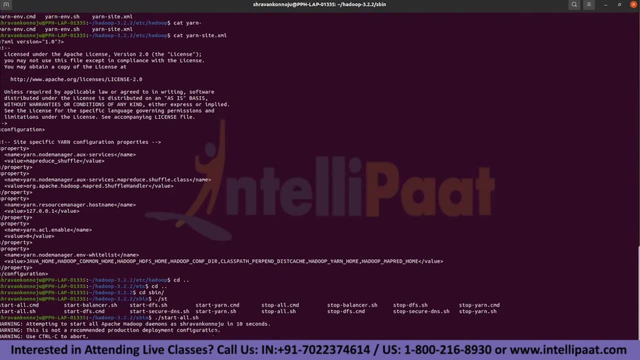 okay, so this is going to start the name node, data node, as well as the resource manager, as we have selected yarn as a map reduce framework. so starting name node. so this particular local host, i mean everything, is a local host for us, even for you and for me. 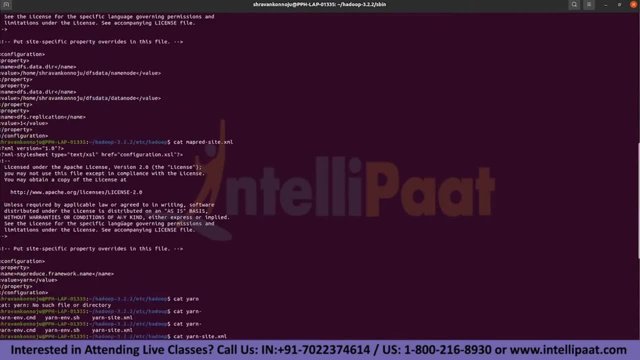 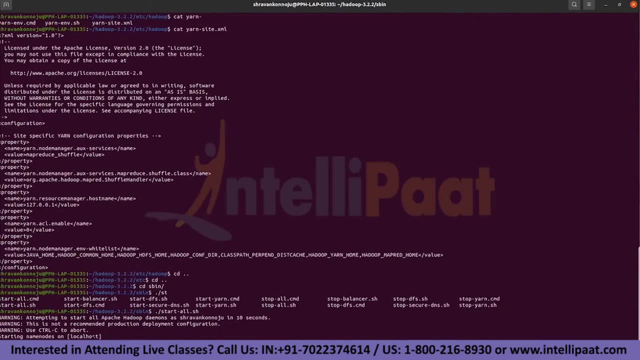 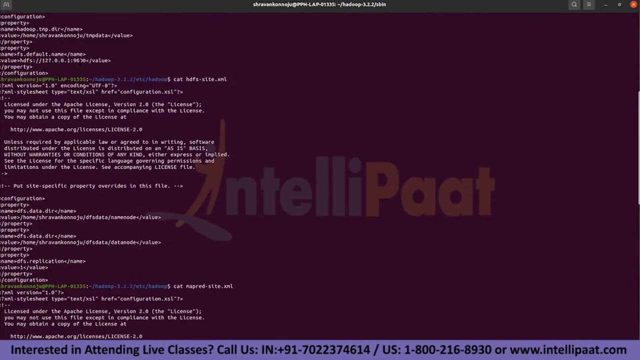 right. so it's all local host. so it's not even looking for this path, it's not even checking whether these paths are correct or whatever it is. so it's here. it will just try to connect to whatever the ports you specify. so this 127.0.0.1, so this 9000 or? 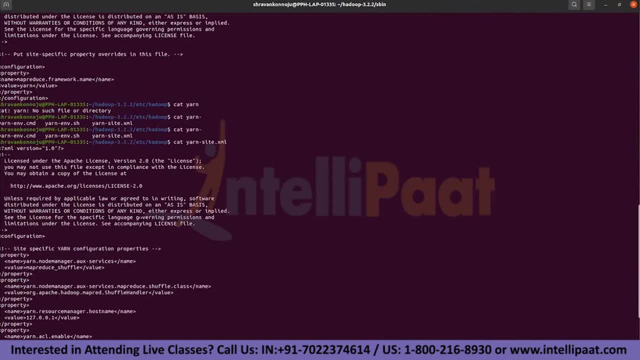 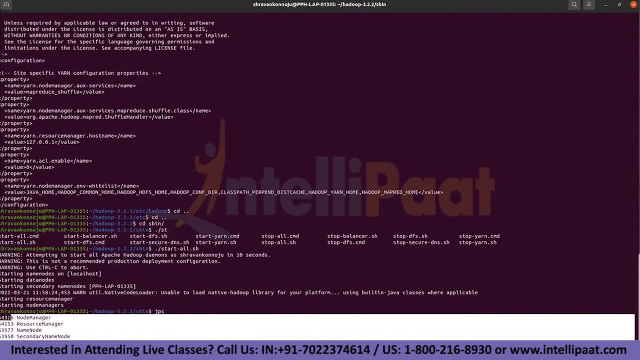 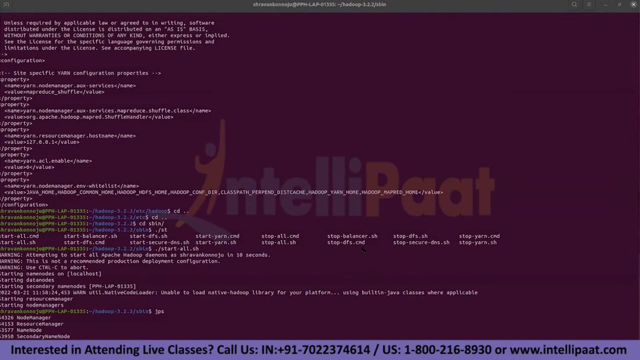 we have other other resource manager, node manager, ports, right, so it just starts connecting to all those. so when i do jps, you can see all the services that are running, and also when i do, let me see which which ports i have created. i think i think one is. let me check the files. 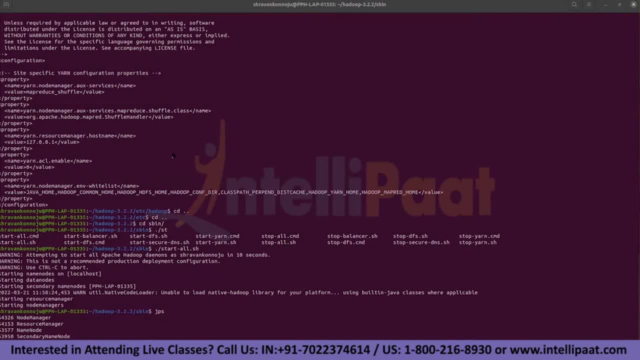 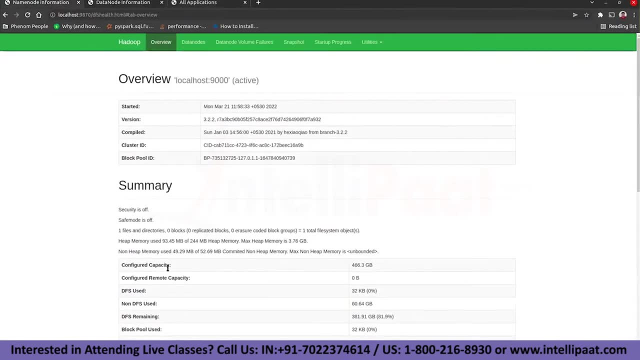 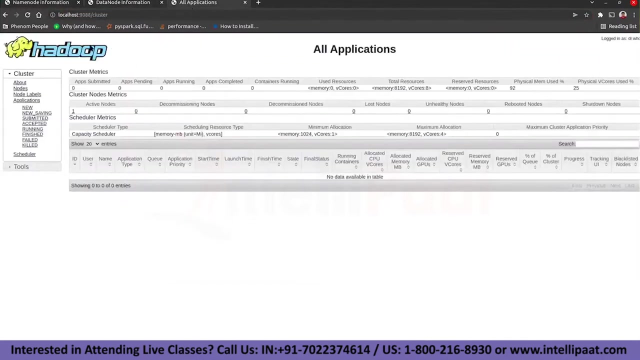 9870, 9864. right, so let me share the chrome browser. right, so this is a page i'm i'm able to load. so localhost 9870 is my. what is my name? node? the entire hdfs uh web, ui, and this 9864 is your data node ui. and, uh the yarn, all the uh applications that. 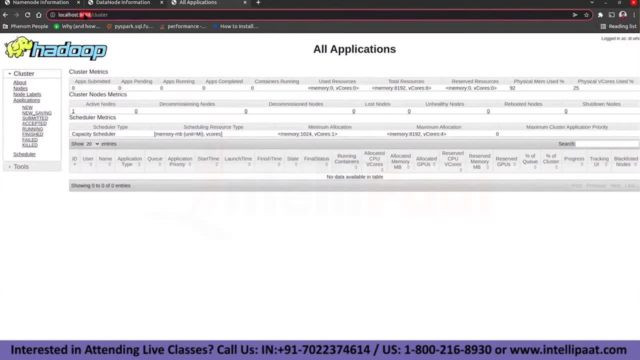 are submitted are: this is the resource manager cluster easier 8088. so these ports have not set up anywhere. i mean this: this comes default with whatever the configurations you make in the shell script. okay, so you have not made any changes to this, so it tries connecting to these ports so. 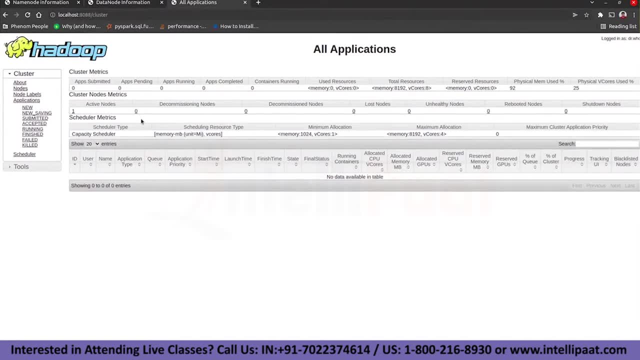 these ports have to be active. these ports have to be active. so these ports have to be active. so these ports have to be enabled on your machines. so, whatever the localhost port that is trying to connect dot 22, so that is not active on your machines, right? so when you, when you start all, 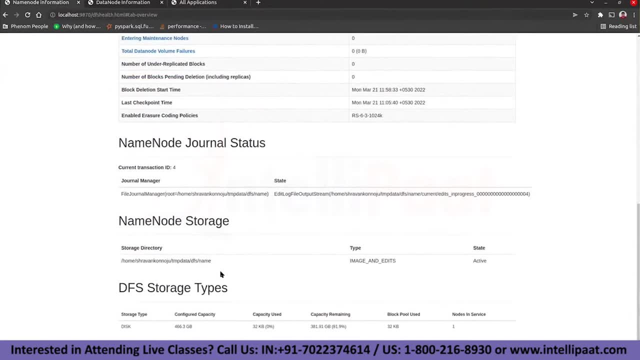 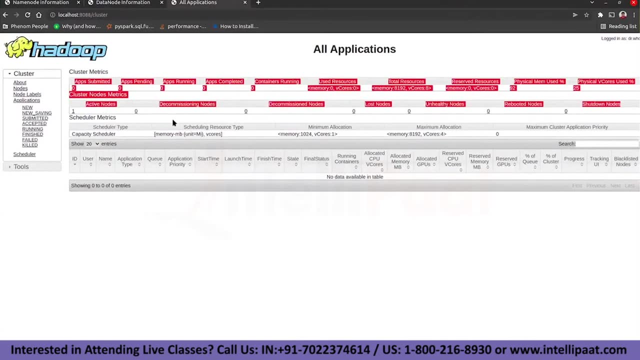 the services. you should be able to see something like this: this is your name node information, this is your data node information and this is your resource manager information. so all the applications that are submitted, whatever the existing memory you have, everything will be listed here putting it. so this is how we need to see. we need to set up. 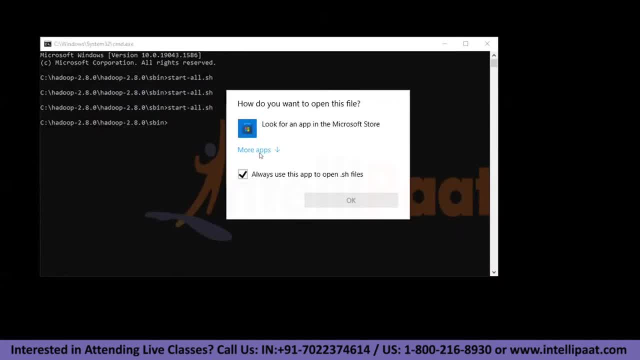 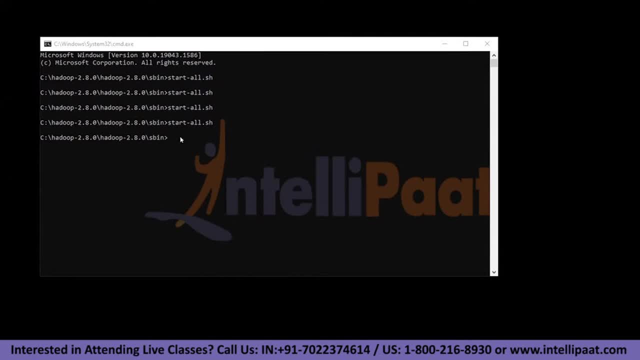 the data interface and uh, so this is how you get the data that you are using. okay, so live jobs, you can use this app. just open the uh chp file. uh, just select. select more apps. just open the uh cmd- just more apps. so do a select. start already, once tomorrow. apparently submitted ones. 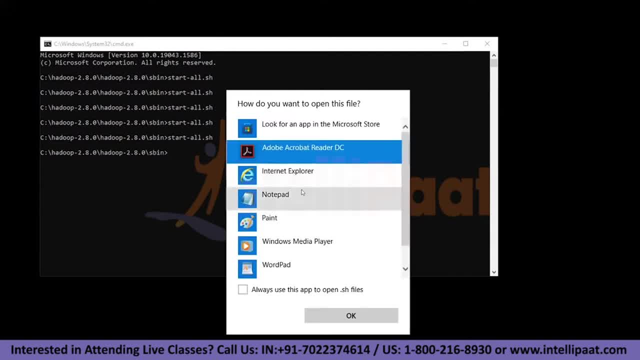 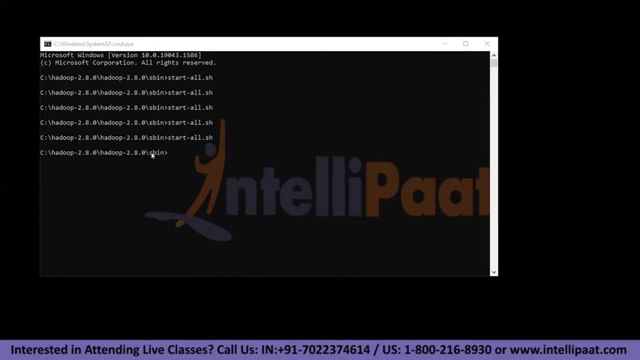 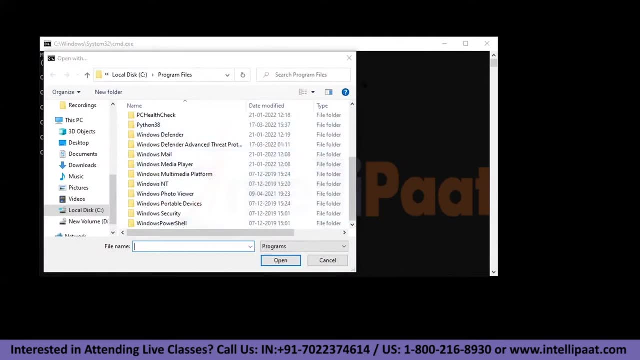 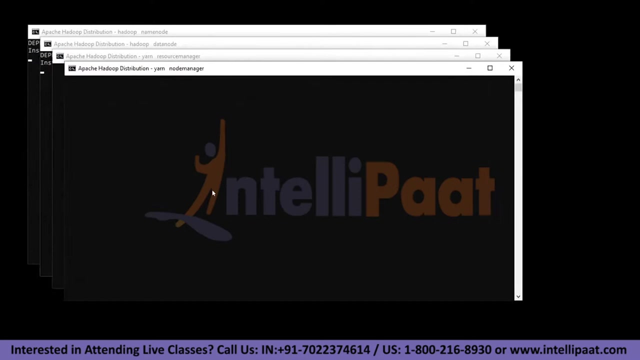 enter. you uncomment this. always use this app to open such files. just click ok. now look for another app in the pc. navigate to the cmd command prompt, cmd. start all at cmd. oh yes, so just go to the name node. what is that you are seeing? so this has some issues. scroll up. you said you are able to open all these things, right. 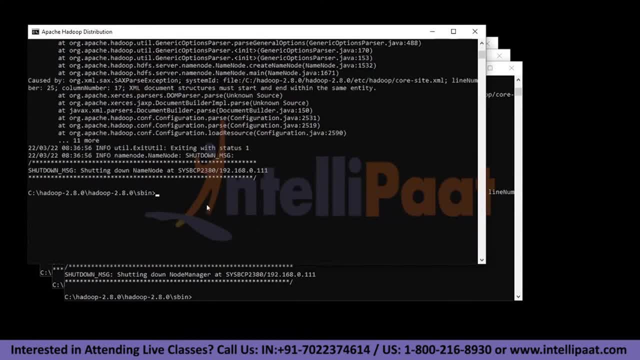 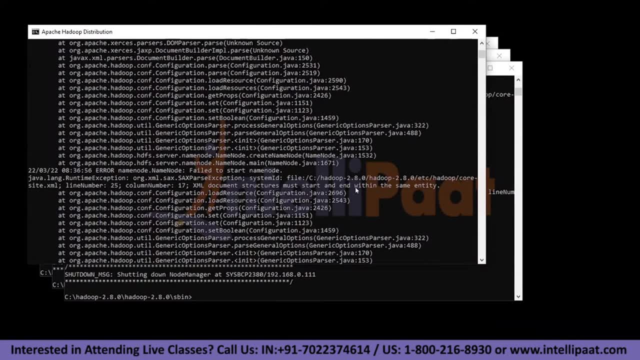 scroll up. scroll up. there is an error message there, right, right, so file. this is not a valid structure. so there you. you have specified htfs site xml files, right? the location that you have specified is not in a proper format, so file three columns followed by c, um, hadoop and all. 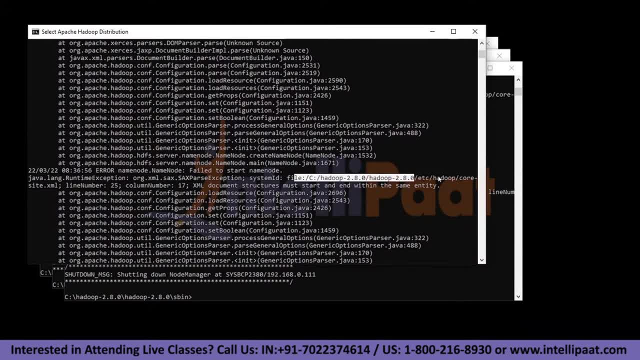 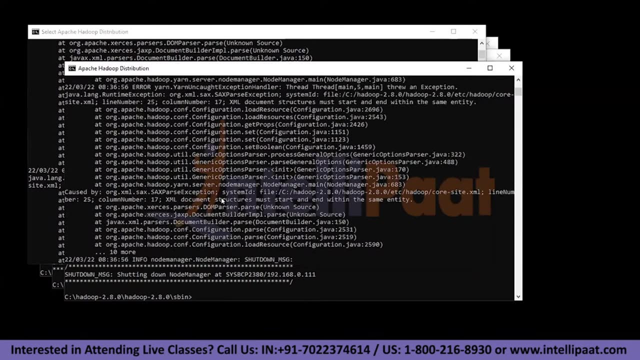 that you are supposed to give. okay, so that property, you can change it and let's then rerun the name node. okay, see, see if you have started the other services properly: the resource manager or the secondary node manager or whatever. so this is still having a problem. close it, close this, yeah, so check the other one. 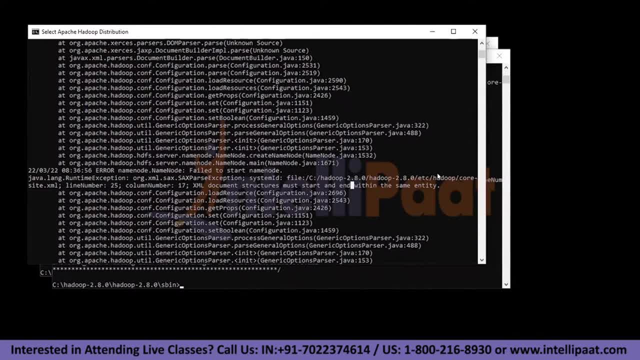 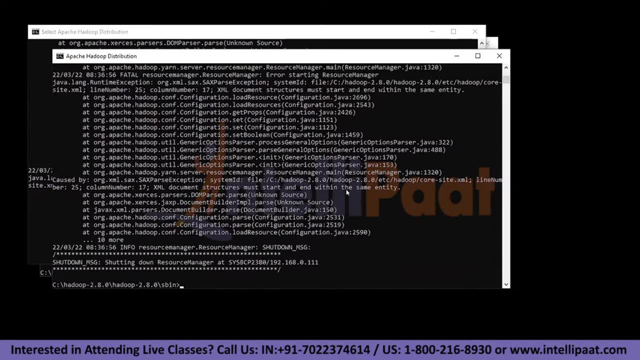 everything has the same problem: file c: hadoop. so if you resolve that issue, then the the uh, the problem is gonna get resolved. so you can see. right, the proper file name is not specified. so in in uh, htfs, i dot xml. the data directory you have given like this: this is: this is not a proper. 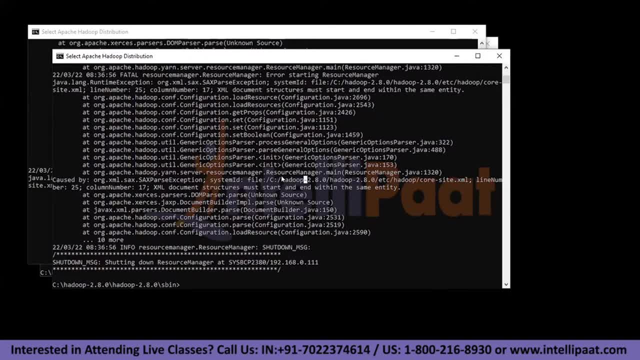 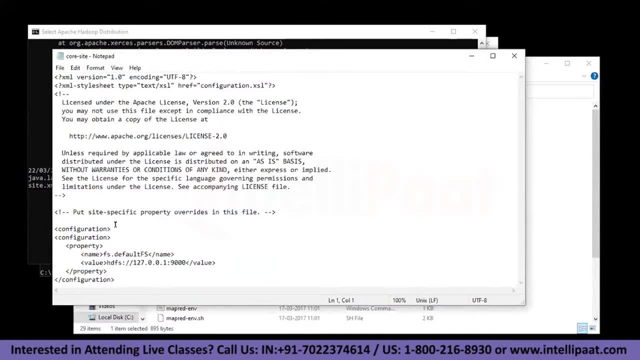 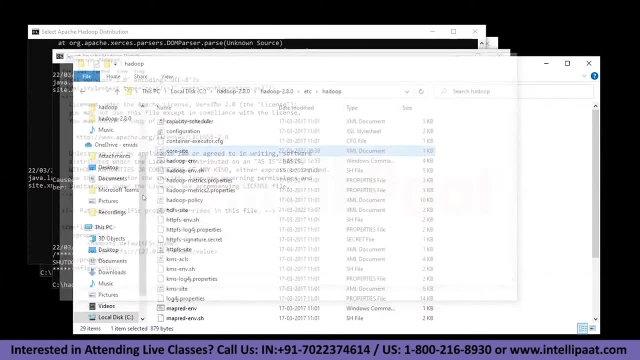 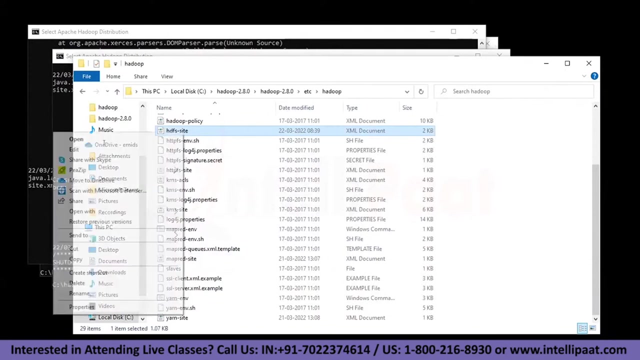 so what is the error? default fs, hdfs, local force, multiple zero, first line. just remove our configuration and then save it and then start again. i don't think there is anything here. everywhere you have the sticker configurations. scroll down. there is okay, yeah, yeah. so it has to be an opening tag. remove that slash there. 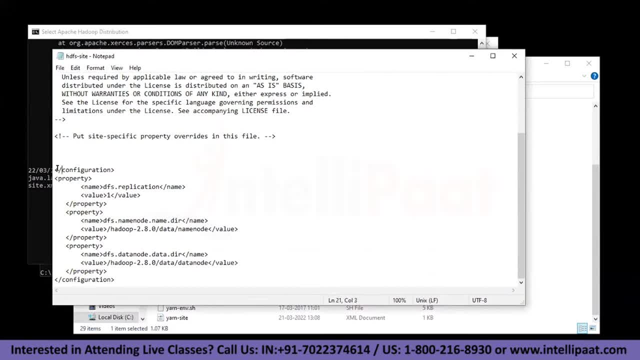 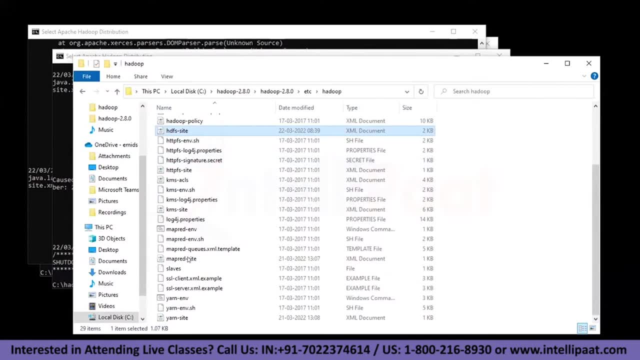 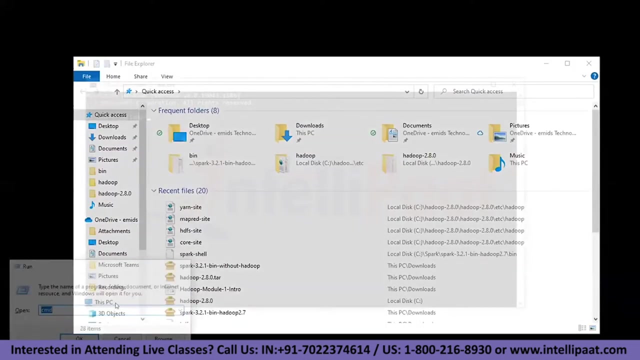 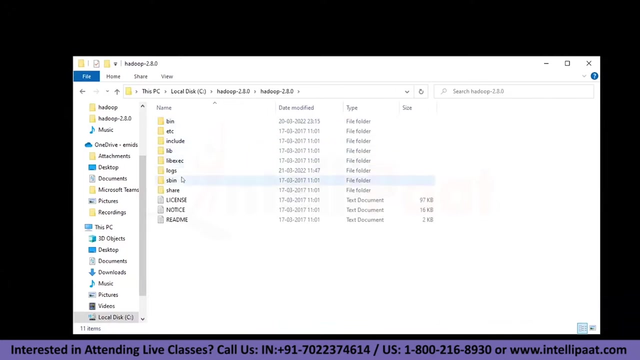 this one. yeah, remove that slash, map red and yarn, remove all, close all these windows. no, no, no, this is fine, this is fine, the last one. whatever he edited last. now, that has to be closed tag, only no, before that there will be open tag. can you open that yarn site xml once again? just do start hyphen and then tab. it will come, it will. 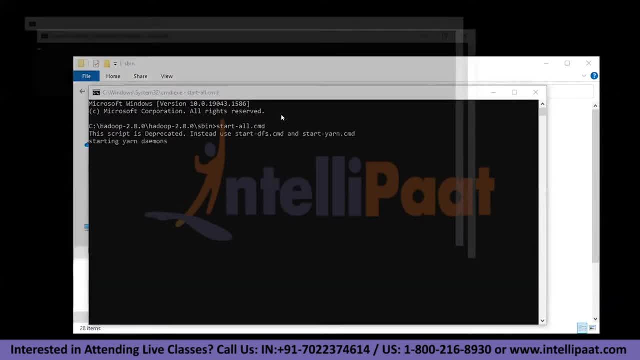 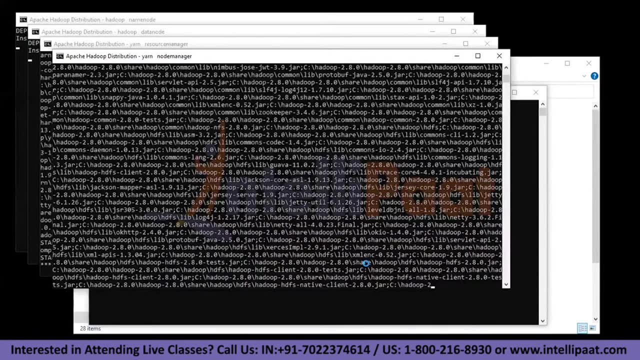 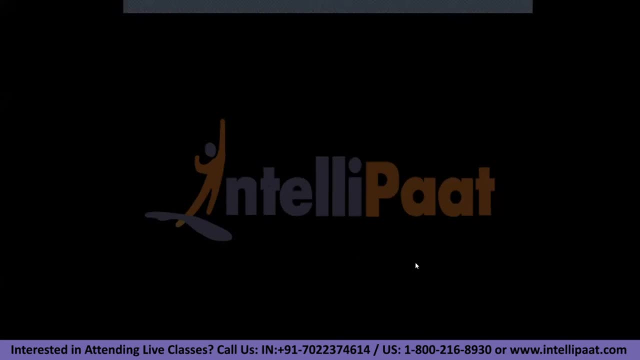 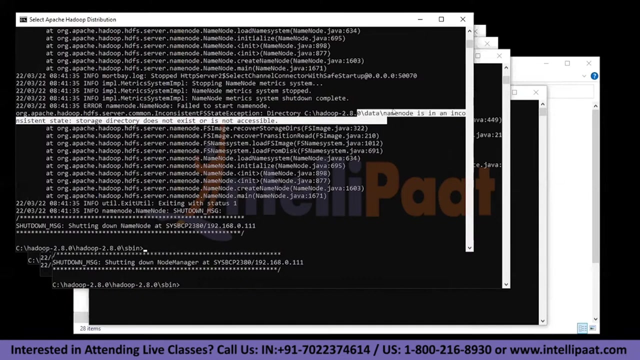 pick you up. yeah, just to submit it. just check the name node, allow access. let's ask you for the admin again. again, cancel it and go to the name node window. why is it asking for java related thing? see date hadoop data. name node: an incorrect state. so storage directory does not exist or is not accessible. so whatever the data, 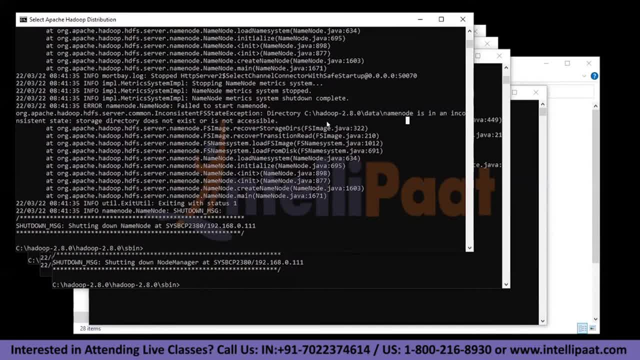 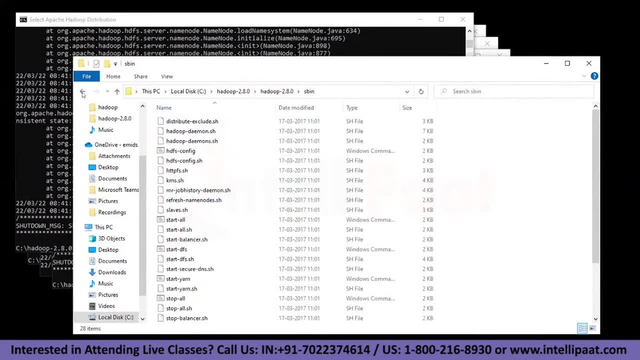 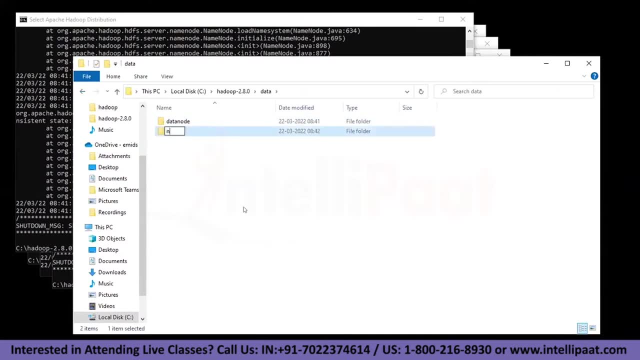 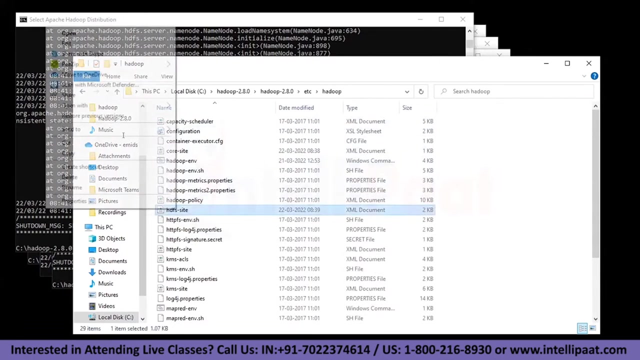 directory that you have specified. this name node folder is not created. you check once. see c drive. c drive: yeah, data here. data name node: yeah, and uh, can you go to the um? what is it? hdf set xml once. what is the format that you gave, etc. hadoop, hdf set xml. in which format did we give the path? scroll down, add to 2.8. data name node. 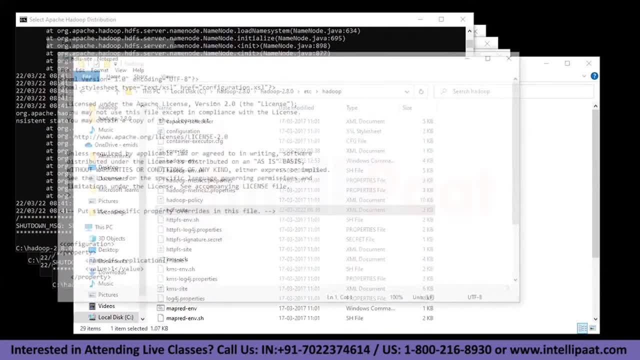 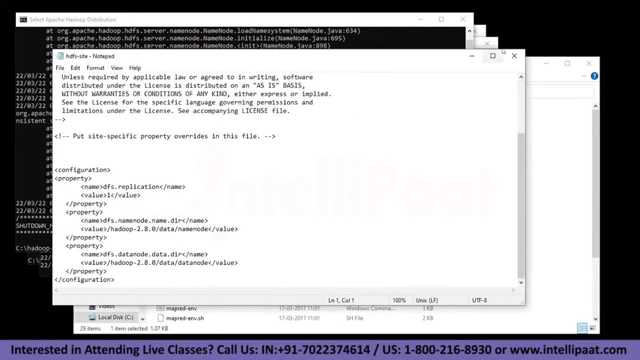 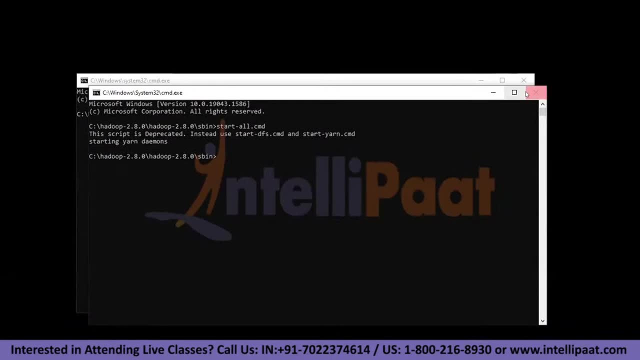 HADOOP 2.8 data name node. so this is something like this. so now let's see how to do it. okay, this is a proper format. fine, let's see, just submit it once rerun. so resource manager has been started, i guess? right, remove the previous back, the one on the back. 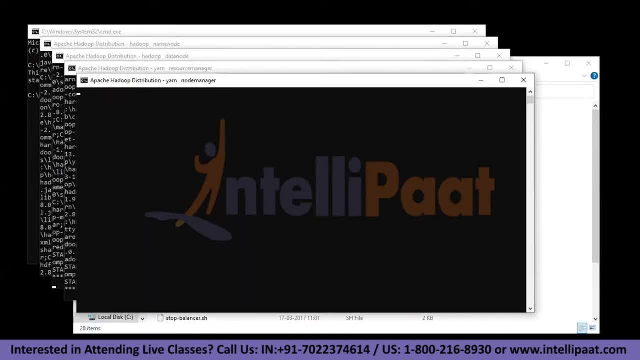 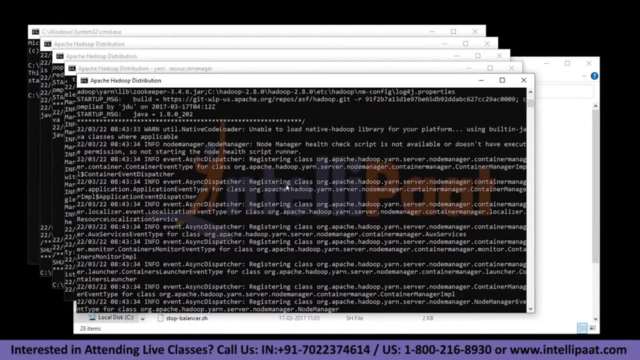 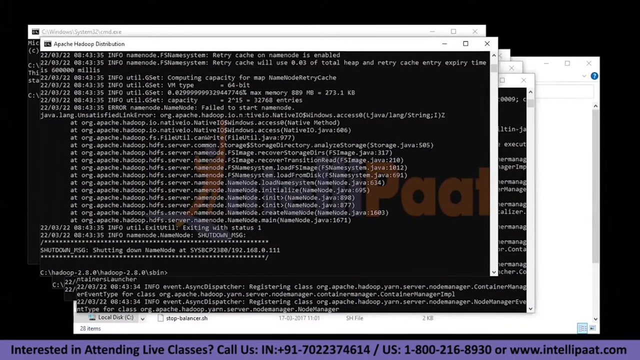 okay, fine, go to name node. what is the error here? unable to load hadoop native platform. so this native library platform has been not loaded, so go to hadoop name node first. what is the problem? fail to start name node. scroll up. this is an error. so native i o windowsaccess. 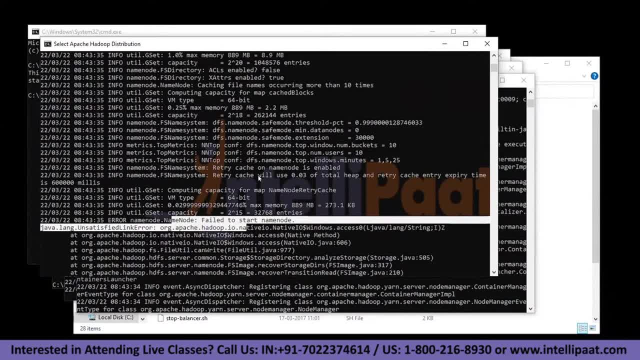 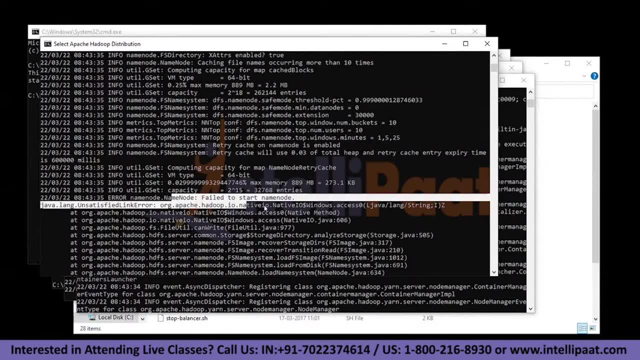 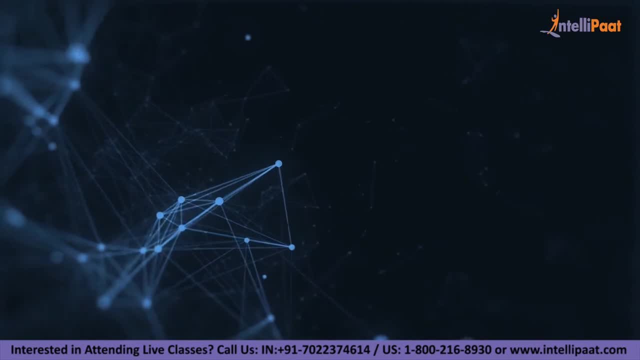 so did you? um, did you update this orgadaptationhadoopionative library in the one second? let me give you that parameter. there is one more parameter that you need to update. just a quick info, guys. if you want to make a career in big data, then intellipaat provides. 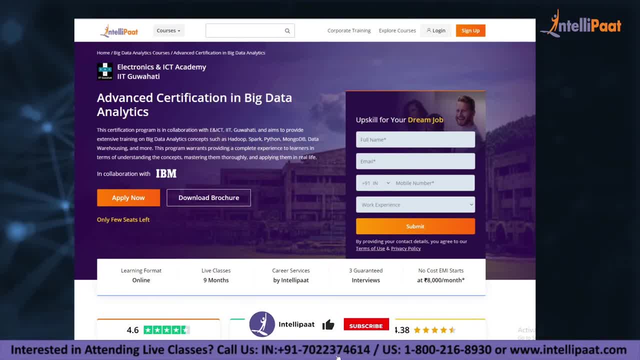 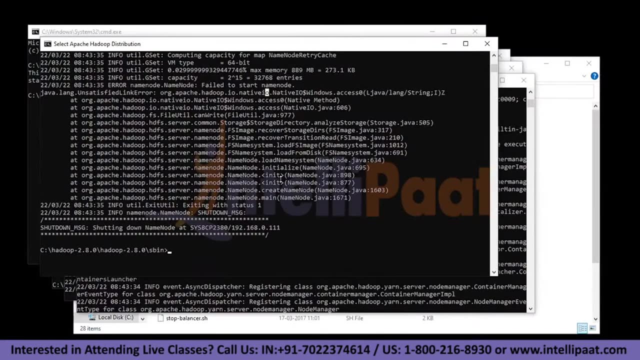 an advanced certification in big data analytics by enict council iit guwahati. it is taught by iit professors and industry experts with more than 10 years of experience. this course is designed to upskill and land your dream job. now let's continue with the session anyone else is facing. 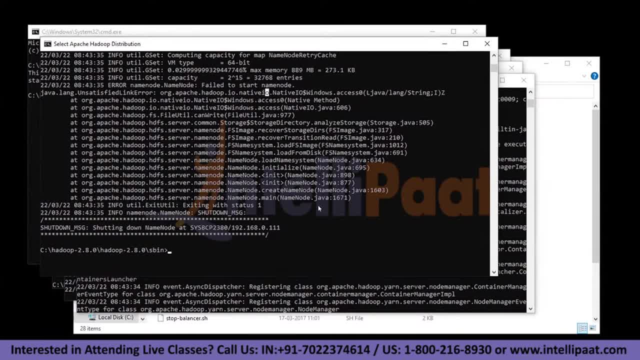 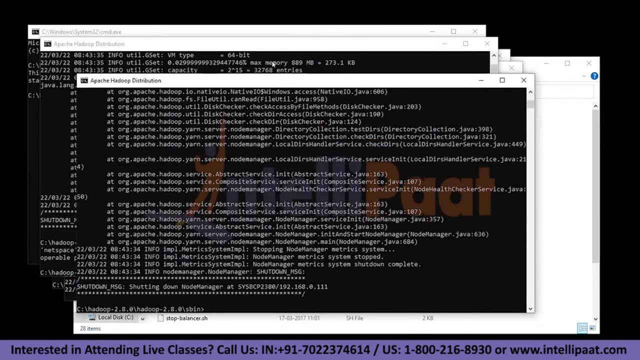 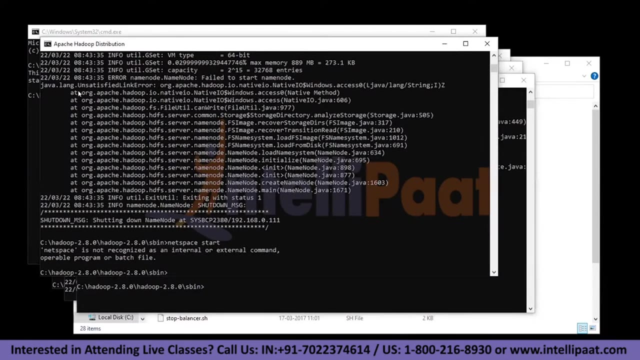 this issue. so can we do next, space start and uh, just see what are the services that are being being used for by port 22.. so can you do? um, uh, yeshwan, can you go to the home page? yeah, hdfs space name, node, space hyphen format. just try same window, whatever window you are in. yeah, just submit it here. 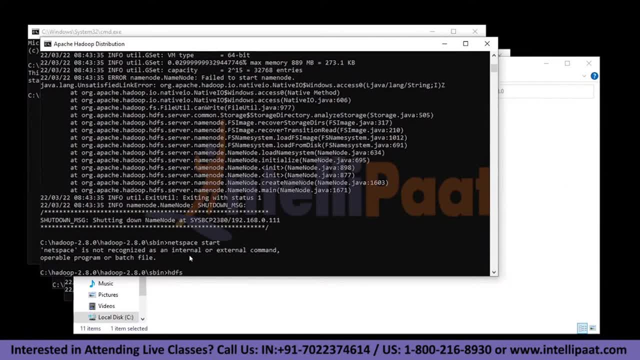 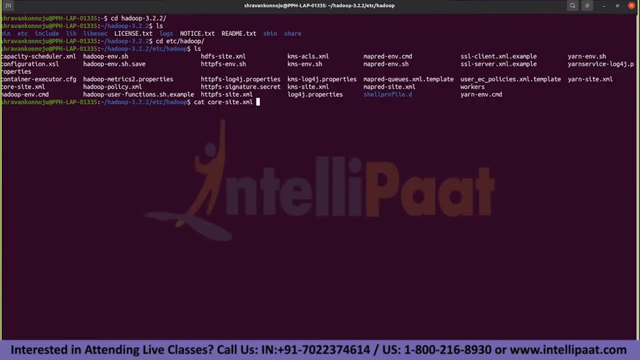 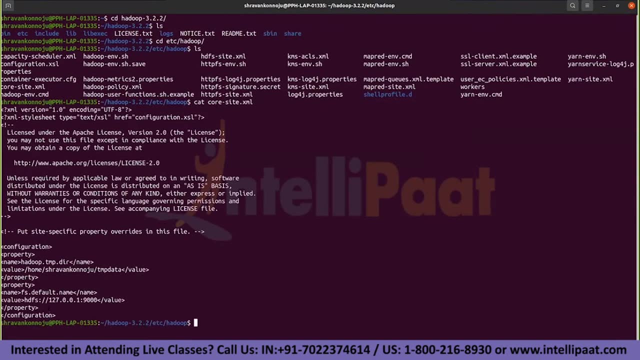 hdfs space. yeah, so with port 22, just check what are the other applications that are out there running hdfs space name, node space hyphen format. so there is nothing that i have updated in the core site apart from the temp directory and the default name, fsdefault name, which is the 127. the 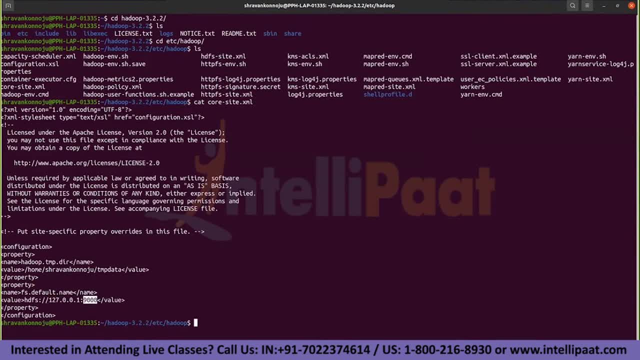 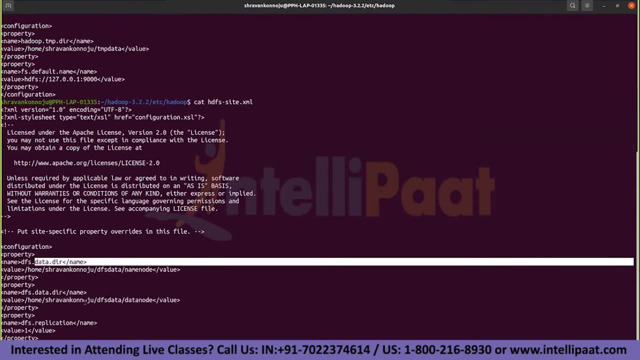 localhost 10, 9, 0 and similarly. i'm just showing you what are the parameters that i've updated. so, data directory, you update some location in your local file system, data dir and the dfs. data dir1 is the name node and that is for the data node and the dfs application. this is a 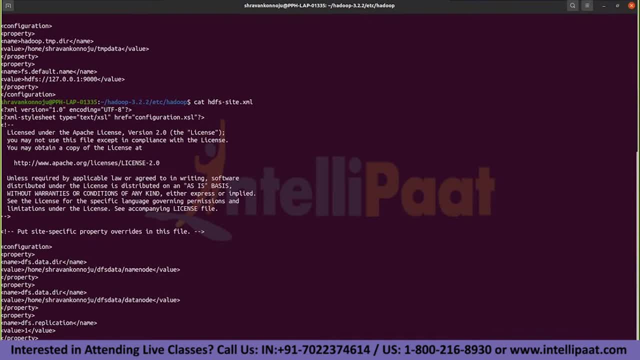 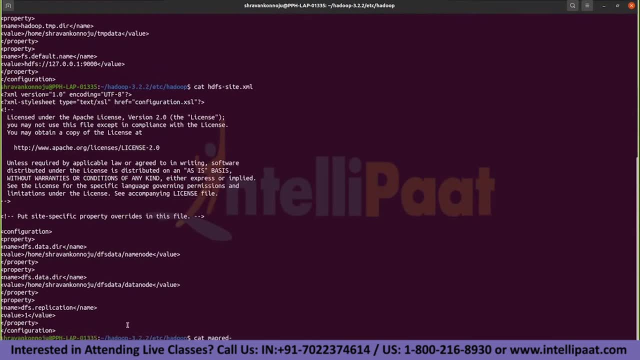 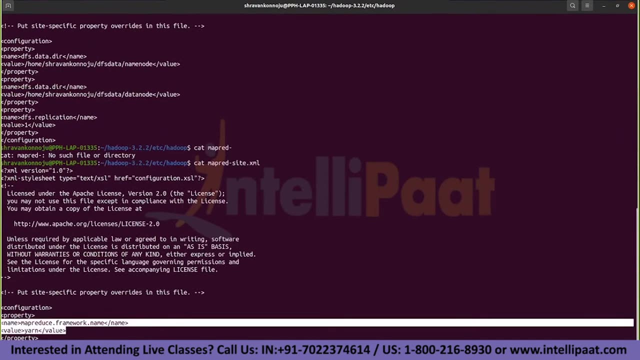 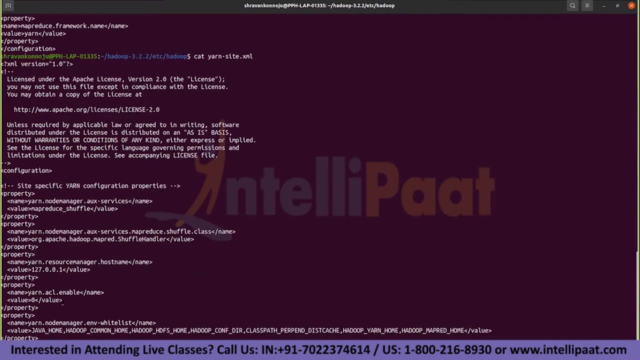 mandatory parameter for you to update, and similarly so map rate site xml does not have anything else. map reduce framework name is yam. this is the only parameter that you need to specify, and similarly with the yarn site xml as well. okay, so where is it this one? so resource manager host name and the acl enable. 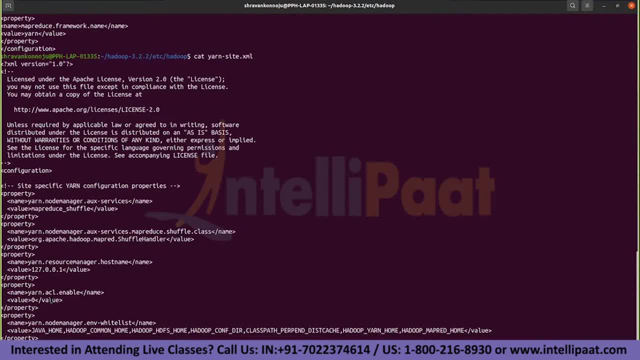 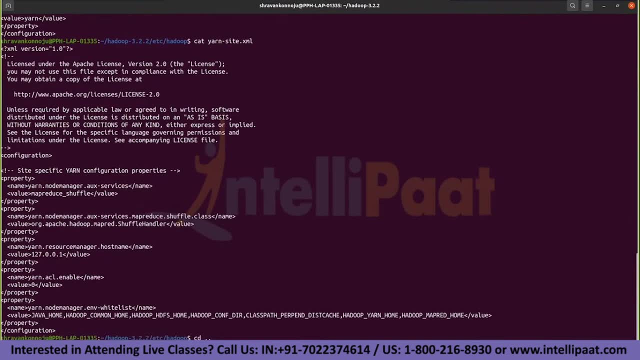 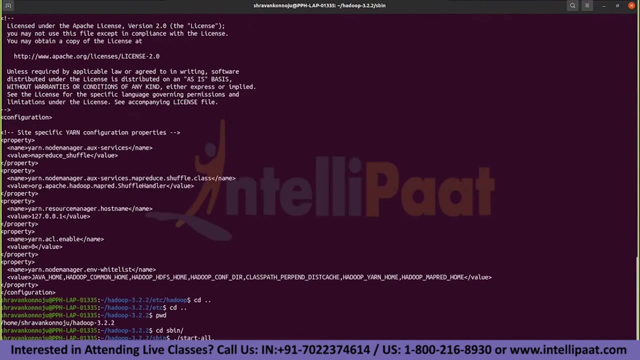 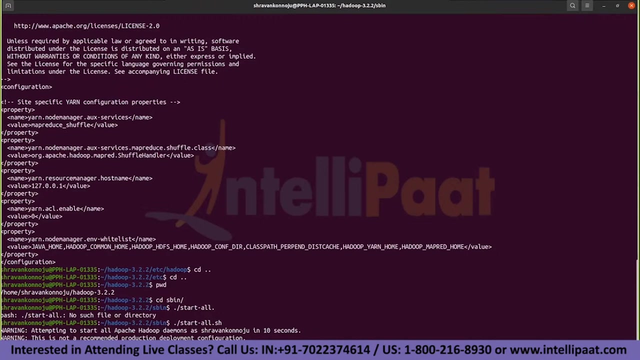 zero. so these all properties i i gave you in the chat yesterday. so after you update all these properties, uh, i'm navigating to sbin and then do a start all, not message. so this will start all the services and also in the other window i'm going to show you the files that are getting. 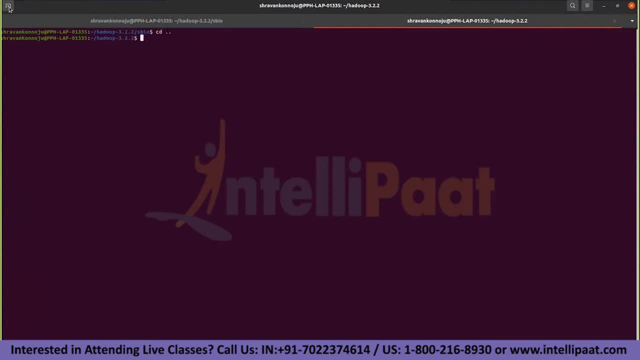 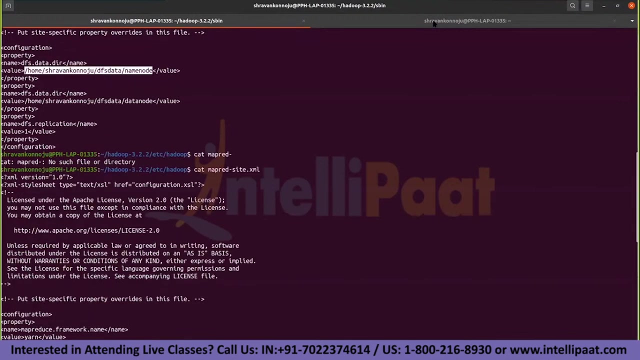 created cd, had to cd and cd. and what is that? what is the path that i gave in name node and data node from dfs data name node, right? so there should be a folder named dfs data under which you have data node. so after you start the name node and data node, when you load some data into the name. 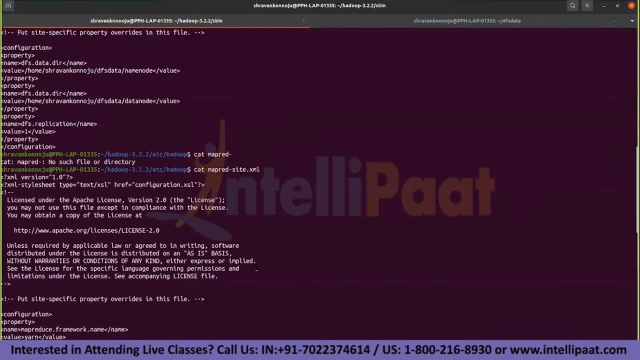 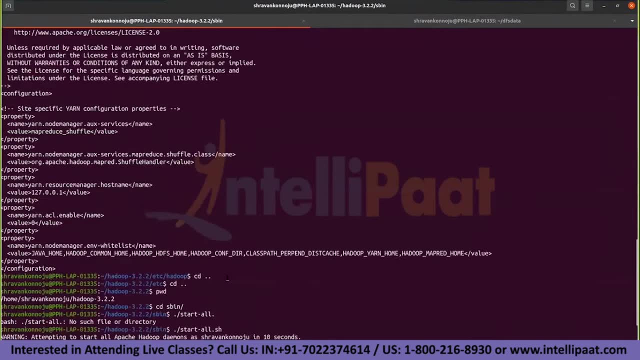 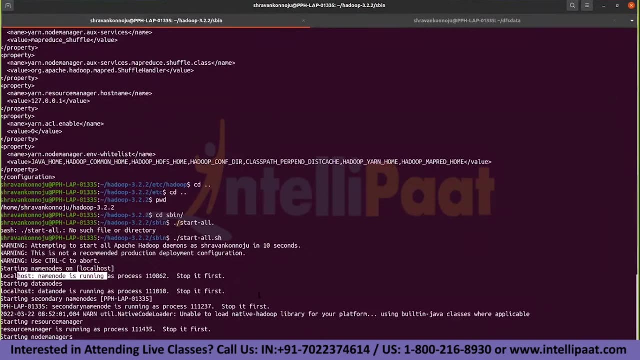 node also it's gonna get created. a name node folder also will get created, okay, so now that i've started all the processes, so it's all running, i mean all the processors are already running. i have not stopped it, so you can just do jps and this will list you all the services which it is holding. so name node. 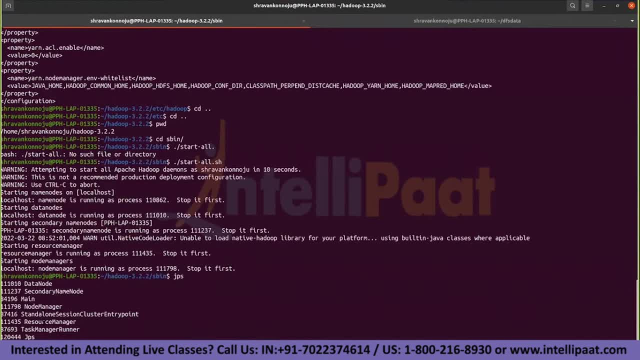 secondary name, node data, node node manager, resource manager, task manager and then the name: okay, so all these services are currently running. so now what are we supposed to do? yes, same same thing. i mean start, all dot search is is same and uh. so now what happens is: you will see if at some point javascript is used or if there's a 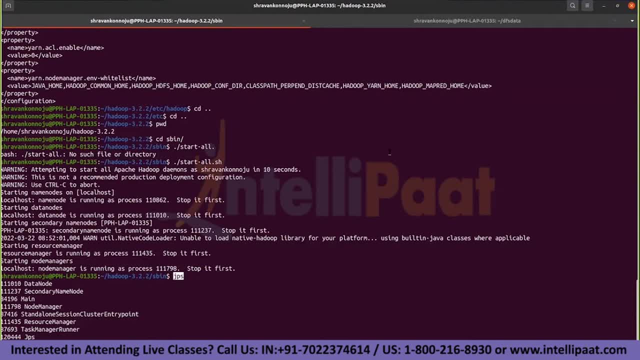 for this. so this is the javascript that is running. so javascript will may be the jps might not work. if you have not, if you have not set the proper java home, storage is everything else. i mean wherever you have the c drive, d drive, and what of the storages? 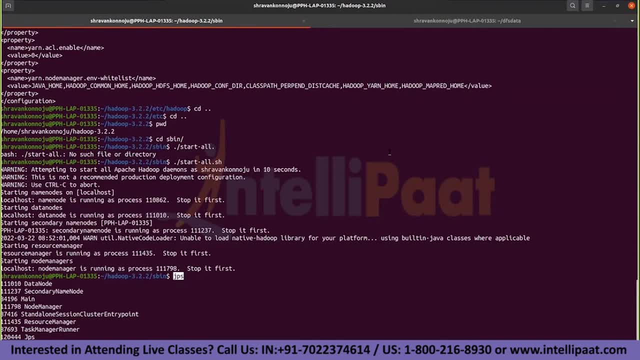 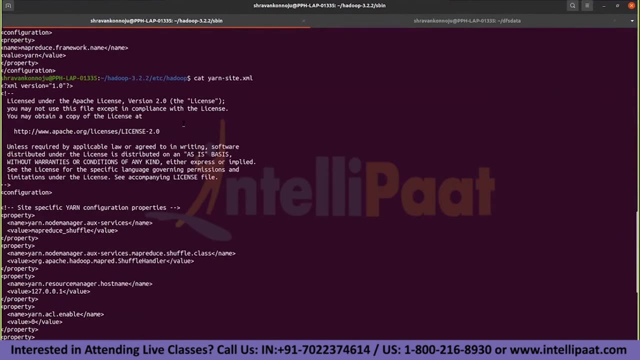 you have will be your local storage, and the hadoop hdfs storage is something which is only the location of this particular data block. this is where here, right so this is the data directory i have specified, right so only this particular portion is your hdf hdfs location and rest all. 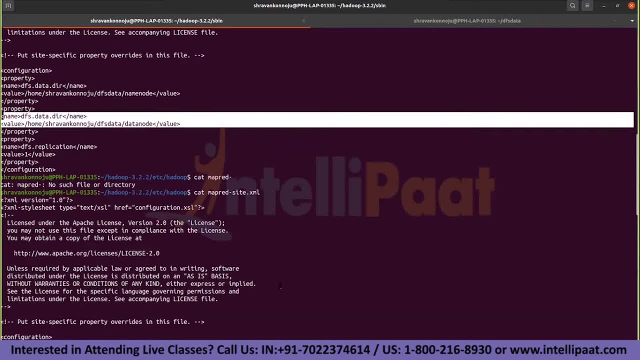 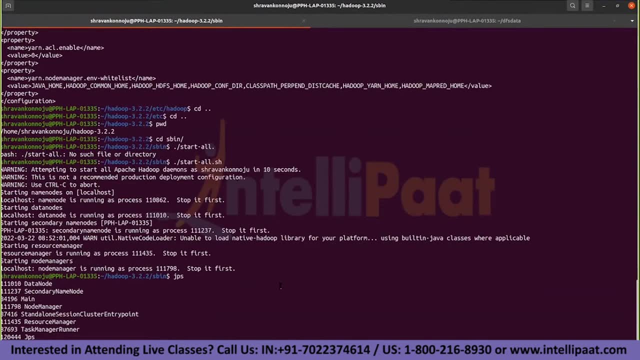 your local file system. so, in in case, if you, if you configure a cluster right, if you're having a multi-node cluster, then also you, you are supposed to update the worker configurations or the data node configurations, the ip address of different missions in the data node folder. 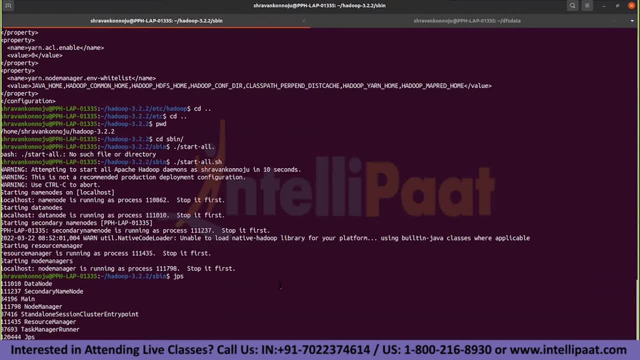 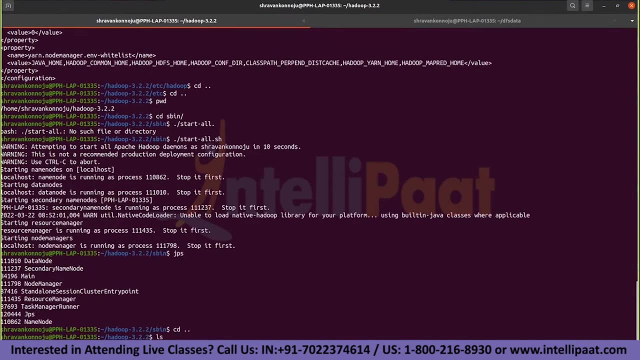 you have to create a file name called as a data node, or workers or slaves, under which you have to give all the uh ip addresses. i can show you that as well: cd, etc- i'm sorry, ls, etc. do we have any worker files in this? so cat, etc. workers. 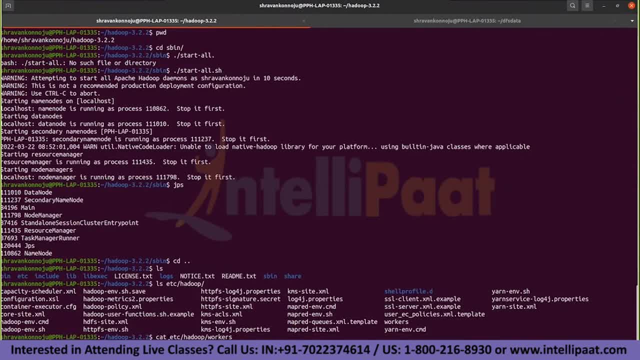 so under cat it under, etc. hadoop, there is a file name called as workers here. right, so what does this mean? all the ip address, whichever you have, which you want to consider them as your slave nodes, have to be provided in this particular workbook. okay, so this will be read by your start command or the name node: name node dot. start dfssh command. 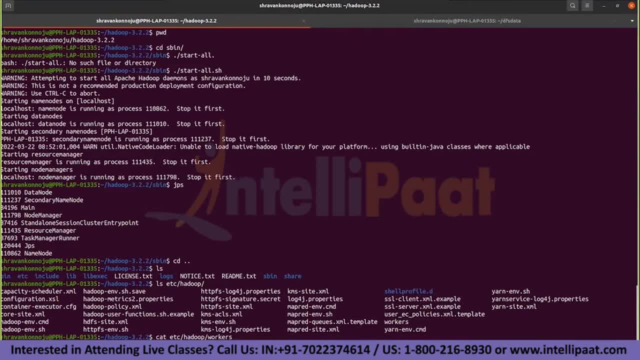 and it will read all, it will identify all the ip addresses which are available in this workers file. okay, so when you are- i mean not now, but when you are- dealing with multiple nodes together, when you want to configure everything together, when you want to configure a distributed cluster with multiple nodes, 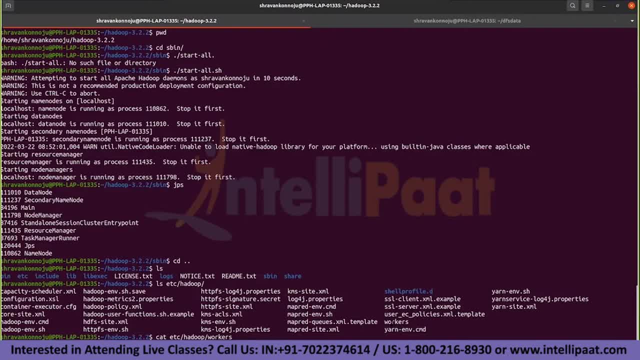 then you have to specify all the ip addresses in this particular location. okay, so, from where you will, you will pick your hadoop will pick those machines. so in that case, your data directory will will be spread across these multiple worker machines. okay, so it's, it's gonna be something. 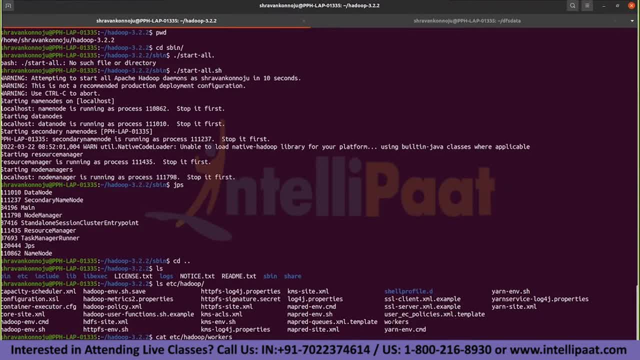 like data: one directory, data two directory data, three directory. you can also specify multiple data node directories there. okay, so that's how we will be doing, and after you have successfully started all the services, so let's get started with the hadoop hdfs command. so hdfs is the 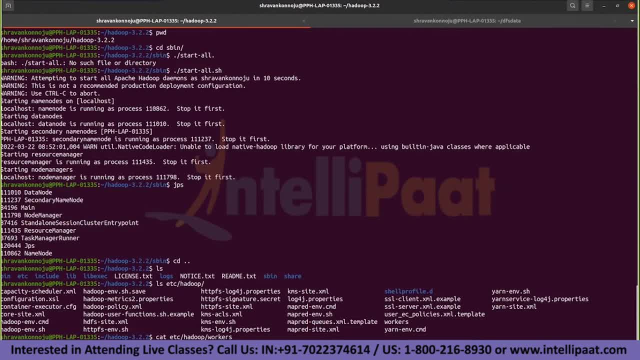 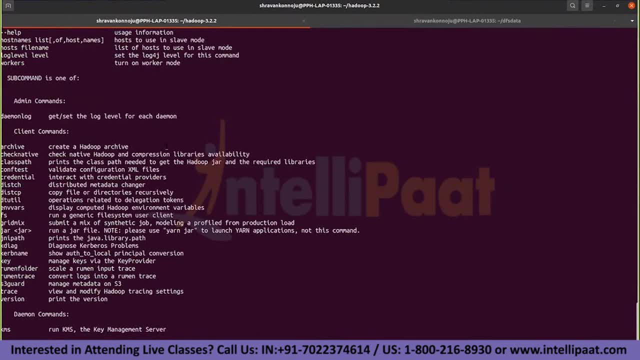 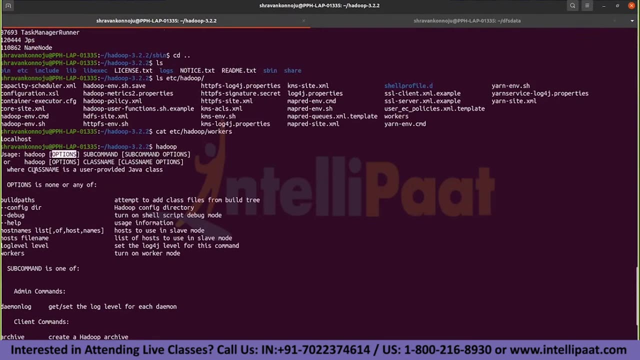 command, or you can also give hadoop and then enter. so it's gonna help you with a list of commands it's gonna take. so, uh, hadoop is a command that i gave. under hadoop, you have different options and there is a sub command. there is a different sub command options. okay, or you can. 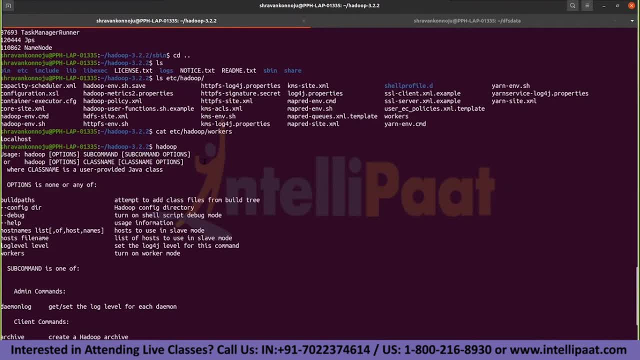 give hadoop options: class name, class name option. so what are the different options which it can take? so options are the config directory, the debug, the help, host names, host file, file name, a log level and the workers. So Hadoop configuration directory and it's going to turn on the shell script debug mode. 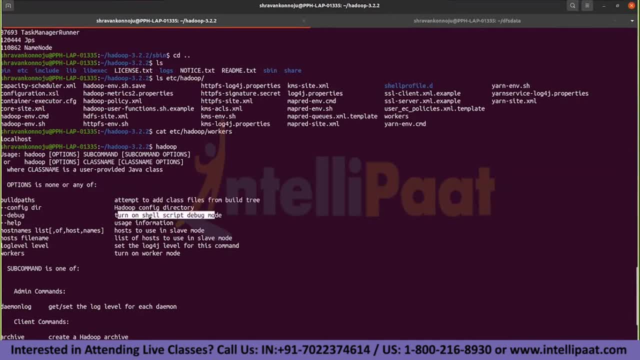 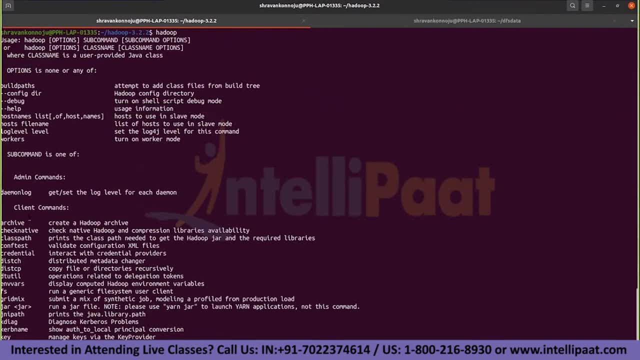 It's going to help you with the. it's going to give you a help, a syntaxical help, for all the commands that you execute And, similarly, you have different admin commands, You have archive, you have class path, and these are all commands we will not be using. 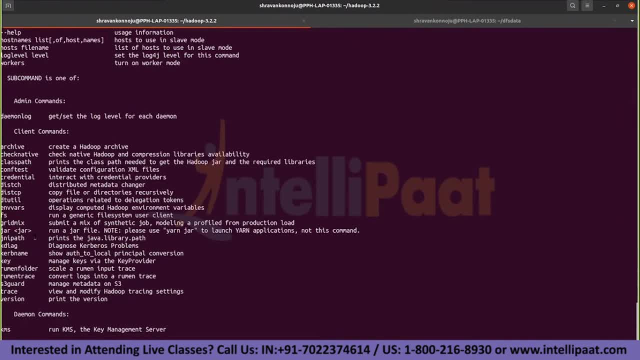 Most probably, we being the developers- you'll not be able to use all this, And there is something called as FS, right? So what is this? FS Run a generic file system user plan. So if you want to interact with the file system, 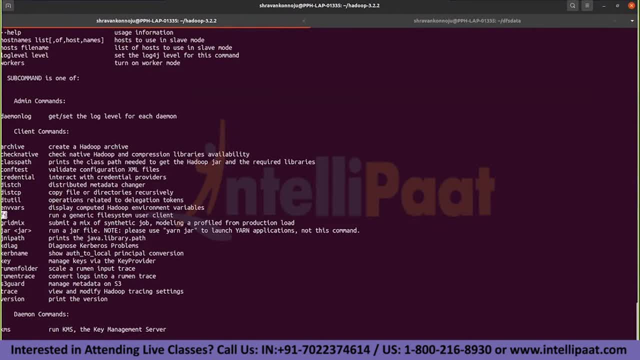 the Hadoop file system. you're going to use this FS command And if you want to add a jar file, you will be using a jar command And similarly the version we already know. and what else? we will be using Class path. we can use the check native, we can use right. 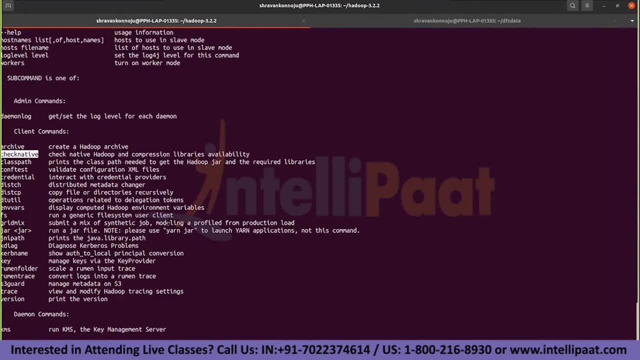 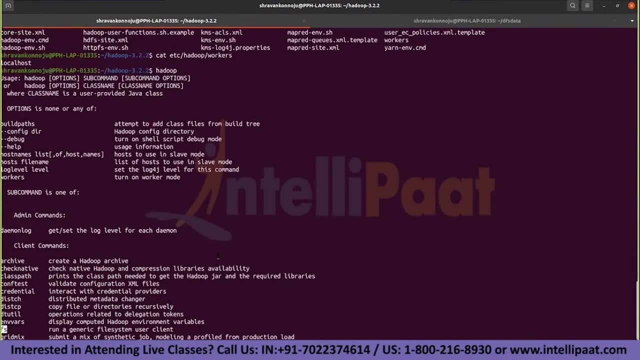 So, but generally, the FS is something which we'll be using to interact with your Hadoop file system. So what do we do? Hadoop FS right? So what all it can take. So, after Hadoop FS, what all the commands it can take. 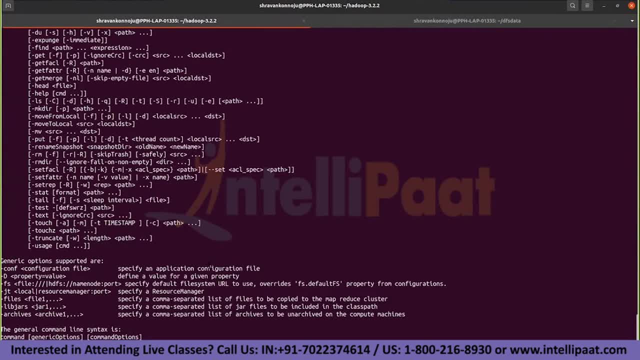 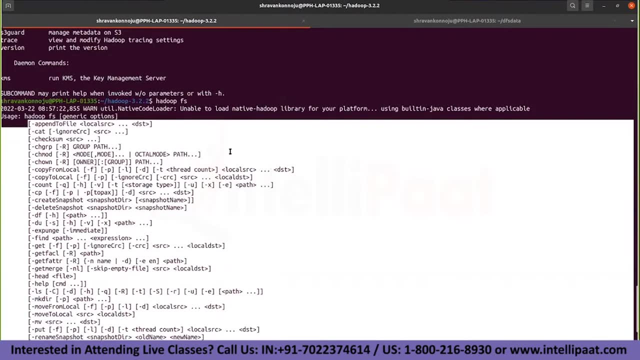 There are different. these different options, you have Getting it. So all these options can be used to make some changes, to edit or to interact with your Hadoop file system. So there is an append Append to file. What does this mean? 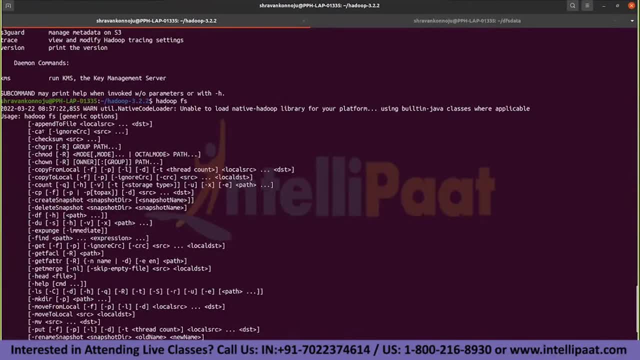 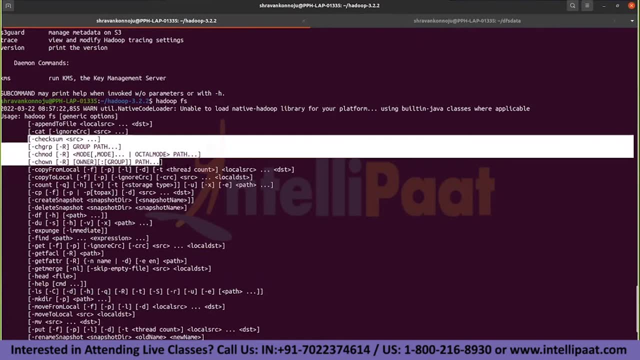 That means you're trying to append some data to an existing file. There is cat, there is checksum, chgroup, chmod- These are all permission related things- And there is copy from local, copy to local. This is all file transfer related things. 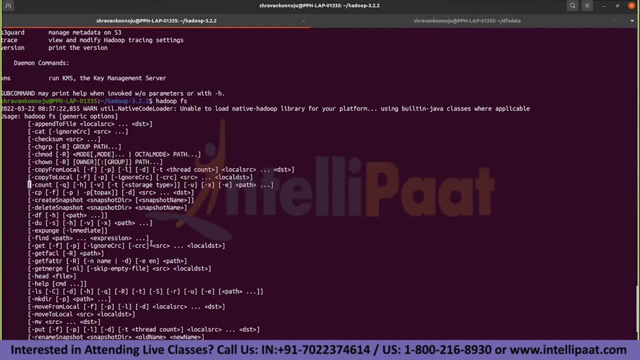 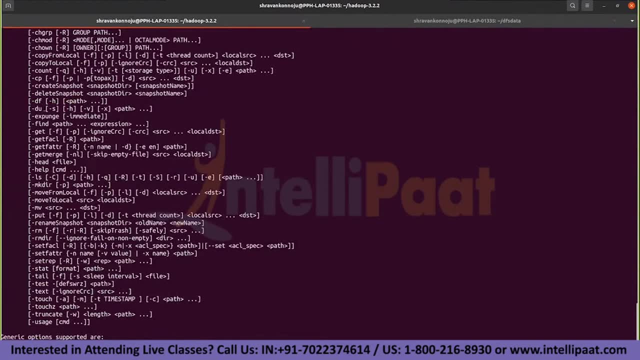 There is a count option, There is a CP. We will execute all these commands, maybe most of them, But these are all the options that you have here, right? So how many of you are familiar with these commands here? The touch, or setrep, or rm. 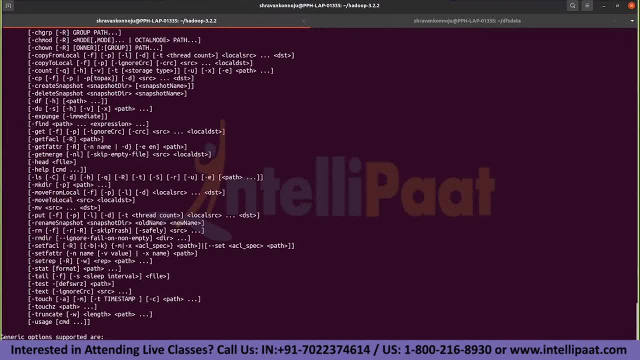 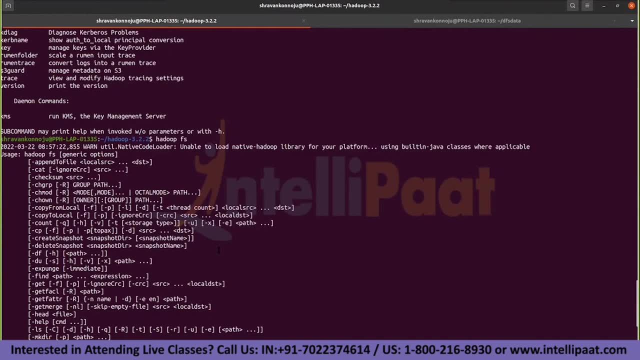 rmdir, put mv, mkdir, ls, all this. These are all the generic Linux commands, Linux or Unix commands. So the only parameter that we are appending to it is the Hadoop FS. okay, So if we use Hadoop FS along with these commands, 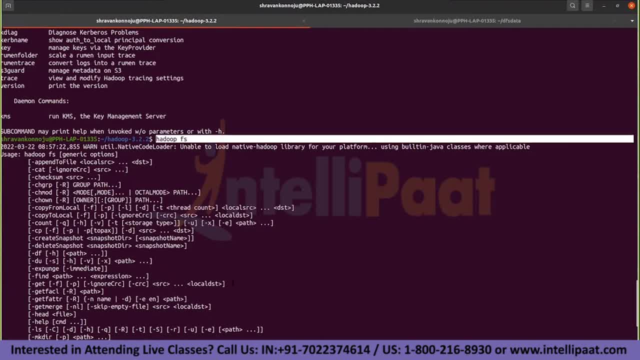 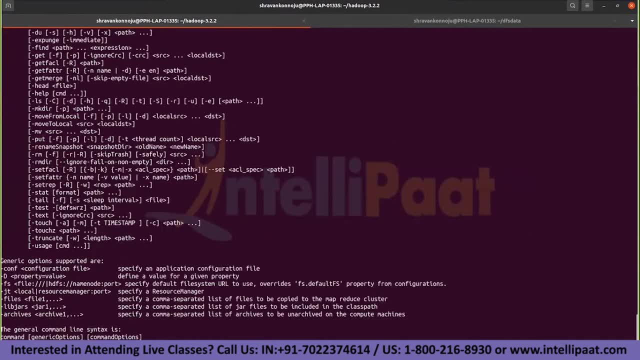 then it's gonna interact with the Hadoop file system and make all those changes So generally in your normal system also, in this normal system also. if I come out of this directory I'll do ls. That means it's gonna list you all the commands. 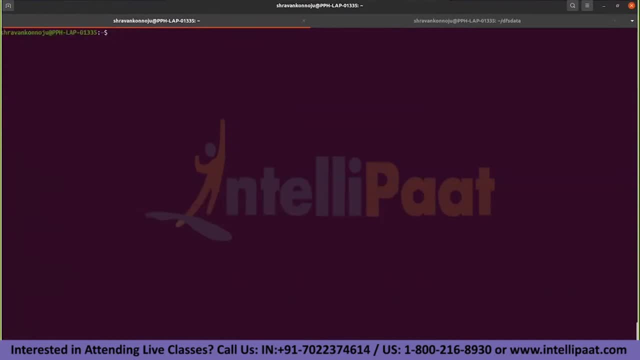 all the files right. So similarly, I'll do mkdir- right. So it's actually creating a folder, It's actually creating a directory for you. So, similarly similar to the commands that you have here, what I'm just trying to do. 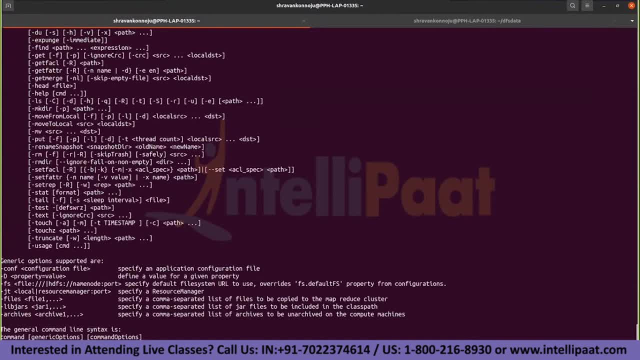 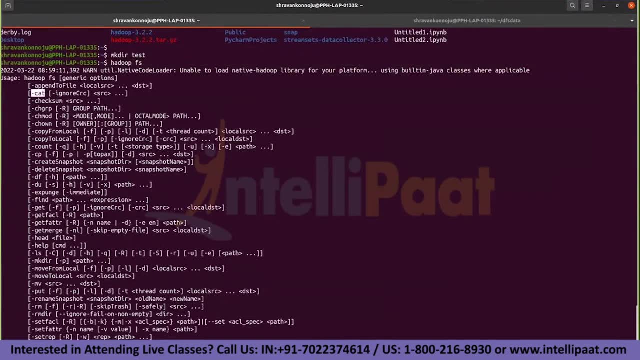 I'm just trying to append Hadoop FS in the beginning. okay, So the activities that they're gonna do is the same. So cat is used to list the contents of the day, the contents of the file. So we have tried and executed all the cat commands, right? 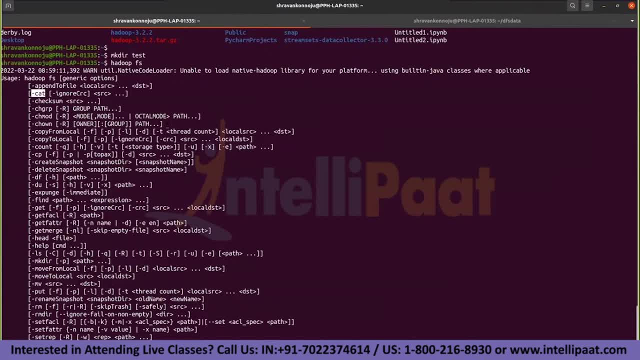 All this while cat htfs sitexml, cat map red sitexml. So we've already executed all those things. So cat is used to let the content get the content. So chmod chown chgroup you specify to provide the permissions. 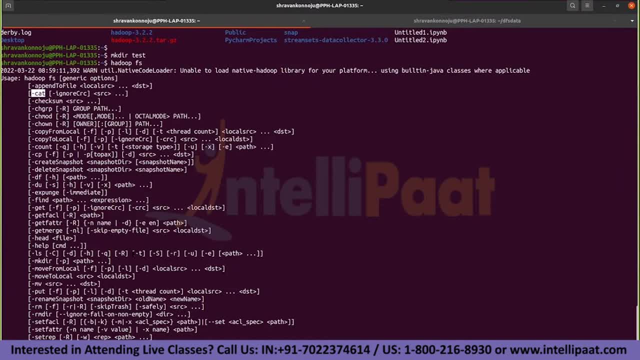 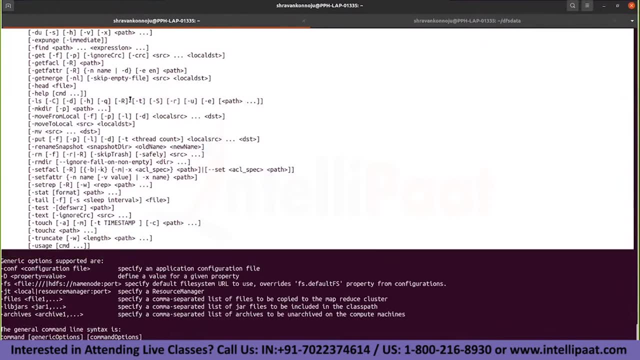 So, similarly, all this, every one of this particular thing, is a Linux command only, but what we are trying to do, we are trying to work them using the Hadoop FS, which is gonna interact with the Hadoop FS, Hadoop file system and make all these changes to it. okay, 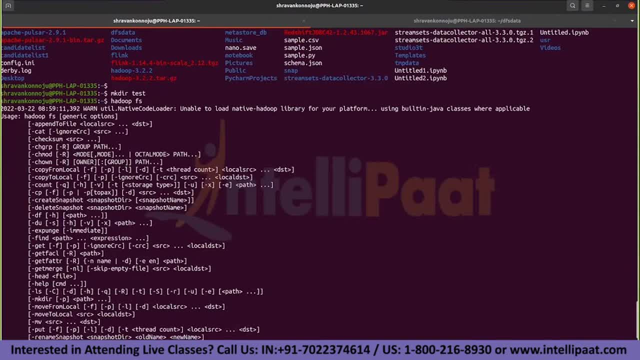 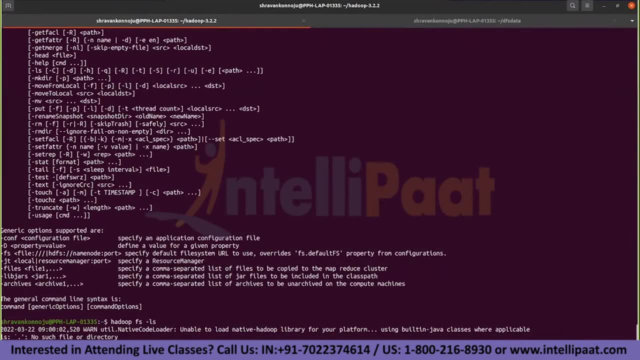 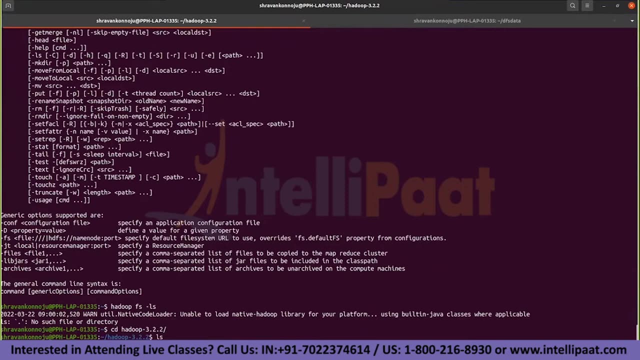 So now I'll do Hadoop FS hyphen ls. okay, So ls is what A normal, the local file system, listing of files, like something you have in DIR. In Windows you have this DIR command right. So similar to that. you have this ls. 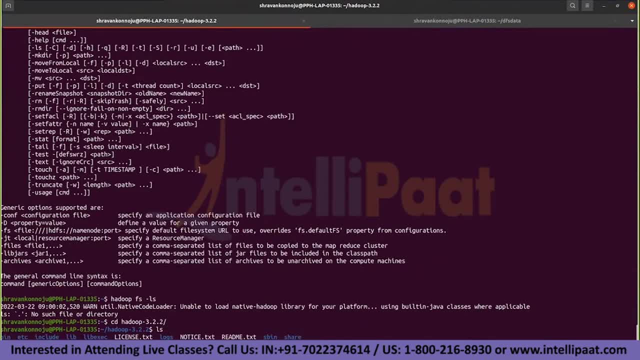 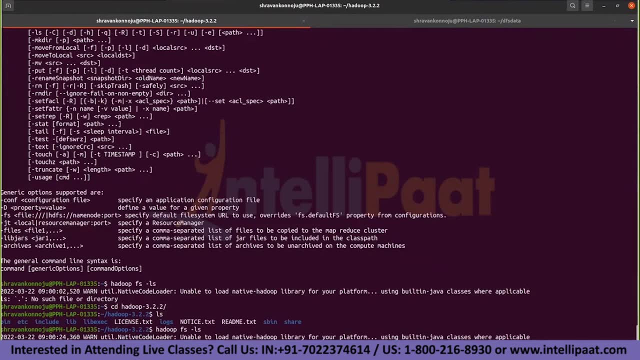 So list all the files And what I've done. Hadoop FS ls is for doing what It's: giving you the files that is available on the HDFS. So what is it saying? There is no such file or directory available. So what I'll do? I'll give some beginning path. 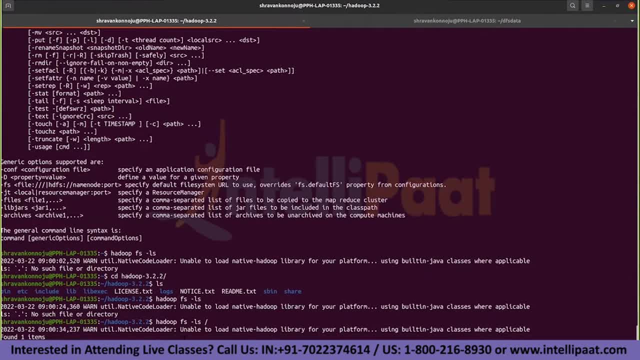 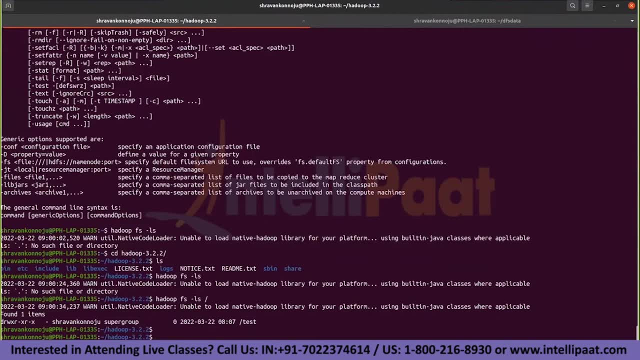 So there is one file, one directory that is available. if it is not visible for you, yeah, So Hadoop FS hyphen ls and a slash is giving you the path of the data which is available in the Hadoop file system. okay, 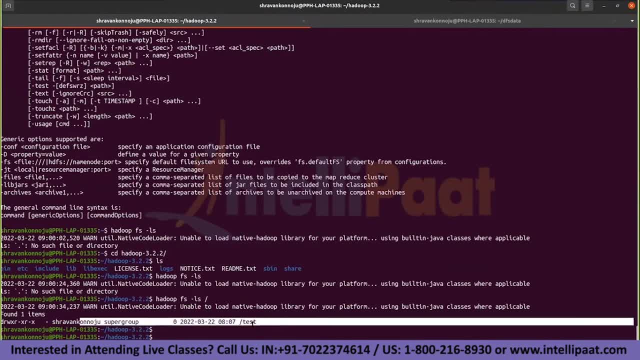 So there is one folder available in the Hadoop file system, So that has been listed. So what do you do then? Hadoop FS, hyphen l, hyphen mkd. let's do. I'm trying to create one file, a folder. 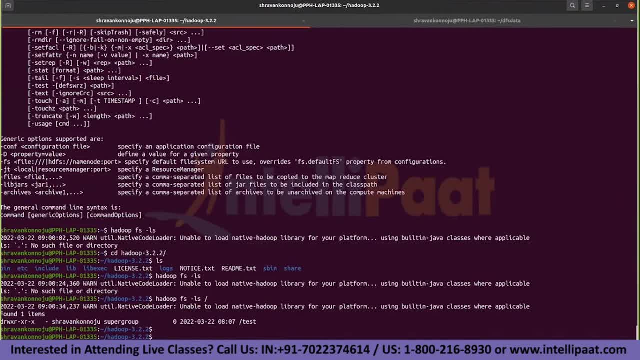 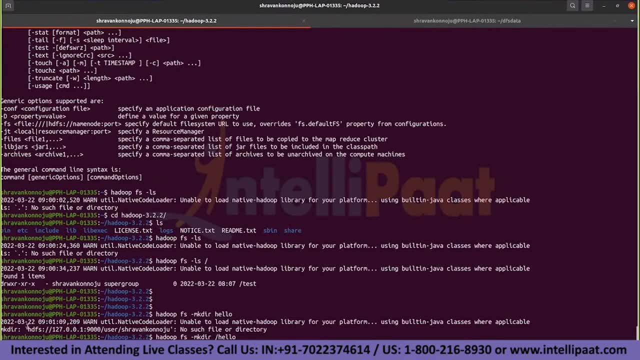 Hello, right, So enter. So I'm starting it with a slash because it's trying to identify or it's trying to interact with this particular location by default. If I don't give a slash And Hadoop DFS, Hadoop FS does not have permissions. 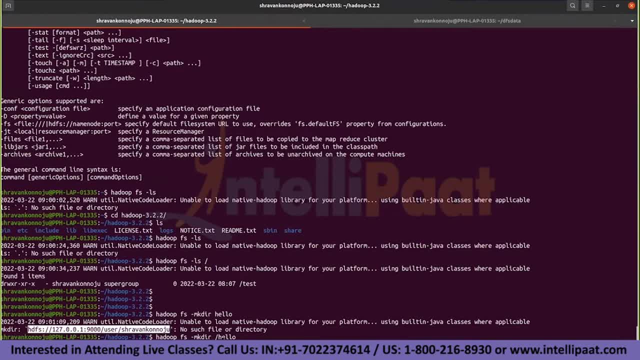 to interact with this folder directly. okay, So if you give a slash, then it's gonna start with user Sravan and then slash and then hello. Okay, if you look at the explicit path of this, it's going to take this particular location. 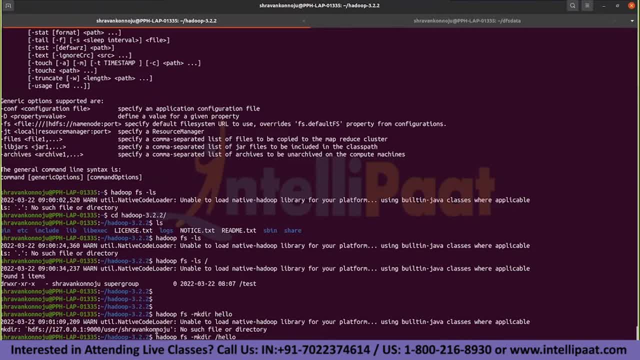 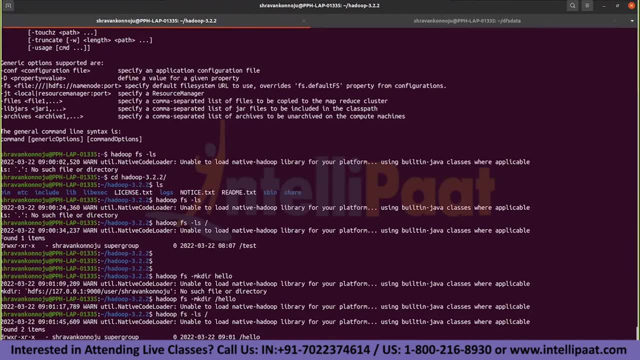 So now do a ls again and then see all the files that we have created. So I created hello and I created a test. If you want to see what are the contents available in a hello folder also, So do a Hadoop, FS, hyphen, ls and then hello. 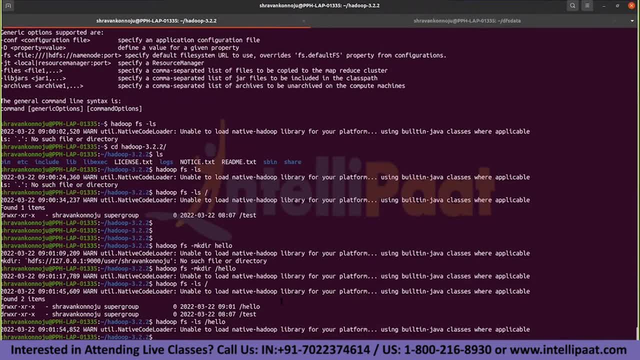 Getting it guys. Getting the difference? Yes, right, So this is all very generic, very basic Unix commands- ls, mkdir or cat or whatever. okay, So if you want to delete some file now, if you want to delete some of this test, let's say: 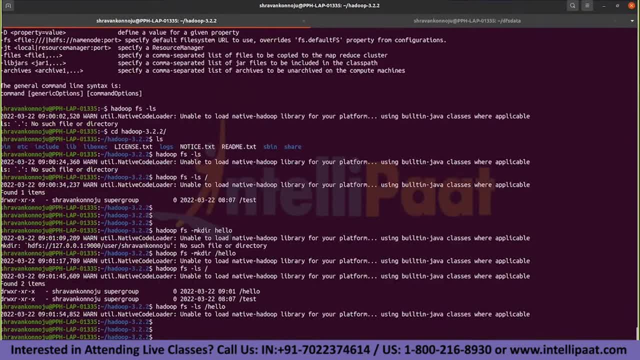 what do you do, Hadoop FS, if it is not okay? So there is a command called rm and I'm giving rm and then I'll do test, enter, So test. no such file or directory available. So if I give slash test, so test is a directory. 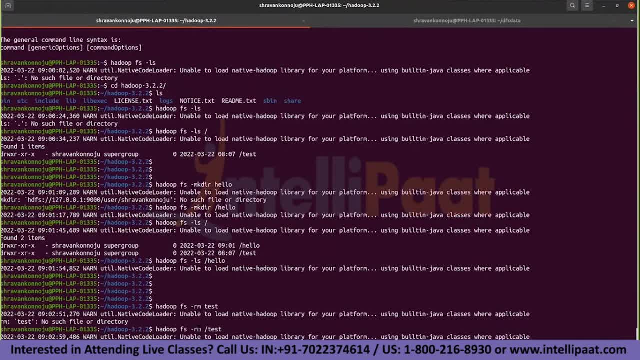 So what does that mean? Rm is a command, is a remove command which is generally used to remove a file. remove the files, okay, Only the text, only the files and not the directories. So if you want to delete a directory, 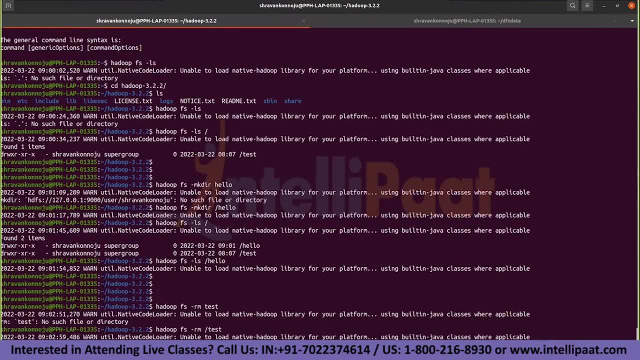 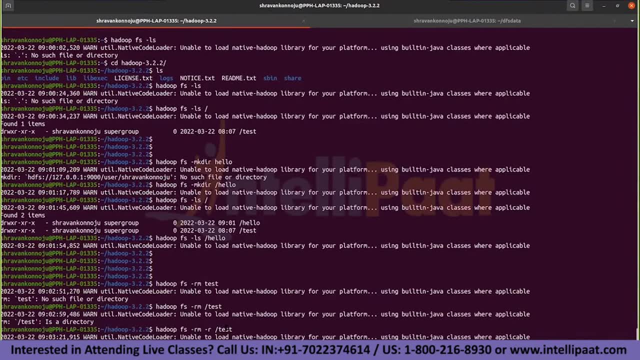 I'll have to append rm hyphen r, okay, Which is a recursive mode of delete. So recursive mode on the test folder. So inside the test folder, whatever the files and directories or whatever the internal files you have, all will get deleted, one after the other. 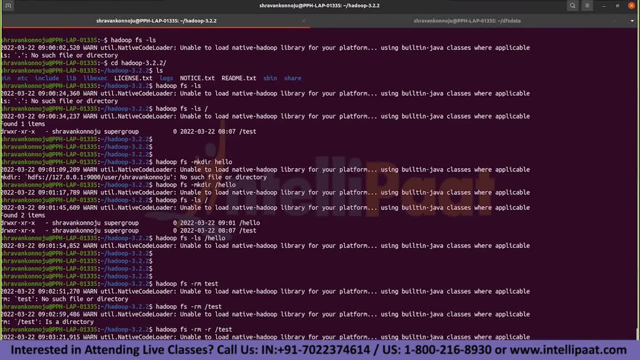 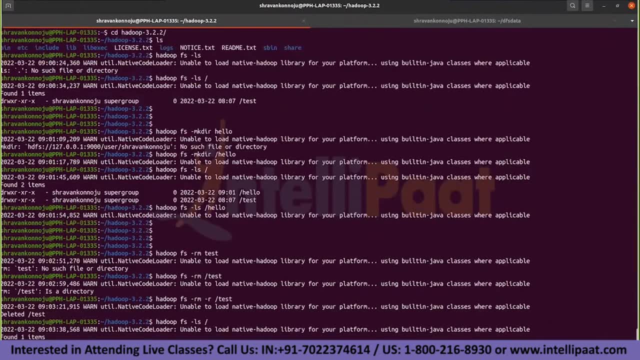 So now, if you do an ls on top of this HDFS, then it's going to show you okay, To show you only one file. the test file got deleted. okay, So now, if you want to write some file or whatever, 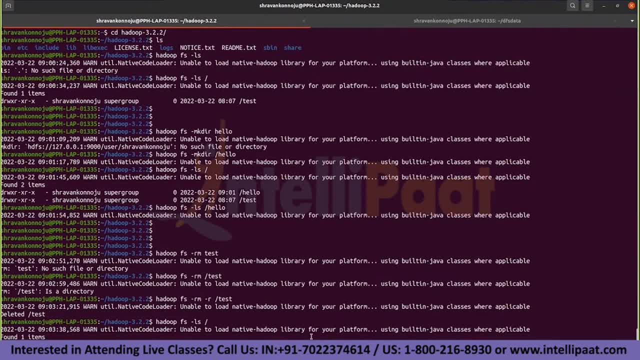 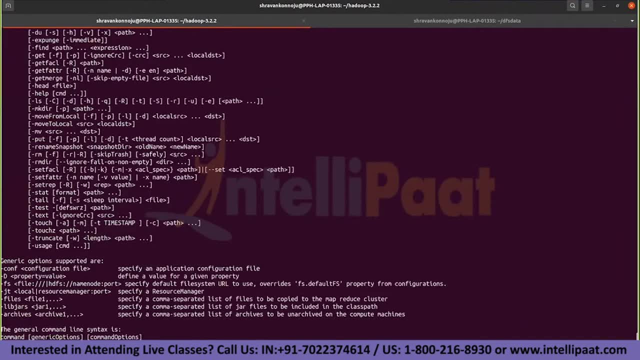 what you say. if you want to create some file in Hadoop file system, So there is something called as just write, just see. So there is this append to file. There is some data which you wanted to append. This is different. 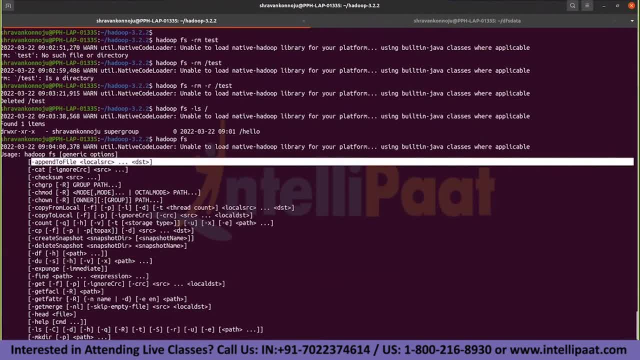 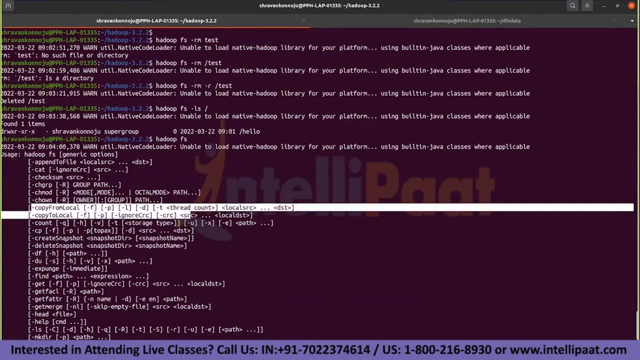 And cat. we know what it is going to do: chmod, chgroup and all that we will see. So copy from local, copy to local. We will do it. So cp is to copy within the file system. So just scroll down, scroll down, scroll down. 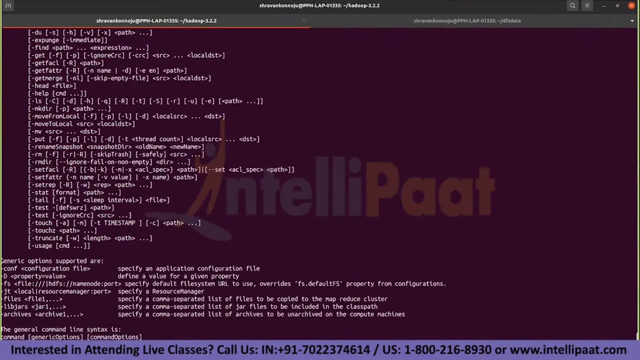 Yes, touch. So what is this? touch, g and touch, So these are the commands which are used to create an empty file for you. okay, So let's say hadoop, fs-touch and on follow sampletxt. So what is it doing? 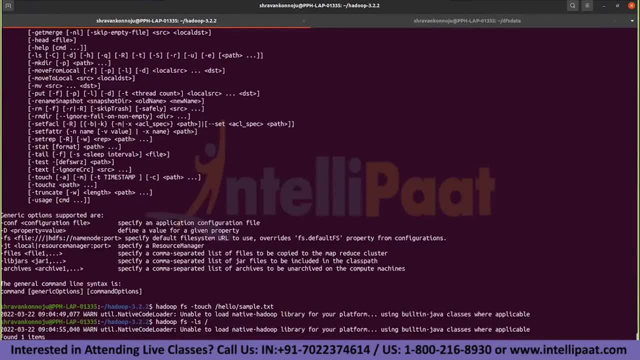 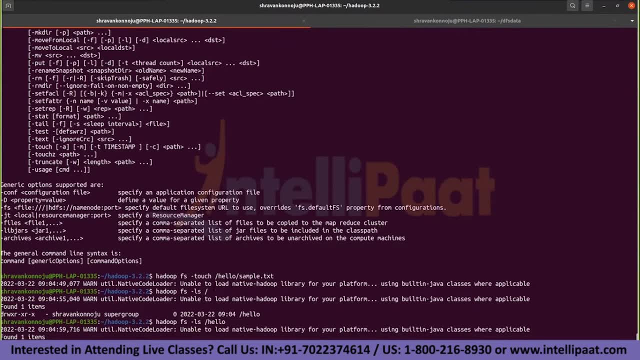 Hadoop fs-ls follow and there is a sampletxt file got created. So touch commands are used to create an empty file inside your Hadoop file system. okay, Inside your Hadoop file system or wherever it is Like, touch is generally used to create an empty file. 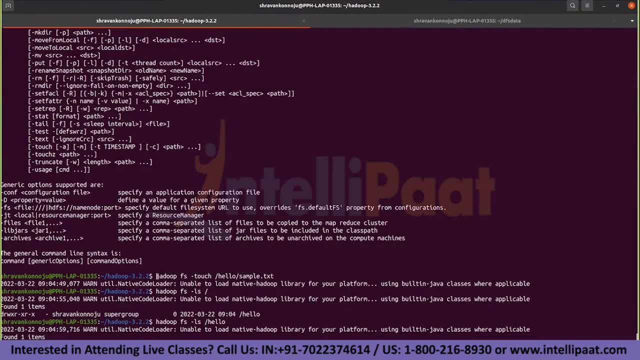 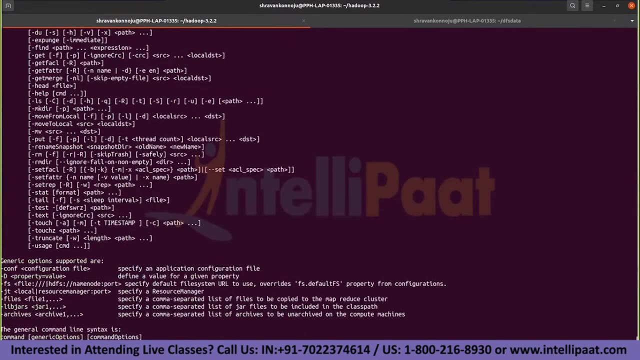 a 0MB file And using Hadoop fs as a prefix. we are creating this file on the Hadoop file system. Similarly to Hadoop fs, you can also write HDFS, DFS also, So both do the same thing. So if you do HDFS, it's saying there is a subcommand. 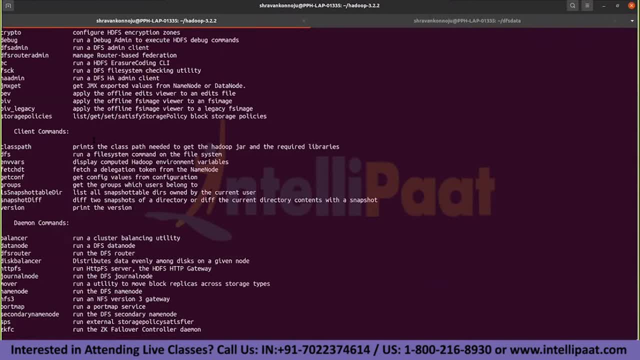 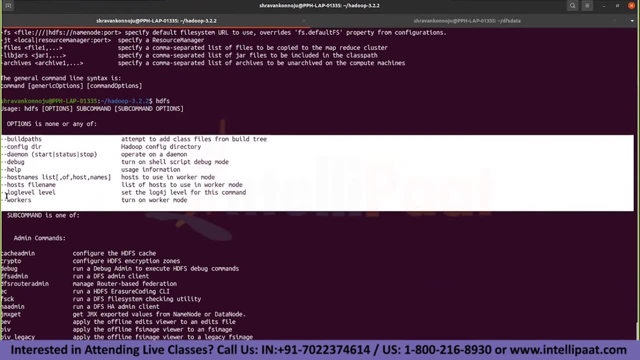 and subcommand options available. So the same level of subcommands are available for this. okay, But the difference is there is DFS Instead of fs. you have the DFS. So when you are using HDFS, give DFS-ls and then give a tab. 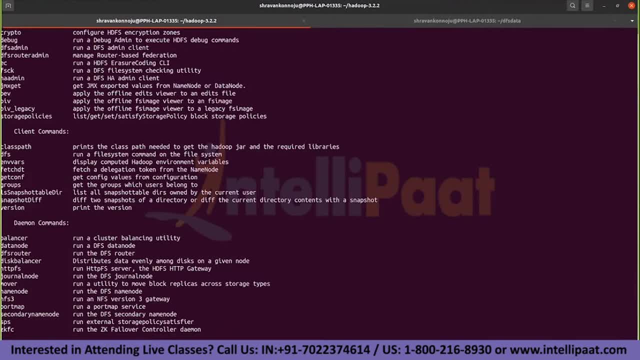 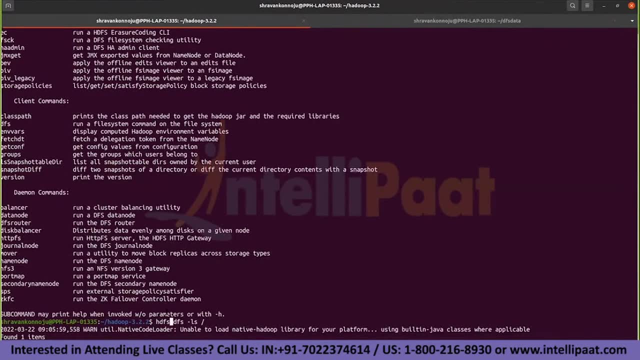 What was I saying? Sorry, DFS, right, So same thing it is doing. So HDFS DFS or Hadoop fs, So both can be used Either. one of it is an older version, is kind of a deprecated version, but I don't know which one is a deprecated command. 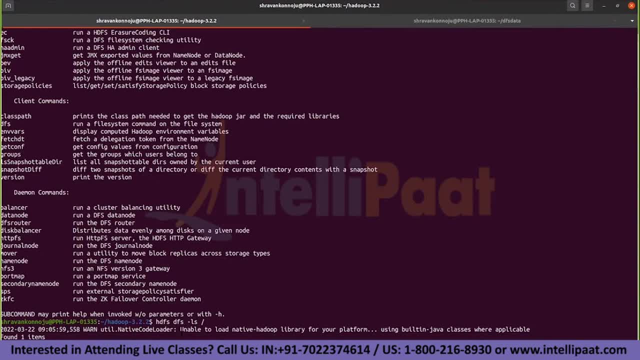 So Hadoop fs, I think, is deprecated. HDFS, DFS is something which has been in use recently. okay, So that pretty much is like interacting with your, both used for interacting with your Hadoop file system. okay, So now, regardless of where you have the data, 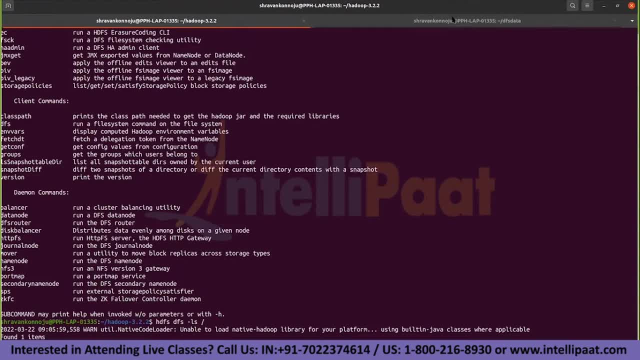 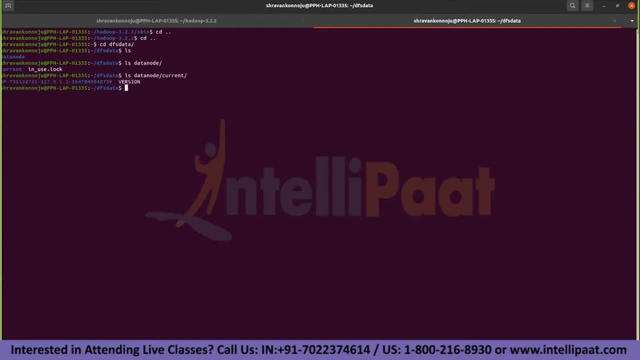 whatever the location you have the data, it actually doesn't matter for us, right? So as long as we are, so there is a file that got created. If you see, there are some files that are getting created, Right? So earlier there is no file. 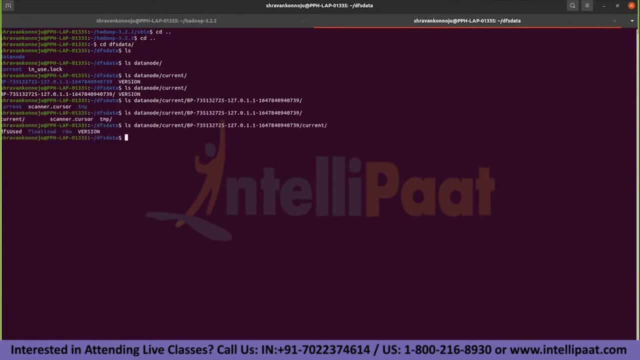 What is that? B? is it So as of now, you, whenever you make those changes to the HDFS location, some data gets appended to the data node directory, right? So I'm trying to create a file in this. 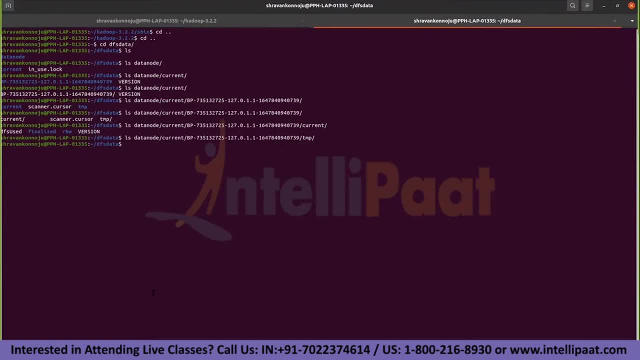 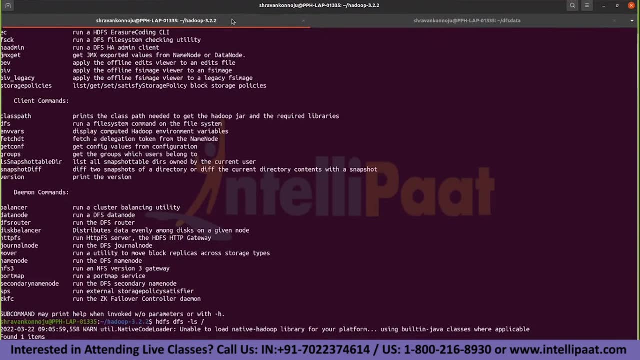 I'm trying to create a file. I'm trying to create a directory. I'm trying to create an empty file. All that changes were being tagged in your data node directory. okay, Because this is what is being used as my data node, right. 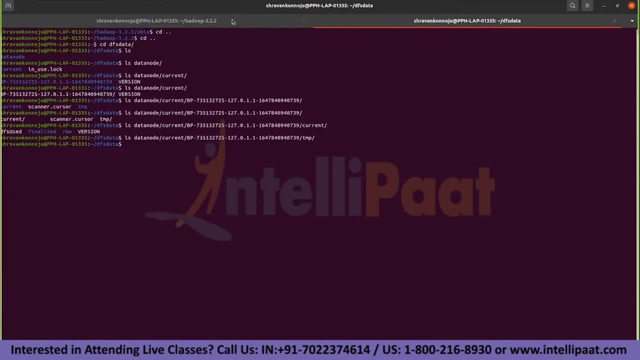 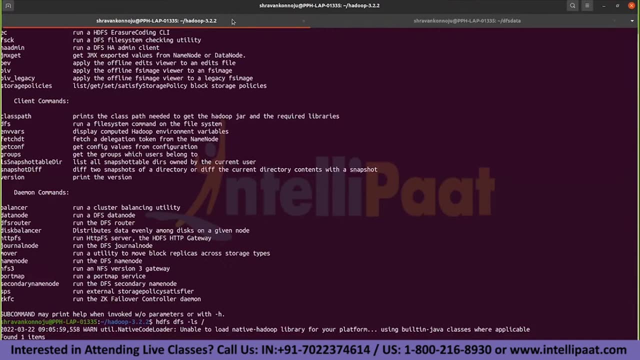 So you may not be able to see the proper format of the data. It might be in a compressed format, but generally your files all will will be in a compressed format. It will will get stored into that particular location only always. 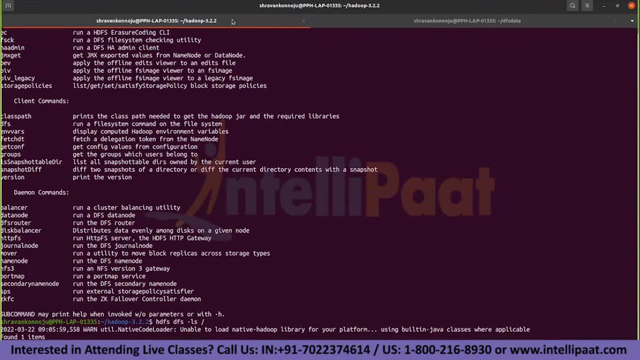 Okay, So is it simple. These are all. these are all very, very basic commands. Yes, agree. No, see, we will have to interact with the HDFS. try to move some data, load some data into it, make some changes to the data. 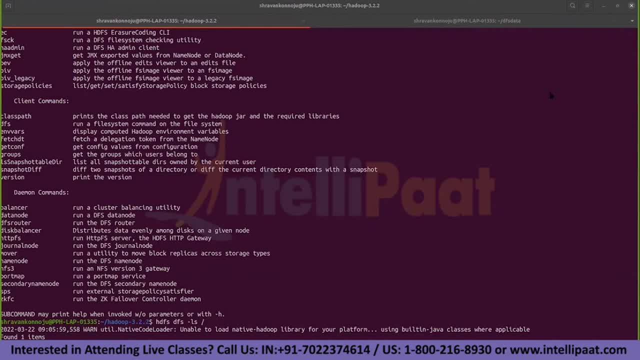 retrieve the data from HDFS to the local. So these are all commands we have. I mean, apart from that, nothing, nothing else we have. I mean, we have not discussed about it. but so what do we do now is: 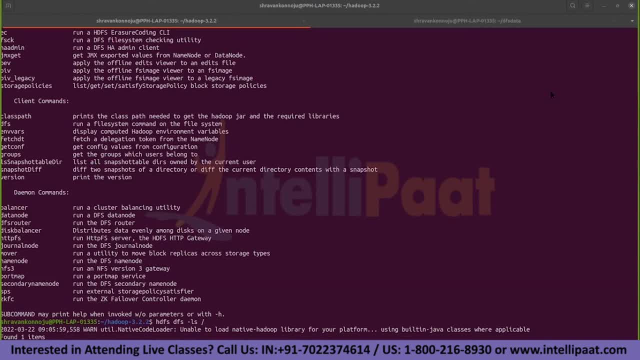 now we have seen only creation of data files and data directories, right. So now we have some data available in some location. You'll be. you'll be pushing that into HDFS, okay, Using a CP command or copy from local or put command or get command or whatever right. 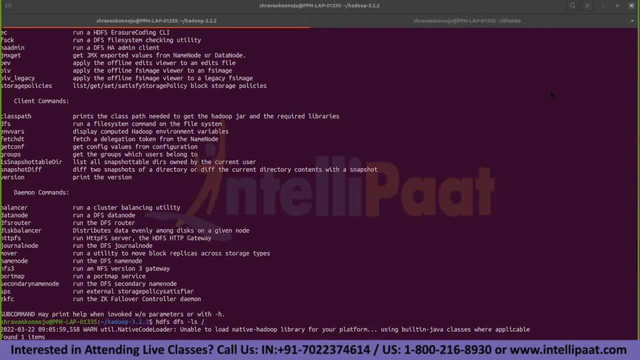 So interact with HDFS, load some data into it and retrieve some data back from it. That is what we have with with the HDFS. okay, So now let me, let's, let's also do that. So in my local file system I can do that. 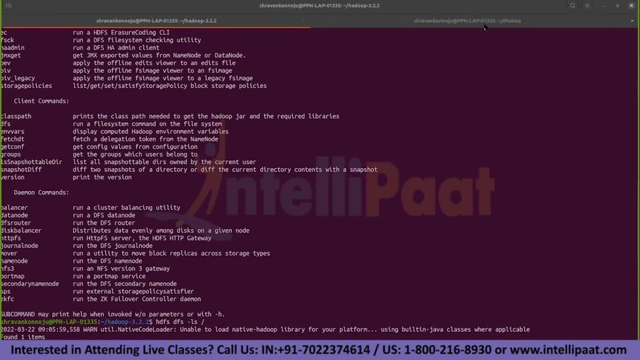 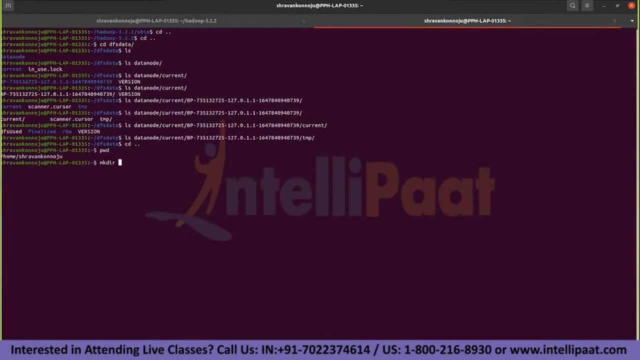 What I'm doing is I'm trying to create an empty file, create a dummy file, So under. so, Under Home, under mkdirdata, I'll just rep cream the data in my local file system, Hello, so I'm writing some data into it. 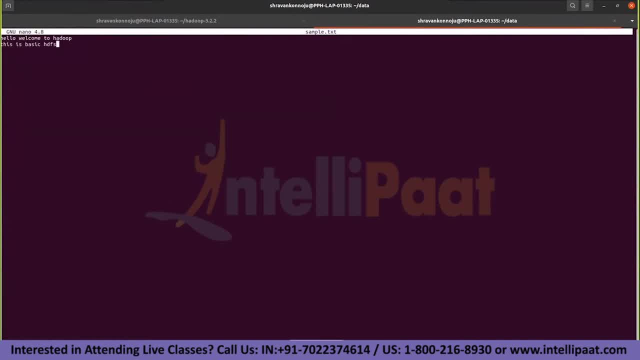 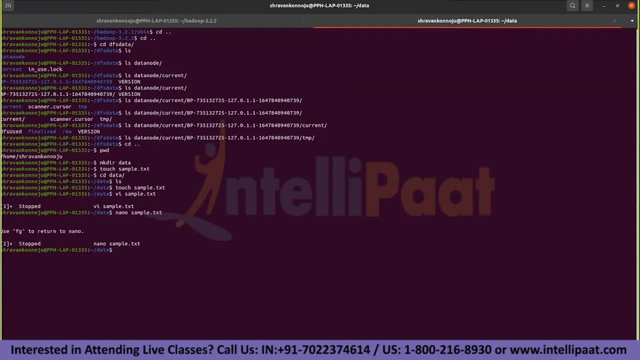 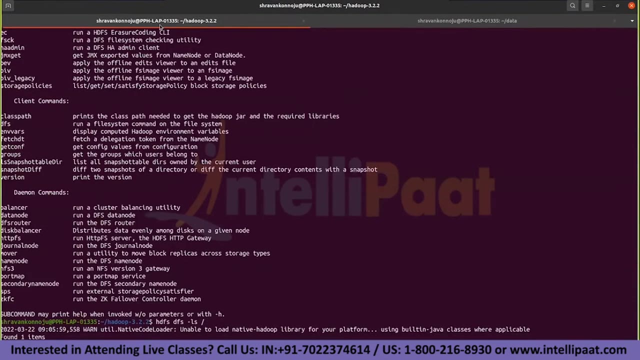 This is so this data, which is available in the data folder I'm I'm trying to and move this particular file to your hadoop file system in the other terminal. so there are multiple ways of doing it. if you look at hadoop fs, enter, so there is a put command and there is a copy from: 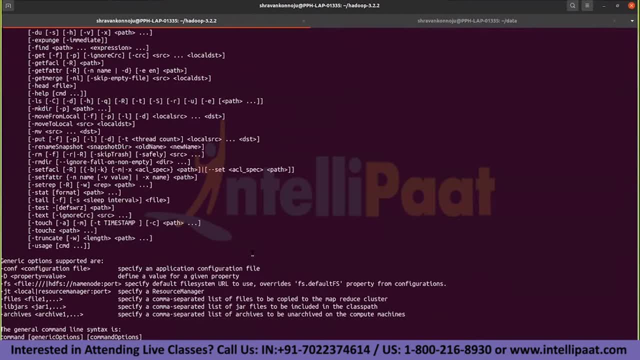 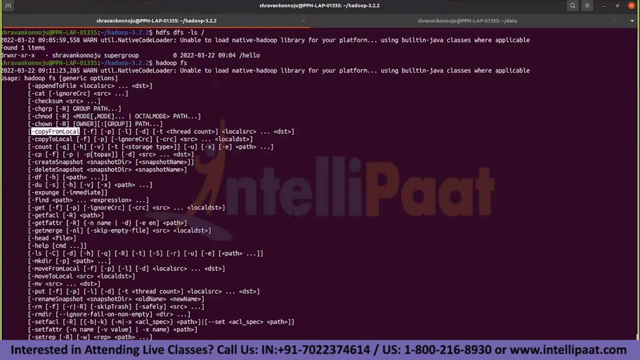 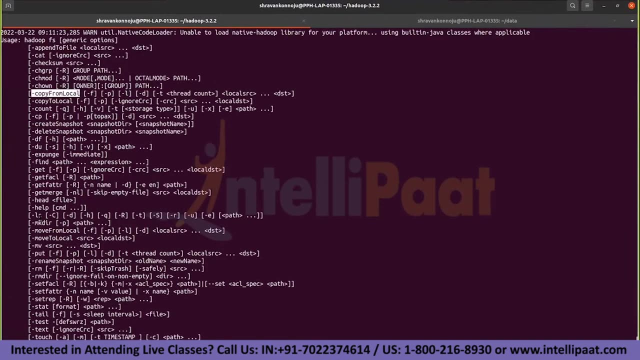 local command. so there are two commands which can load the data from your local file system or from some location of your network drives to your hdfs locations. okay, so copy from local is one command and put is another command. so put command can- can actually get the data from any network location. 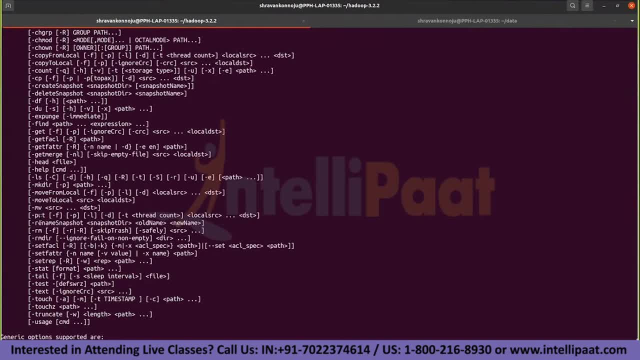 okay, so it's need not be. it not be need not be available in your local file system alone. okay, so copy from local is something which is available in the local file system of your machine. so whichever machine you are interacting with in the local file system, whatever the data you 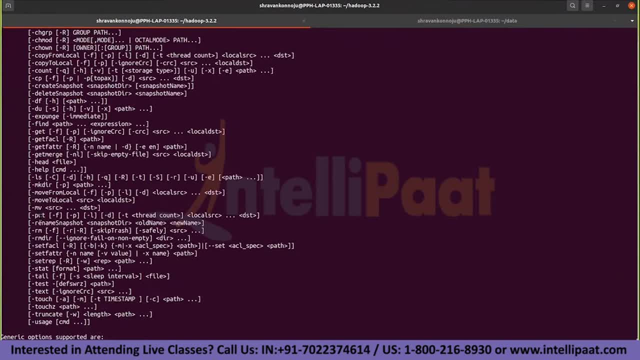 have. if you want to copy the data into HDFS, you can use copy from local or put also will do the same thing. put is the data from used to move the data. copy the data from the local file system or to from any of the network location drive to your HDFS. okay, and there is also something called as move from local. 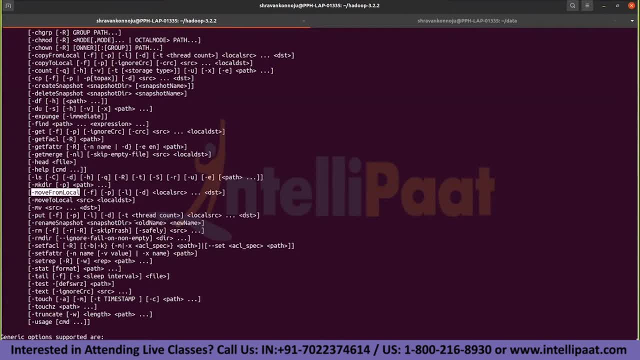 which is a delete from the local file system, and load the data into HDFS, move from local or move to local. move from local is local to HDFS and move to local is from HDFS to local. okay, so copy from local, move from local and put. all these three commands will do the same activity almost. 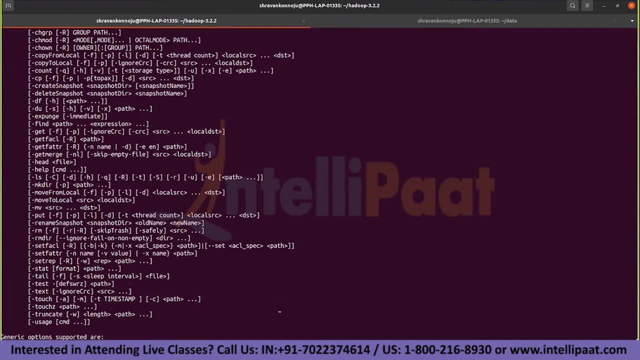 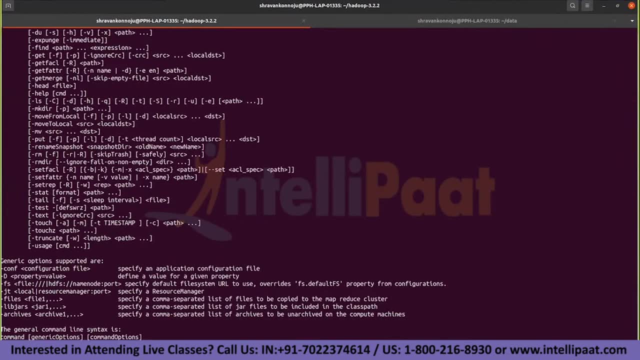 the same activity, which is loading the data from the local file system to the hadoop file system. so how do we do it? hadoop fs hyphen copy from local. what is a path- this is, i mean the, the data you can just give it from data sampletxt- to just give an empty folder. okay, i'm not giving. 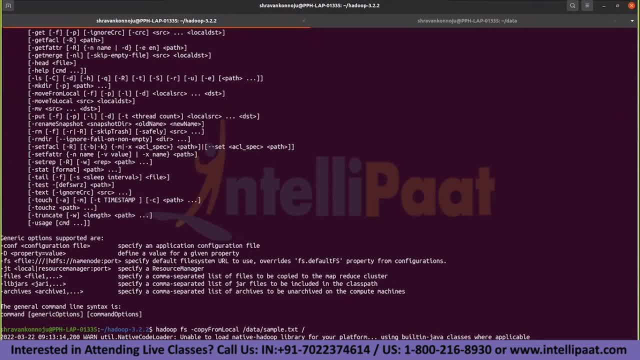 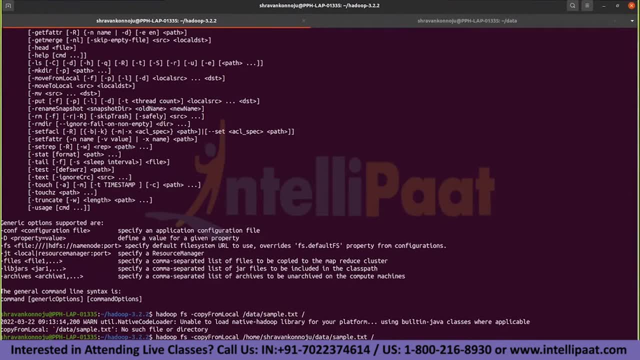 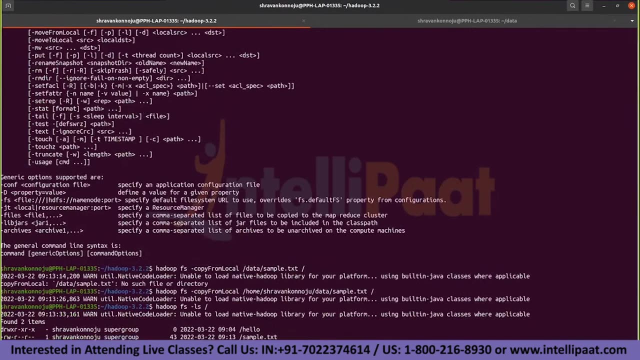 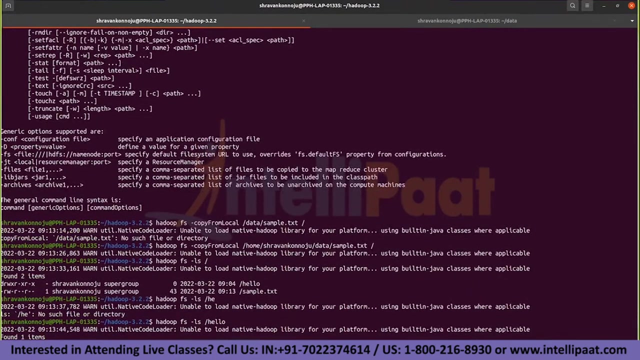 any data sampletxt. it's not identifying. okay, enter. so now check in hadoop fs hyphen ls. so there is a sampletxt got loaded right. so similarly, you can also do it using using the put command also, or copy from move from local command also. so similarly, how do we get the? 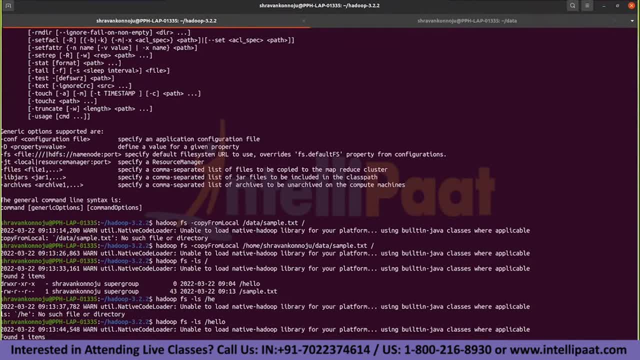 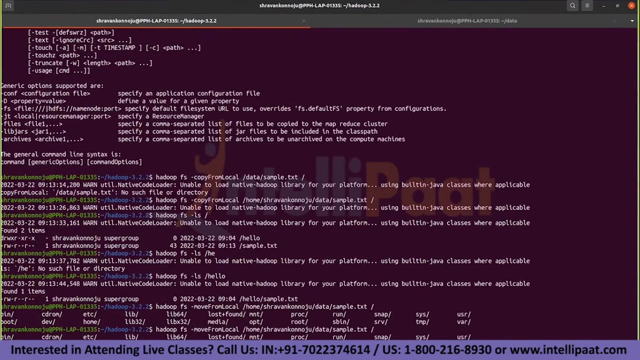 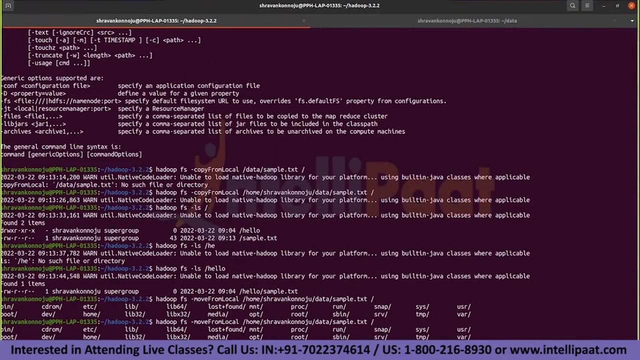 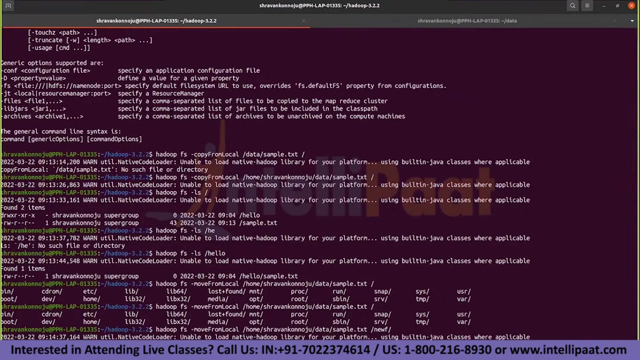 data back. so all these commands will will point to the same thing: copy from local is one and there is put is another, and then move from local. so move from local. what is it gonna do from home data sampletxt to user, whatever it is user? no, not user. this is hdfs location. so hdfs location. i'm trying to create one new folder. inside the new folder i'm trying to dump the data. let's see. so nf is not available, is no such file or directory. so i'm gonna do that in hello. but hello already has a file named. 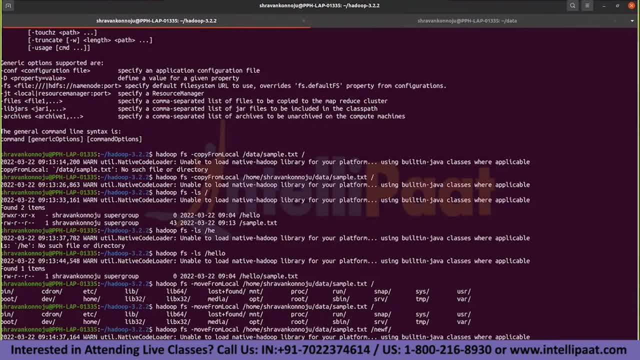 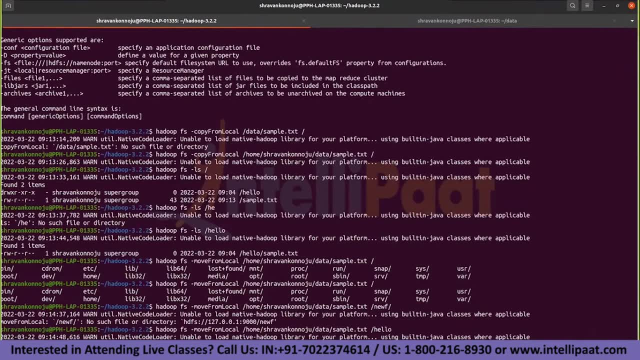 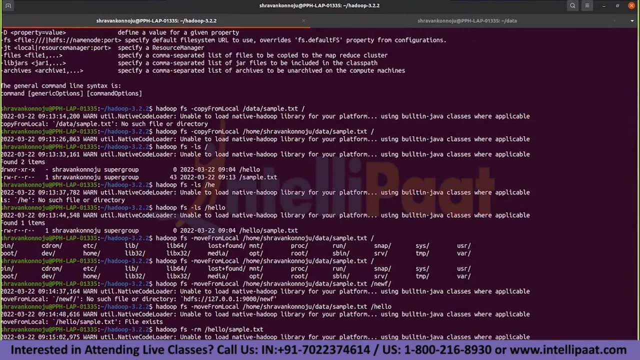 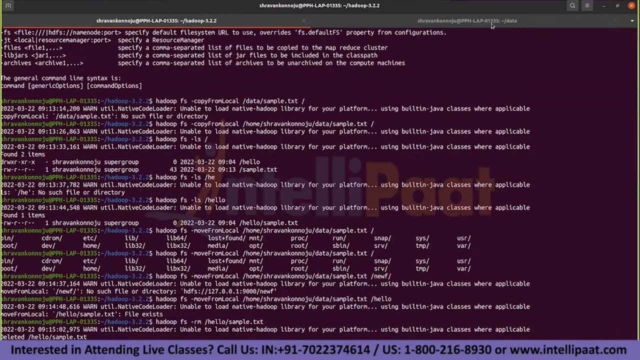 sampletxt, right? so in that case, what they will do? hadoop fs, hyphen, rm, hello sampletxt. so now do a move from local to your hello folder. it will load the data into sampletxt and it will also delete the data from your the local file system and generate the normal. 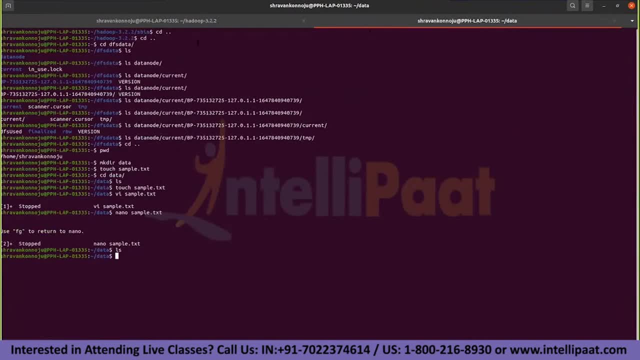 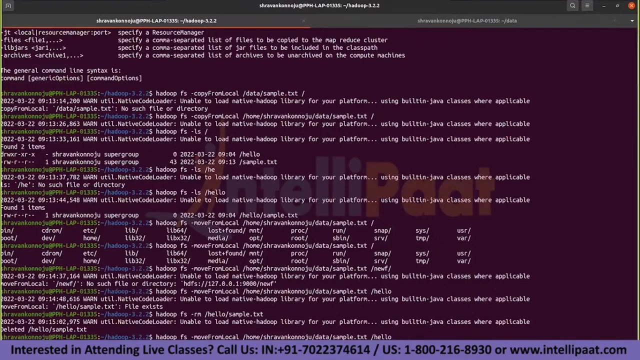 functionality like we do. okay, so similarly, from hdfs to the local file system, you can do the same thing from local. you have again three commands. uh, hadoop, fs hyphen. copy to local is one. move to local is one in and and get is another one. three commands, so put copy to local. copy from local, move from local get. 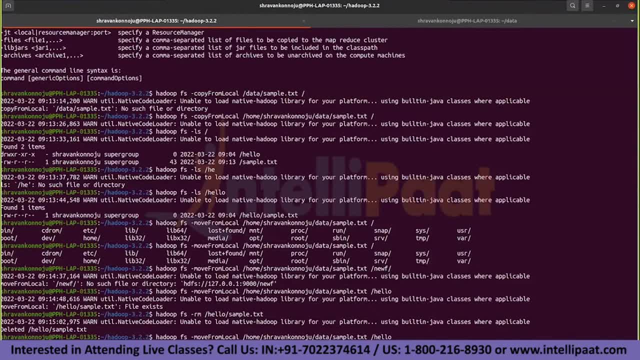 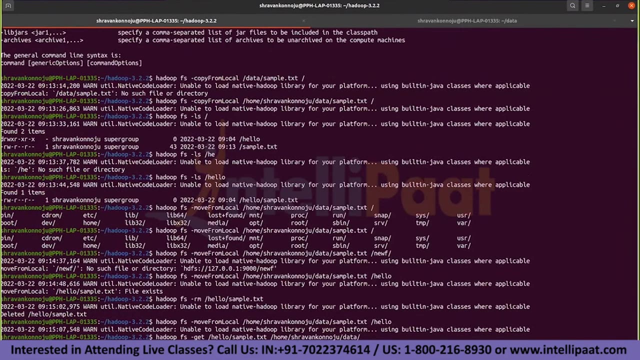 copy to local, move to local so you can use any one command to retrieve the data from hdfs to your local file system. so get hello sampletxt to home data, so this will get you the data from the hdfs location. okay, so simple data transfer commands, either from uh, using, using. these are all file level data transfers, guys. 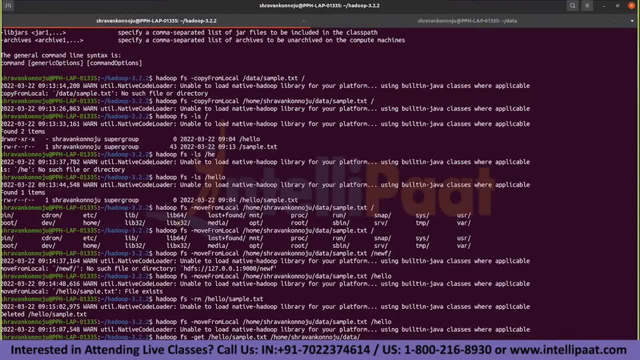 so not very much. we are going to use these commands in day-to-day activities very rarely. we will be using it and and within the hdfs. within this hdfs, if you want to move the data from one directory to the directory, you have a cp cp command. okay, so how do purpose hyphen cp uh? source will be hdfs and destination also will be. 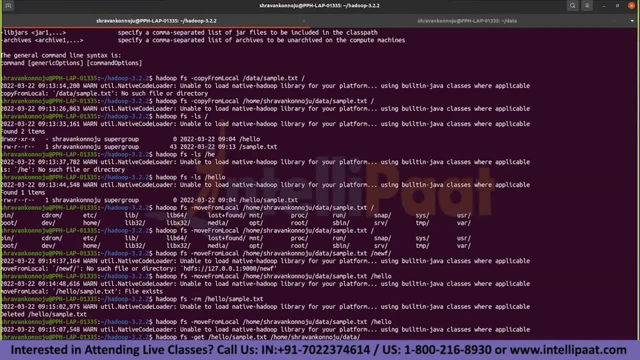 hdfs. within the hdfs, you're trying to migrate the data, and so these are all very generic, right? and and where exactly the data actually comes from. see if you look at the data commands that we are actually executing. these are all. these are all very, very generic or very basic commands, right? 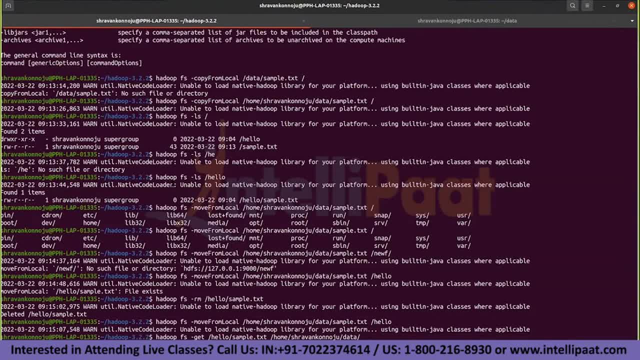 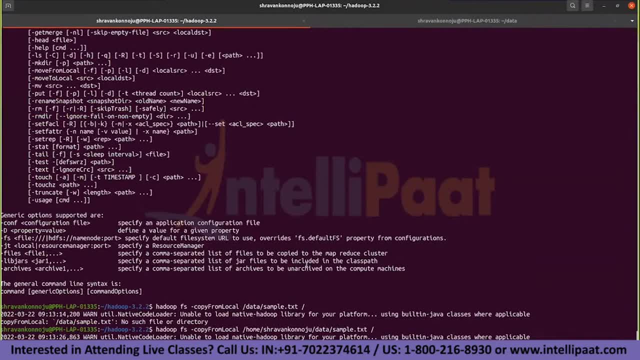 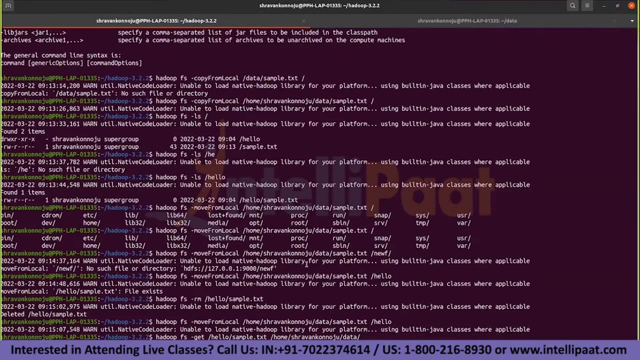 so you would not expect to load the data. something like this the hdfs would not actually interact with. it is not meant for this copy from local or copy to local or not, not something like that. so in general, when you do a copy from local, put or move from local generally you are trying to 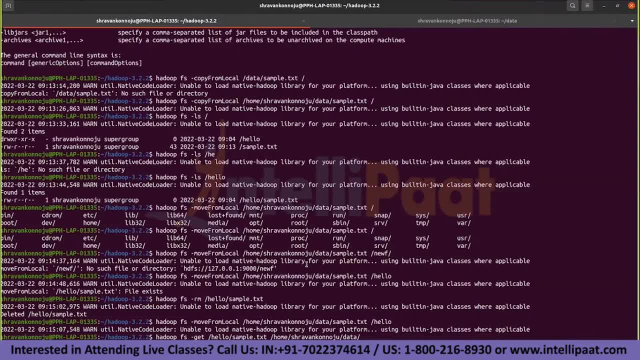 interact with the hdfs cluster. that means you are interacting with the name node to write this sampletxt into your hdfs cluster. right? so all that, all that operations will happen. it will check the name node, it will check the name node, it will check the metadata for available data nodes and 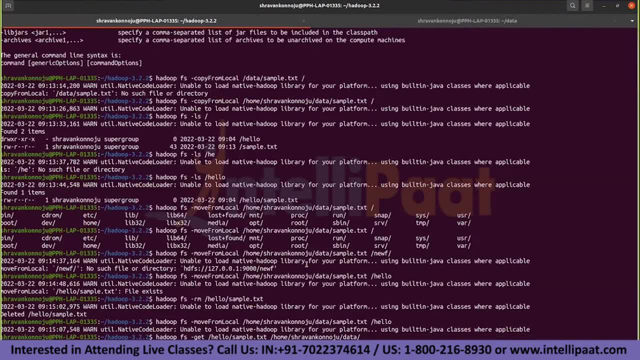 it will allocate some set of data nodes to it and then you write the data to the hdfs cluster so you can see the data blocks. so these are all operations is going to happen. but in general, guys, the data mostly comes from the external systems. okay, so it can be a relational database or it can. 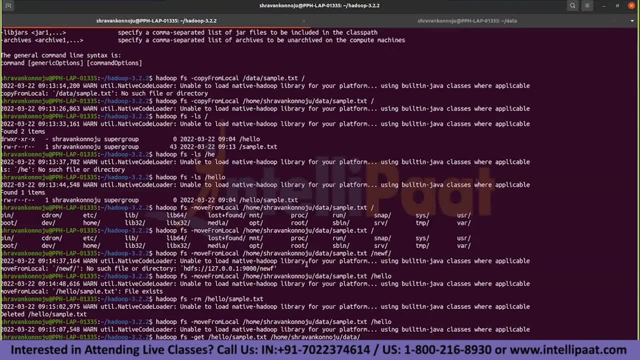 be some online stream or it can be some other network drives. okay, so which which can be inserted or ingested using different tools? it's not. it's not using a command line copy or a put command, but generally via external tools you'll be loading the data, most of the data. so if it is from a 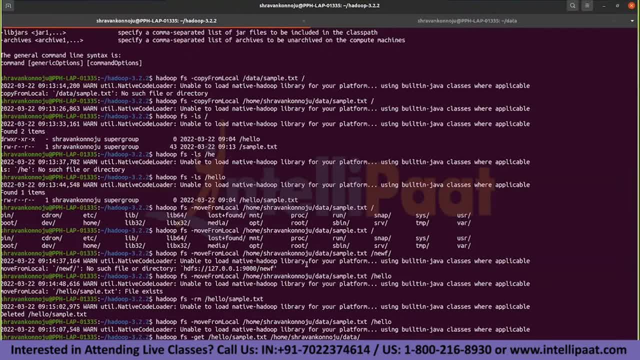 database. you're going to do it using a scoop command. okay, so you'll run a scoop command, give the source table and the destination hdfs location right. so that's how your major data operations are going to happen. but this is all very generic. you just need to understand what. what commands do we? 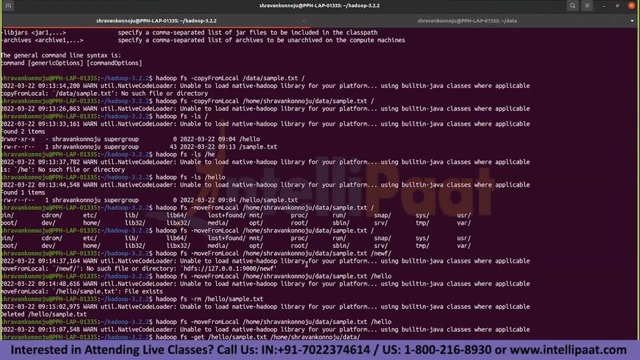 have and how do we use them? and similarly, you also have this permission related commands. how do we change the permission modes- read, write, execute modes, ch mod and ch group. how do you allocate the permissions to a group of data, group of people, that is, ch group and ch mod and ch own you. you can. you can update the permissions of the files in the 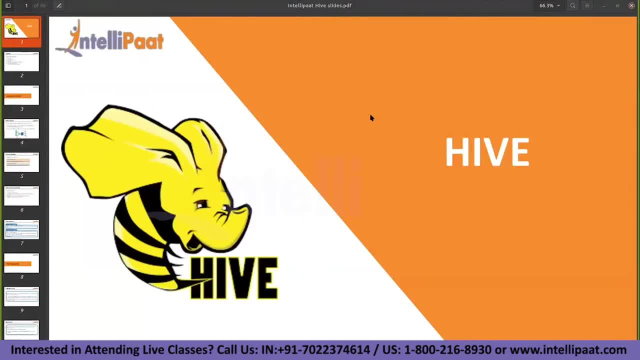 hdfs: okay, see again for hive installation. for hive setup you may have to download- because you've already done a hadoop setup right- 2.8 version of hadoop setup. so you may have to find a compatible version of hadoop hive for your hadoop 2.5 2.8 right. so all those issues will come. so if you, 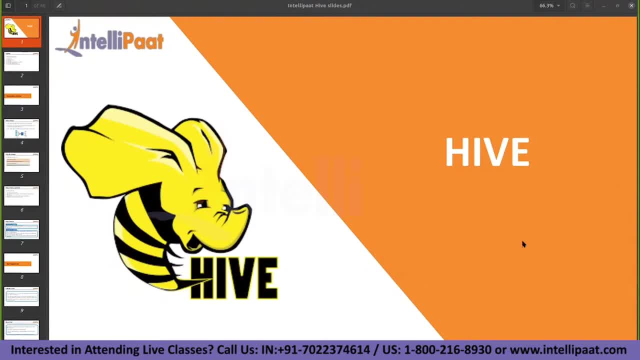 if you want to use that file, i can send you the vm file. i can send you the drive link. you can download the file and you can start working on it. okay, so all that you need is it will have a around 5.3 or 6, 6 gb file. you just have to download it and, in addition to that, you 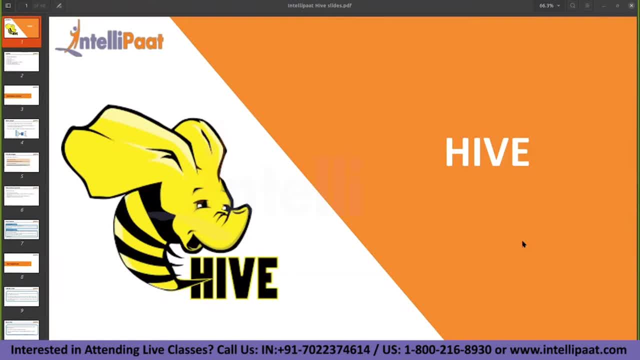 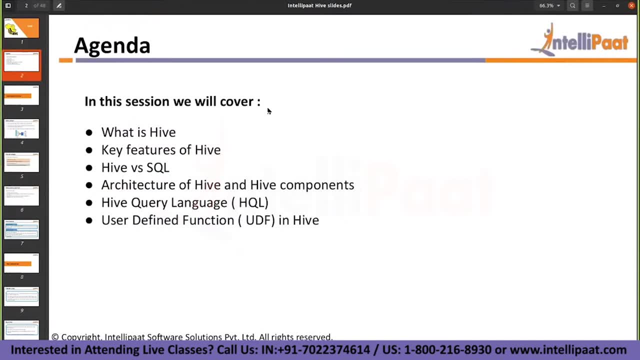 have to install oracle virtualbox. okay, fine, so let's get started. so what do you know about hive? what is it used for? yes, thoughts this type, at least a very high level understanding. what do you know? um, you're seeing here just a few things, okay, so you can see a lot of perspectives. 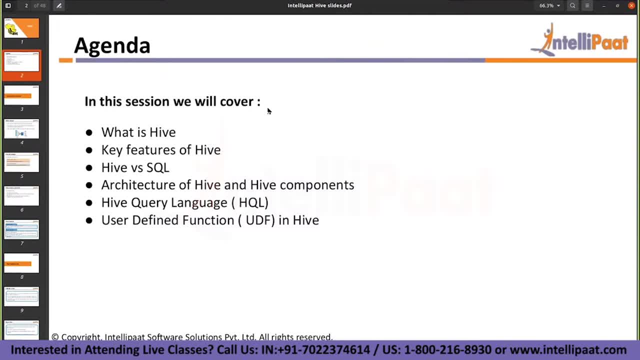 right once you see this kind of image right now. so let's give it a few more looks. so the first thing that people are asking in this type of file is: what is the organization of the file and the primary system of the file? is it a device that is? 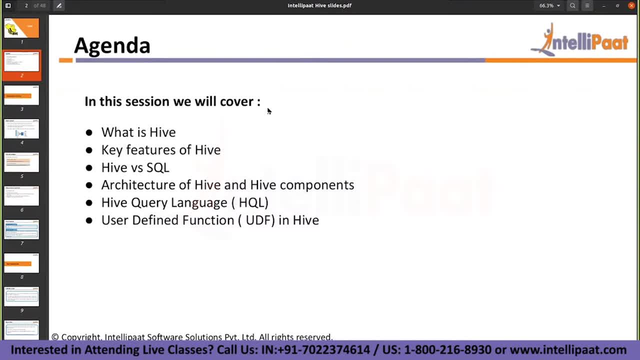 using a high-tech device. okay, so that's a very big topic and that's very important, but what do you know? the first thing that people ask when you talk about a high-tech device is using it because there are their existing systems, are still built on top of it. then there is no other. 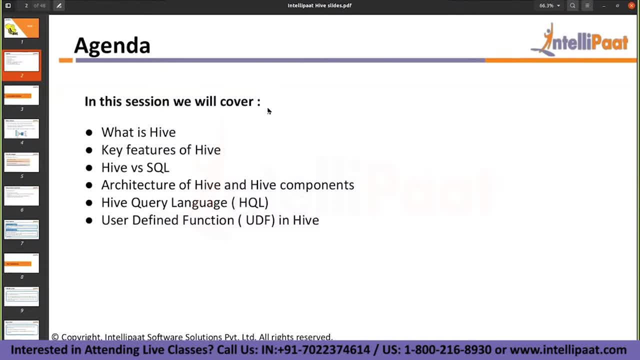 choice, they have to use it. but other than that, there is this: this: this map reduce programming, at least hands-on, is completely out of market, okay, so that's the reason we don't include map reduce programming in any of our sessions, hands-on in any of the sessions, because that's just just 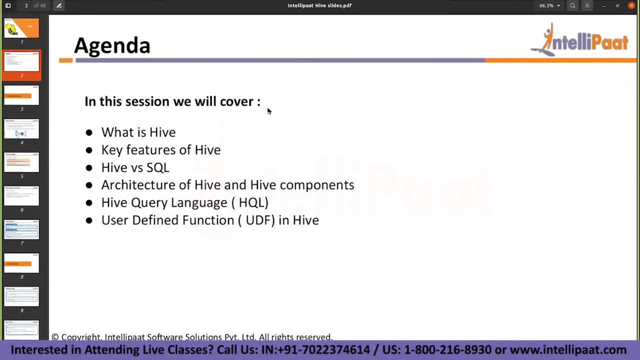 not required at this moment. you just need to understand the flow or architecture. that should be sufficient. okay now, so we've seen, uh, we've at least. uh, we at least know what map reduce programming is is like it's written in java: you have some classes, methods defined and spark you. 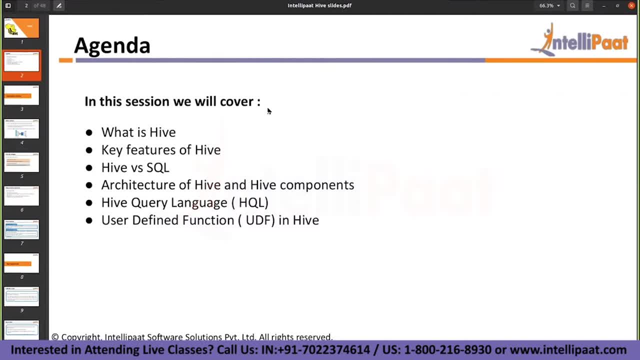 must be knowing this is something related to scala and python or whatever, right. so so when you, when you before, before the existence of spark, we were always discussing about map, reduce, pig and what scoop, different, different tools. so all this data, you processing tools that we're talking about have their own programming, programming framework. 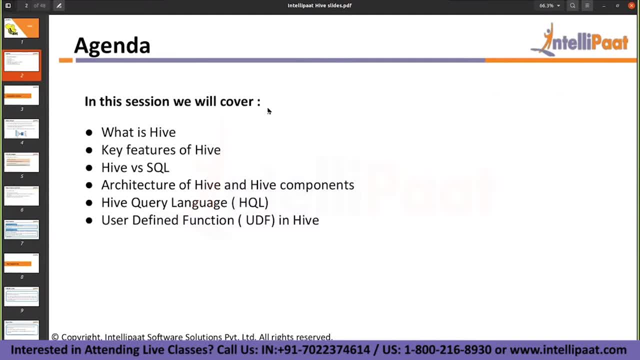 right. so they are. they are kind of considering the data to be generic. so regardless of whatever the format the data is available in, if it is in a csvg, is in park, it, avro, doesn't matter it. it just takes data in a summon so and so input and it will just process it. but if the data is actually 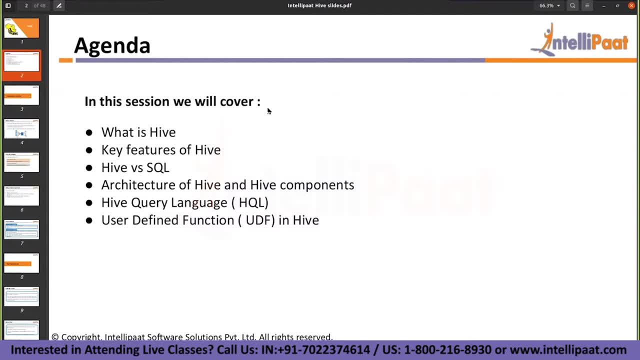 in a structured format, right so most of the companies, what they generally do, is in the existing environments. they generally definitely have the data in a structured format and they have the data in a database- right so they have the data in their databases: oracle, postgres- most most frequently used- and some other teradata or whatever, right so when they want to migrate everything into 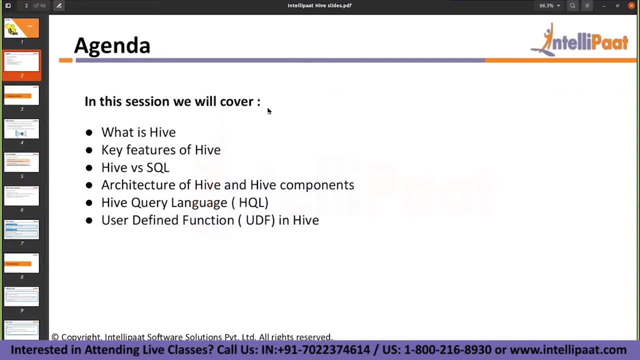 a hadoop ecosystem into the hadoop platform, they should be able to migrate the data that is already available in their databases, so relational databases. i'm saying right, so there is no other tool. if you can, if you can, uh, reiterate this again: there is no other tool or there is no other. 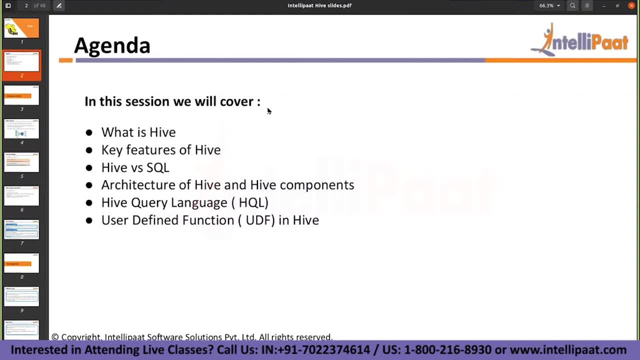 way, which is which is, uh, better compared to an sql way of handling a structured data, right? so sql way of handling, or sql storage or relational database handling of a structured data is the best way to work with it, right? so, even in hadoop, when we, when we get the data into hadoop ecosystem, 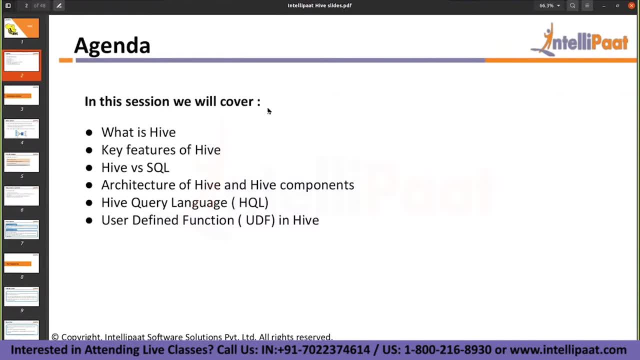 so, whatever the structured data we received into the hadoop ecosystem, so using it with map register program or pig doesn't, doesn't give you proper results, doesn't give you so much control on the data because the data is not so much control on the data because the data is not so much control. 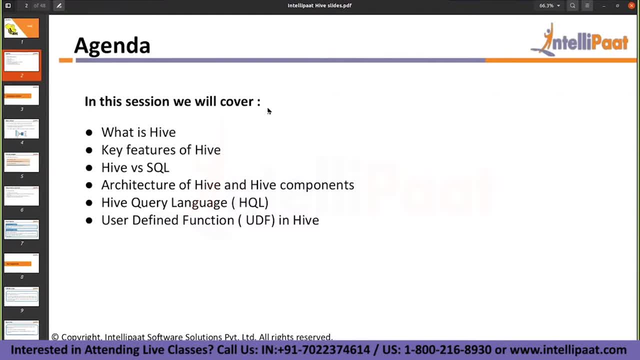 on the data, because the data is not so much control on the data, because the data is properly structured. you can. you can create the databases, you can create the tables, you can store. you can do a lot with it. so when you have such a framework, when you have a such a facility, why to? why to go with other? 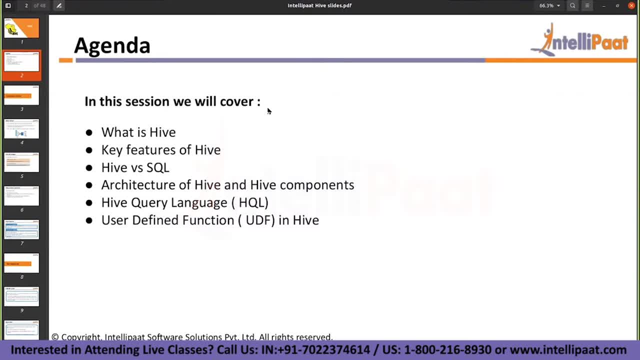 tools and technologies right. so to avoid all that, they have developed an sql kind of a framework for the data which is coming in from an external databases. okay, since this is only meant for it. so if the data is coming in from the external databases, from the relational databases, most, most, 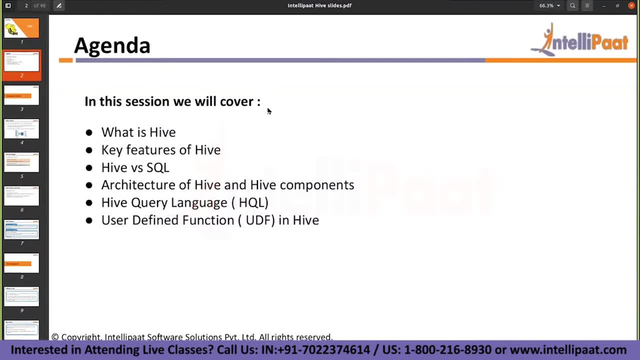 precisely if the data is in a structured format. to to be very precise, if the data is in a proper structured format and if the data is coming from a relational databases, that's that's that's when we will be using hive as a processing tool or a. 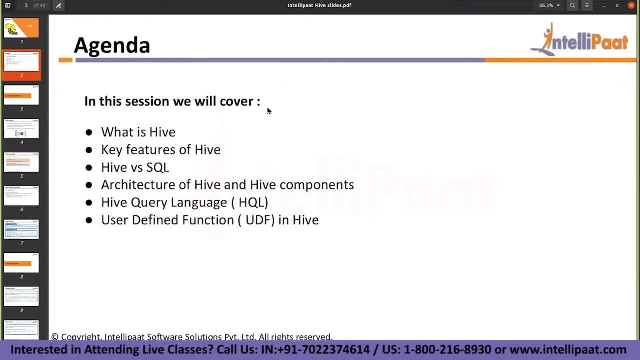 storage mechanism. okay, so internal to it it's again a map reduce framework or it's a yarn framework. whatever the processing mechanism hadoop is using, it's going to execute the same way. but uh, what we are gonna write is is a hype query, a simple sql query. so internally it's going to get. 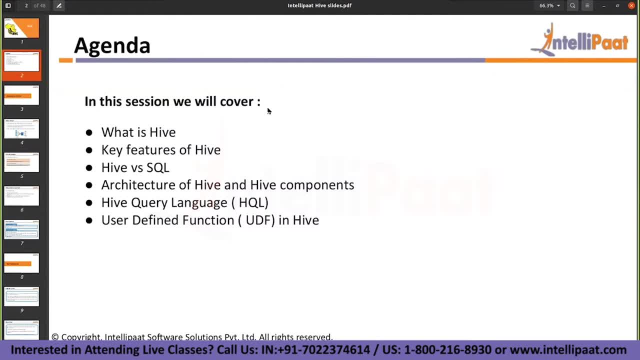 converted into a map reduce program and it's going to execute it. but that's not our concern. okay, so we don't have to worry about what it is it is executing. but as long as we are writing a simple sql query, we are fine with it. so this is kind of a sql like a framework. like i said, 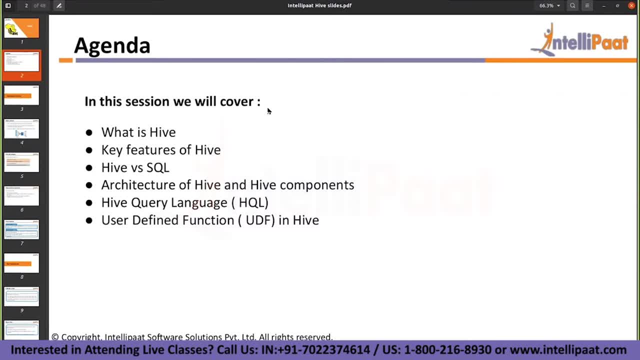 which is used to process a simple structured data, tools, data formats. okay, so what are its sources? generally, most of the times, the sources would be the relational databases. so how do we get the data from a relational database? this also we discussed. we just had a quick chat about it. if the data is available in a relational database, how do we get it into a? 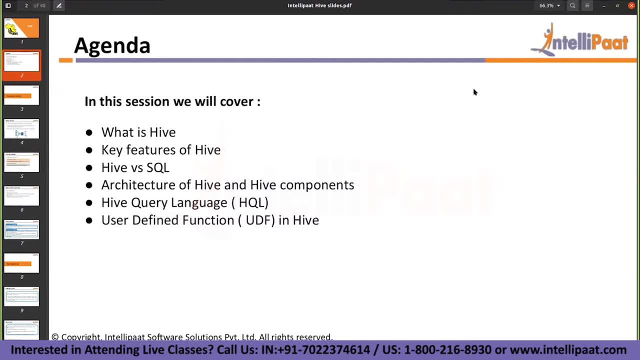 hadoop framework. using what tool? okay, so we have something called a scoop. okay, so scoop is a tool which is used to interact with the relational database and migrate all the data that you have in a relational database to your hadoop file system. okay, so, after you migrate the data into 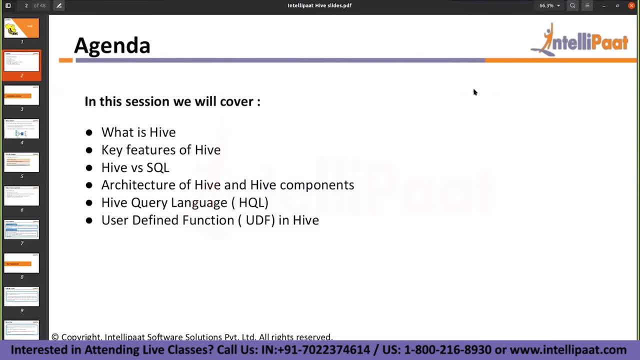 hadoop file system. it's. it's gonna be in a proper simple plain text format. okay, so plain text format or a csv format, whatever a tab supplement data format. so, depending on the use case, you'll be creating whatever the data format, but it's going to be in a structured format only. so on top of that data you'll be creating the tables. 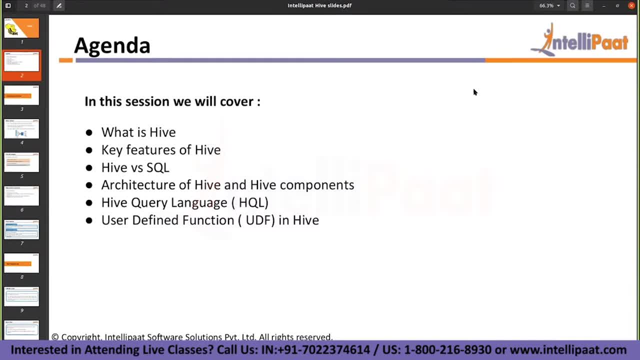 okay, so, similar to whatever schema you have in a relation database, you create the same schema on hive and you you load the data whatever you have in the hdfs locations. okay, so that's how you'll be migrating the data from a relational database to your hadoop ecosystem and create. 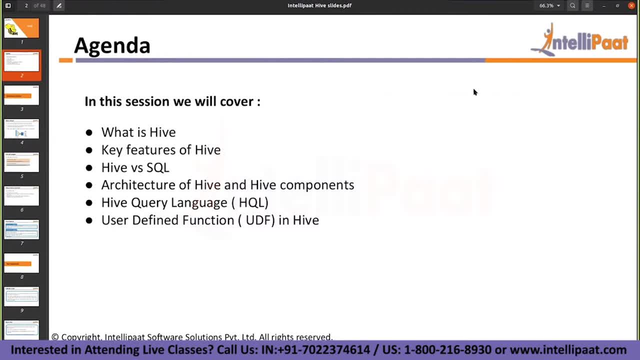 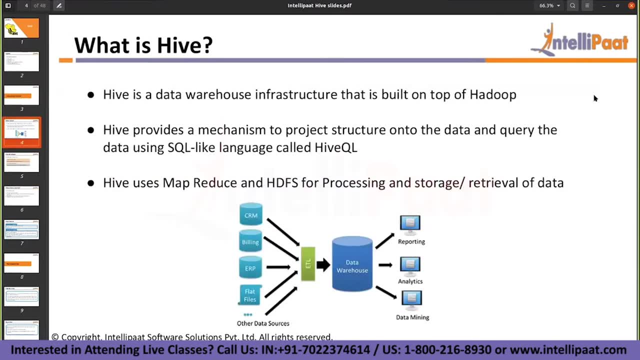 hive tables on top of it. okay, so that is the main purpose of it and we'll see how exactly, how exactly it is being done and what are the different features allocated to it. so now, generally it's a data warehouse, uh infrastructure that is built on top of hadoop. 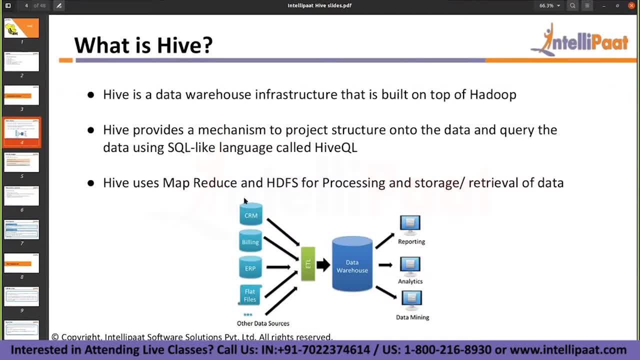 you know it's a skill like language and hive uses map reduce and hdfs processing and storage retrieval of data. so internally, like like i was saying, it's always going to be map reduced and hdfs is going to be the storage and what. what you actually write to interact is a. 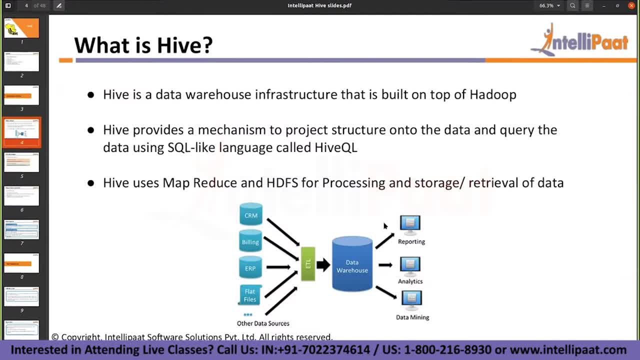 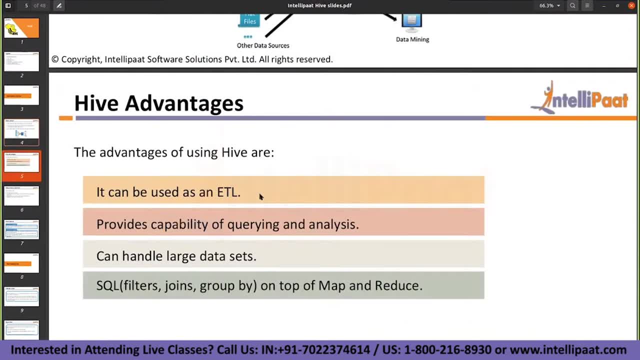 square like program that is hql, hive query language. okay, so similar to sql, you have something called as an hql then. advantages: it can be used as an etl. uh. etl mechanisms- extract, transform and load, provide capability of querying analysis and can handle large data sets. and we have this. filters joins group by on top of this map: reduce. 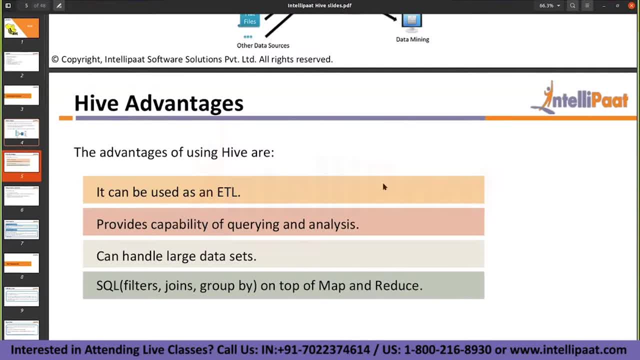 so all these things? we know it is an etl tool, it's used for querying and we it's. it's meant for dealing with large data sets. obviously it sits on map reduce and hadoop and um filters, joins and group by on top of this paper: reduce. so if you have to perform a filter simple. 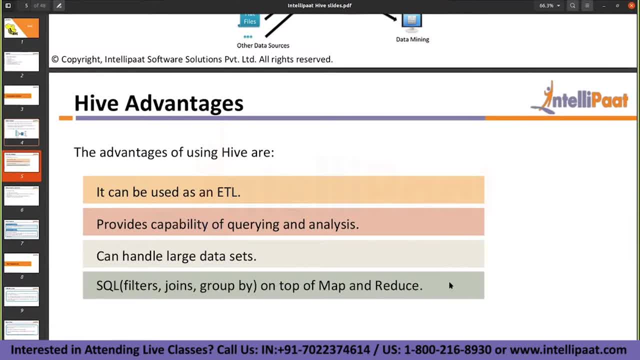 filter condition using a map reduce program. it's a complicated process. it's not a complicated process for a java developer, but there is some amount of code that needs to be written right. but that's simply executable using a simple high query and where not to use hive if the data does not cross. 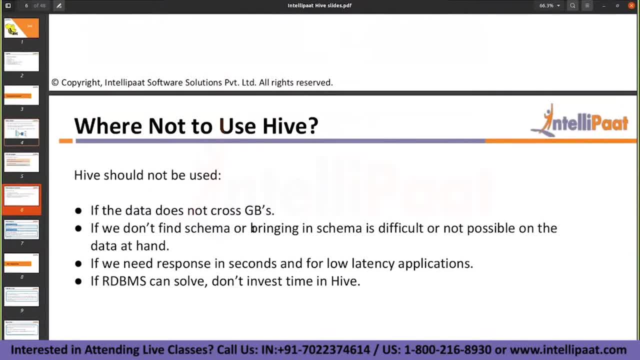 gb's if the data is less than gb. if you don't find schema or bringing in schema it's difficult or not possible on the data at hand. if we need response in seconds of a low latency applications if the data rdbms can solve, don't invest time in hive. so this is the use case. so if there is no problem with the relational 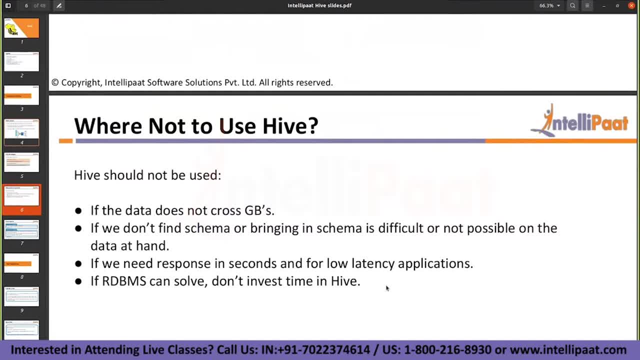 database, then there is no point in migrating the data to hive and rewriting the same amount of queries. first thing right, and this is a low latency application. if you, if you, want a query to generate the results in in some seconds of time, it's it's not. it's not a suitable solution. so this is mainly. 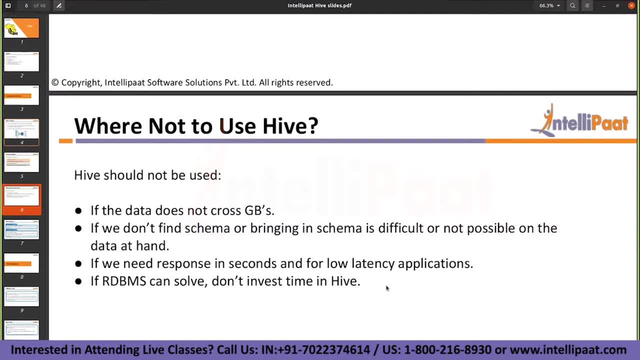 meant for large amounts of data sets and dealing with large data sets or large amounts of joints or partitions if the data does not cross gbs. if the data is very small, then then what is the need for you to load it to hive or what is the need for you to use hadoop framework at all in this particular? 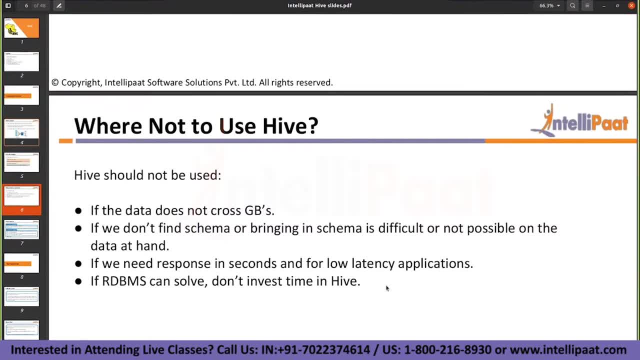 case, right. so it's only meant for large data sets, large data processing use cases, and if if there is no problem or if you are comfortable using the rdbms framework for a specific use case, then then don't invest time in high. this is what it's going to, be right it's. 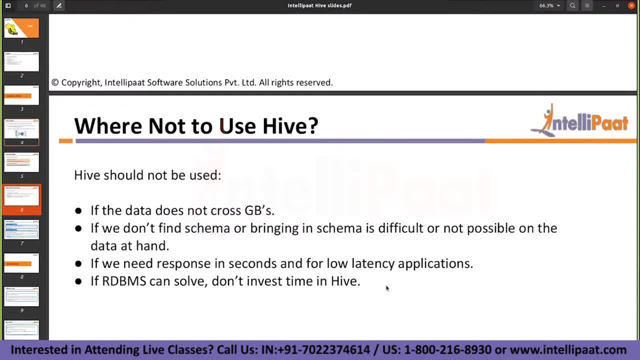 just a replica of an environment on a hadoop framework, but there is. there is nothing um hive can provide which rdbms cannot, at least okay. so if you are, if you are fine with the relational databases, if you don't have any issues managing the data or handling such large amounts of data, 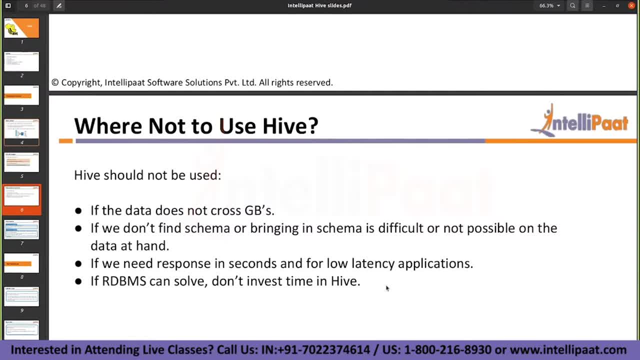 sets, then there is no point in bringing the data to hive. okay. so in most of the cases, guys in. in most of the real-time scenarios, the problems would be something like if- if the data- upstream or downstream is- is somewhere interacted to hadoop, let's say the data to a 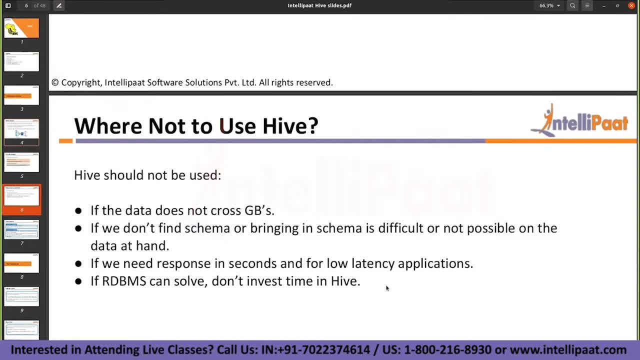 relation database is coming from so and so source, or the data from a relation database is going to a so-and-so source, so-and-so destination, right? so in that cases, if the upstream or downstream is is somehow related to a hadoop framework or a hadoop ecosystem tool, then there might come a possibility. 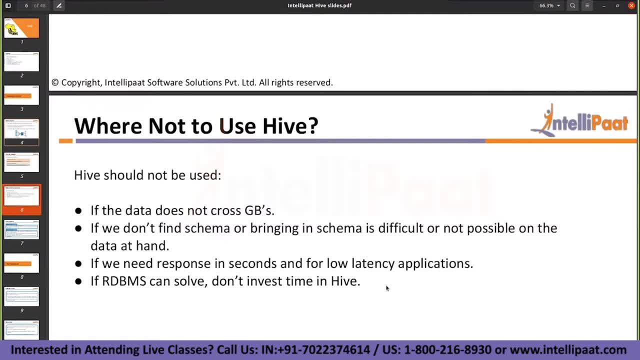 where you have to migrate this relation databases because, for example, if the data is coming from a hdfs location, we we don't know where the data is coming from, but the data is being loaded into hdfs. now your rdbms has to load the data from a hdfs location getting it. so the scenario is from: 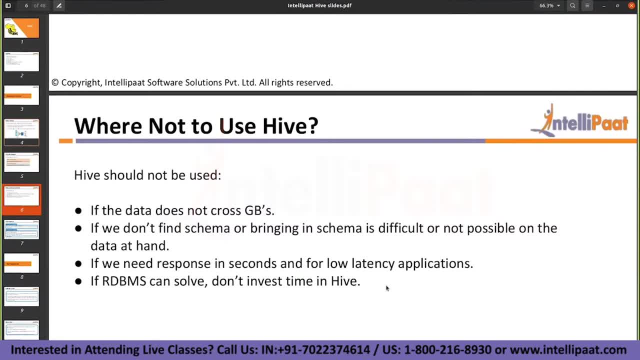 hdfs, you are extracting the data outside the hadoop framework and loading it into your relational database and from relational database. whatever the applications that are hosting, that are hosting on top of this relation database, relational database are also interacting with the hdfs data or also interacting with some of the tools in the hdfs in hadoop. so 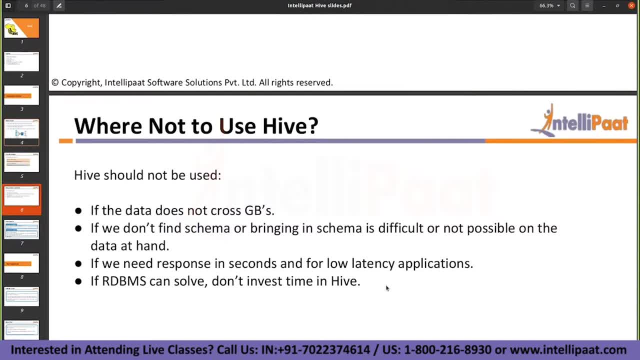 in in these particular scenarios. so only relational database is something which is out of your environment, out of your hadoop framework. so rest, all are sitting inside inside the hadoop framework. so in these kind of scenarios you may have to migrate everything into hive and you you'll make everything local to hadoop framework and it's going to be fast retrieval okay. 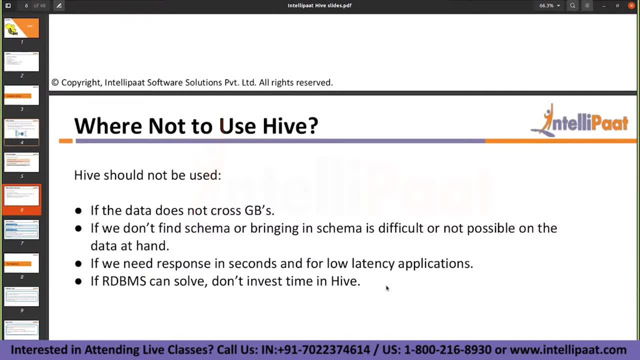 it's going to be helpful in the quick retrieval of the data because, uh, apart from that, apart from that, if, if the entire, uh, some of the time, some of the times, most of the times, clients are gonna request you to migrate into hadoop framework, that's okay, because bulk elemental integration management would be under hash vampire. 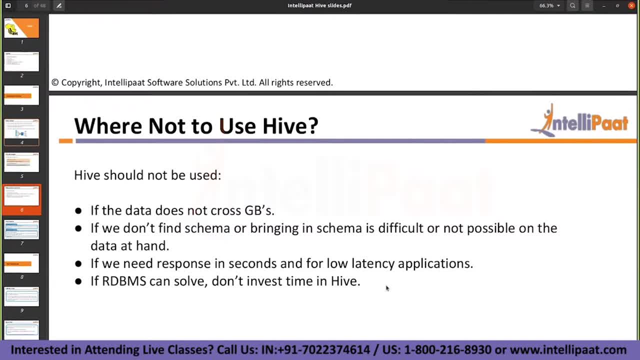 one of the requests you can, you're gonna get. there is no other option other than to migrate it and in some scenarios, like i said, downstream or upstreams are somewhere related to the hadoop ecosystem. so these are some of the scenarios you might encounter wherein, uh, there comes a need for you to migrate. 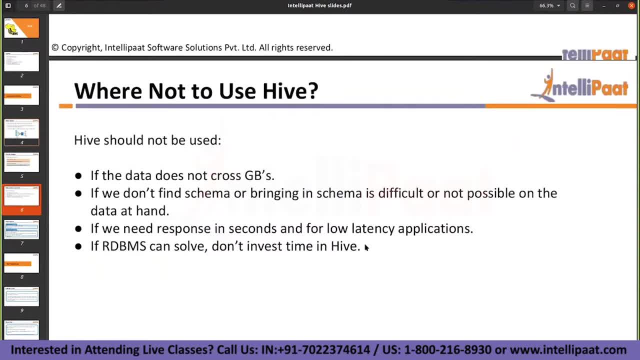 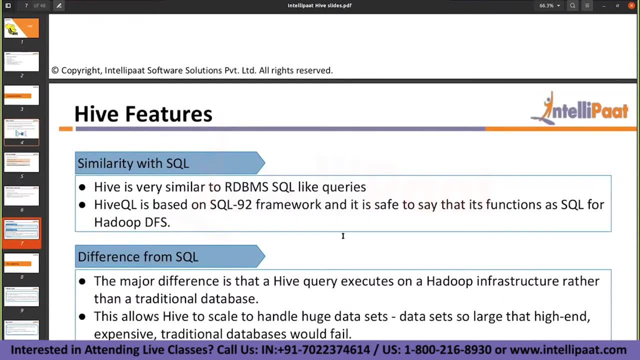 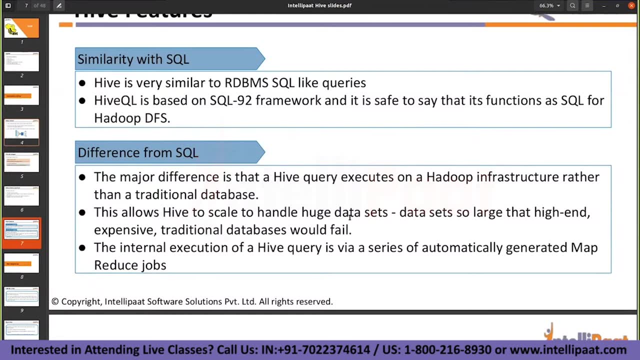 to a high, high environment. okay then, the features being um similarity with sql, that's, that's a major feature, okay, uh, difference from sql, the major difference is that high query executes on hadoop infrastructure rather than a traditional database. yes, i have to scale on a huge uh data sets, um data. 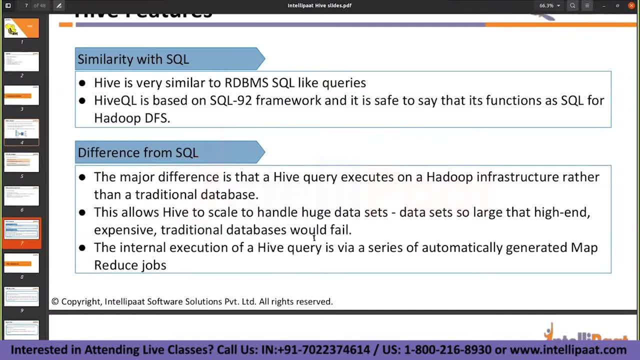 sets so large that high-end, expensive traditional databases would fail. the internal execution of high query is by a series of automatically generated map- reduced jobs. so any any new thing that we have seen? so, uh, yes, highway executes on a hadoop infrastructure and, uh, that's different with the. 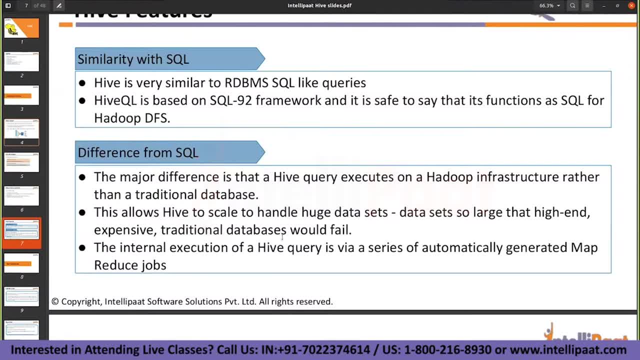 databases and where you have large amounts of data sets where your traditional databases would fail. that's where your hive is gonna help you to scale the data across multiple clusters and the internal execution to hive is again map reduce, like i said, every query, every operation that you perform on. 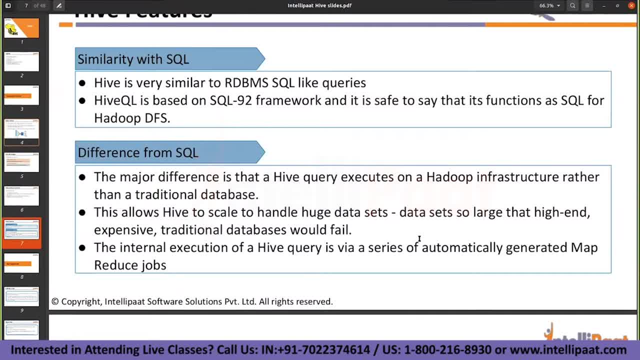 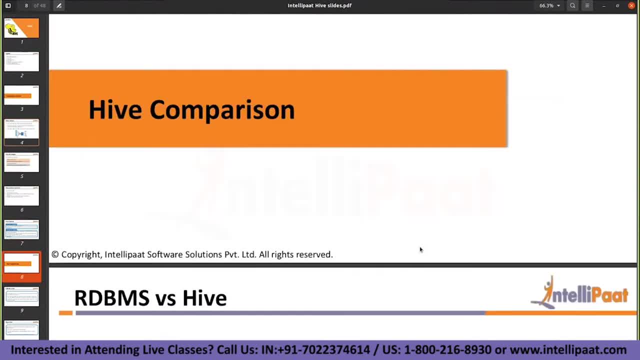 hive is getting converted into a map reduce program, ultimately, and it's going to get executed on top of the map reduce engine and will get you the results. okay, rdms versus hive, you can. you can just just read through whatever the comparisons we have. so pig versus high, we don't know what is. 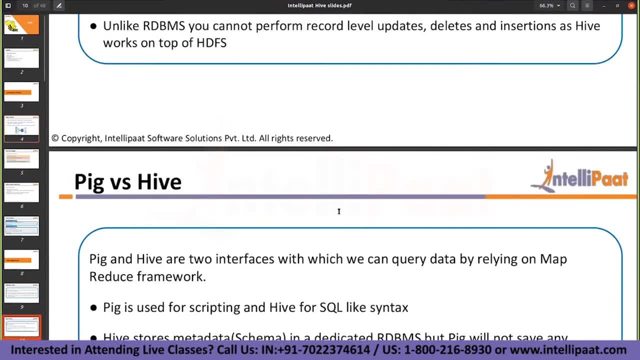 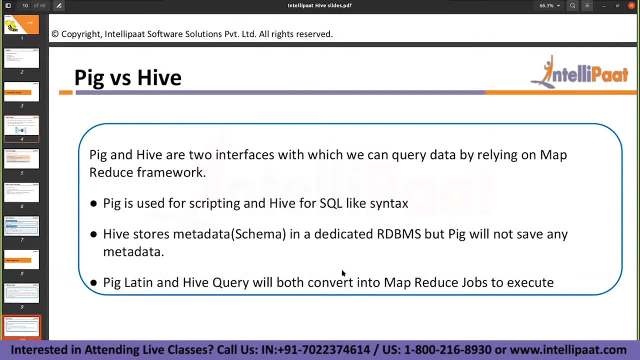 pig at this moment. so forget about this comparison. so pig is mainly used for non-structured, unstructured data sets, okay, where you do not have a proper schema. so pig is also out of the market now, guys. so there is no company which is using pig in their 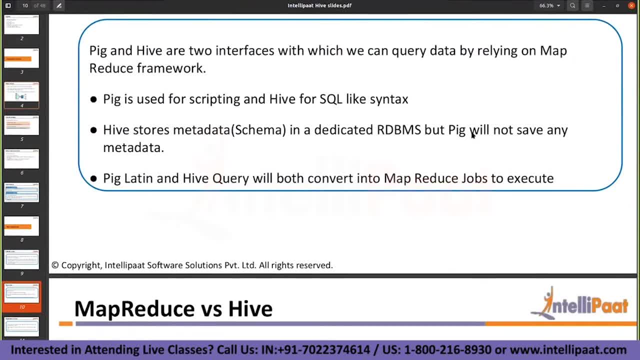 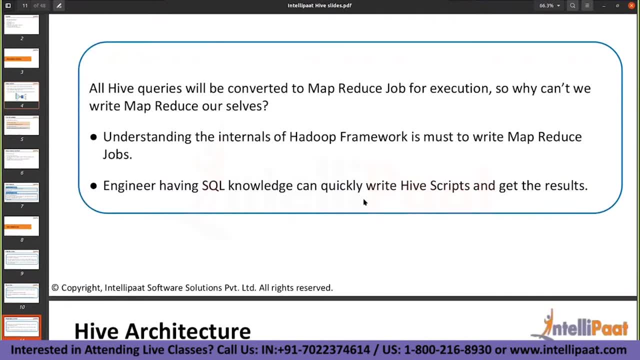 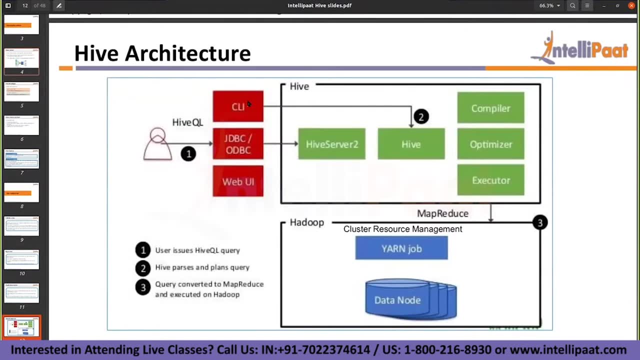 environment, because there are. there are many better tools than pig. okay, so map reduce versus hive, you can just read through them. and there is something called as hive architecture. okay so cli, jdbc, odbc and a web ui. so there are different ways of interacting with your hive interface: high engine, execution engine, um. one of it is using a command line, so using a command. 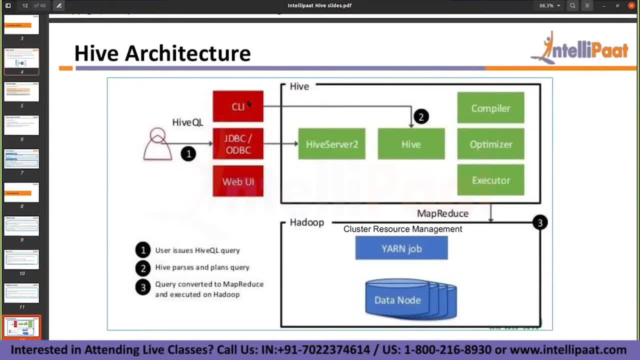 line window. you write a hype query or you write an insert query or whatever the queries you want, and there is a jdbc or overload bc. so when you are trying to interact with an external system, like i said, there is a scoop connectivity right. so on the source side there is a relation database. 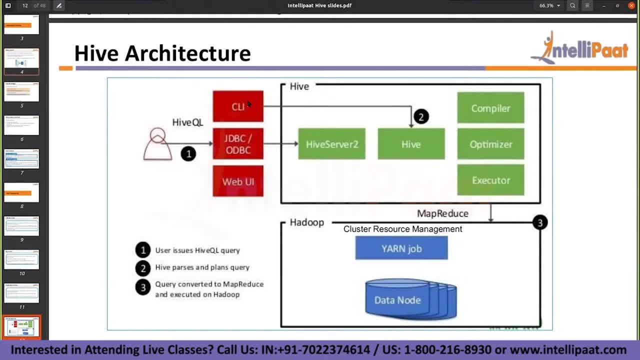 on the destination side there is a hive command, hive hive terminal. so how do you interact with this hive execution engine using scoop? so it's going to be through a jdbcrn odbc connection here and there is one more web ui, so using the web ui it's not. it's not available. uh, for for all the 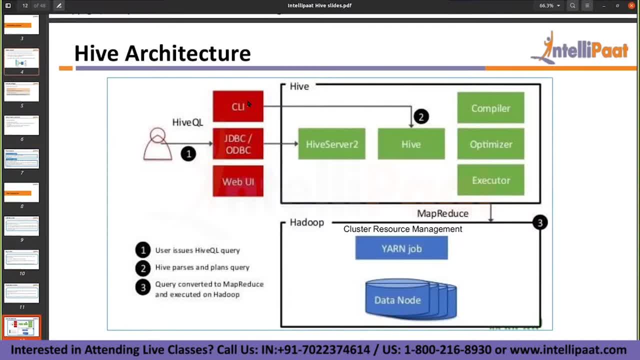 versions of hadoop it's. it's not available in the open source version of hadoop, but in cloud era. uh, in a cloud era interface there is something called as a hue terminal. okay, h u e hue terminal. so in hue terminal there is an option for you to um write a query in the in the in the web ui itself. 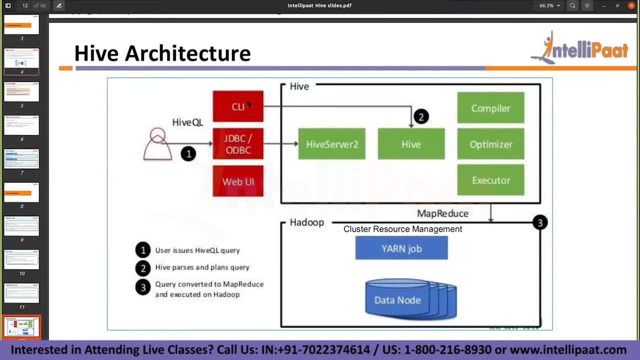 okay, so there is an option, a hive editor available within the cloud era hue terminal, wherein you can write the query and you can actually interact with the hive tables. okay, so there are different ways of handling it. that's why i'm showing you how to do it. so there are different ways of handling it. 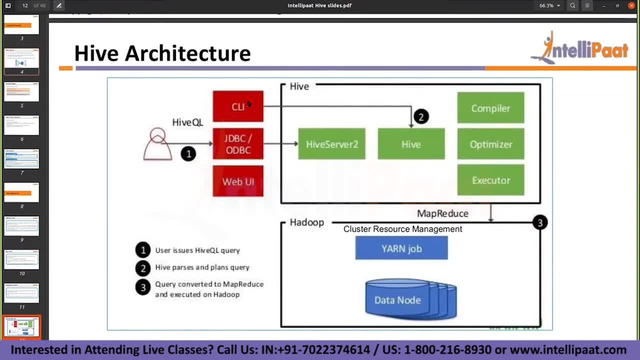 what it's it mean to say, using a command line or through a jdbc, odbc or through a web ui. so now, whatever the query you submit is is gonna get to the hive server 2. so this hive server 2 is is kind of a master or it's kind of a main execution engine, that's that's going to get the request. 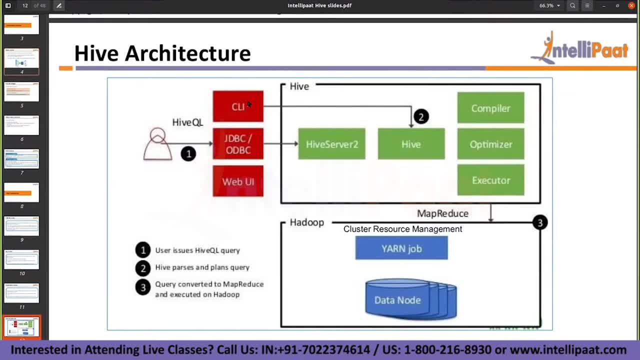 and so this is again. hive server 2 is an external interface where you are trying to interact with the external servers. that's when you will hit the hive server, the command line it's. it's directly running on top of your hive execution engine. so that's what it means to say: using a command line. 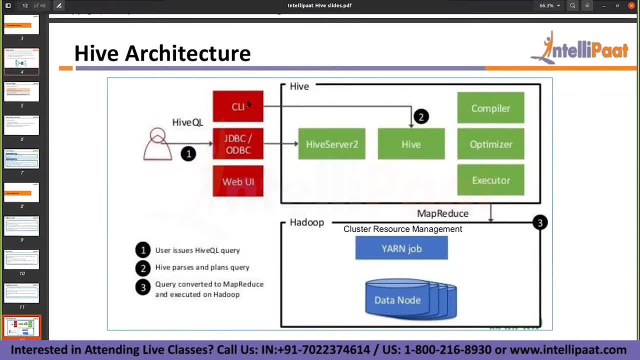 so that's what it means to say using a command line: it's. it's directly running on top of your hive. so that's what it means to say using a command line: it's, it's directly running on top of your hive. and there is compiler, optimizer and executor. so compiler is used for compiler and optimizers are. 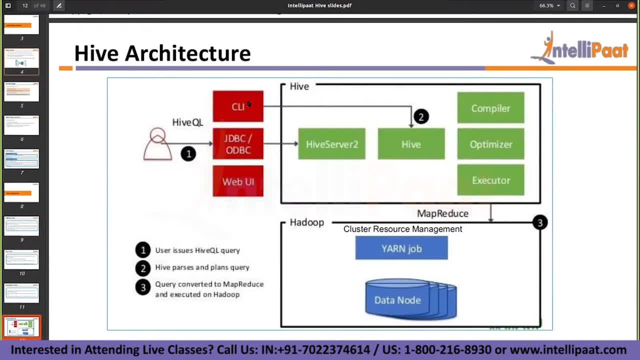 mainly used for the syntactical verifications and validating whether the particular schema is available, uh, in in the particular table. so when, for example, if i'm saying select id from emp, that's the query i i submitted. so first thing is whether the syntax of the query is correct, so that that 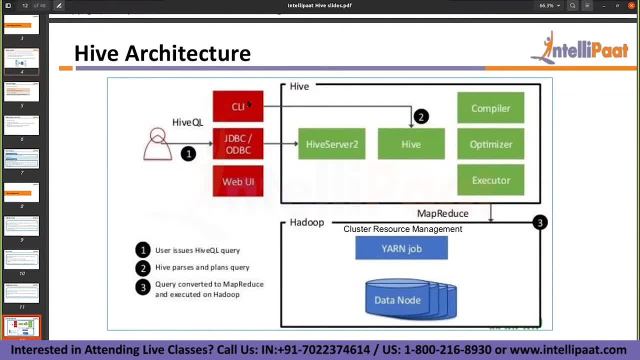 validation is done and the next next next process will be uh- whether the table emp is available in the uh hive environment hive metastore and whether you have the column id available in the hive metastore. that validation will be taken care of and then your executor will start executing it. so 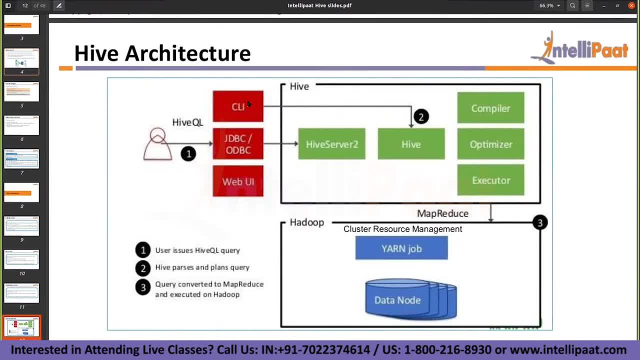 what executor will do is it will convert a high query into a map reduce program. okay, so, whatever the select star from query you have written, that gets converted into a map reduce program and it's going to get submitted to a map reduce engine. okay, so hive submission is done here, whatever. 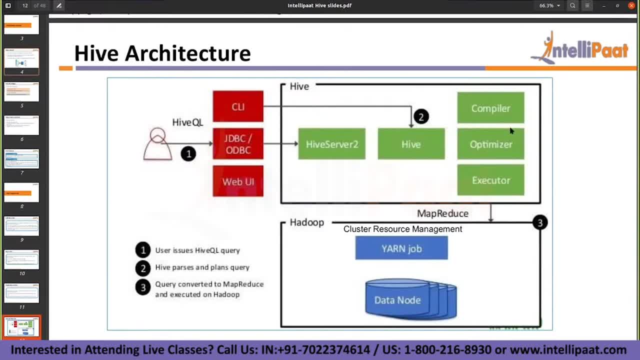 the query you're submitting. it is done here. compiler and optimizer will will make sure that. make sure the um syntax and the uh validation of the query is done on the hive side. whether the proper table is available or the proper column name is available, proper syntax is provided. 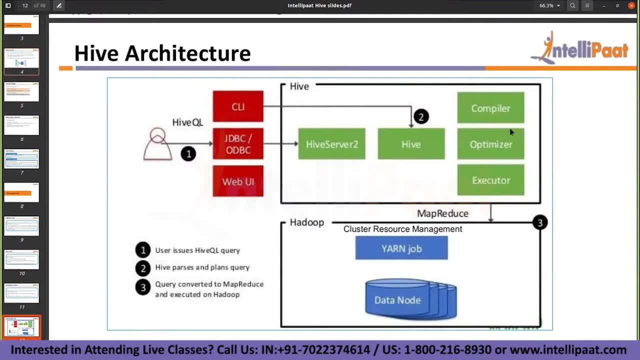 and then it will send to multiple executors wherein they will convert the hive query into a map reduce program. okay, so this is where actual conversion happens and that's when your map reduce job will get executed and the result will be shared with the in the in the, whatever the user interface you submitted the query. 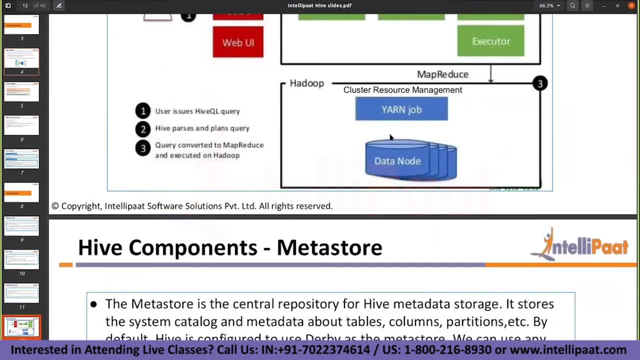 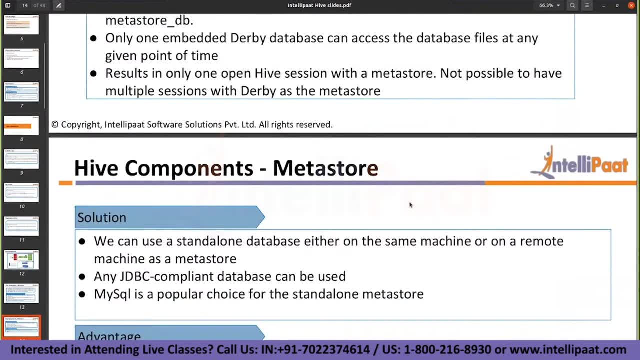 okay, so there is this metastore available. so metastore is something which is used to store the schema or the data type formats of a particular table. so by default, hive metastore is is kind of a database. it's a derby database which is available within the hive environment only. 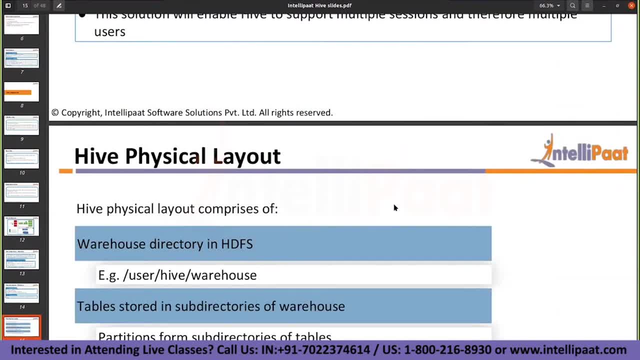 okay, you're not supposed to. i mean you are not. you need not create any external database for it. so hive itself is a database for us. it's itself is a etl data warehousing tool. but for that, to store the schema, to store the table information, to store the database information, you have some internal database for it. that's we. 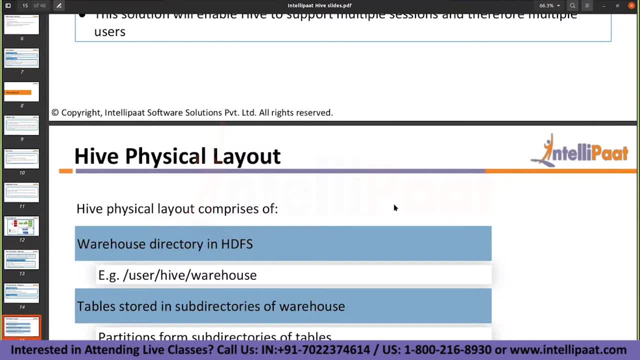 call it as a derby database, which comes with a default derby database, and that is what we call it as a metastore. okay, so you can also integrate it with some external databases also, but that's again some kind of a complicated process, as in when- i mean only when it is required- you will 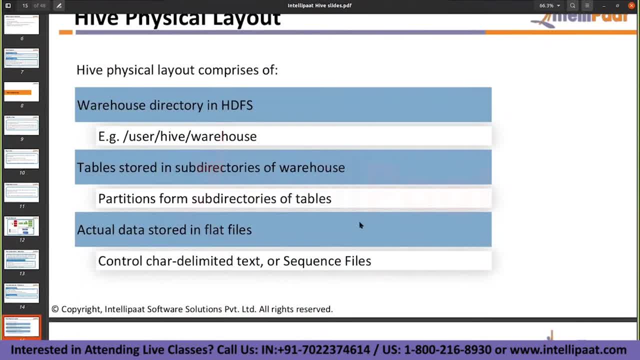 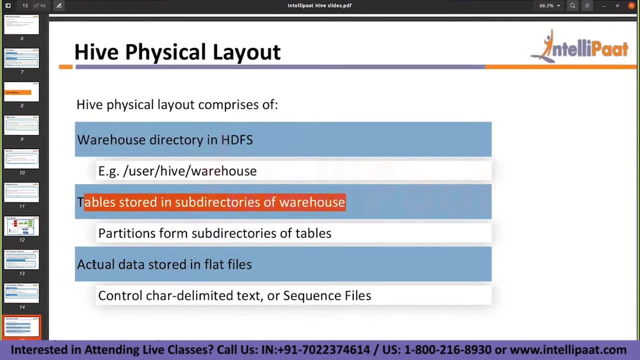 take care of that particular thing. other than that, it's. it's fine, it's straightforward, mislead and physical layout is a warehouse directory. uh, tables are stored in sub directories of a warehouse. actual is stored in the flat files. so how a data is stored in a hive table. so one thing you need to. 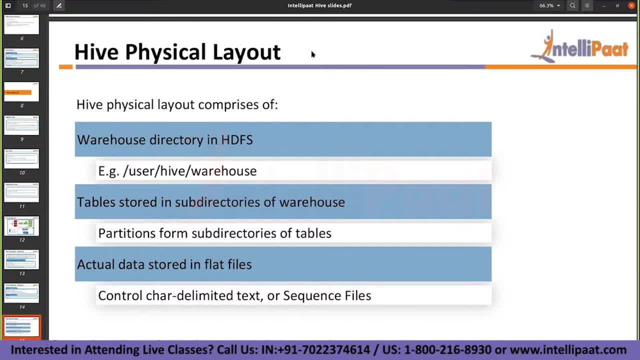 understand here is whenever you are loading some data into a hive table, so generally in, if you, if you look at the relational databases, for example on oracle database, so when i do an insert into a so-and-so table, where is the data actually getting stored? will you be able to see the 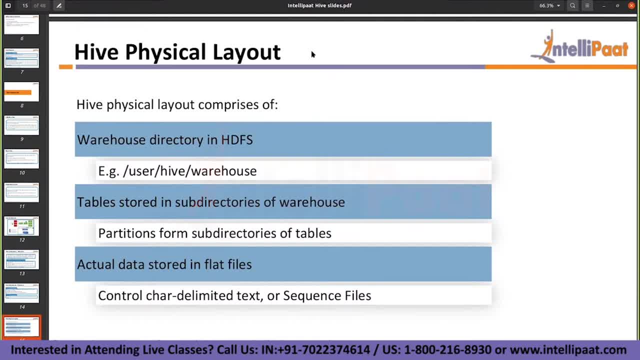 physical storage of the data, where exactly it is being stored. how many of you have interacted with the oracle database or postgres database, any of the relation data bases, mysql or whatever? how many of you have actually worked with them? okay, so you have a table, mysql, is it? so you have a table? uh, you have some data- 100 records- in it. you. you now inserted. 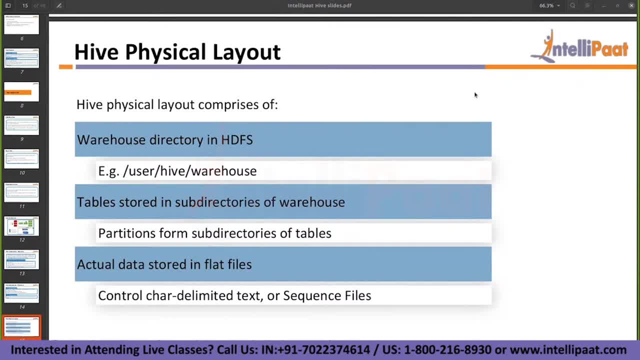 another 100 records. so where is the data actually getting stored? where is the physical storage of the data? can you see that? yes, so you'll have something called as a mysql server which will hold all the information, but you will not have a privilege i can say or see, not even the actual. 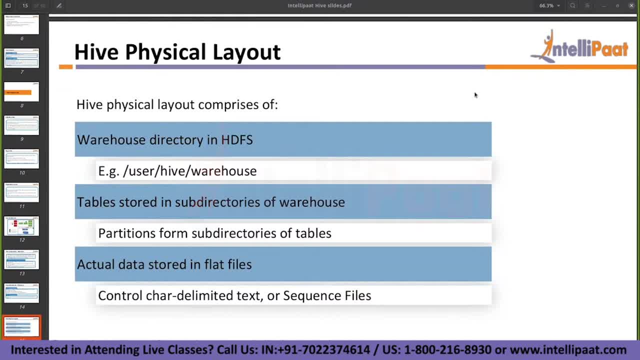 access. but see, you will not. you'll not have a segregation of these tables, data, databases, and all that in the hive server, in the mysql server as well, right? so in in high. what is going to happen is there is no data that is holding on the hive table. i mean, what i'm trying to say is, for example, 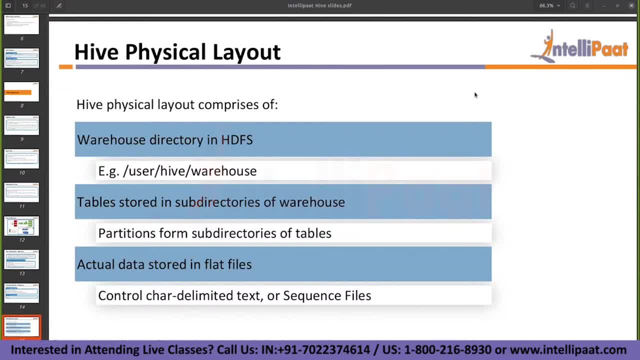 i created a hive table, emp, with id name and salary as the um, as a columns. so when i insert a data, your data will get loaded into htfs. it's not on the hive table that you're loading. when i do an insert command or when i do a, whatever the load command, the data will. 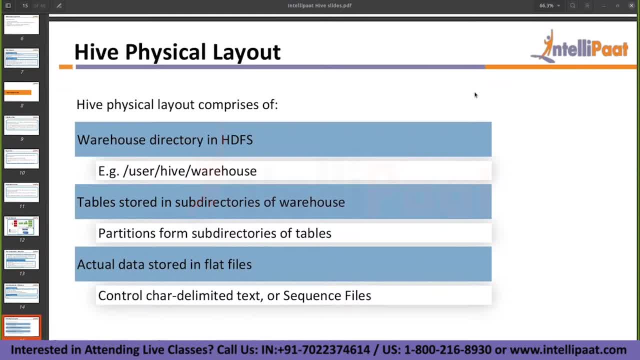 get loaded into hdfs and your hive table is actually pointing to that hdfs location. okay, so whenever you are creating a hive table, you will allocate some location for it in the hdfs. that means whatever the data you load from there on will get loaded into that location. 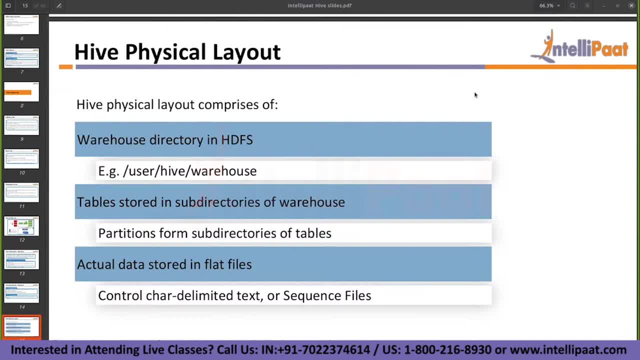 or whatever. the data you load into that location will be displayed on the table getting the different. okay, so whenever i'm creating a table i'll give some location in hdfs for it. okay, so when i do an insert on the hive side you will find a file getting loaded into a hdfs. 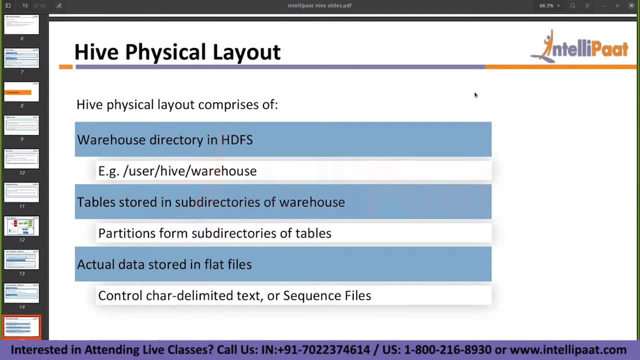 location in the same hdfs location. or when i do a normal cp, okay, you know cp command, you know move command. right, you know copy from local, copy to local. all that commands. so when i, when i load some file into that location, when i do a select star from emp, whatever the data, 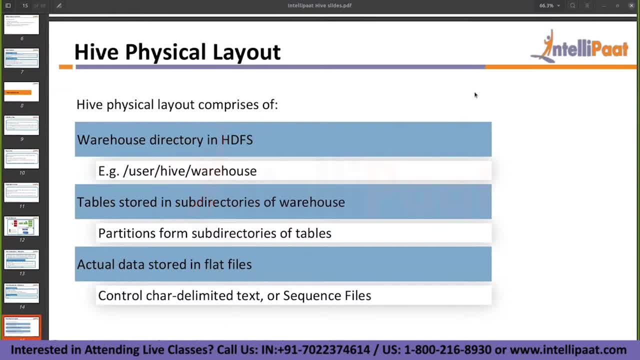 you have in that new file also will get displayed in the hive table. that means the actual hive table is actually is only pointing to that location in hdfs. so whatever the files you load, whatever the data you remove, whatever the files you remove will will reflect in the table information. that's what. 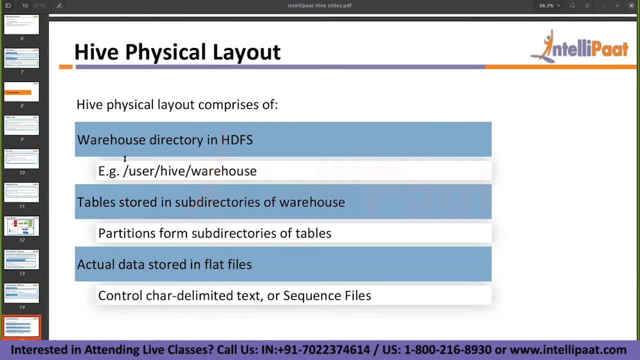 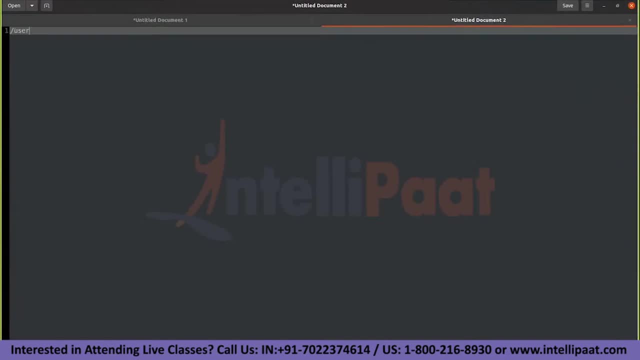 i mean to say getting it. so now, if i have to show that one second, okay, so let's do this. i'm sharing my- is it visible? notepad, so you know the hadoop locations. now, right, so this is uh user, um, some hadoop. this is all hdfs. let's say default hdfs location. 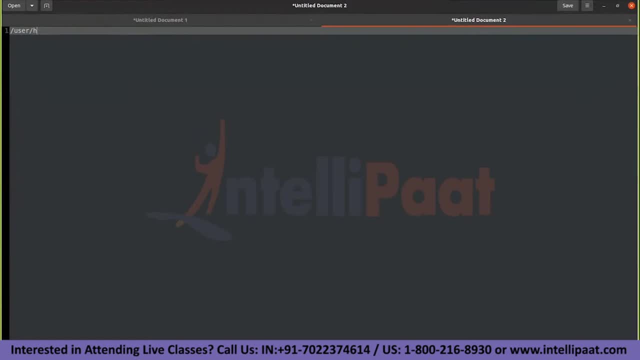 okay, so inside user hadoop i have um user hive warehouse. this is a default location for your hive. that means so this path is your hdfs, like in the command line just now we have. we have executed hadoop fs, hyphen ls. this is the command we executed, right, so after a slash. 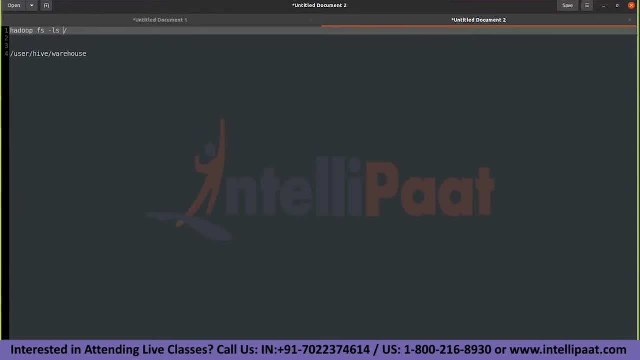 whatever the data you have inside this particular root directory, everything is hadoop file system storage, right. so within that you are allocating some location, some directory. user is one directory, hive is one directory and warehouse is one directory. so this particular location you are pointing as a high warehouse. that is a default location of your high. so so i'm calling this: 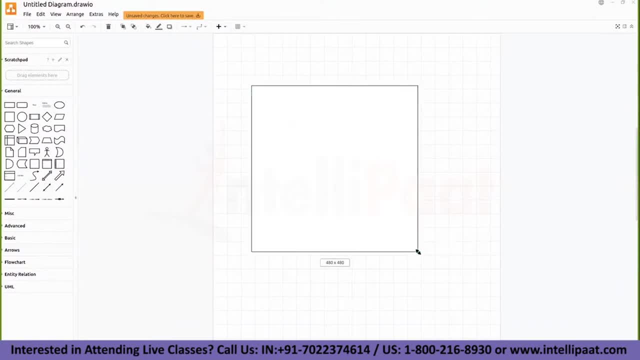 entire thing as a hdfs. okay, so inside this hdfs, some portion of it will be allocated for your. okay, so this path is your slash user, slash hive, slash warehouse. this is your you directory, hive default directory- getting it. so this entire thing is htfs. okay, so it doesn't. 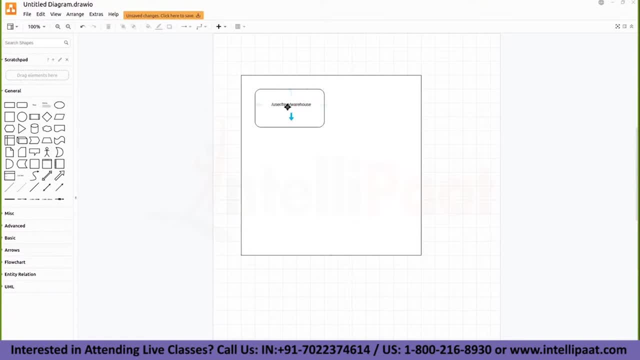 matter whether this is only this particular portion, is under the control of your hive execution engine or hive framework. okay, so, whatever the tables you create from here on, okay. so let's say i created a database, let's say i'm creating create, so create um database database sample. this is one command that i'm computing and then 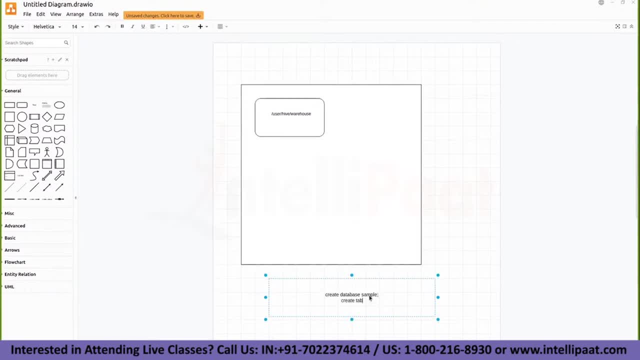 and then i created table employee and inserted, let's say, load data into table. okay, so these three activities i have done. so what is going to happen here? so, after i create a table, after i create a database, for that matter, after i create a database, there will be a directory named slash user- slash hive. 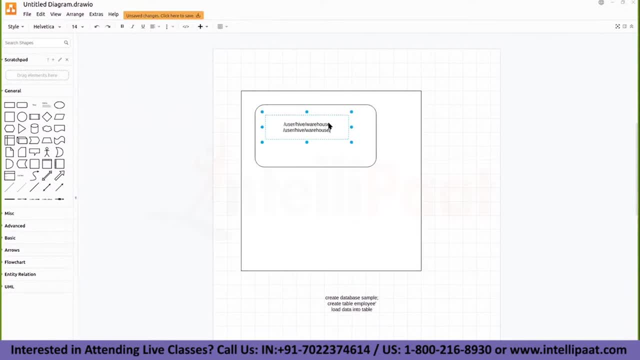 slash warehouse, slash sampledb. under sampledb there will be a directory named employee. getting it under employee employee, i'll have whatever the file. i mean. you can say uh, hollowtxt, or some part, file, part, hyphen zero, zero, zero. so that means under user: hive warehouse. this is my core directory for your. 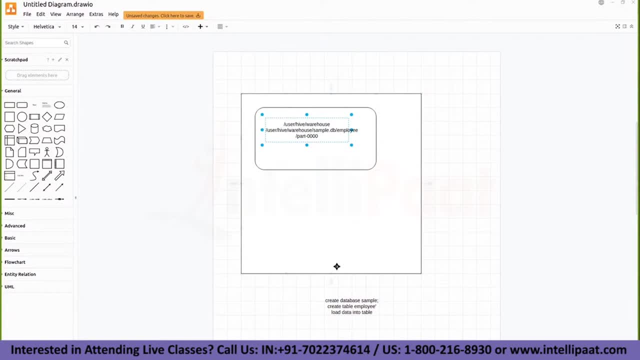 hive execution. so now you logged into the hive shell and you created a sample. so sampledb will be your primary directory under your user hive warehouse. so when you create a new directory there will be a new directory path that is getting created. so now you logged into the. 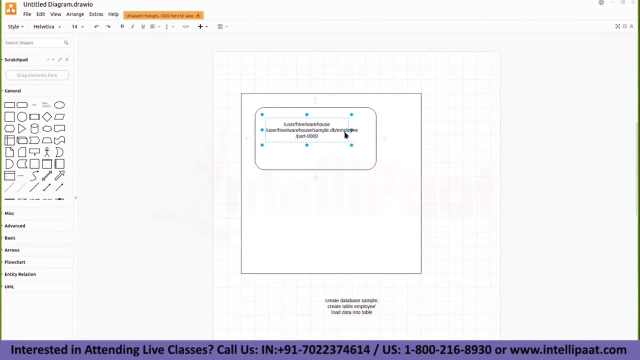 sampledb and you created a table so table name will be your employee, so table name will be a directory name inside your sampledb folder getting it. so sampledb is also a directory and every table you create inside this sampledb will also be a folder, will also be a directory. 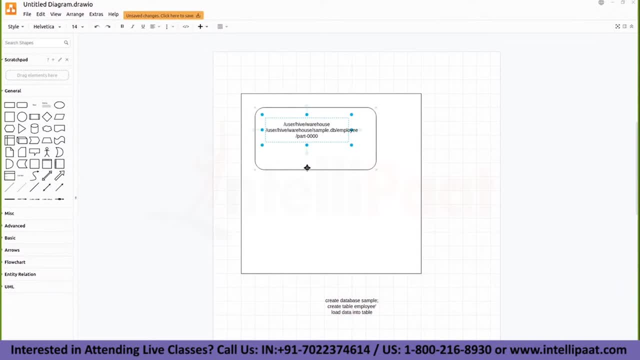 so inside the directories, whatever the data you load will be loaded as a text file or whatever the formats you want to specify: csv, text or whatever the format getting it. so this is how the structure will be. so now you create a new db. how it is going to be. 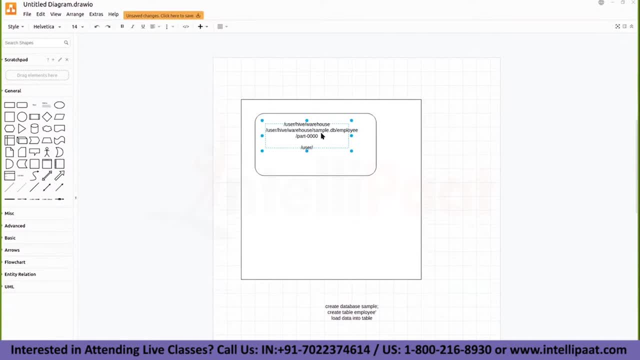 so under slash user, slash hive, slash warehouse you'll have um new db dot db. so there is a new db dot db which is getting created. so there is a new director getting created with that database name. so inside that all the tables you create will have, uh, individual directories again are. 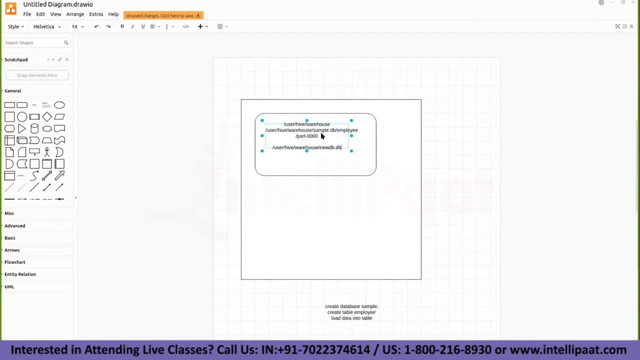 you getting it? yes, guys, clear. so whenever you load some data into this table, there will be a new file getting created. so now there is a new file, slash part hyphen zero, zero, zero one. and when you load another, when you do any other insert command, there will be a new file called part hyphen zero, zero, zero two. so let's say 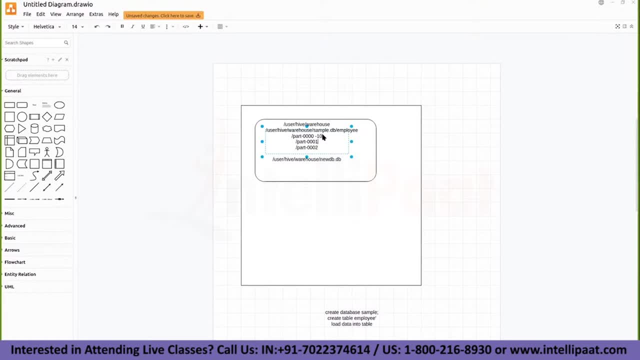 i have. i have some 10 records in it and i have some 10 records in it and i have some 10 records in it. okay, so this is all i'm doing: an insert from this table. so i'm doing an insert from this table, the command line, from the hive command line, doing an insert into table. table name: so and so records. 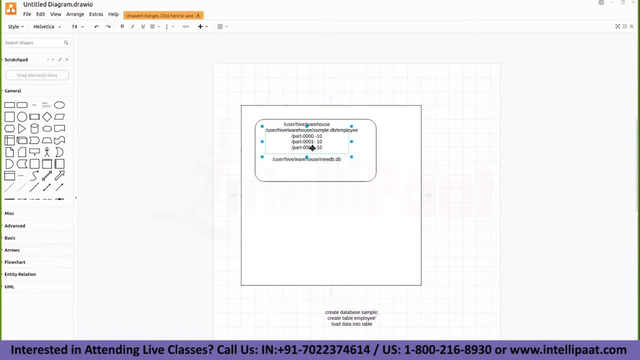 this is how it's going to get created. so now what i've done is in htfs. there is one more file. let's say there is hollow dot txt in htfs, somewhere in htfs. now what i've done: hollow dot txt. i copied it into using uh, hadoop fs cp. hollow dot txt. i moved it into whatever the location user hive. 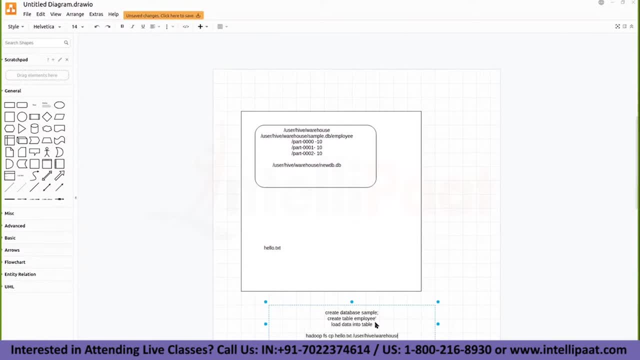 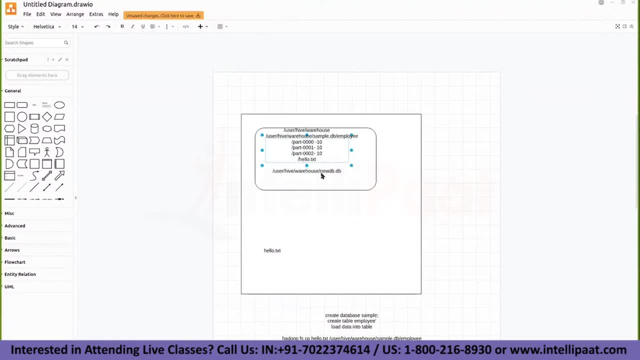 this is a normal copy command. it's a normal copy command. all these are insert commands and this is a normal copy command. this has how many? let's say, i have some 15 records. so now, on the hive shell, when i do select star from emp, i'll get. 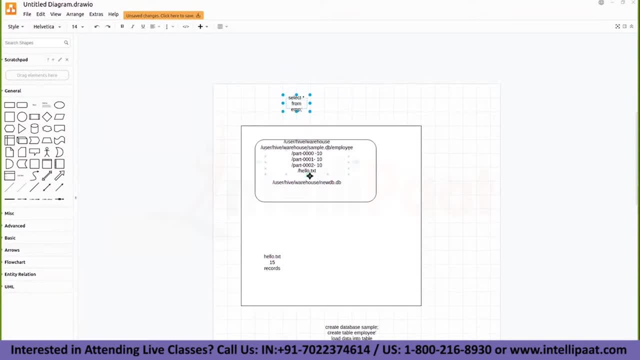 10, 10, 10, 30 plus 15- 45 records i'll be getting. that means you can either load the data into a table using a cp command, or you can load a file into a htfs location, or you can also do an insert. 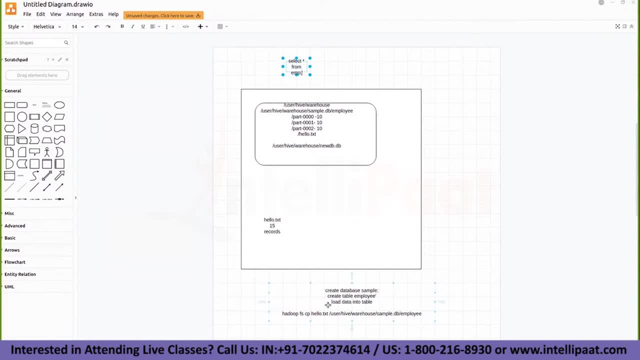 into a hive table. both ways you are ultimately storing some file in your employee employee directory. so whatever you have inside that employee directory will be displayed on your table. info: select star from emp will will show you those info, information, this data. getting the point now right. so the only reason, the only constraint should be: whatever the structure. 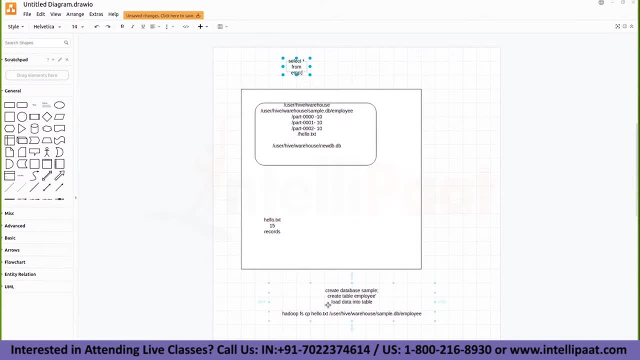 whatever the schema you gave for your hive table creation, the data in hellotxt also should be in the format of a same scheme. okay, so same format, whatever the tab separation, the three columns, three records, how the columns are separated, how the rows are separated. that schema you have to. 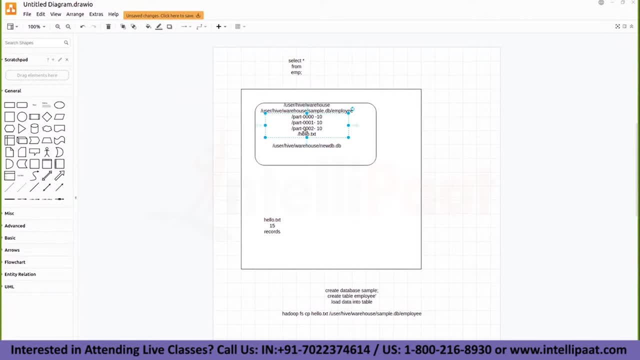 maintain in the hellotxt to be able to display that in the table. if the schema is not maintained, it will be formed as null. all the 15 records will be formed as null. okay, it will take 15 records, but it will show null values of it because it can't align the schema with the table schema. okay, so that's. 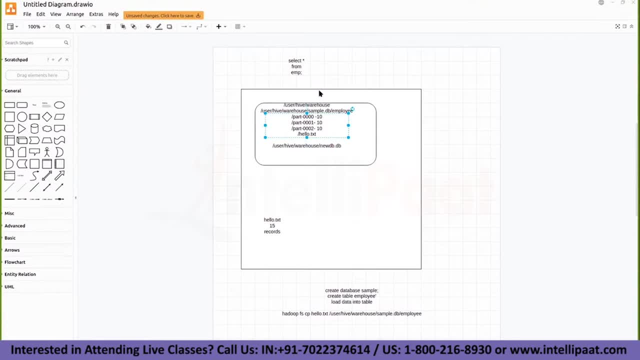 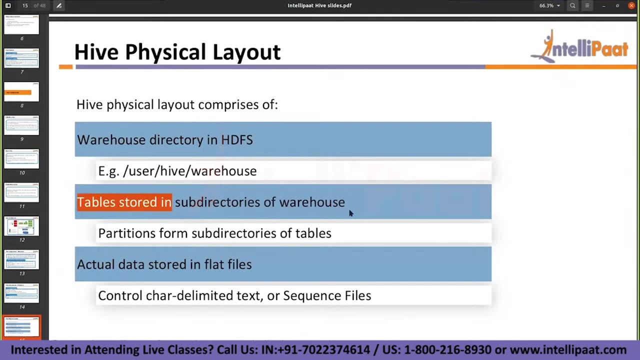 a difference here. now, we will do that. we will do some simple basic hands-on also if required. okay, so this is where we are. so user warehouse directory is, by default, user high warehouse only and the tables are stored as subdirectories of the warehouse. so inside the database you have. 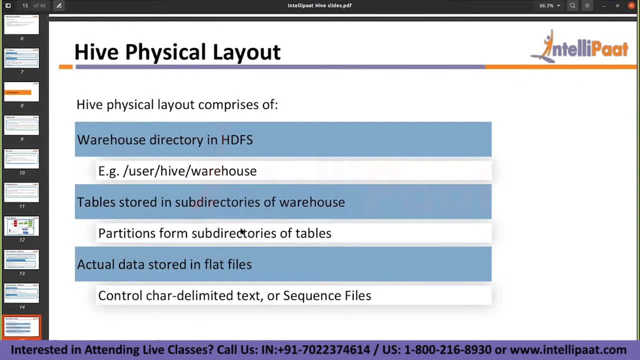 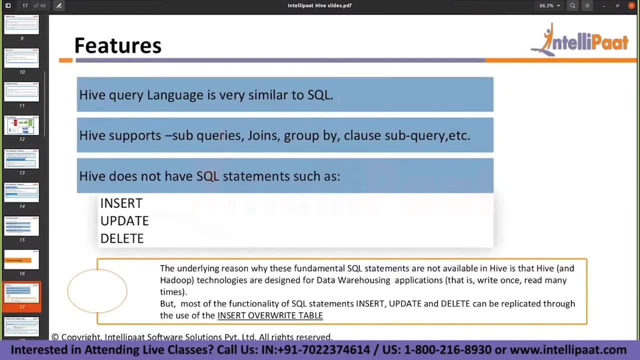 this sub directory with the table name and all the data is stored in the form of a flat file, so txt or whatever the extension. that way you'll be storing the data. okay. so now moving on to the hive query language. we know it's a very similar. sql. sub queries joins groups, does not have any. 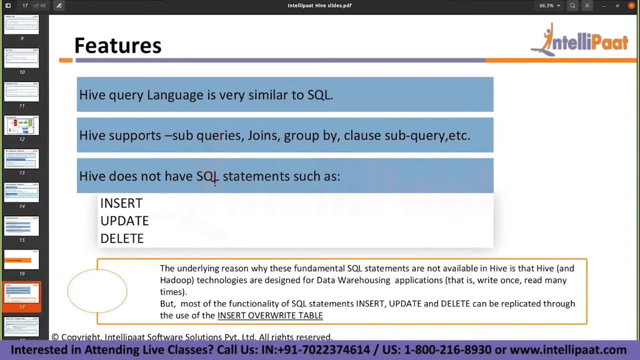 sql. okay, so here's a point. so hive does not have sql statements such as insert, update and delete. so what does this mean? so generally see, you can, you can do an insert command or you can do a delete command, or you can do an update command also. but theoretically, see what is hive used for generally. 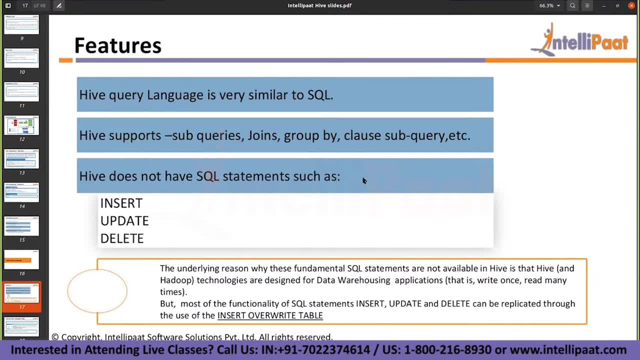 it is meant to use or if it is meant to deal with large amounts of data sets, right. so when, when you have this large amounts of data sets, you can do a delete command or you can do an update command. also data sets, do you? we are talking in terms of some millions of records, so do you actually have to? 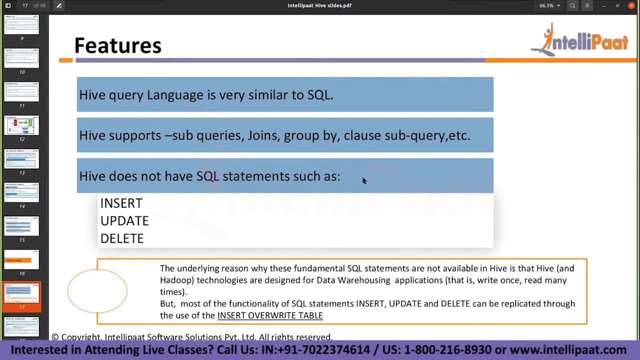 do an insert command on on one single record- see insert, update and delete. how many records are they going to change? if you do insert, it will only insert one record. if you do update, it will only update one record. if you do delete, it will only delete one record. so this record level updations. 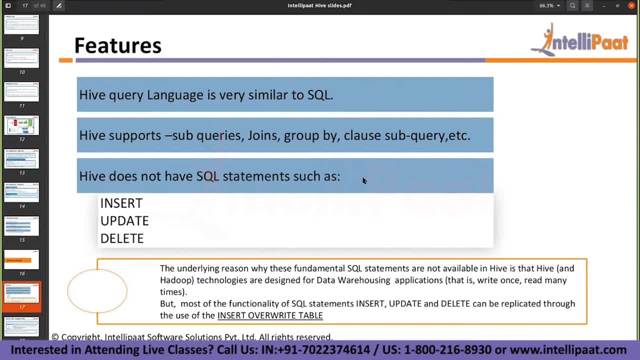 record level insertions or record level deletions are not preferred to to be done in hive terminal. okay, so when? when we talk about the underlying functionality of hdfs, we are only meant for writing it once and reading it many number of times. so, whatever you write you, you dump it once. after that you read: 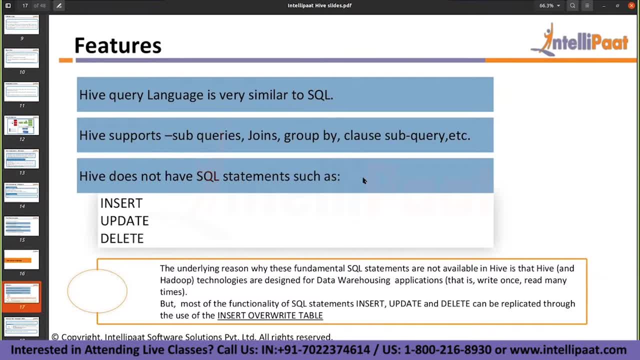 it any number of times. okay, so when you dump the data into hdfs, there is going to be some metadata that is going to get created and, using that metadata, you're going to read it any number of times. so for every single record you write, there has been a new metadata that is getting generated. 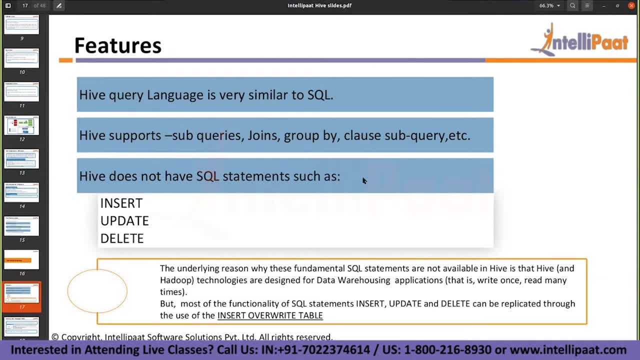 or there has been some actual data that has been generated and now you need to do something about that activity that is going behind in the HDFS right. So when you're doing an insert, that means you are writing some data into HDFS. 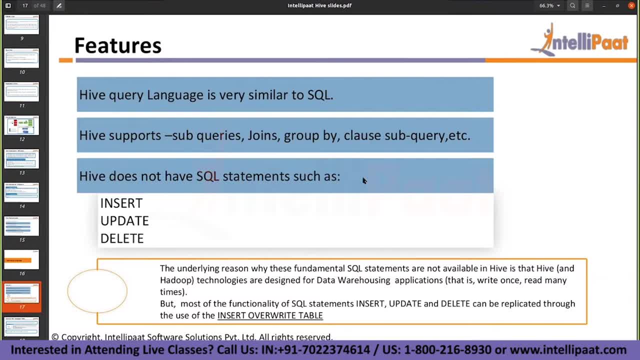 So in HDFS the concept is write once and read many, So which is not in line with insert, update and delete, So using insert. when you have some hundred lakh records in the table already and you use insert command and do one record, insert. 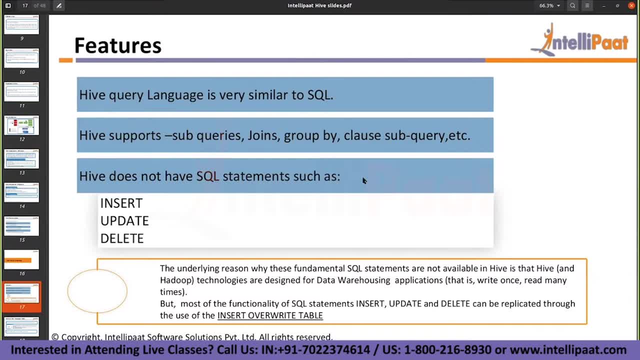 that's not a suitable scenario for your HDFS operations. So you can definitely do it, but update is not gonna possible. but insert and delete, I think you can definitely run it, but it's not preferred, it's not preferable to use them. 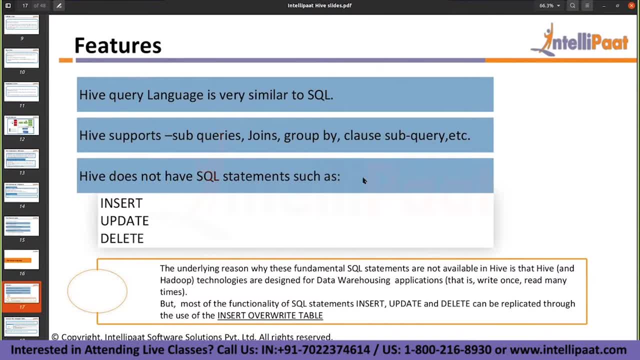 And generally you use insert override table using which you can do some data. you can extract some data from a different table and dump it into this insert table, okay. So it's not that it is not possible, it can be done, but it is not preferred to use, okay. 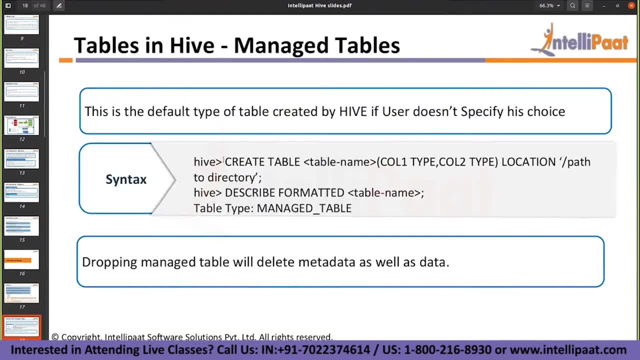 Then. so create table syntax. there is a create table command. create table. table name: the data, column one, column two and the location. So this is where the location will come. So location is in HDFS where you want it to store this data. okay, 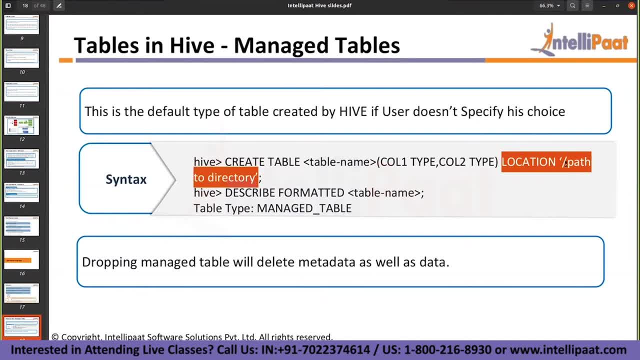 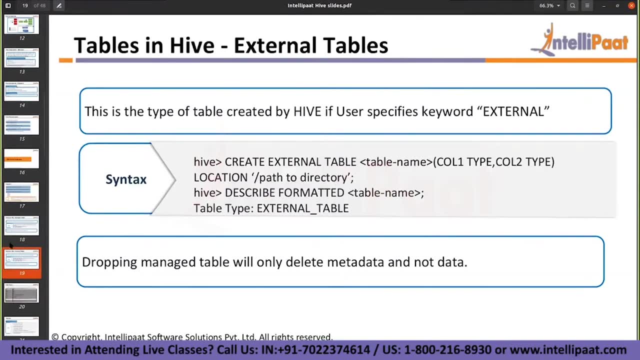 So I have to specify a location in HDFS so that it would create a directory with the table name and all the data. from here on, whatever the data you load into, it will get loaded into that particular directory only. okay, Then. so there is something called as an external table. 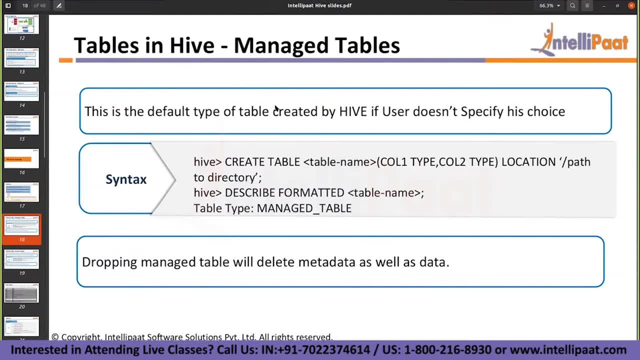 and internal table. the managed table is internal table And there is something called as an external table. So what is the difference here? So now going back to the diagram. So now we know this is all Hive warehouse, right? So whenever I say Hive warehouse, 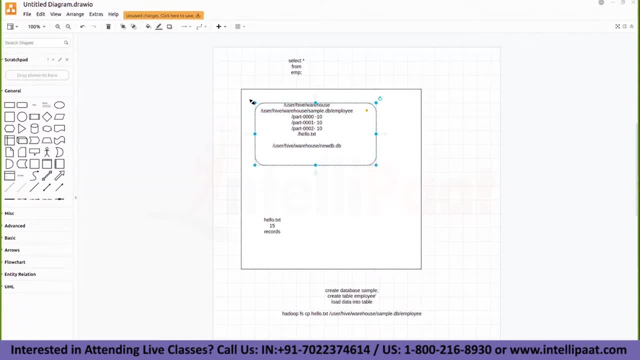 that particular location in HDFS is completely under the control of Hive framework. okay, So user Hive warehouse this particular folder, this particular directory and all the subdirectories in this particular location is all under the control of Hive warehouse, Hive framework. 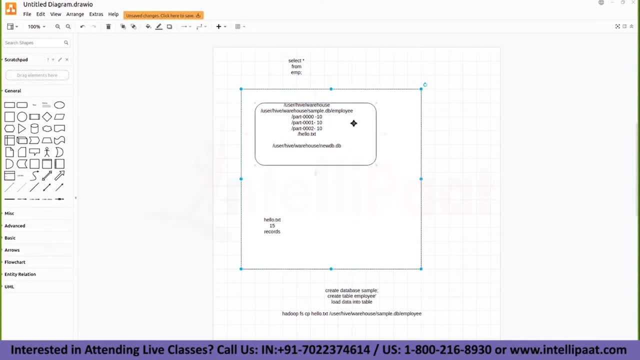 It's not that this is not HDFS, this is all within the HDFS only. but this particular portion has some control on Hive, has some control on this particular location. So now, when I say I create a table, I don't give any keyword: create table, table name. 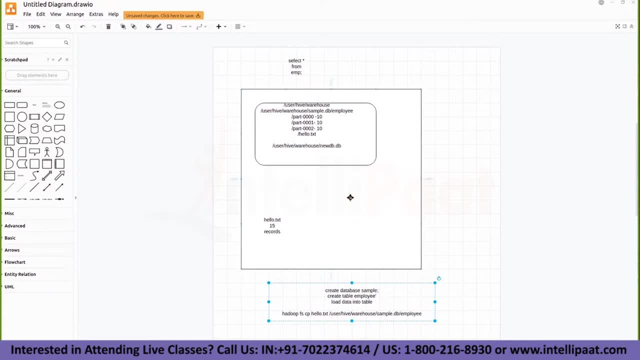 and I just give some location. So that will create and manage a table and the location will point to some location in the user Hive warehouse. So that means the data folder is getting created in the user Hive warehouse. only This data folder is getting created. 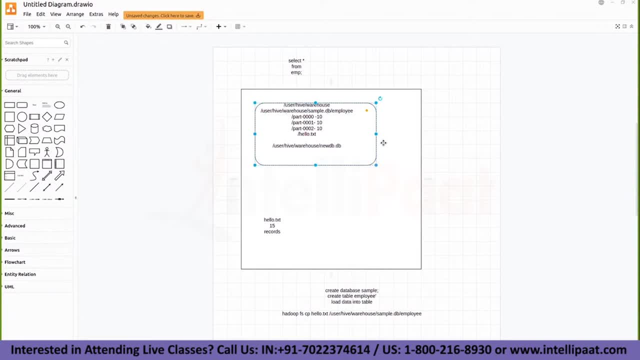 in the user Hive warehouse only. But if I give external it gets created anywhere in the HDFS. It can create here, it can create here, it can create some user home or whatever. whatever the location, anywhere it can get created. 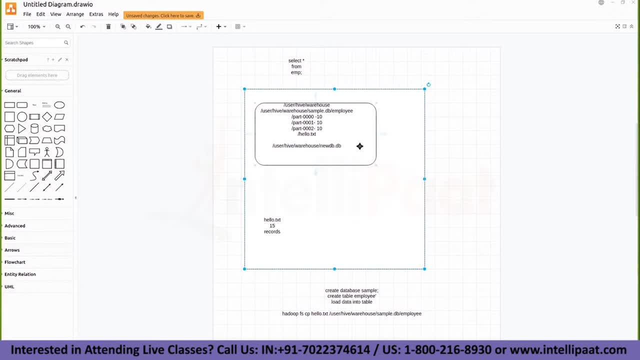 When I give create table, create external table table name. So where is it going to matter? How is it going to matter? If I create and manage a table, the data is in your user Hive warehouse And whenever you delete or when you drop a table, 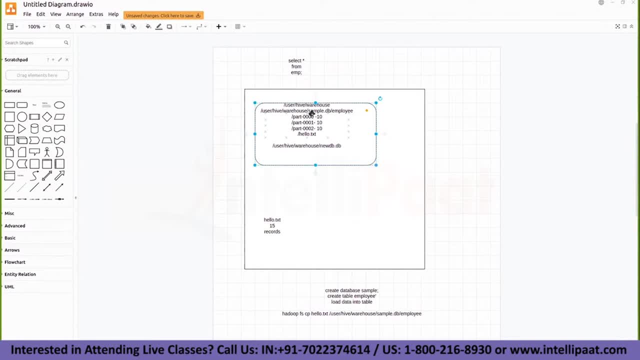 the table will get deleted and also the data will get deleted in the HDFS. But when the data is external table, when the table is an external table, it can be loaded anywhere in HDFS. When you drop a table, the table will get deleted. but the data will not get deleted. The data will still be there in HDFS location because it does. it does not have control to delete the data from HDFS If it is an external table. if it is external to Hive, it cannot control the data in HDFS, right. 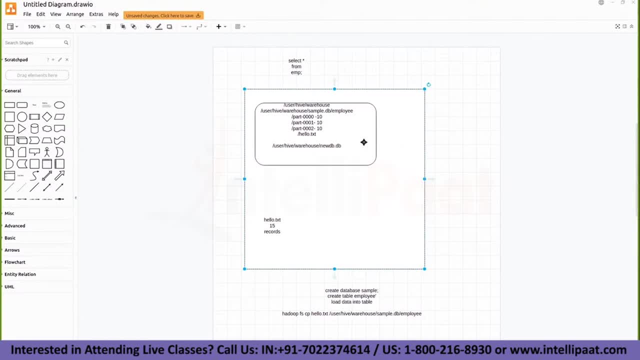 Hive. if it is internal, if it is within the Hive warehouse, then it can delete it. It has the control, It has the complete control If it is a managed table, if it has every control control to it getting it. 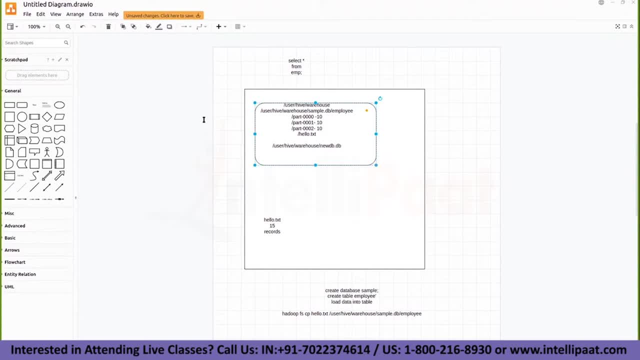 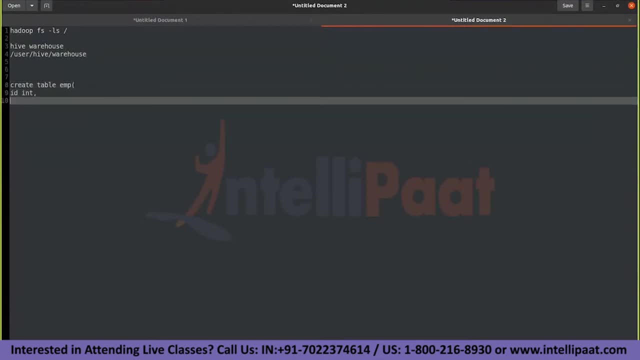 So my syntax will look something like this: So create table: EMP, IDN, name, string, salary, int location, user, Hive, warehouse and then EMP, some location in HDFS. This is my table creation table table, cache table. 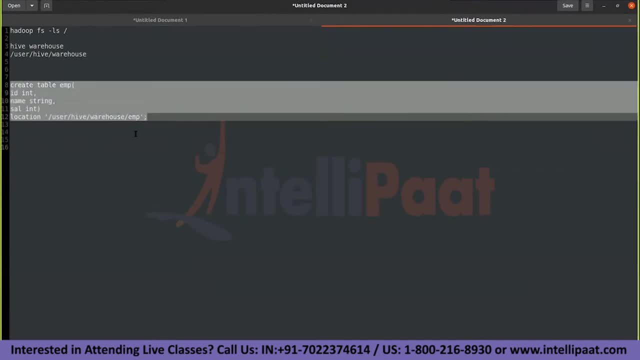 So I didn't give any keyword here. So same command, I'll be using it and I'll write external keyword. So this is the difference between if you give external keyword, you can give any location, user, Hadoop, some other location, okay. 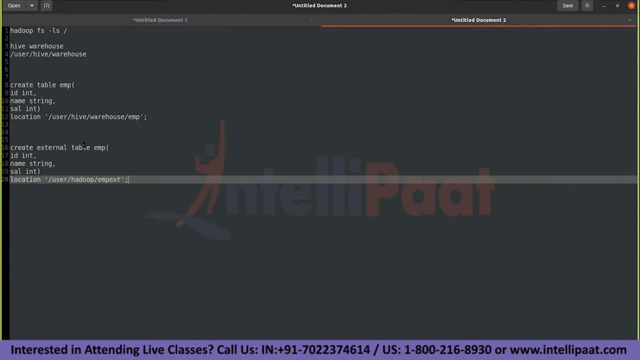 Some EMP EXT, some location I'll be giving it. So this table is getting created internally within this Hadoop framework and this table is getting created externally anywhere in the Hadoop framework. So now when I do a drop table, EMP. 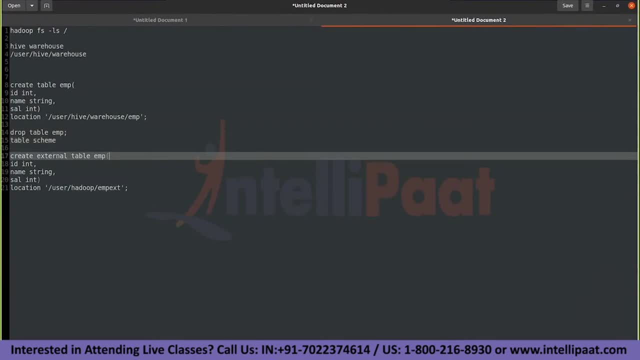 table, schema table and schema and data in HDFS gets deleted, But whereas here table and schema will get deleted, data in HDFS will not be deleted. okay, Understood. Manage table and external table: yes, 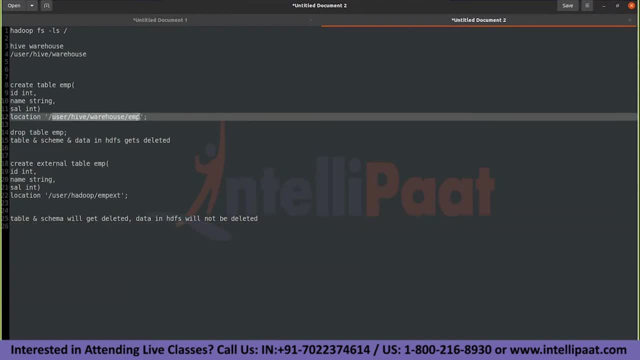 See, this is getting created in user Hive warehouse- EMP folder. This is getting created in user Hadoop, my EXT folder. So this is your user Hive warehouse is the core Hive warehouse location. Okay, internal table. I'm creating it here, okay. 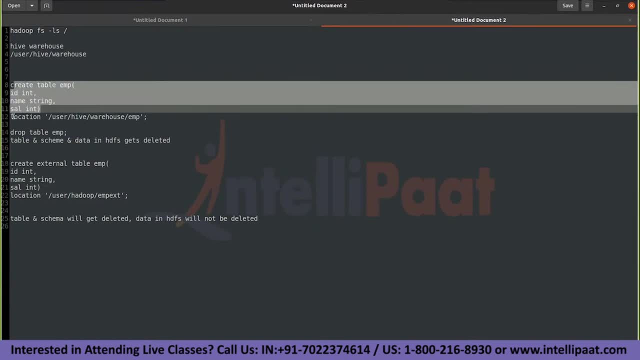 So now I created an internal table and I gave a location which is local to Hive, which is user Hive warehouse, So it has control of it and it is deleting EMP data also, And I created an external table. I don't have to give this user Hive warehouse. yes, 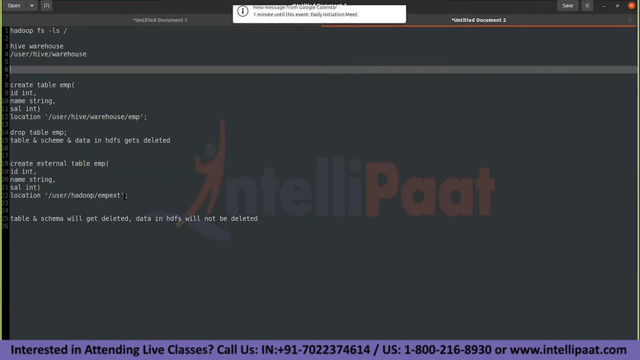 Now this external. I'm creating it externally and I'm giving a different location. So now I have a question for you. Okay, So what if I create an internal table? Just a quick info, guys, If you want to make a career in big data, 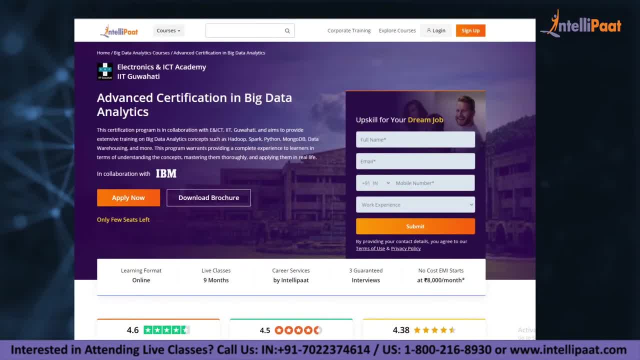 then Intellipaat provides an advanced certification in big data analytics by ENICT Council, IIT Guwahati. It is taught by IIT professors and industry experts With more than 10 years of experience. this course is designed to upskill and land your dream job. 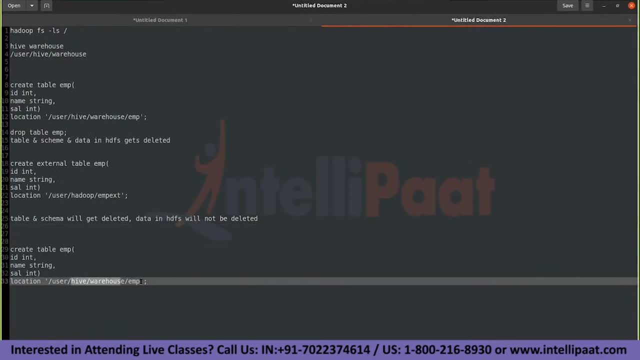 Now let's continue with the session. Some location outside the user Hive warehouse, Anything okay. Users Hadoop, some dummy location? This is not user Hive warehouse. If you see the difference, I'm giving the location external to Hadoop. 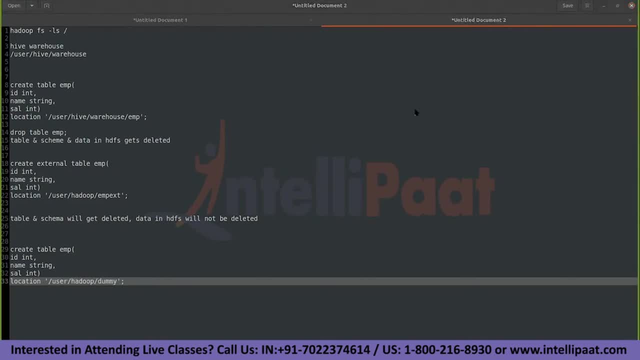 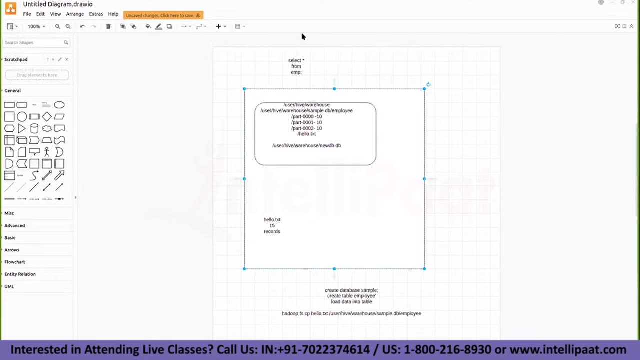 Means getting the scenario right. I'm creating somewhere here, I'm creating the location somewhere here, Outside user Hive warehouse And I'm creating internal table only. Okay. And there is one more scenario: I'm creating an external table. 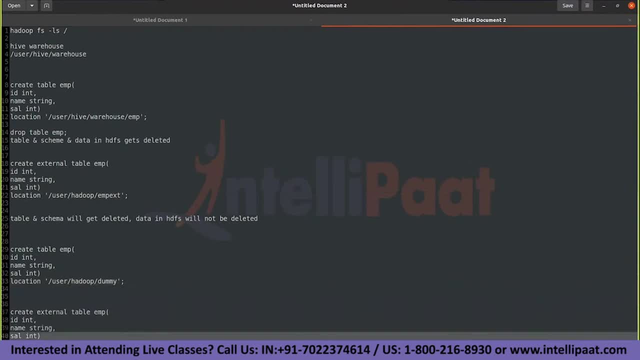 With the location user Hive warehouse. Opposite scenario. So now, if I drop this table- internal table, which is outside the external location to Hadoop, will the data get deleted? And if I create an external table with location inside the user Hive external? 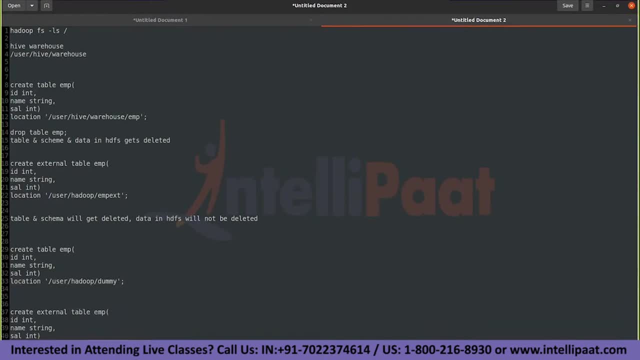 user Hive warehouse, will the data get deleted? So just find out these two scenarios and then we'll continue the discussion. So just think about it. What is going to happen? Think about this: internal table, External table, external location. 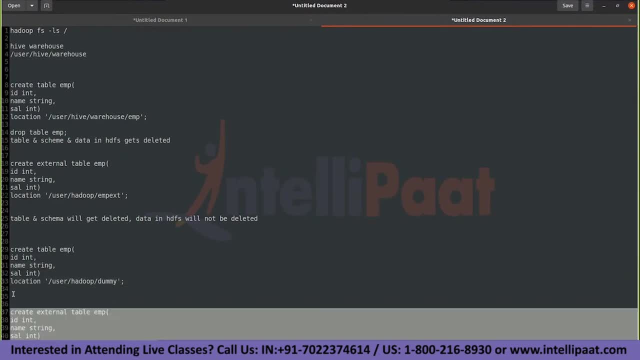 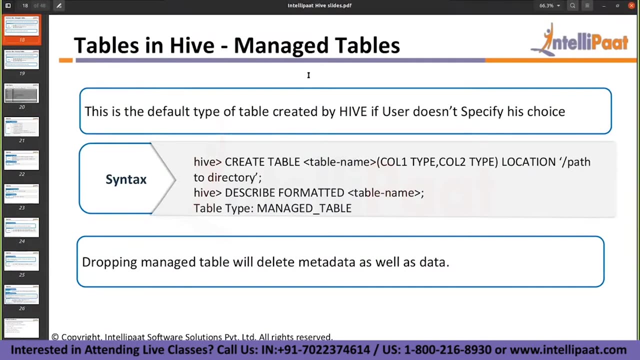 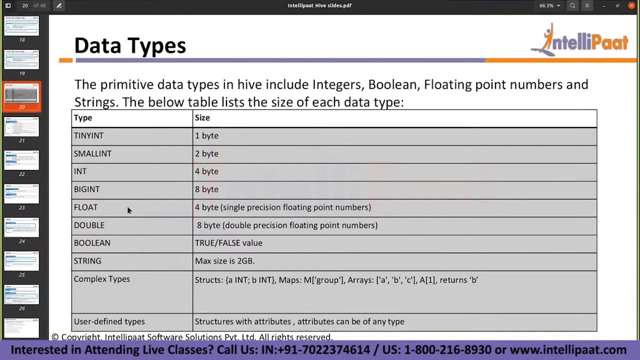 external table, internal location. Okay, Can you think of this too? So here, this is your manage table, This is your external table And these are the data types, So all the data types that will support strying and small and big in float. 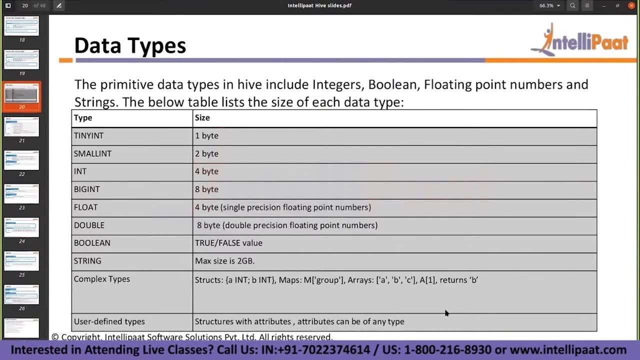 double boolean string, complex and user defined, whatever are the date types, Right. So all these things it will support and examples for creating a table: create table column name data type. create table column name data type. name data type. 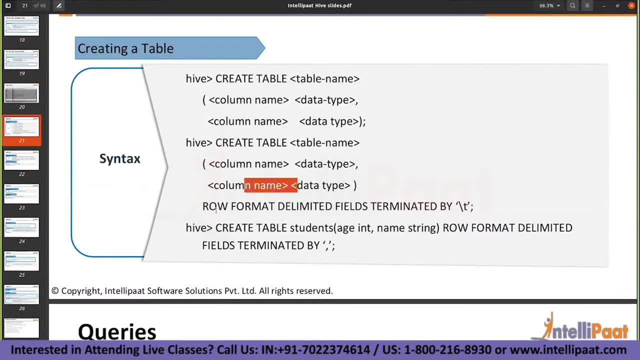 create table: column name, data type: name, first name, title and user. defined whatever data in� column named data type, and there is something called as a row format: delimited fields terminated by a backslash t. so what does this mean? so now, going back to rls, we will talk about it when we 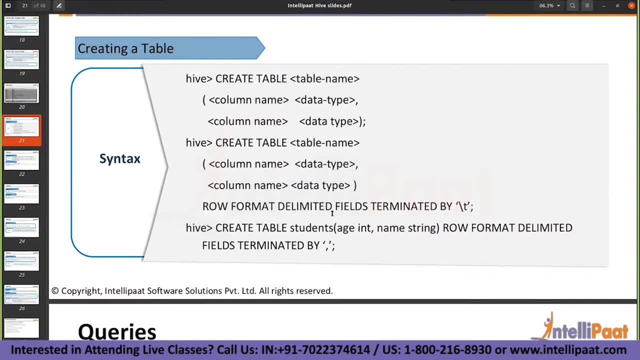 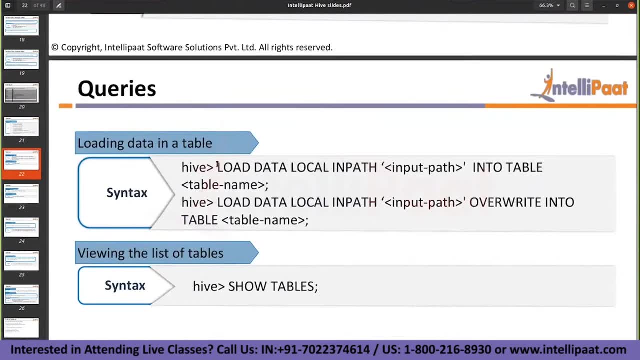 do hands-on, is that okay? fine, so i'm doing a create table and there is a load command, so load, what is this load? so, like i said, insert command, insert up the overwrite. so, generally, how do you write an insert statement so when you already have a table? 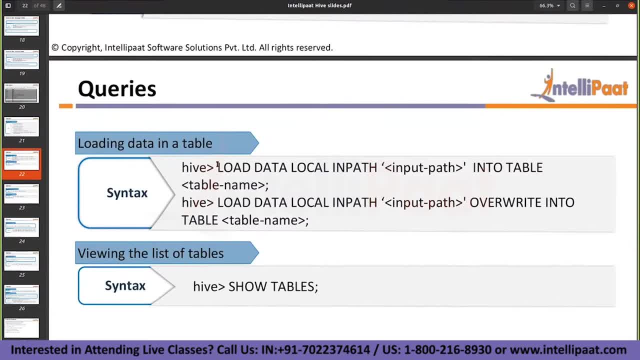 insert into so and so table select star from the other table. is it? is it possible? so you have table one which has some hundred records and you have table two which you created now, okay, so i'm writing: insert into table two, select star from table one. what is it gonna do? you dump all the 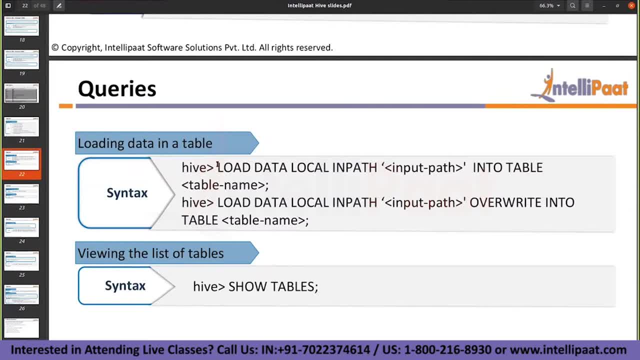 hundred records from table one to table two. that is one way of doing it. so i'm writing insert into table one and i'm writing insert into table two from table one. so that way is possible when, when you already have the data in the hive environment itself, when you already have the data in the hive, 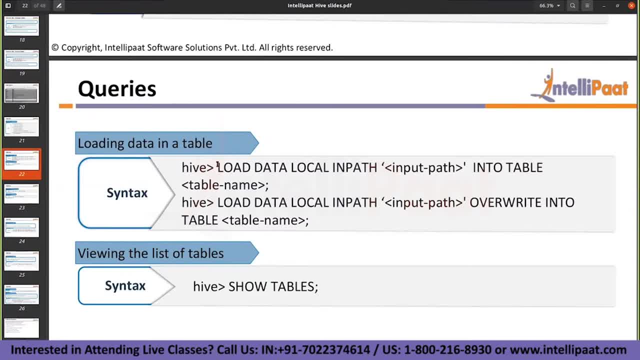 tables. you move the data from one table to the other table. but in general, a normal insert statement is something which you provide manually. you, you give the data manually, right. so insert into table values and so and so columns, so and so data. that's what you give right. that is not. 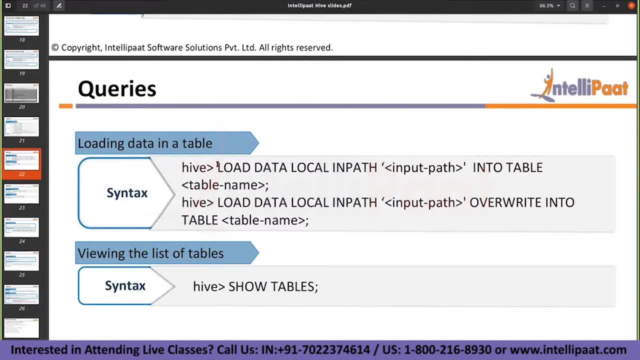 a possible scenario, because hive is meant to work with large amounts of data sets and doing the insert, update, delete on single data, uh is is not a preferred scenario, so for that there is a bulk load option. okay, so when you have the data available in in in a file or in a in a in, 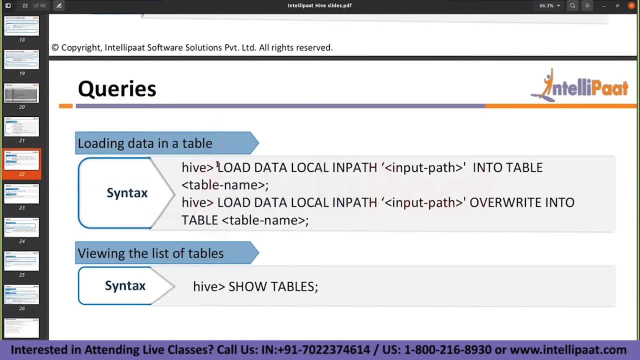 a proper, uh some, some flat file, uh, some hundreds of records. then you directly load the data into a hive table, uh, in a, in a bulk way, okay, so it's not one by one. so what is the command? load data local in path and then you load the data into a hive table, and then you load the data into a hive. 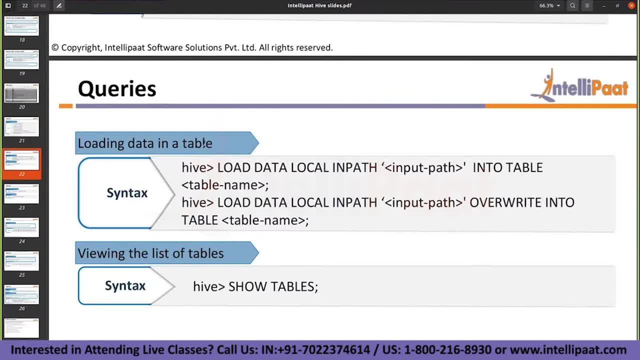 path into table table name. so what is the data? load data local in path, so in path, as in the data which, where the path, where the data is available. so let's say you have some file, uh, followtxt- which is available in so and so path. so load data local in path into table, the table name. 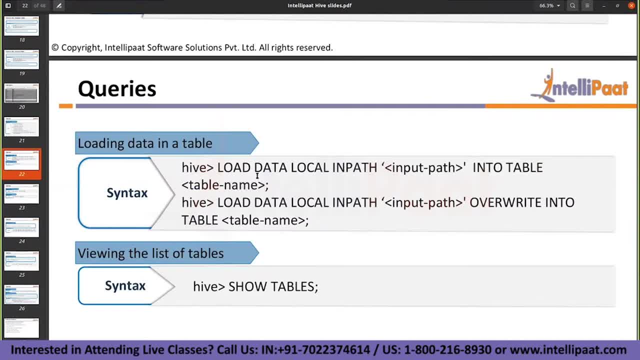 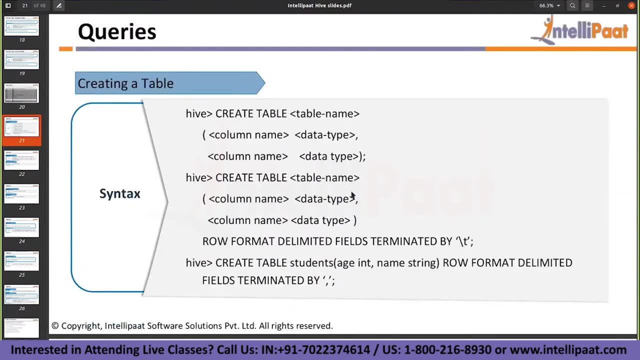 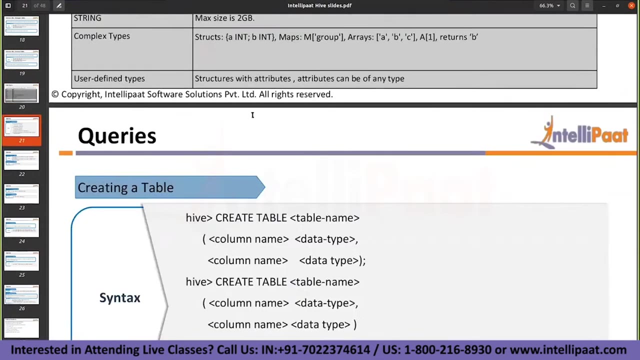 so what it actually does is it will just transfer the data from this location to your hive table location. getting it so, you created some location for your hive table right in the previous scenario. this location, so wherever the data is available in hellotxt, whichever path the data is available, you just move this data to your hive table. so load command is not an actual insert. 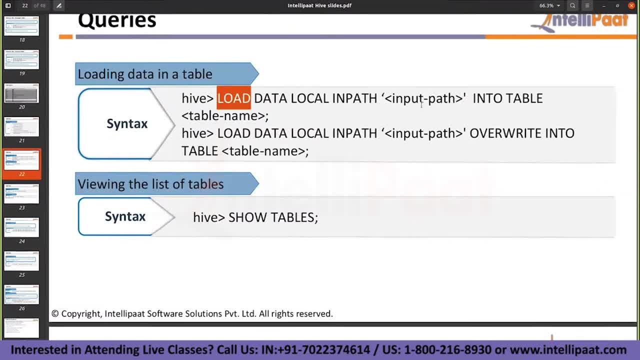 command, but it is a cp command which will load the data from an external location to your hadoop hive table location- clear, is it clear? and there is something called as a keyword- local. so what is this local keyword? so there, the actual command is load data in path. so there is a keyword called as local when the data input path is in your. 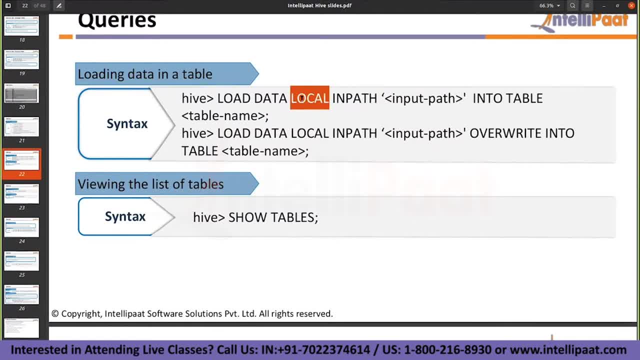 local file system, then you have to specify the local. otherwise, if it is within the HDFS only, you don't have to specify this local keyword. okay, so local keyword is only used when to when you have the data in your local file system getting it. so when the data is already available in HDFS, you just 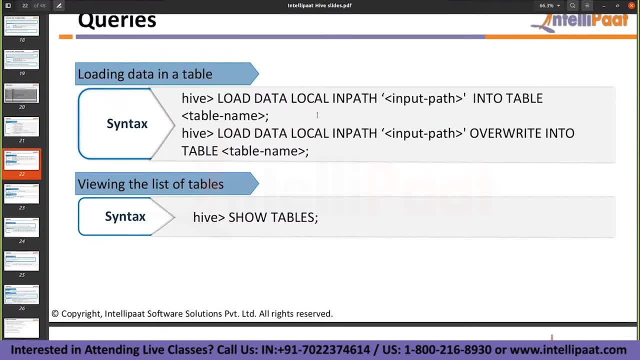 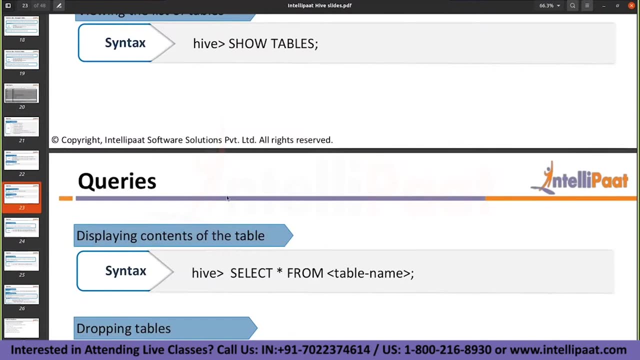 load data in path from this location to a table table name. that will move the data from from from the file location to the table location. that's it, okay, then. show table. show databases is all generic. there is nothing new in it, and select star from table name is also same. drop table table name is: 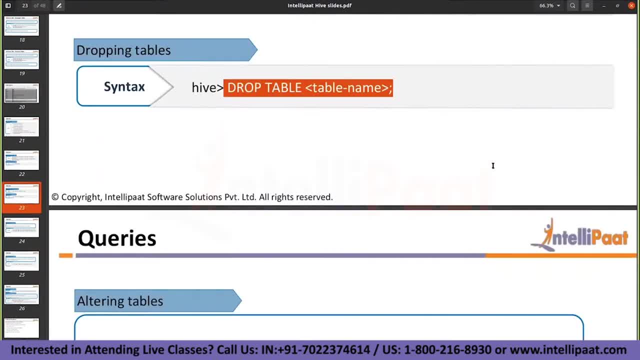 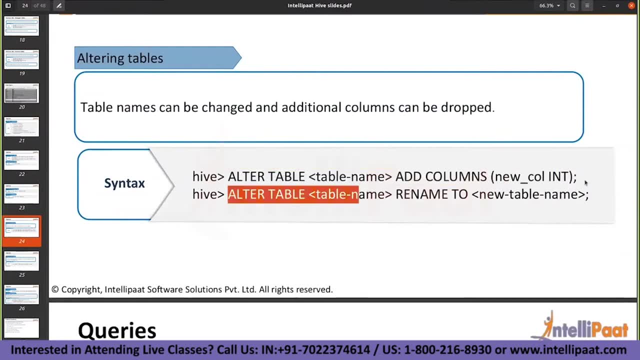 also same, and altering altering table is also same. you just have to do alter table table name, add columns, whatever the columns you want to give, alter table table name, the table rename command and in in addition to this, there are many other alter statements. the syntax is going to be the same. 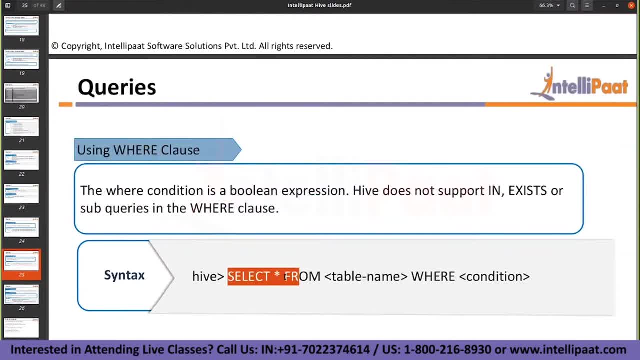 for everyone and using where condition is again the same, select star from table name. where. what about the condition? if id is greater than 100, name is so and so all that. where condition filters you can write- it's similar to a scale statement and group by condition is also same the column names. 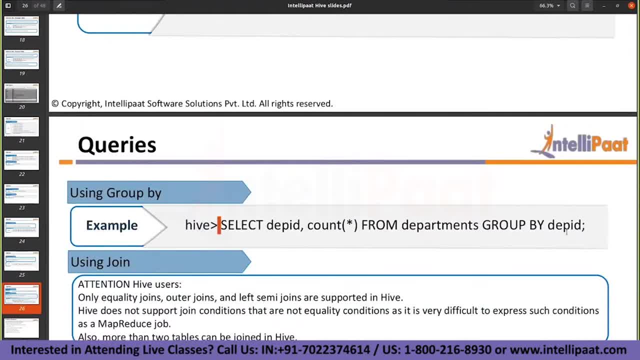 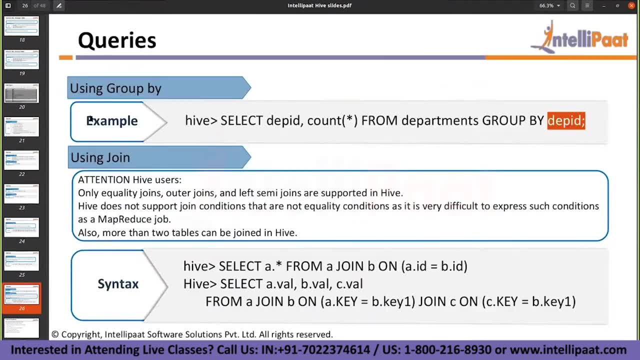 from departments: group by the column name. so it's going to group all the columns depending on the questions. all the columns are going to be the same. not going to change so right here, except once there are many your columns, that is the columns that is going to be there for you or your state. 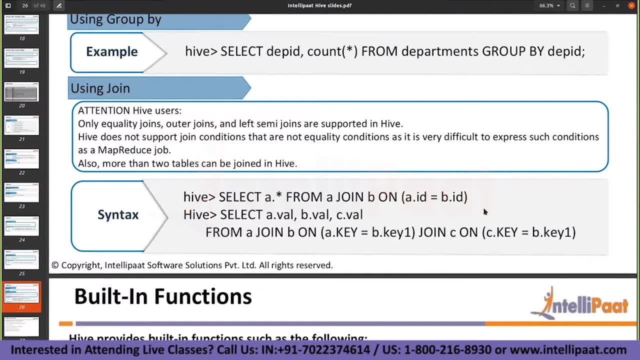 so you will have to edit it always. okay, so an, so a given right inside a cuestión. we will have to continue the field right, because Article Renee, we will have to take this one. so that is going to be one comma. column of cross. affix x to the column number to your table. okay, and here you can of course look 그렇게. 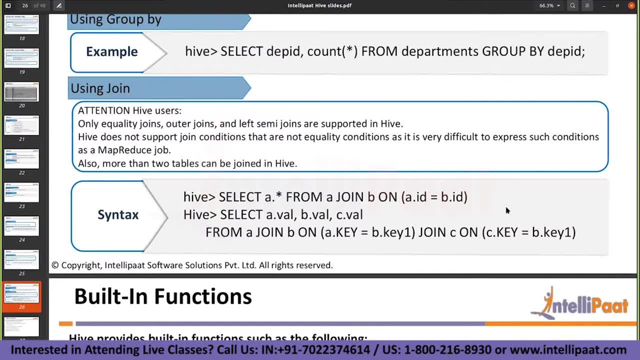 And right outer. join is all the columns from right outer and common matching columns from the left table. So we will execute them anyway. So it's again the routine scenario, whatever you know. So, built-in functions: there are some built-in functions available. 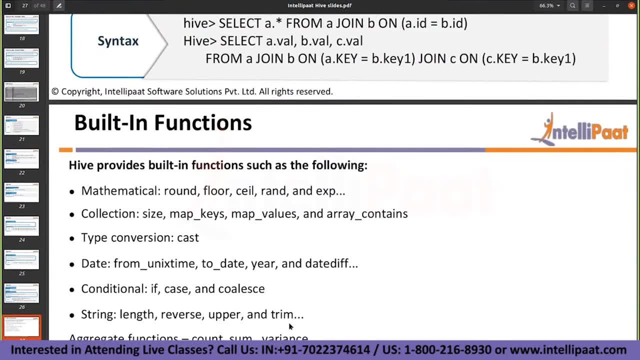 round floor seal random expression and these all upper lower count value sum variance if cast function unix, time to date year. all these functions you'll be using on top of the data on a specific column. 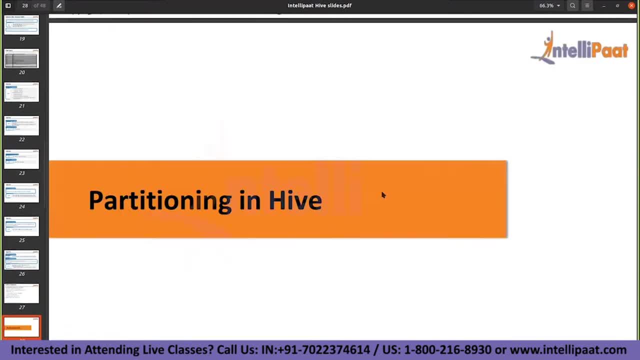 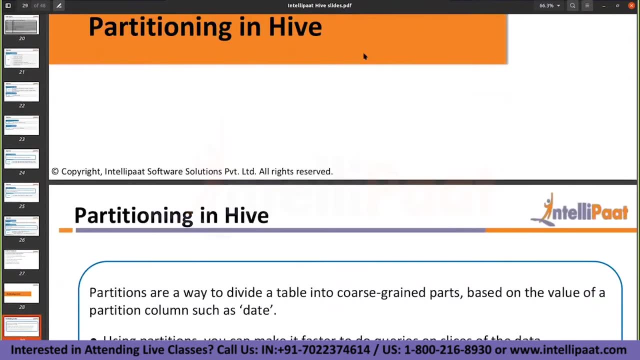 We will execute some of them when we do the hands-on, And there is also something called as partitioning in Hive. So have you heard about partitioning in normal SQL tables? Do you create these partitions So generally when you have see most of the times. 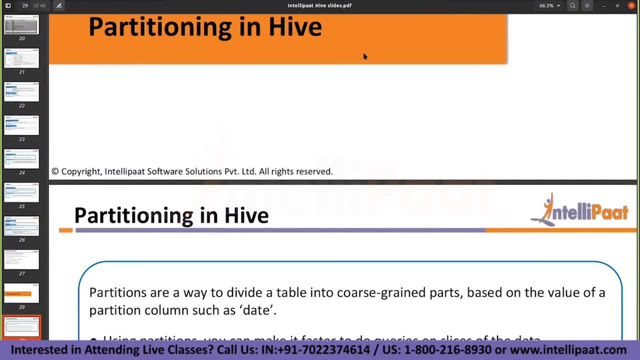 the partitions will be on. let's take one scenario, For example. I have some thousand records in a table. Okay, ID name and salary same. Okay, I have some thousand records in a table And I have written a where condition saying: 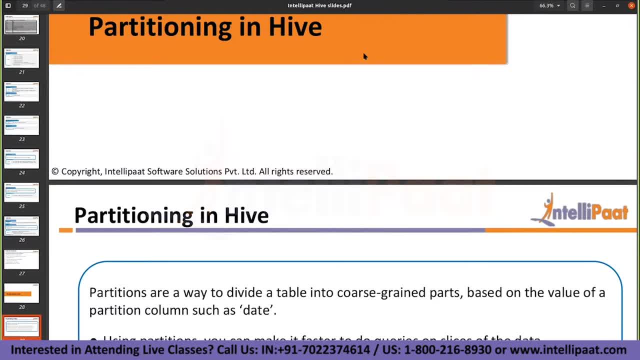 select star from EMP table where ID equals to some 960, whatever. Okay, Where ID equals to 960.. What is going to happen? So you start searching for the records from the beginning. So start: ID equals to one If it is equals to 960, no. 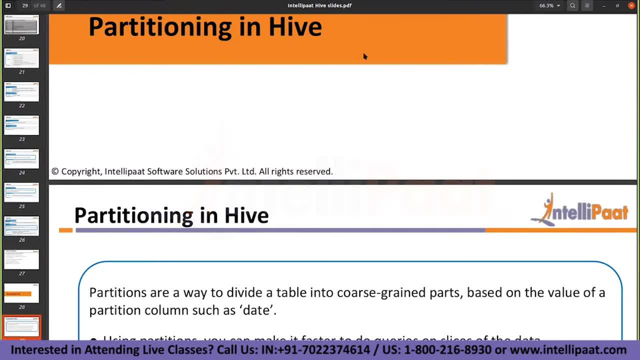 You start the next record, next record and you traverse through all those 960 records So find the proper matching ID column. But let's take another scenario. I have four columns now: ID, name, salary and gender. let's say: 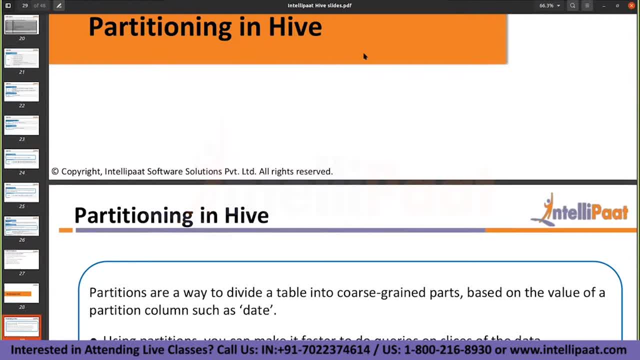 Okay, So out of thousand employees, 500 are male and 500 are female. Okay, So there's a gender column also available in the Hive table. So now I have written a filter condition. I've written a where condition saying: select star from EMP where ID equals to 960 and gender equals to female. 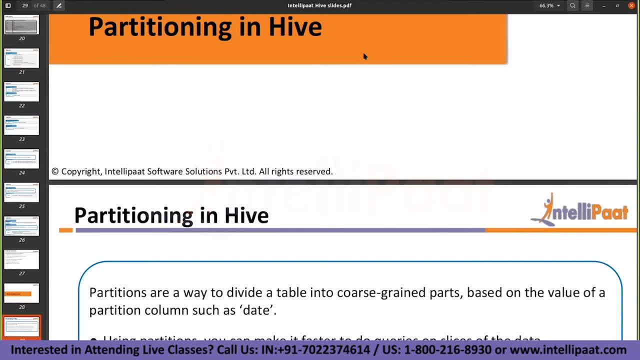 Let's say, okay, So whatever, the 960 column is a female candidate, female employee. So now, what is the scenario? Again, you have to search through all those thousand records, all those 960 records, and find the relevant value. So now, if I partition this table, so what is this partitioning going to do? 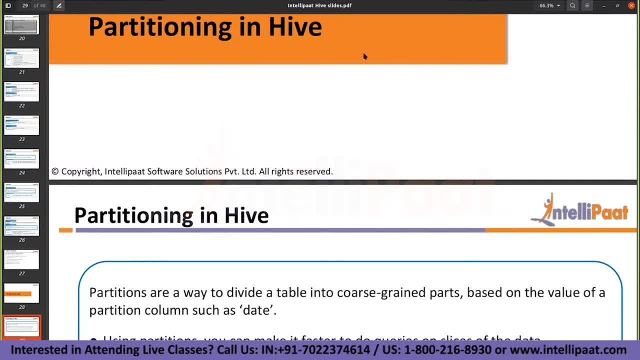 So partitioning is done on, you have to identify a proper column where the number of occurrences, the number of different occurrences of the column values are very less. So how many uh uh different values you can have, for gender, for ID, for example, you'll have all unique values, right? 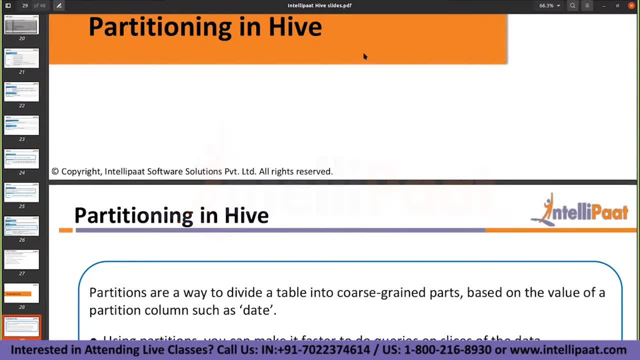 So ID is a primary key for me most of the times. So you'll have different unique values. You cannot have a partition on that name You cannot have. name can be different, salary You cannot have. there is no fixed bracket gender You can have, because there are only two possibilities: gender, male, gender female, right. 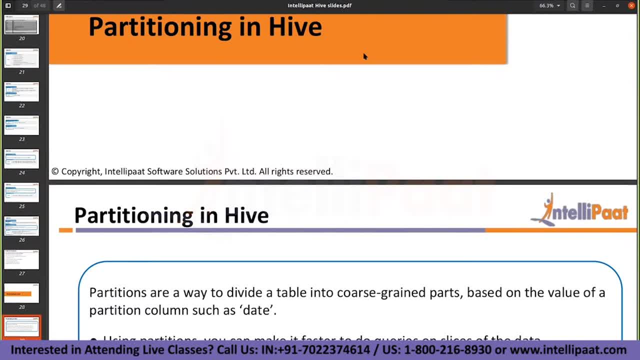 So now I create a partition on top of the gender column. So now in HDFS there are two folders getting created under table. under directory EMP There are two sub folders with partition gender equals to male, partition gender equals to female. 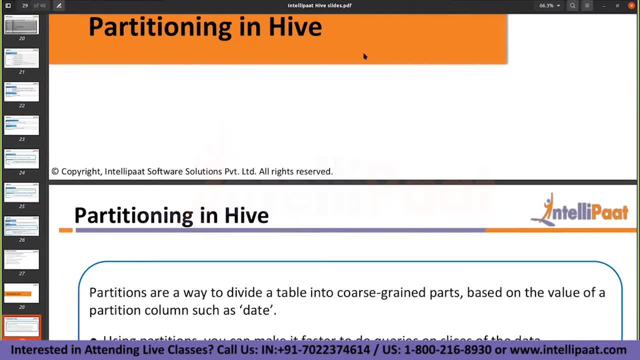 So all the records with the gender equals to male will will sit in the first directory. All the records with gender equals to female will sit in the second directory. Now, when I write the same query: select star from ID where ID equals to. select star from EMP where ID equals to 960 and gender equals to female. 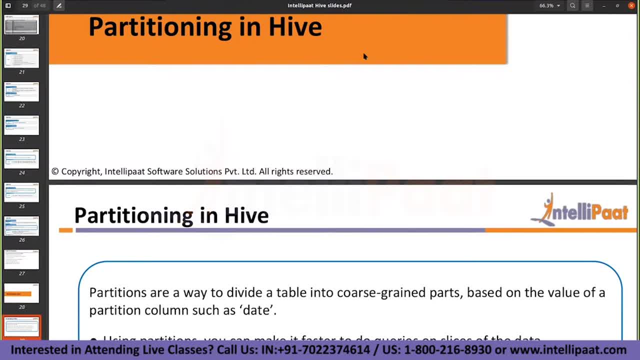 I'll traverse to the HDFS location, I'll get into the EMP directory And now I'll directly get into the gender equals to female directory. I'll not even Search for record gender equals to male. So you are almost removing half of the possibilities. 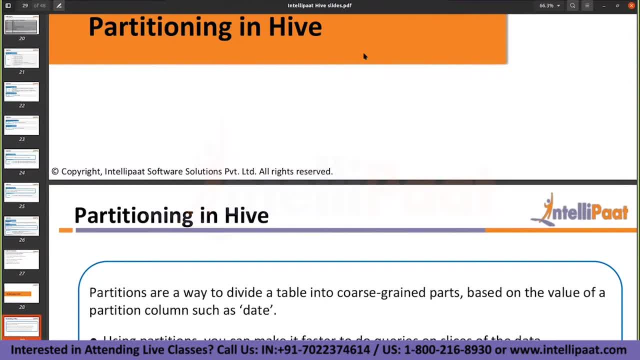 Agree, Understood. Oh you, you. you are trying to reduce the number of records that you're searching for in the filter condition, in the, in the, in the where condition, Right? So for that reasons you'll be doing the partitioning and not just for this uh, uh, when, when you have uh large amounts of data sets, like when you have, uh every day, you have some hundreds of records coming in. 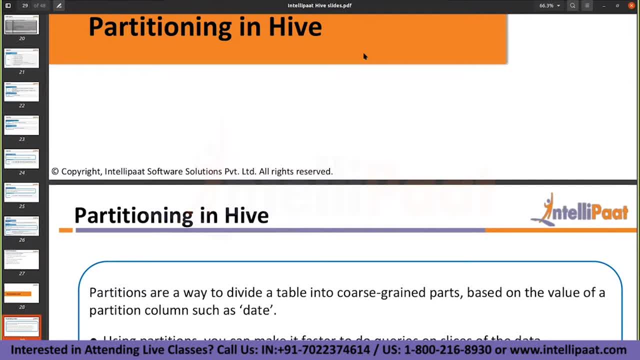 So how do you differentiate or how do you segregate the data from a status You've got to do? today's records is using the some some date column. Okay, So you'll be partitioning it, uh, via a date column. 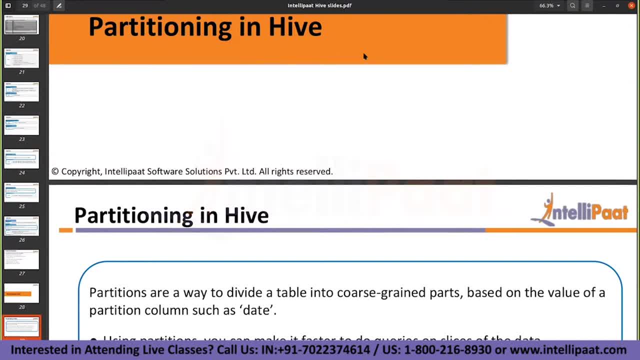 So whenever a new record comes in, a new partition file will get created for so that it will be easy for you to identify. Okay, These are the records which have been received today. These are the records which have been received yesterday. So most of the times, guys, in real-time scenarios you will. your partition column will be a date for them only. 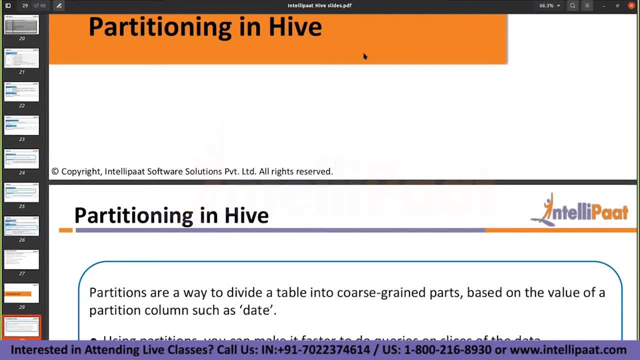 Okay So, but it may vary. but in real-time scenarios it will be mostly a date column. Okay So, segregating the data depending on- Okay, Different possibilities. So how do you select the partitioning? quality column is important. 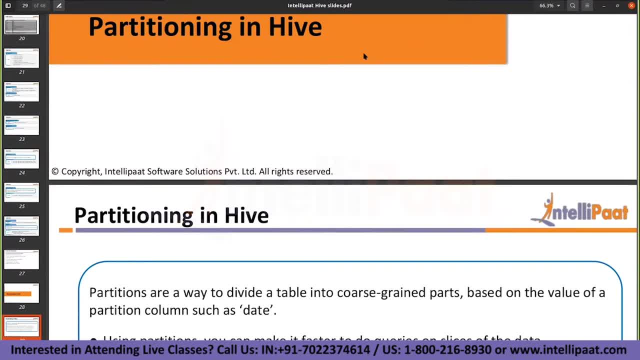 Uh, when you have ID name and salary and gender, you, your partition column will be gender, because the least number of possibilities the gender can have is only two. So, for example, let's say: uh, ID, ID name, salary, gender and city. 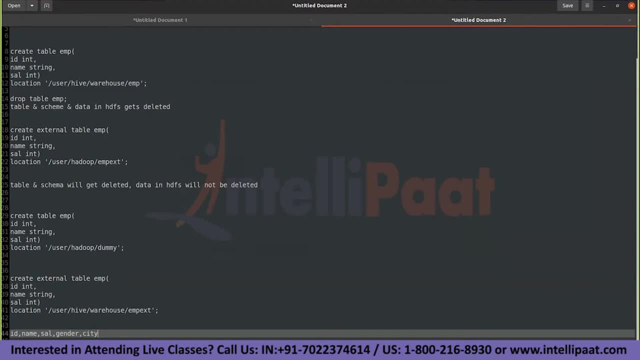 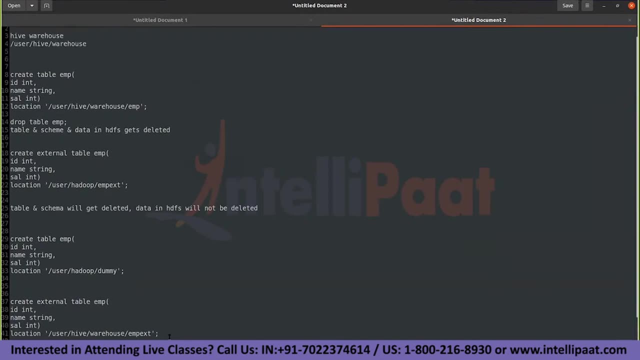 If I have five columns like this, what will be your partition column? Gender, again, And why not? city? So in that case, what you're supposed to do is you have to Find out the generic um, uh, uh, uh, distinct values for a city. 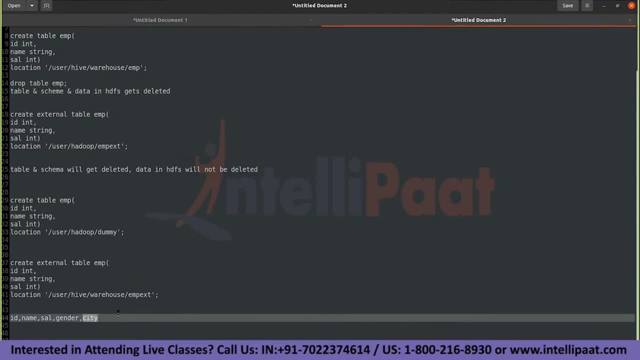 Okay, From the table you try to find out the distinct values for the city. If the distinct values are only three or four, that means your entire data set is only revolving around three or four cities. So, for example, your company has locations only in Vizag and Hyderabad. 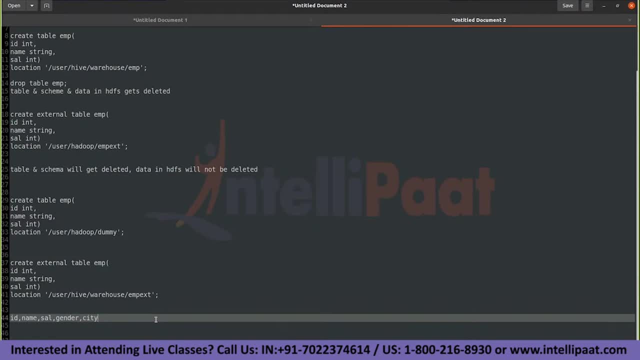 Let's assume we'll definitely have employees within only Vizag and Hyderabad. So in that case, what will be your partition column? Is it going to be gender or is it going to be city? You can choose both, but if I have to choose only one, 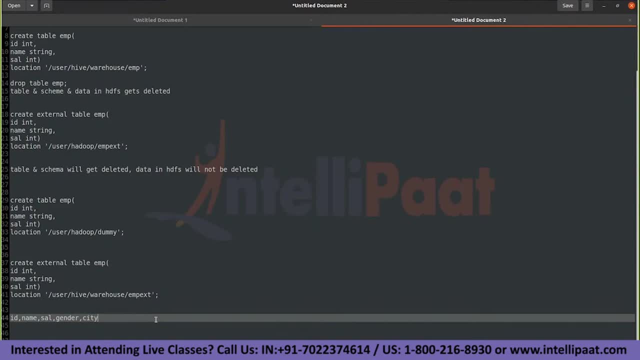 So it depends on what criteria as you are using for search again. So if, if most of the searches are on gender, if you're, most of your searches are on city, then, depending on that, you'll have to sell it, Okay. 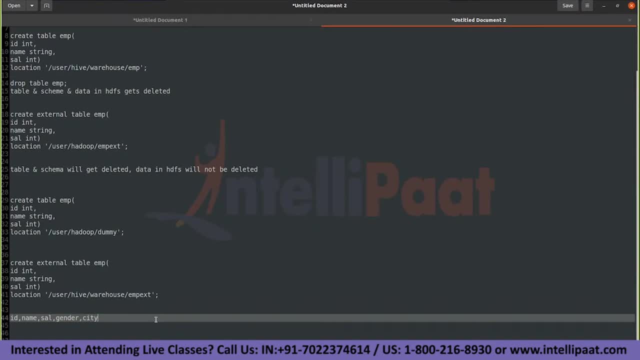 So if if I'm searching mostly on gender values, then it doesn't make any difference if I'm doing partition on city, Right. So again, if you are, if you are still confused, you can select both. So in that case, what is going to happen is partition by, by gender comma city. 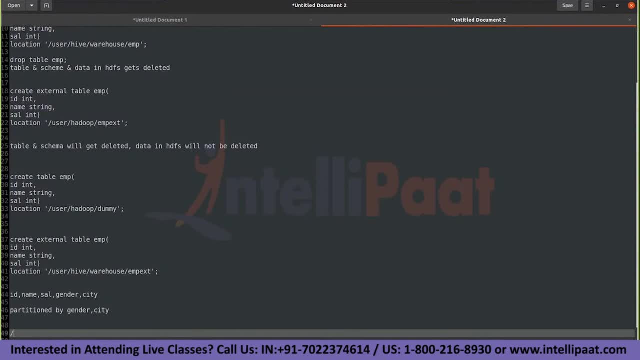 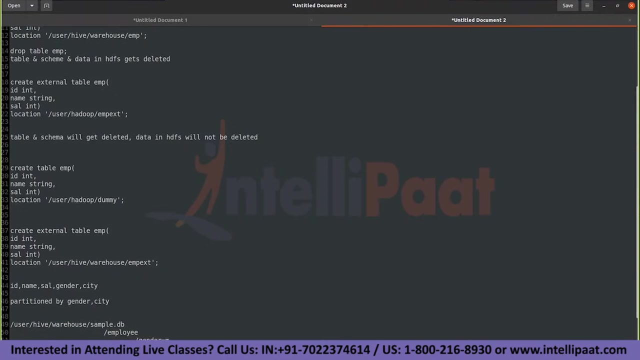 This is how you'll be selecting, So how is Your data will be looking like? user five warehouse, under which sample DB is my database, sample dot DB, under which you will have a table named employee, under which you will have a folder directory. gender equals to male and gender equals to female and under gender equals to male. 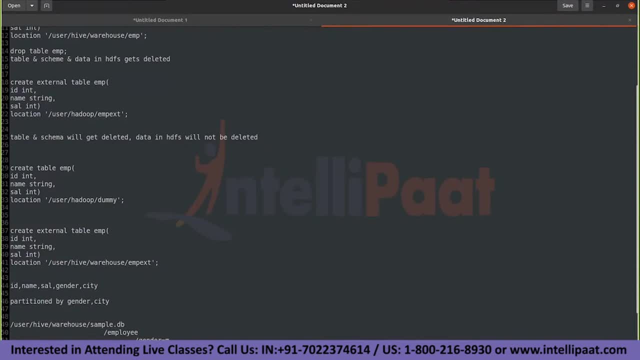 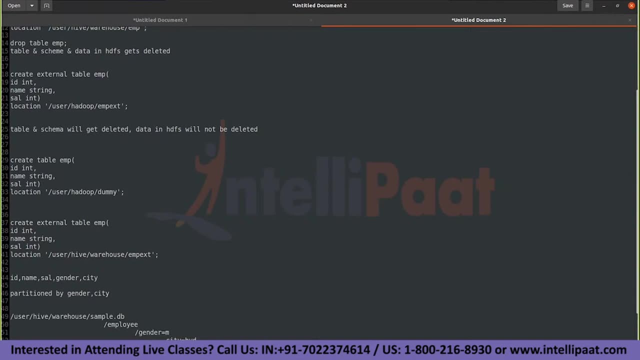 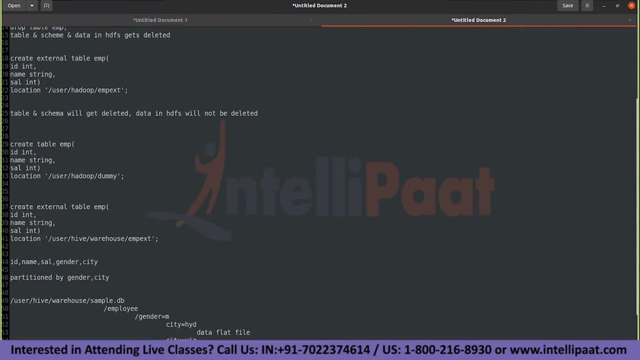 You'll have city. There is another folder: City equals to uh, Hyderabad, city equals to YZ. So inside this you will find data file, flat file. Okay, Here again that fellow TXT file. So this is how your directory structure will look like under gender equals to male. 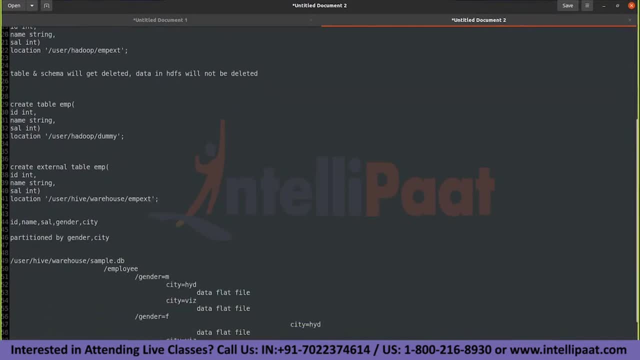 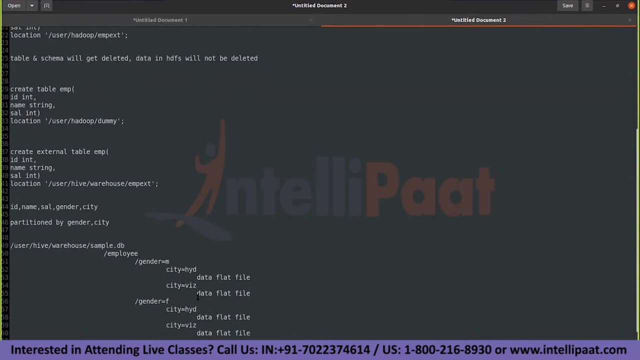 You will find two more folders and under gender equals to female Also, you'll find two more folders. Agreed, Got it. This is how your folder structure in HDFS will look Like. this is a folder directory. This is a directory. 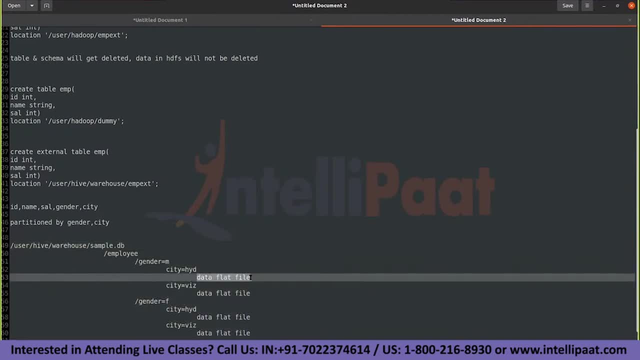 This is a directory. This is also a directory And this is where your file is available. So this file has only values with gender equals to mail and city equals to Hyderabad. This file has only values with gender equals to mail and city equals to YZ. 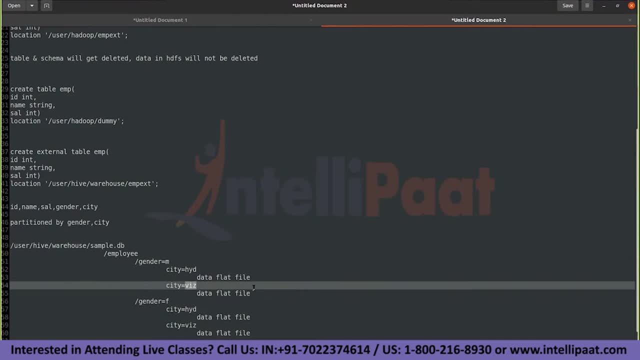 So if I'm searching for a specific record with gender equals to female and YZ, it will exclude all these values and it will come and search only in this directory. So almost 75% of results we are skipping getting it, So you can also. 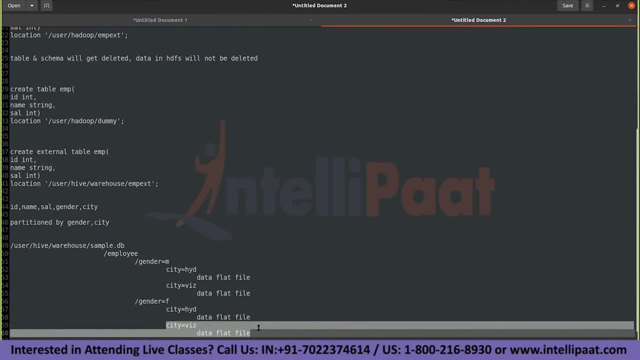 Have, like this, multiple levels of partitioning, but it is preferred to have um- at least I mean um uh- not more than two levels of partitioning, because it's going to complicate the uh uh structure. 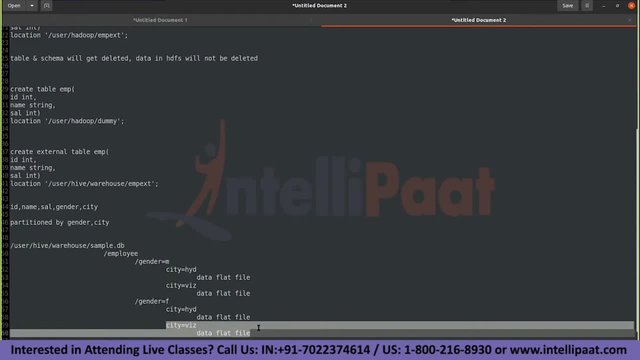 Okay, So it's going to complicate the entire uh flow of it. So not more than two partitions You can, it's it's preferred to create. So just try and maintain, try and make sure you have only two, two or at most, three levels of partitions and not more than that. 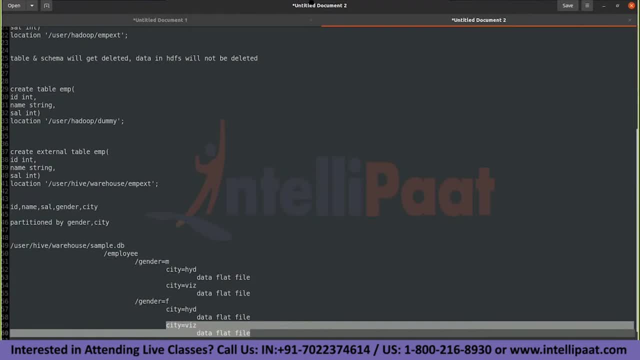 Got it. So this is what we do in partitioning, We will do this and uh like this. you have uh uh dynamic partitioning and custom partitioning. also in this, in Hype, We will see what is the difference. 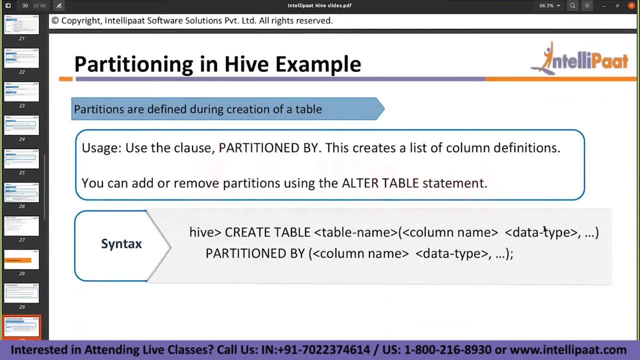 So how do you create a partition table? So create table: table name, column, data type: everything and partitioned by the column name, right, This is how you specify. So, okay, We will talk about this example. loading scenarios. 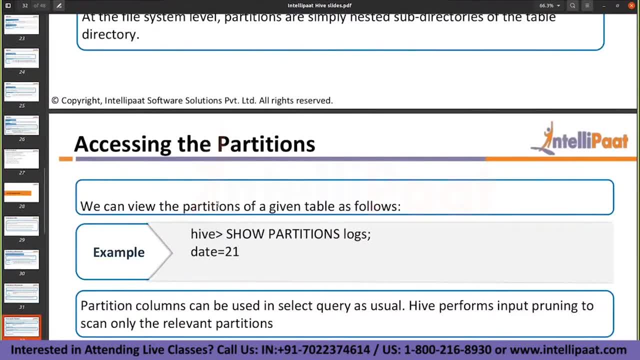 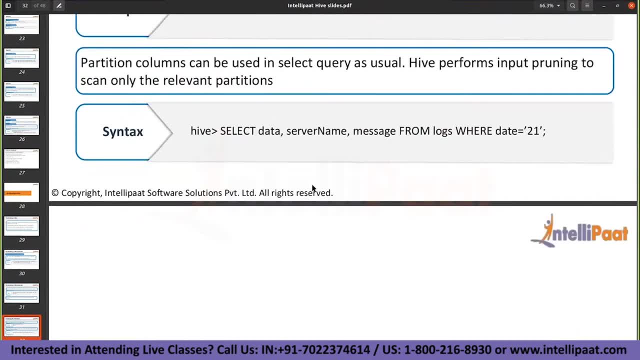 So if you want to Uh list out all the partitions that are available for your table, you can run a show partitions on the table name. It will tell you what are the list of partitions. it has got Okay And Hype queries has scripts. 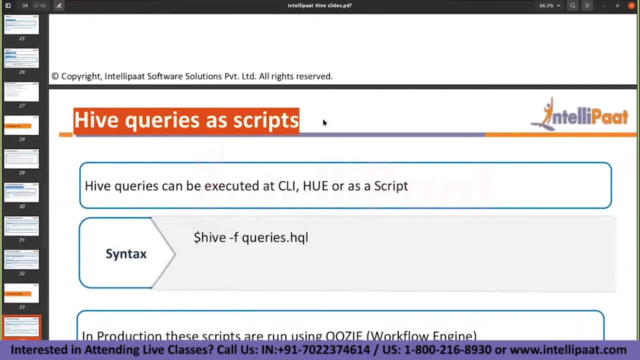 So if you if you want to write an SQL statement, if you want to write some series of SQL statements, you can put that in the form of a dot HQL file and you can run through the command line using Hype, hyphen F and the queries dot HQL. 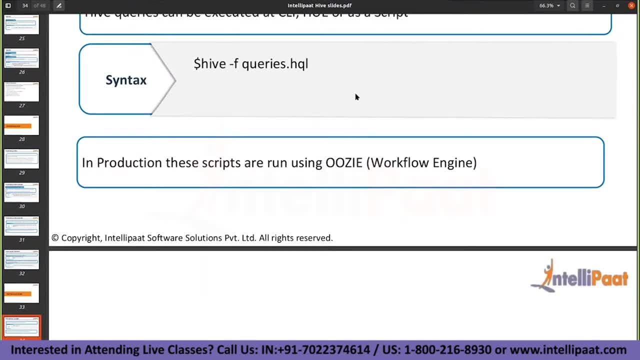 It will run all the scripts uh, one after the other. So this is mainly used when you are doing the scheduling jobs. Okay, So when you have to schedule some uh set of SQL HQL statements, then you can provide them and you can trigger them through an external uh window. 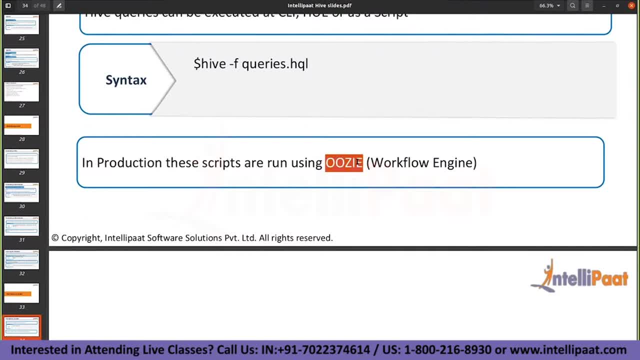 Okay, So there is something called as an Uzi, which is a workflow engine, which is mainly used for scheduling the jobs, uh, at regular intervals, For example if there is an insert operation happening or if there has to be some load operation. that is supposed to be scheduled at every one hour. 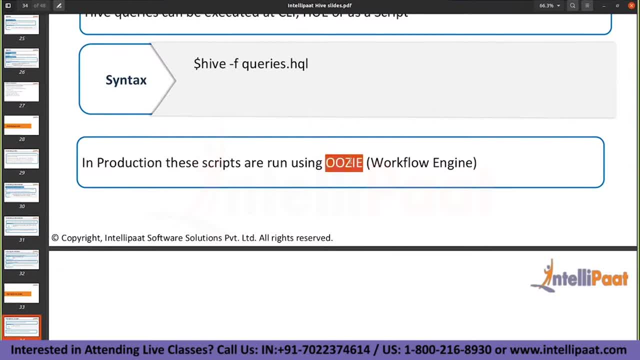 So that can be done using Uzi. So Uzi is also out of production, guys, This is not being used correctly. So most of the companies are using airflow, for They're scheduling now because it has got uh very much feasibility or very much uh a reach to almost all the technologies. 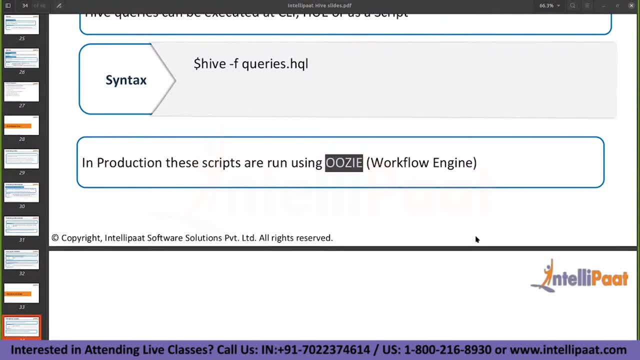 So Uzi is completely out of market. It's only relevant to, it's only restricted to, a Hadoop framework, right? So airflow has got a better reach, So it's something similar to airflow, right? So that is done. and data management using Hype. 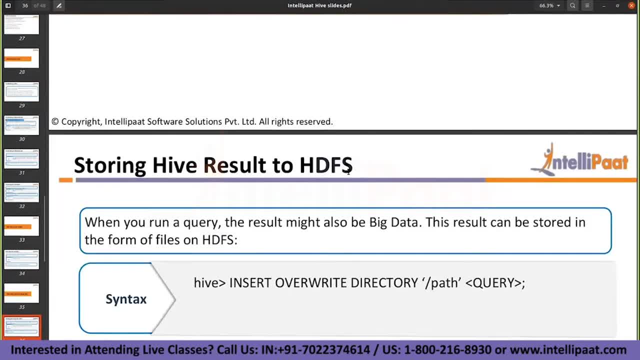 So how do we store the Hype result to a HDFS location? So insert, overwrite directory, whatever the path, uh, you wanted to specify. And what about the query? So, for example, if you are writing some complex query and whatever the data output you receive from that query, you wanted to store it in a file. 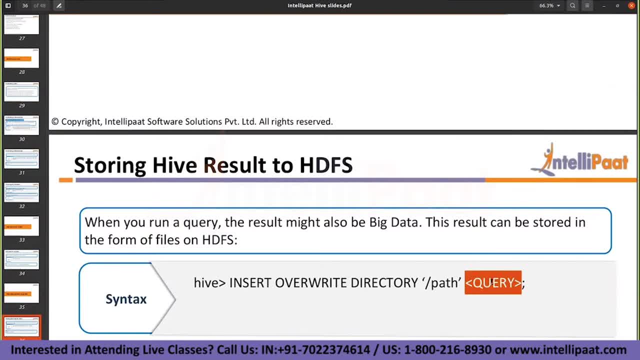 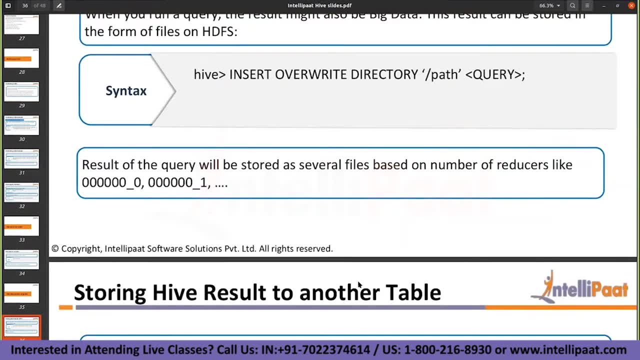 So this is how you are supposed to write this query will have. whatever the result you generate from this query will get loaded into this location in HDFS. Okay And uh, you want to create another table on top of this, similar to like we have done here. 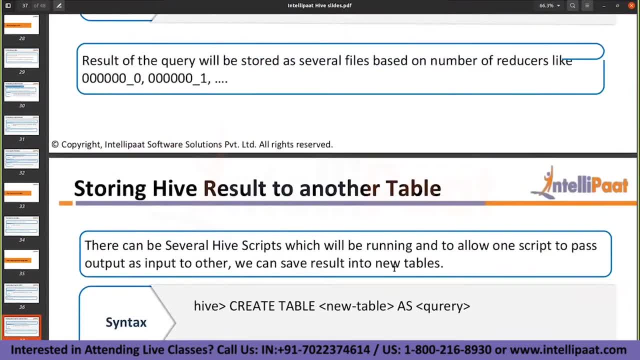 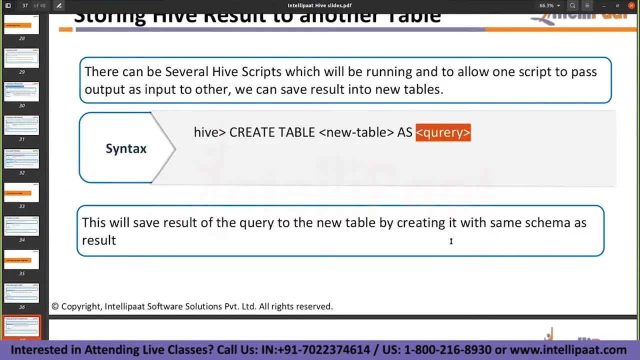 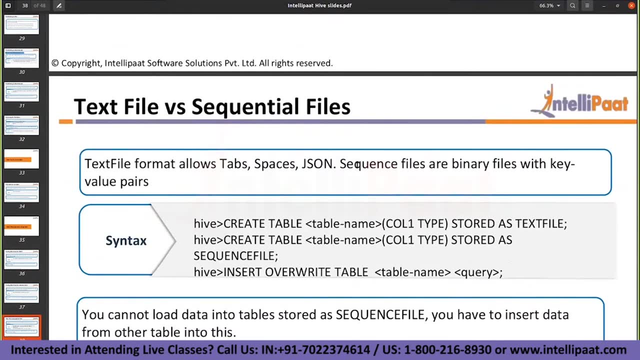 Uh, you can write create table, a new table as whatever the complex query you wanted to write. Okay, So all all of that, All generic SQL statements, There is nothing new here. and X file versus the sequence files. So generally, this text file format allows tab spaces and, Jason, sequence files are under binary files with key value pairs. 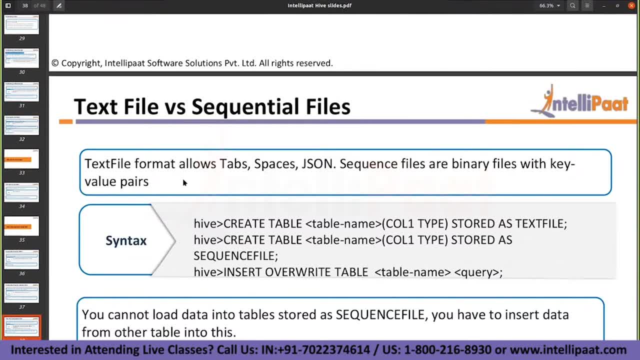 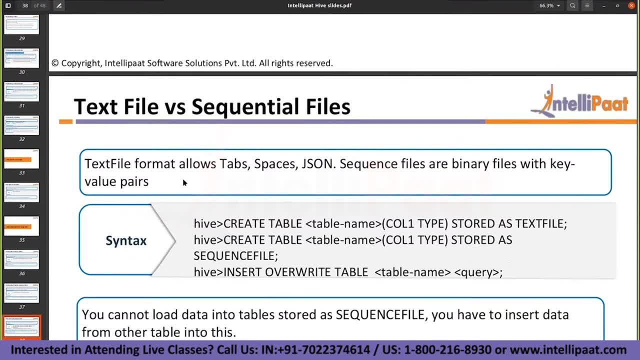 We have been using an ORC format, So the format is also something which we tend to use most, most, most often. Okay, So R, C, Avro, pocket. So these file formats provide proper uh compression and proper mechanism to store the data. 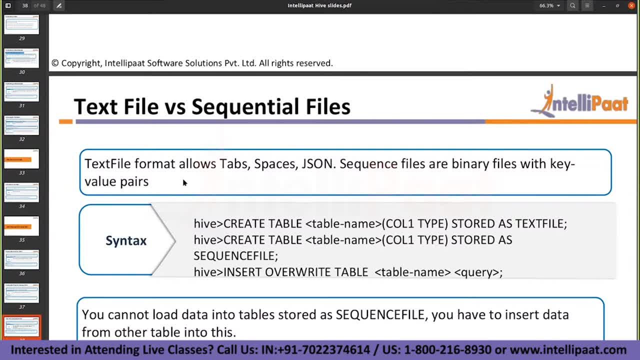 Uh, some of them store it in binary format and there are different, different advantages and disadvantages for each and every format. So but, for example, if a file is off some hundred GB, so using ORC, you compress it to some 60 GB using. uh, uh, I've. 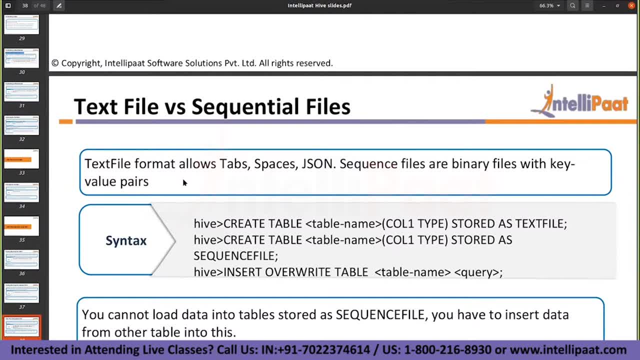 So, instead of using the hundred GB of storage, uh, by storing it in a plain text format, you you compress it and store it into different, different formats. Okay, So there is. there is another separate concept altogether for different file formats. 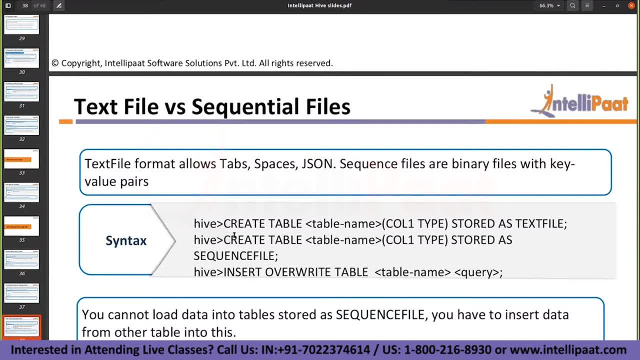 So you can specify. So how do you specify in the table creation statement? So create table table name, data types and stored as sequence file. stored as ORC file. stored as Avro file. stored as RC file. All these are Different file formats when you can use while creating the table. 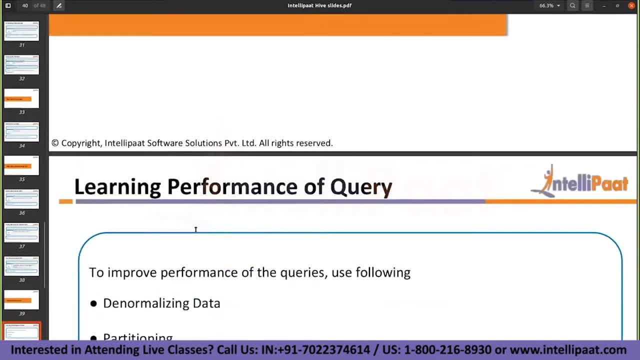 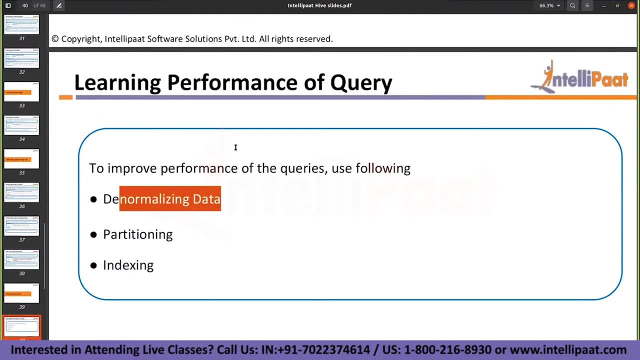 Okay, And the optimizations, the denormalizations, partitioning and indexing: These are some of the concepts we can discuss. How do we create the index? So this is all again advanced concepts. how do we index, How do we create the index and how do we use that index to, uh, better retrieve the results? 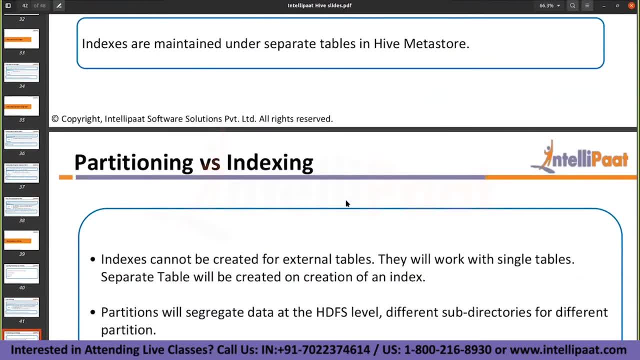 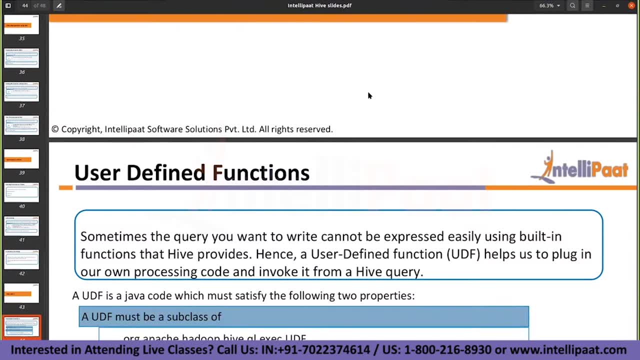 So partitioning, we know what to do, and there is something called, as a user, different functions. So in, in, in one of the slides we have seen, uh, different, uh built-in functions that are available. Right, 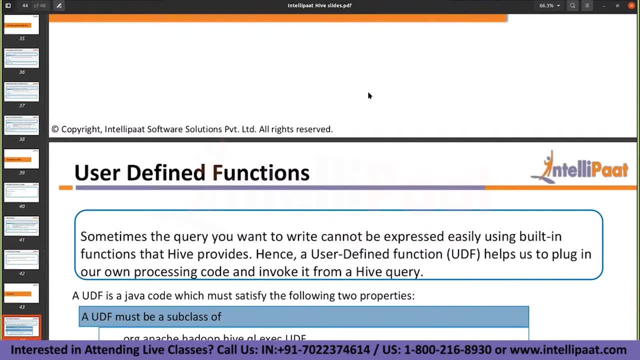 So if there is a functionality which you wanted to uh, which hive does not support, if it should, I have your hive, as hive does not have any function for it and you want it to create your own function for it. Okay, 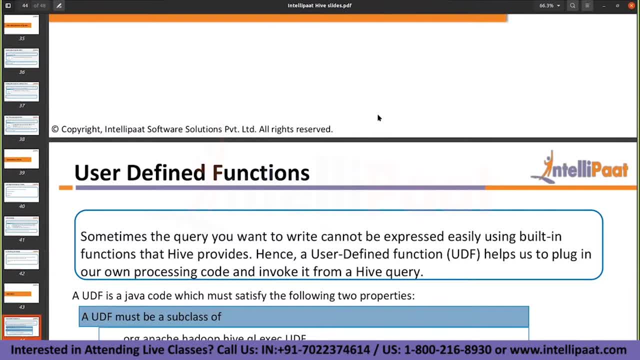 So let's say something like: um, for example, there is a column wherein you have the data in the format of timestamp. Okay, So you know the timestamp format, the date, month, year, uh, hours, minutes, seconds and the time zone, right, 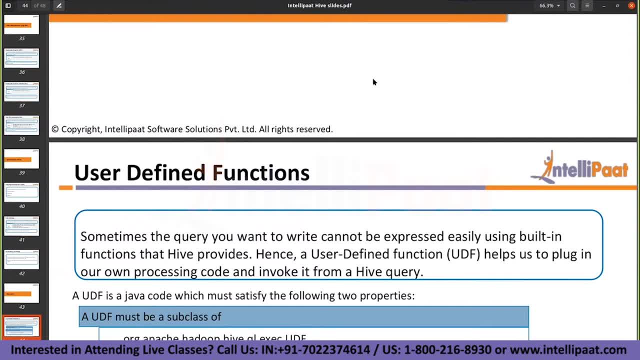 All these things together, You form it as a timestamp. Okay, So you don't want a timestamp column, You want it to extract only the month out of the timestamp column. So your requirement is something like this: Okay, So I, we, we cannot tell where, exactly where exactly you'll be using this scenario. but what if your requirement is something like this: 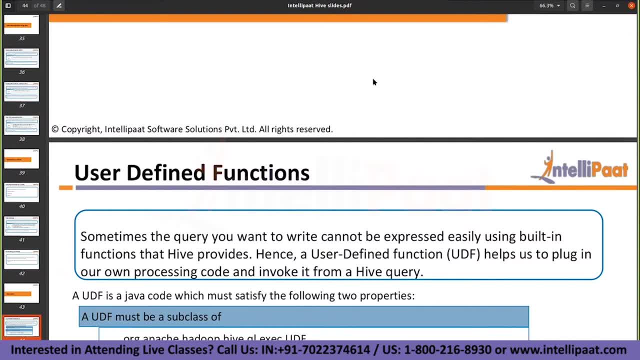 So you don't have any function to extract month out of the timestamp. Let's assume So you will be creating your own function, You'll be creating your own Java program. Uh, so this is how you'll be writing. So there is a uh method, there is a class abstract class, abstract class. 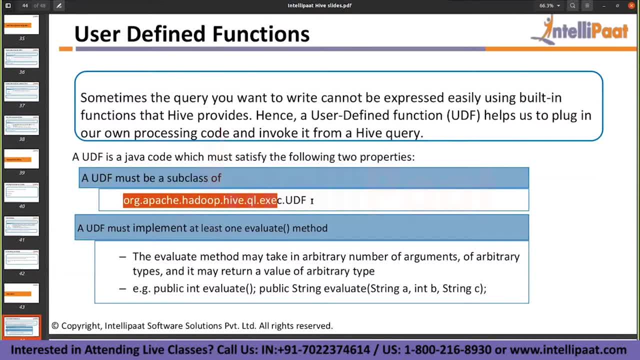 Okay, Abstract class- UDF abstract class. You extend this UDF abstract class and define your own logic for it and create one function for it And then you will start using it. So there are six steps. I guess five to six steps available. 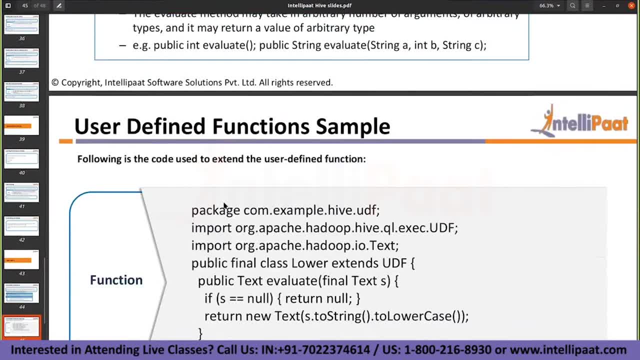 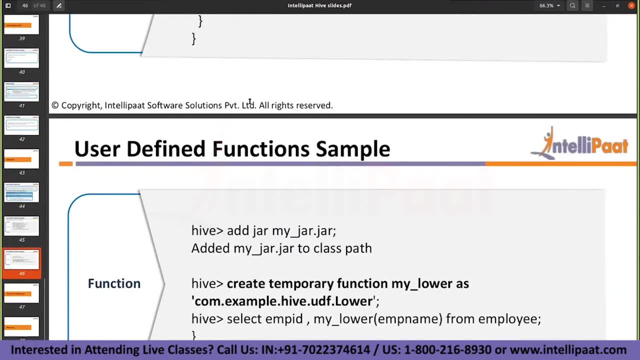 This is how you write the program. So this is again a MapReduce program. and how many steps. So add jar. I mean, uh, creating this particular program is one step, uh, creating a jar from this program and adding the jar to the hive class path and creating a. 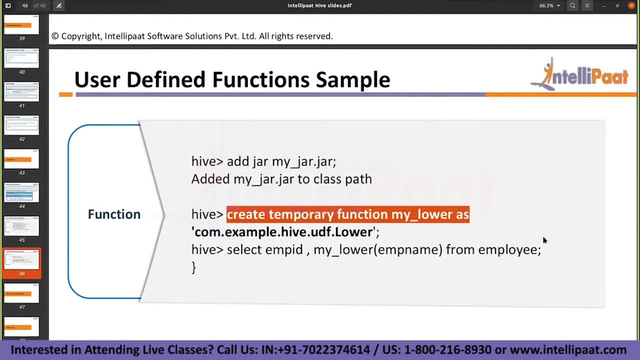 temporary function and then using the temporary function. So four to five steps are available in the UDF process creation. So generally user different functions are used when you don't have any built-in function for a specific functionality. If you frequently use that uh particular functionality, it's it's. it's going to take time for you to implement every time. 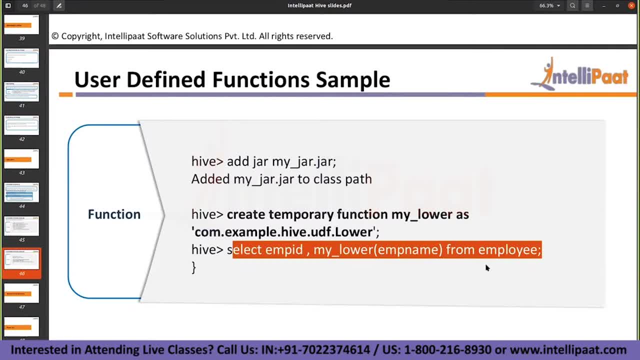 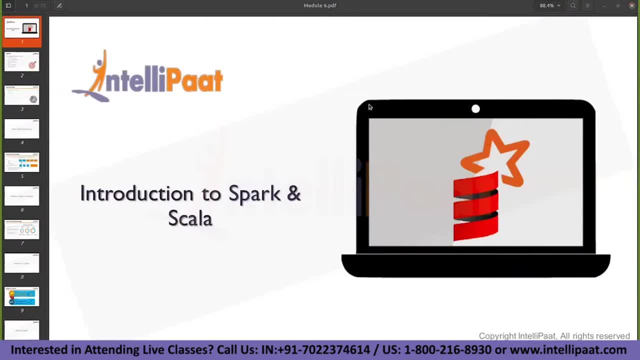 So you create a built-in function, you create a custom function. That's because there's a user, different functions. Okay. So introduction to Spark and Scala. So yeah, tell me, what do you know about Scala or Spark? Let's just start with Spark. 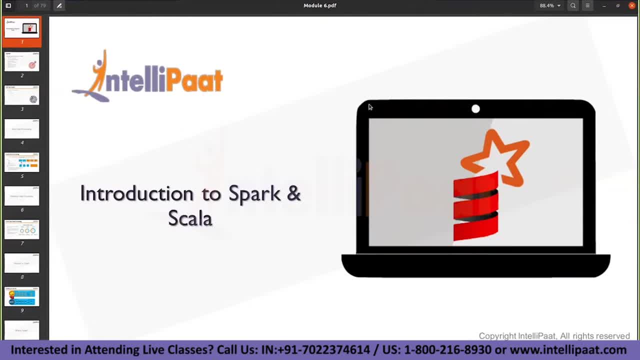 So what do you know about it? Any basic understanding in simple terms: what? what is Spark and what is Scala? So it's processing the large data. What is the advantage that we get with Spark? I mean, see, we already know that there are some frameworks, for example Hadoop, that can process large amounts of data. 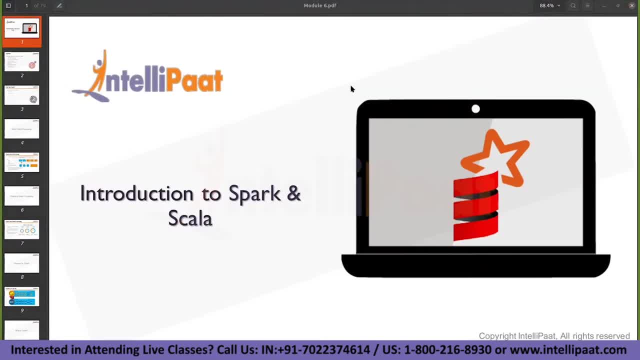 So why? why Spark? It's open source. Hadoop is also open source. Okay, Faster than Hadoop. Why? How? how is it faster than Hadoop? Any any specific reason? What's the main core concept behind? uh? the Spark or the Scala function like this: 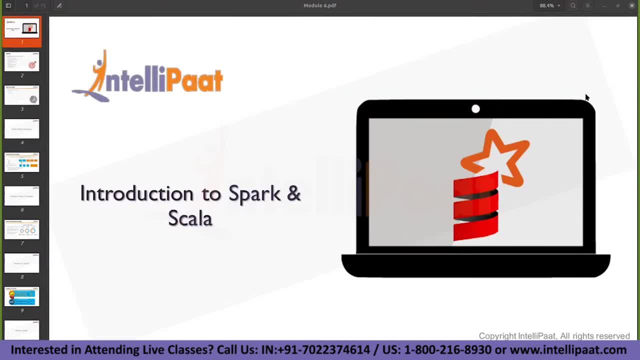 So generally, we we consider Spark and Scala. uh, Spark, let's say, and let's talk about Scala in some time, But so generally, Spark is mainly used for The real-time data processing, both both batch as well as the real-time data processing, and it's considered to be a fast processing tool. uh, almost like a hundred times faster than whatever the MapReduce way of handling it. 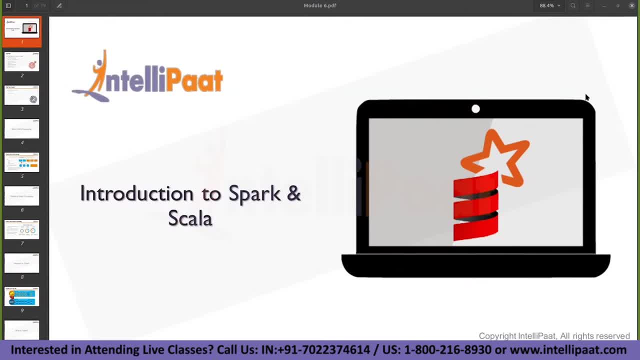 Okay, So the reason why we, we, we say it's fast, because it is, it is, it is doing the in-memory processing. So that's the most important factor for the speed that it is, it is, it is achieving. 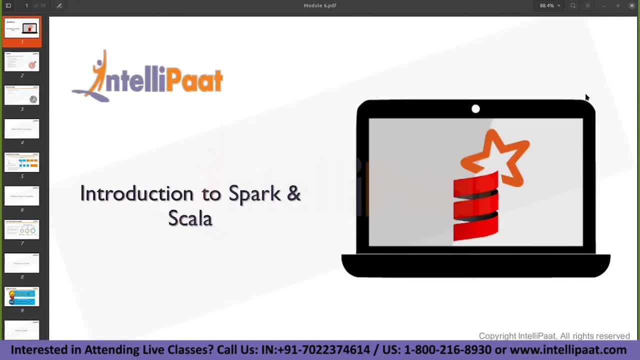 Okay, So in-memory processing is something which is going to increase the speed drastically And uh, uh, that is why we are- we are getting this kind of an advantage. Okay, So what do you mean by this batch and real-time processing? 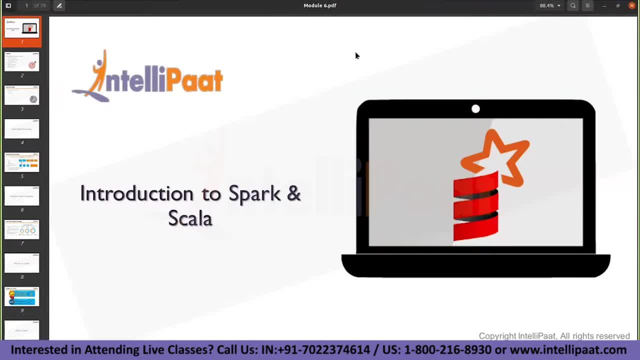 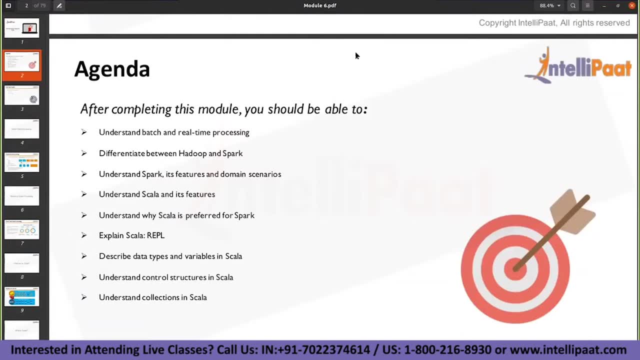 Okay, Let's get to that slides. So, for the agenda being so, we should be able to complete the uh. we should be able to understand the batch and real-time processing, the difference between Hadoop and Spark, Uh, uh. these are all the concepts. 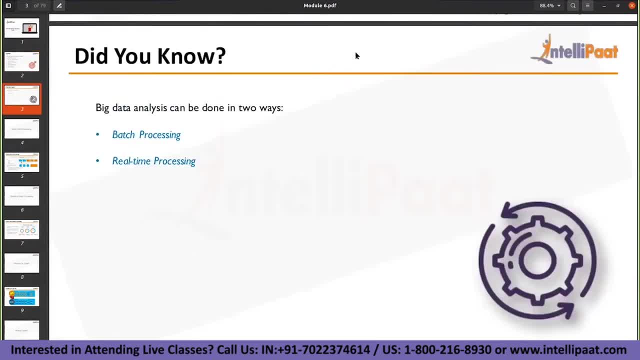 So we will be discussing- and big data analytics analysis can be done into- so there is a batch processing and a real-time processing. So what? what exactly do you mean by batch and real-time? What is batch data processing, So real-time? you must be knowing it right. 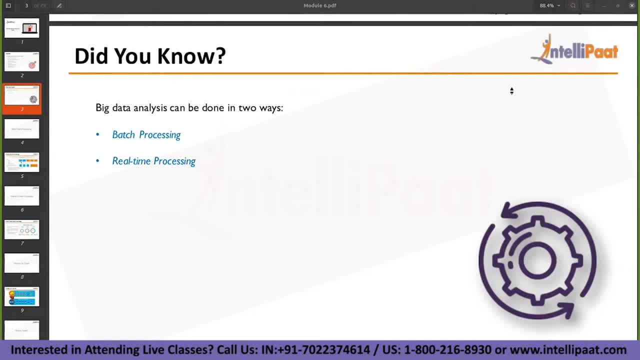 Okay, So we'll divide the data into batches and then process it Then. then, what is real-time So generally? uh, the batch processing is something where you have the data. You have the data already available. Okay, So the file has already been generated. 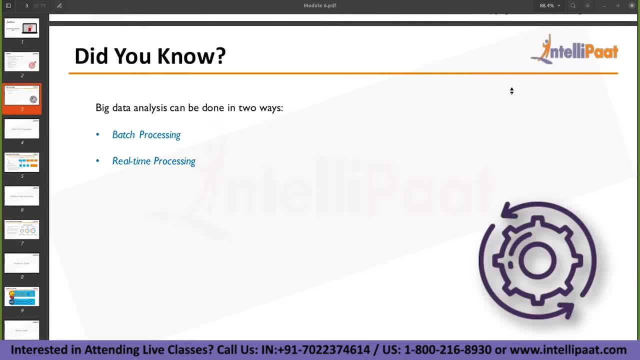 Okay, So it's not a scenario where the file keeps getting updated every every second or every minute. Okay, So the file has already been generated and you already have- uh, uh, whatever the extension, you already have the file getting stored. 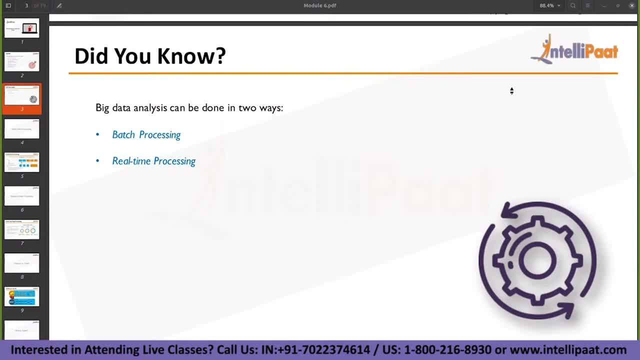 And then now you are, you are trying to analyze that particular data file. Okay, So let's say I'm generating a CSV file, So I completely loaded the CSV file in so-and-so network drive And you have to read that file and do some kind of analytic process. 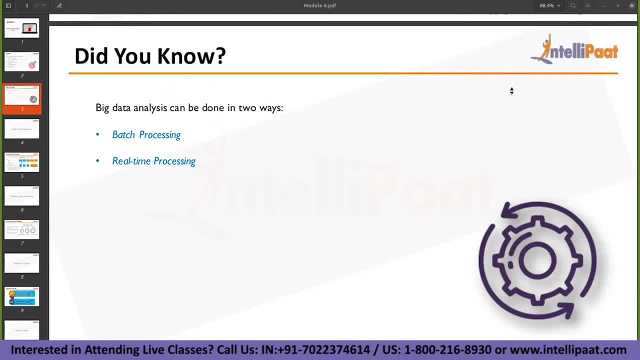 Okay, So the file is already available. It's it's already got loaded, It's already completed, It's in completed stage and you're trying to access it now. So how you're going to access it is is is secondary. 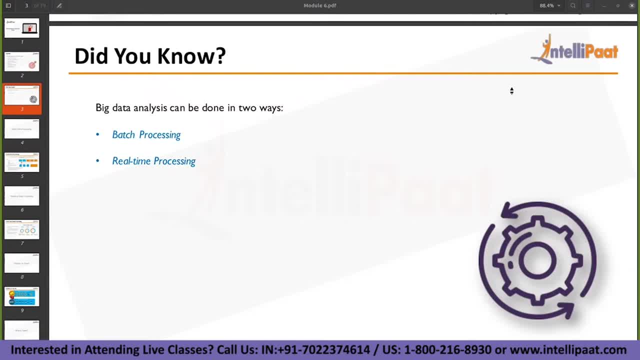 You use Spark, you use Hive, whatever, whatever the tools and technology you wanted to use, But that all comes under the batch processing. You, you, uh, you read the data which is already available, You break that into multiple batches and you'll be loading it into your framework and process it. 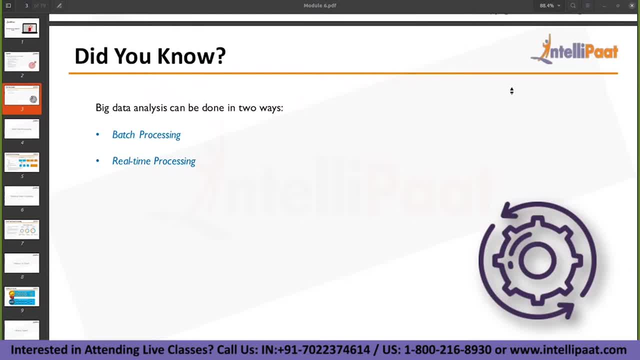 But realistically, Hitler time, is that something that keeps changing every, every instance? Okay, So there is a file that is getting updated, that is getting, or there is a database that is getting updated. So, for example, I have a database, I have a table and I I kind of inserting that records that every. 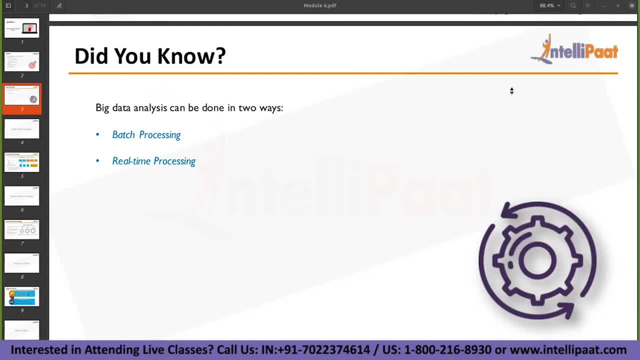 So what you need to do, as and when the data gets generated, you are supposed to extract it and you're supposed to process it. That's that's what we consider to be a real type process. Okay, So that's the difference: when the data is already available, when it's not moving. 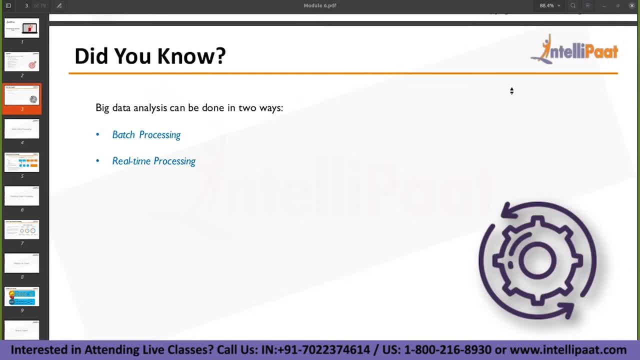 Yeah, it's not. it's not changing frequently. then we consider it to be a batch processing and real time is something which keeps updating every time and you are supposed to access it in in a real time manner. so there is no system which is going to access it in a real-time manner. it's always. 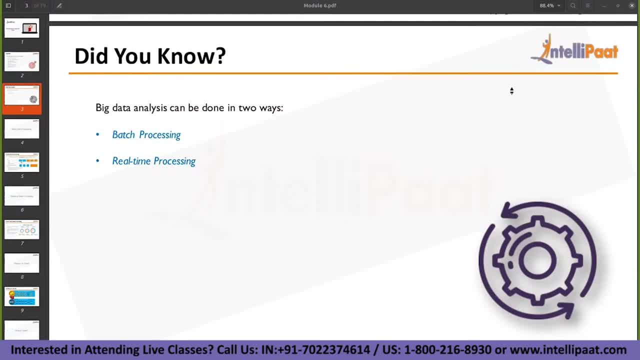 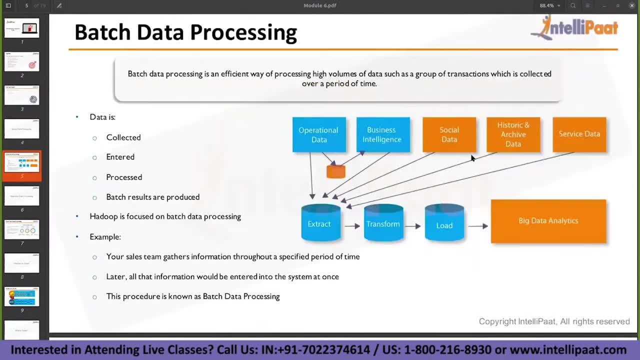 near real time. okay, so near to the real-time process getting it. so let's let's understand what is batch data processing. so batch data processing is an efficient way of processing high volumes of data, such as group of transactions, which is collected over a period of time. so how do you handle this data, which is which is very huge? you you kind of divide that into. 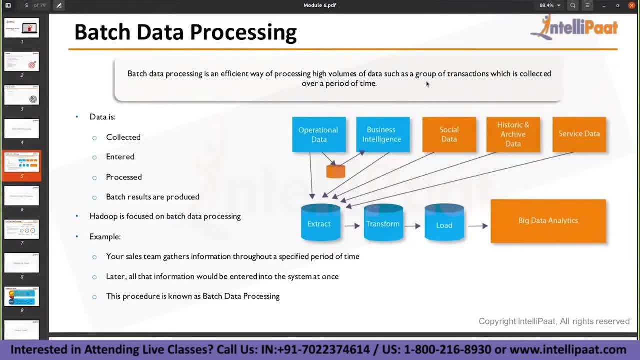 multiple batches and do whatever the analytical process that you are trying to do, so data is collected, entered, processed, batch results have been produced. hadoop is focused on batch data processing, so there is one example that i can share in real-time scenario. so there is one requirement where we have 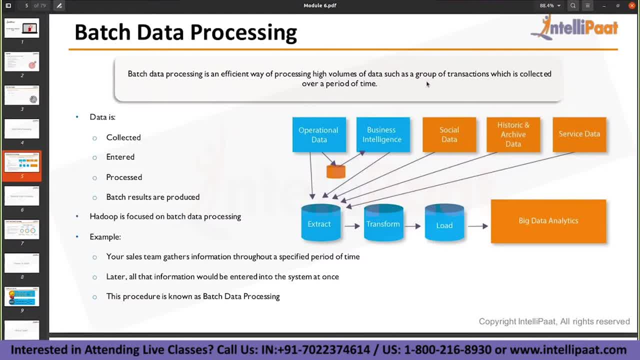 some um 20 lakh records in in one of the uh database, in one of the no sql database. so we have written a program, we have written a python program, we have written a spark program and see, in both the scenarios you are using some kind of a connector to a relational database or 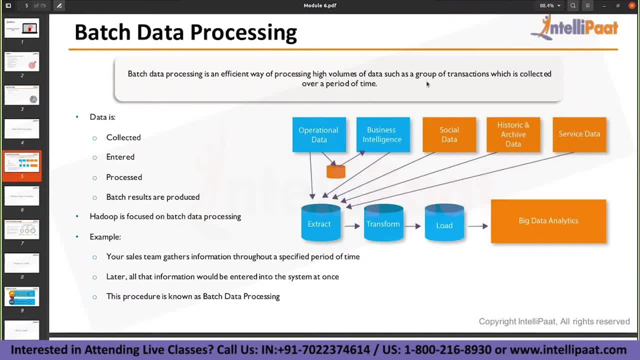 no, no sql database, it's mongodb. so you are using a connector to a no sql database and you are trying to extract the data from a no sql database, uh, which is a zero sql database, into your uh python uh data frame, partner's data frame of the spark data frame. so how many of you are aware of python? it is very high level. 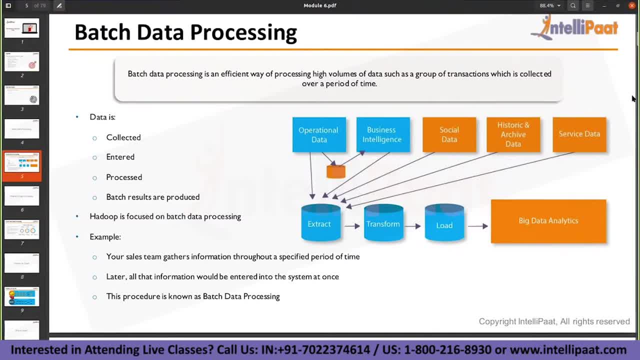 okay, that's fine. so, using some connectors, we will be extracting the data. so it's it's always not possible. it's always not possible for you to load the entire 20 lakhs of records into your whatever so-called processing frameworks- python or spark. so what you're going to do is you're going to do it. 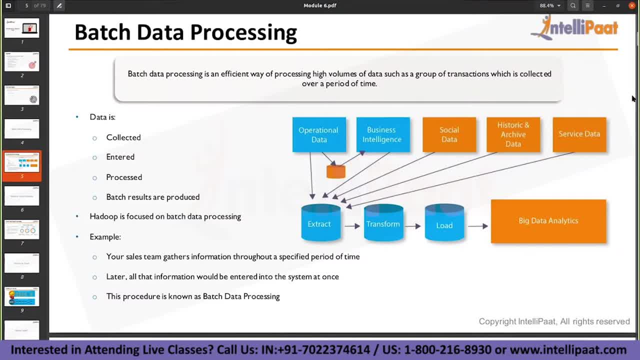 to do you. you divide that into multiple batches. so the first time, whatever i'm doing is i i have to, i have a job- to import all the records, all the 20 lakh records. but 20 lakh records at a time is not possible. so what you will do, you will. you will break the data into multiple batches. i'm not. 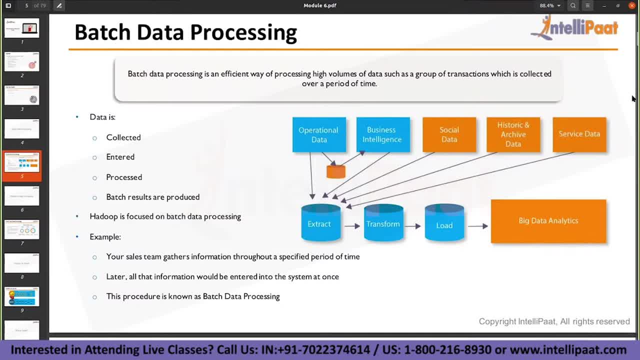 breaking it actually. so i'll only collect the data. whichever is is is uh, with with some timestamp, let's say okay, so if the data has been generated from so and so time to so and so time, i'll select that as a first batch and i'll i'll flow this particular batch of data through all the processes. 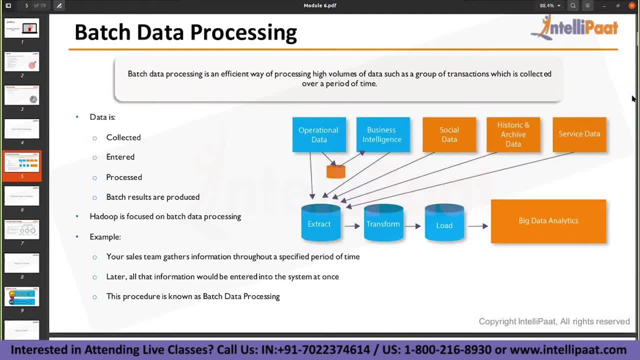 and i'll dump it into whatever the destination it is okay. so you're extracting some amount of information, some batch of information, transforming it, then loading it into some, uh, destination system. so all these things you are doing it in batch wise, okay? so depending on some timestamps, 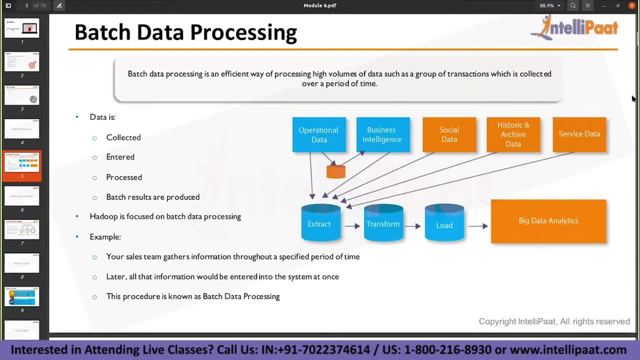 so, from here to here, here to here, something like that- uh, giving an upper limit and lower limit, you'll be able to do that. so you'll be able to do that. so you'll be able to do that. so you'll be extracting some data and you'll be processing it. so this is batch data processing, which is 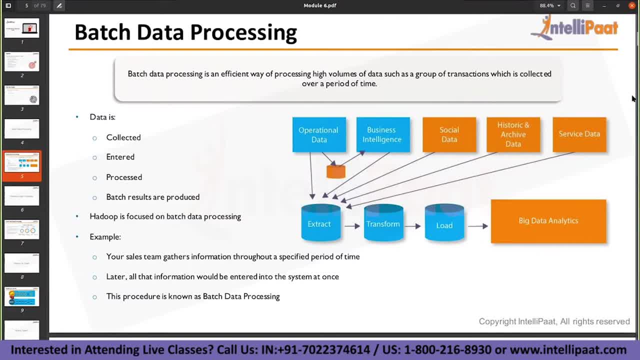 already been generated, which is already there. that is the historical load. i can say, okay, when you want to migrate the entire data into your uh hadoop ecosystem, then comes a near real time. so after you have loaded the entire data, whichever, you have all the 20 lakh records, whichever you. 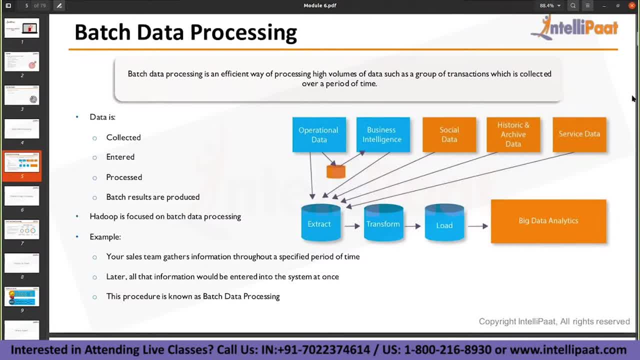 have into your hadoop framework, into htfs. let's say, now, whatever the records keep generating every day- for example, today i have run the job, so tomorrow the same time i'll i'll trigger the job. so whatever the records that have been generated from now to till tomorrow morning till tomorrow the same time, those records, i'll be pulling it. so that is. 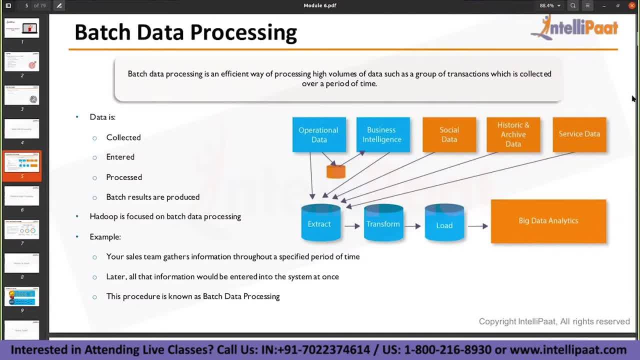 a near real time. i'm calling that as a near real time. it's not a very near real time scenario. we are giving one day interval, but that's how it's going to be. so you, you generate the, you generate the events or extract the data as and when it is generated, so there is a real-time streaming also. 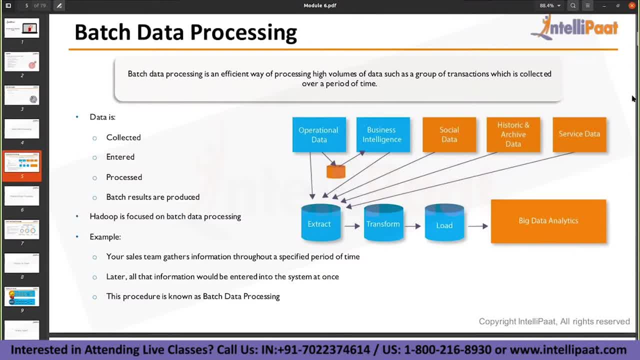 available using cup and different tools. you can do that as and when the data gets generated, the trigger will happen. but again, everything, everything comes under the near real-time process. okay, so etl, etl process, extract and transform and load, uh, the data which is already available, and you do that in the form. 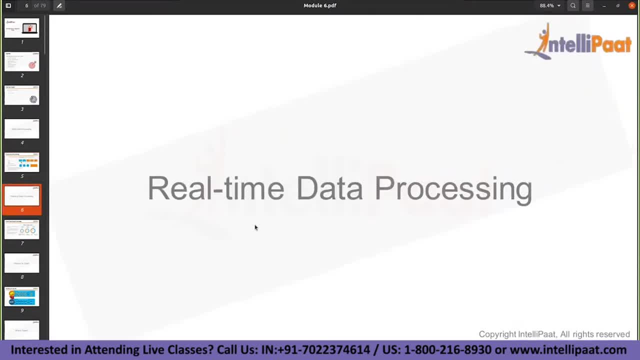 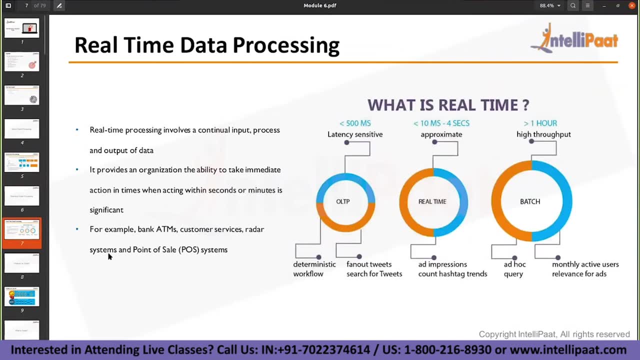 of batches. okay, then what is real-time data processing? so real-time data processing, yeah, involves a continual input process and output of data, so it provides an organization. the ability to take immediate action in times when acting with within seconds or minutes is significant. so, for example, back atms, customer services, radar systems and point of sale systems. 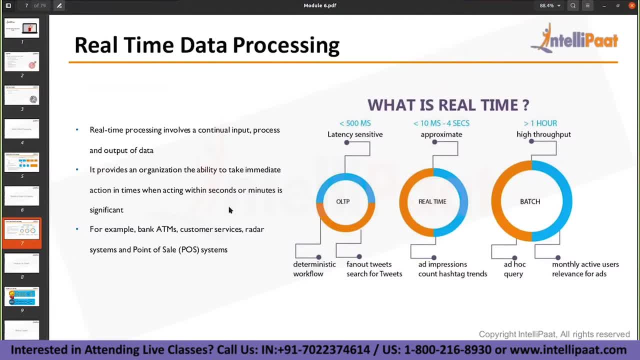 so what are they trying to do here in near real time? so the data keeps coming continuously within within seconds interval or within some minutes interval. so your job is to try and read the data as soon as possible it is generated. okay, so as and when it is generated. so how do you do this? 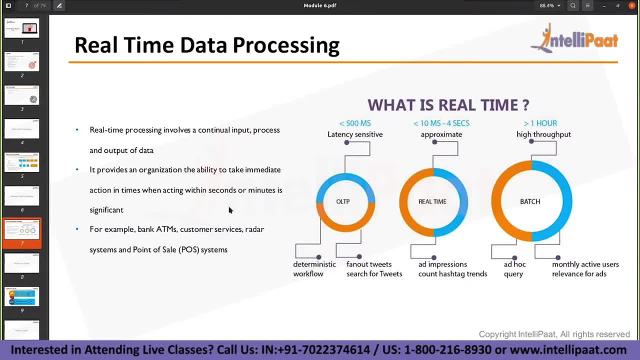 uh, you kind of um establish a trigger with the source system, with the database. let's say, on the source side you have a database, on the destination side you have a hdfa system. in between you have some process, so you will establish some kind of a alerting mechanism on the another source. 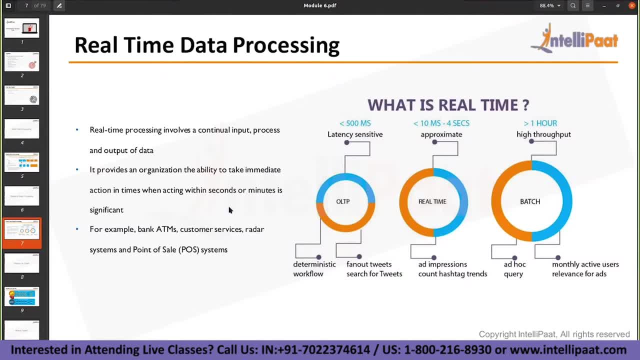 site. so this is a very odd term to use alert mechanism on the source side. so the source site, that the source site should be an alternating alert cycle, either early색ing mechanism or an extended alerting mechanism, an in- 필요. So it will just keep watching that database. 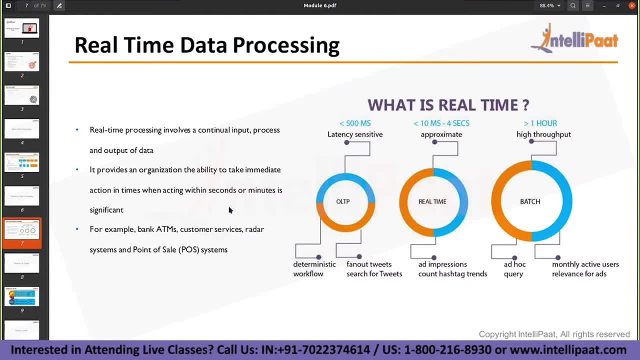 watching the table. So whenever the table gets updated with some new records, it will trigger a specific set of process. okay, So what does this process do? It will start importing the data, it will start processing it and it will load the data into whatever. 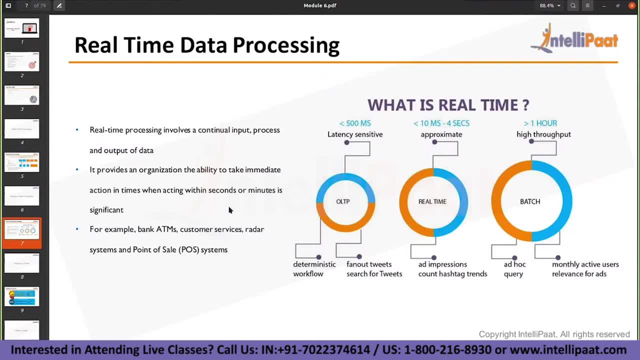 the destination storage system, HDFS or whatever. okay, So what is that mechanism, How that mechanism is being triggered? There is something called as Kafka, you can say. There is something called as Spark streaming, you can say: So what are they gonna do? 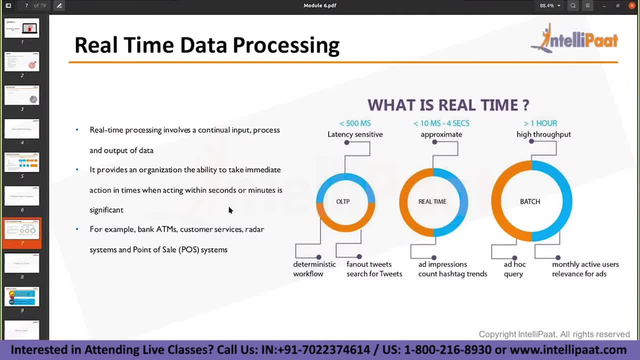 They keep. they just try and watch the database or watch the table all day, always. So whenever there is some change happening, they will trigger some other process. okay, So that's the near real-time processing. So how is it going to be used? 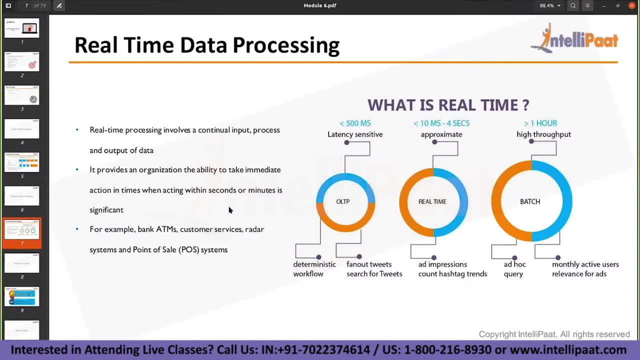 In most of the live examples, like I can say, like in bank ATMs, in POS point of sale system and radar system. So whenever there is a, the change in the temperature, you kind of get alerted, you get alerts on the mobile. 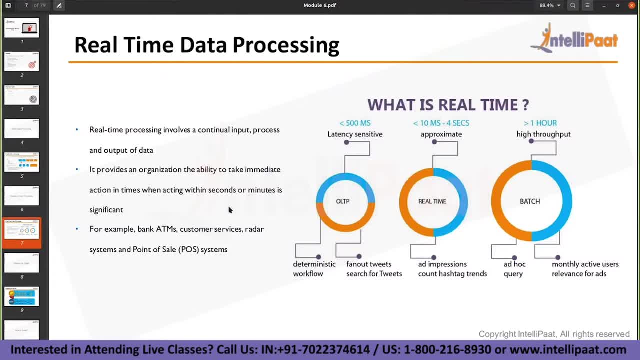 or you alert whatever the authorities wanted to alert them. okay, So this is the near, this is the real-time data processing And, like I said, there is no system which is real-time. Every system is almost near real-time, processing only okay. 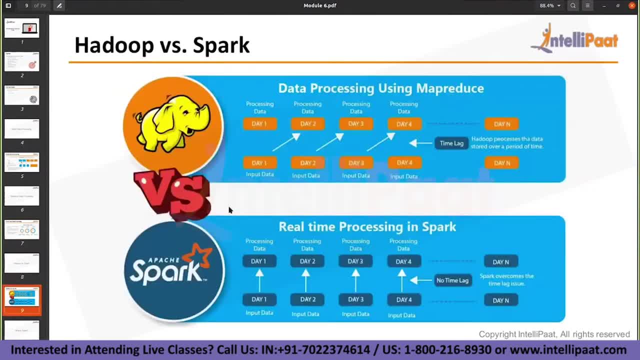 So now the comparison. So data processing using MapReduce, data processing, real-time processing in Spark. So if you look at the comparisons between these two in Hadoop versus Spark, so the processing, the input data, is on day one and this has been processed on day two. 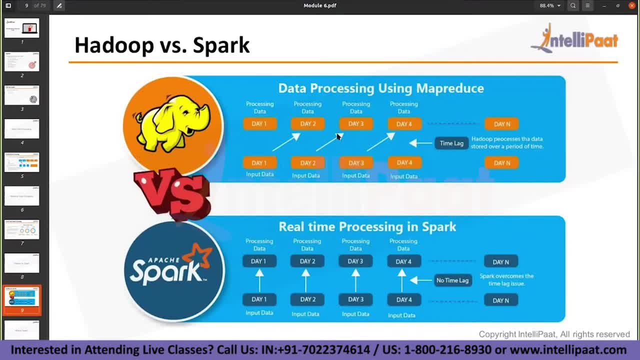 And whatever the data that you generated on day two has been processed on day three. That means there is some time lag between the data getting generated and the data getting processed using MapReduce, So it's not feasible for a real-time processing. okay. 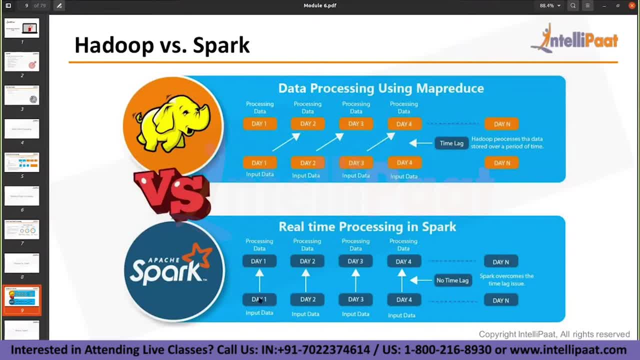 So, but whereas in real-time processing there is no time lag, as in when the data gets generated on day one, the data gets processed on the same day. So it's not in terms of days, but generally there is no time difference between the data getting generated. 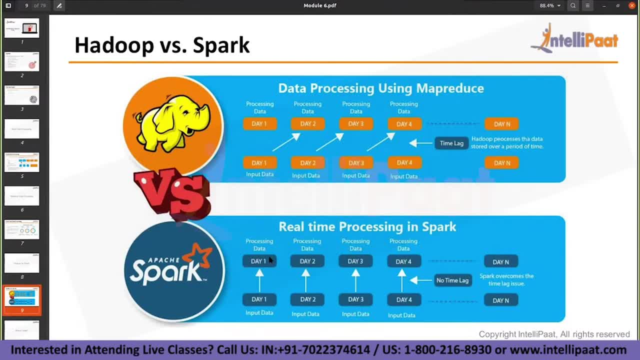 and the data getting processed. okay. So there is very, very limited time lag in terms of the data getting generated and the data getting processed. okay. So this is one representation that I've selected to use, but it's not gonna be something like this. 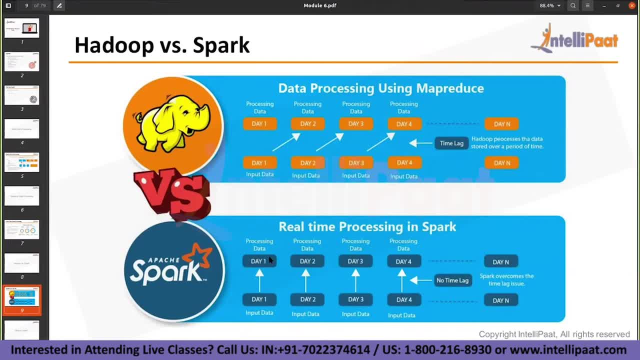 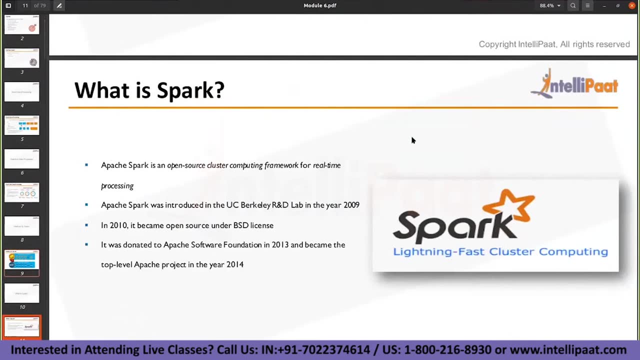 So yesterday the data got generated and then, something like today, you will be processing it. There's definitely some time lag in MapReduce and there is hardly any time lag in your Spark processing. Okay, And then we'll now understand what is Spark. It is an open source. 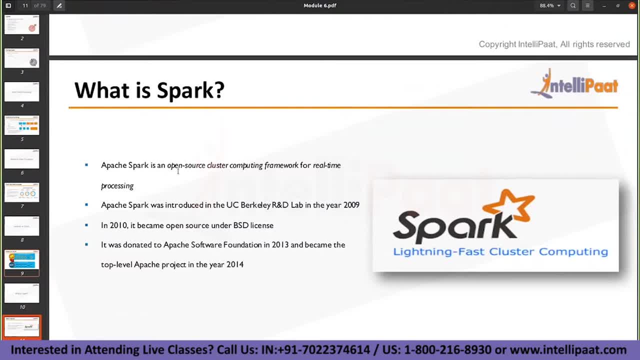 cluster computing framework for real-time data processing. It's introduced in 2009 and some history about it, So 2010 it got some license and 2013 it got donated to Apache Software Foundation. So once it is under Apache then it is termed as an open source solution. okay. 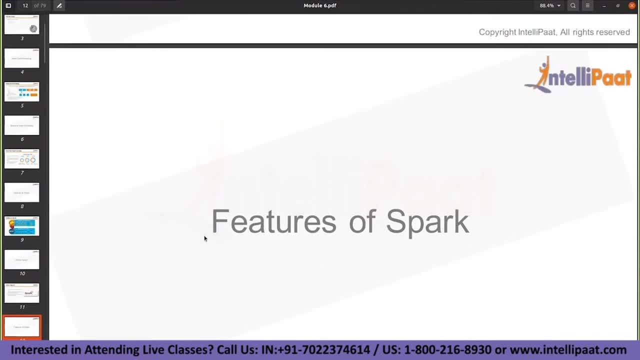 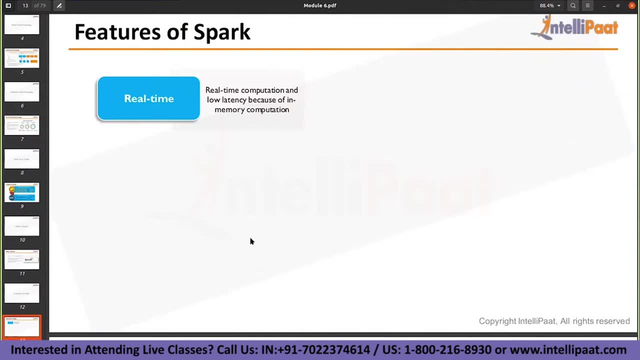 So all the tools under Apache would be open source solutions only. Then features of Spark. What is it? first feature of Spark: It is real-time. So what does this mean? Real-time computation and low latency because of in-memory computation. So what exactly is happening is 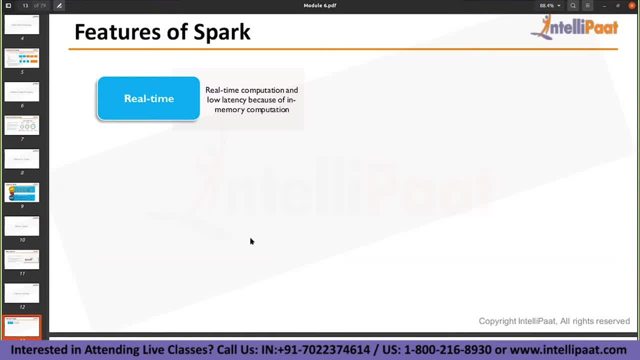 you are doing a real-time processing and you are able to do the real-time processing because of this in-memory computing, Because, see, for example, I think we have discussed about the scenario earlier as well. So there is some data in HDFS. let's say: 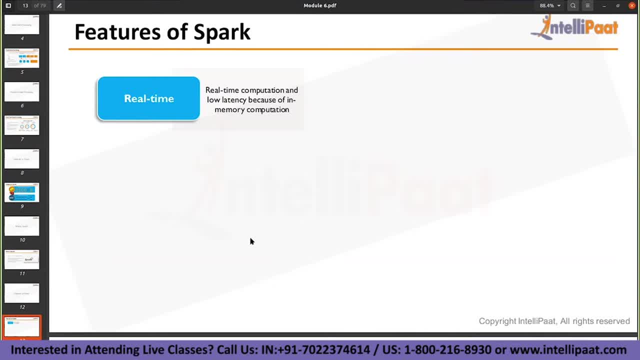 So there is some data in HDFS and you are doing some kind of a processing. I mean, you have written some program to process it. So what happens? You extract the data, you run the operation, you process the operation and you load the data into HDFS back again. let's say okay. 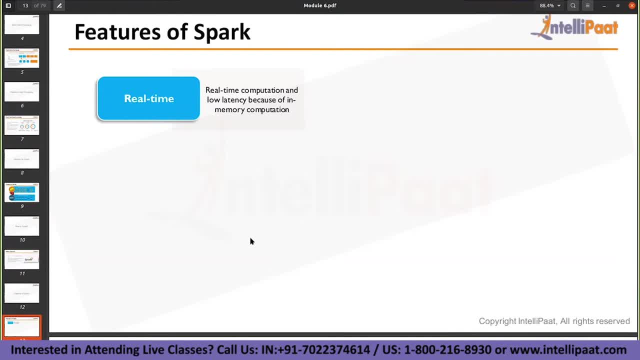 Or there are some multiple set of operations running. okay, So there is a task one, task two, task three, task four. These are not MapReduce tasks, just to let you know. So there are multiple, multiple tasks within the same job, okay. 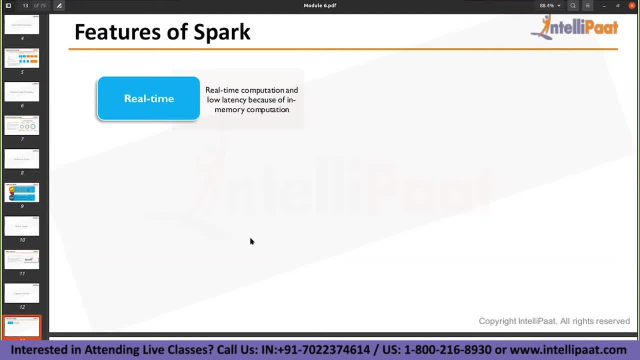 So this is kind of an iteration which is happening within the same kind of a processing activity. So you run a specific task. The output of the task one has to be sent to the task two. The output of task two has to be sent to task three. 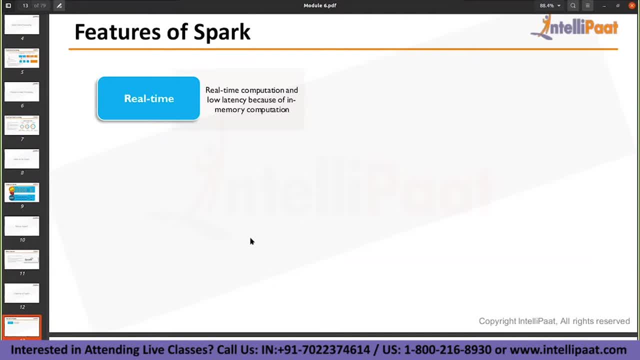 So something like that: you have some series of tasks that are getting executed. So what happens? The data initially was in HDFS, some location in HDFS. So you ran that job. You got some output of that particular task one. So where do you store this output of task one? 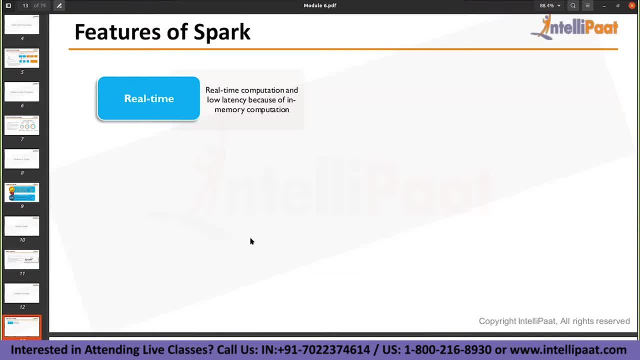 In general, in general. So you have some list of jobs to run: job one, job two, job three, job four. So after generating the job, where do you store it? You again store it in HDFS, right. So after executing that particular job, 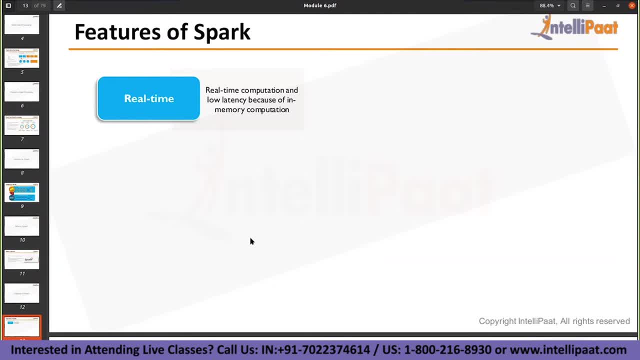 But here, in this particular scenario, what is happening? My job two is also dependent on the job one, So it will wait for job one to complete After the job one task is up. after the job one is executed, the output of job one has to be sent to job two. 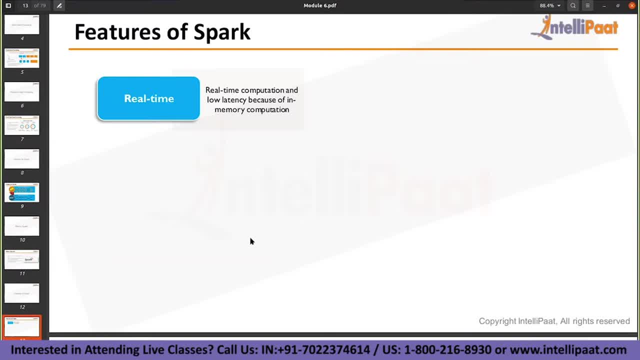 Similarly, the job two will complete execution And then the output of job two will be sent to job three. So here, after the output of job one is getting generated, you are storing it into HDFS. You are not directly sending it to job two. 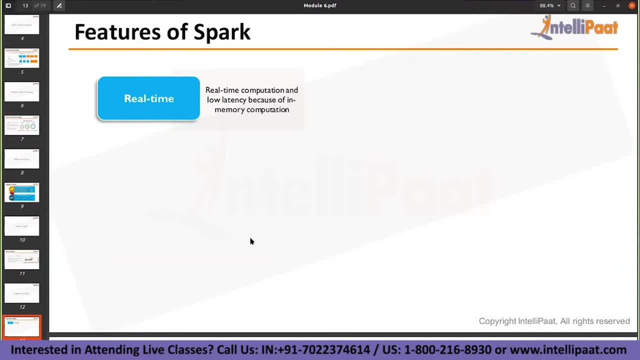 You are storing it in HDFS And that part, the job two, is using it. So when there are multiple jobs getting executed in the form of an iteration, in the form of a loop, multiple reads and writes to HDFS, okay, 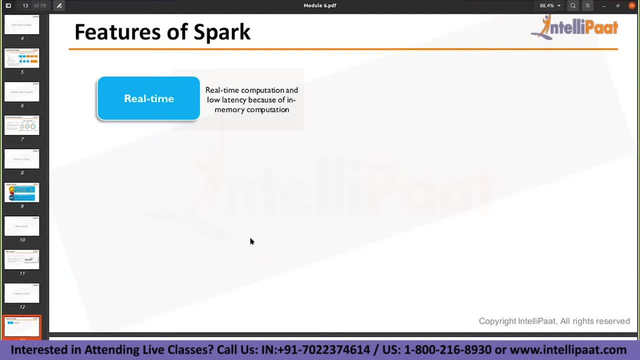 are going to happen, right? so in that case, the time consumed for actual write and read of data in hdfs is going to be more compared to the actual processing time, or whatever it is. i mean the, the time taken for the read and write is going to be very, very huge. so, to avoid that, what, what, what. 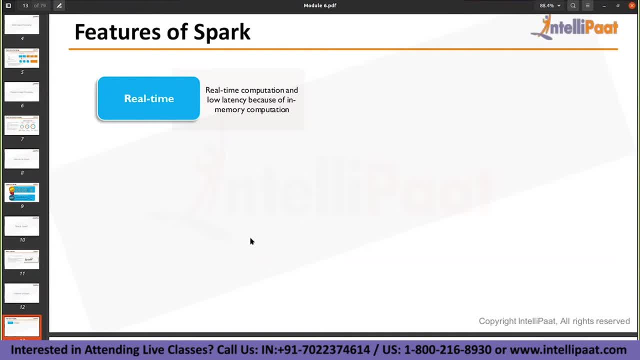 spark does is it's going to do an in-memory computation. so, whatever the results that you generate, intermediate p within the, within the set of jobs, this task, job one output, job two output. so you'll be storing that output, resultant output- in the memory itself. so it's, it's very. 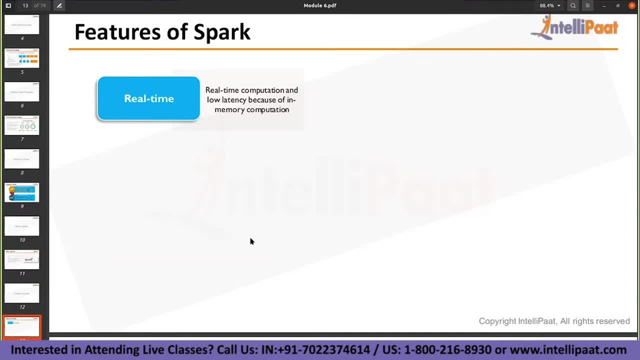 faster to retrieve from that, retrieve the data from the memory rather than retrieving it from the hdfs. hdfs is a physical storage, a hard disk storage, whereas the memory is is something which is available to the processing unit. okay, so the processing, everything is happening in the memory. 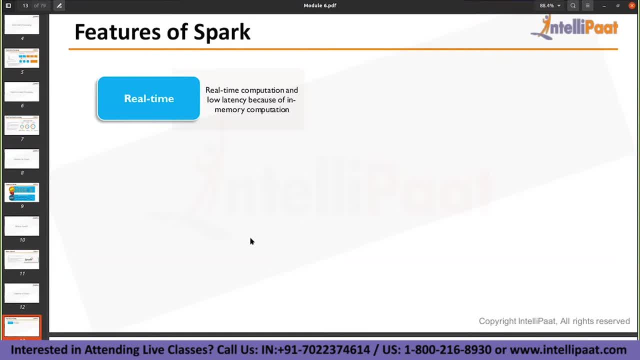 only so. the data is also available within the memory and you tend to process it. you tend to retrieve and store it very quickly. so all the intermediate rhythm, you store it in the memory only. you'll not do the storage in the physical. uh, you'll not give it to. the hard disk and that is the reason why the the time uh taken for the entire execution is going to be very less getting the difference. yes, yes, guys. so that is the reason. mostly your spark applications, or your spark nodes, when you define them, the ram size of their spark cluster is going. 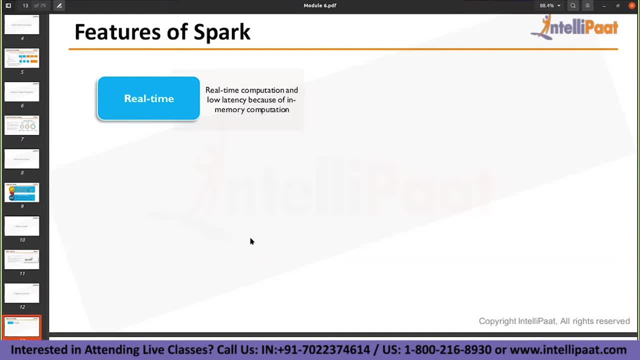 to be very huge, around 64 gb. 128 gb of ram is something which you're going to select. so when we were working, we were having some 64 gb of ram. i guess. i don't know that exactly, but in development environments you have to run 32, so that is how. 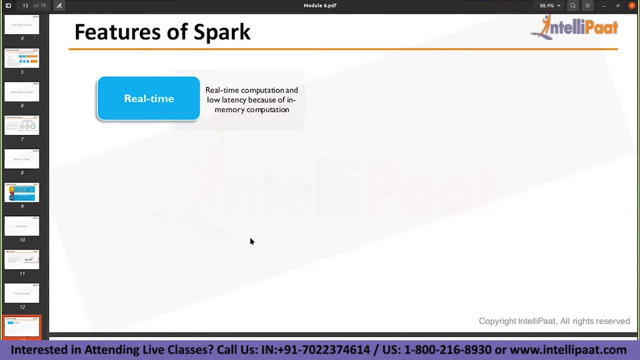 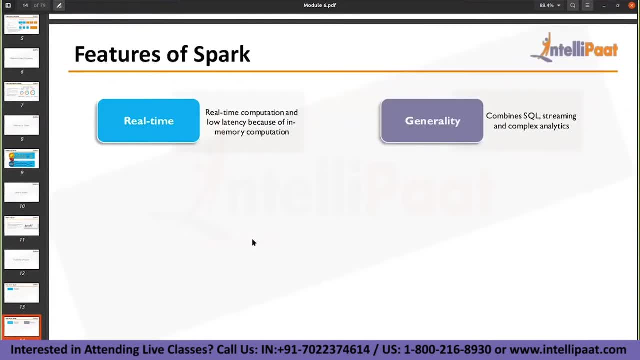 your ram size will be when you are dealing with the spark applications. okay, then, coming to the next feature, there is a generality, so combines sql streaming and complex analytics, so now? so now you're saying there is a better framework compared to map reduce and uh, that is, that is. 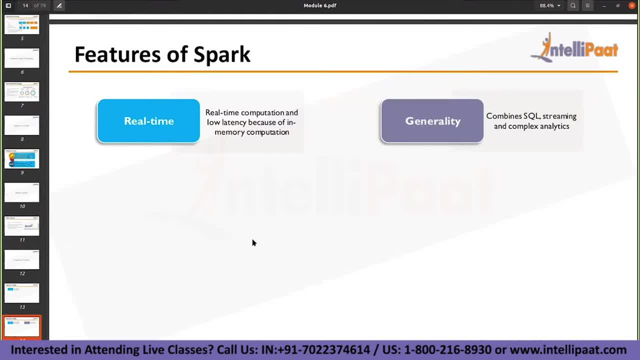 called a spark. so when i say i have spark, i should, i should be able to handle any kinds of data with that, for that right, for that matter. so any kinds of data as in c, unstructured, structured, everything can be handled. there's no problem with that. but how about this high functionality? so hive has a. 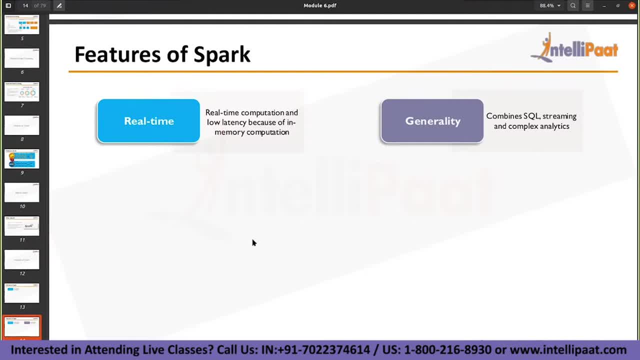 better features or hive has. hive has some better working in terms of dealing with the sql related data, the structured data. so in hadoop framework you have something like hive. when you are migrating to spark, what do you do? i mean, how do you handle the data which is in terms 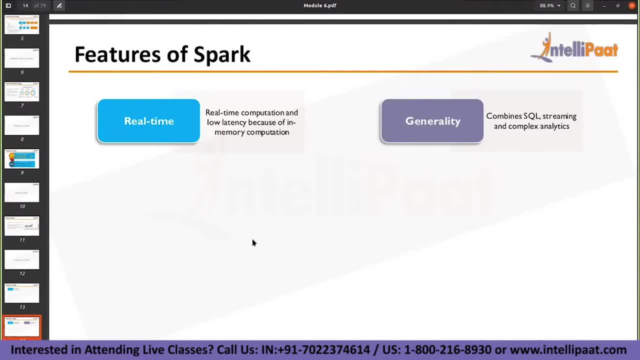 of databases and tables. so for that reason you have something called a spark sql, which is again similar to your normal sql statement. so whatever the table structure, the schema, the column rows and database tables, all that, all that mechanism, all that scenarios are going to come into the spark sql also. so you're giving some kind of a support for the sql way of. 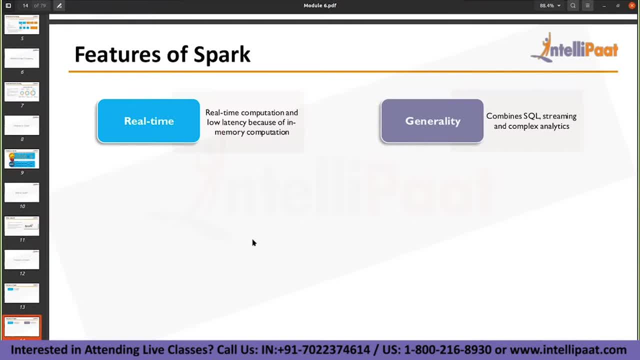 handling the data, also in spark. so there is a completely different module, spark sql, which is going to help you deal with this structured data and what happens when with with, with regards to this streaming data. so in in streaming, in hadoop framework, we had something called as: 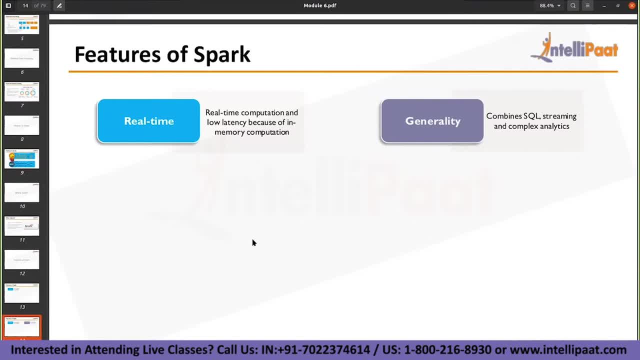 kafka, we had flume. so do you have something similar framework in spark environment also, in spark spark framework also? and there is, yes, there is a streaming platform also available. there is an another is a completely another module listed, that is spark streaming, which is going to deal with the 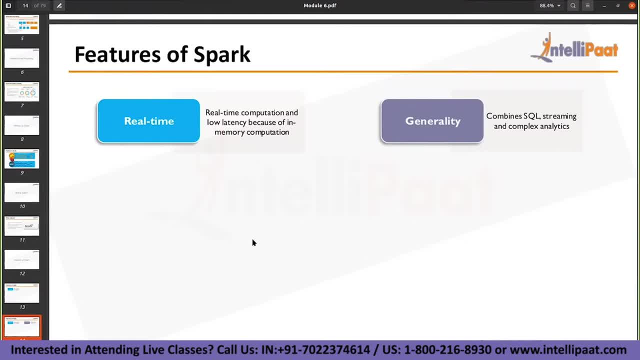 streaming sets of data. okay, so now you have spark sql, spark streaming. in addition to that you have spark machine learning, spark graphics. so these are all different modules within the same framework to deal with different types or different forms of data. if it is an nsql format, you deal with. 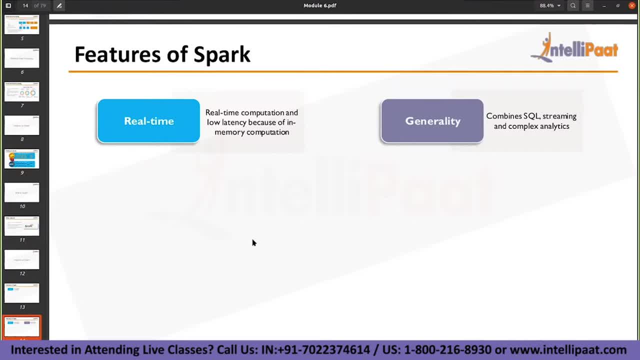 spark sql. if it is in a streaming data, you deal with spark streaming. if it is, if it is some graph related data, spark graphics. if it is a machine learning algorithms you are supposed to execute and you have this spark machine learning right. so for different forms of data, you have different. 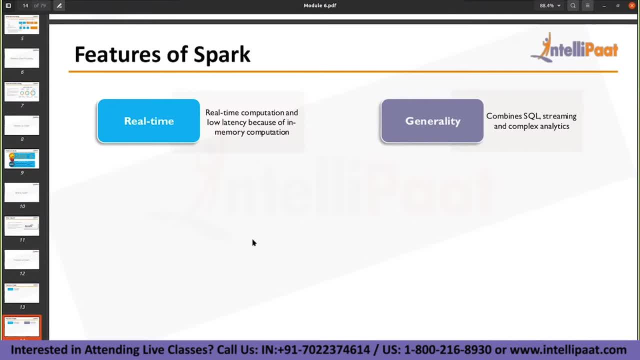 modules allocated within this spark framework. and one simple thing, one, one most important thing here is the uh. there is a concept of rdd. i mean, when we get into the details we'll discuss more about it, but there is a concept of an RDD that's a basic building block in in your 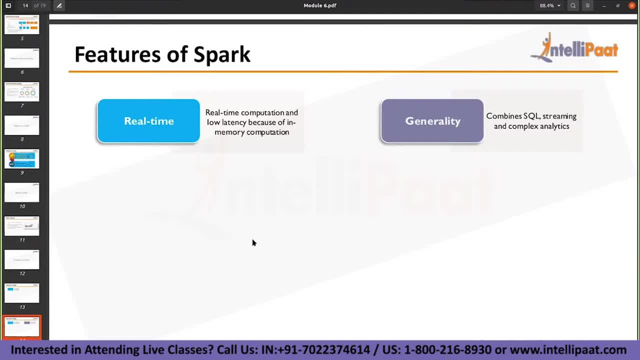 Spark framework and it's going to be common across all the different modules. so you, you have an RDD. you Spark SQL, you have an RDD. in Spark streaming, you have an RDD. so that is something generic across all the different modules or something right. so that means you are creating, you are. 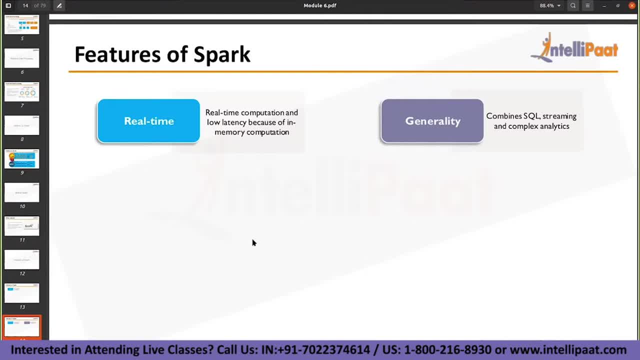 you are taking one input, whichever is it in in, whichever is it in any format, or forget about whatever the format it is. we still don't know which module to use. let's say so: I still create the data, I still take the data, I read it in the form of an RDD and then I'll be using it for. 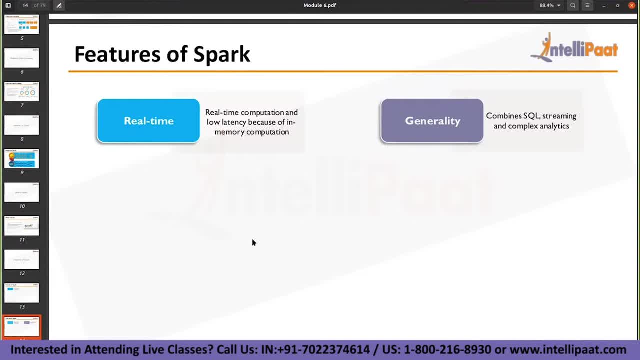 different modules, so the data is being flown across different modules using a simple data set. that's an RDD. okay, so we'll get into the details. it's. it's going to be very disconnected now, but in, in terms of generality, what does that mean? generality, it's, it's. it has got features, it has got. 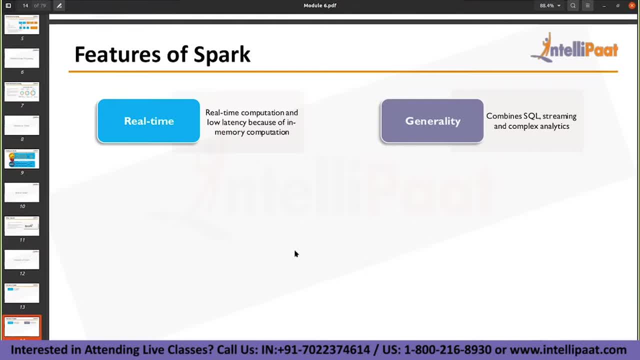 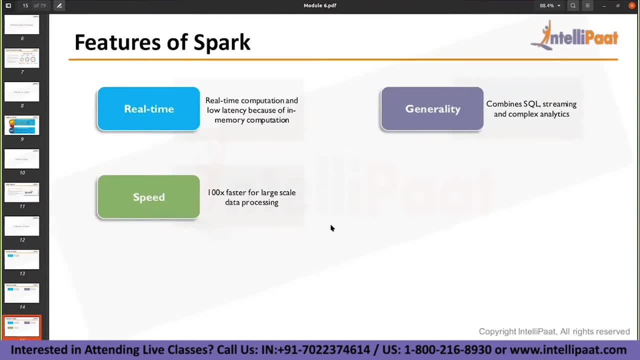 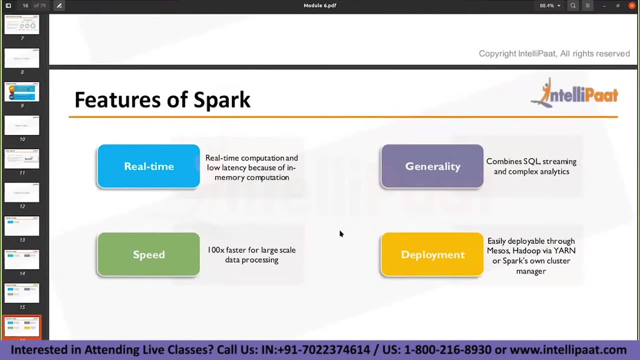 um support for all, all the any forms of data sets and the speed. like I said, it is almost like four times faster, actually a hundred times faster, than the large-scale data processing frameworks. and the deployment is very easy to deploy it. it can be deployed along with Hadoop or it can be. 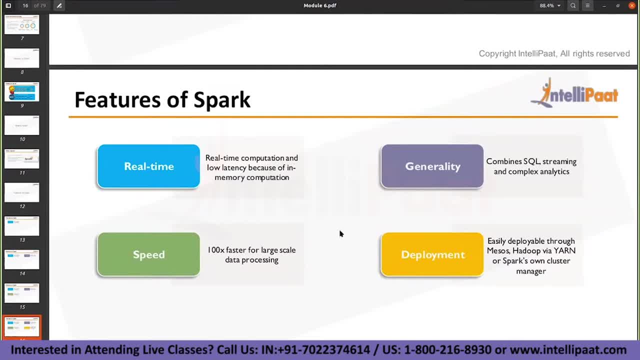 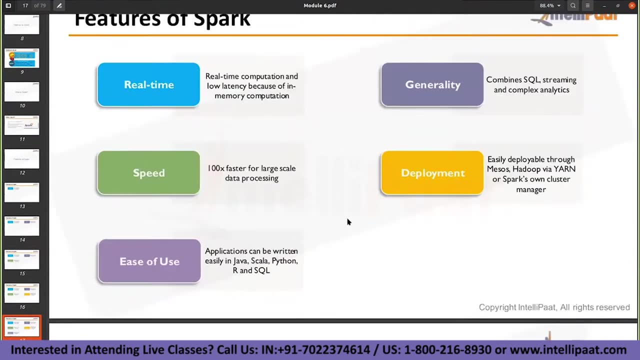 deployed um on its own platform, standalone, on its own cluster, with a specific cluster manager, and it can also run with Hadoop, or it can also done run run with the mesos application. and then the ease of use. so what does this ease of use mean? it is, it is flexible with any kind of a programming language. 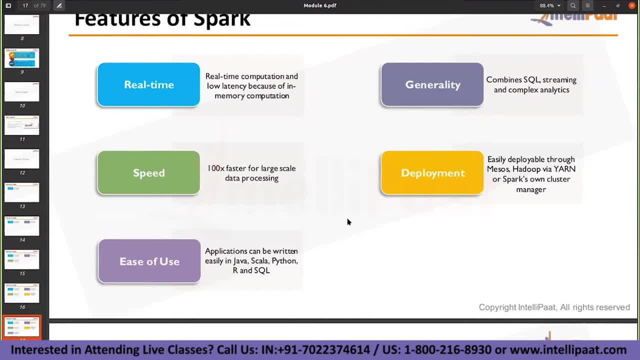 so mostly what? what do the programmers do in general? what kind of programmers do we have? we have a java programmer, we have a python programmer, some kind of a dotnet programmer, and all that right. so if you are familiar with java, that's fine. if you are familiar with scala, if you are 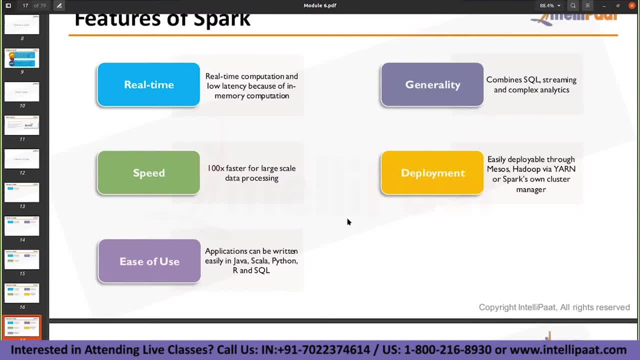 familiar with python, if you are familiar with r- very recently r has got its importance- and if you are familiar with sql, so all this kind of support you have got with your spark framework, okay, so you can, you can write your program in python. you can write a simple sql statement for spark sql. you can write it in. 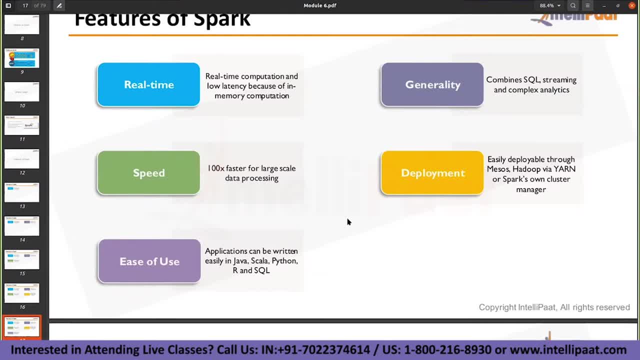 scala. you can write it in java. okay, so java and scala again. I mean, I'm merging both of them together. both both seem to be the same right so you can write. you can use any of the programming listed programming model to to interact with your spark framework. 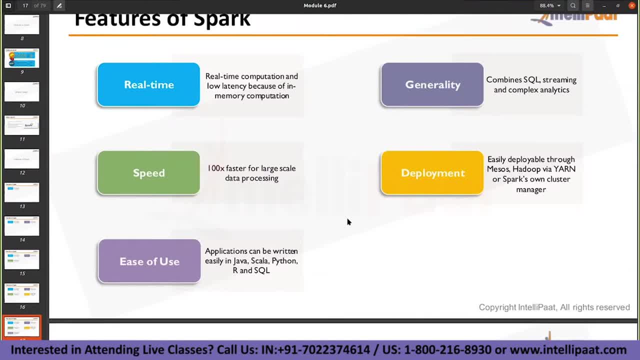 okay, so it's. it does not have any uh uh language or the program uh dependency, the coding dependency. so whoever is familiar with whatever the frameworks or whatever the programming model, they have, they, they, they know, they're there, that that won't be a limitation for anyone, right so powerful caching. so 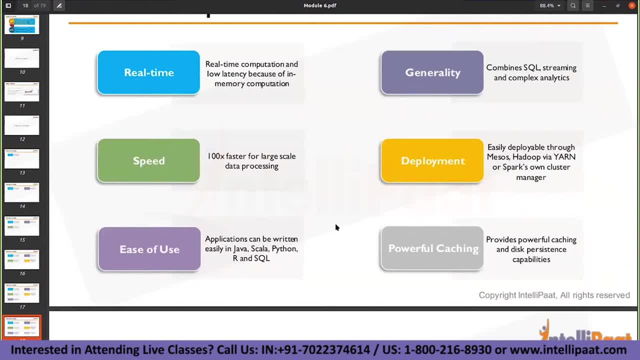 provides powerful caching and disperses to capabilities. so what does this caching mean? discuss that in detail, but generally, uh, even for, for frequently running operations, you, you tend to cache the data in the memory or in the disk. so the caching mechanism is is properly done, is it's a? it's a very powerful mechanism. 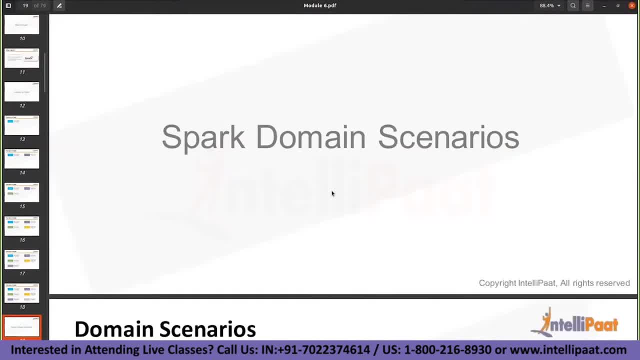 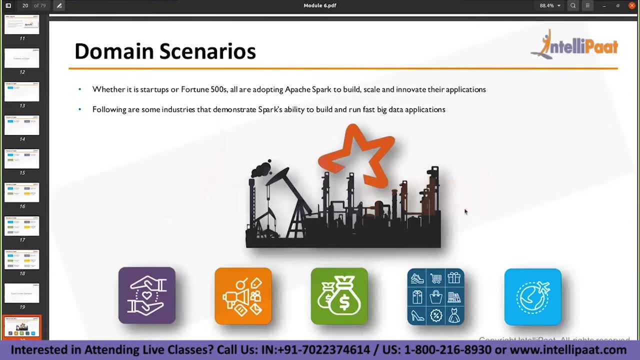 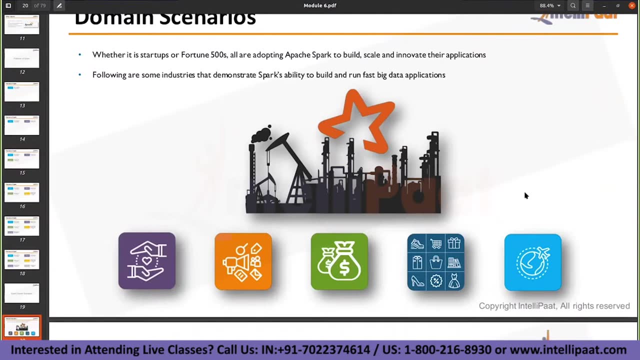 component in your spark applications and there are some domain scenarios that have been listed. so what are these domain scenarios? there are some real-time examples that we can see. okay, so in in most of the most of the- um- what do you say? most of the applications in most of the uh domains. so when i say domain, it's, it's going to be. 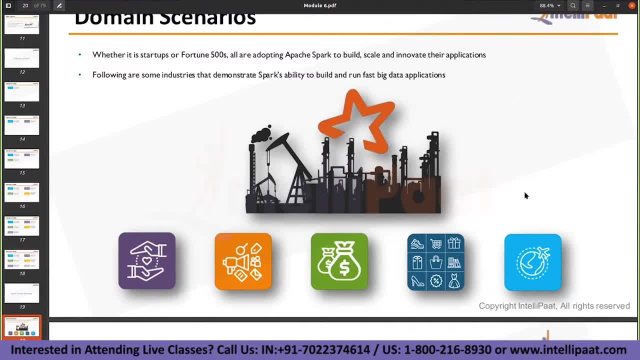 uh across different industries: the financial domain, the the uh, the the tourism domain, or the retail, e-commerce or the social media or the health care right. so all these like this can be healthcare, this is social media, the movie industry or the financial domain, the retail e-commerce domain or the tourism. 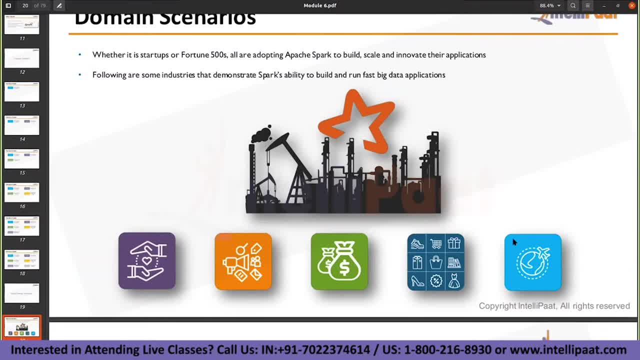 so whichever, whichever domain it is in, like it has got its own importance. it has got its own uh, own own um features. okay, so it it's. it's across the domains. i mean it has got its features, it has got its applications running across the domain. so most of the clients are now running on this. 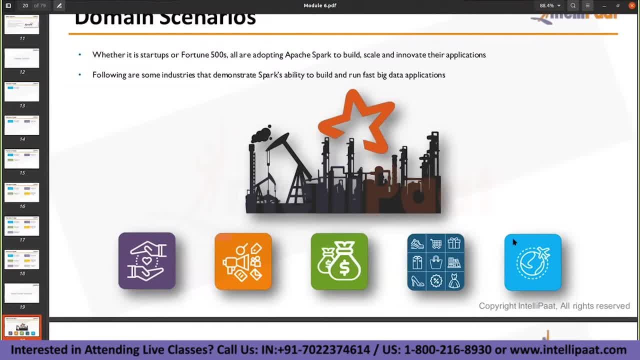 spark framework only right. so now hadoop is something which is which is gone. i can say gone as in like, regardless of you use hadoop or not, the, the companies are using spark. okay, so that is how the importance is: and, and, and, and, even though with a lot, of, a lot of. 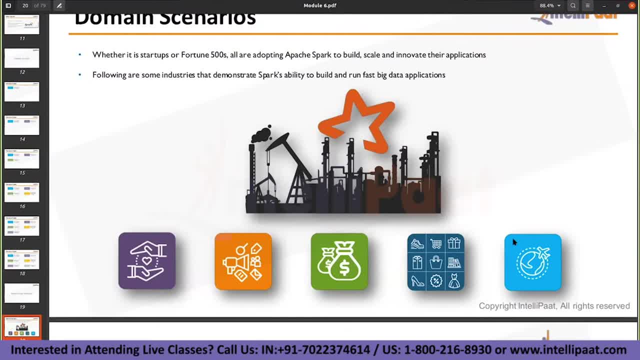 competition with spark sql or the other sql ways, hive is still being used. for most of the use cases, hive is a better, better or, uh, it's a better- tool compared to other sql frameworks. so hive is still in the market. it's it's being vastly used. 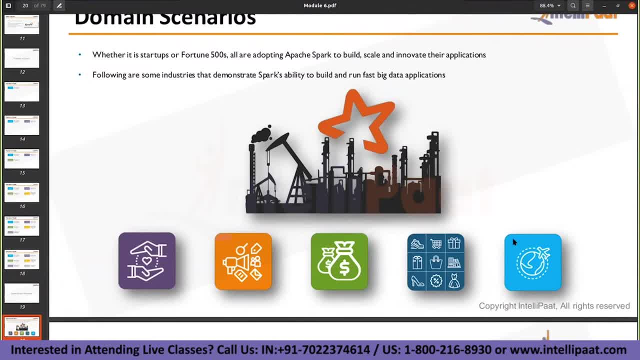 in most of the companies and there is kafka also. even though you have kafka, even though you have spark, streaming, kafka also has has got its importance. it is still being used by uh most of the companies. yeah, right. so even though you have the uh, the, the uh, competition, the the better. 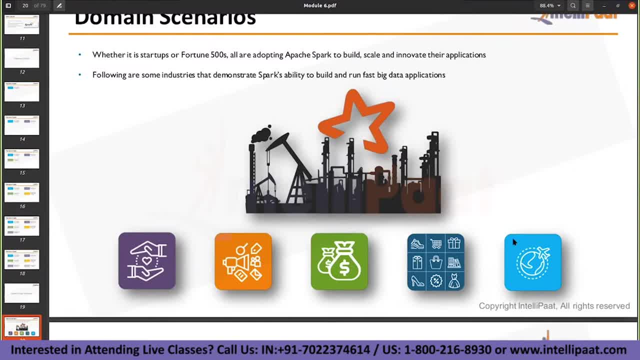 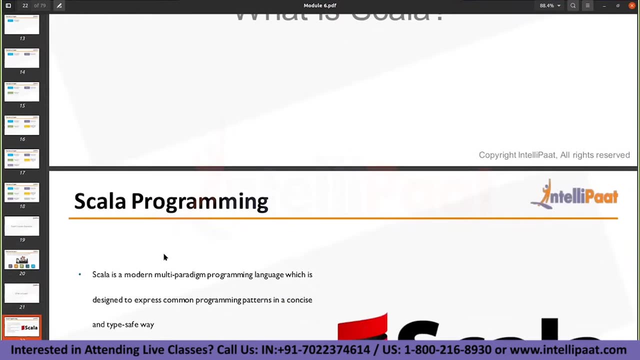 tools, but people tend to use uh first, for various reasons. hive is still and kafka is also still in the market. okay, sustaining, sustaining, spark sql and spark streaming. okay, then now getting into what is scala. so scala is one way of interacting, or there is, there's one way. 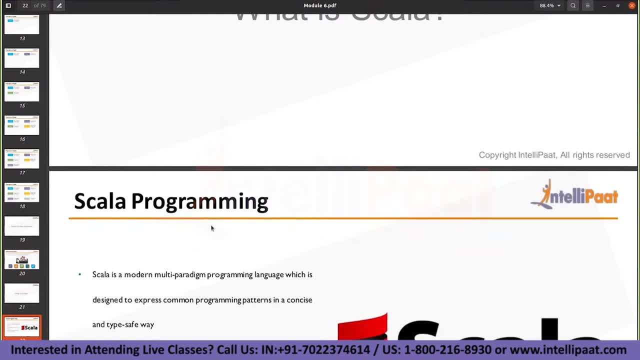 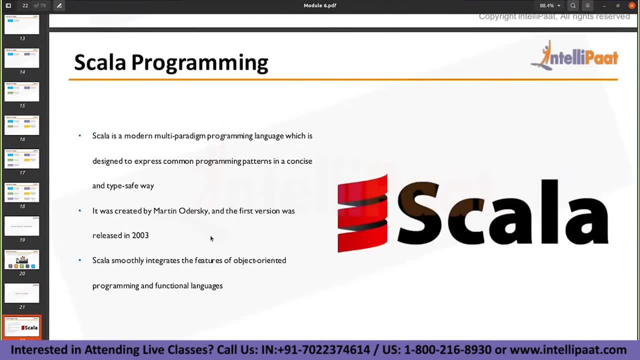 of interacting with your spark framework. so it's a programming language. and how is it designed? when is it designed? all that history you have. and it's a multi uh paradigm programming language which is designed to express common programming planter patterns. you know concise and type safety. so 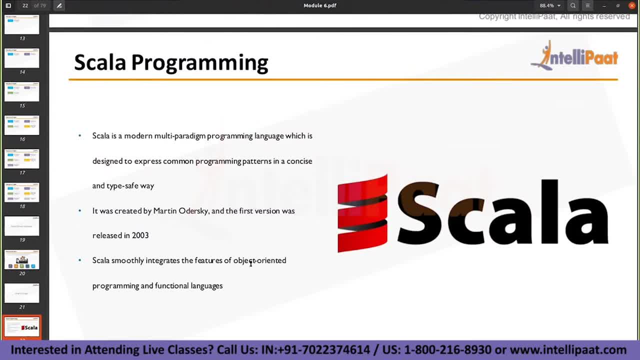 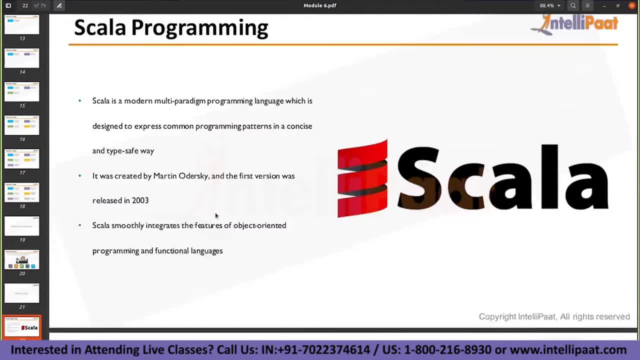 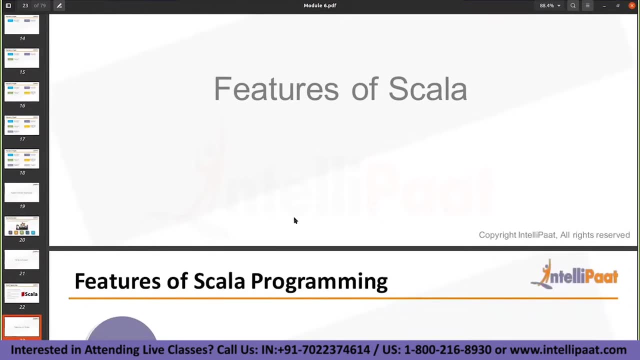 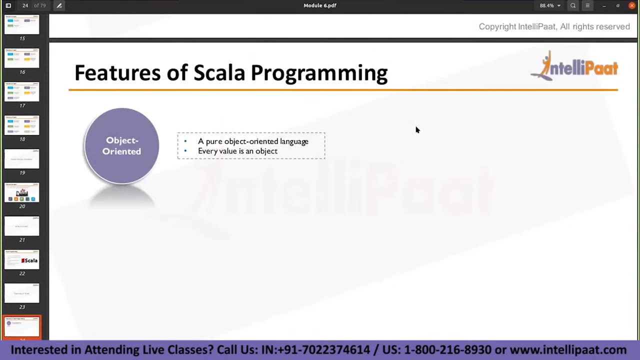 we will get into the details anyway. but so it has been um released in um 2003. okay and yeah, so we'll get into the features of scala. first one is the object oriented uh. what do you mean by an object oriented program programming model? what do you mean by object oriented? 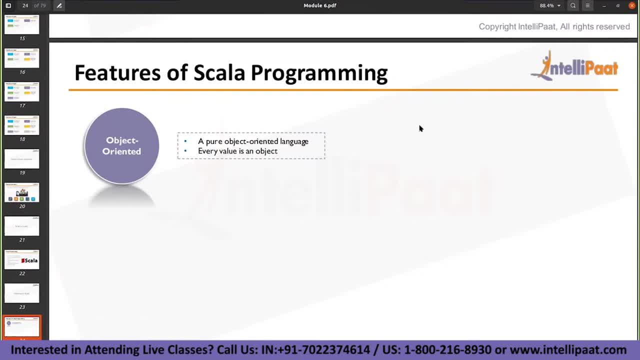 so what's your core background? uh guys, is it java or is it python? what? what's your core programming language? which are you? which which one are you comfortable with among python and java? most of you are java. then i think it won't take much time for us to get into this spark, scala and. 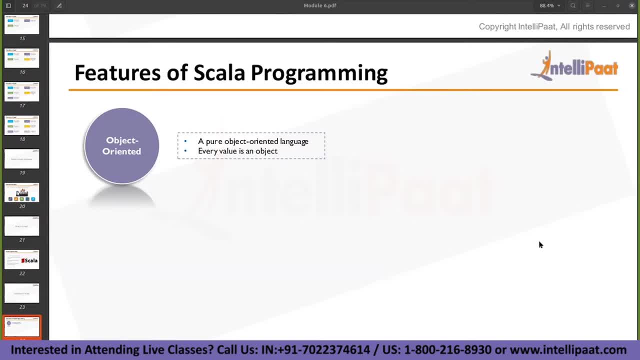 the other concepts of scala. right, you are already familiar with all those object oriented models and all that, right, anyone from python background? yes, no, so we'll. we'll see the features of scala here. so first is object oriented. so what do you mean by object oriented programming model? 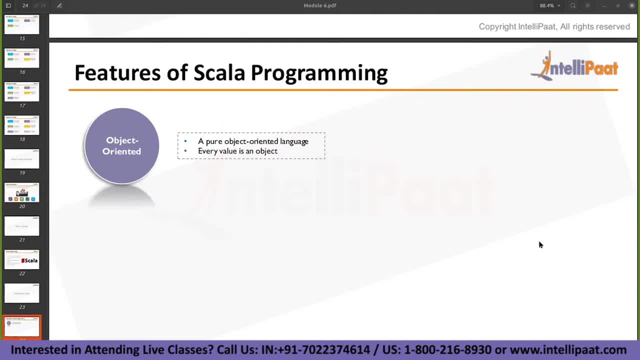 see, all the questions are going to come to you, so you guys are already comfortable or already been into java, so let's, let's keep it interactive, like what? what do you mean by object oriented model in simple terms? what do you mean by object oriented programming model in simple terms? 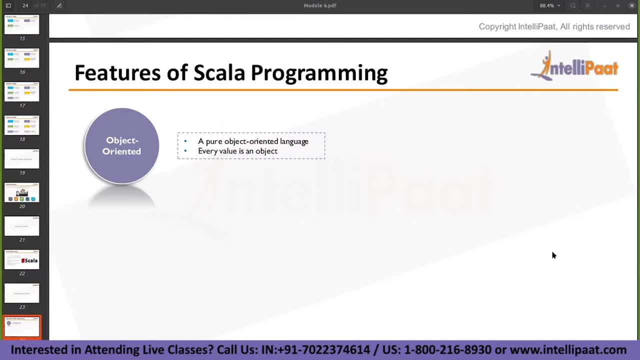 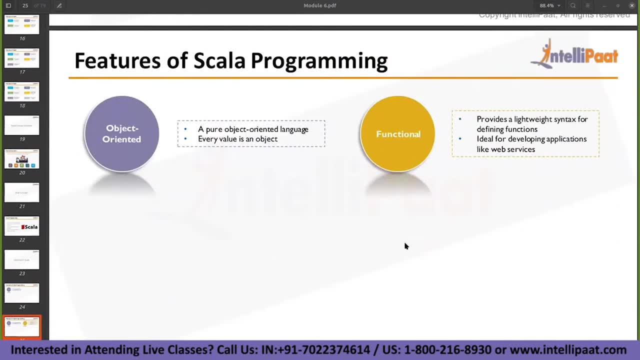 so we'll see what's the main characteristics for an yes, for an item to be called as an object, right, okay, so it is a pure object oriented programming model. and what else? it is also functional. so what does this functional mean? so it's suitable for defining. 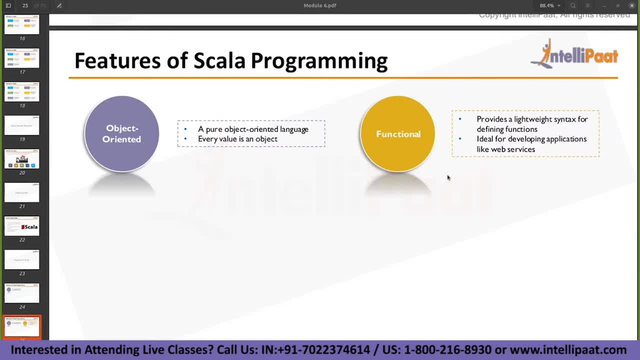 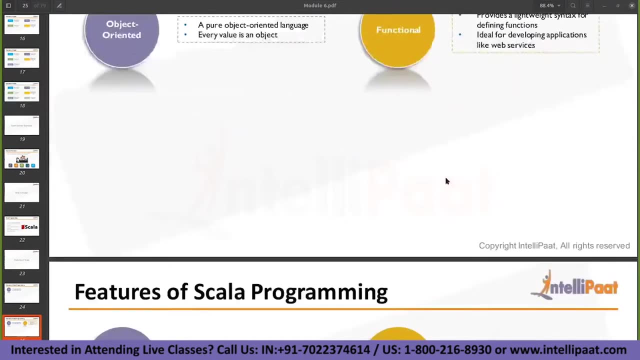 various functions functions. so it's, i mean, compared to java, it's very easy or it's very, um, lightweight. i can say yeah, so as a term itself suggesting so it's very lightweight. uh, syntax for defining different functions and and working with it, and statically typed. what do you mean by statically typed? 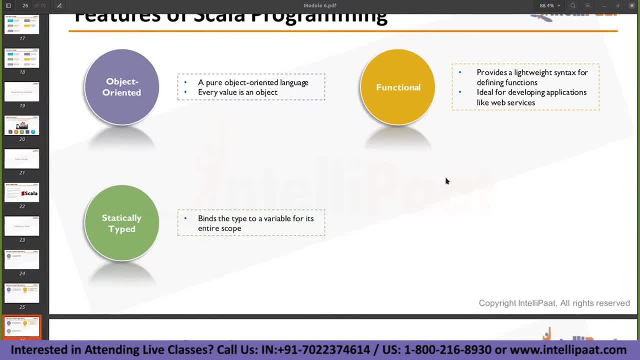 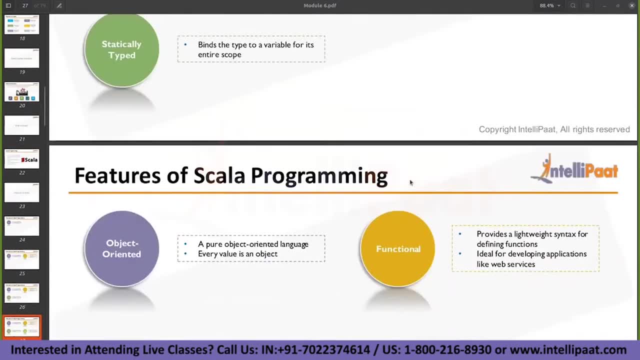 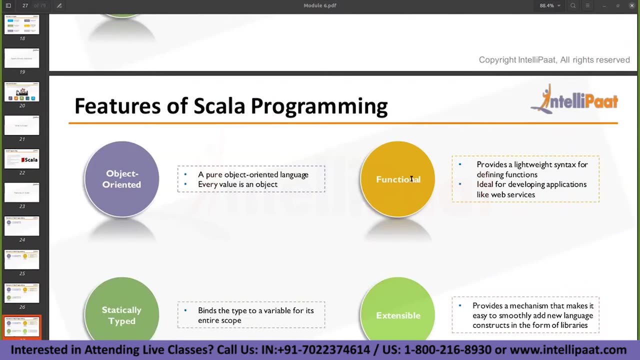 so it's going to bind the type of a variable for its entire scope. so, whatever the data you you have, you you allocate it to some kind of a variable and you're going to work with it. and extensible, so provides a mechanism that makes it easy to smoothly add new language constructs. 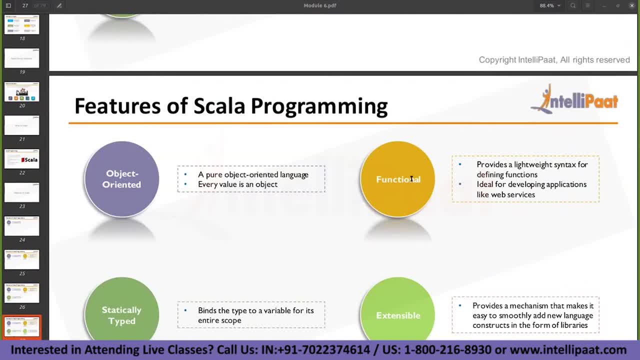 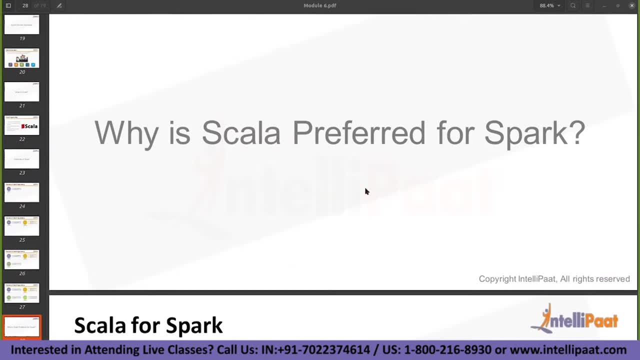 in the form of libraries. so what does this? what are these libraries mean? what do you mean by these libraries? what are the different libraries? can you? can you name one, any simple library that you can that you have worked with earlier? okay, so fine. so why is color preferred for? 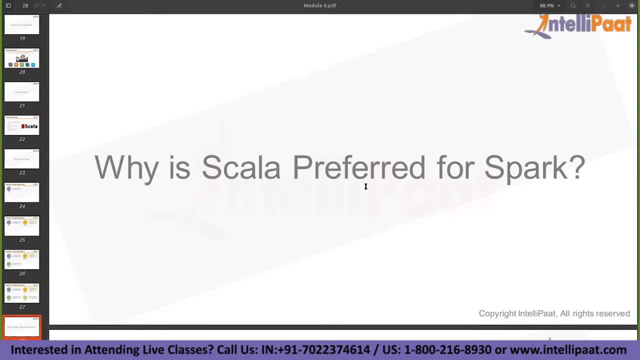 spark can. can someone tell me one simple reason for for, uh, referring scala over python? so i mean, i understand you guys have come from a java background, but in general, why do you think sparks is preferred? scala is preferred for spa, for spark rather than python. so which one is faster? do you think whether python with spark is faster or stella with park? 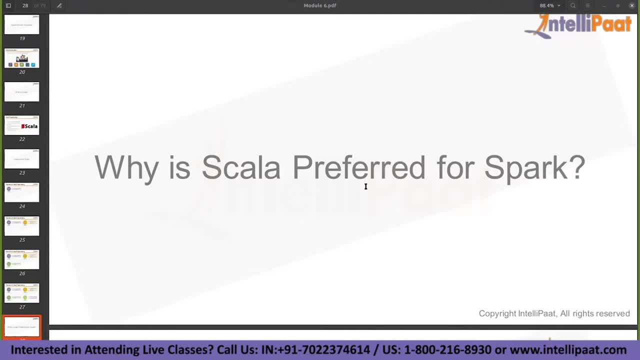 is faster, so spark itself is faster, but which one is is faster in in terms of style and python? yes, any guesses? okay? so why did you say python? yes, because, uh, the programming model of python is designed such a way that it's it's very interactive or it's it's not that complicated. i mean it is. i. 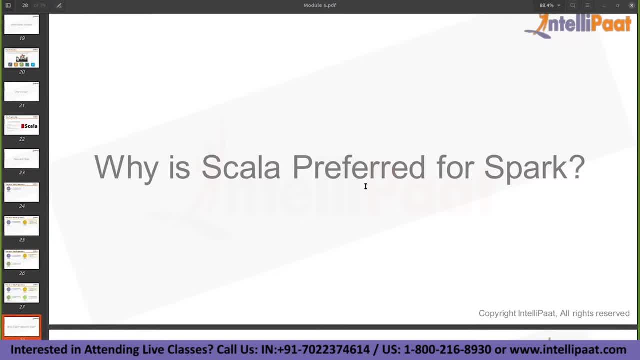 feel complicated, uh, working with scala and uh, because it's it's very close to java. maybe that's the reason i feel kind of a bit complicated. but so, yeah, i agree, uh, python with spark, pi spark is kind of easy to understand, easy to work with, but in terms of performance, a scala is something which 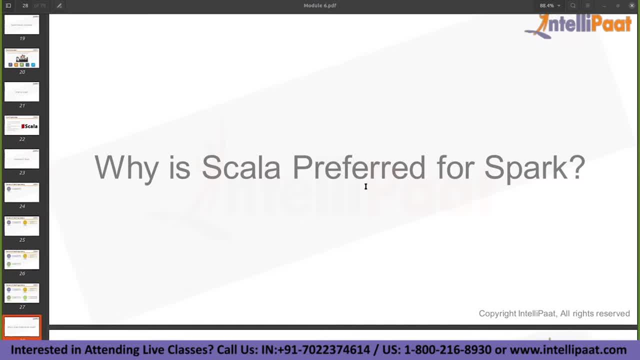 which which gets an edge. okay, so it is something which is better than python spark by spark. the only reason being it is it is uh, uh, running on a jvm. okay, so scala park, scala spark, is running on a jvm and, moreover, if you compare it with the, the program that you write in java, it's almost like. 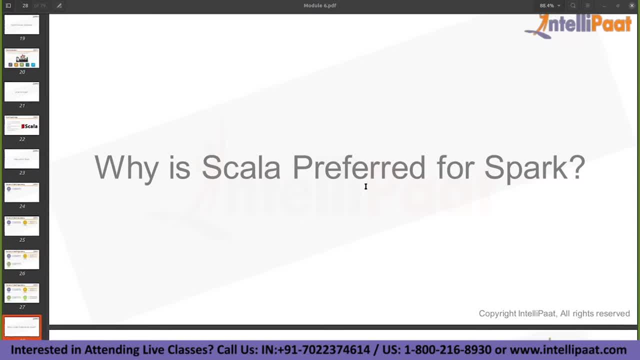 it's almost reducing the um complexity. so, whatever the program you write in java, it's- uh, let's, let's say you have some 20 to 30 lines of program in java, you can, you can simply replace it with one single line of code installer. so there are. there are methods defined, there are very efficient methods. 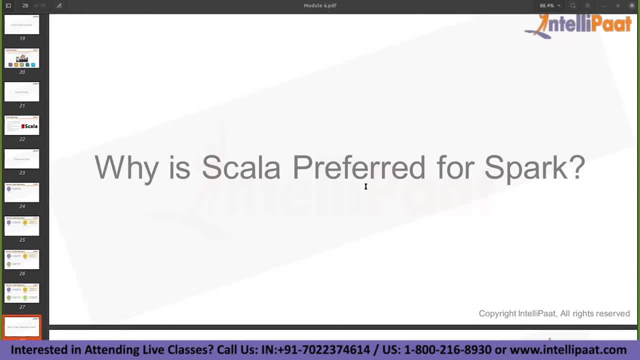 defined and um there is. there is a predefined subset of libraries also available within within scala. the support for these libraries and the um complexity- the reducing complexity of uh complex java code- and the reason that it is working- it is running on a jvm will- will make it. 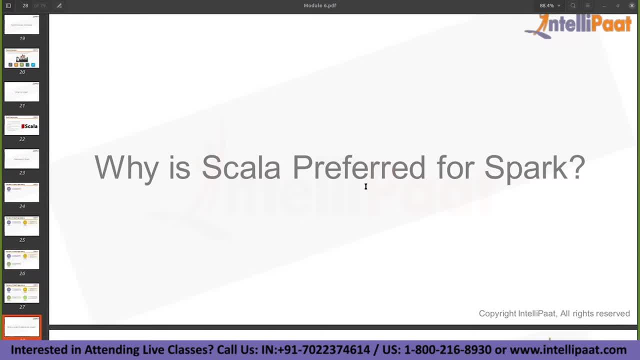 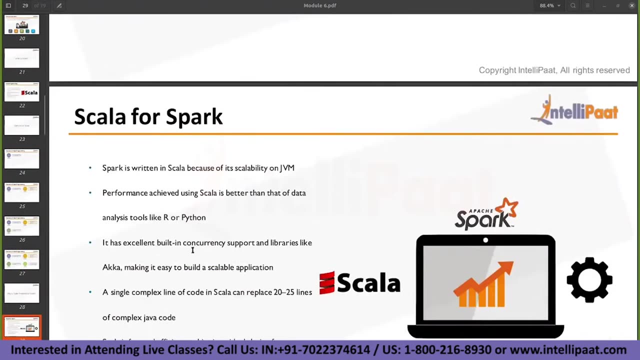 more, more effective. okay, so that is the reason we uh, if, if you have an option to compare, or if you have an option to uh select between scala and python, it's definitely going to be scala because of the performance related advantage. okay, so that is some things we have and uh, the scholar shell. 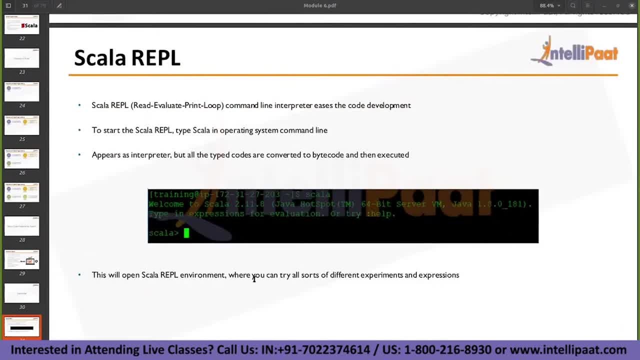 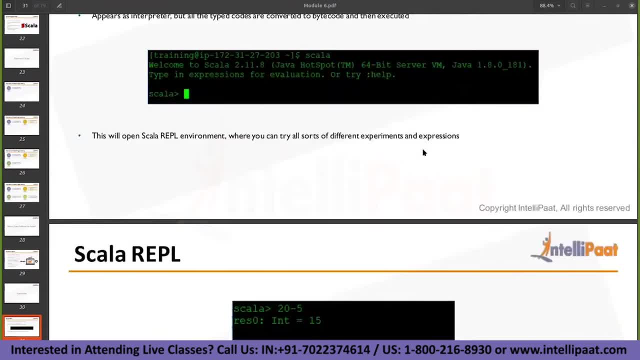 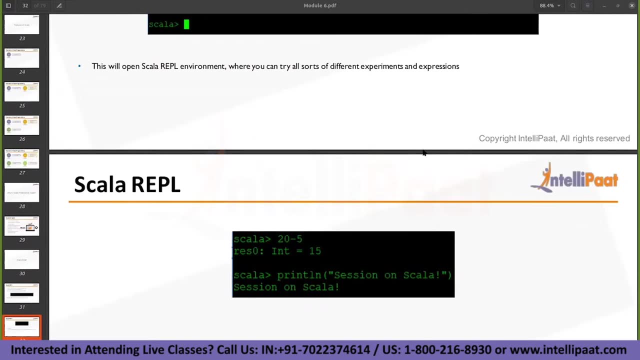 how do we spark? how do we start it? it's. it's, i mean, when you have a scholar alone installed, you just run scholar and it will open a scholar shell. but generally we started using this spark shell. okay, so using spark shell, we will be starting it and that's going to, uh, start a spark environment with a scholar programming. 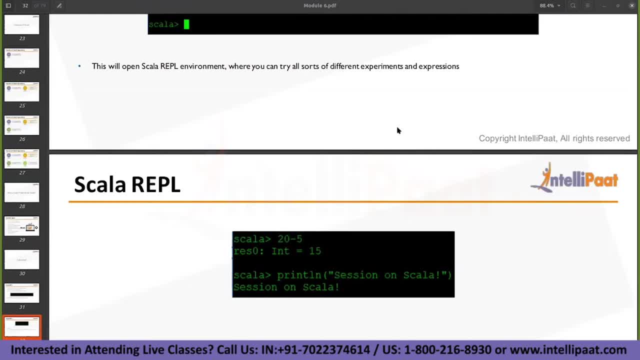 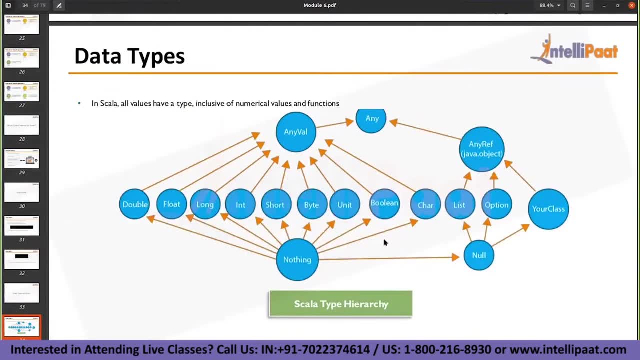 okay, so for for starting pi spark, you will be running pi spark command. for starting scholar spark, you'll be running spark hyphen shell. okay, so the data types: um, you can see, uh, the different data types that it is supporting. okay, so double float. long in short, bite unit. 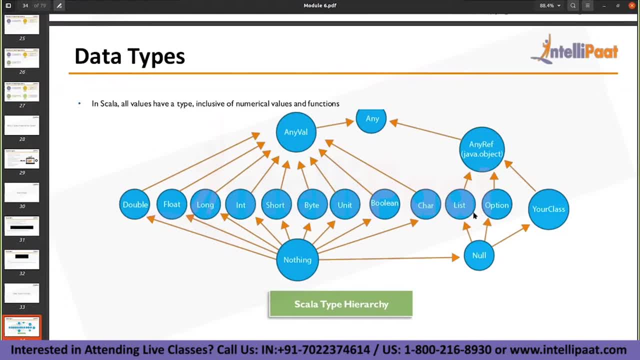 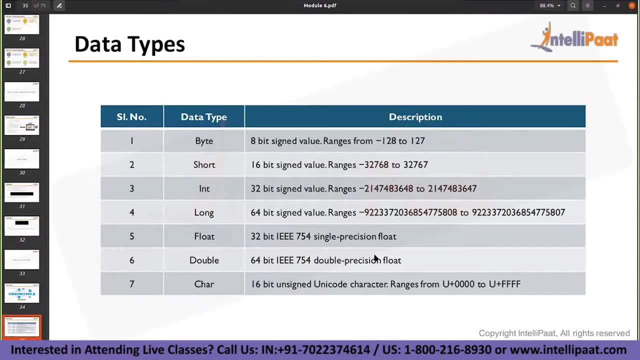 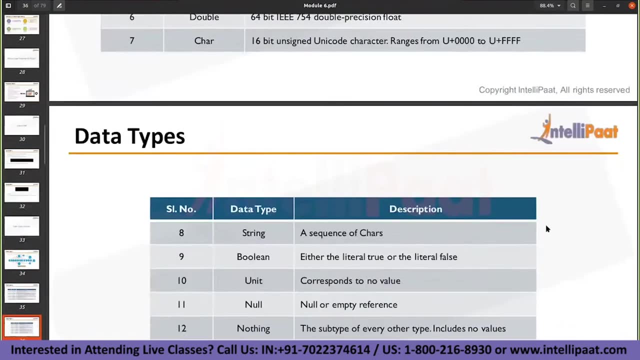 boolean care list option and whatever the null data types you have, okay, and the range, uh, the data data types range. what is the range for each and every data types is listed here, so nothing changes, it's. it's the same uh thing that you're going to see in other programming frameworks. 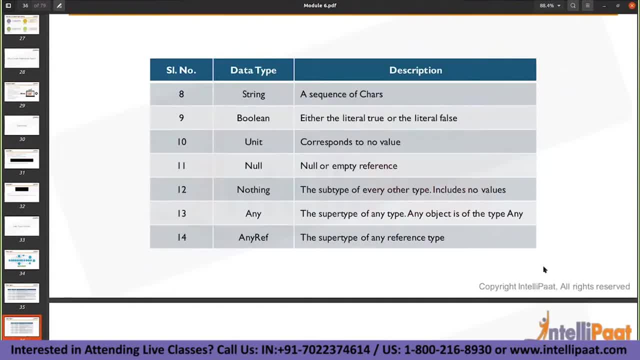 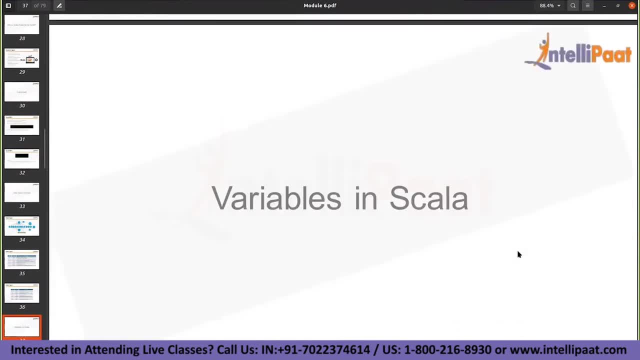 okay, programming models. the string is all that, all that, all that is going to save, all the is going to be the same compared to everything. okay then, uh variables. so what are these variables? you, you allocate some data, you allocate some value to, uh a variable. we, we store that in the 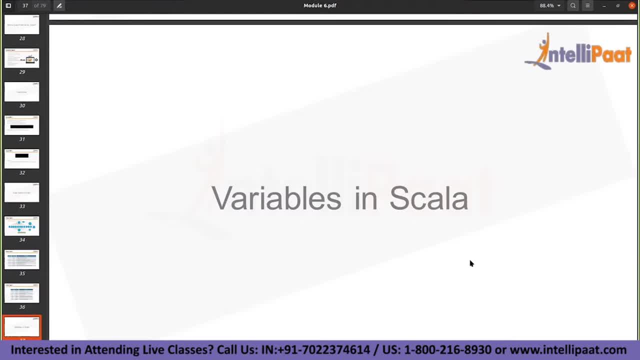 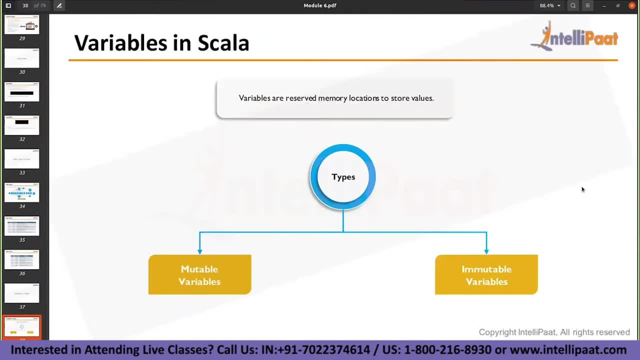 form of a variable. every value is stored in the in the form of a variable, and we have two types of variables available. one are the immutable variables and one is the immutable variables. have you heard about these two anywhere before? so in that case, what is mutable? what is immutable? okay, so where is mutable? val is immutable. is that what you're saying? 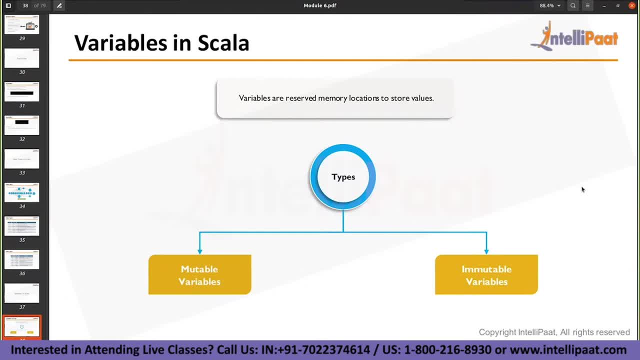 so where is mutable and we can change the value of it. so what if i'm saying where a equals to 5 and then i'll say a equals to 10, is it possible and val a equals to 5? i say and i define and a. 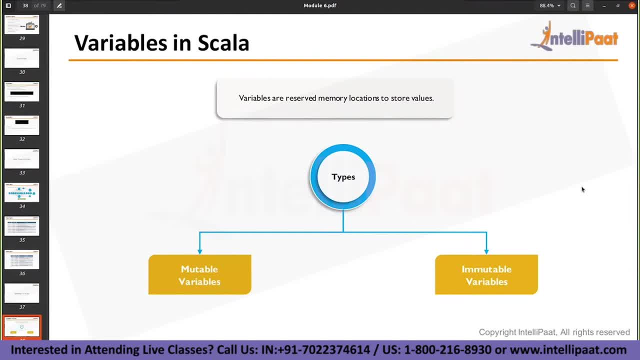 equals to 5. again, is it possible? no, so val a equals to 10 is one statement. then i do val a equals to 5, is it possible? okay, so reassignment of a variable is: is can be done in both the scenarios, but it's something that 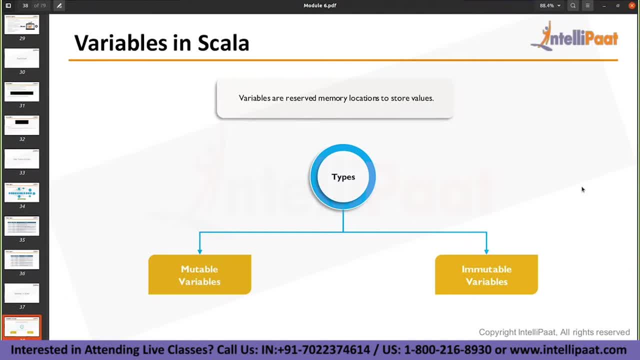 you cannot assign a new value to the existing variable. are we clear with these two concepts: mutable variables, immutable variables? mutables are where mutables are well. mutables cannot be a. mutables can be changed. the value can be reassigned or allocated with a new, new, new value. 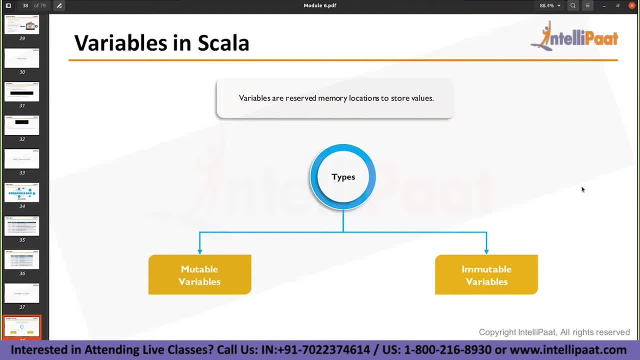 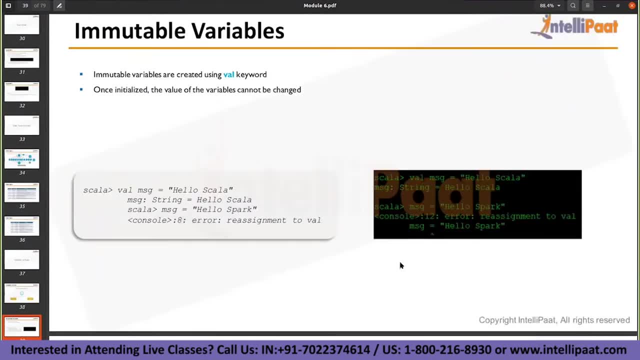 but immutables cannot be assigned to a new value. so you guys are pretty much clear about this mutable and immutable concept. so there is some example also listed here. so that's fine. it's just a string example that we gave now multi-variable assignment. so what does this multi-variable 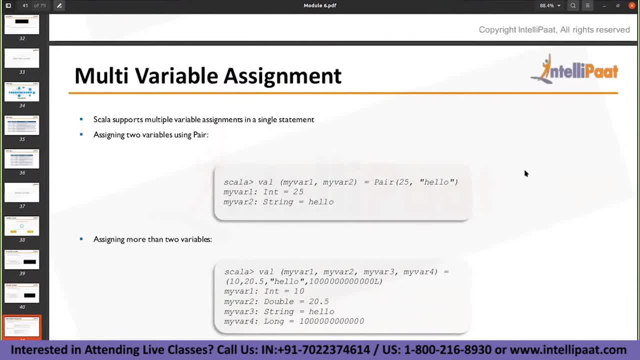 assignment mean. so supports multiple variable assignments in a single statement. so you can assign multiple uh variables in a using a single uh line command. so val multiple variables in a line command. so val my var 1 comma, my var 2 and you. you gave the value as 25 and hello, so there. 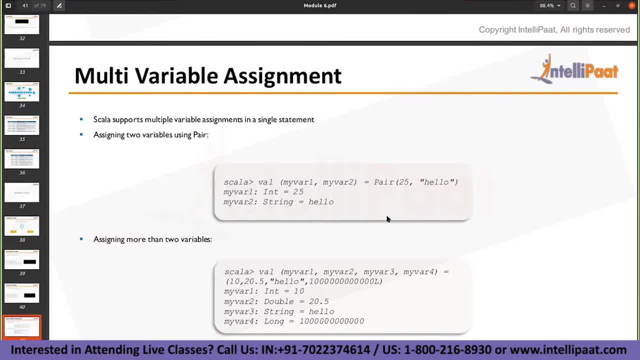 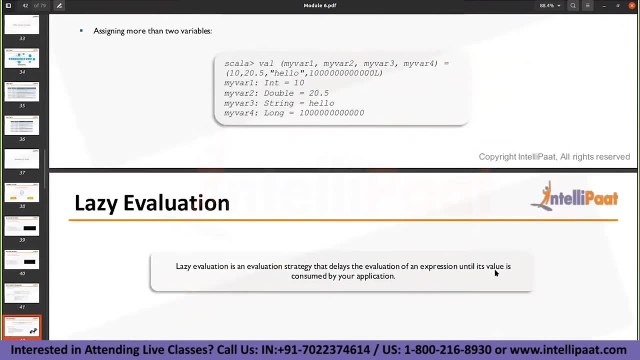 are two values getting assigned using a single assignment statement. okay, so two or more is also possible. my var 1, 2, 3 and 4 you are allocating with so and so values. all these are val variables, immutable variables. okay. now then lazy evaluation. so lazy evaluation is an evaluation strategy that 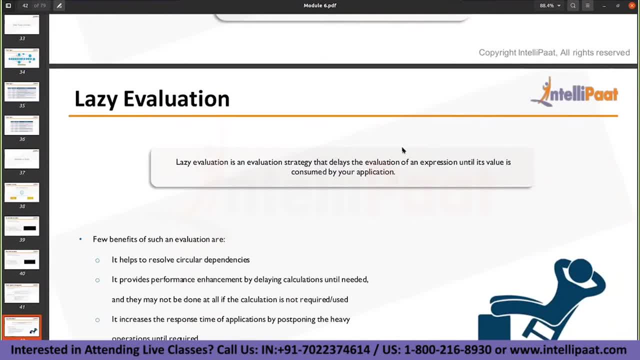 is the evaluation of an expression until its value is consumed by your application. so have you heard about this lazy evaluation concept before? it's one of the most important feature for the spark. so what it actually does is, let's say: i have created a value. okay, i've created. 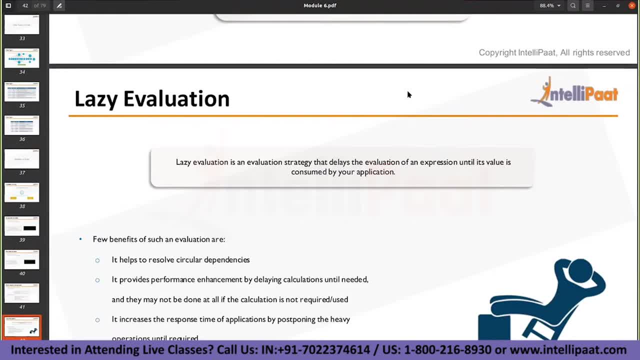 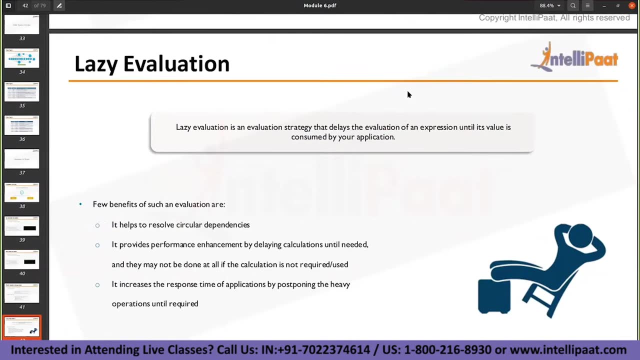 some variable and i've allocated some data to a variable and what example you can take. let's say, okay, so maybe we can take one simple example. so, uh, for example, i'm uh, have you heard about this concept before? do i have to tell you from the scratch? or you guys are aware of this lazy evaluation, not aware of it? okay, so in, in terms, 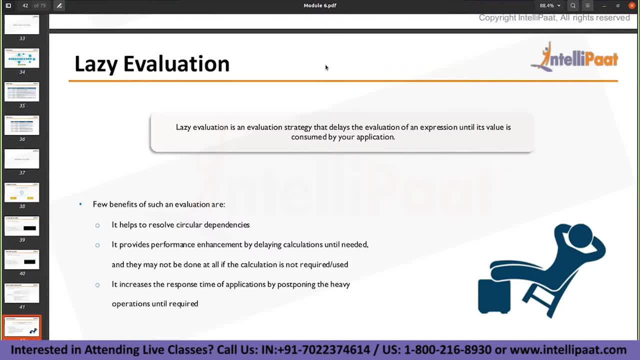 of spark. let's talk about it. see, i have a data in a so-and-so file, okay, so home training, some hdfs location. i have a data file, okay, and you allocated that data, you, you read that data using mechanism and you located that into some variable. okay, some, some, some whatever, some variable or. 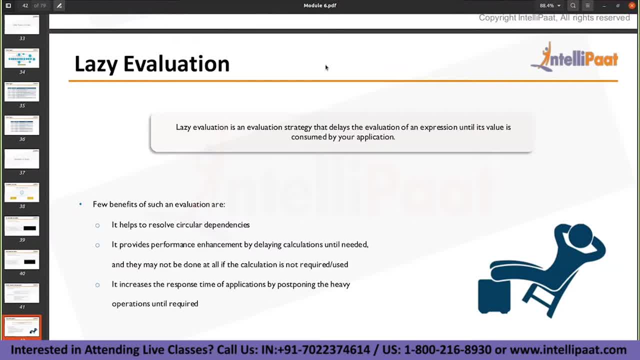 where- variable or value- you allocated some data to it. so now, when you are doing this allocation, it actually does not matter whether the data file is available in hdfs or not. see this. spark or scalar is not going to look for the data in hdfs at the time of the value assignment, only. 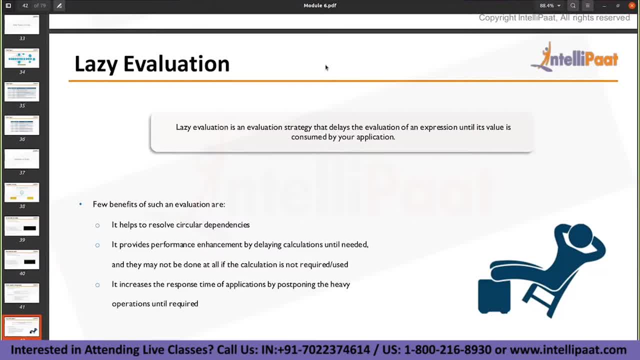 when you are actually using it. for example, in the next line i'm doing print off, whatever the variable. so only then you are, you are trying to look for the data file and it's going to try reading the data file and try allocating the data file to this particular variable. so in the first statement, when 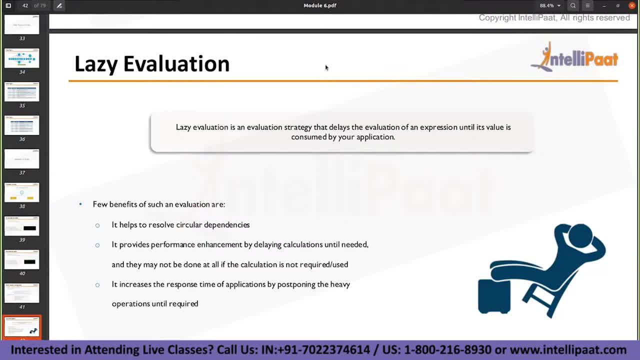 i actually assign the data, assign the data to this variable. it is not even looking for whether the data is available in hdfs or not. it is just one single statement that it is going to execute. it is not taking care of the assignment of the data to this variable. because now 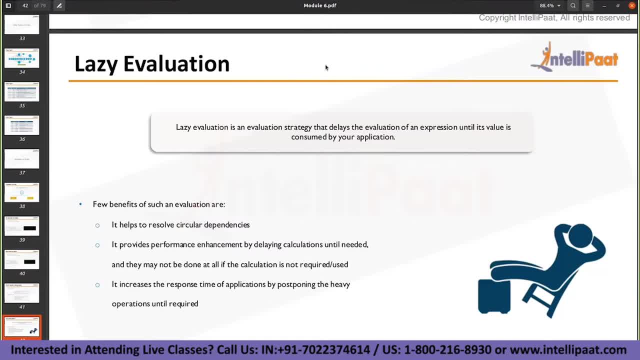 now. at this moment, the variable is still empty. okay, so spark or scala has not spent time today. go to the hdfs, get that data and allocate the data to this particular variable. when is it actually allocating it, when you are actually using it? next statement: what did i do? i have written print variable name, so that's when it's going to go to the hdfs location. 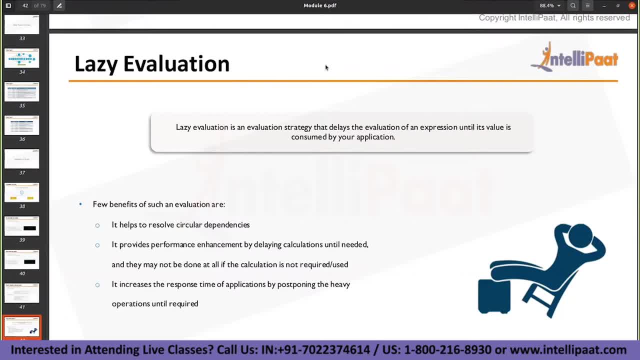 check whether the data file is available and then assign the data to that particular variable and then print that data in the variable getting it. so what is the difference? is in the first statement. it actually does not matter whether the data is available or not. okay, so if the data file is not, 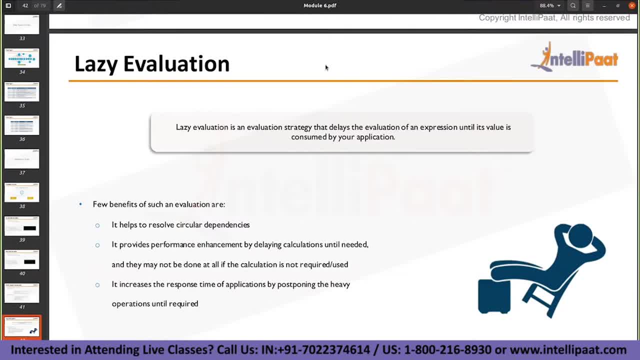 available at all. you gave that var statement allocation statement. it won't give you an error in the print statement when you're actually using it. that's when you'll be getting an error message getting it. so that is a lazy evaluation. you're evaluating it is lazily okay, you're not doing it. 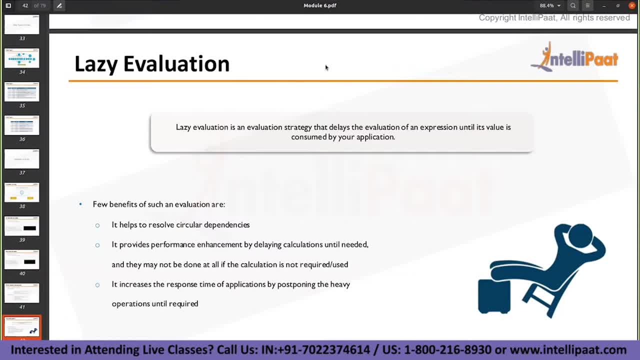 in the first place, but when you're actually executing them, when you're actually performing some kind of an operation on top of that variable or some type of an val or a var variable, that's identifying, it's actually evaluating the data. that is what we call it as a lazy evaluation. so 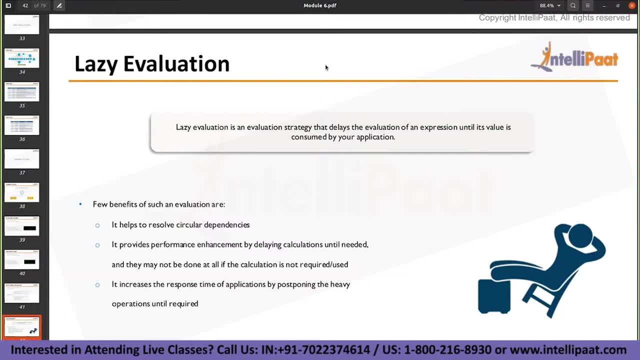 the same concept is going to get applied in spark as well, in spark data frames on in spark rdd creations. when you, when you assign some data to it, it will not allocate any memory or it will not allocate any ram to to perform that activity. it is not going to execute at that time, only when it. 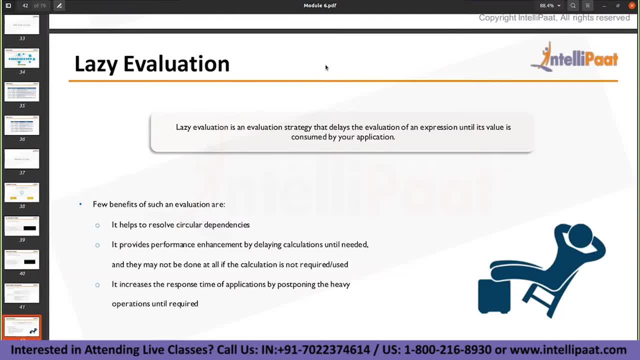 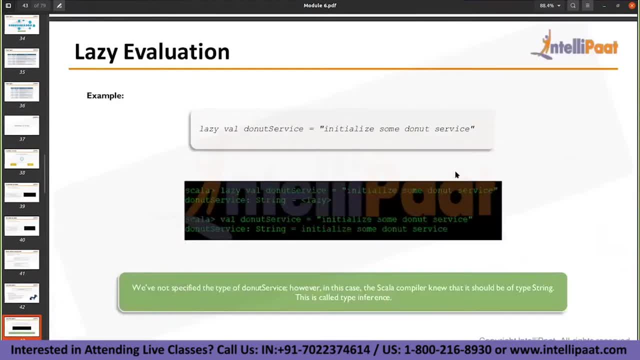 is being used by some analytical process, for by some transformation. that's when it is going to be used to try and execute it. so that is the most important factor of your lazy evaluation. so what is the advantage that we get? so it helps to resolve the circular dependencies. it provides. 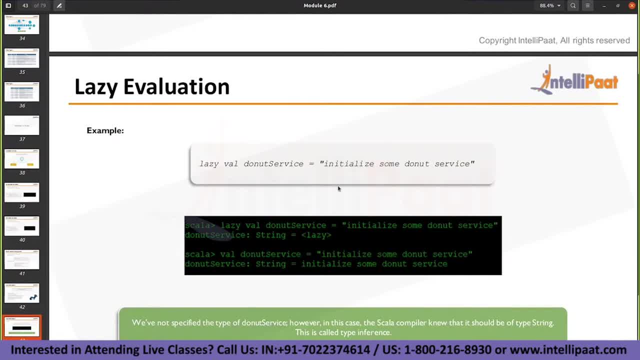 performance enhancement. sorry, yeah, no. okay. so there is one example defined lazy val donut service. uh, there is some data allocated to it and, uh, this is your uh value and when you have actually printing it, val donut service equals to this one. it is allocating some data to it. 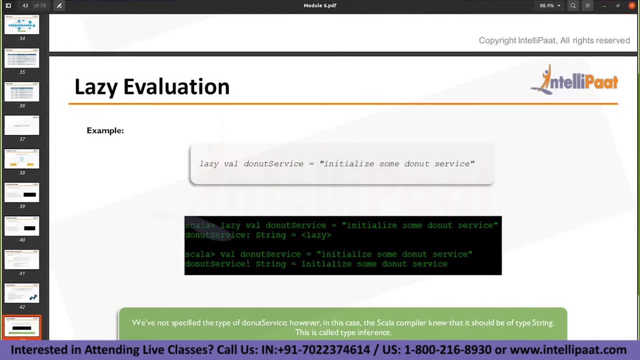 okay, so that's the difference between a lazy allocation and a normal allocation of the data. okay, so in scala you have this lazy allocation, but in in spark or in, if you get into the spark concept, software, every variable for that matter is, is gonna, is gonna be a lazy allocation only. so 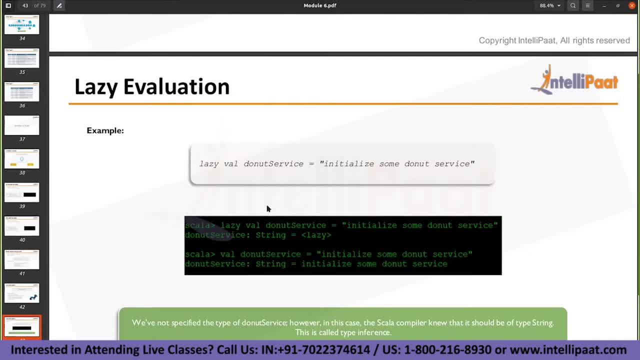 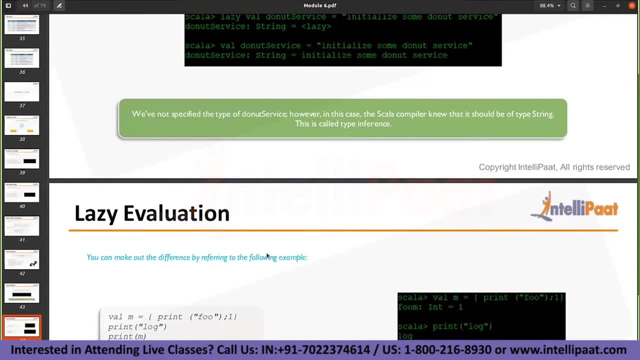 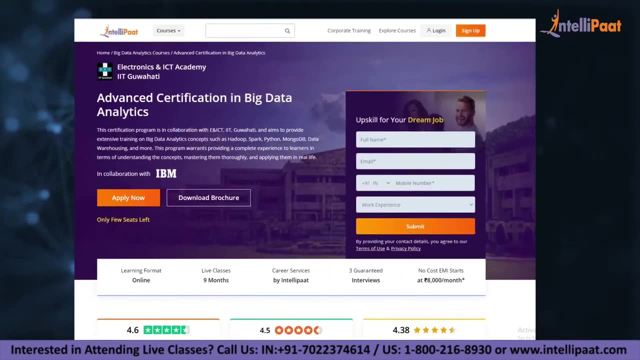 no matter what the data, when you allocate it, it's not gonna get executed. only when you um start using it for some kind of an operation, it's going to allocate, it's going to execute that particular data. okay, just a quick info, guys. if you want to make a career in big data, then intellipad provides an. 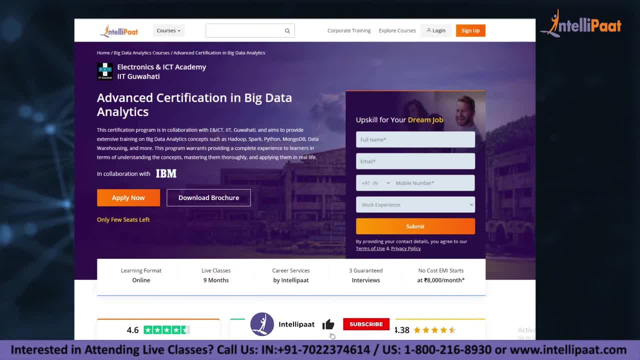 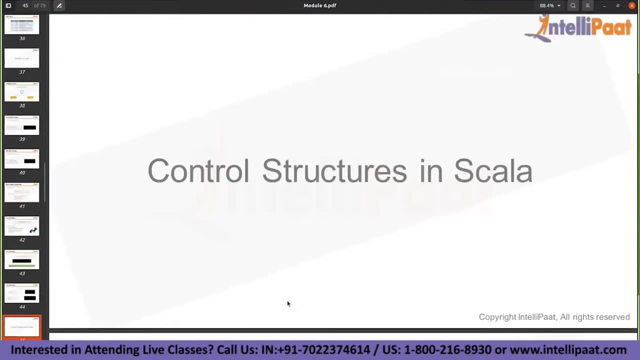 advanced certification in big data analytics by enict council iit guwahati. it is taught by iit professors and industry experts with more than 10 years of experience. this course is designed to upskill and land your dream job. now let's continue with the session. so there are some. 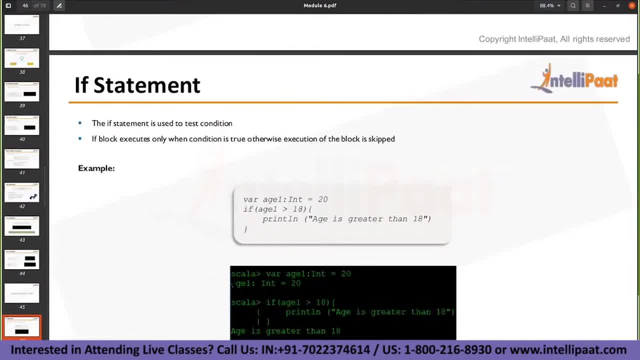 control structures. you must have thought about them. what are the control structures available? control statements: there is one if statement. what is it going to do? it's going to validate for a specific condition. if the condition is failed, you execute whatever. the following statements: if it is, if the condition is successful, it will execute the. 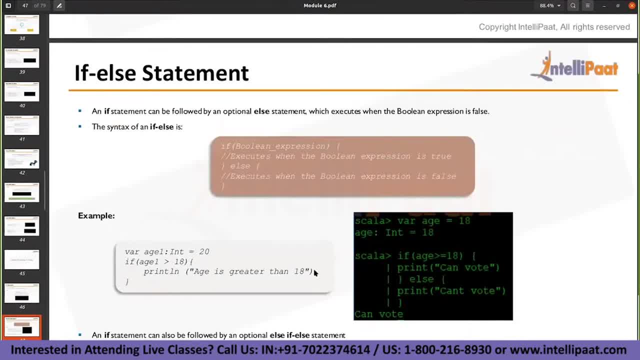 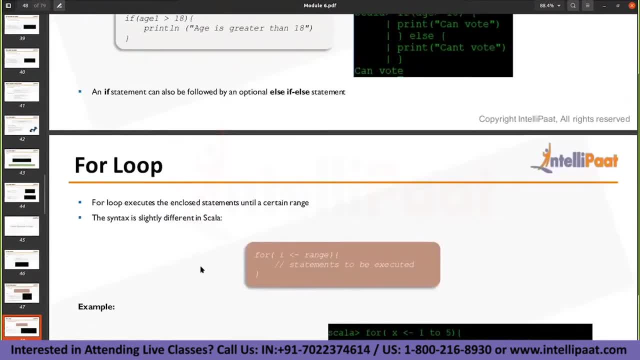 following statements: if it is failed, there is an else component which will be getting executed. so you must be aware of all these basic concepts anyways. and there is per loop for a specific range. it. it keeps executing, whatever the statements that are, uh, listed here. uh, you will be giving a range in the beginning for per loop and all the statements will execute it first. 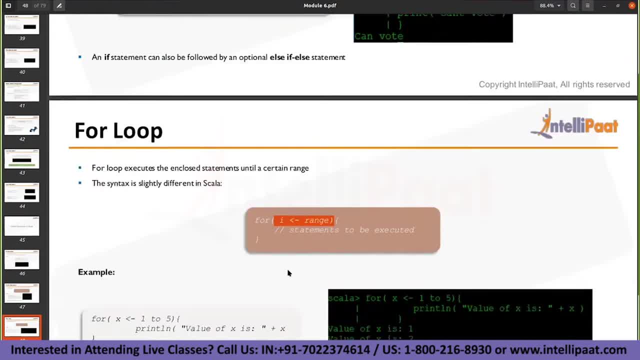 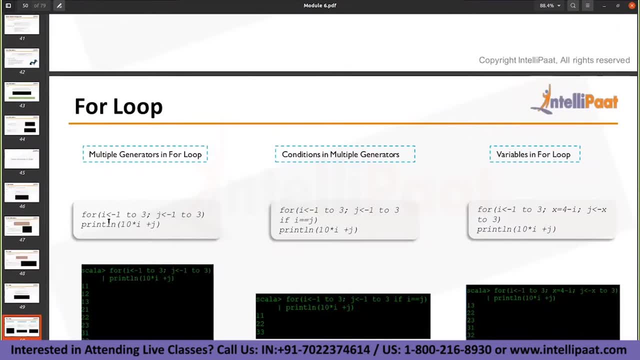 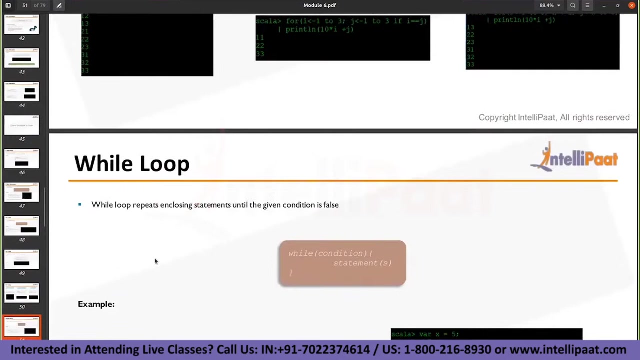 so, and so range right and then: okay, so there is multiple generators, there's conditions in multiple generators, variables in for loop, so there are all different conditions. there are multiple conditions listed here, right, and conditions in multiple generators. this is how you can define. there is and this is the variables in your for loop. so here there is a while loop, so the while loop is: 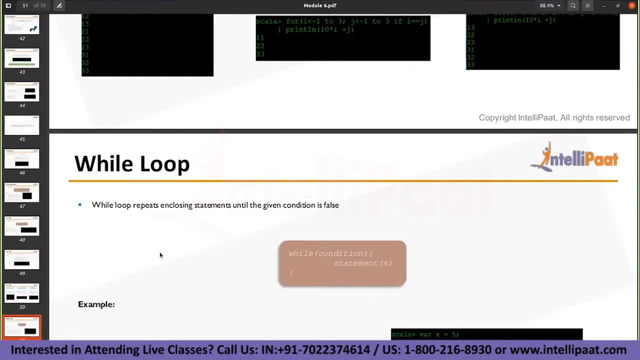 difference. the difference isn't like your condition will will will get executed, whatever. the statements will get executed in the form of a loop until the conditions get failed. okay, so it will keep. it will keep checking for this particular condition. until this condition fails it, it executes this set of statements. okay, so very, very generic and there is something called as a do, while 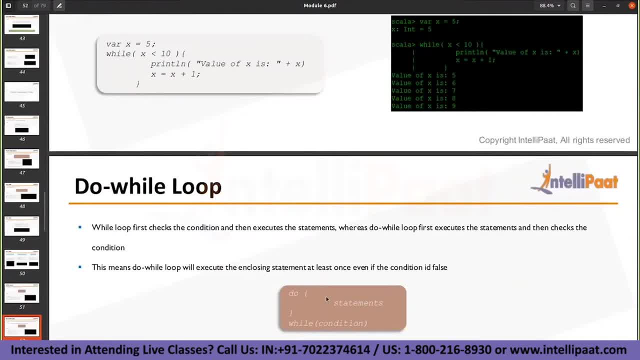 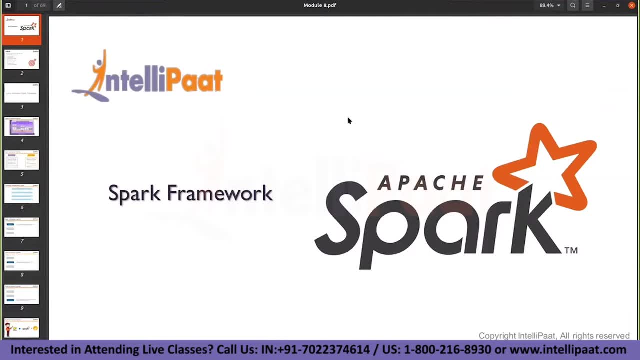 so the difference between while and a do while is the do while will first execute the statement and look for the condition, whereas a while will check for the condition and then execute the statement. so that's all right. so in in Scala, we have just tried to understand what this framework is. what are 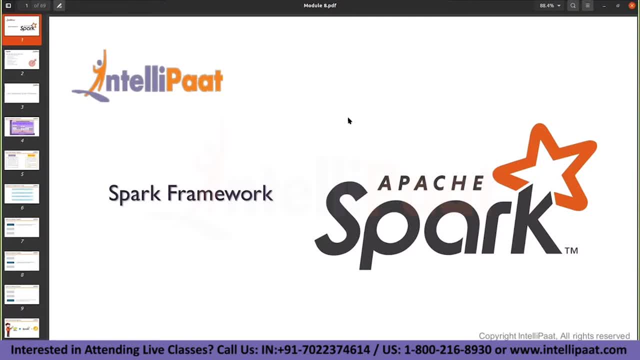 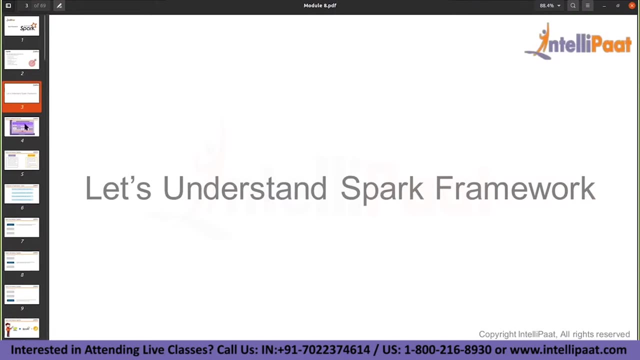 the different control statements are and see. firstly, we need to understand what's the core concepts of Spark, how Scala can be used to interact with your Spark framework. okay, so let's dig a deep, a little deep, into what this Spark framework is all about. what is the architecture? what are its? 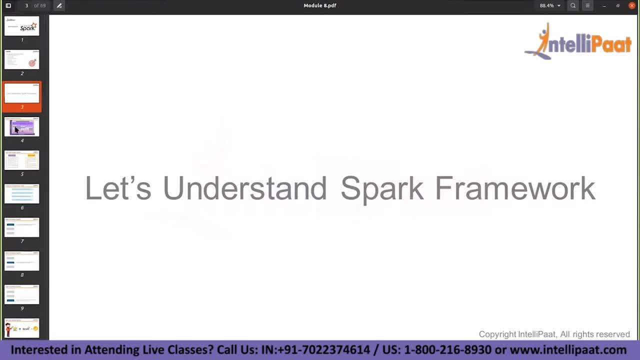 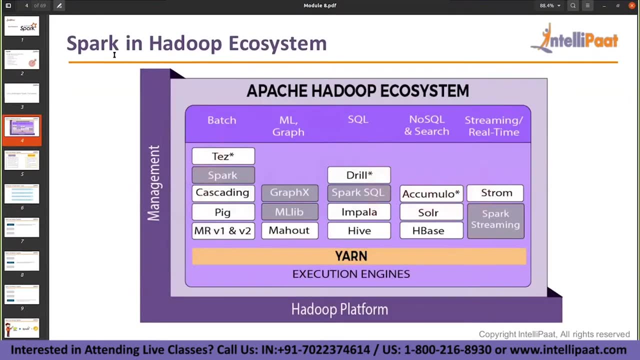 different components. so I've just tried to see what are the features of Spark, right? what are the different advantages that we get. but let's also get into some understanding of architectures, right? so Spark in Hadoop ecosystem, so here in Apache, Hadoop ecosystem. these are the components. 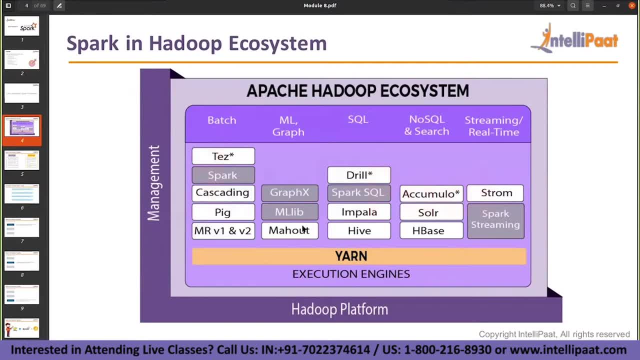 that we already have right. so the ones which are grayed out are something related to Spark, so forget about it. so, Hadoop platform: we know there is a yarn execution, a yarn processing component framework that is available on. under that you have this HDFS location, HDFS storage. on top of these there are different tools allocated. 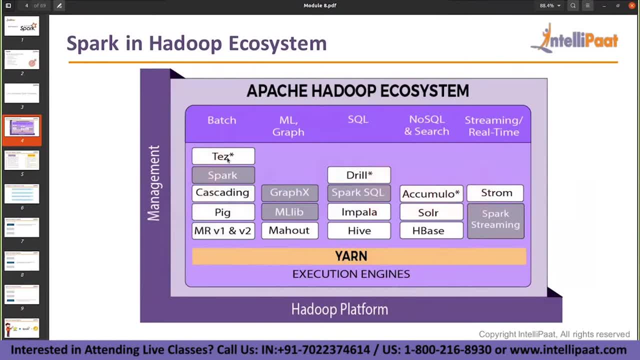 for it. so right, this is MapReduce version 1. version 2, Pig, Taze and Mahout, Impala, Hive Drill and HBase and Storm. this is not Strom, this is Storm. okay, so for batch processing we have Pig and MapReduce version 1 and Mahout and HBase and Storm. this is not Strom, this is Storm. okay, so for 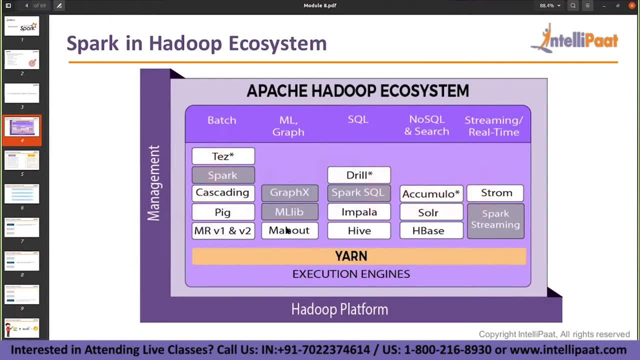 batch processing. we have Pig and MapReduce version 2 and for machine learning we have Mahout. no one- I mean very hardly we use this Mahout related things- SQL: you have Hive. we have seen how to use Hive or what what Hive does, and there is also something called as Impala which is almost similar. 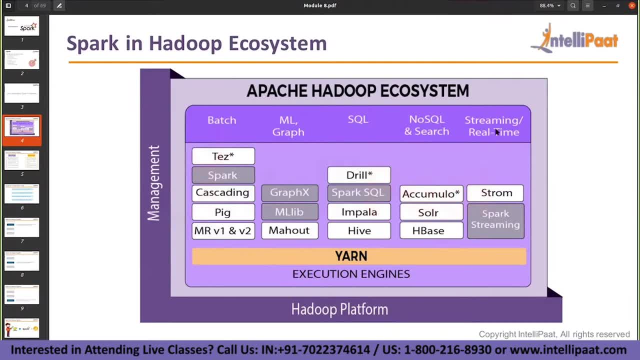 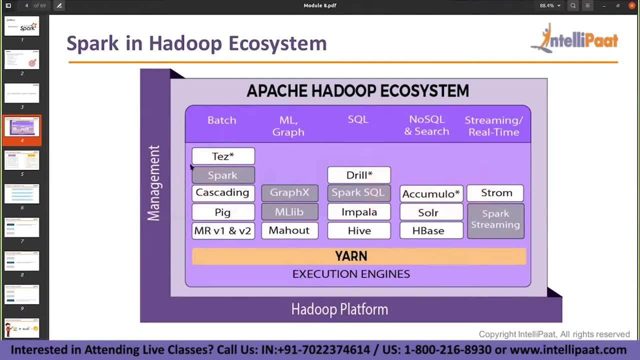 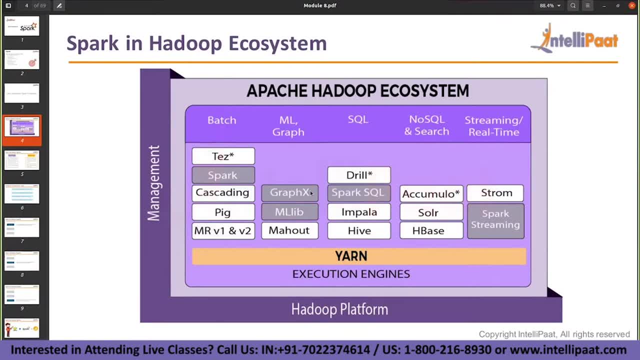 in Spark using it right. so some component in Spark helping it. so for batch processing, your core Spark framework itself is going to help you. for machine learning, you have graphics and machine learning libraries of component and for SQL, you have Spark SQL. for streaming, you have Spark streaming. so there is no component for NoSQL way of handling in Spark. okay, so apart from that, it 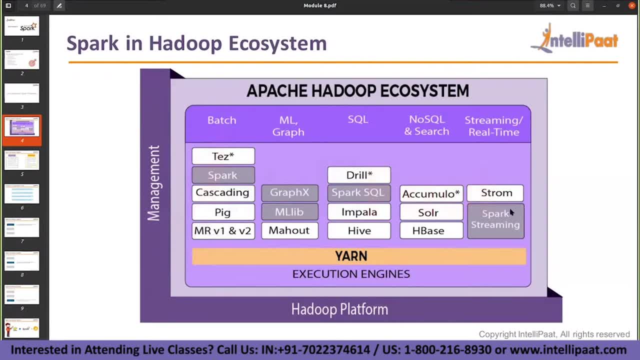 was almost handling all the other modules. it, it all. it almost got its existence in all the other modules of your Hadoop ecosystem. so for every tool, or for almost like for every tool in the Hadoop ecosystem, you have got some alternative in this Spark framework. that's what it, that's what we mean. 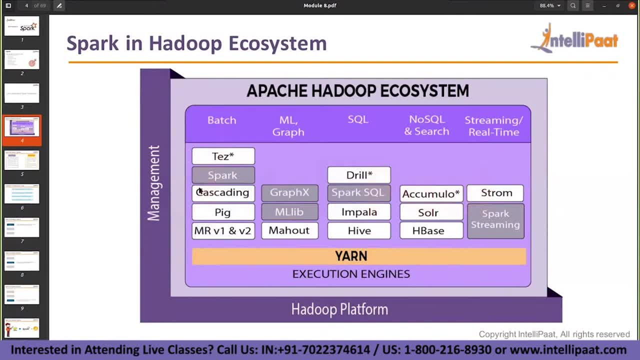 to say: okay, so for any kind of a data handling, you have some kind of a module, some kind of a framework inside your Spark component. Okay, so that's the difference. that is why Spark has got its importance, like it tried to. it's almost overcoming or it's almost replacing Hadoop in terms of data processing or whatever. 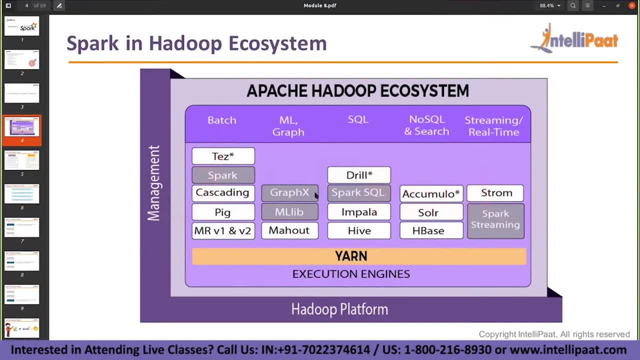 right. so there are many systems there are in in real-time systems like, at least if you look at my, my particular project. so it does not have Hadoop at all. so Spark has been built on its own cluster. we have a specific cluster built on top of it and Spark is running individually. there is no Hadoop at the back end. 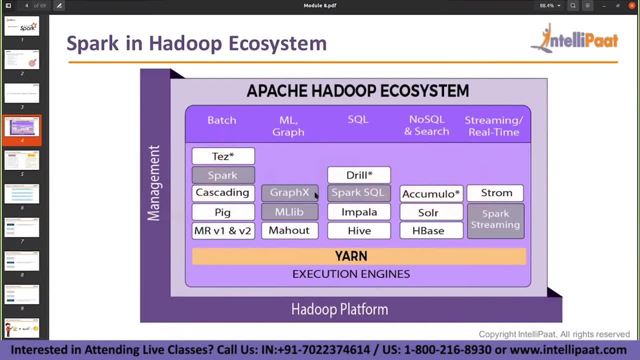 so we don't need Hadoop, at least right, so we don't need Hadoop components or whatever it is. so HDFS and all that, MapReduce and YAN and all that can come. I mean HDFS. you have a better storage mechanism, you have the cloud storage anyways. now, right, so you don't need a HDFS component. so 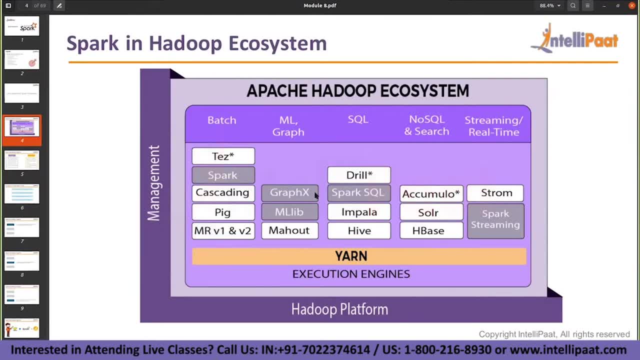 everything, all the all the storages are now on hosted on cloud. so there is no point in having an HDFS storage here. so there is no reason why I'm saying that. so just to make sure everyone knows: for your Hadoop ecosystem to exist, for Spark to run, 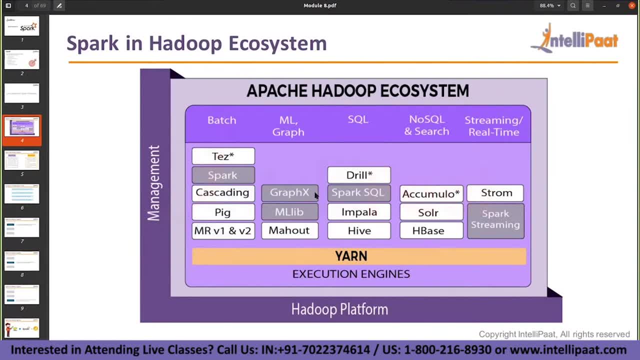 It can also run independently, And there is also something called as Databricks, which is giving you a proper Spark cluster creation. So have you heard about it, Databricks? Have you heard about it, Databricks? So it's a cloud-based Spark framework. 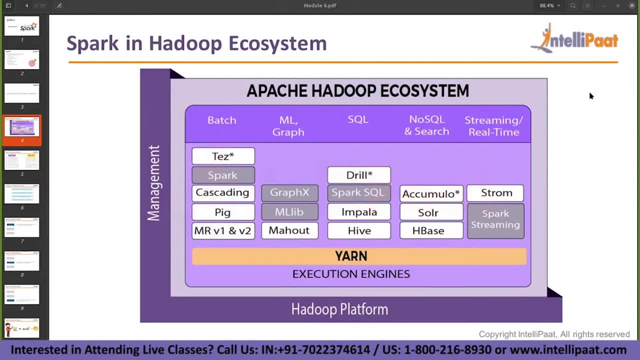 It's going to give you access to the Spark clusters. It's going to create the clusters by itself and it will just give you access. You just have to configure. you just have to let the system know that what configuration you would need, how many clusters you would need. 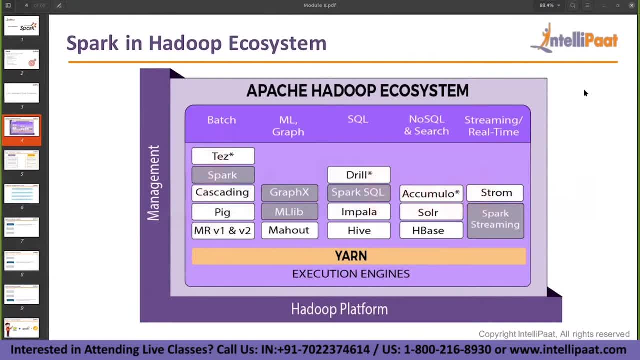 what is the version of Spark and what is the version of Python and Scala. So that's going to create a cluster for you and it's going to give you so all your applications can be hosted on top of it. So it's a paid version. again, it's a paid company. 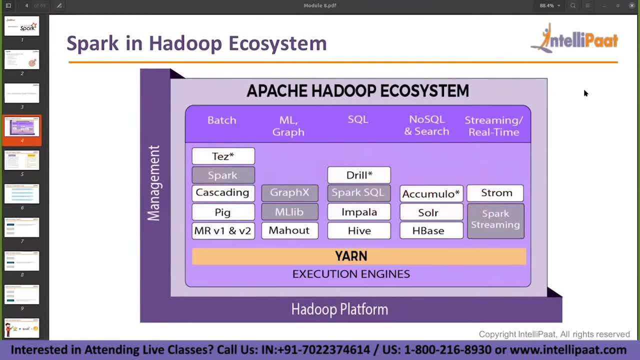 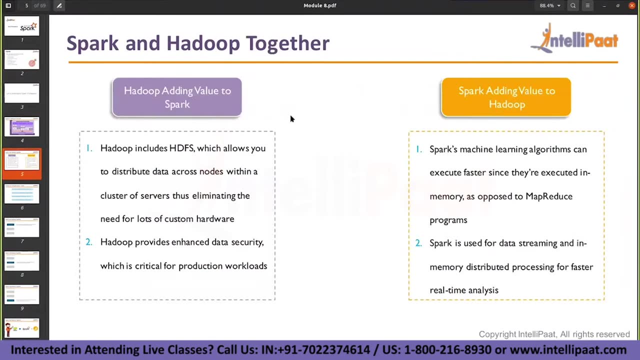 So that's one of the way of working with the Spark ecosystems. So different again, different scenarios, different use cases there are for your Spark applications to run, And how Hadoop is helping Spark or how Spark is helping your Hadoop ecosystem. 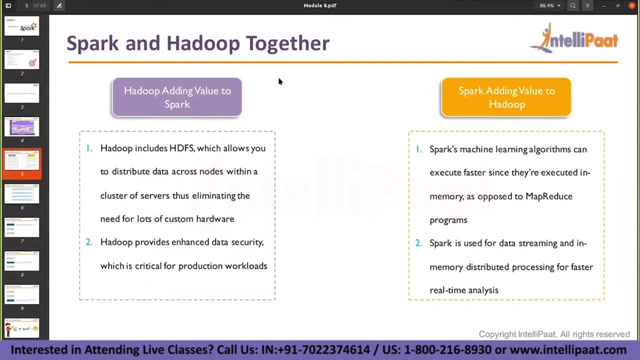 So there are two scenarios can be considered: Spark and Hadoop together, So Hadoop adding value to Spark. So how Hadoop is actually giving some advantage to this Spark. So Hadoop includes HDFS, which allows you to distribute data across nodes. 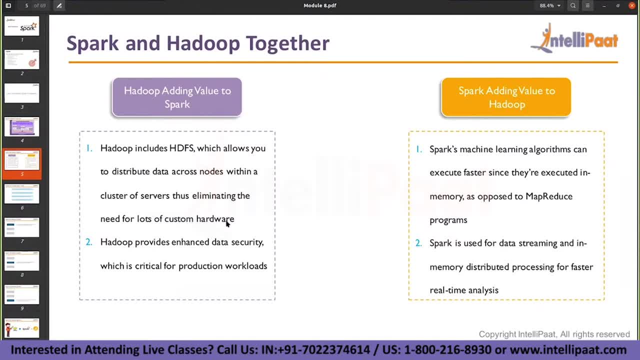 within a cluster of servers, thus eliminating the need of lots of custom hardware. Hadoop provides enhanced data security, which is critical for production workloads. So when you want to run Hadoop and Spark together how both are helping each other. 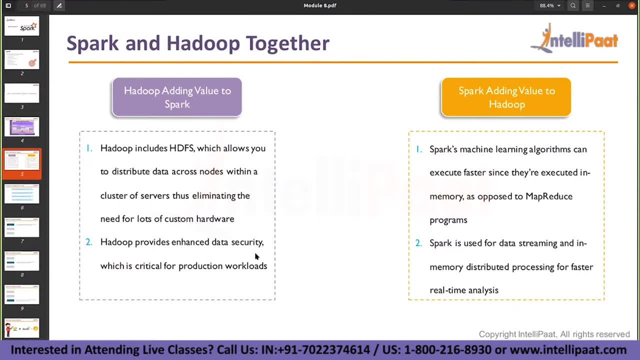 So Hadoop is helping it by providing a better storage mechanism- HDFS, for distributed data storages and also with respect to the security. So it's not that Hadoop alone is gonna provide these kinds of features, but there are other storage mechanisms also. 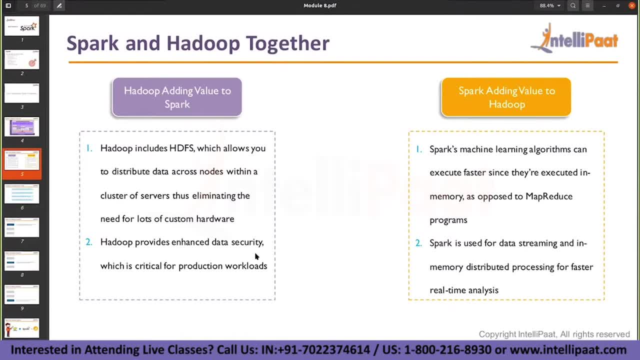 which are pretty much doing the same thing, But as we are working Hadoop and Spark together, this is the advantage we get from Hadoop to your Spark framework And how Spark is adding value to the Hadoop. So, whatever the machine learning algorithms that we have, 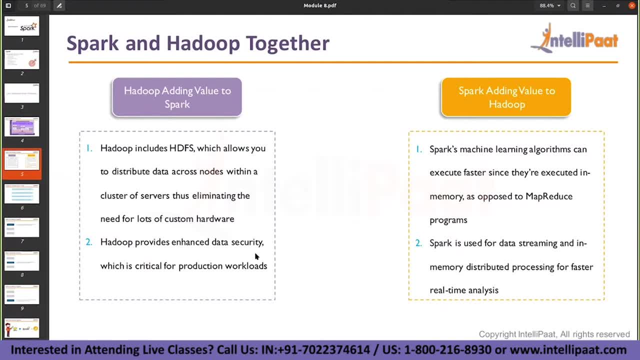 they can execute faster than the MapReduce programs, or any particular programs can execute faster with the in-memory feature of your Spark framework as compared to the MapReduce framework. Okay, So Spark is used for data streaming and in-memory distributed processing for faster real-time analytics. 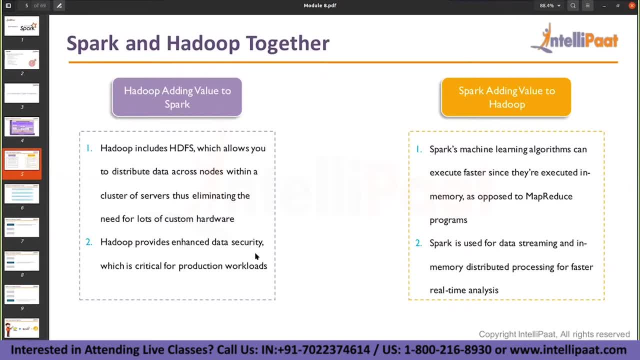 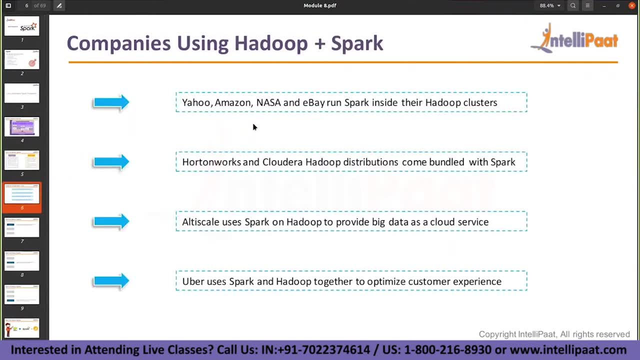 and, moreover, for the real-time data processing also. we have been using it for Some of the components. Then the companies that are using Hadoop and Spark together. there are Yahoo, Amazon, NASA, some of the examples, okay, Uber, Altiscale. 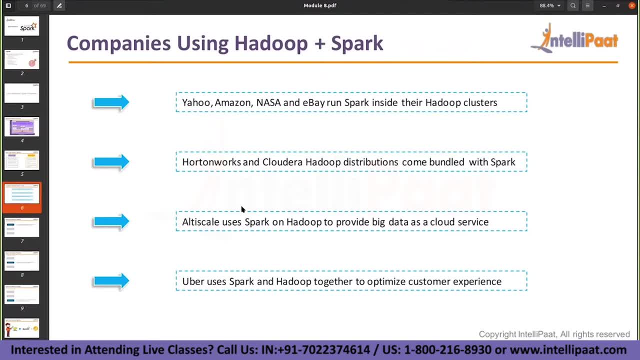 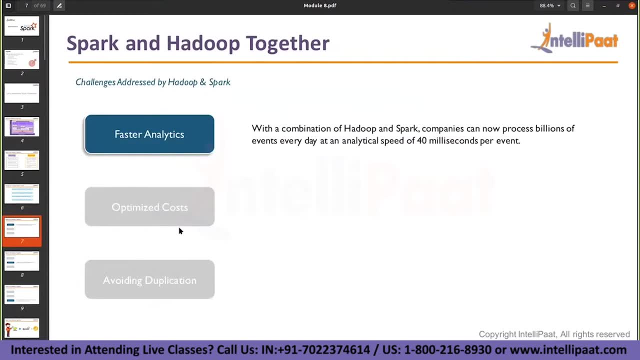 how they're building both Hadoop and Spark applications together and they're leveraging the use cases of both Hadoop and Spark. some of the examples And what is the advantage we get with Spark and Hadoop together is using faster analytics and optimized cost. 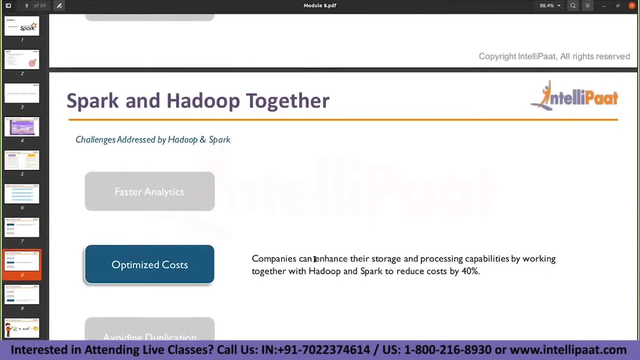 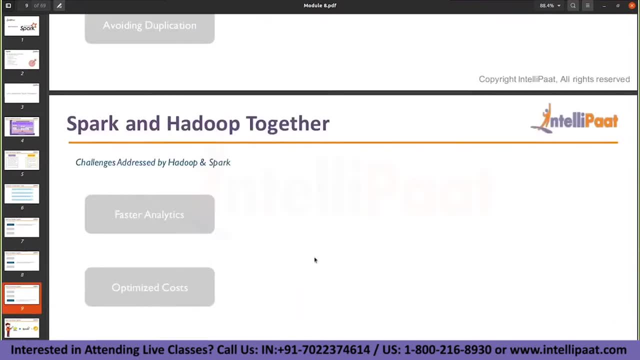 So how do we get this optimized cost? Because of this HDFS cluster, because it has got its better storage mechanism. HDFS has got its better storage mechanism in terms of building the clusters, the custom clusters, which is built on top of the commodity hardware. 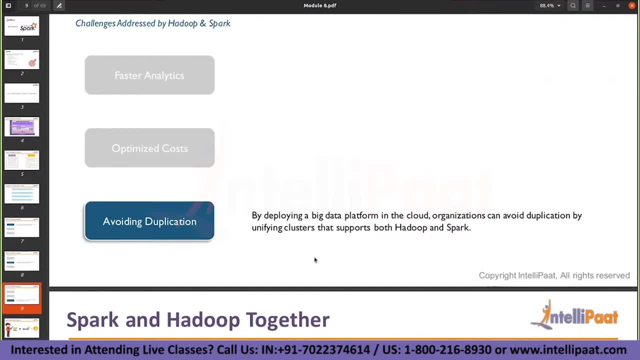 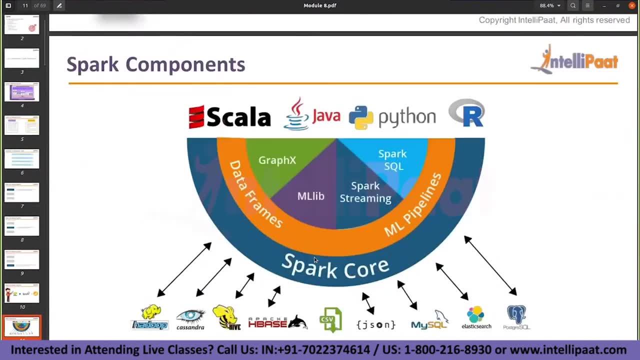 and avoiding the duplication, how HDFS can remove all the duplicates using your Spark programs. Okay, And then Spark components. it has a Spark core, it has this data frame, concepts or machine learning pipelines, and it can interact with any of these programming models. 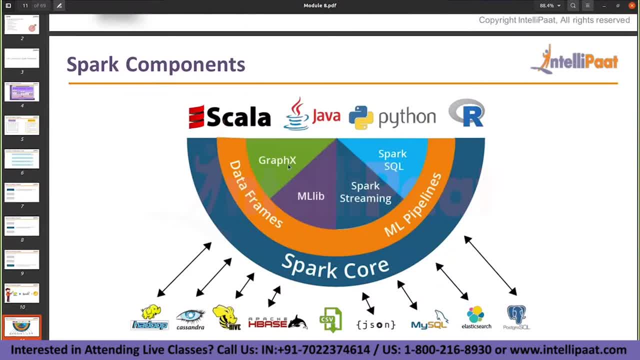 Scala, Java, Python and R, and the modules which are coming along with it will be Spark, Streaming, Spark, SQL, Machine Learning and Graphics. We've already seen how these modules are built and the external systems, how we can interact with each other. 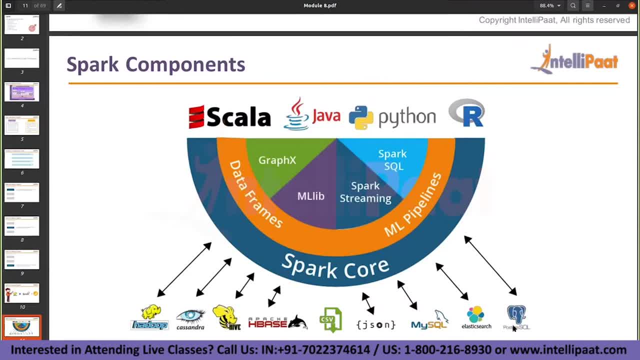 all these things have got some connectivity with your Spark core systems: Postgres, Elasticsearch, MySQL, JSON, CSV files. It's a direct read and write format of a JSON and CSV. It has got its connectivity with HBase Hive Cassandra. 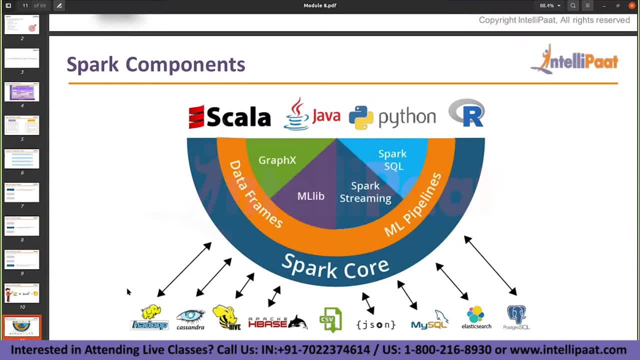 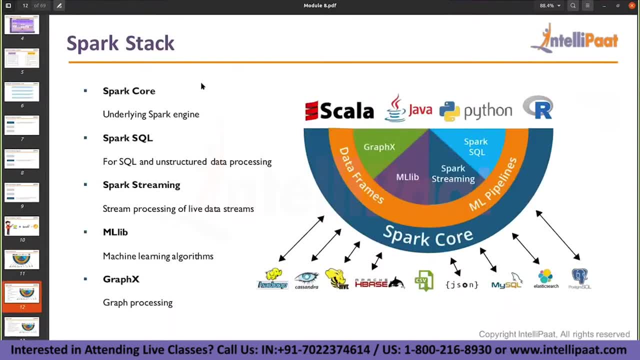 and all the other Hadoop components. Okay, So very high level, very basic concepts, just to understand. And what is your Spark core doing? It's the core functionality of your Spark framework. So all the modules, whatever you run, I mean you create data frames, you create 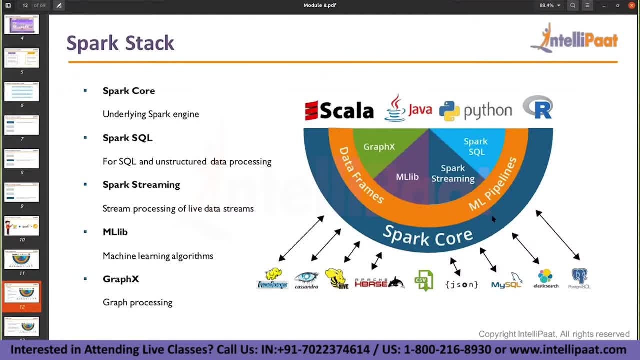 RDD is on top of each and every component. Everything is done execute on the Spark core framework only And Spark SQL is used for SQL and unstructured data processing. structured data processing pretty much. Spark Streaming is for streaming related use cases. Machine Learning: for Machine Learning algorithms. 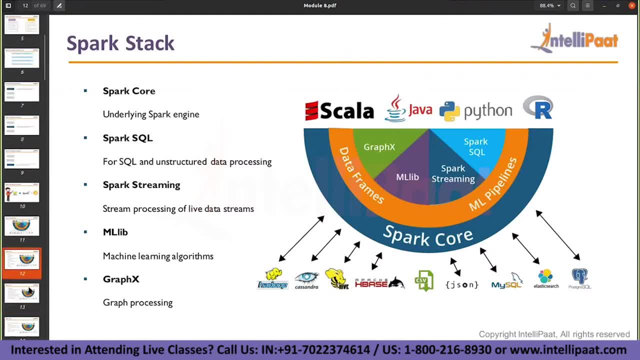 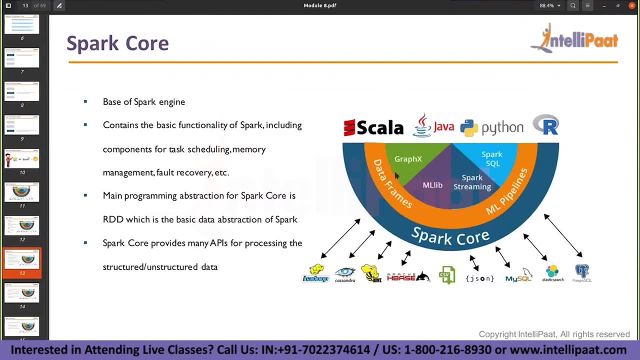 and Graphics for graph-related processing. Okay, So we've already seen these things And so base of what is a Spark core? It's a base of a Spark engine. It's the core functionality of every Spark framework, regardless of what you're executing. 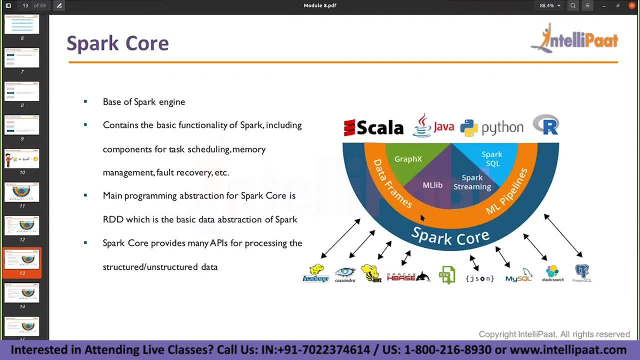 what component you're using. everything's going to get executed on this Spark core itself, And this is where your RDDs will get created. So RDDs are unified across all the other components, your Machine Learning or Spark SQL. So once your RDD is created, 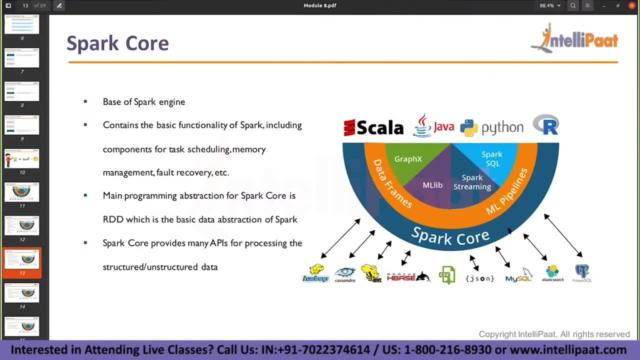 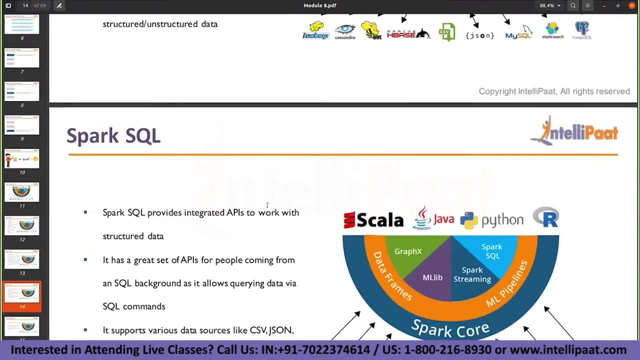 that was set on Spark core and you can access it through any of the other modules. And there is some introduction given to Spark SQL, how they work, How the SQL is going to work. Anyway, we're going to deal with Spark SQL in the details. 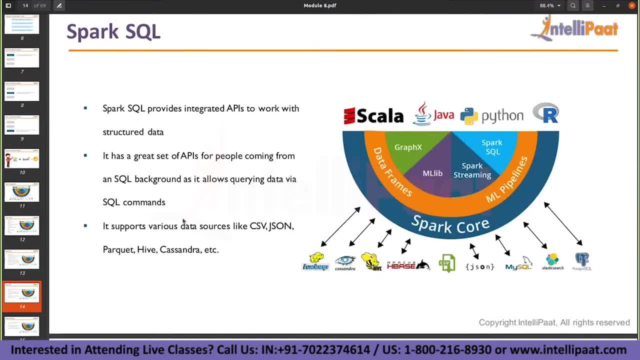 How do we create a Spark SQL component? How do we create a data frame? How do we can load all these kinds of different data files and create the data frames on top of it? How do we access them? Okay, So Spark Streaming. there are some limitations, I can say. 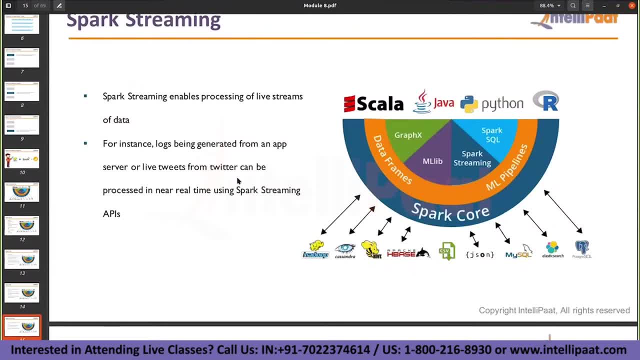 Okay, So this is mainly used for the streaming applications, So Kafka is better use. I mean, Kafka is pretty good. It's preferred over Spark Streaming for some of the reasons. I'll let you know what are the challenges that you have. 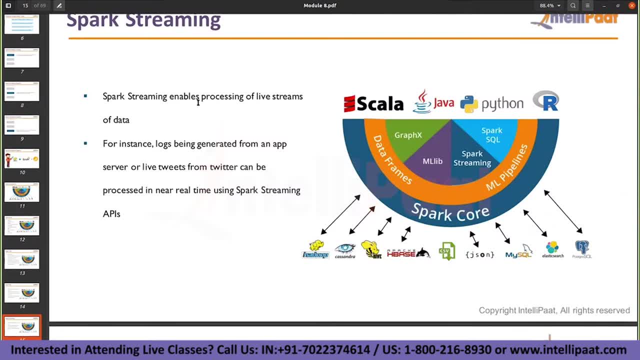 challenges that you have when interacting with the other third-party tools. See: Kafka can easily interact with the third-party tools using an API console. It has got some built-in connectors also, And the advantage, the most important advantage that they have is: 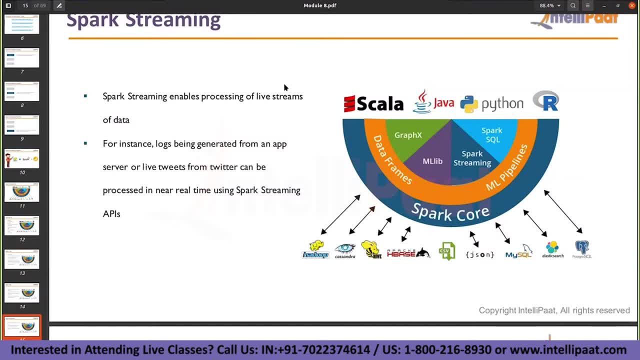 there is some kind of a component called Confluent Kafka. Have you heard about it, Confluent Kafka? There is a company called Confluent which has, which is providing a licensed version of Kafka with better features and better connectors. 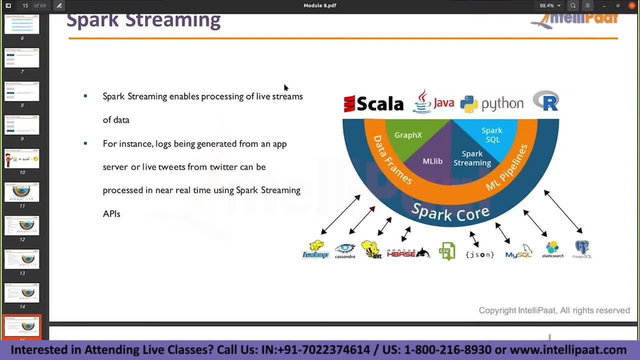 So you need not write any code or you need not build your code in Kafka components. So Confluent itself has got its own connectors to different mostly used systems. So that is one advantage we have over Spark Streaming, but that's a paid tool. 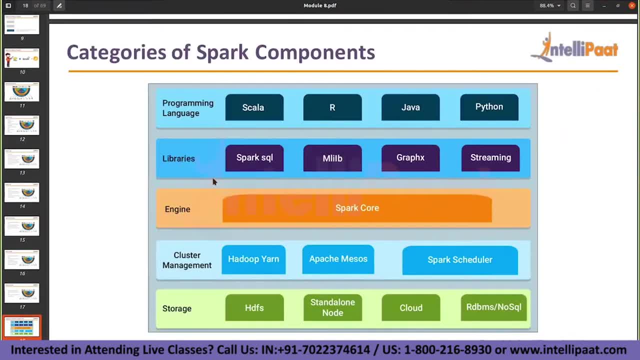 Again, Spark Streaming is an open source, definitely So if you see the categories of Spark components. on the storage side, it can be anything. It can be HDFS, It can be a standalone node machine and it can be a cloud storage. 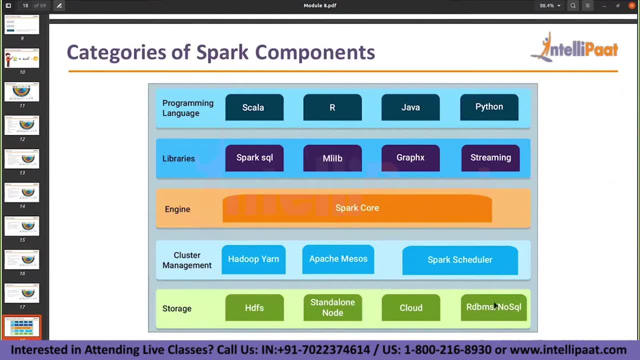 or it can be an O-SQL ad in the storage. So, depending on whatever the storage requirements you have, you'll be selecting any one of it. So it need not be only HDFS, It can also post. it can also be hosted on any of the cloud enterprise. 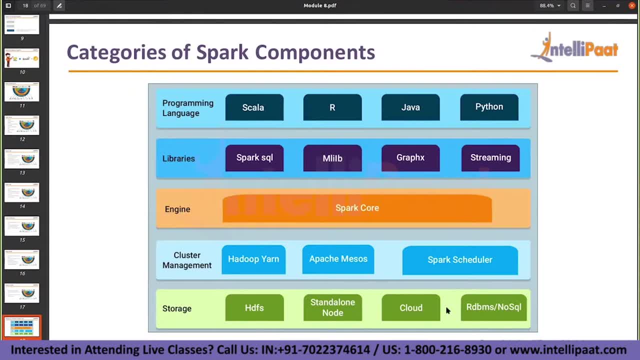 So, for example, you have posted it on an AWS cloud, So your storage will be an S3 bucket. Okay, so you'll be pointing some location and the S3 bucket for the Spark framework and it will keep using whatever the storage you have there. 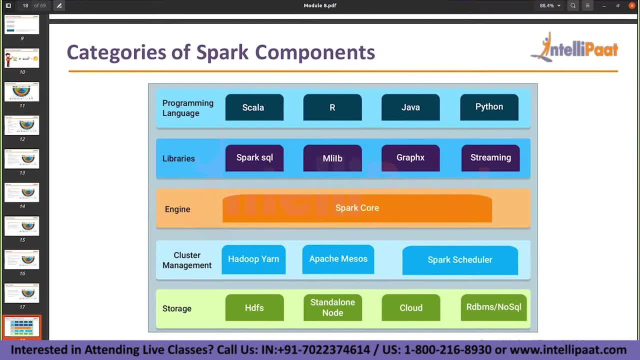 Okay, so you'll be building a system on an EC2 machine or an Azure VM. You'll be hosting the Spark application on an Azure VM and the storage allocated for that Azure VM will be your underlying storage for the Spark framework also. 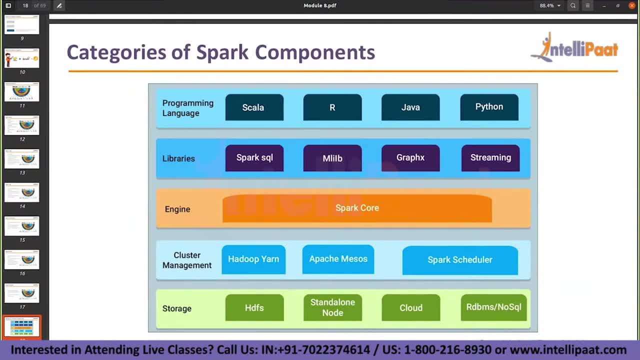 Okay. so, guys, am I deviating? Is it clear? Is it making sense what I'm talking? This is all very high level information. there is nothing in detail where we can get into. Okay, so how Spark is being deployed. 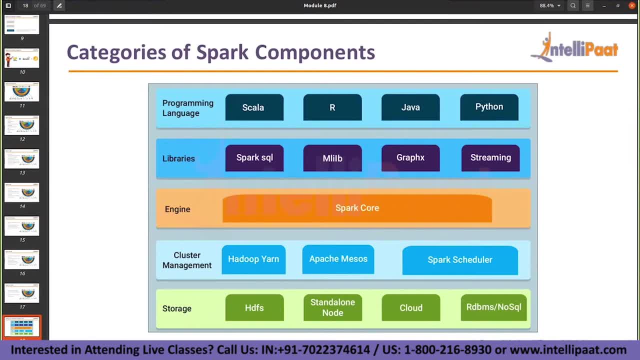 how Spark can be used, all that things. Okay, so same thing we are kind of repeating. Okay, so there are some repetitive slides available, So let's just quickly move on. Are we clear guys? Any questions do you have? Let me clarify once again about that. 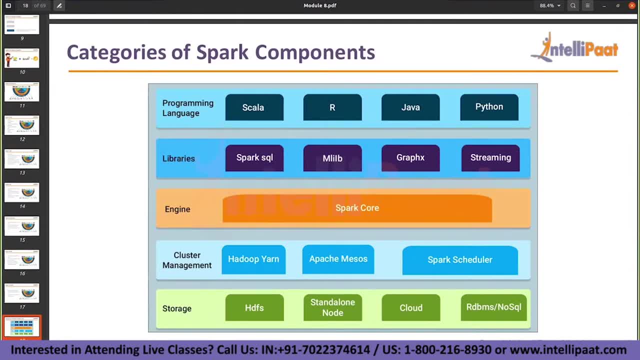 I mean for now we can continue, okay. So the cluster management, the Spark scheduler, is one Hadoop Yarn how we manage the nodes in the cluster and Apache Amisos. So Amisos, we have not used it before in time. 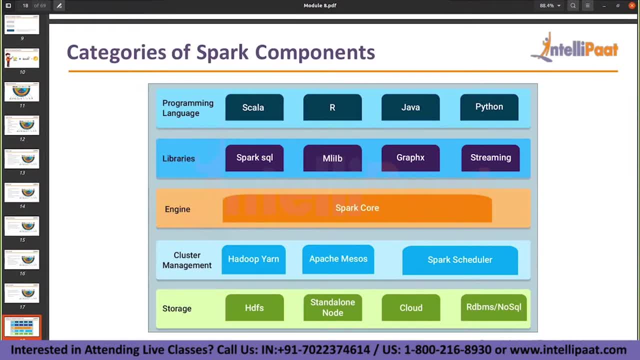 I've not worked on Amisos cluster but Hadoop Yarn and Spark scheduler alone. we have used it And the execution, the core execution engine, will be the Spark core right And on top of it we have this different modules. 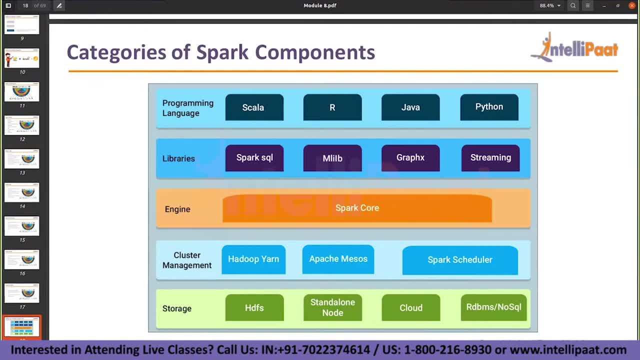 different libraries: Spark, SQL, machine learning, graphics and streaming- And the programming languages are the Scala, R, Chakra, Java and Python. okay, So on the storage side are where you deploy Spark is depending on what storage you get. 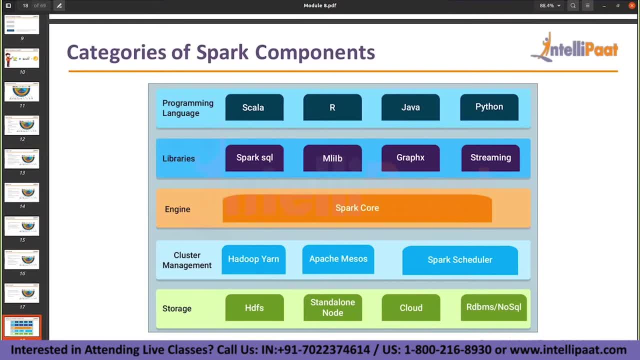 or what the cluster management you're gonna get. So, generally, we have the deployment done on the cloud systems. Like I said, it's going to be done on a particular VM, okay, So if it is an Amazon AWS, you have this EC2 instances. 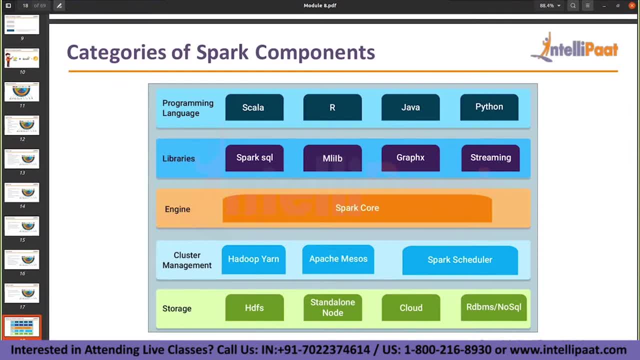 you deploy Spark on top of it. And if it is, if it is an Azure related environment, you have this Azure VMs posted right. So similarly for data for GCP, you have this data proc environment. okay. So in AWS you have got also another feature. 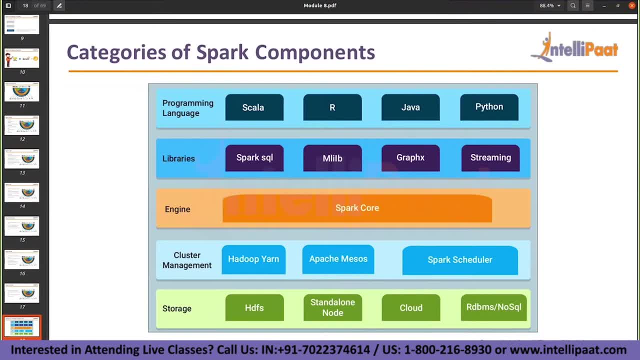 where is? this? is EMR Elastic Map Reduce wherein you build the cluster. The AWS instance, the AWS itself will build you a cluster with Spark and it will take care of all the installations and everything. You don't have to worry about that stuff also. 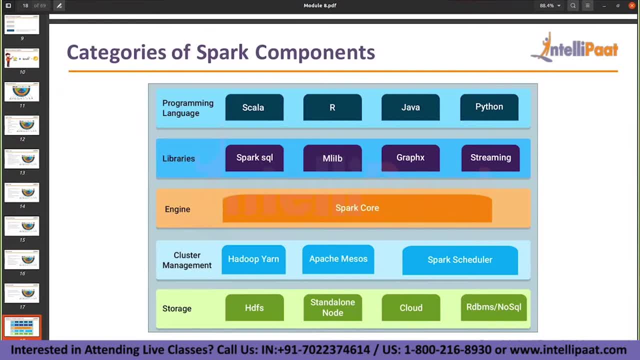 So when you define an EMR, it's something like it's going to create a Spark in a station and it's going to give you the access. So all the setup, everything will be done by the AWS itself. Okay, So there are different ways of different ways. 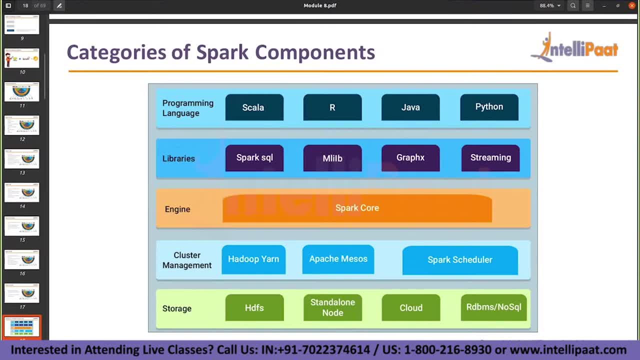 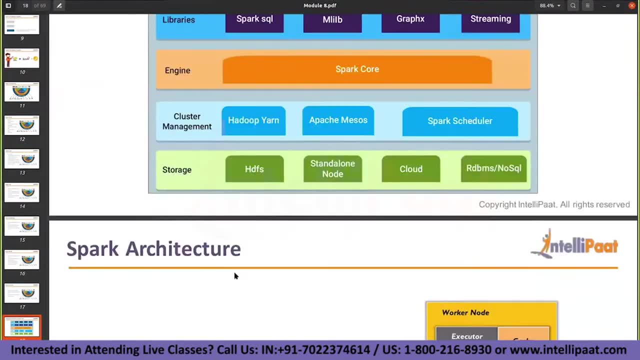 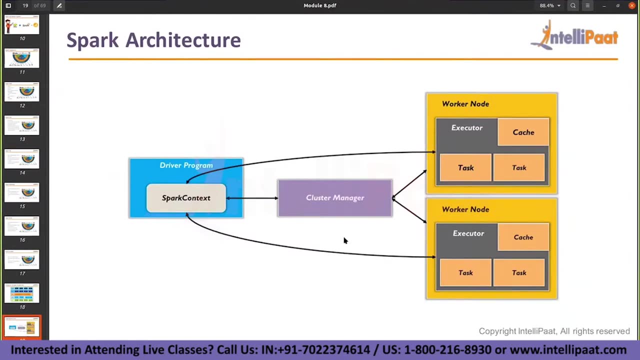 how you can execute this Spark applications, different environments where you can execute the Spark applications, okay, And then we have this Spark architecture. So there is nothing, much, nothing in detail. There are two things again: master and a slave. So cluster manager is going to be the master. 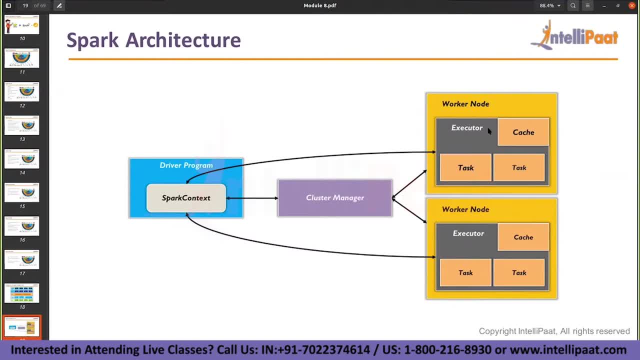 and worker nodes are the slaves. where the worker node in the worker nodes. you have this: executors, multiple executors running the individual tasks. okay, So for each and every executor you'll have a cache memory. This is the in-memory component. 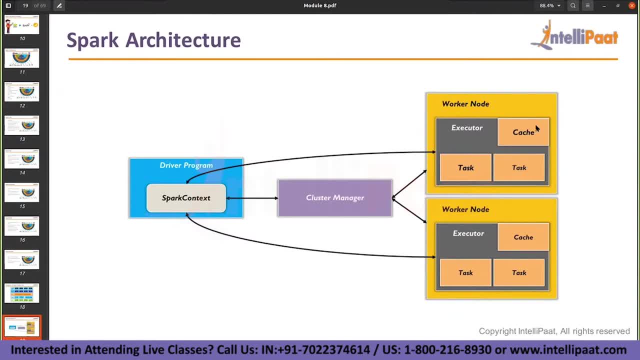 wherever the frequently running outputs or frequently running data frames will get stored into the caching And the driver program will have the actual code, whatever the Scala or the Python code, where you have written the program, and you'll be submitting that driver program to the cluster manager. 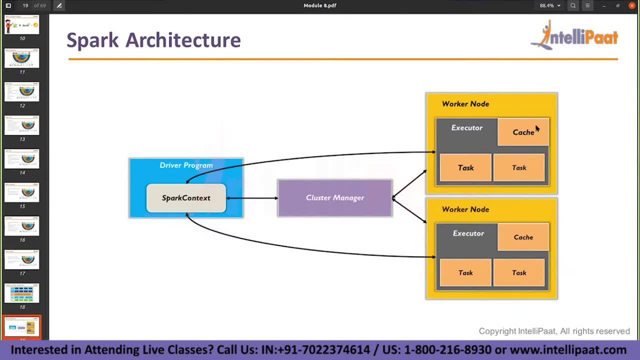 So once you get access to the cluster manager, it will interact with the worker nodes. whichever worker node is available, it's going to allocate this particular program to run on the specific worker node. So now for a driver program. so when you're actually defining a driver program, 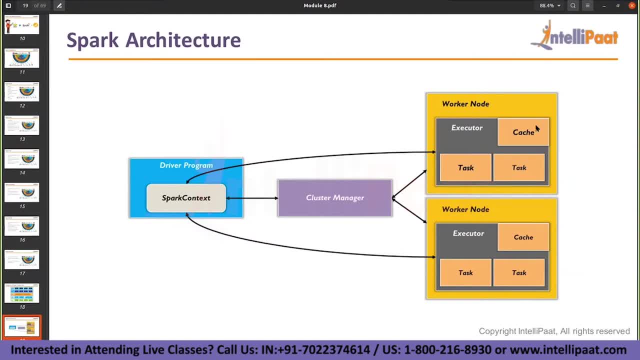 in the program, in the actual Spark program. what you're going to do is you're going to create a Spark context. So that's the initializing, the starting point for any Spark application to run okay. So you'll be creating a Spark context in the driver program. 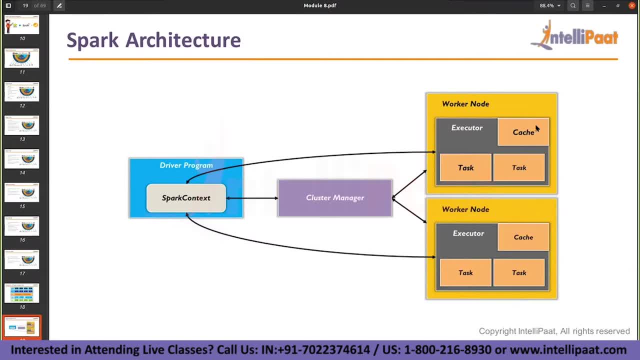 in the Spark program And when the workers are allocated for your program to execute, you will execute this Spark context. you will execute these kinds of operations on top of this worker nodes directly. okay, So there are two ways again: this driver program or this client. 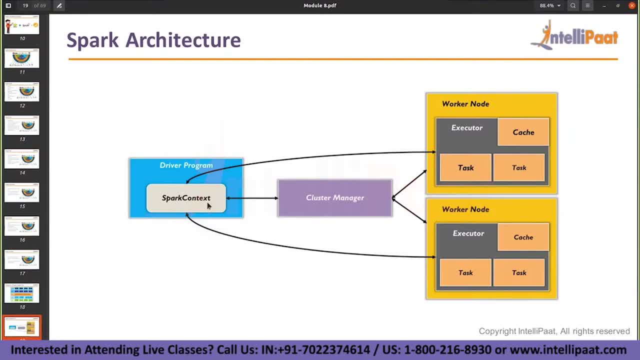 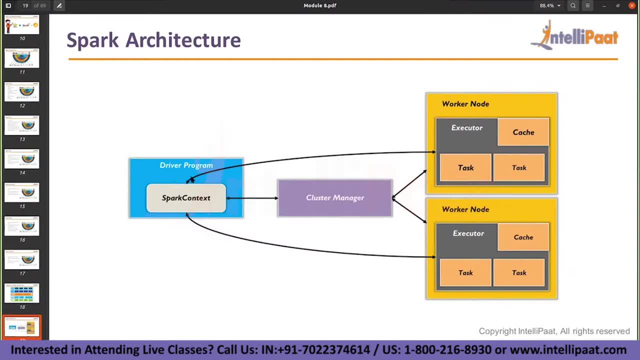 on the client side or it can work on the cluster side. So, whatever the program I have, it can stay away from the cluster manager, it can stay away from the architecture of the Spark and it can work independently- Independently as in, from the client node itself. 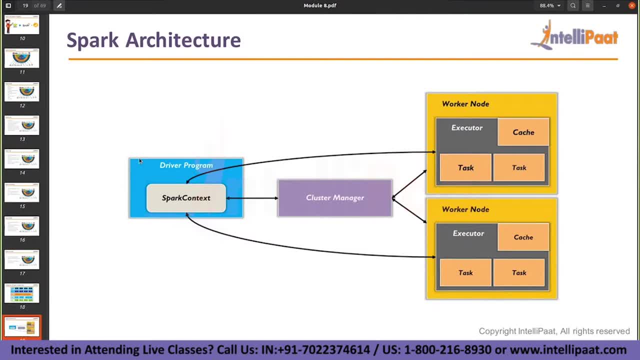 wherever the, from wherever the location the client is submitting the program, from that mission itself it will start executing. it will start using the worker nodes and it will start executing the program. Other way of doing it is you. you move this driver program to the cluster manager. 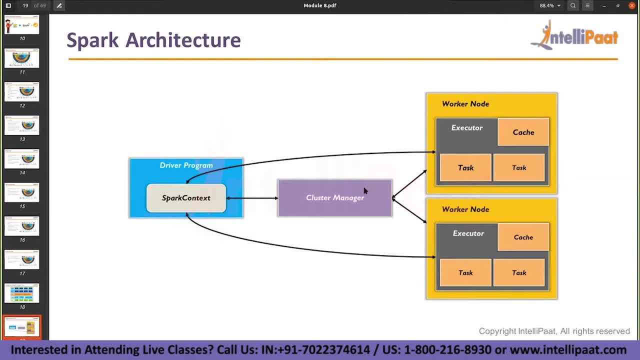 and it will be available locally to the Spark environment and it's going to run the what about the Spark program that we have defined? So in both the cases. so the driver program is in one scenario is in the client location, the one in the other scenario 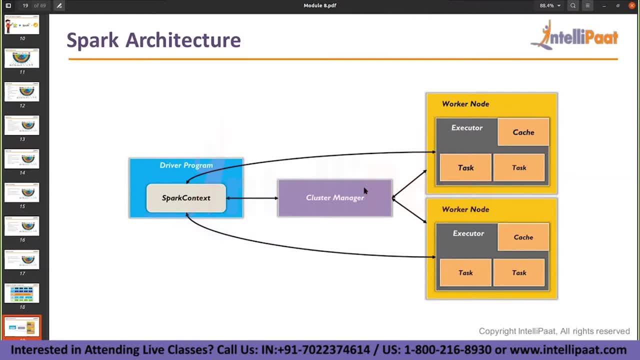 the driver program will be in the cluster manager in within the Spark environment, So that the only difference it's going to make is when it is available. when the program is available in the client location, you are not supposed to disconnect, You're not supposed to get disconnected from the. 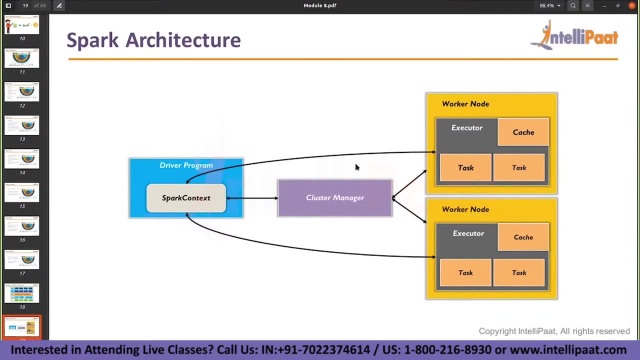 the Spark framework from this, from the cluster manager, because it has to be intact, because the program itself is in the client side, But whereas in the other mode, in the other way of execution, the driver program will be available within the cluster manager. So your client can get disconnected from the Spark framework. 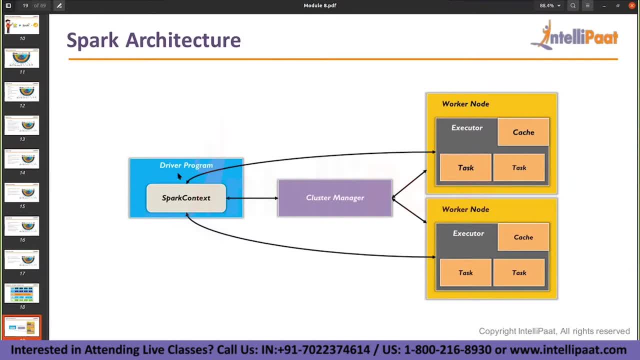 even if it is getting disconnected, your program will still run as usual because a driver program is available within the cluster management. So there are different modes. We'll get into the details, but this is how we will be running the Spark program, okay. 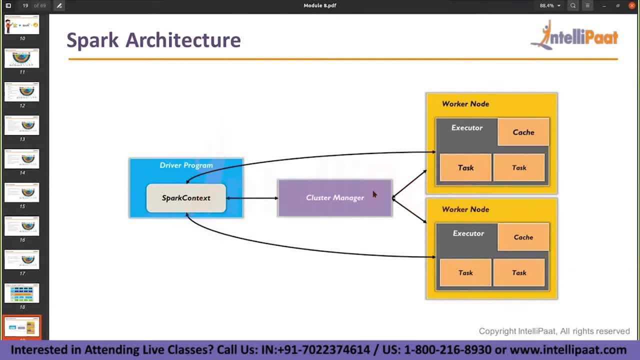 So in the program you'll be defining the Spark context. that's the initializing point for any of your program to run which interacts with the cluster manager. Cluster manager will identify the list of available worker nodes, So those worker nodes will be allocated. 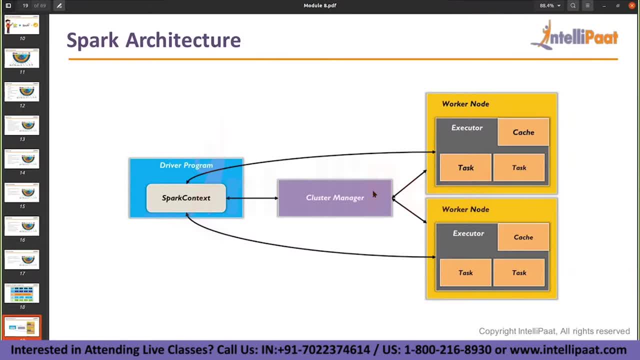 for your Spark program driver program to run. So generally, if you are talking in terms of a single node, if it is a standalone node, Spark environment, if your Spark is set up on a single machine, then your cluster manager worker node. 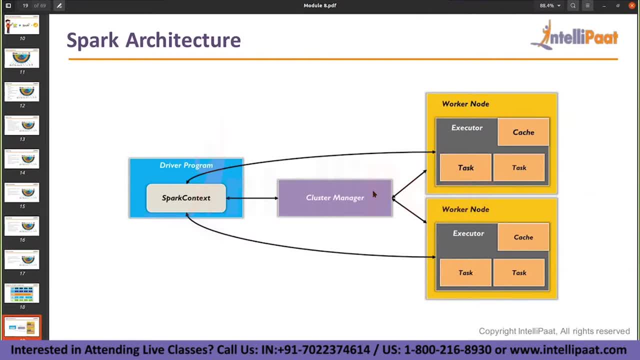 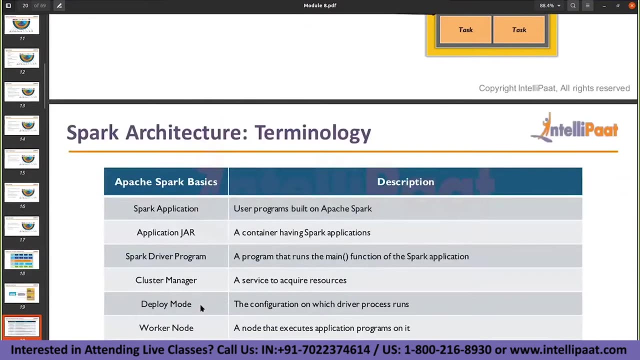 everything will be the same machine and whatever the RAM you have for that particular machine will be considered as a will be divided into this worker nodes- okay. Will be used for executing this particular program, okay. So we will get into the details of each and every component here. 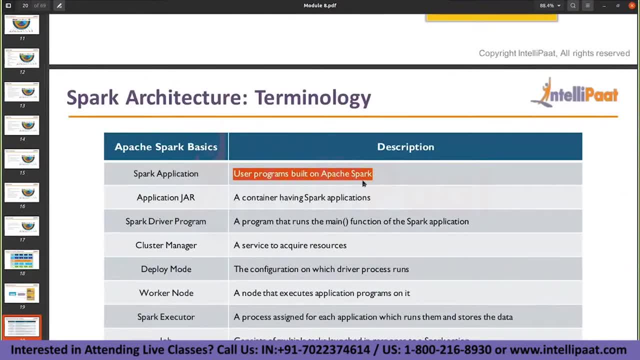 So there's a Spark application, a user programs which is built on Spark. Applications are a container having a Spark application. a Spark driver program, a program that runs the main function for a Spark application. a cluster manager, a service to acquire the resources. 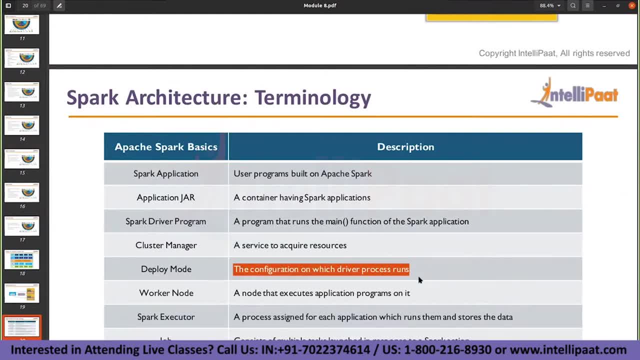 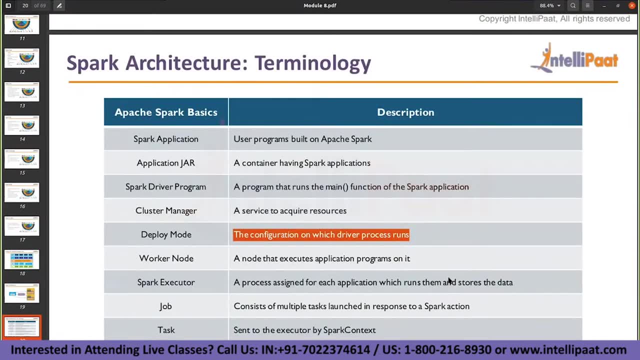 and the deployment mode, the configuration on which the driver process runs. okay, So what is this worker nodes, A node that executes the applications, And what is this executor? And what is this job? What is this task So similar? I mean very known terminologies for 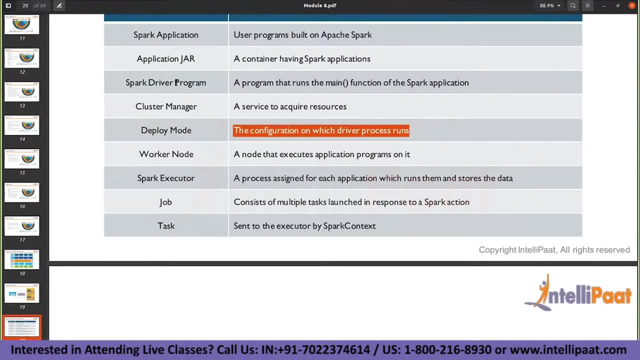 I mean we have been talking in terms of the same terminology as a cluster manager, whatever the program it is. I mean, if it is an application jar, you are converting that program into a jar file. that's the only difference. And Spark executor: what is the job? 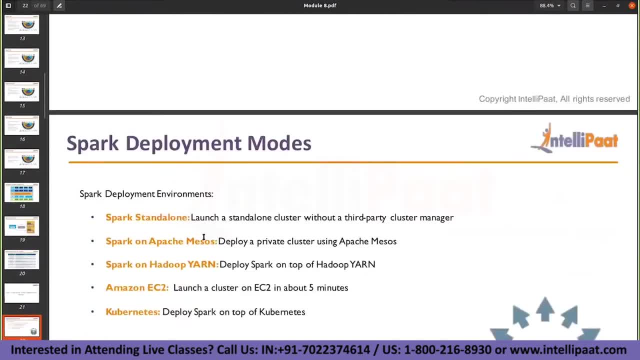 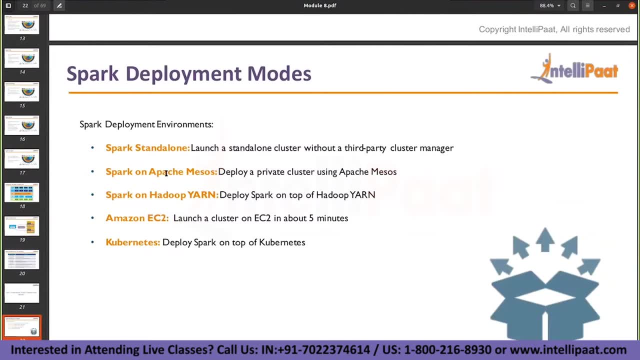 What is the task? Like all these things we have heard And the deployment modes, is a standalone deployment and Spark on Apache resource and Spark on Hadoop Yarn, on EC2 and on Kubernetes. So we've already seen, we already know what is this Spark standalone meals, right? 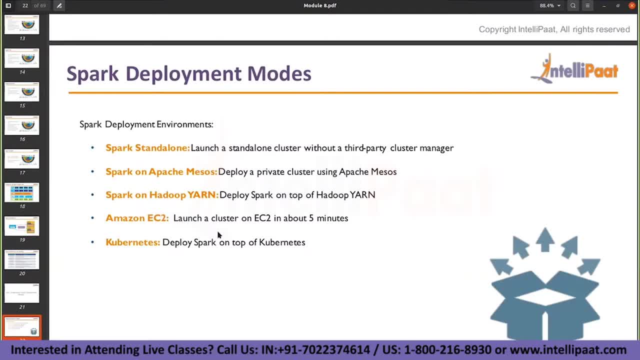 It's a standalone cluster where you have installed- where you have installed your Spark cluster on your own machine- okay, On your separate individual machine And Apache resource. it comes along with the Apache resource component. We are not sure about what this resource is all about. 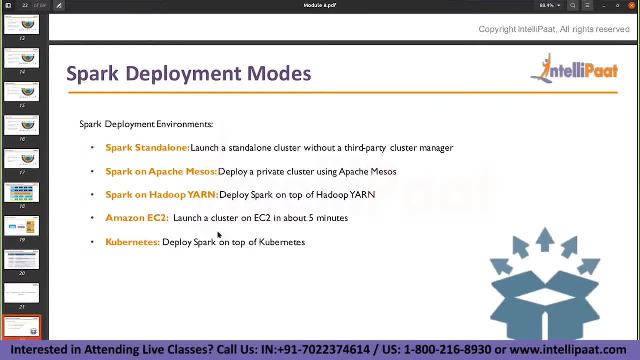 I've not used it before. And Hadoop Yarn. we know how we can deploy Spark on top of the Hadoop environment using Yarn resource management. we will be executing the applications And on EC2, this is using the cloud instance. on AWS: 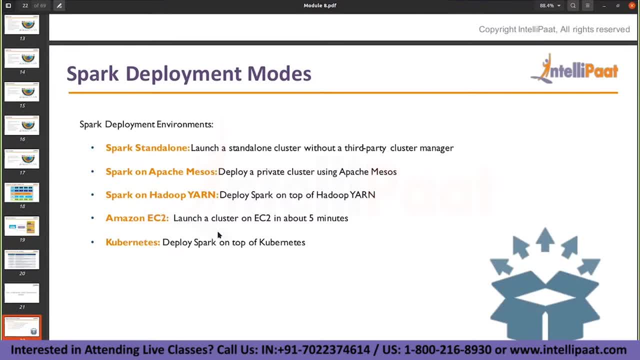 Amazon EC2.. You'll be launching a Spark application. You'll be launching the Spark installation. Like I said, this also comes along with the EMR cluster. This is not an EC2, basically You can call it as an EMR. 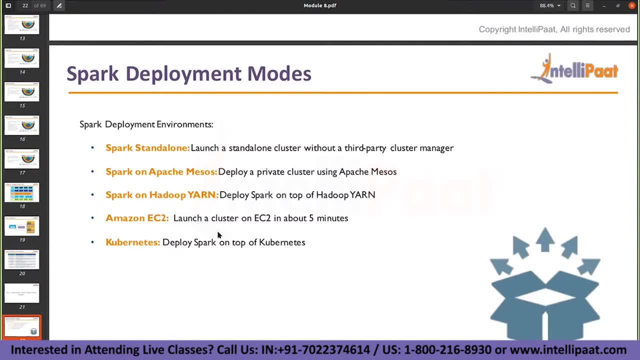 where the Amazon itself will launch a Spark cluster for you. It will launch a Spark cluster, It will create a Spark cluster and it will be configuring everything. All the applications and everything will be configured and will be handed over to you. So that, basically, is an EC2.. 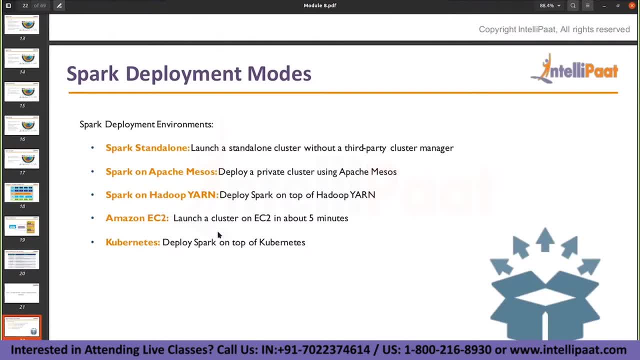 This is an EC2 instance only, but when you install Spark and everything, when you configure everything, we call that as an EMR. So how many of you are aware of this terminology? EC2, EMR, AWS related cloud instances. 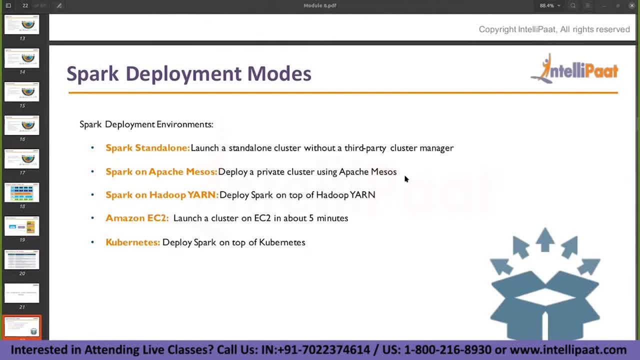 Have you heard about these things before? Do you know what is a VM, a virtual machine? A virtual machine, Virtual machine is something which is virtual and you've got some RAM and you've got some storage for it. So there is a machine which is available remotely to you. 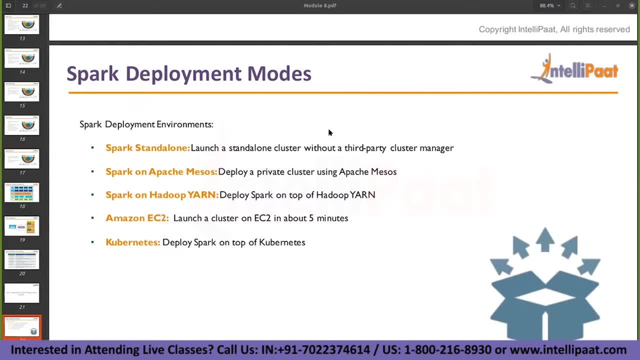 So, using some IP address, you'll be connecting to that machine and you'll be executing your tasks. So, instead of you running the programs on your own machine, you'll be connecting it to a remote version. So that's what we can deends as a virtual machine. 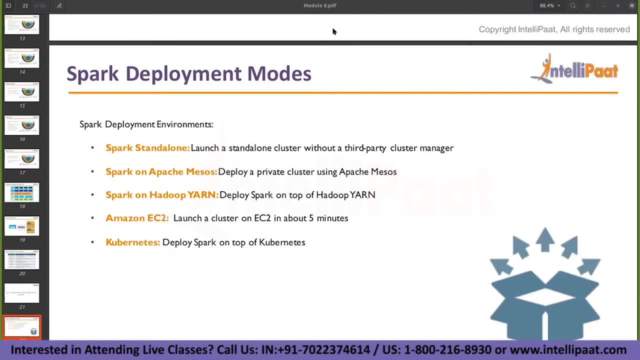 So if the machine is posted on an Amazon cloud, AWS cloud, that instance we call it as an EC2.. So EC2 is nothing but it's a virtual machine. It's a machine machine which is hosted on cloud, amazon cloud. okay, so every ec2 instance when you are configuring it. 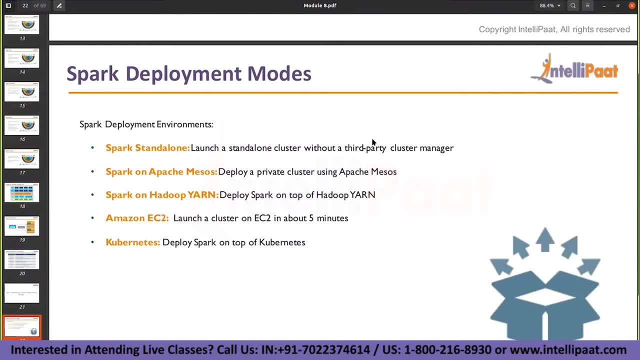 you will have the privilege or provision to specify the amount of ram you wanted to allocate or the amount of storage you want to allocate. okay, so this is how we will be defining and we will be creating a virtual machine on amazon or azure or whatever. so on amazon, we 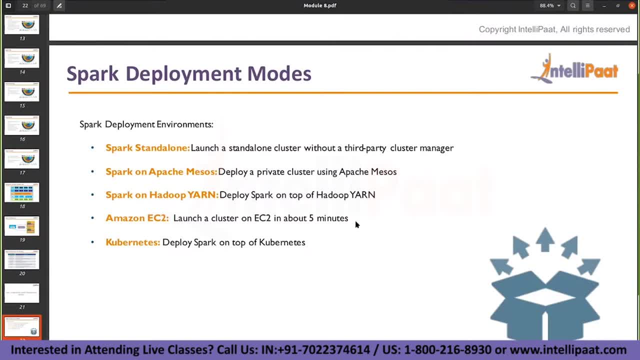 call it as ec2 and, on azure instance, we call it as azure vm. that's it. that's the only difference. so, ultimately, what is it? it's one machine which has some amount of ram and some amount of storage for it. so, instead of you doing it on your own machine, which is a, which is a physical machine, 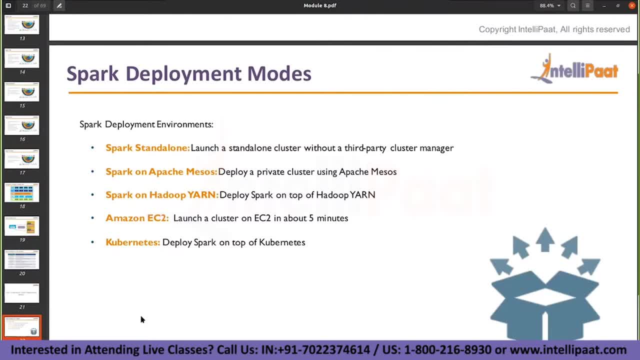 available that to you. instead of you doing it on your own machines on premise, you are connecting to a cloud machine and interacting with or running applications on top of it. so now you understood what is ec2. it's a virtual machine which is hosted on an amazon cloud similar to 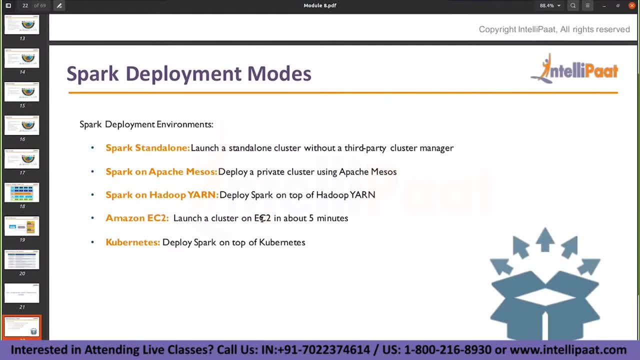 ec2, you have azure vm, which is hosted on azure cloud. that's the only difference, and i have used a term called as emr, right? so what is this emr? emr is also a neat ec2 machine only, but the only difference is it comes with a hadoop installation. 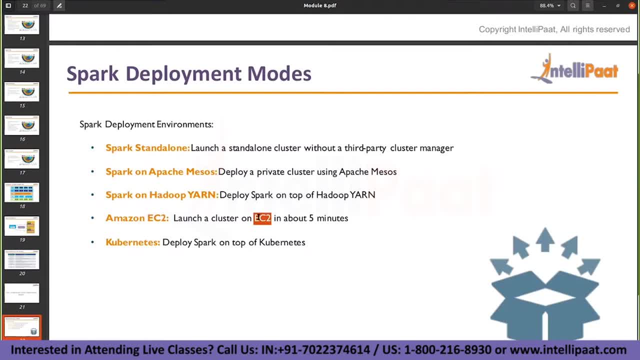 or it comes with a spark installation. okay, so if you select an ec2 instance, who has to do the installations? you have to do the hadoop installations or spark installations. if you select an emr instance, it will give you an ec2 instance with installations run by hadoop. 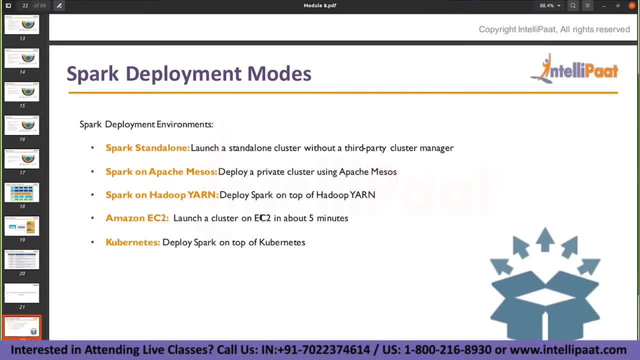 by amazon itself. okay, amazon itself will take care of the installations and it will give you it. so both are the same. both are the same ec2 instances only, both are the same virtual machines only. but one is amazon itself is doing the installations. it's creating a cluster for you. 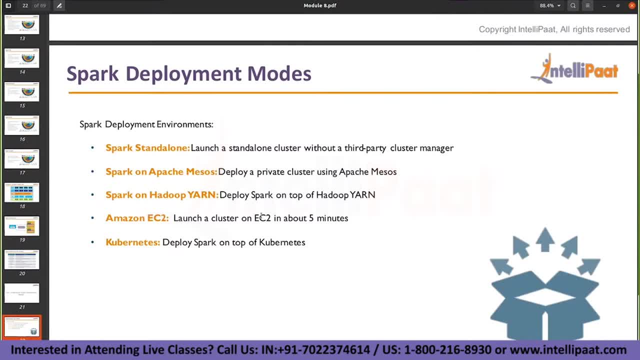 and giving it and, on the other hand, if you wanted to manage it, if you wanted to create it, you can do it by taking an ec2 instance alone. now you have some clarity idea. better, same thing if you are migrating to gcp. there is a, there is a virtual machine instance. we call it as. 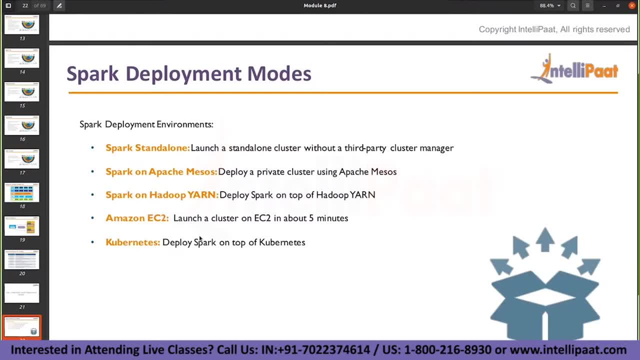 so the same thing again: you configure. whatever, uh, the requirements, whatever the cluster storage you want, you can configure and you can create your instance. so how do we connect to those ec2 instances? or azure vms is using an ip address, using an ip address and a key. there is a ppkp. 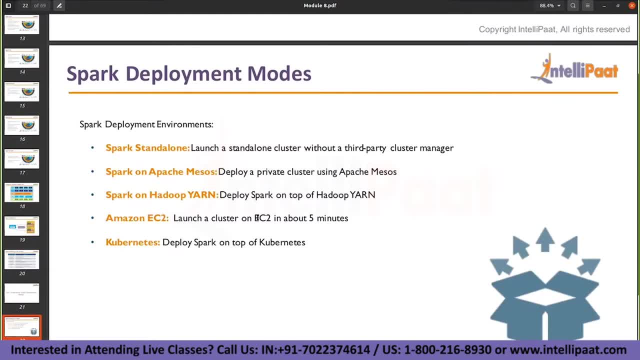 p and key files available using which you can connect to it. okay, so right. so this, this spark, can be deployed on all these things. it can be deployed as an individual machine, standalone machine on a fashimi source, or it can also work along with hadoopian for the resource management. 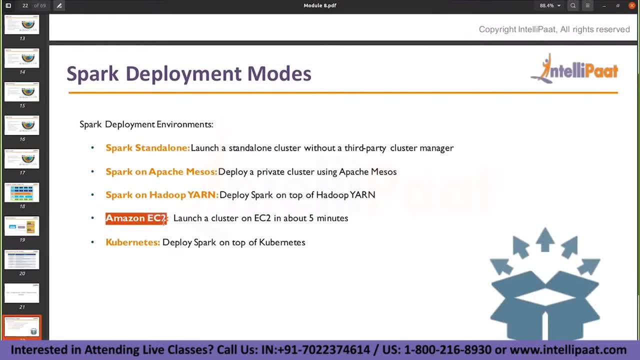 component. it can be deployed on an amazon ec2 and it can also be deployed on a kubernetes environment. so, using some docker containers, you'll be deploying it on a kubernetes environment. using some yaml file, you'll be deploying it. okay, are you aware of this? kubernetes? have you heard about it? 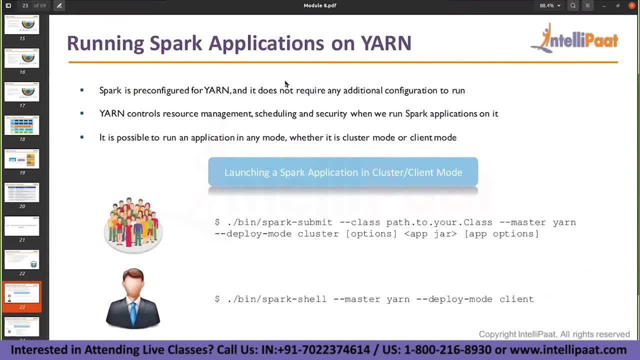 so kubernetes is some kind of a container related approach. so you'll be deploying, you'll be installing spark in the form of a container, so it's easy to kind of deploy on different different instances. it's not. it's not environment dependent, so you can deploy. 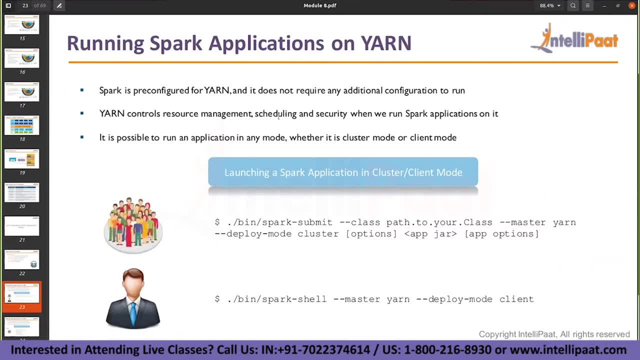 it anywhere you want it to. so the same version of spark, the same version of all, all the environment, whatever the variables you have set, will be generic and when you have different applications using the same version of spark and the environment variable, it can be deployed. it can be. it's some. 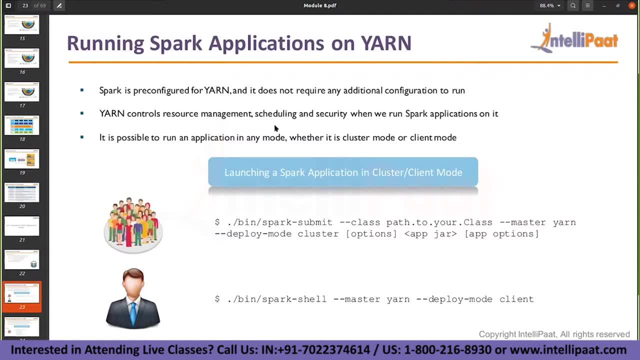 kind of a container. you deployed everything and you're keeping it ready. you can take it anywhere you want it to. okay, so you have some requirement in this particular application. you run it here, you go to different applications, you run it there and wherever you wanted to, you can maintain the. 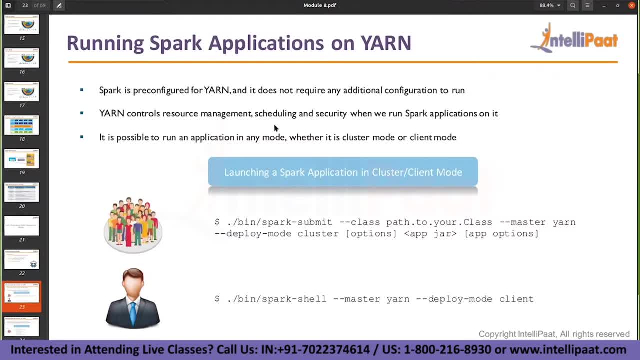 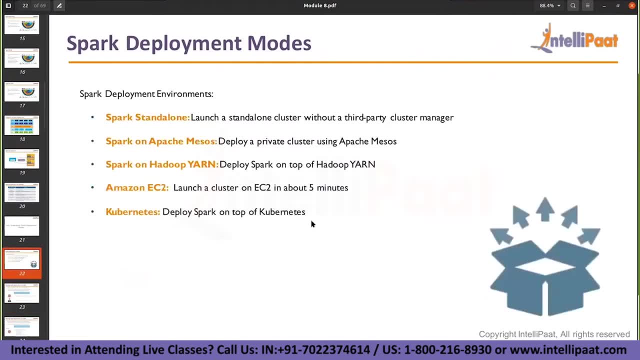 same. you can maintain one single spark cluster across different applications wherever you wanted to run. okay, so running spark applications on yarn. so forget about whatever unnecessary things that we discussed. see if it is going on top of it. just just just ignore. you'll get to know more about. 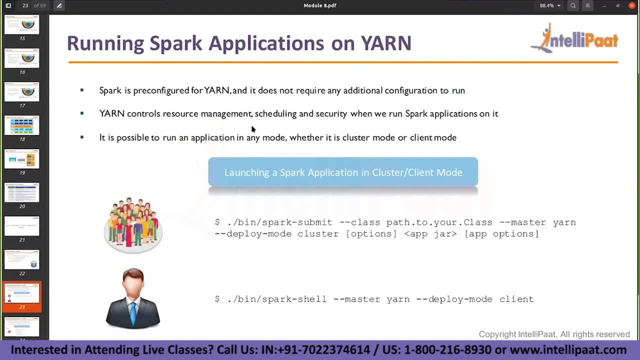 those details, but our core feature is like it can be deployed. our spark can be deployed on different ways. it can be deployed on a standalone cluster or a cloud vm or wherever. wherever you wanted to deploy, you can deploy and running spark applications on yarn. how do we run this spark applications on? 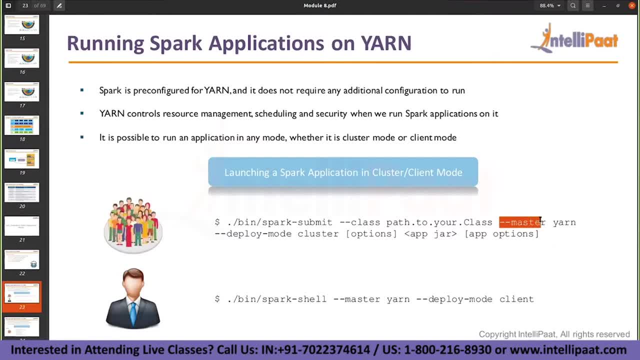 yarn, you will be setting the master hyphen, hyphen, master, you will be setting it as yarn and that will use the existing yarn installations or yarn cluster management resources to run this particular application. okay, so how do we run a spark application? there is something, yeah, so 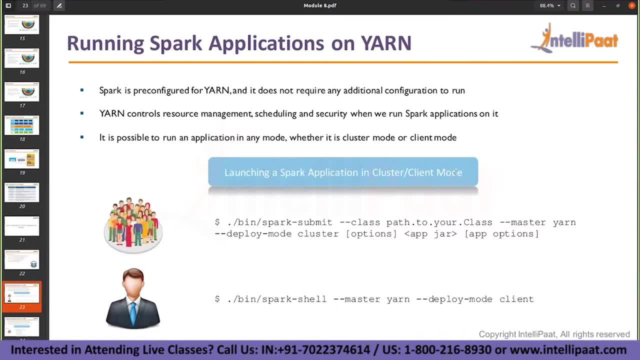 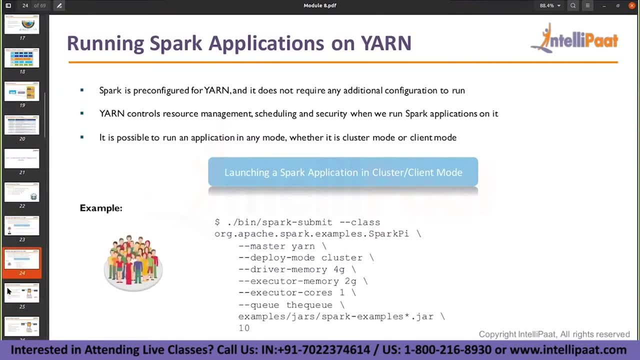 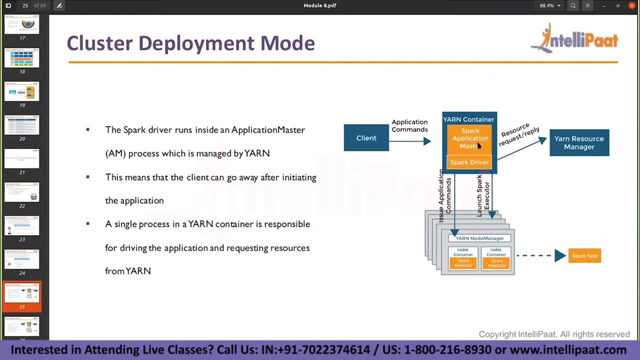 launching a spark application in client and a cluster mode. so this is what i was saying. if you go back to the diagram, i think they we have a better diagram available. yeah, so this is the entire spark framework that i was talking about, right? so, spark, you have a application master, you have the node manager, you have this container, you have this. 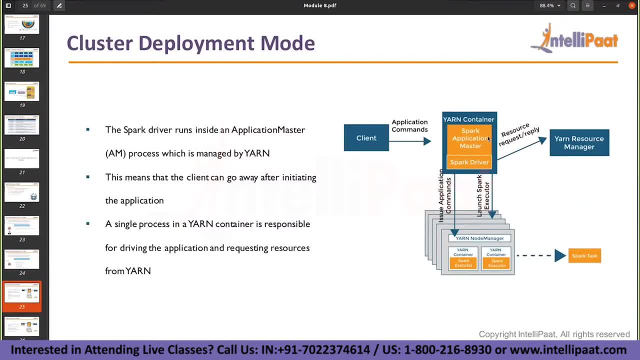 executor. so forget about whatever the yarn related components you have. you have this entire spark architecture here, okay. so one way of running your program is: you are pro, you are keeping the spark driver program inside the spark environment here. okay, inside this spark environment, inside the application master, to be very specific. so here: 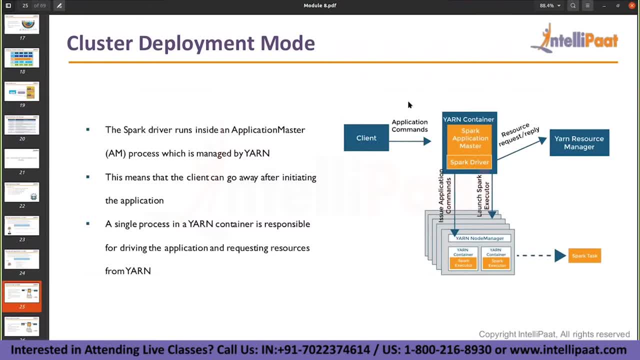 your client can get disconnected. your client can get disconnected from the application and the program can run as it is. i mean it. it won't. it won't disturb the execution of the program, even if the client is connected to the application or if it is getting disconnected to the application, because this spark driver is already available within. 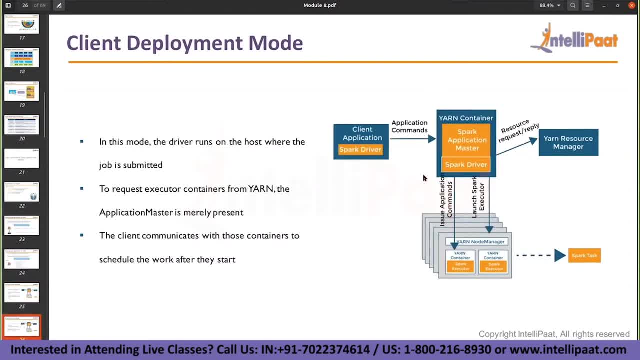 the spark framework. and in the other example we have a client that is connected to the application, For example the Spark driver. you have it here in the client application. So in this case, as the Spark driver is available on the client application, your client has to be intact with this execution process, with this application master. 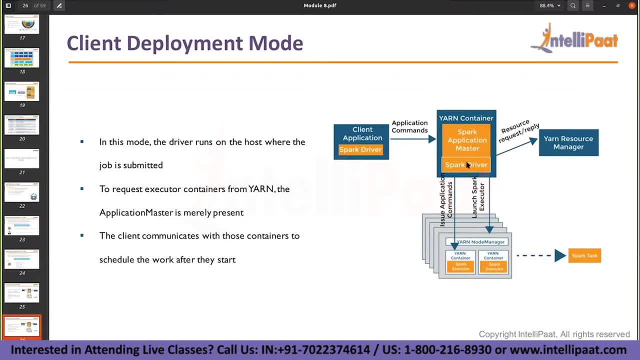 For you to be able to execute the Spark driver program. So the Spark driver shouldn't be here. Only this particular Spark driver has to be here. So when your Spark driver is on the client side, your client has to be intact with your application master for your program to run. 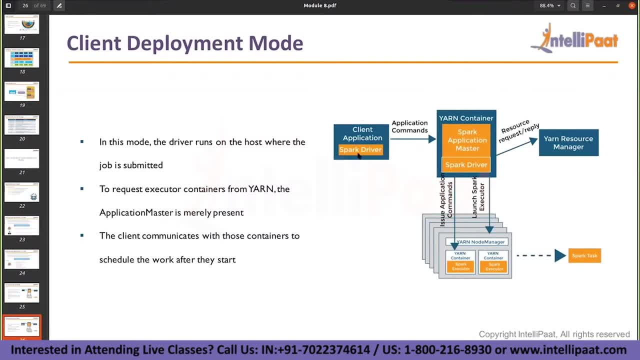 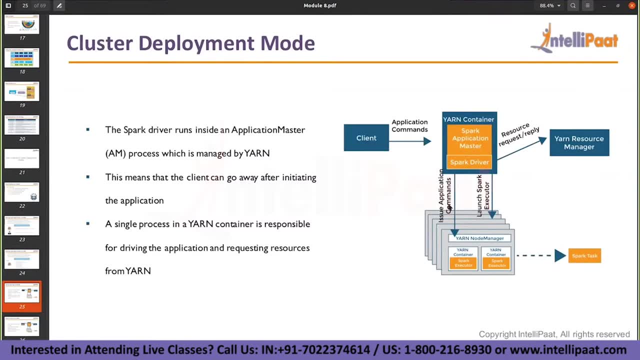 So these are the two things. One is Spark driver working on the client side, Spark driver working on the application side. So if the Spark driver is on the cluster, we call it as a cluster mode. If it is on the client, we call it as a client mode. 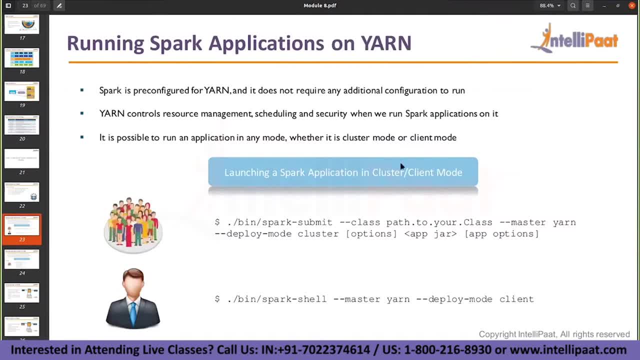 That's the only difference. So cluster mode and the client mode. So where do you specify? deployment mode is cluster and deployment mode is client. So, depending on what mode you select, your Spark driver will be sitting on either sides, on the client and as well as the cluster. 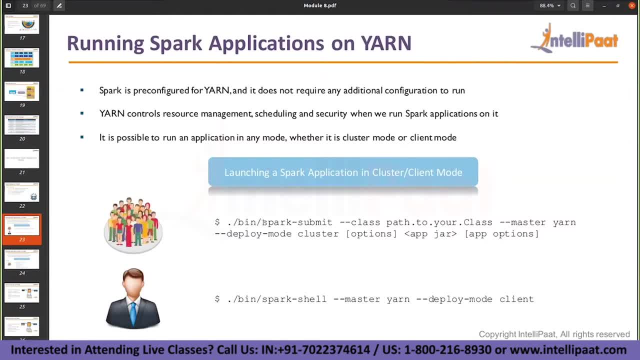 Getting it. So now, how do you submit a program? There is a command called a Spark submit. You write some program, you write some Java, you write some Scala or whatever the jar program you define. you convert that into a jar program and then submit this using a master parameter. 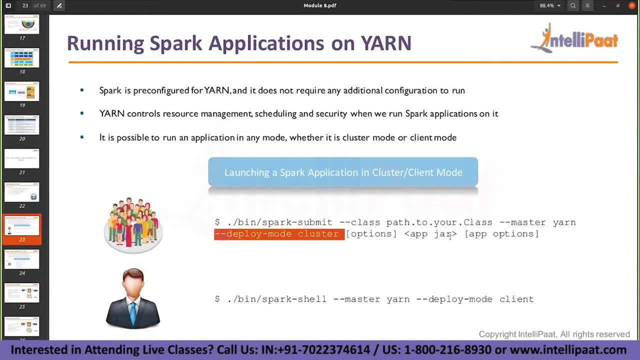 as well as a deployment mode parameter. It will run. this particular jar will run on this particular Spark. So you see, Spark is running on this particular Spark cluster. now, Okay, getting it. So, similarly, this is: you're submitting using a Spark submit command. 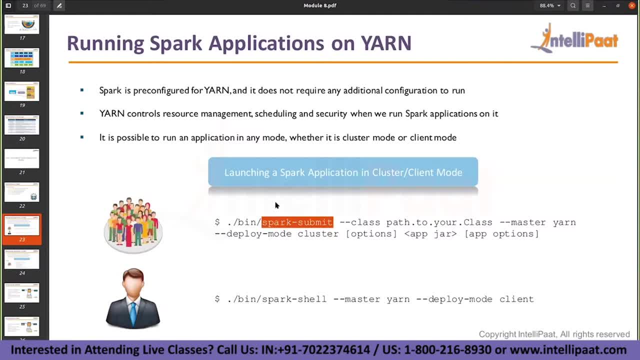 So using Spark submit command, you will not log into the Spark shell. You'll directly execute this program on top of the Spark cluster. But using Spark shell, you are using the Spark shell, you are navigating to the Spark command line And after you navigate to the Spark command line, 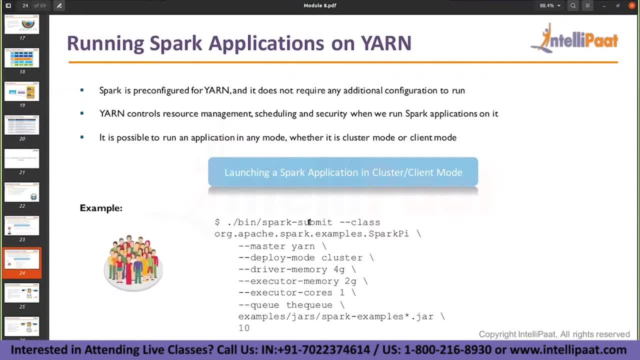 run or whatever the commands you want it to. okay, So this is Spark Submit. There are different parameters allocated to it, So we will look at what each and every parameter is. What is this executor? memory driver. memory deployment mode. What is this master? 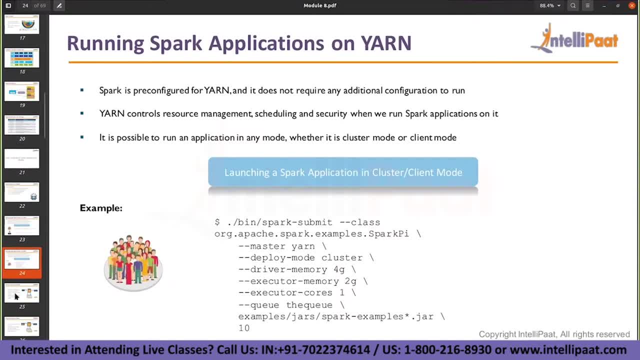 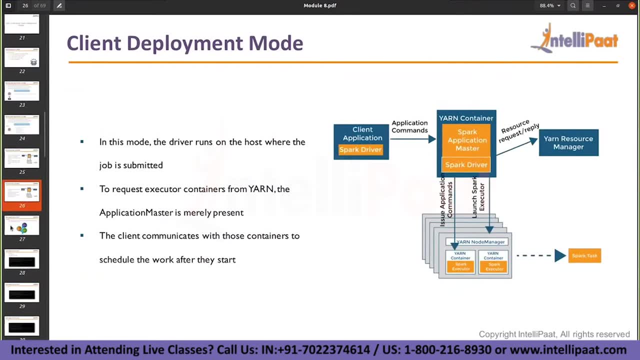 What is this queue And all that? we will see that one by one. okay, Now are we clear with this: two deployment modes: the cluster deployment mode and the client deployment mode. Do we have any questions? Okay, So how do we start this Spark Shell? 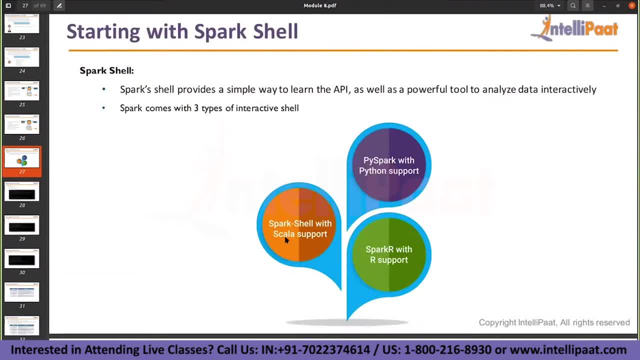 There are different ways of starting a Spark Shell. You can start a Spark Shell with Scala support, with Python support and with R support. So Scala support, it's going to be. a command is going to be spark-shell. For Python support, the command is going to be pyspark. 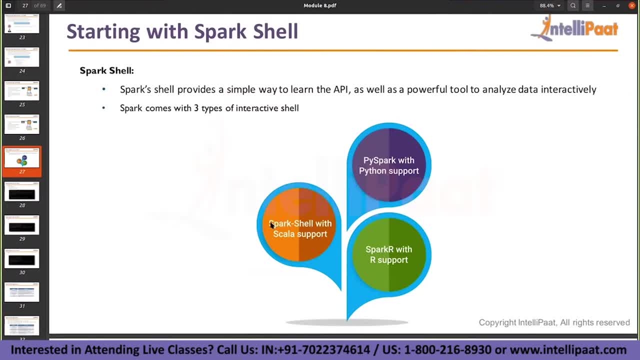 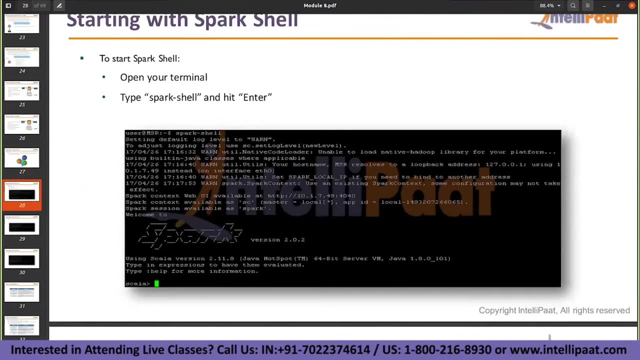 And for R support it's going to be spark-r. So for our concern for our, in our sessions, we are only going to do a Scala support, So we will always start it with spark-shell in there. So spark-shell, this is how it's going to be. 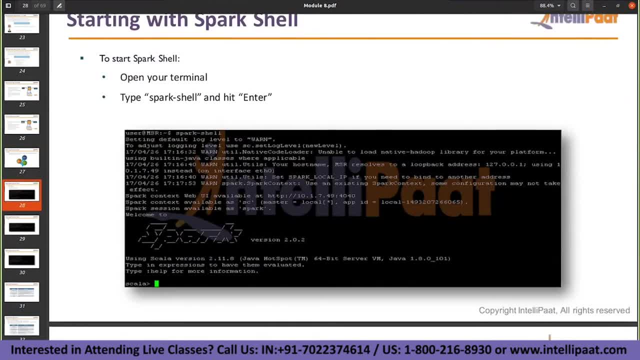 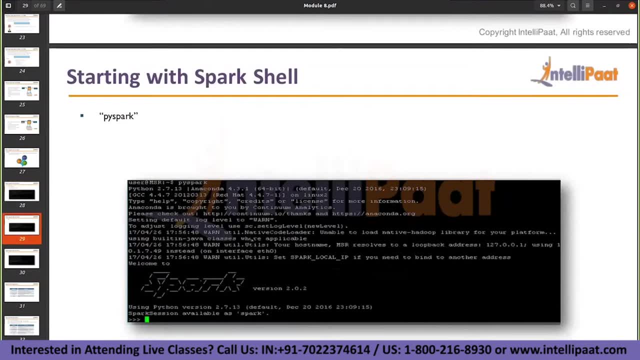 So some of you might have already seen it. We've already finished the installation for some of us, and using spark-shell, you were able to launch the Spark environment. okay, So this is pyspark- the same thing, but here you can see the Python version. 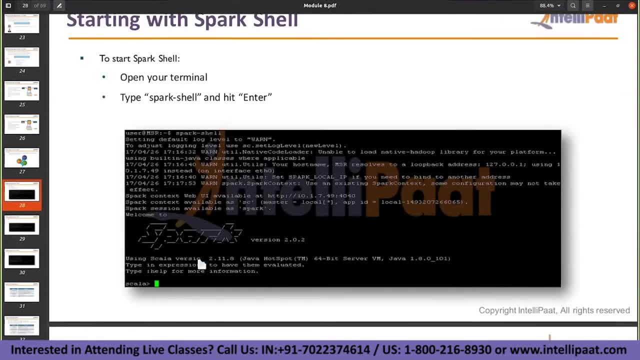 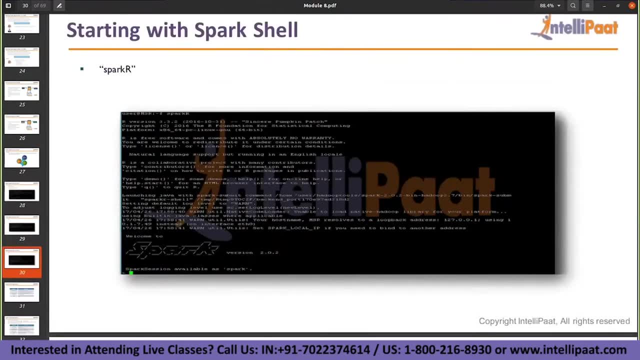 And in the previous slide. you can see this Scala version somewhere here using Scala 2.11, using Python 2.7.. And similarly for spark-r, you can see whatever the version of Spark or it is running and it's going to open up R shell. okay. 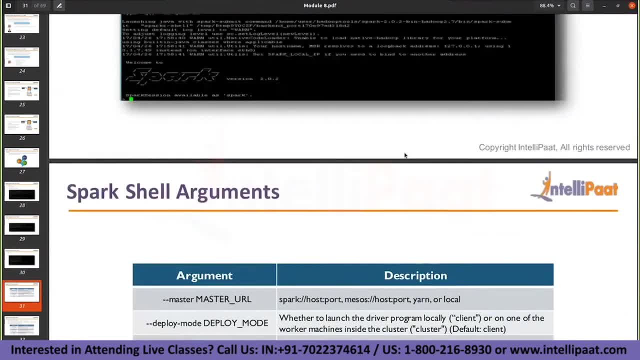 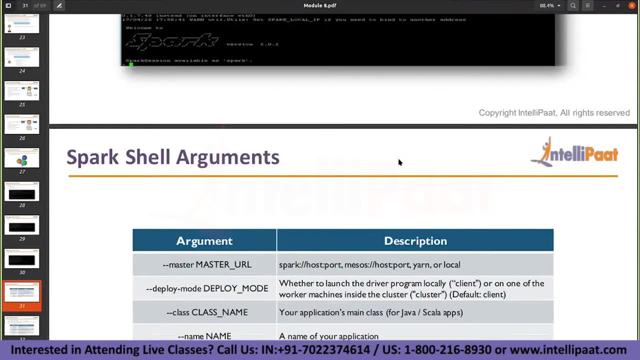 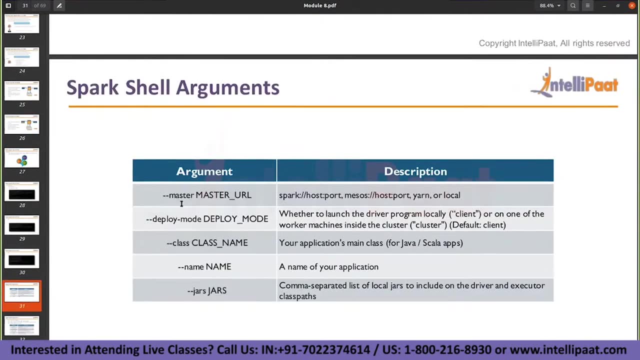 So that's the only difference by running it in different modes. okay, Are we clear? Okay, so now we will look at some of the arguments that we have. There are different arguments that we have passed while submitting the applications. So, firstly, what is the master? 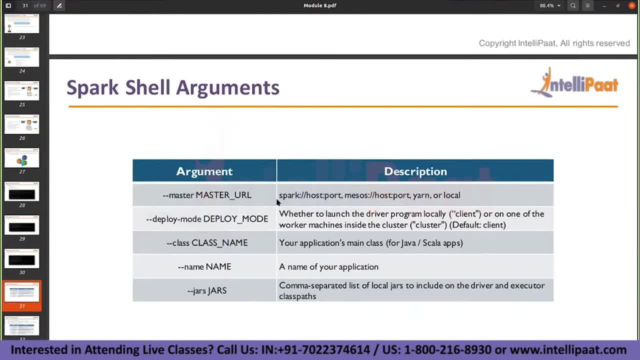 Like we discussed, master can be your standalone node where you can give the the host name as well as the port name, or it is a Mesos, Apache, Mesos cluster with a specific post and port. It can be a yarn or it can be a local machine, okay. 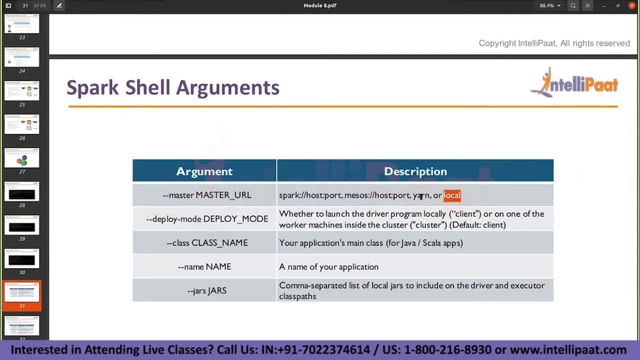 So, depending on what deployment you have done, you can specify whatever the master URL. okay, Then deployment mode: hyphen, hyphen. deployment mode will be a client mode and the cluster mode. We have seen these two parameters already: what is client mode and what is deployment? 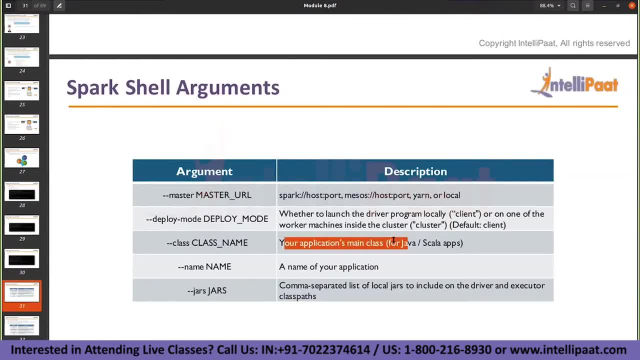 what is cluster mode And the class name. whatever the application main class, whatever the program you have written, whatever the main class name you have, you'll be specifying the class name And here in the jars you'll be giving the jar file name. 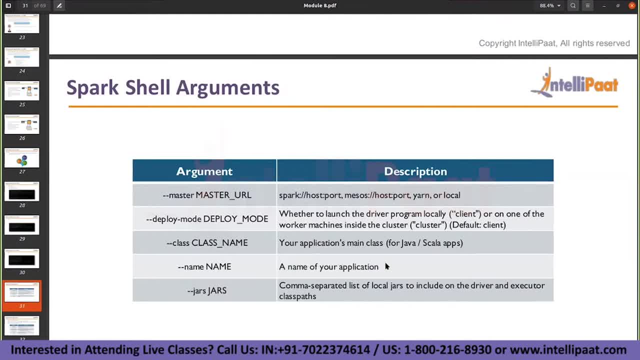 Okay, And the name: you can give any specific name for the application, So this is only required for you to identify in the web UI. So after you submit this application in the web UI, you can see the list of applications that are running. 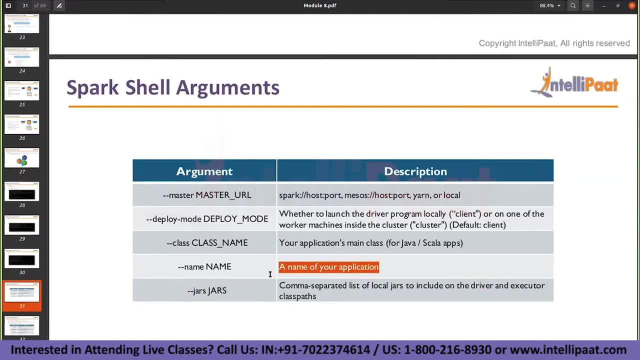 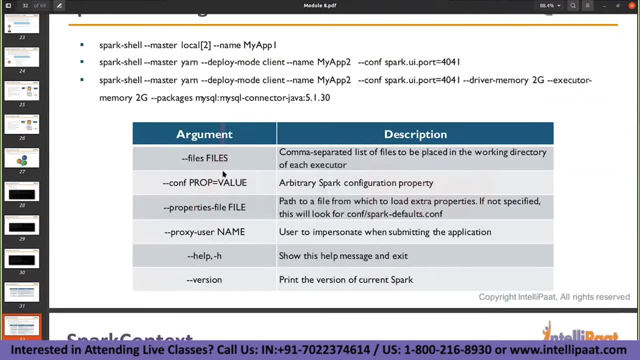 So you can differentiate using a specific name by giving a specific name to it. okay, So this is one. these are some of the arguments And in addition to that, we have files, So a comma separated list of files to be placed in the working directory of each executor. 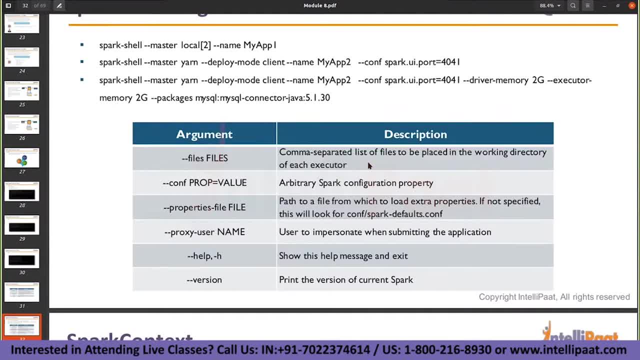 So, whatever the files, whatever the input file locations or whatever the output- for example, if I'm giving an input file or an output file for you can specify the input file name and output file name, It will get created And there is a configuration parameter. 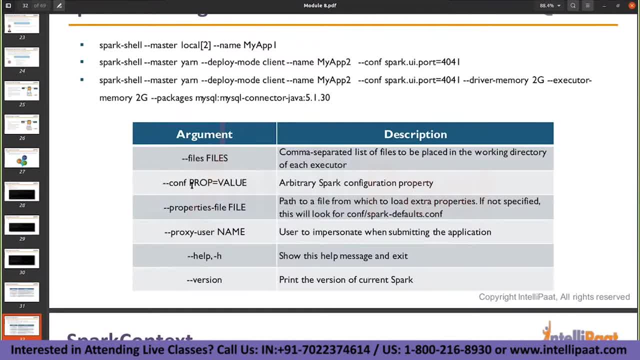 whatever the property and whatever the value. So hyphen, hyphen, conf can take a lot of values. there are a list of values which it can take. i'll take you to take you through the different values which it can execute, so the property name and the property value. so you can give any number of properties, for that matter, under hyphen hyphen. 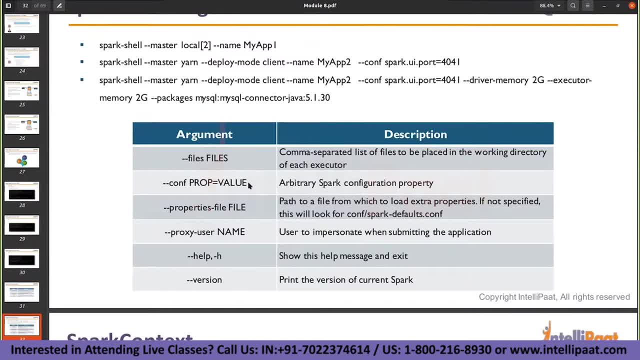 conf. okay, so this- this varies from application to application if you are interacting with a different third-party tool, so whatever the parameters that you want to set with that third-party tool will be listed everything using a hyphen, hyphen conf only, and there is a property file. you can. navigate it to spark defaultsconf if this is not available. if you want to use a some other property file, if you want to give some extra properties, you can create one own property file and you can give the path of that particular thing. so by default it's going to look for spark. 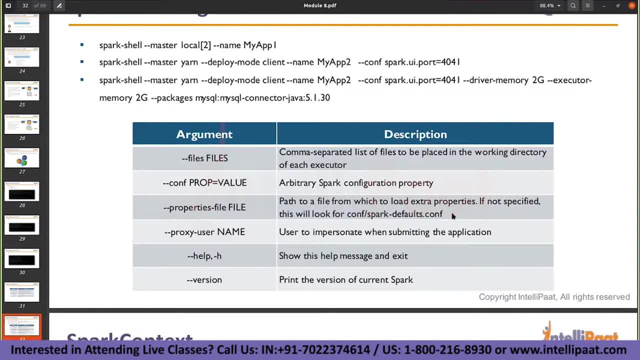 defaultsconf only if you want to update some additional properties to it, you can add this to the existing property file, or you can also create one new property file and you can launch it and the proxy name- just to give some name for your application- and hyphen. hyphen help will give you the list of commands and 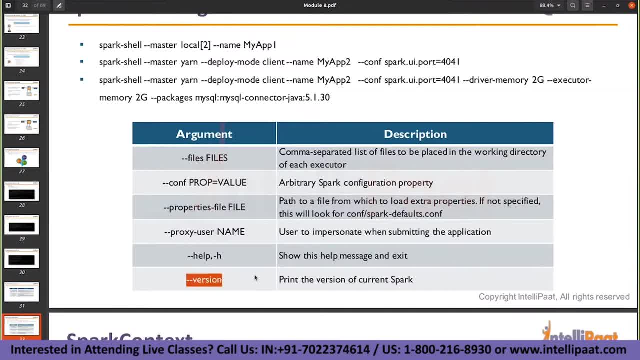 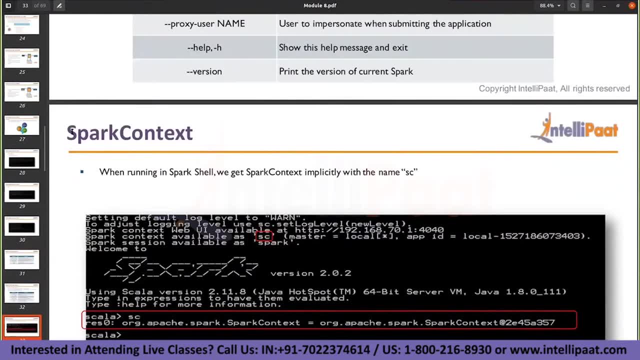 the usage for each and every command and version will give you the version of current spark application, that it is running okay, and then spark context. like i said, it's going to be the um initial step. the beginning of any spark application is going to be using a spark context, so spark context is kind of an 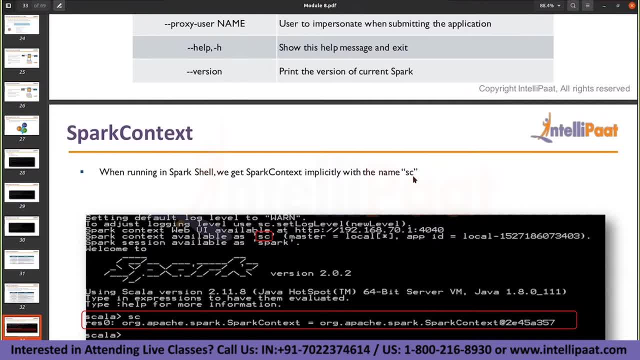 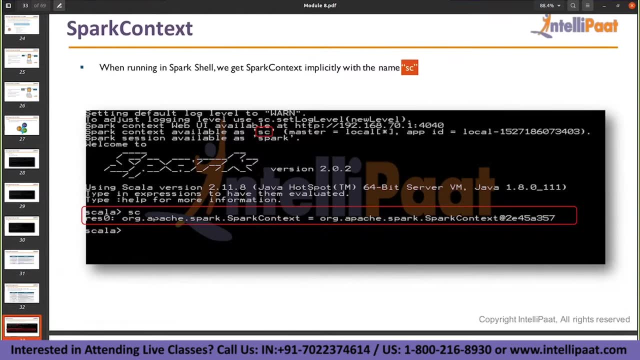 initializer to initialize a initial piece of execution to your spark application, whatever the application that you are trying to run. okay, so by default there is sc spark context that is getting created when you launch the spark shell, so you can use the existing spark context or you can also create your own spark context for a different set of applications, if you are trying. 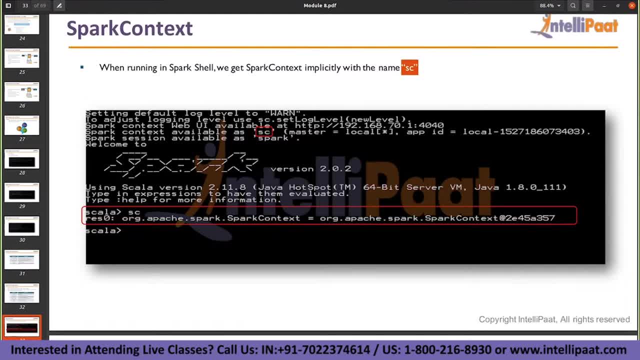 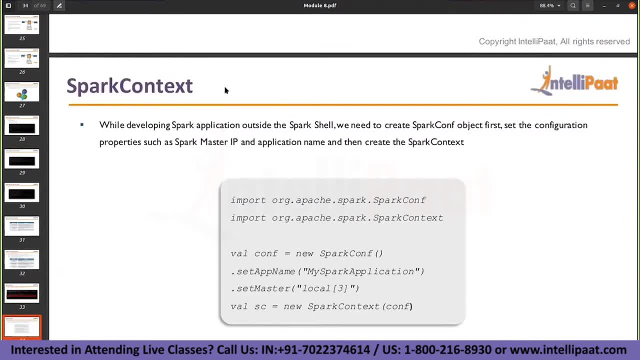 to run. okay, so by default, sc is the spark context which comes along with your spark shell. then, like you can say, you can also create a spark context, explicit spark context, by using some of the configuration properties. so here the configuration properties are: uh, the application name, app set and the master. 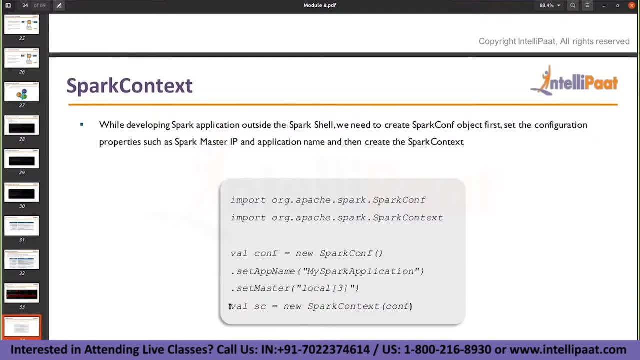 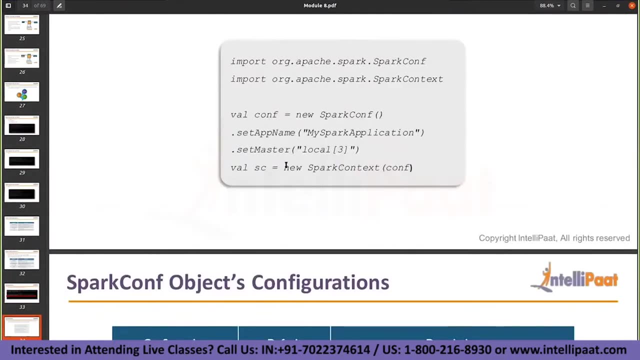 app set local uh application mode and you are creating a spark context here using this property files, using these properties, so you can define whatever the properties you wanted to. you can add all these uh additional properties here and you can create your own spark context or you can use the existing spark context which is coming along with your spark version. so this 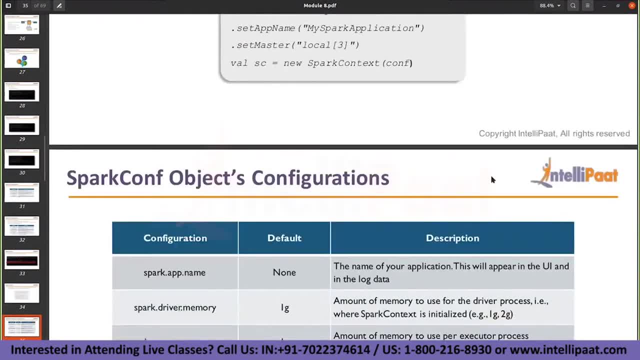 is coming from, uh, the recent versions. in the earlier versions, we used to create the spark context by default. we used to create a spark conf and then used to create a spark context. okay then, what are the parameter? what are the configurations it can take while you're creating? 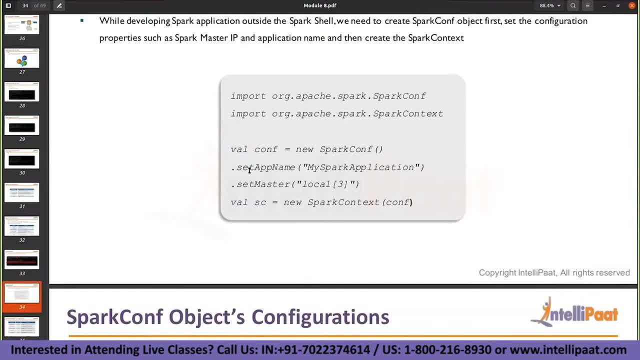 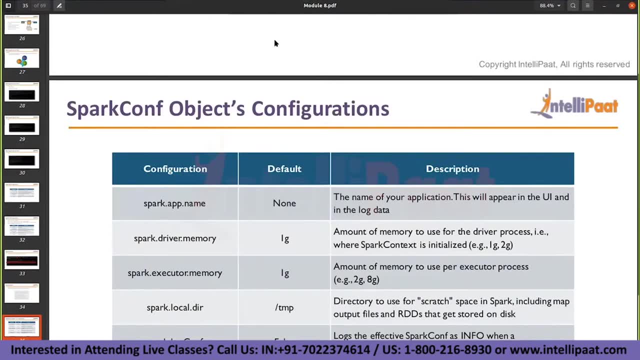 the configuration file, configuration properties, what all the parameters it can take. it's a uh uh initializer. it's a beginning step of your spark application. okay, so it's some kind of a door for your spark framework to a spark application to execute. okay so you have written a program, so where do you? 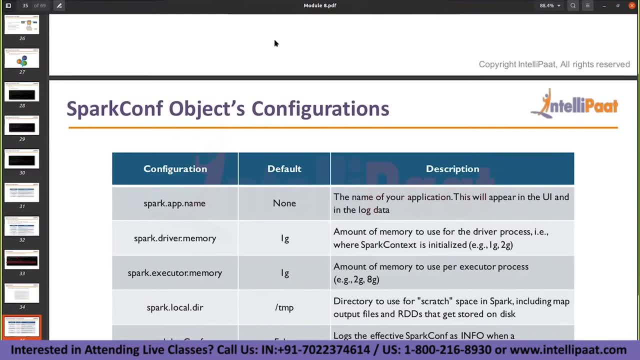 execute it. you have to execute it within the spark environment, right? so how do you execute it? with the help of spark context, you'll be you'll be allowed to run this program on top of the spark framework. okay, so it's a. it's an initialization for every program to run on your spark frame. 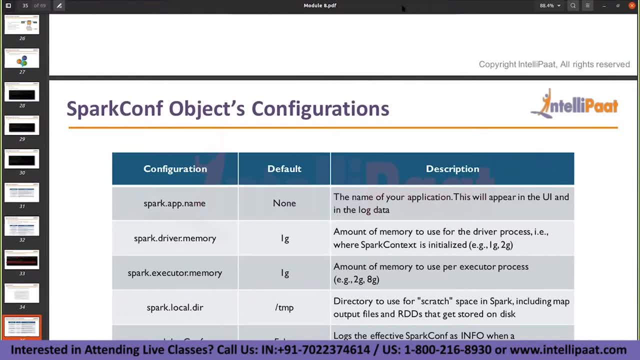 we'll create one spark context and we'll be running spark programs using that spark context only. so by default it comes with sc, so you can run whatever the applications you wanted to use in this path context. see again, there are two ways of doing it again. so if you have logged into the 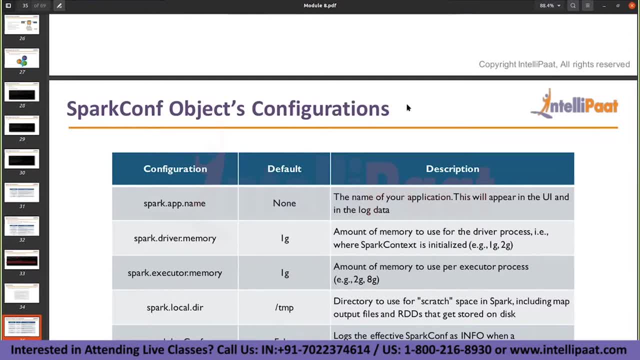 spark shell. now you're already available in this parcel, right, and you already have a spark context with the name sc. okay, so you already have a spark context. so now you can run whatever the commands. i mean you will be running sc, dot, so and so. so, as you see the command, you can run it with this splash. 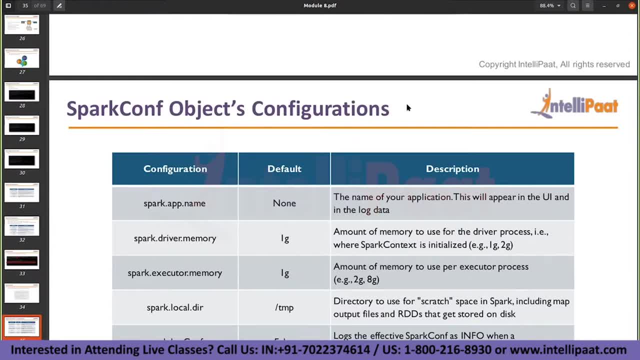 So read operations, so-and-so write operations or whatever. right, So you can run whatever you want with this SC. But when you're submitting the programs externally, that means without logging into the Spark shell. you have written a program. you have written some Python program. you have written. 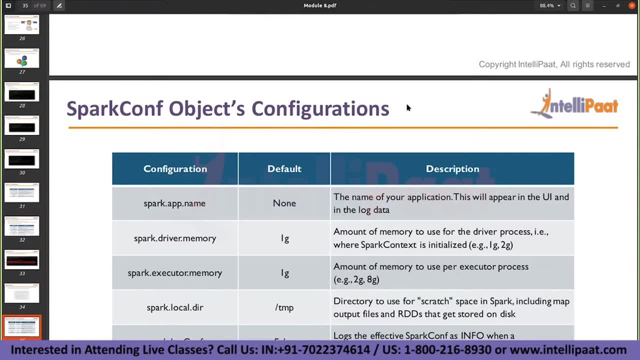 some Scala jar and you wanted to submit it explicitly. So those will be multiple. Spark contacts will be getting created for each and every application. So when I'm saying I'm creating an application, there will be multiple, there will be a Spark context getting created for this. 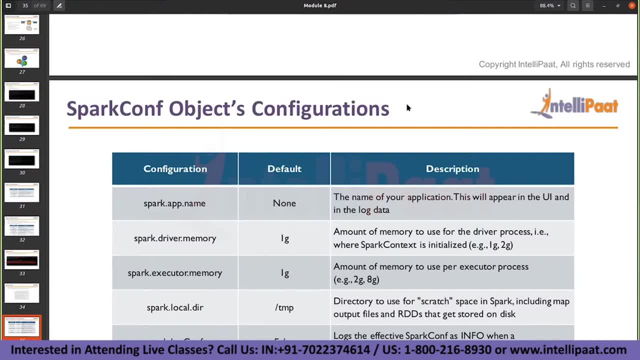 I'm submitting another application, there will be another Spark context getting created for it getting it. So, using this Spark submit, whatever the commands I'm executing is signed up an external. what I'm saying is an external way of running a program on this Spark application: Spark framework. 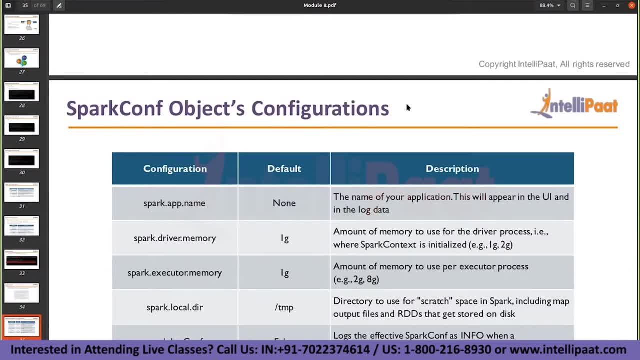 Okay. So in simple terms, let's say I'm using Spark context to establish some kind of connection to the Spark cluster. Okay, So now I have a Spark cluster available, I have a program available. Using Spark context, I'll be connecting to the Spark cluster and I'll make sure this. 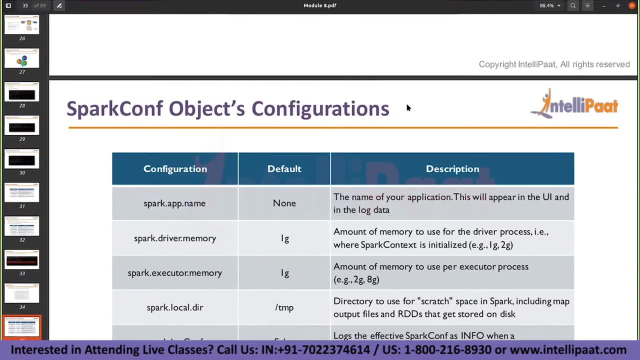 application is run on top of that Spark cluster. Getting it Spark context will help you connect to the Spark cluster and execute your applications. in simple terms, Are we clear with this now? So now I logged into a Spark shell that created a Spark context. 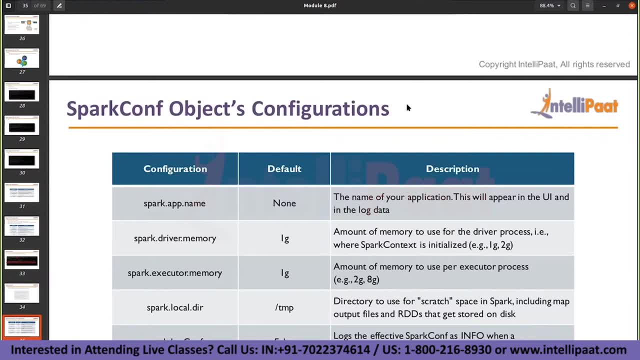 That means that created a connection for your Spark. So using that Spark connection now, I'll be running all the applications. I'll be running all different processes. Okay, So I don't have to create a Spark context now, because already a connection has been. 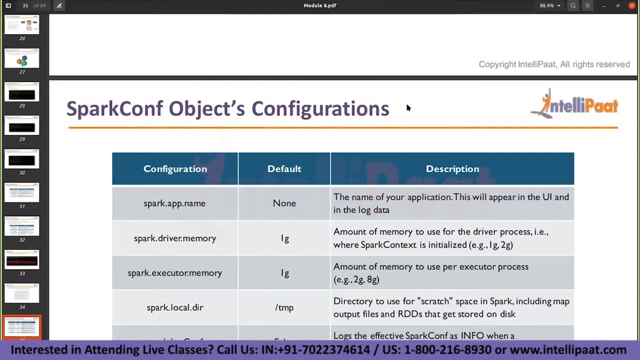 established and you're already inside. But when you're running the programs externally without logging into the Spark shell, you have to write in the program, you have to write a methodology, you have to specify some parameters. So now I wanted to establish a connection. 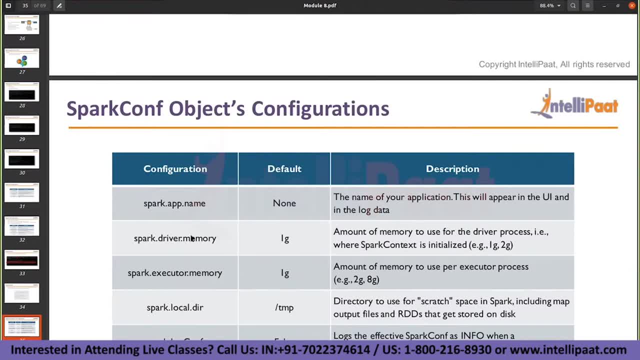 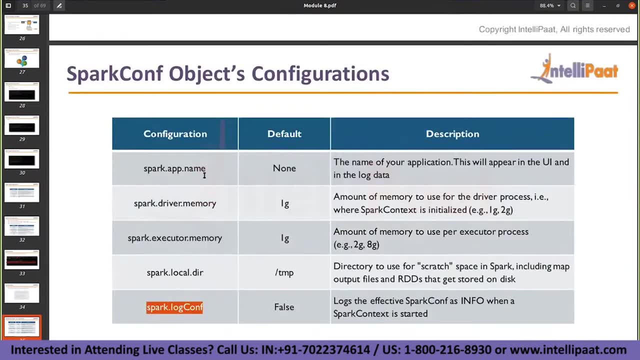 What parameters I should use. I should use all these parameters. How much memory I should allocate for this connection? How much executed memory I should allocate for this connection? What is the local directory that it has to look? What is the configuration folder that it has to look? 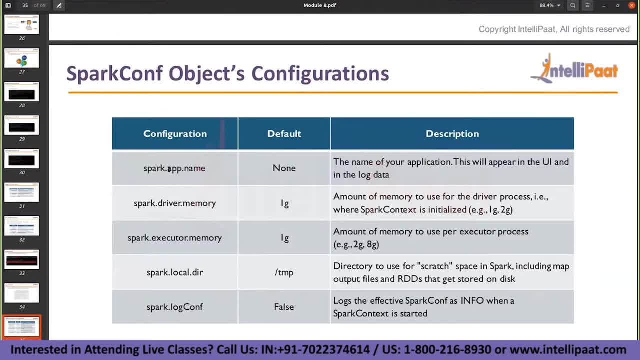 What is the name of this connection I have to give? So all these parameters I'll use. I'll call this as a configuration parameters. Using that configuration parameters I'll create a connection. I can say SC1, okay for application one. 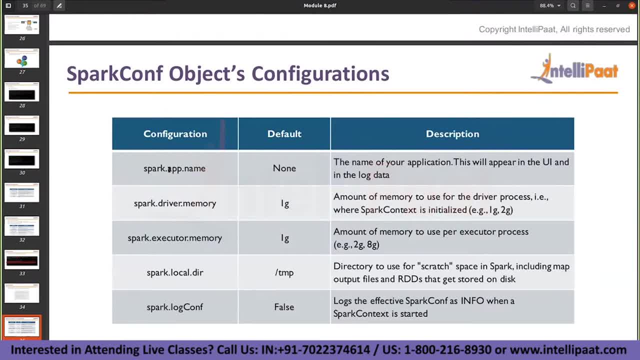 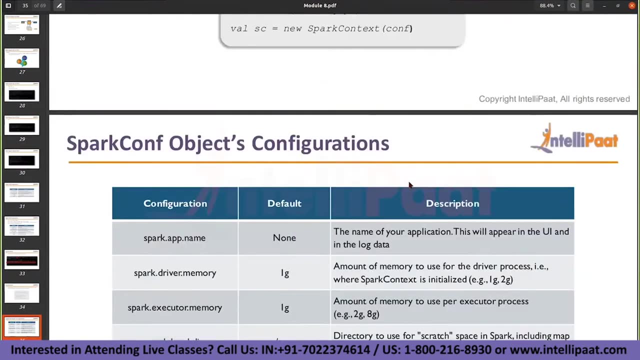 I created some SC2 for different application. I created another connection- SC3- for different applications. All this is going to hit on the same cluster, But what parameters or what configurations they are using for different connections is different. Got it Fine, So this is it. 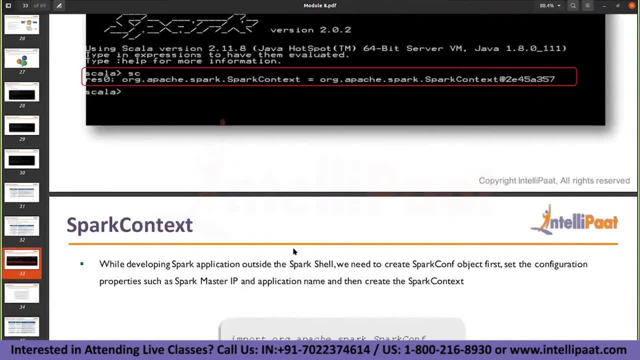 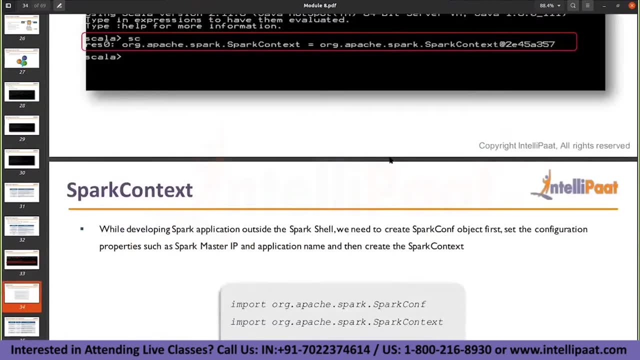 So here I'm. I'm establishing a connection, So I have already got the Spark context created with some set of parameters. This is master, is local and application ID I receive, and explicitly, how do you do it? I'll be creating your own configuration parameters and using the configuration parameters using 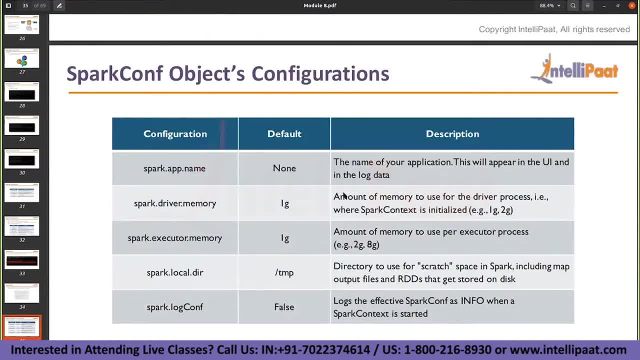 this conf. I'll be creating a Spark context Here, right? So what all configuration parameters you can give is listed in this particular this thing. whatever the sheet, okay, Application name. you can specify the driver memory, the executor memory, how much memory. 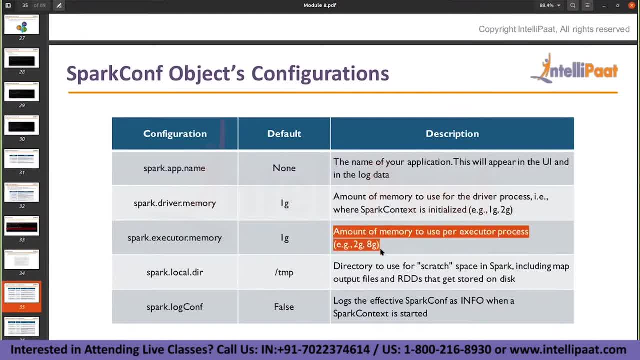 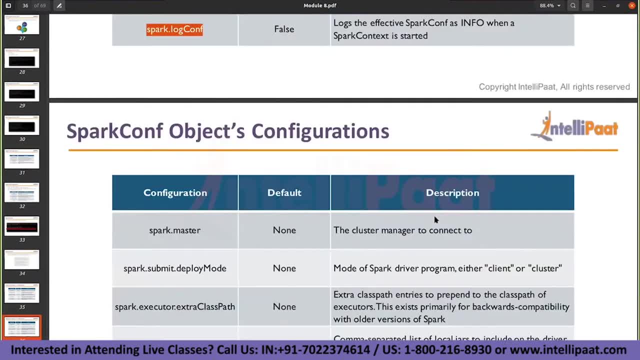 you can allocate for the driver, how much memory you can allocate for the executor, What's the difference between this driver and executor? We'll we'll discuss that in detail. And what is this local directory? What, what? what is the log directory? 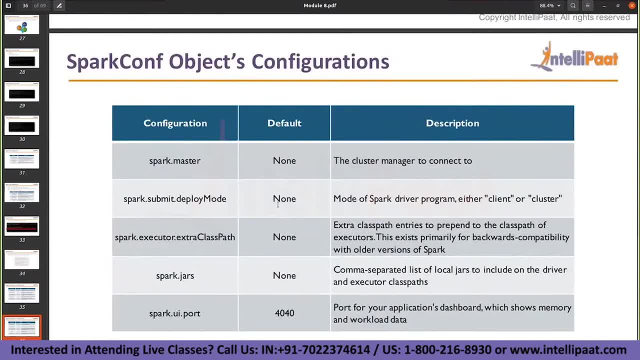 So everything you can specify, These are all optional. There is not nothing is mandatory component here, Much more So master: you can specify what master you have to specify to if you want to. for example, I want to run this particular application on Yarn system. 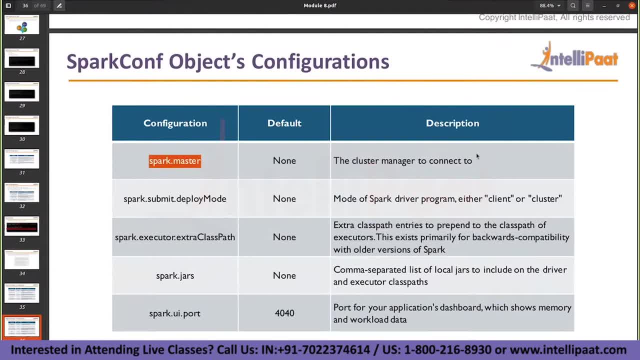 Okay, I'll create one Spark context. I'll I'll be specifying that configuration as master, as Yarn. So this particular connection, this particular application, is running on Yarn. Let's say I have another connection, I want to run it on Mesos. 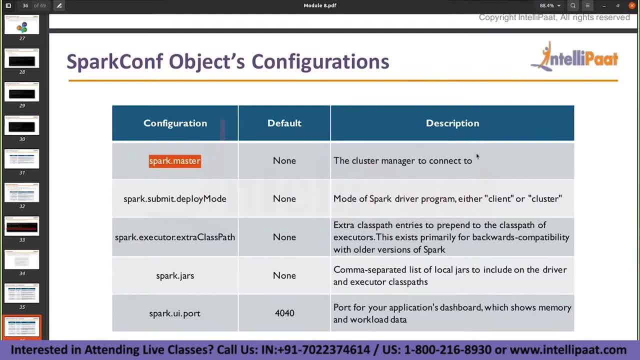 I'll give the host name, I'll give the port name. So different connections running on different different modes of execution, different, different execution modes. Okay, So deployment mode: you can specify the client or cluster. for every application, You can specify whether it wants to run it on client or a different cluster, and the class. 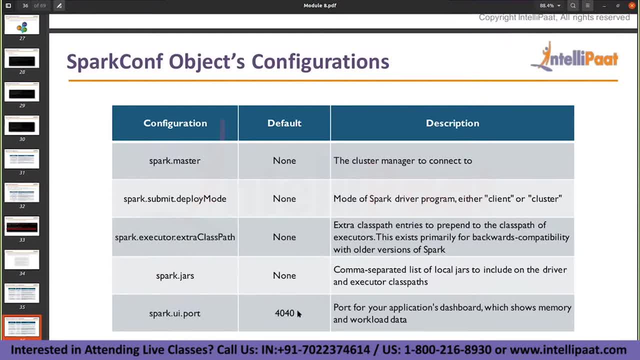 path and the jars and the UI port. So this is by default going to be 40, 40. So when you open the web UI, for every application that you are running, there will be a URL that is going to get generated. 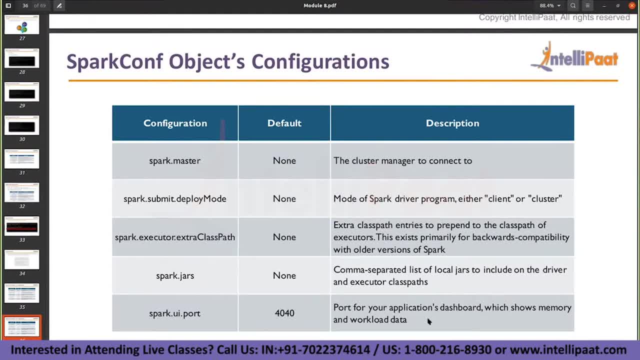 When the execution is happening, there is going to be a URL. So if you click on that URL, it will take you to the application statistics, So how the application is getting executed, What are the logs or what is the progress of the application? 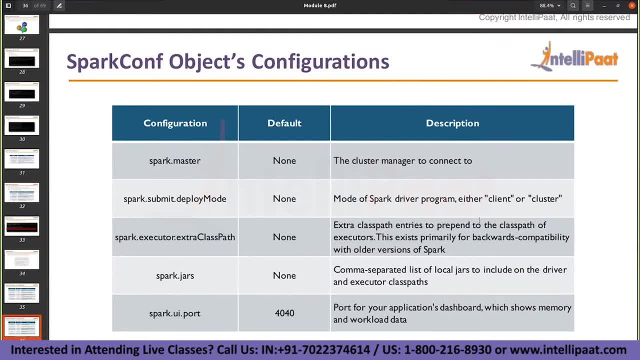 Otherwise, there is also a default URL, default web URL for your Spark that is available on 8080 or 8081. I'm not sure. So there is a conflict between these two. 8080, 8080 is the default value. 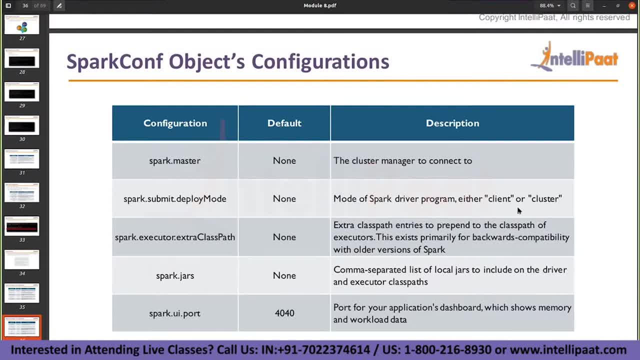 But if you already have some applications running on it, then you can specify. you can change it to 8081 or 8082, whatever. Okay, So I can also show you the default web UI. in the default web UI also, you can list out: 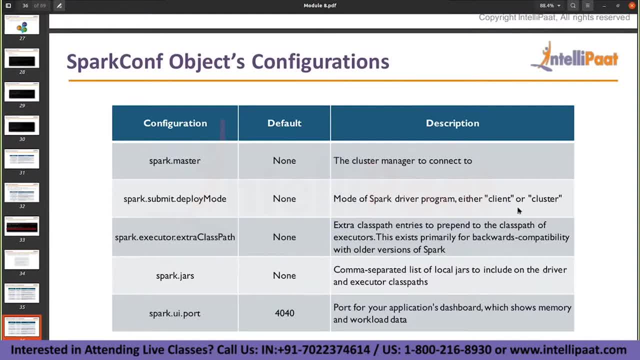 all the running applications, All the completed applications, all the failed applications. So why is it? Why is it failed? You can also check the logs and statistics of it. Okay, And and again. for each and every application, you'll also be getting a URL separately. 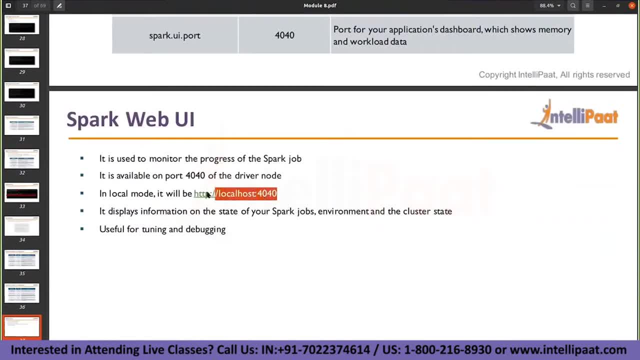 Okay, Right, So web UI 40,, 40,. uh, this is 8080, actually, I mean, whatever the configuration in 3.1.2,, whichever we are using is 8080.. And there were some problems with this 8080 port. 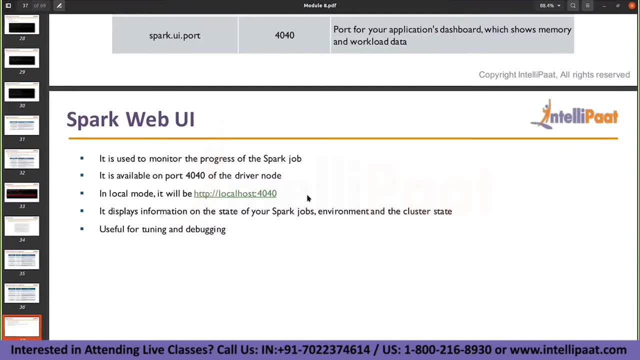 I mean 40,. 40 is maybe. Yeah, This is the older uh URL. So in in 8080, there might be some problems because there are many applications which use the same port number. Okay, So if your local machine is already uh running some other application on 8080 port, then 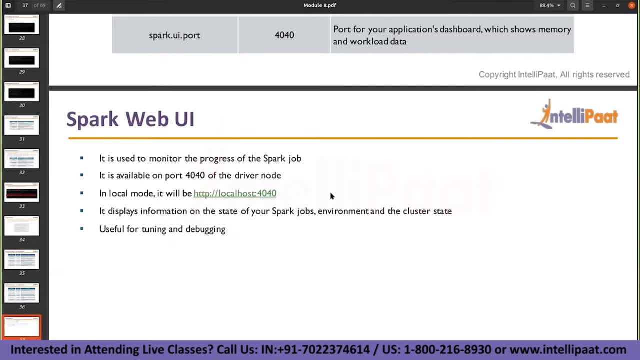 it's going to throw an error. You have to get into this configuration folder and you have to make the changes. You have to change it to some other port name- 8081 or 8082, whatever. Okay, So this is how your UI will be shown. 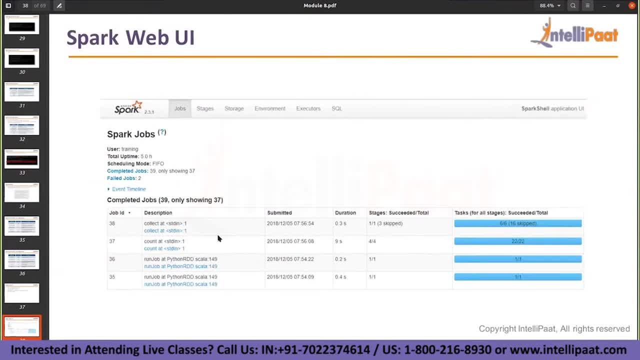 All the completed jobs, All the failed jobs and all the uh statistics when it is submitted, what is the time it has taken, how many steps it has, and you can see all the uh information in the Spark web UI. 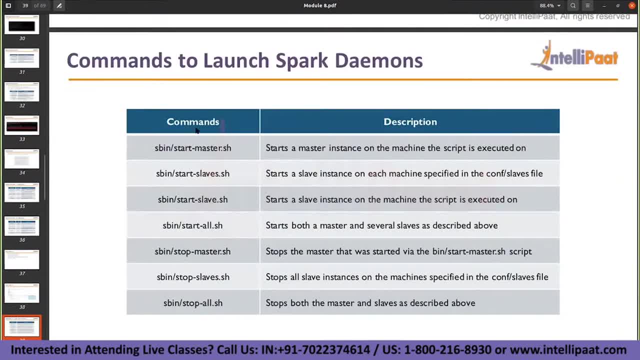 Okay, Is that fine? Uh, I can, yeah, So commands to launch Spark daemons. there are multiple daemons. the master there slave is there and you can start them by running this startallsh. Right, So using startallsh. 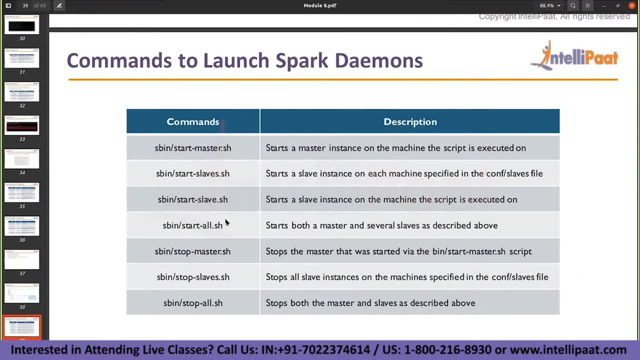 Your Spark cluster will start And then you can uh navigate to the web UI and you can see the um uh UI page. Okay, So there will be no applications that are submitted. Zero, Everything is zero. You can just go through what are the list of completed and successful applications. 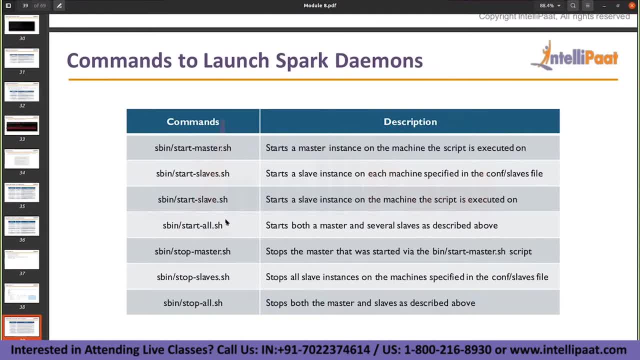 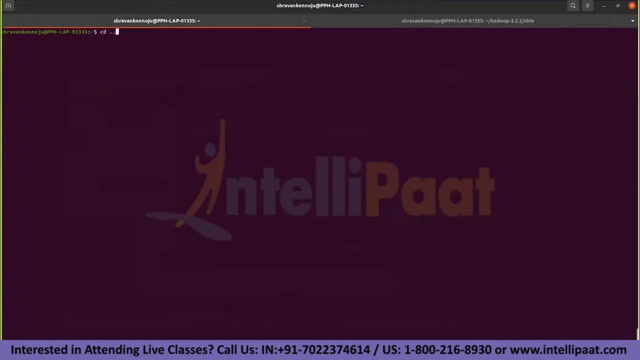 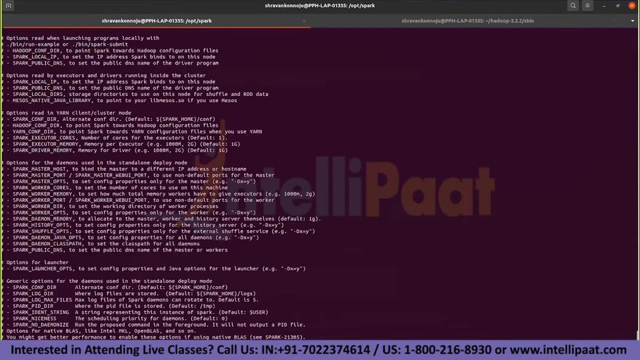 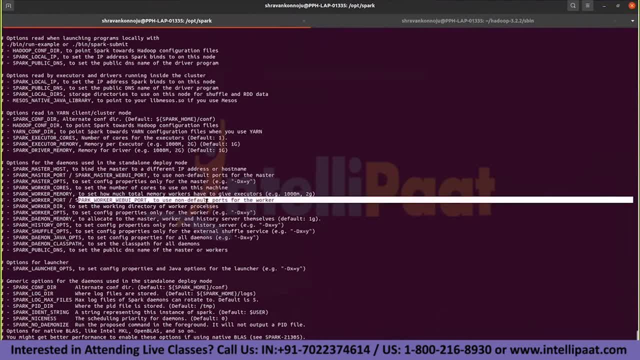 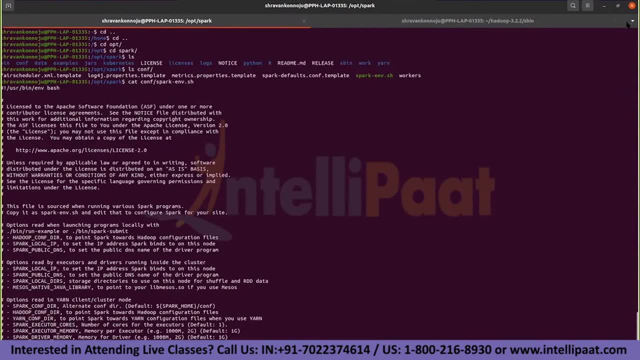 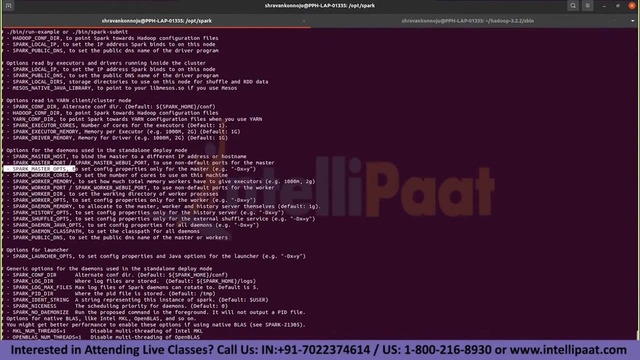 I've just bought my master webus port here. I have to make the changes to this file to be able to point to a different directory. Let's see I'm navigating to sm. I'm navigating to a spin, unless and start. Okay. 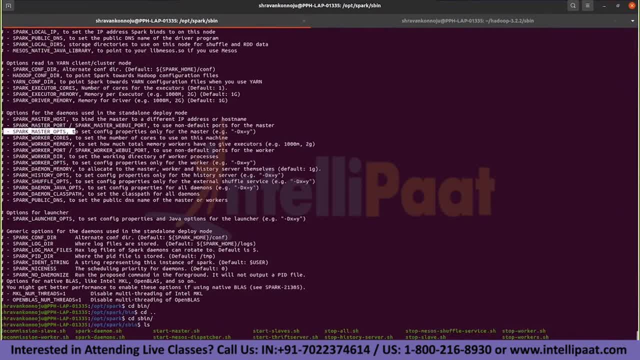 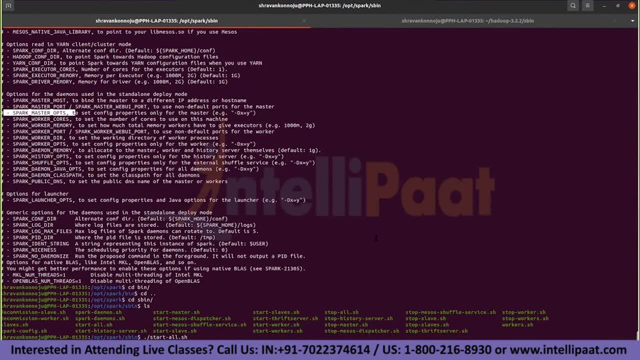 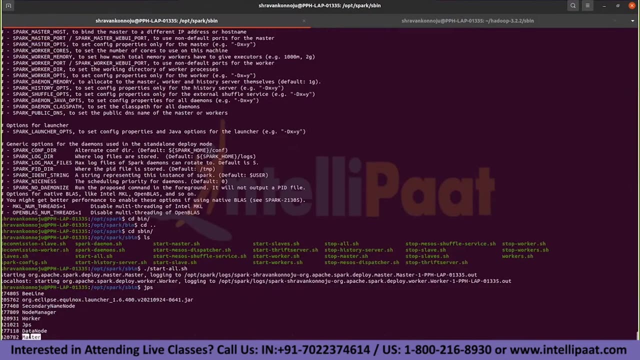 Okay, Thank you, Thank you, Thank you all. dot sh. this will start the master as well as the worker nodes. okay, so do a jps will list you the spark master as well as the spark worker. so after you do this start all you may navigate to. 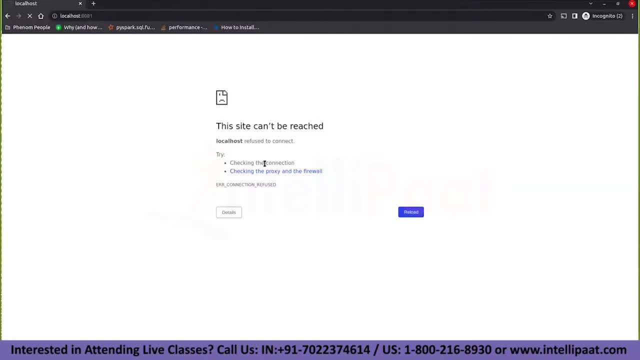 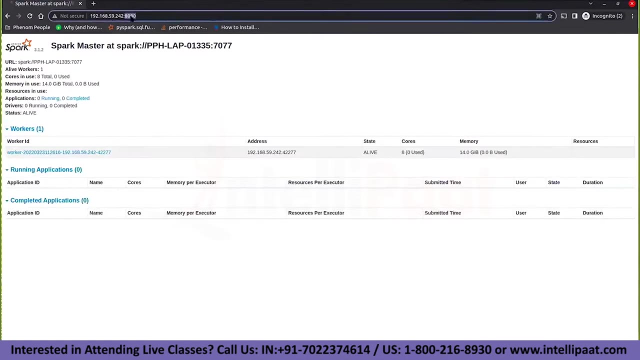 a browser- i'm sharing my screen, so just refresh this page- and 8081 is a port that i allocated and it is running on this particular node. okay, so the running executors: you can just navigate to the master. this is running on 8080 port. this is your spark, master ip, and the number of workers is the. 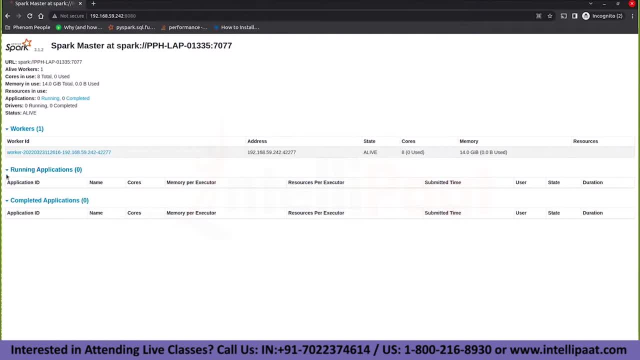 same again, the same machine is being allocated as a worker and running applications and completed applications. so this is how you, your master web ui or the worker web ui will be understood, will be shown. so for you to just check what parameters i have updated, what parameters i have made changes to, 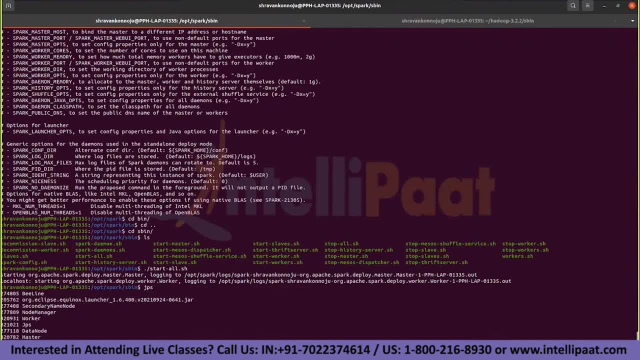 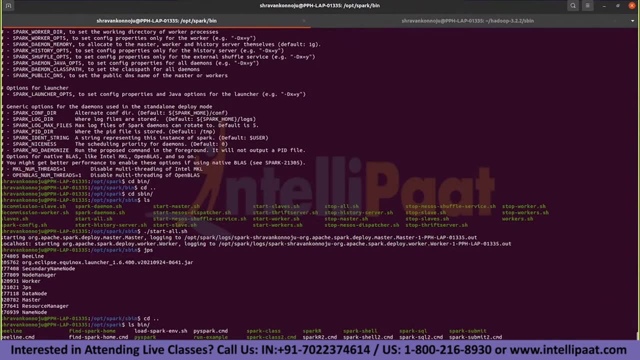 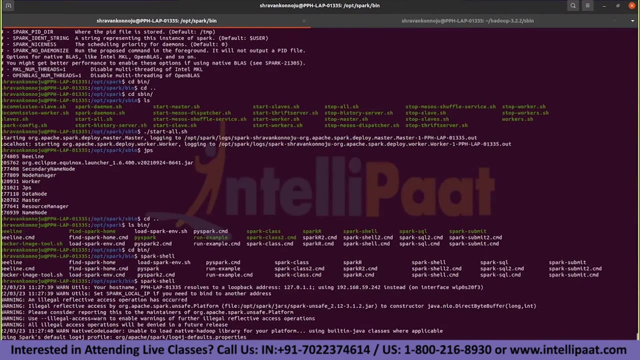 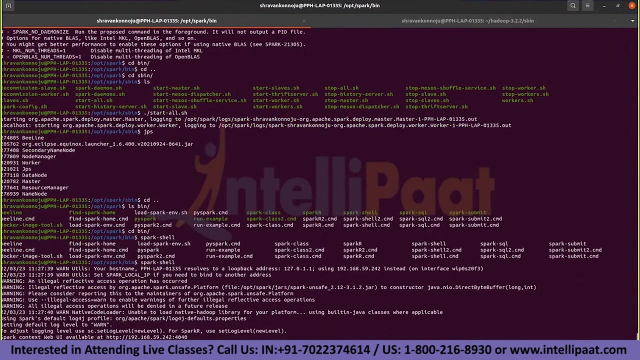 so cd, cd, um, okay, so cd bin spark shell. we'll launch your spark shell with the scala version. so, guys, i even i'm using a different version of spark here, so my spark shell will be running on this particular node. so my spark version is three point, two point. one second- let me check- it is um three point. 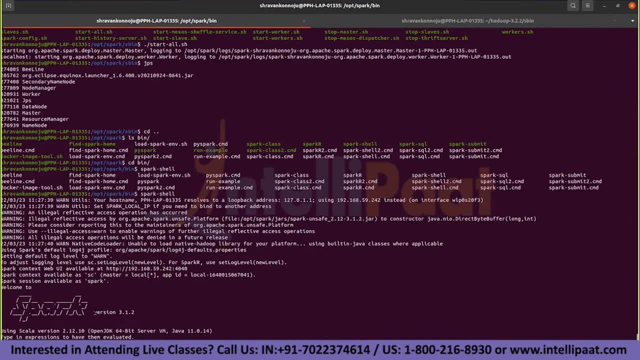 uh, what is that? yeah, spark is 3.1.2 and scala is 2.1.1, but hadoop is, uh, built on 2.7 only. okay, so even then i was able to load, because my latest hadoop version is around 3.1.2. okay so, 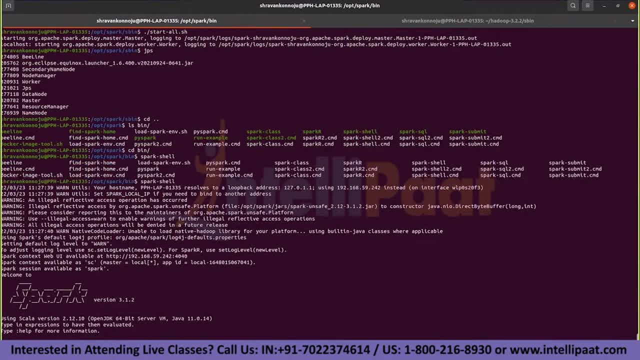 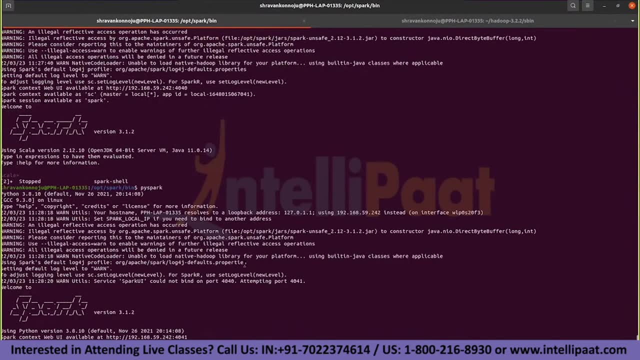 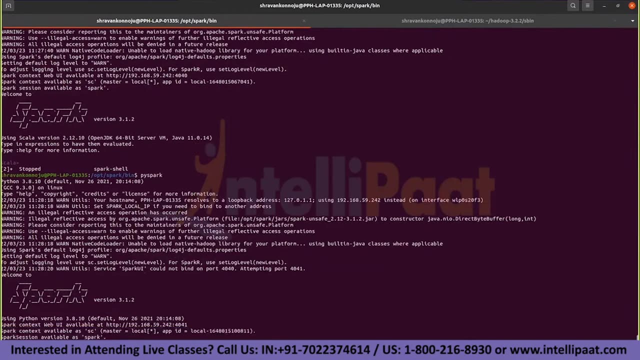 i was able to load. i didn't have any problems with it because i have done spark installation first and then on top of it i've installed hadoop. both are both are independent. there is no uh interlink between those spark as well as hadoop, so both are working for n5 spark as well as spark shell. 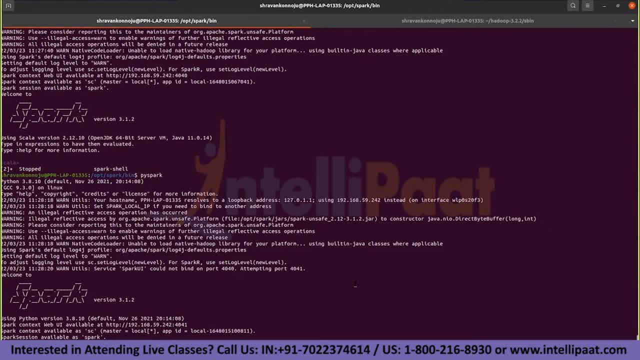 i would request you to downgrade or upgrade the hadoop spark version. or else- if i mean, as we don't to do with Hadoop- you can just remove all the parameters or values that are set for Hadoop, remove the entire directory itself and just change the Hadoop home. you can even remove 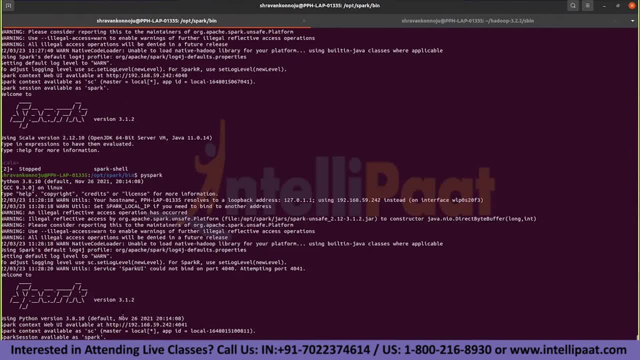 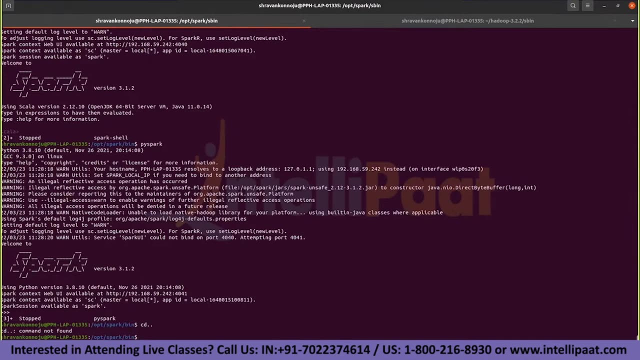 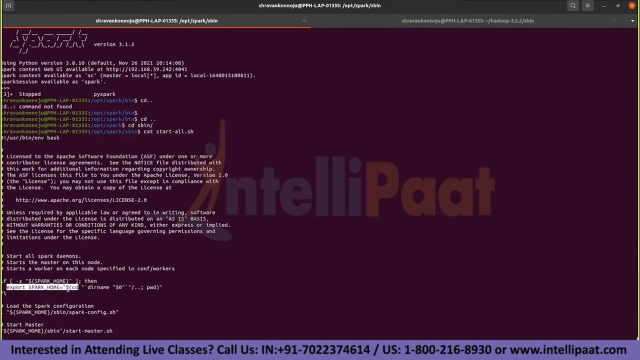 the Hadoop home. that is not not required at all. so if you look at um cd spin, so if you look at cat start call, there is no parameter required for Hadoop home. so the only parameter that it's taking is spark home, right? so it's not required at all Hadoop home. so i would suggest you to do this better, okay. 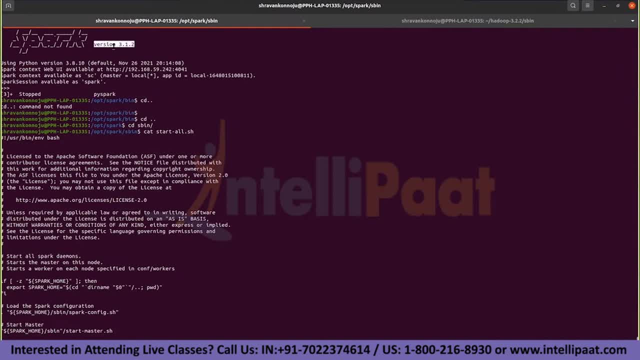 so um, the spark 1.3.1.2 version and we have downloaded the 2.7 Hadoop related tar file. so that's fine, let's beat with it and you just remove the entire Hadoop setup. remove the Hadoop setup and remove the Hadoop home from the environment variables. 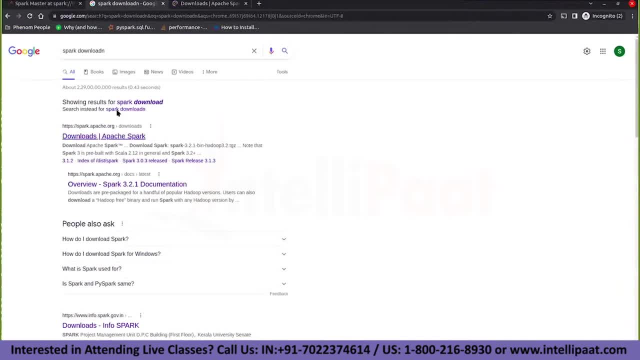 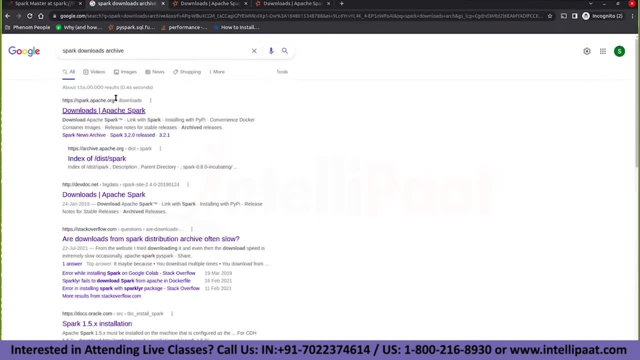 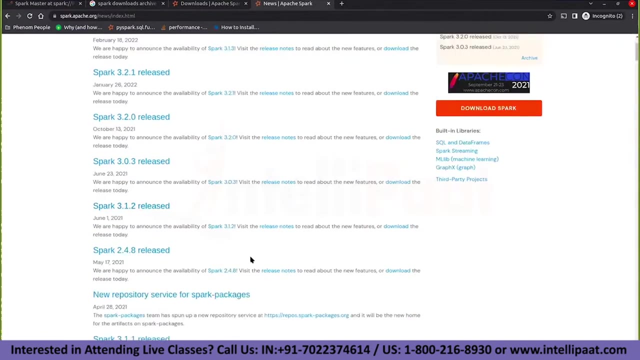 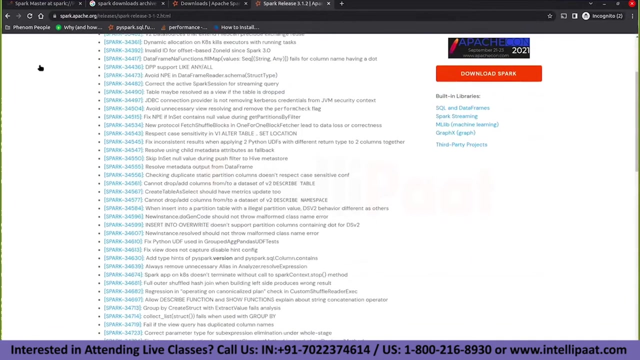 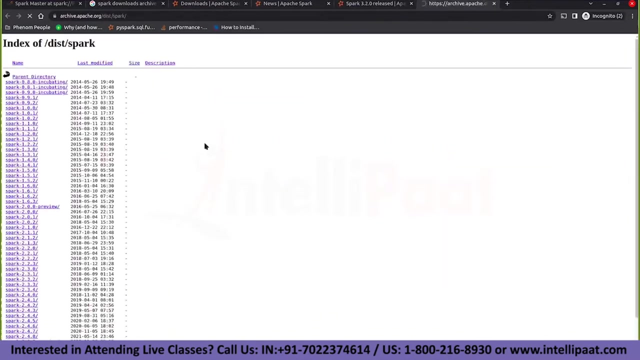 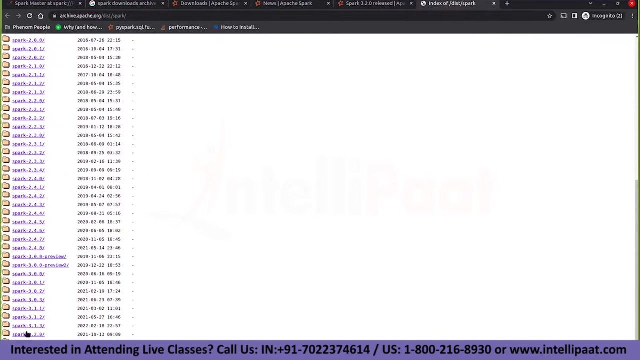 is that fine? so here on the downloads, maybe you can get into the archives. this will give you all the other pages also. so 3.1.2 is what i'm using. just navigate to 3.1.2, this page, this one, mark this here. yeah, so here from dist spark, i'm navigating to 3.1.2. right, so 3.1.2 and 3.1.2 built. 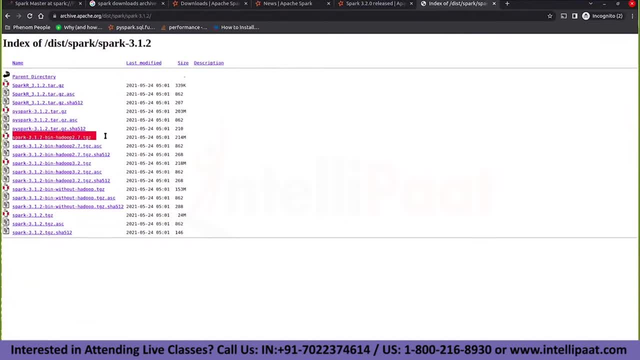 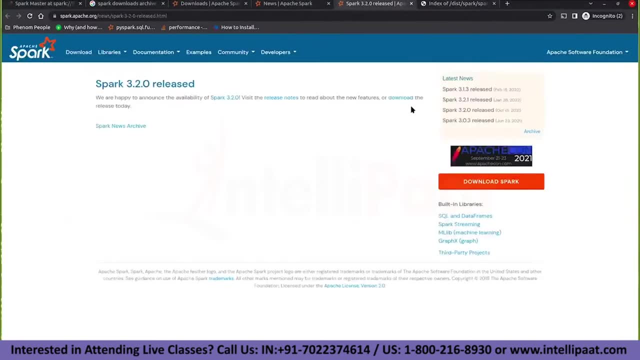 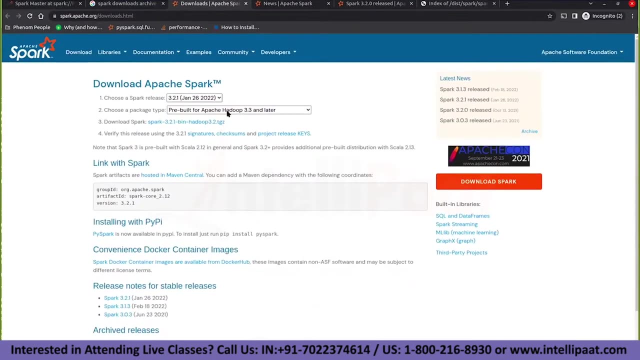 on top of Hadoop 2.7, point this one. so try downloading this file. this is the file which i have used for my setup and the venue tails. where do we get the venue tails? so okay, this is 2.1.1 for 2.7. okay, so fine, um. 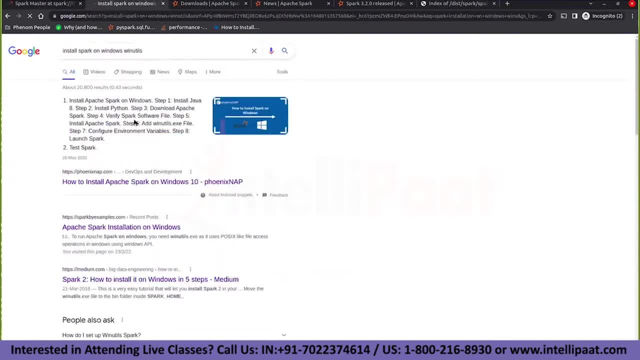 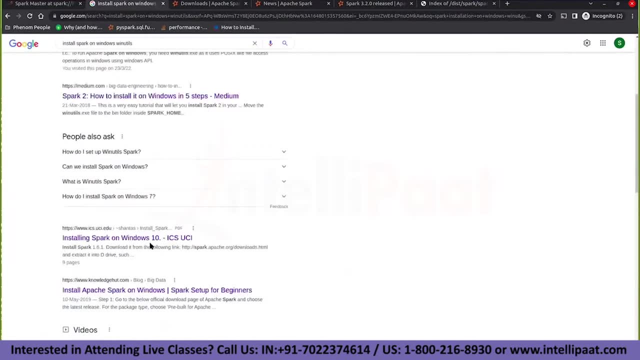 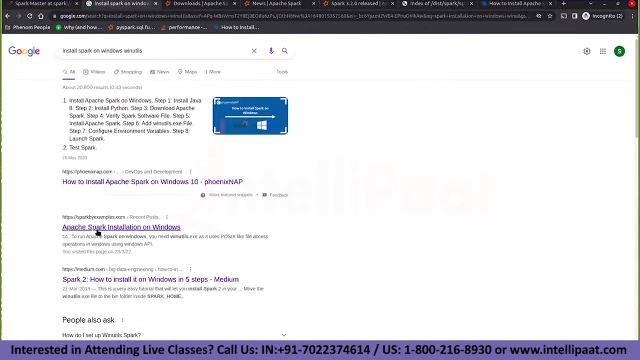 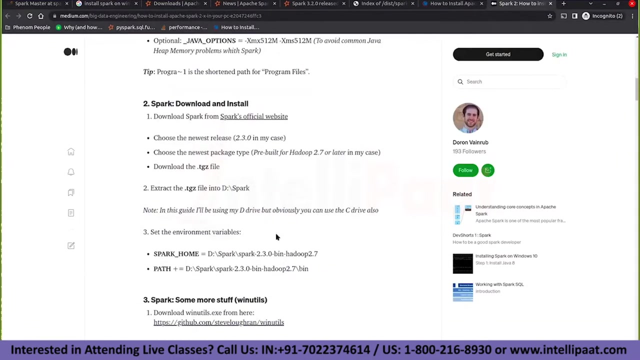 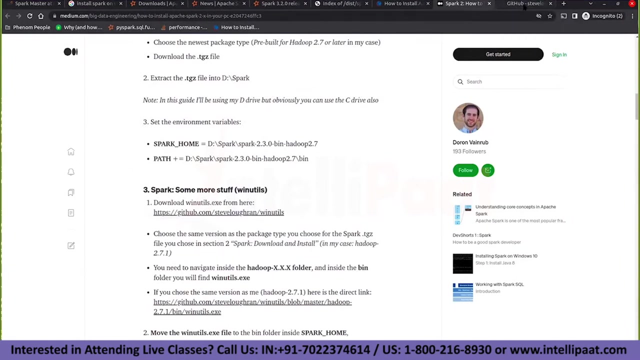 those, not this, not this. there should be a GitHub repository. fine, i can get it from here also, so just scroll down. this is a page that we have used right. let me take another one. so scroll down and you will find that video directory path here. so, as you can see, these are not verified github repository page, so there is. 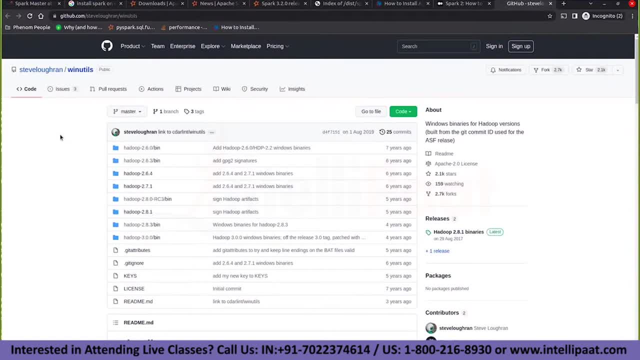 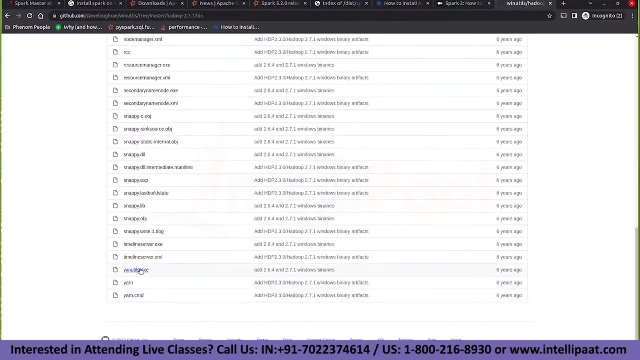 someone named steve. let's see how many downloads have been done. there are 2.1 stars, so it's not a verified thing, but we can. we can still use it, that's okay. so this is a winutils file. so do you have this path? you have to download this file from here. okay, so this is one path and there is one. 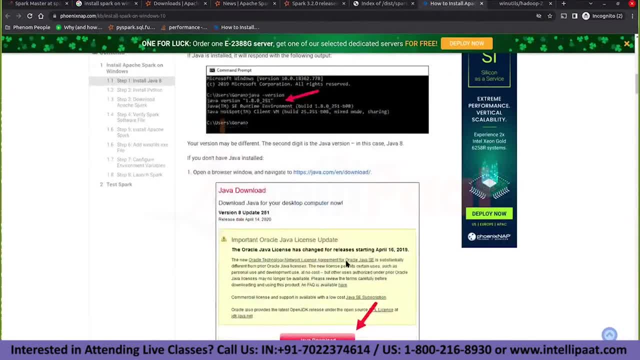 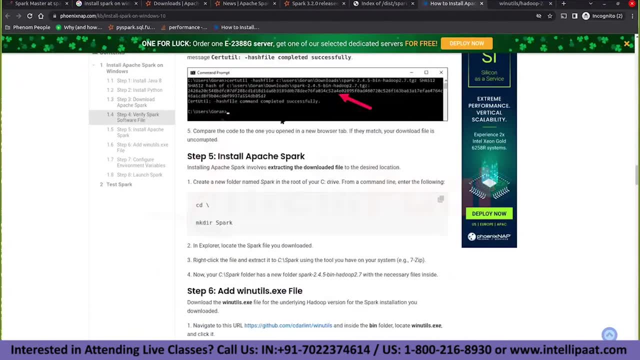 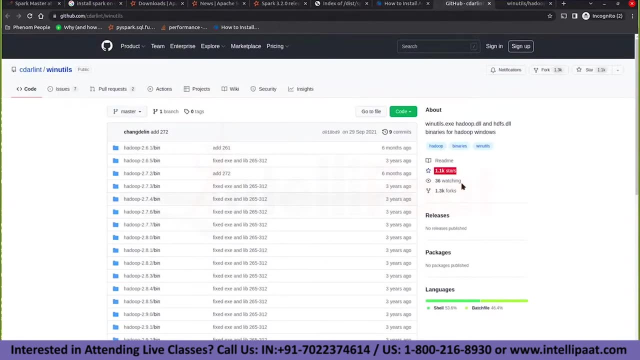 more. let's see what is the other guy telling. scroll down, winutils. where is it? this is done. this is done here, so you can see there is another guy. this is a cedar link, right? only 1.136 watching 1.3k folks, so here.